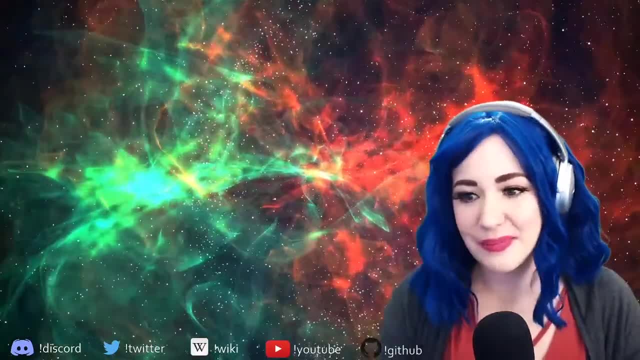 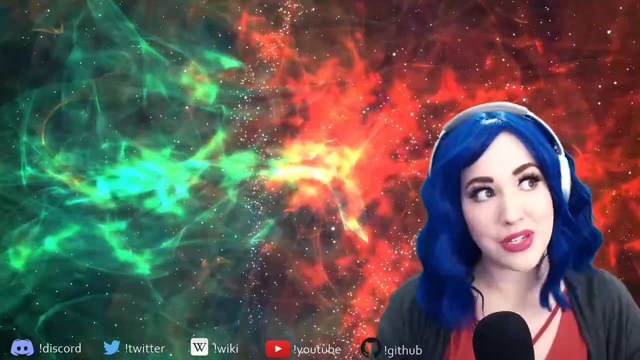 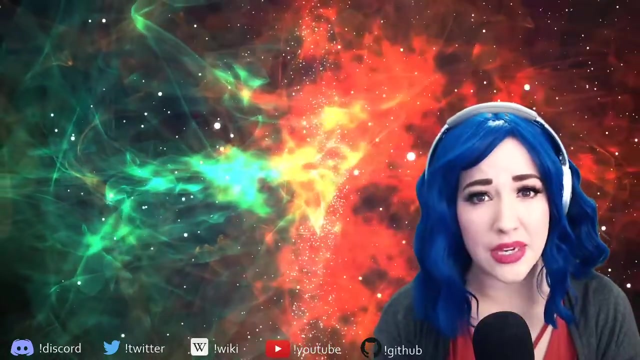 Hi everyone and happy Science Sunday. I'm excited to to do more fundamentals of data science tonight and in particular we're going to be talking about machine learning. So for those of you who did the 12 days of machine learning myths, a little bit of this will be a review. 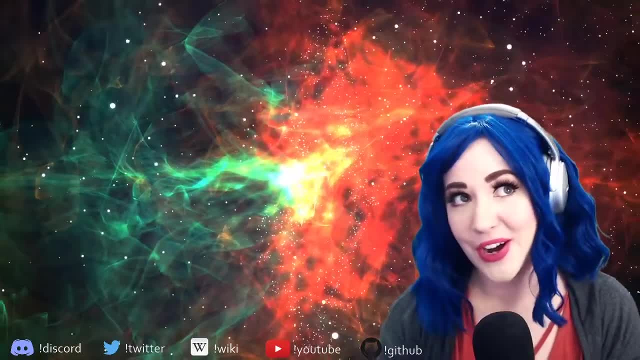 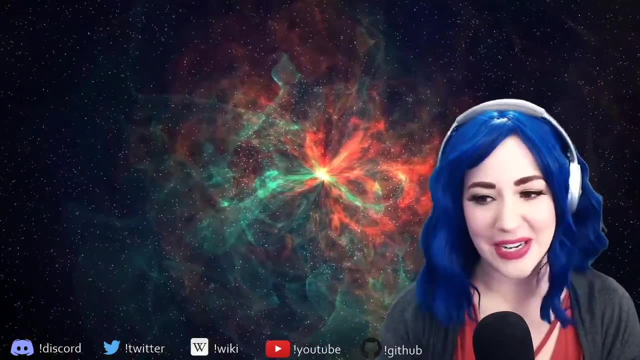 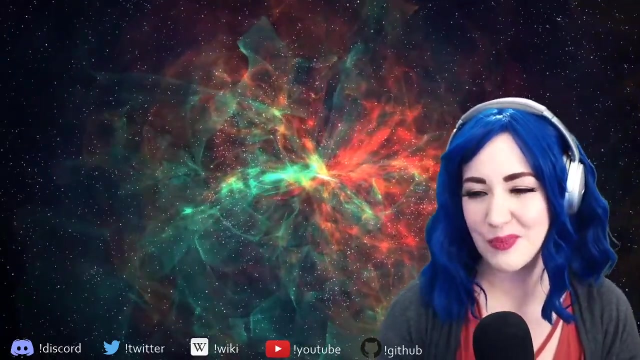 but we're still going to be doing something new. so hopefully, no matter if you were with me for 12 days of machining machine learning myths or not, you should get something fun out of tonight. But hello in chat to loafbone, as always, and to potion. I always want to say potion, but it's like. 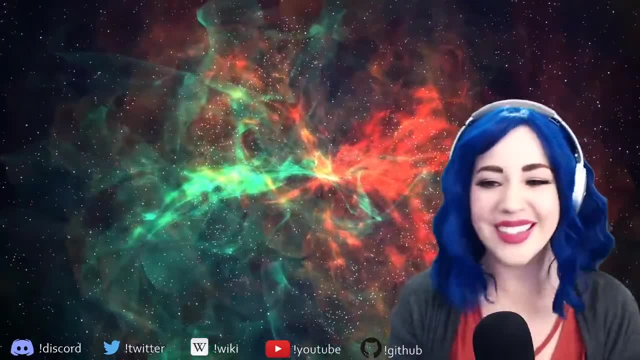 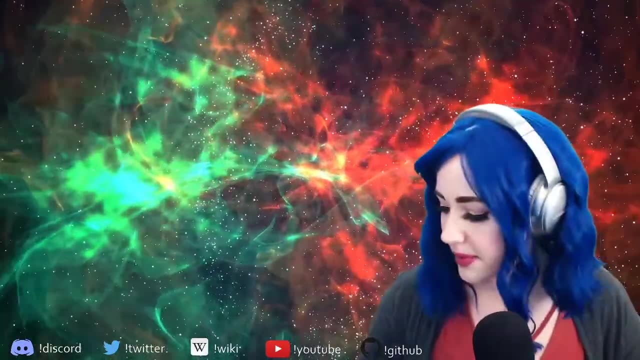 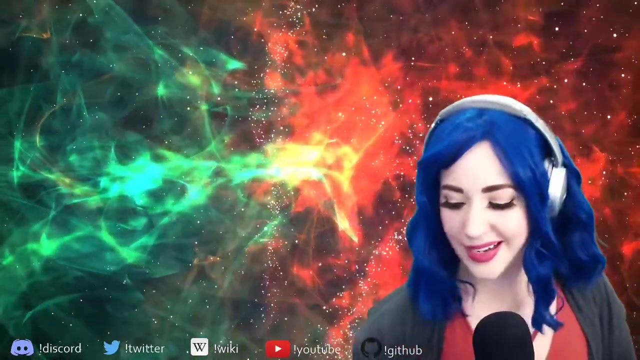 you've got an extra i in there, so it's like po-ition Welcome, welcome, hello. I'm just getting a few last things here set up, Got my stylus, so you know it's gonna be a fun night Getting the, getting the tablet all set up. Exegidicris, have I decided to do a? 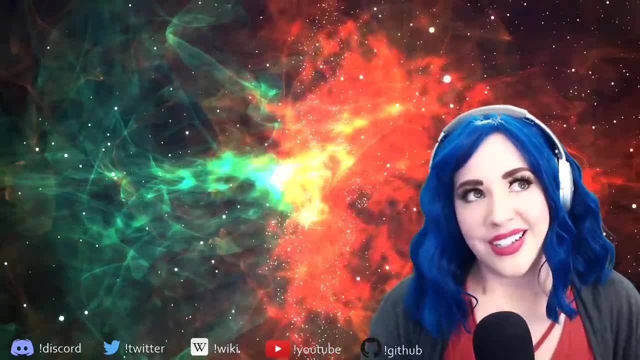 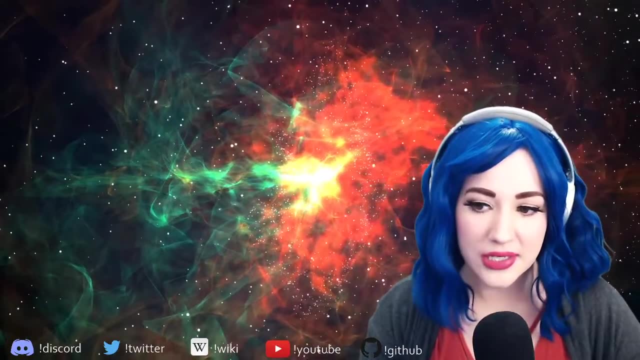 trial of machine learning. I'm not sure if I'm going to be able to do a trial of machine learning or not. How's the transformer stream? Oh, I would love to. I've gotten, I think, more requests right now for more introductory level machine learning stuff, so I would. I would love to do that actually. 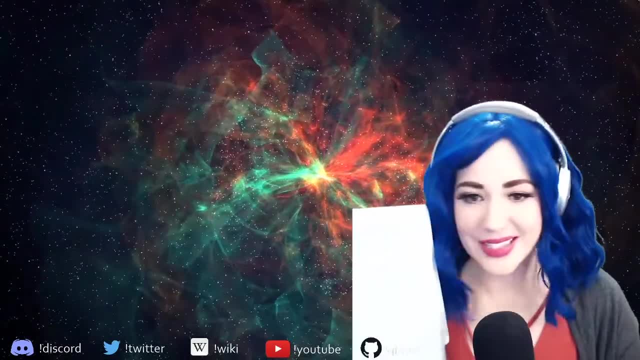 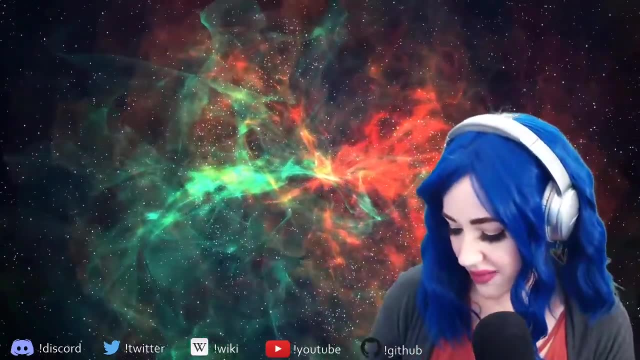 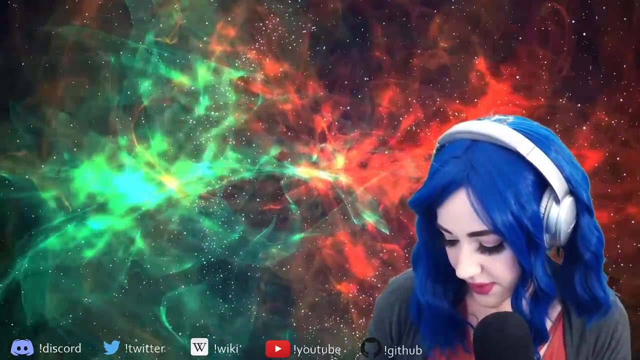 Let me grab my, my trusty legal pad that I don't go anywhere without that. I should probably actually switch to like a notebook or something. but yeah, who cares? All right, so stream ideas. I gotta write that one one down- transformers, because also there would be so many pun opportunities. I 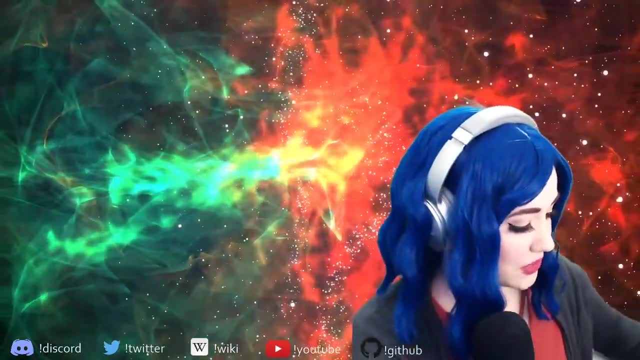 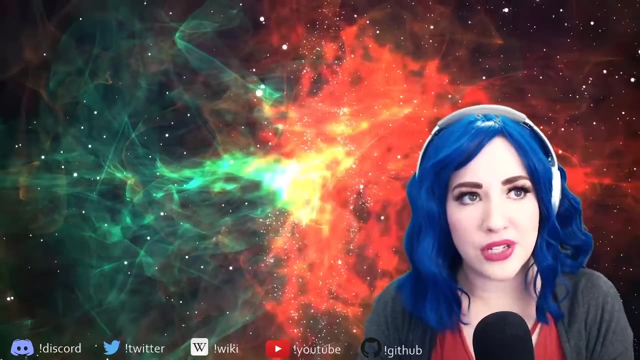 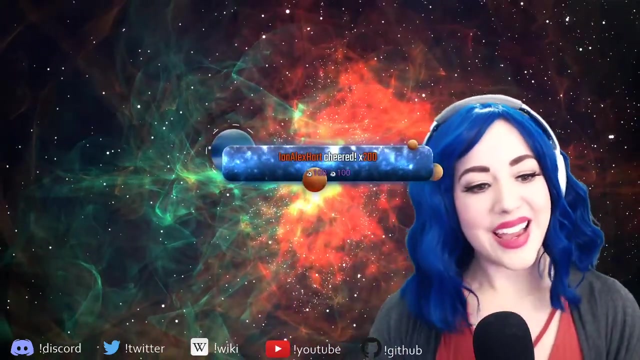 feel like that'd be, that'd be really, really cool. but no, we're not gonna be doing transformers tonight. I've had a bunch of people interested more in in machine learning basics, and so what I thought we could do today is we're gonna be talking about classification. I'm going to- and, oh my goodness, Ian Alex. 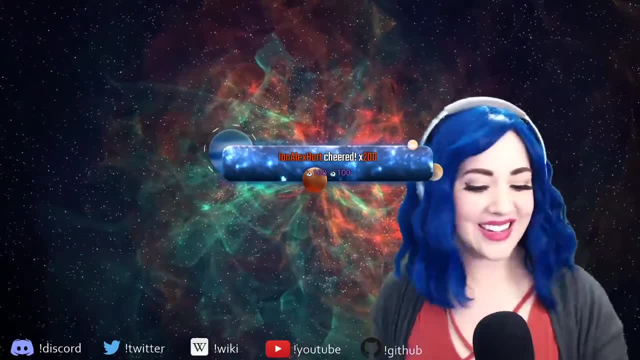 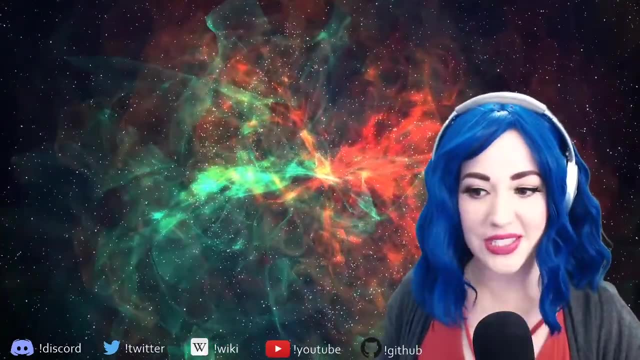 Hart with two 200 bits and that that is two dog treats. so I've got my little dog treat counter here- two dog treats, so I will. we'll see how we can make that work. I might have to like be right back and like set everything up, because I'm 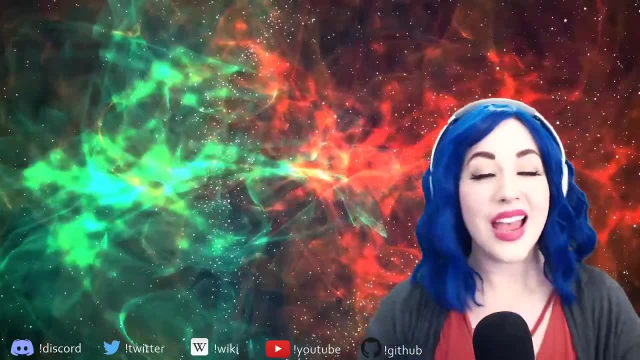 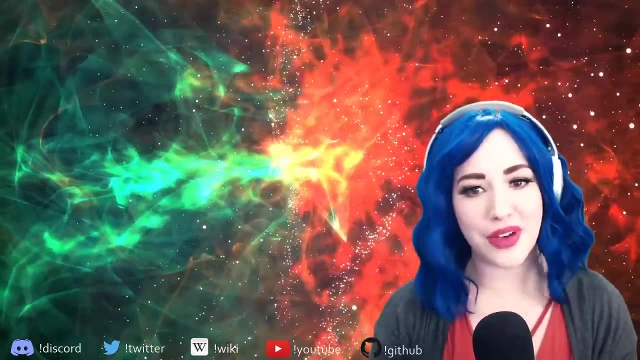 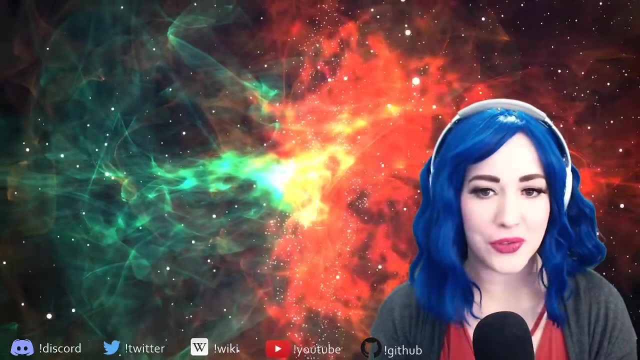 without my trusty assistant today. in any case, hi, welcome Ian, Alex, and hi strawberry Jesus, um, so yeah, so here's. here's what I've got planned for today. we're gonna, um, we're gonna review what machine learning is for folks who just want to get started, who 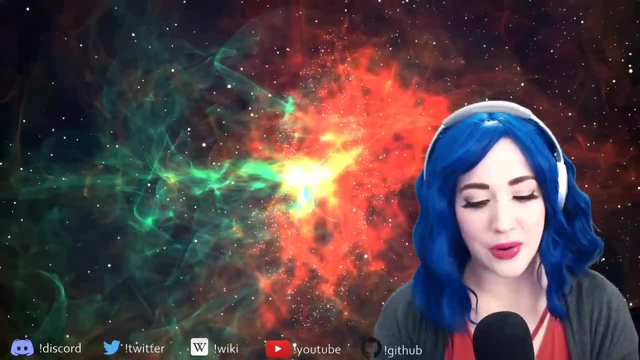 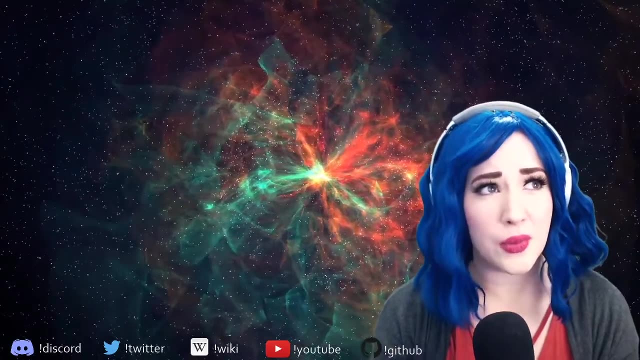 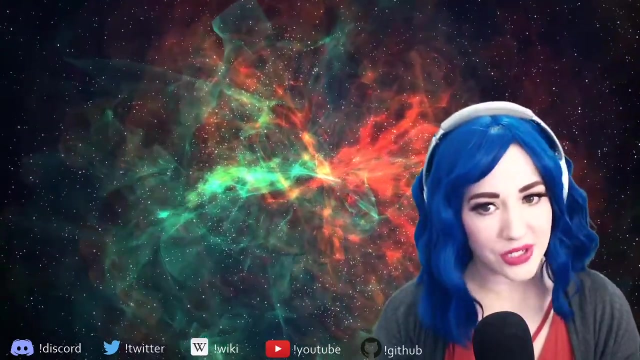 are new, have never done machine learning before. I want to do a little bit of an overview of what machine learning is, the different kinds of machine learning similar to. I think the intro to machine learning must day one, and then we are going to review decision trees and random forests. now that's something that 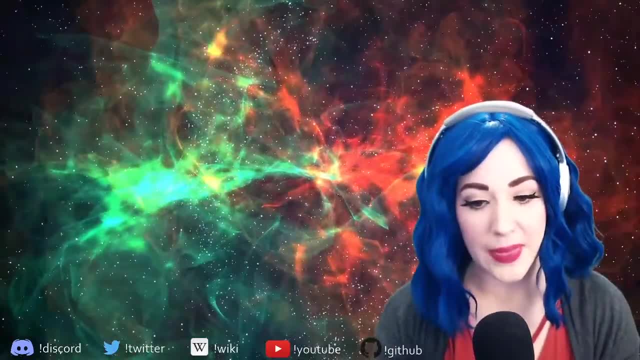 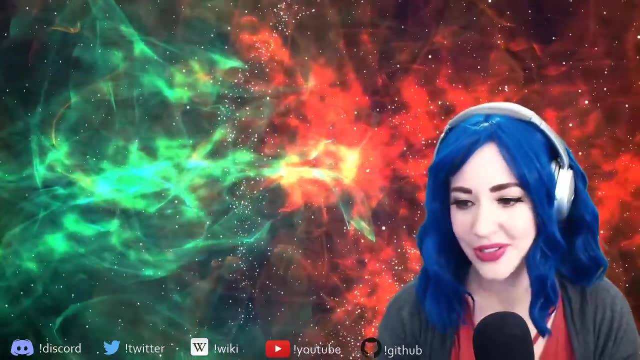 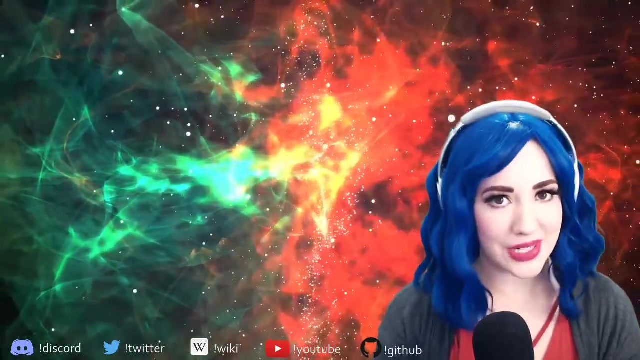 I have a like deep dive video on, so if you're interested in that, check out day five of machine learning myths, which is all about ensemble models, but I'm gonna review it a little quicker than I did in that video. and then we're gonna talk about gradient boosting, and so this is something I touched on at the very 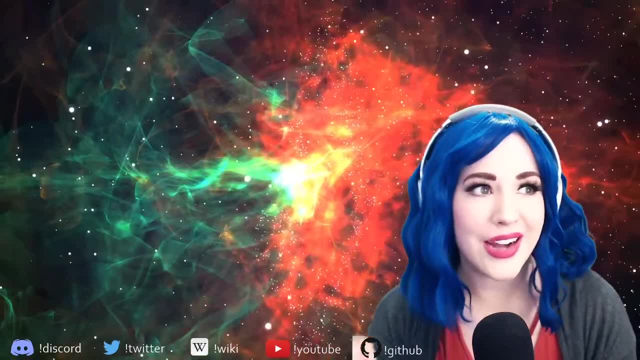 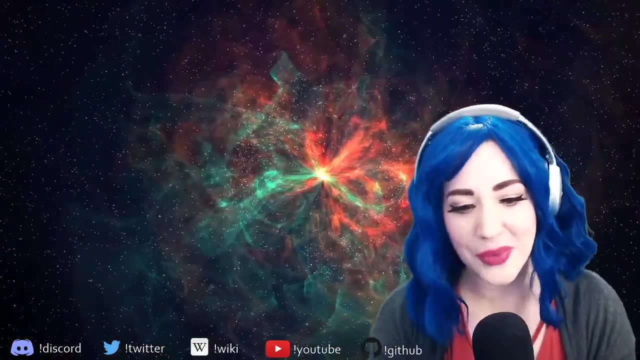 end of video five. and I kind of just like dangled it a little bit, like oh, isn't this cool, like this is something else you can do with trees, but I figured we didn't have time to to build it and so today we can build it and look at. 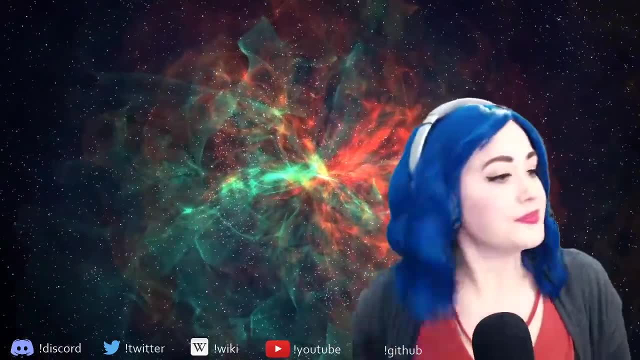 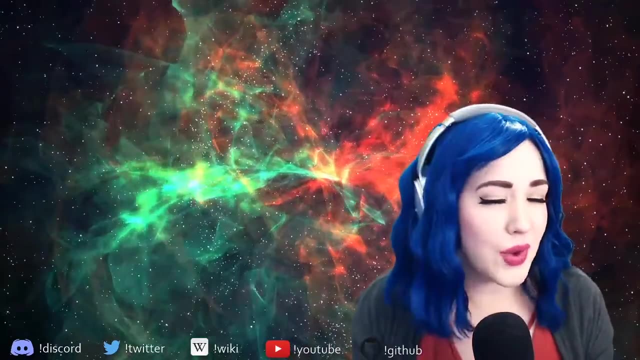 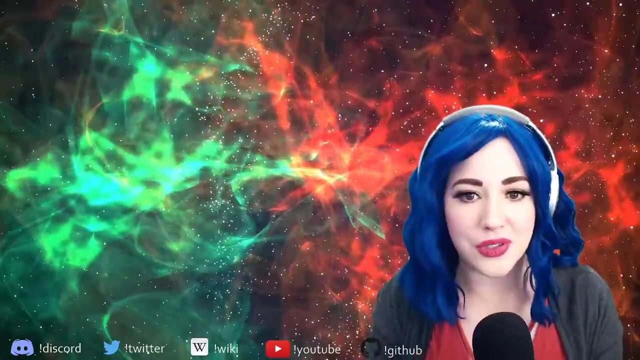 look at how wonderful it is. it is all right, so i'm gonna get a few other things here set up. feel free, though, if you have questions about previous days. you want to make suggestions for topics, go for it. um, that is all fine here while we're in kind of our just casual intro part of the stream. um. 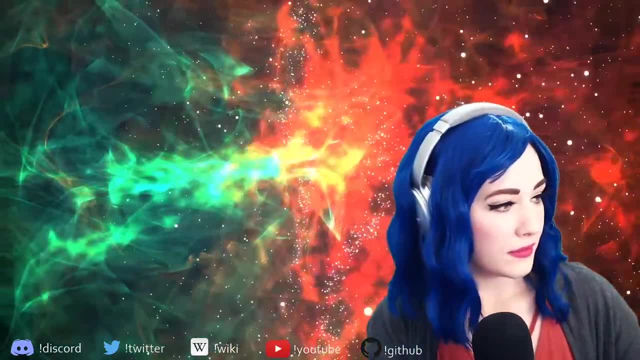 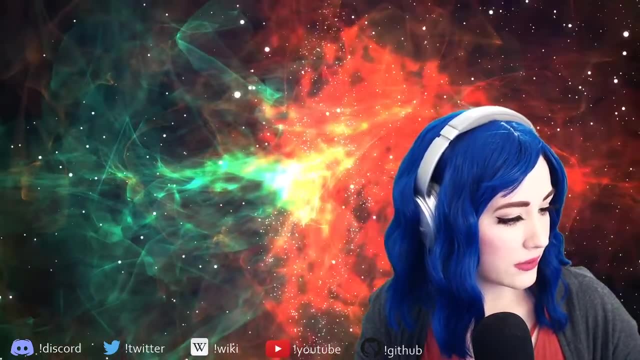 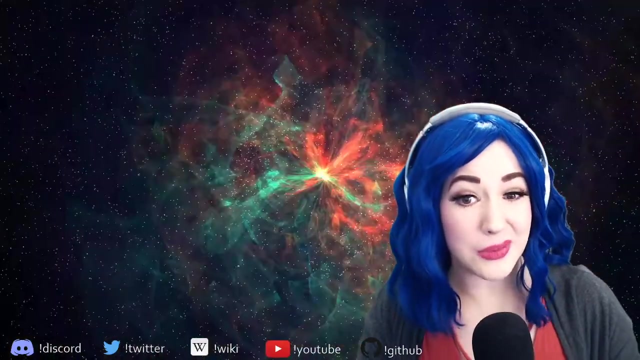 just looking up a few things, getting a few things set up here. how are the captions? is anyone getting those working? i just want to double check. i feel like these captions have been more reliable than than previous caption services i've used, but um, still want to make. 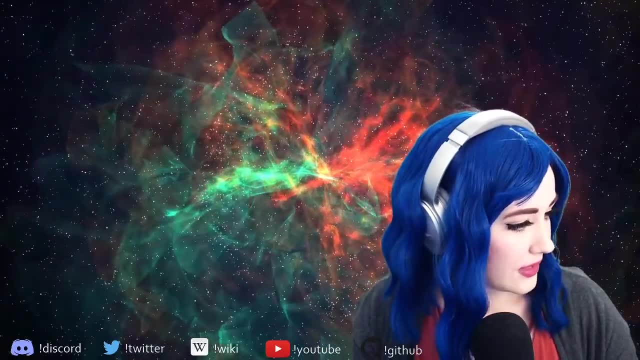 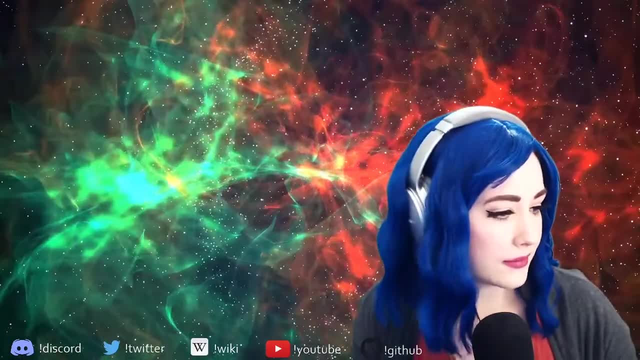 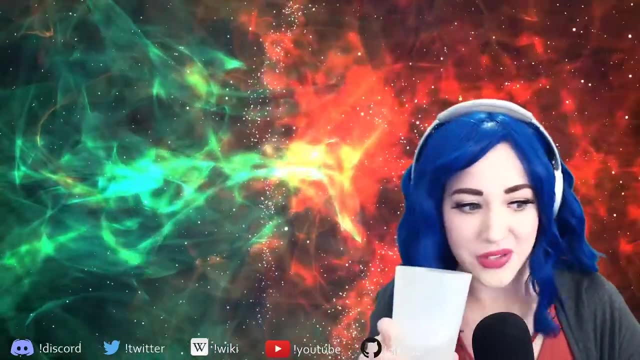 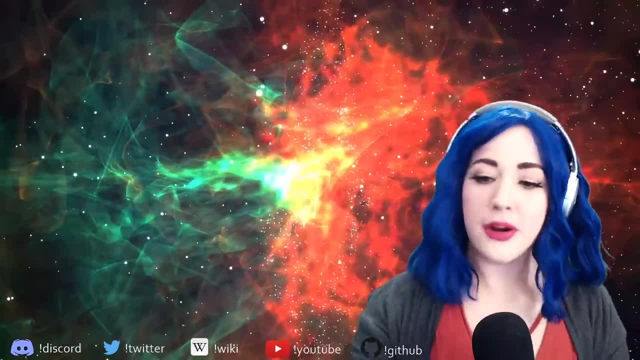 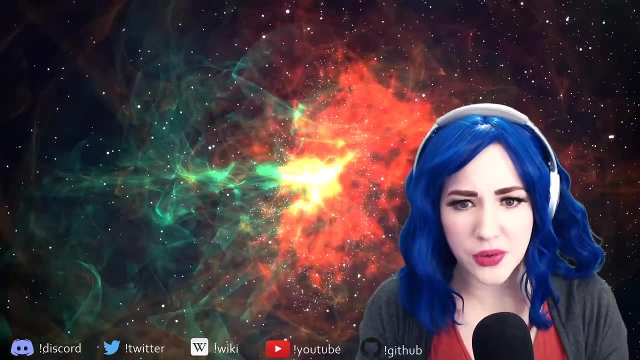 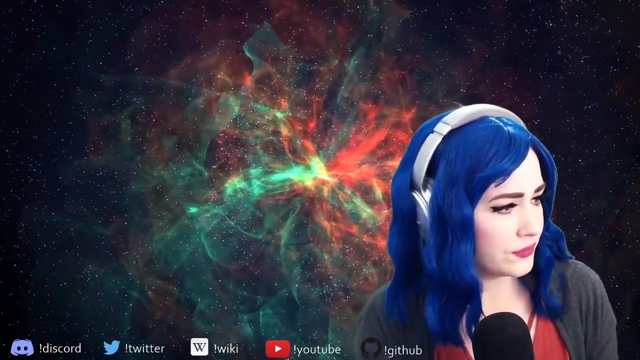 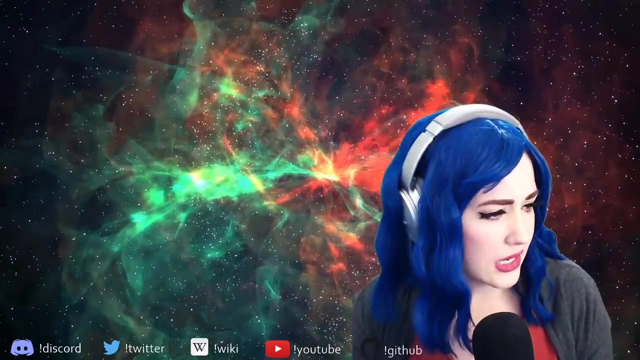 all right, so let's think here. so far in the fundamentals of data science series, we've talked about exploratory data analysis and what was the other? what was the other thing we talked about? I can't believe. I don't even remember my own topics, but you know, if that was two weeks ago- two weeks ago, I think, we did the EDA. 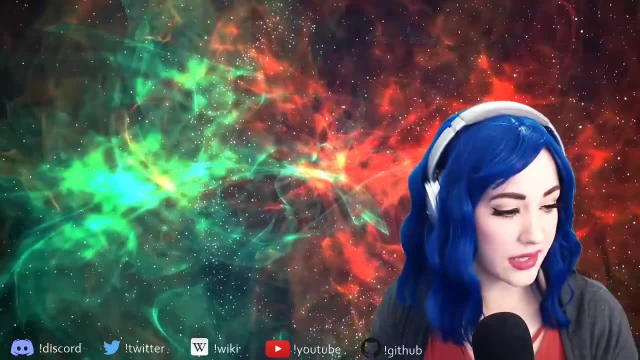 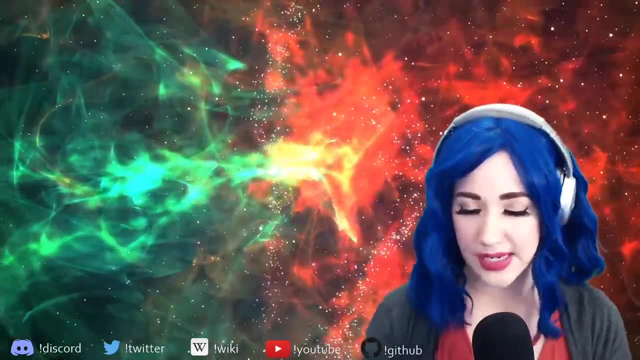 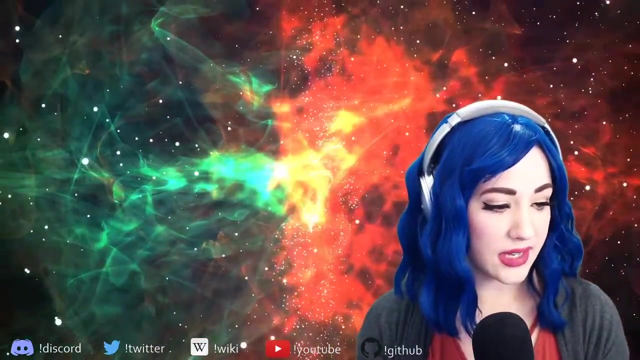 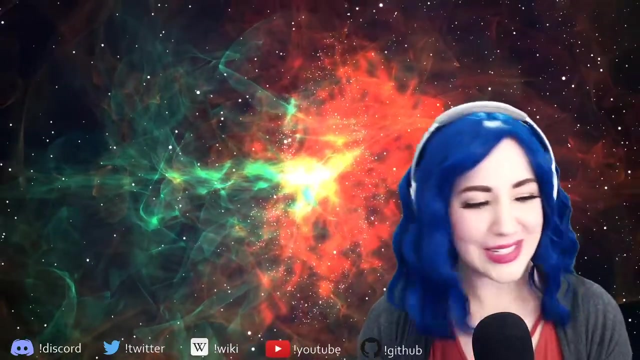 oh, we did, nope, two weeks ago we did pre processing, scaling and dimensionality reduction. so if there are any questions about either the EDA exploratory data analysis stream, which was data science fundamentals number one, or pre-processing scaling and uh dimensionality reduction, which was fundamentals of data science two, though i guess these really shouldn't be done. 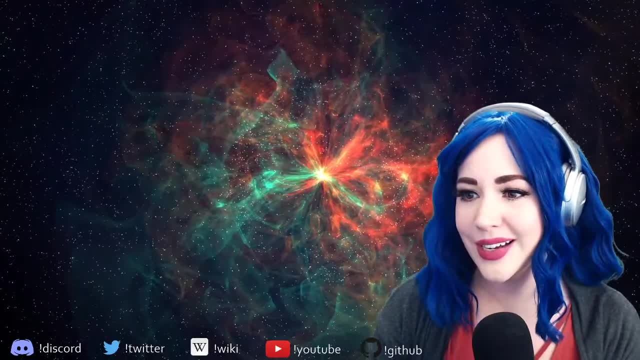 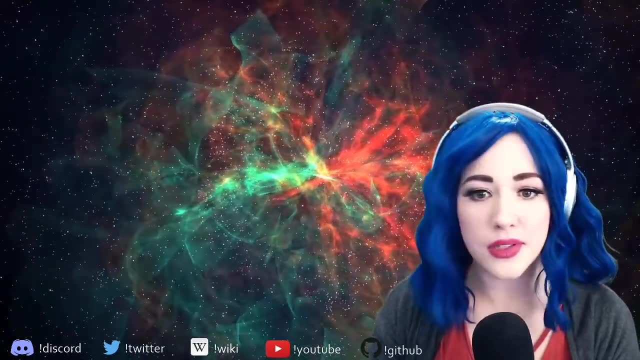 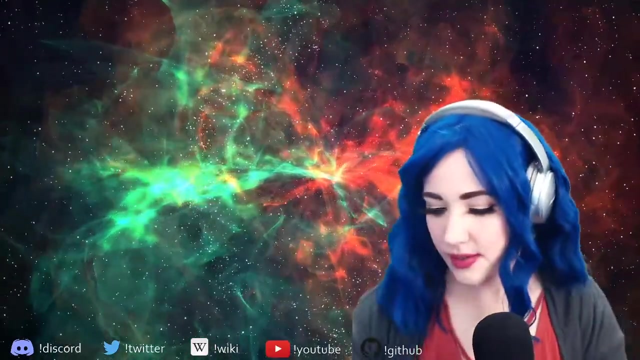 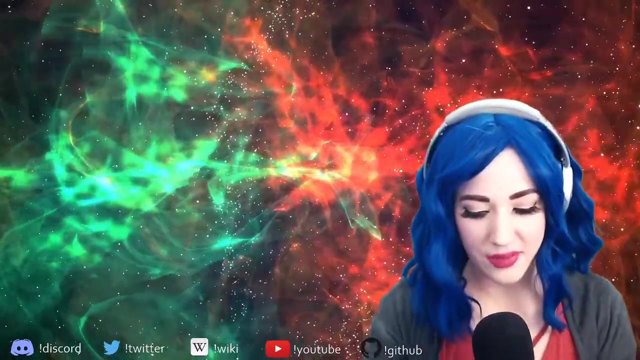 in order, because i'm sort of just picking random topics and going for it, um, but if you have any questions about those, please, please, please, feel free to speak up, um, and i will get our whiteboard here all set up. okay, too many things on my desk. i say this: i feel, like every stream, that i need a. 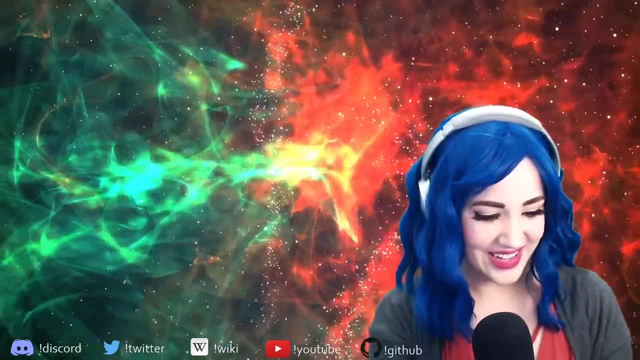 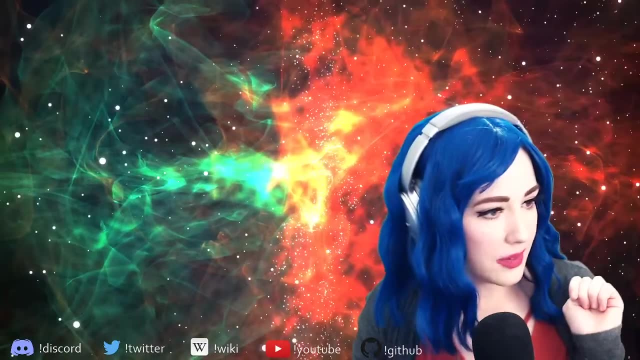 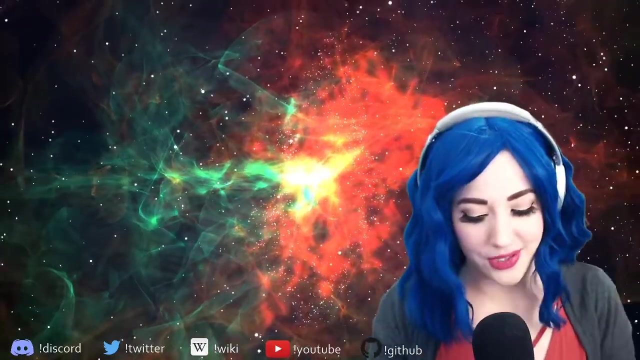 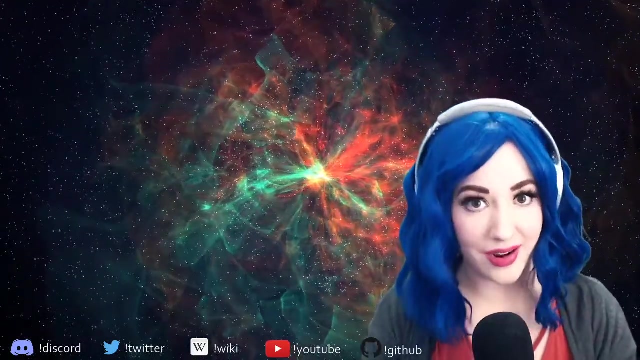 bigger desk. all right, um, that is all set up. that is set up. that other thing is set up, and i left my door open today, which is which is risky, because that lets the dogs into my room. so hopefully they are going to be very good boys and not knock over the green screen, um, but i wanted them to be able to come in. 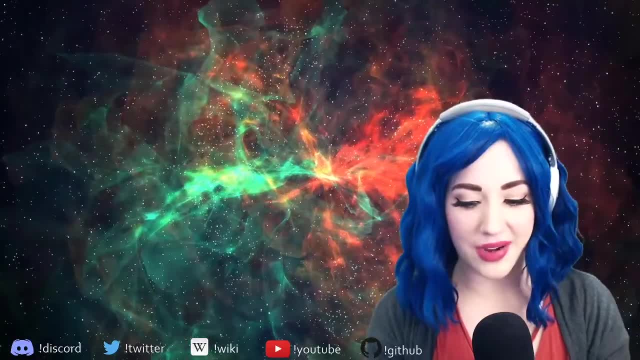 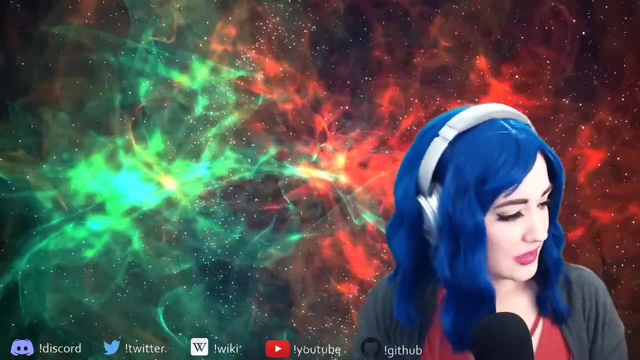 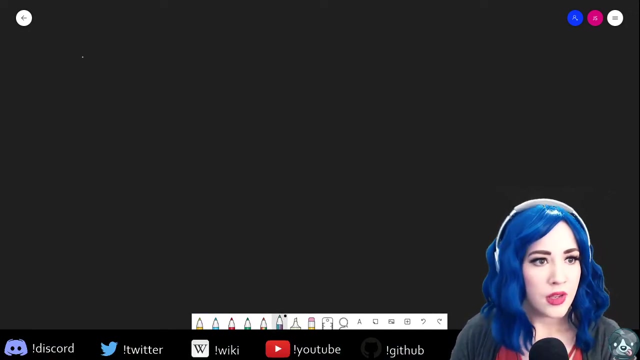 and like lay down and kind of be, be near me if they wanted to, um, so we'll see. we'll see how this goes. all right, friends whiteboard. all right, so let's, let's get started here. um, um, um. and what are we talking about tonight? so we are talking about getting. 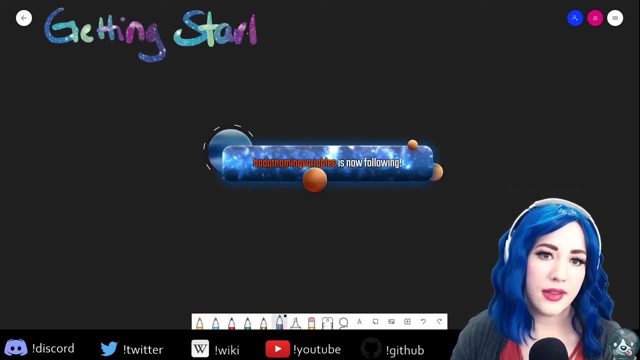 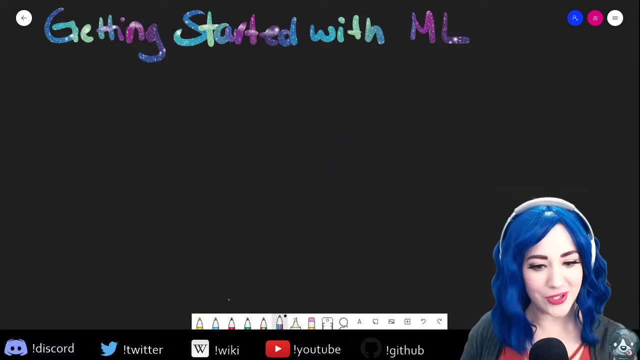 started with. oh no, it's not gonna fit. ml, i'm gonna abbreviate machine learning, so i'll do a little like machine learning. this is cheating because i can't fit the whole title at the top, and bad at naming variables- me too welcome. welcome to stream. i hate naming variables. there's definitely that challenge. 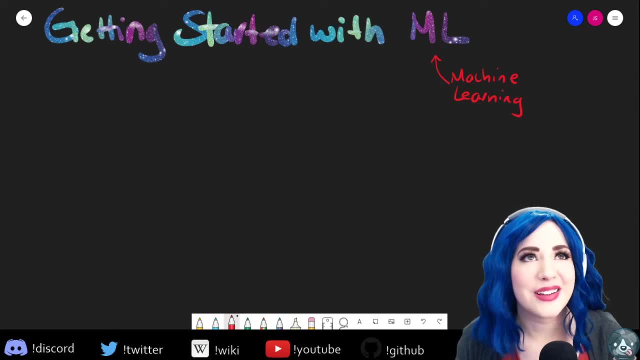 sometimes. so i'm sitting there like what do i call this? like, how do i keep it succinct where i don't have to type a lot of things but also keep it informative? so i'm right there with you. um, the nasty code that nobody ever sees that i write just for me. oof, those are. those are some, some icky. 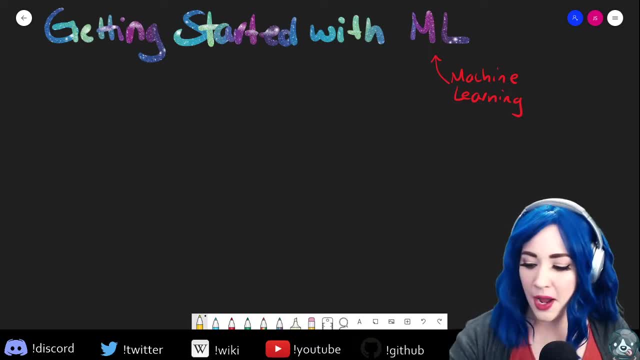 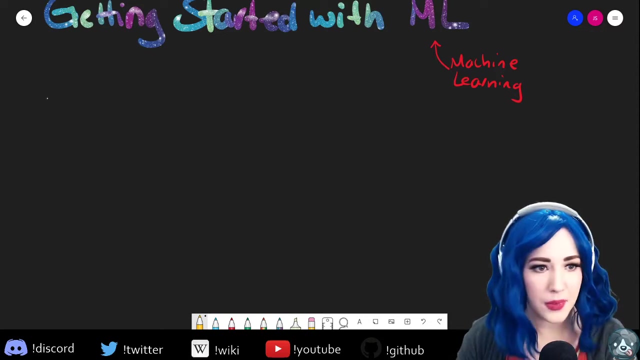 variables. all right, so let's see da day two. thank you so much for following. welcome. welcome to science sunday. welcome to stream. all right. so this is part of a broader series um of streams, all about the fundamentals of data science, and so let's just like let's do a little bit of review here. what even is? 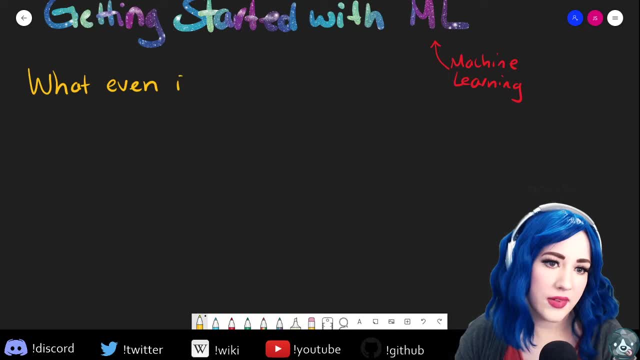 what even is data science? what goes into it? what do you think i want? i want, i want chat. i want some of you to tell me what do you think goes into it. what do you think i want? i want chat. i want some of you to tell me what do you think goes. 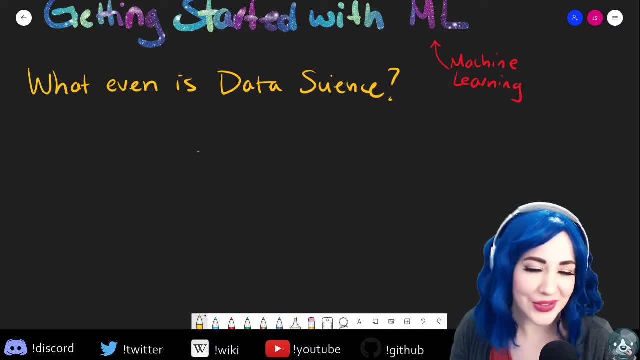 into data science and asaluja, welcome hi to you too. happy sunday. hopefully those of you who are in the united states have a three-day weekend. um, we met at shirley's stream. i, yes, okay, yes, oh, i loved her stream especially. um, yeah, i feel like it's amazing to watch people be. 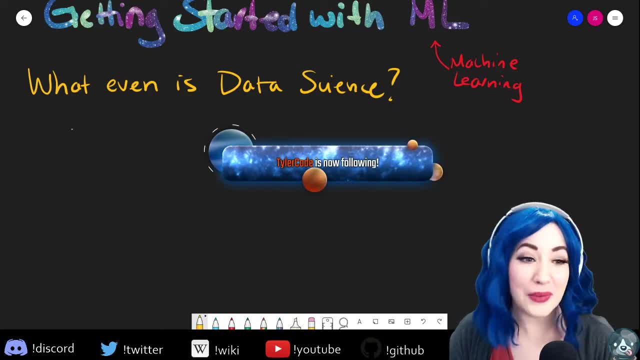 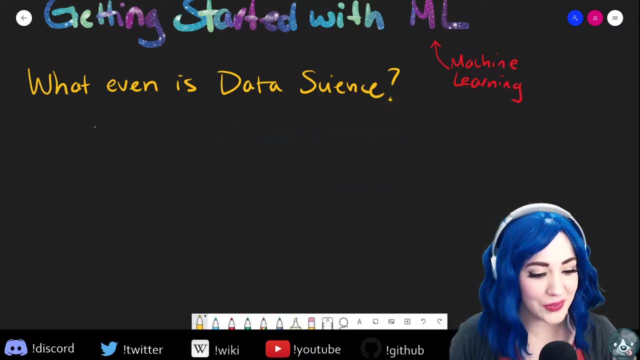 good at things that you're bad at, so i really like her stream and tyler code welcome. thank you so much for following. and angry chair. you say waffles. well, i i love waffles. personally, i think they're better than pancakes, but alas, waffles are not entirely part of data science. um what? what for real, do you think? 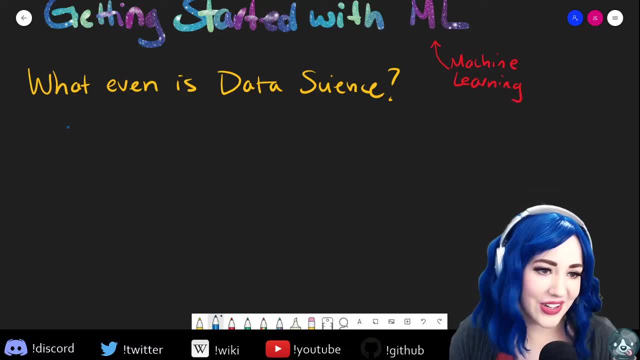 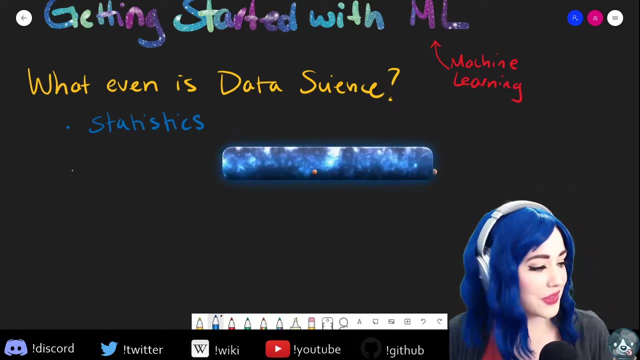 um, statistics, mechanically, dev, yes, good, all right. so statistics, absolutely, what else? what else do you all think might be part of data science? and wallflower 639? thank you so much for following. really bad data sets, poke gecko. oh, really bad data sets. ain't that the truth, unless, unless you're in. 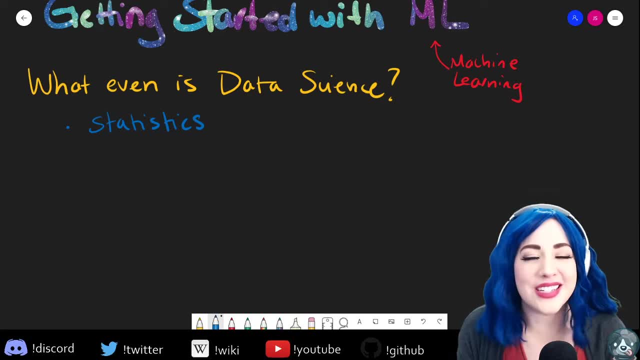 a boot camp, in which case the data sets are pristine and raid, oh my goodness, okay. so i'm gonna give myself a little reminder here to wait a second for the raider to enter chat, because i always get way too excited when people raid. so i'll i'll wait for tyler code to be able to enter chat. 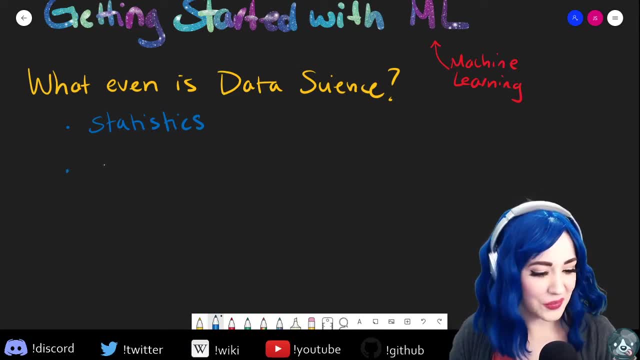 So I can, I can thank them very kindly for rating, But in the meantime, gaze into the iris. You say cleaning up lots of data. Yes, data cleaning, Absolutely Data clearing. apparently, from the way that I'm writing, data cleaning. 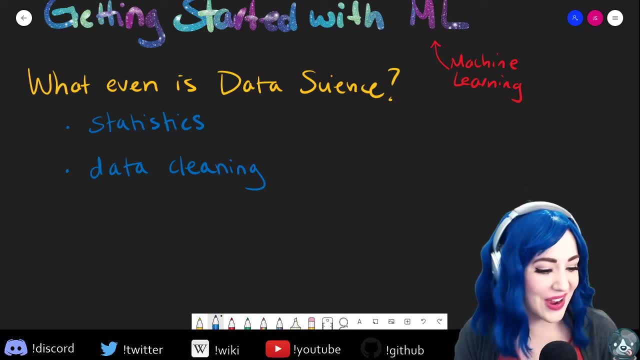 You've got it. And hi, Tyler, Thank you so much for the raid. It's. thank you so much. Let's give you a shout out here. How is your stream? What were you doing? Tell me all about it, And mechanically. thank you so much for following. 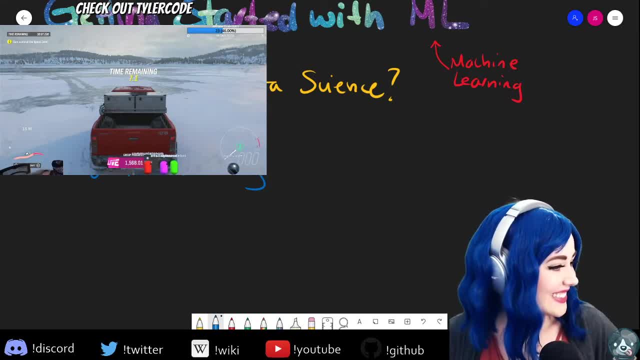 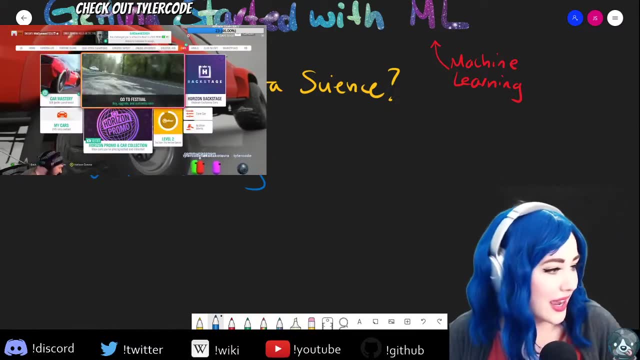 Let me see: Oh, yes, PUBG. Is that? I think that's PUBG, isn't it? It kind of looks like PUBG. No, but I don't. Oh, I haven't played in ages, so it looks like there's much cooler cars now. 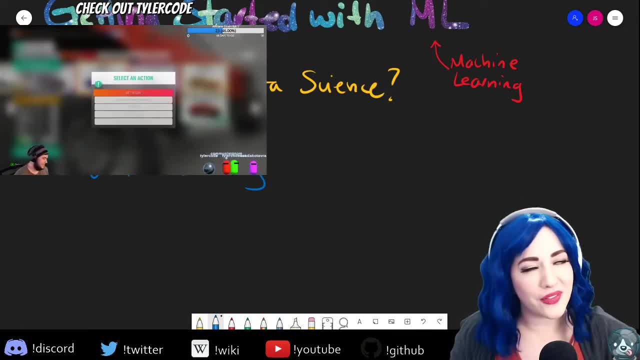 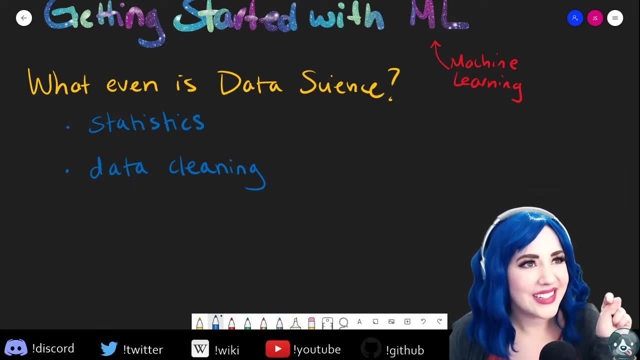 No, that can't be PUBG, So it's Forza Horizon. OK, see, look, I'm a failure already. I saw the countdown in the middle and that the shout out box is like super, super tidy. So I saw the the counting down in the middle and then I don't know. 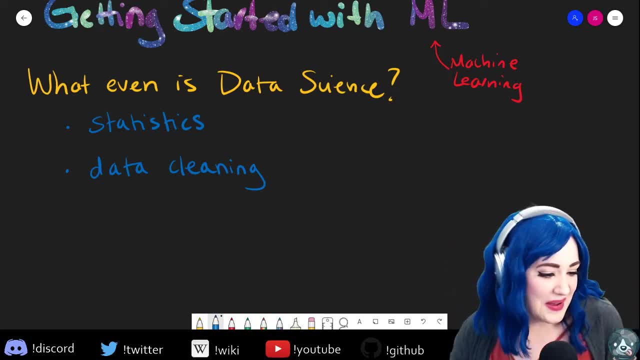 It looks like PUBG to me for a second. But- and yeah, Tyler, it picks a random, picks a random clip. so I can't control it, Or maybe I could tweak it, I don't know, But it picks a random one. 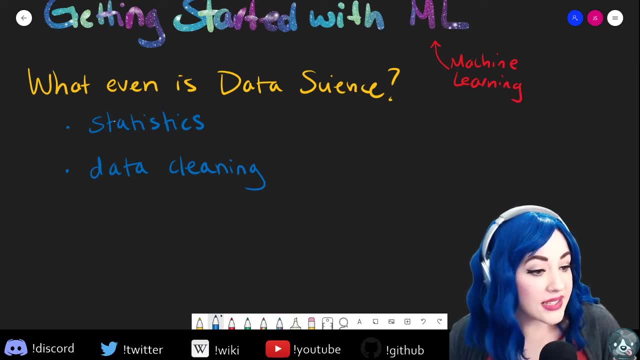 Sometimes they're really funny. And also you say: data science is finding insights and taking actions based on it. OK, so let's, let's say maybe like extracting Insights. I like that. And Oh look, everyone knows each other. 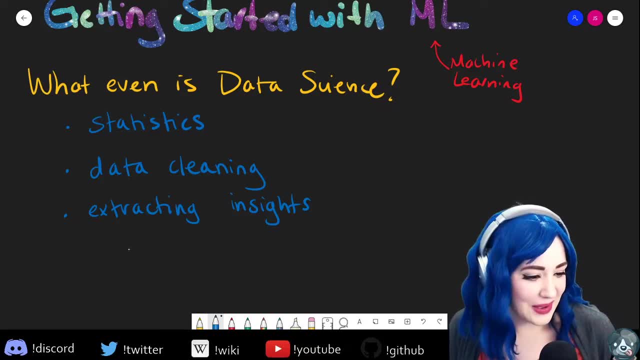 That's awesome Small, small world. But let's see, Twitch is a small place and Twitch is. Twitch is an even smaller place in the science and tech community. Like we're growing, I think we're growing- and there's some heavy hitters. 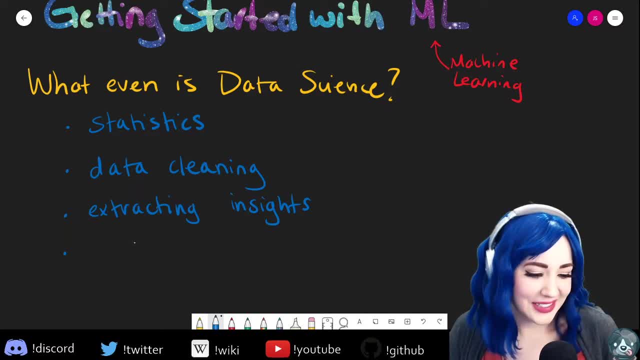 that like pull in some good numbers but nothing like gaming. So I feel like eventually we're all just going to know each other. But in any case, you say your stream is game dev. And how do you say it? Valheim, Valheim. 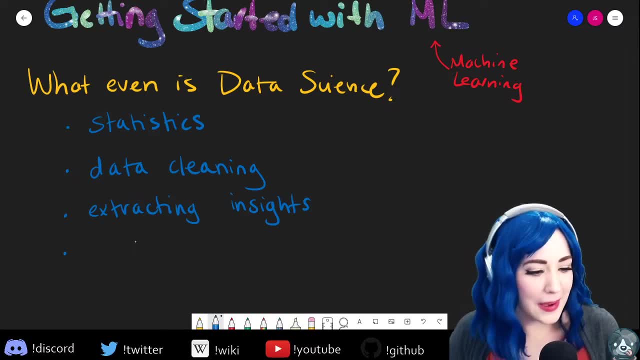 Like. I've seen people play the game. I just actually have never said the word out loud, But that's awesome. What kind of game dev do you do? I'm, I'm. I do game dev on Thursdays, but I'm very much a beginner. 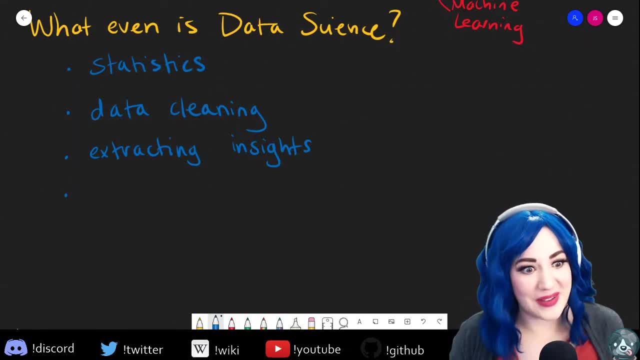 So they're very much a beginner, But in any case, statistics, data cleaning, instructing, insights- well, obviously I'm going to spoil something here for you, because this is what we're talking about tonight, But obviously machine learning is going to be part of it. 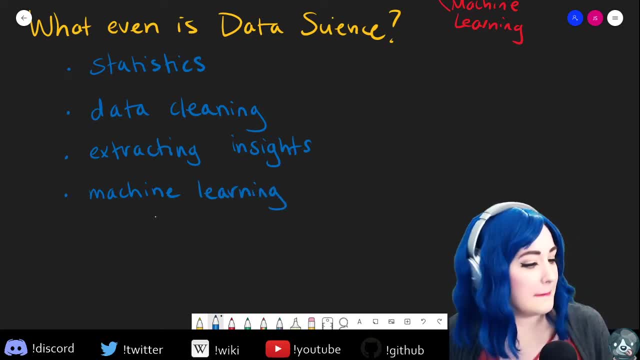 because that's what this whole stream is going to be about. But unity, Oh awesome. I'm learning unity too, But again very basics, But I love it. Unity is really cool. I'm loving learning C sharp- Good, good, good stuff. 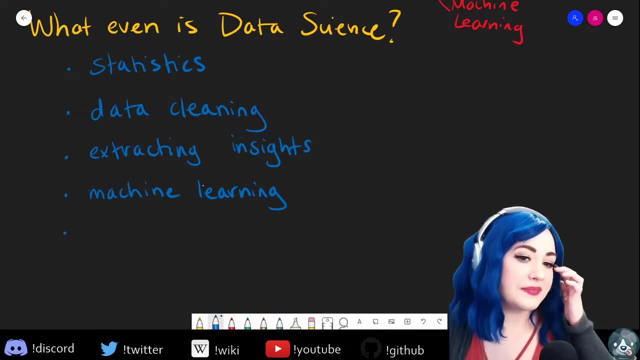 OK. so what else? What else goes into data science? Um, obviously I'm learning C sharp. I'm learning C sharp. Obviously I'll put a little star here, because, yes, this is, this is going to be what we're going to be doing tonight. 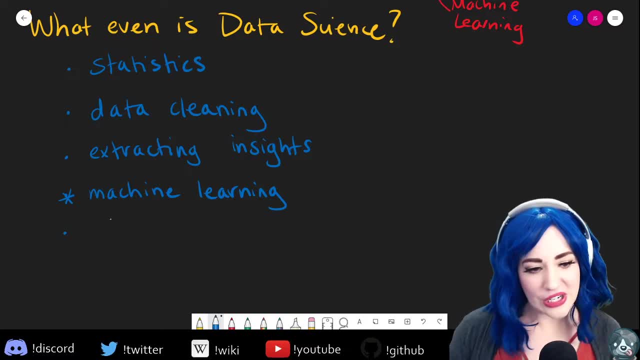 and be talking all about machine learning, getting getting folks interested and giving you a place to start with machine learning. But there obviously is more to data science And I want to like fill this out just a little bit. So what else? 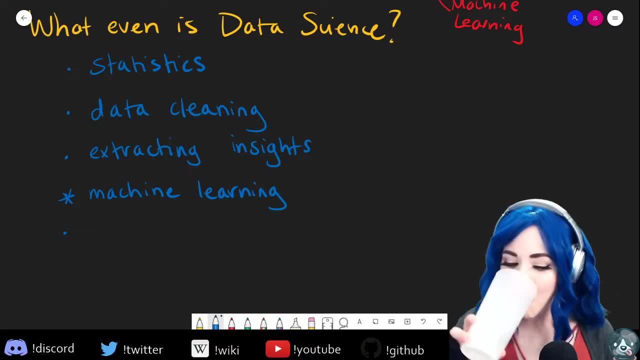 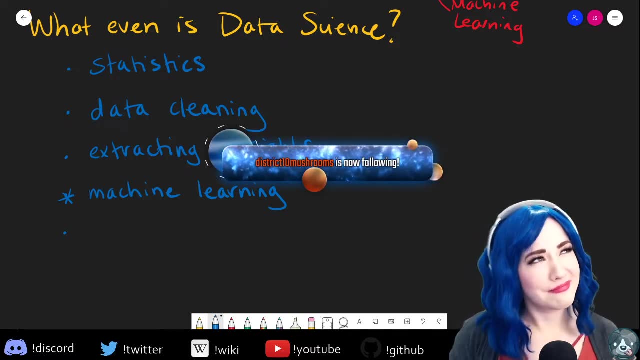 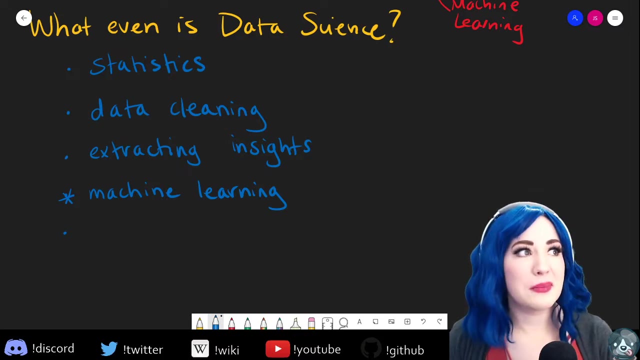 What else goes into data science And district ten mushrooms. Thank you so much For following. I love people's usernames. And just as a reminder if you are more interested in a deep dive- or yeah, deep dive- into specific machine learning topics, 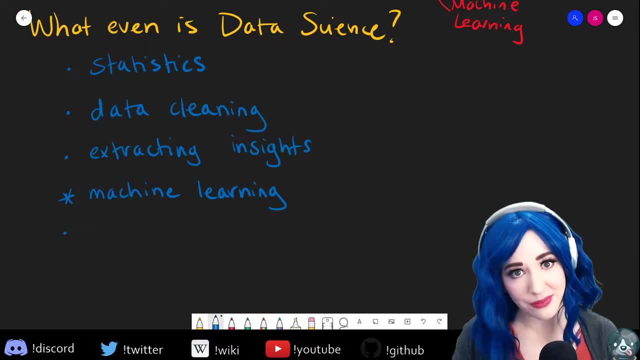 you can check out YouTube. I have the twelve days of machine learning, the streams that we did over the holidays. twelve different topics of machine learning, from everything like linear regression, logistic regression, all the way through computer vision. Those are all on YouTube. 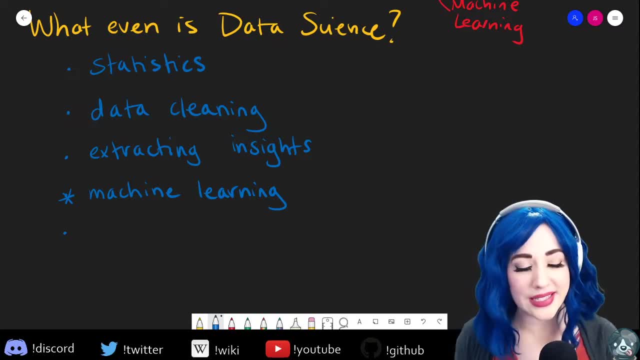 And if you missed previous science Sunday streams where I was working on the data science fundamentals and you're interested in more of, like you know, exploratory data analysis or dimensionality reduction, those two, those two videos or streams, VODs- are already up on YouTube. 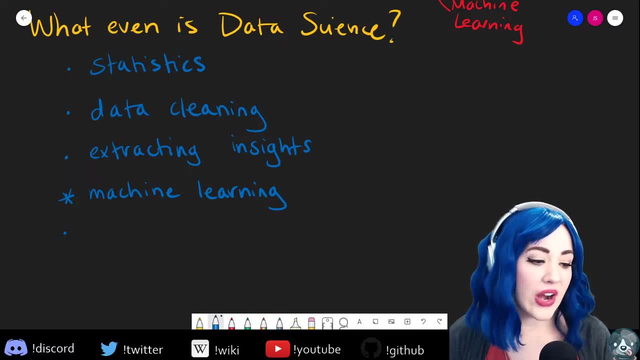 And the playlist is the data science fundamentals playlist. For everything I do, though, the, the VODs. well, not game development, because I don't know if anyone would learn from that, because I'm a total noob, But the, the streams that I prep for all of you. 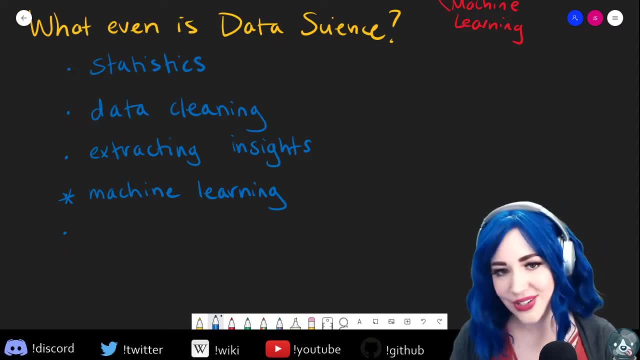 So the data science, machine learning stuff, like that, All of that's on YouTube, All the code and notes you can find on GitHub. Now the what was the Math Mondays is the other series. Sorry, duh, Tomorrow Math Mondays. 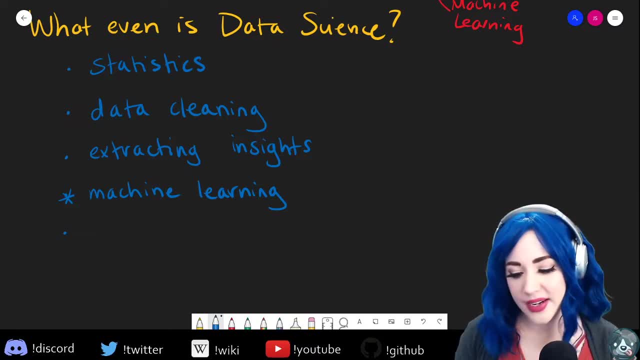 And we're starting all the way, all the way back with algebra, And it's a beginner friendly stream. So like, even if you hate math, even if you haven't done math in years and years, like this stream is for you. And if you go to YouTube in the 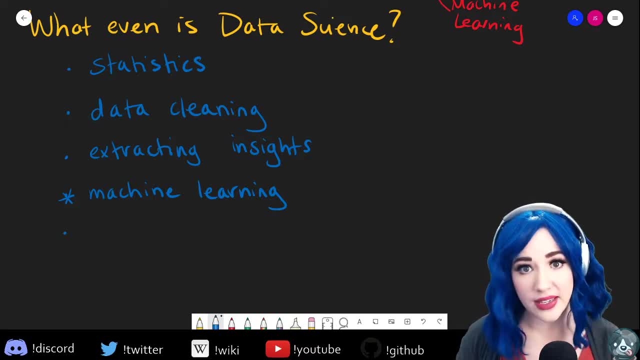 video descriptions. you can find the Google Drive link that will have all of the whiteboard images, blackboard images for those streams as well. And let's see Asaluja. you say data engineering. OK, yeah, absolutely Data engineering. 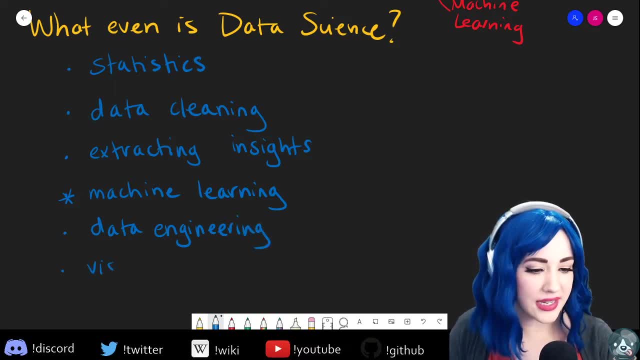 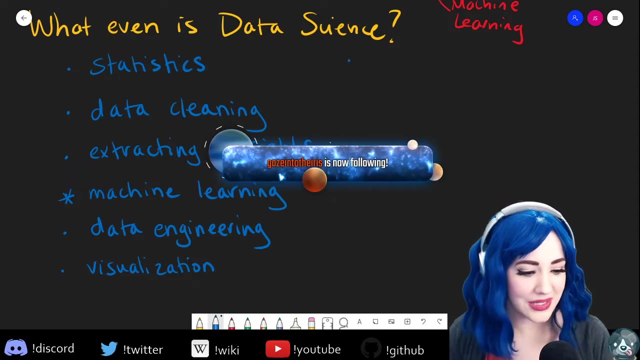 You, you got it. And you also say visualizations. You are totally right. This one sad face, That is what I'm very bad at, But and gaze into the iris. Thank you so much for following Welcome. Welcome to Science Sunday. 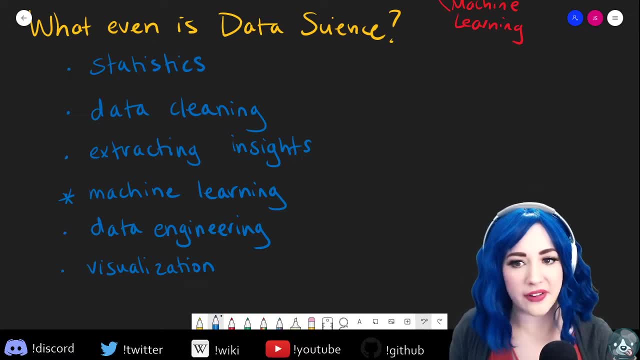 And domain expertize, Yeah, So I'll put this kind of- I'll put this in a slightly different color, because I would say: this is: this is a cool part of data science, but it's not strictly like if you want to learn data science. 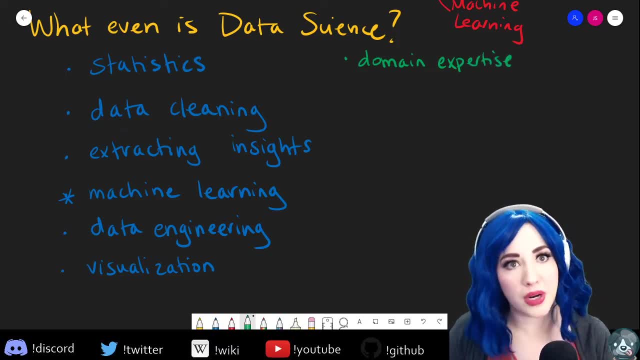 you. often you don't learn the domain. expertize Like this is something that you bring to the table. So, regardless of what you know, you did previously, a lot of data scientists come from a different domain And they bring that expertize with them. 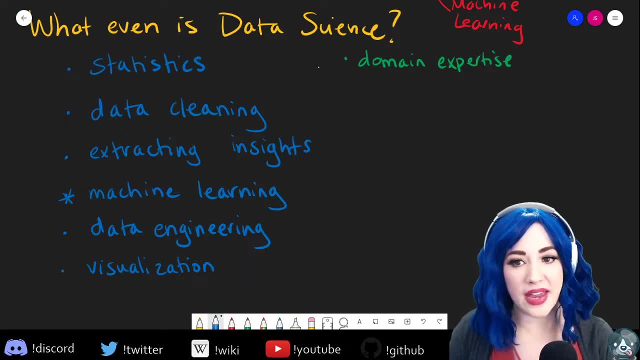 So they'll learn all this other stuff. But then you know, this is kind of almost like previous experiences that they've had. But you're absolutely right, That's part of it. I'm going to add in here that communication. So being able to communicate, whether it's written or verbal, being able to communicate your results and these, like you know, these insights. 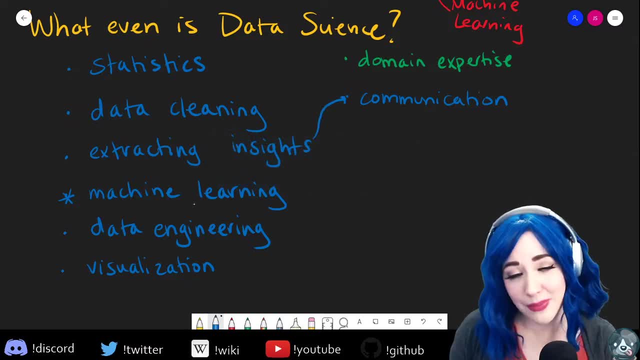 So being able to talk about them and communicate them. So being able to talk about them and communicate them. So being able to talk about them and communicate them to whoever your customer client stakeholders are, That is a critical part of data science and a blends. 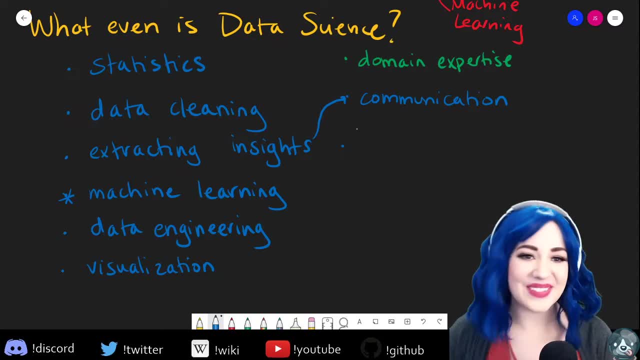 Thank you so much for following Welcome. Welcome to Science Sunday. OK, so let's think what else I mean. so I'm going to do statistics and math here, because there's a lot more math that we need, other than just statistics for data science. 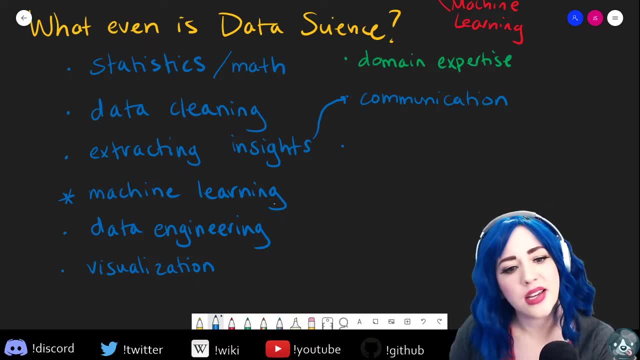 data cleaning, data engineering, visualizations, extracting insights, machine learning- What else? Programming? Programming- And even though it's often overlooked, some good like software development skills always come in handy. What else did I write down? So extracting? 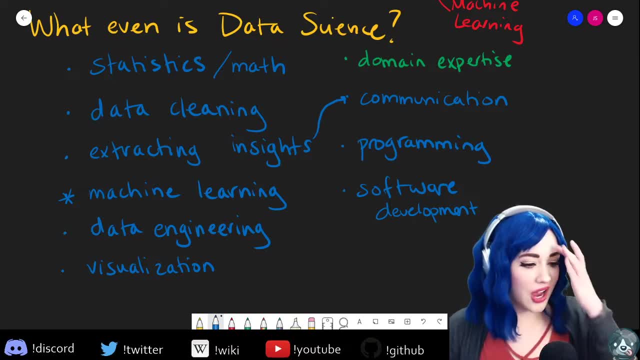 I'll say this is like data analysis, kind of: Do I need some JavaScript help? Wait, no, I'm going to be positive. All programming languages are fine. All programming languages are fine. All programming languages are fine. I just I think I don't know what it was, but my one attempt, many, many, many years ago, to learn JavaScript went terribly. 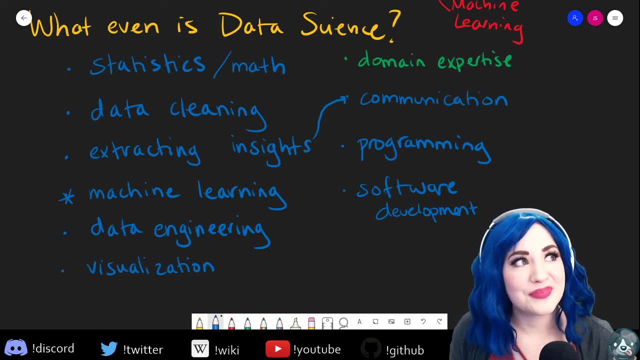 And so I am. I am open minded and will someday tackle that again, probably actually someday soon, because it would come in handy. But but I definitely have this knee jerk of like: oh no, because I had a really bad experience with JavaScript first. But? but I definitely have this knee jerk of like, oh no, because I had a really bad experience with JavaScript first. But but I definitely have this knee jerk of like, oh no, because I had a really bad experience with JavaScript first. 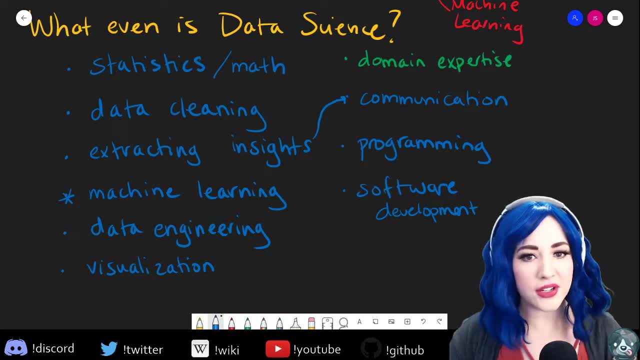 All right, I think this is a good, a good, a good starting place for for what is data science? And so, as I, as I mentioned earlier, this particular, this particular stream, we're going to be talking about getting started specifically with machine learning. 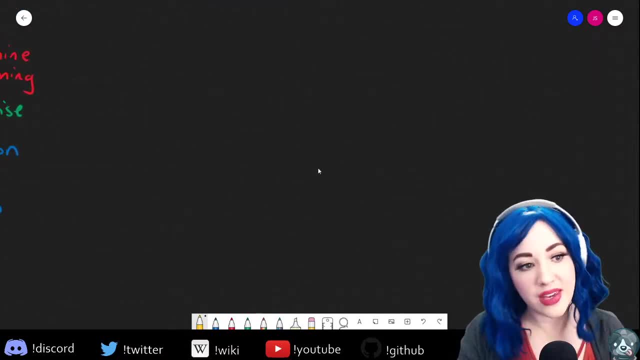 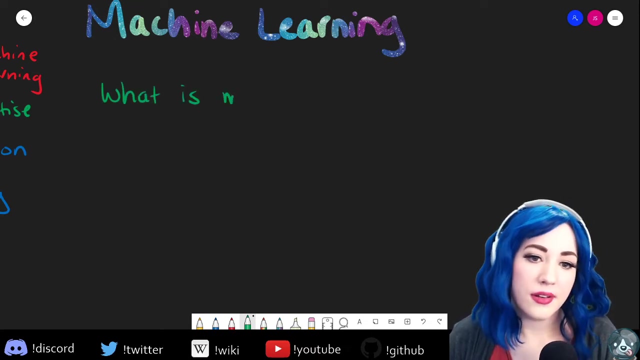 So That I might abbreviate as ML just for the sake of my wrists. but all That I might abbreviate as ML just for the sake of my wrists, but all Machine learning, Machine learning, All right. now here's a trickier question. 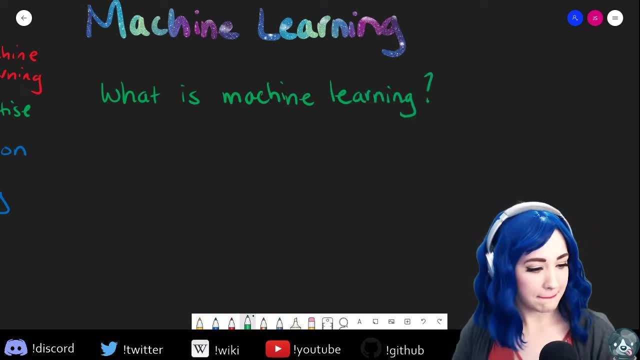 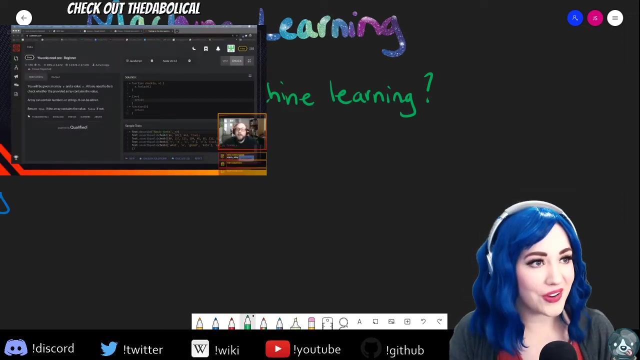 What is machine learning? Oh yeah, the topological. yeah, so actually let me give you a shout out, because you do such amazing code reviews. shout out the topolical. hopefully I spelled that right. the topolical does really wonderful JavaScript code reviews and wonderful like very, very friendly, very. 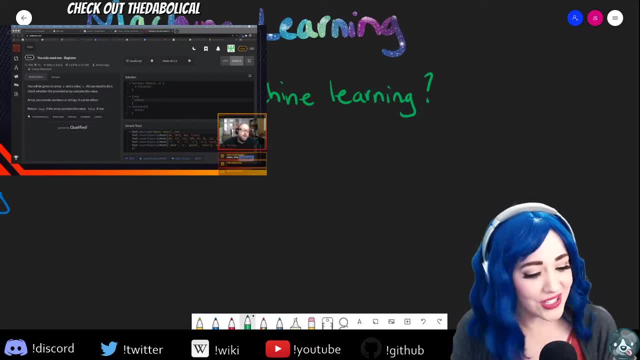 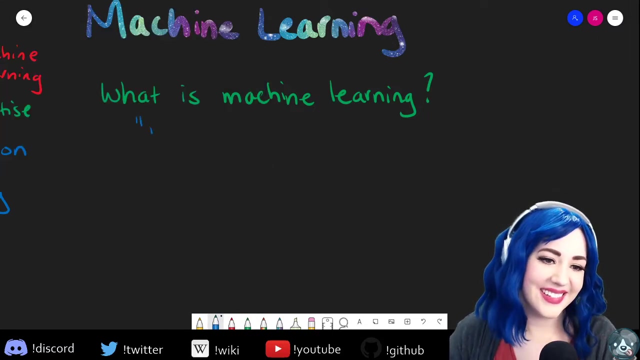 beginner friendly. he's, like always there answering questions, so you should, if you're interested in JavaScript, definitely give him a follow. lots, lots of fun. I sit there not knowing anything, but yeah, Okay, All right, Robot schooling. okay, who's into the iris? I like that. 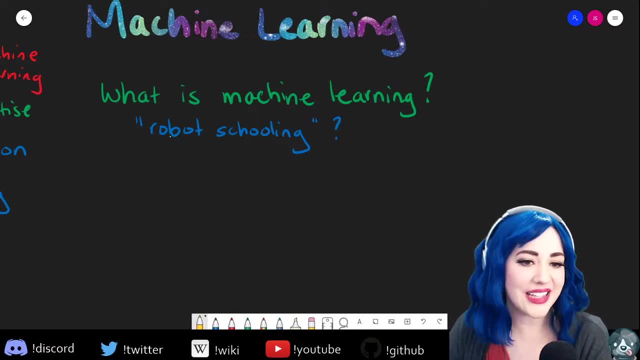 What else? What do you? what do you think machine learning is? and in this case I will say I I slightly push back on the use of robot, because I think a lot of people hear ML and what they actually think of is like robotics, maybe robotics combined with ML, but they're thinking more. 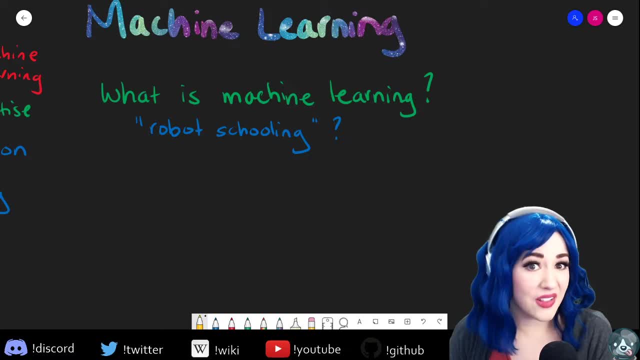 of like you know, I don't know- Cylons or something, whereas machine learning really isn't so much about robotics, it's not about creating like a walking talking machine. but what? what do you all think? but? but I get what you're saying: the schooling I. 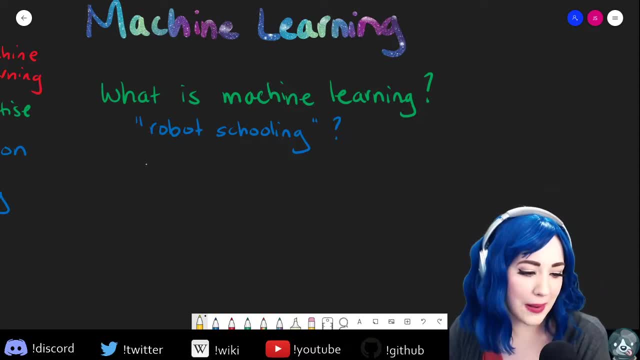 I kind of like the play on words there. but but what else? what do you? what do you think? machine learning is A hacker, the sass. so it's okay if you only have part of an answer. it's okay if you're. 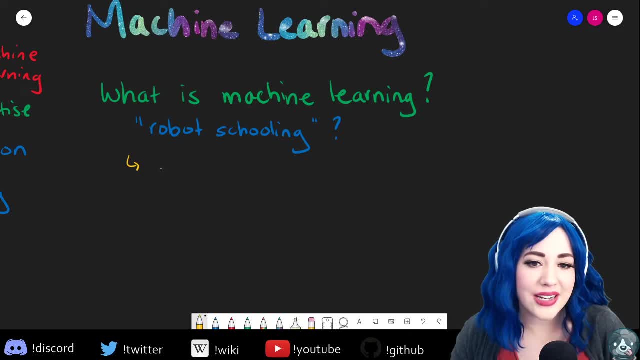 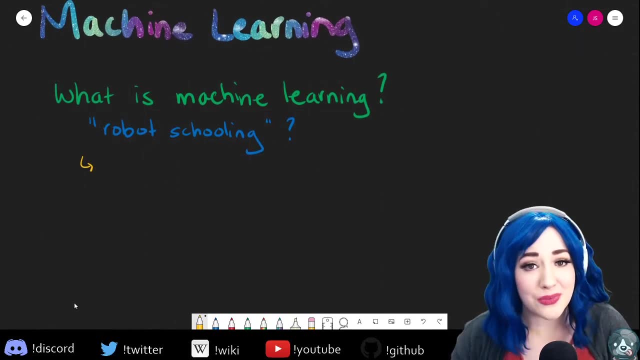 like you want to guess, but let's, let's try, try to define this, because I think there's a lot of confusion around machine learning and for a lot of folks it is a buzzword, but it's it's. I think it is something that we can define. 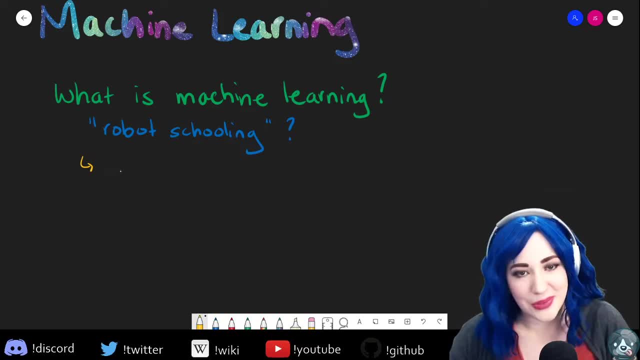 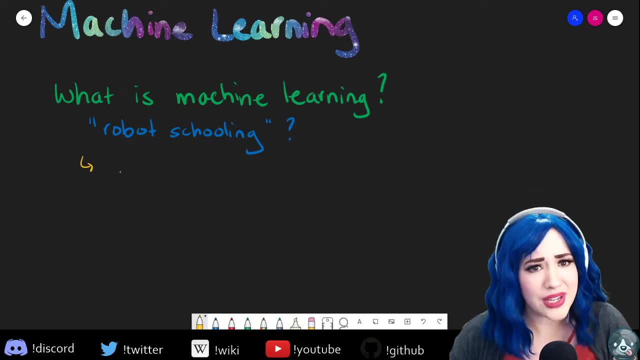 Machine learning is is more than a buzzword, though, And I think kind of putting some boundaries on it and talking about what it actually is, is is really important. So I think what did I write? okay, so this it isn't like it isn't robots walking down. 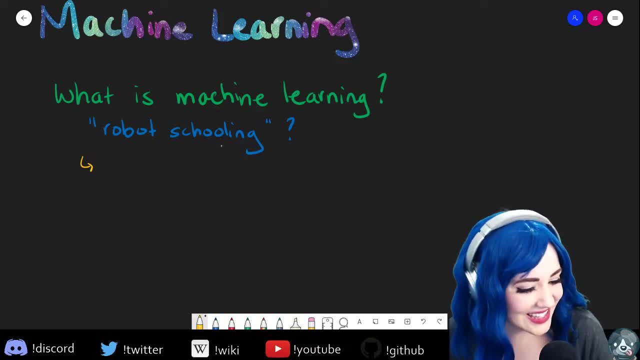 walking down the road. Let's see, gaze into the Iris. you say I'd say software capable of extracting insight from data. onends on its own. so i like that. so you say, on its own, which i really really like. um say it's more than. 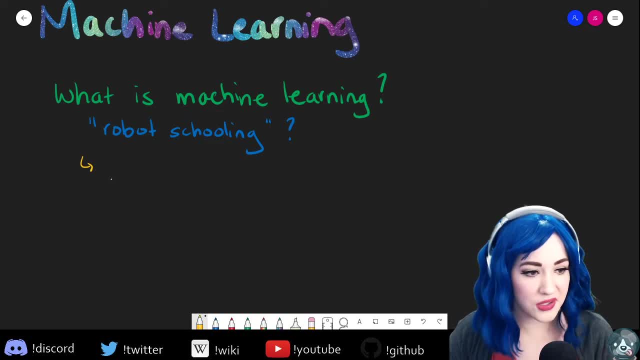 software, though often software is involved, obviously, because you have to like deploy it um extracting insights from data. so that applies to some areas of machine learning, but not necessarily all of them actually. um, so let's see, uh oh, i had like five definitions i wrote down, so 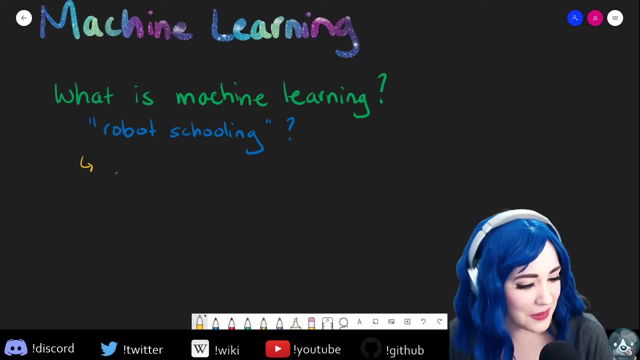 good job, me see. even i'm like: oh, how do you define this? um, also, lucia, you say building applications to become more accurate at predicting outcomes using the big data. so so yeah, people are kind of like there's on its own. so there's this element of maybe like independence. 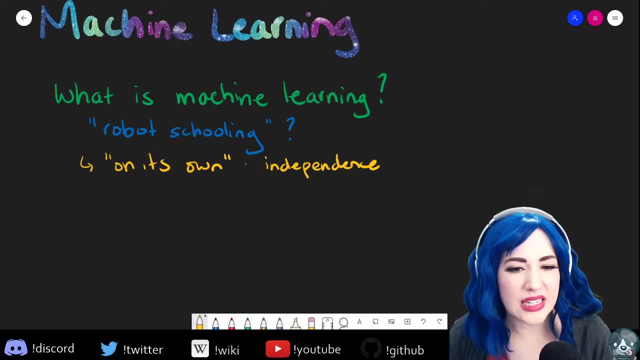 like it's not necessarily programmed to do the tasks that we want it to. um, and then also, lucia, you say predictions. now, one of the things, one of the ways that i like to define machine learning is: it's a method, it's an approach, it's a tool. oh, i can call you aman, okay. 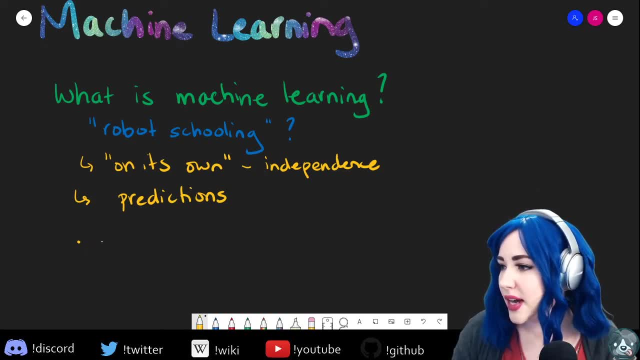 um, so a tool. let's see here what did i say? i said no, i again had like four definitions. um, i said how, it's how we get computers to learn to. so that's a little bit of a uh, a little bit of a uh, a little bit of a love havences and 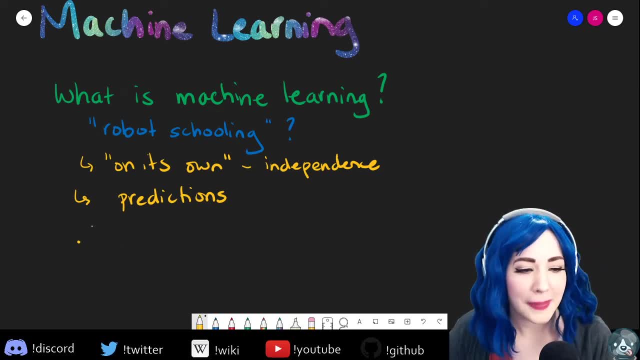 form tasks they aren't explicitly programmed for, because I wanted a definition general enough to encompass all of the different areas of machine learning, but also something that's not going to invoke um thoughts of like Skynet. essentially. so, it's um the method and this is this is what I'm. 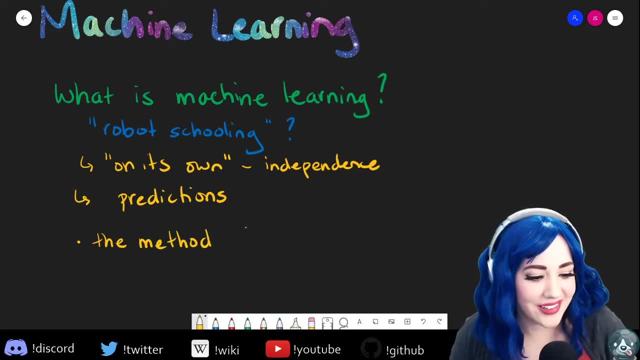 going to run with. but like there are as many definitions for machine learning, um well, Skynet isn't necessarily a method. so this is, this is a tool in your toolbox, it is a tool, it is an approach. um so, method for getting, let me see when I run into my face getting computers. 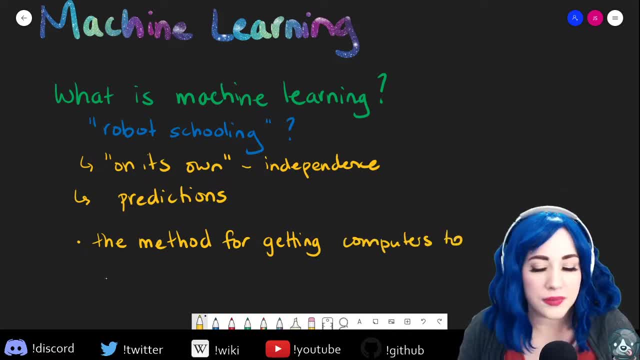 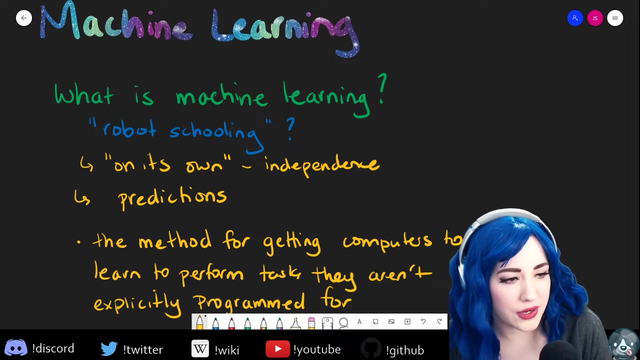 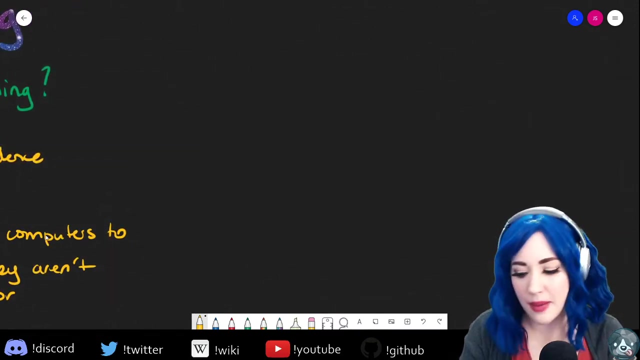 to say, learn to perform tasks they aren't explicitly programmed for, and this, like tasks that they aren't explicitly programmed for, is is kind of. is is critical because machine learning is part of a broader, a broader topic, and this is where maybe our, our thoughts of Skynet lead us, which is artificial intelligence. 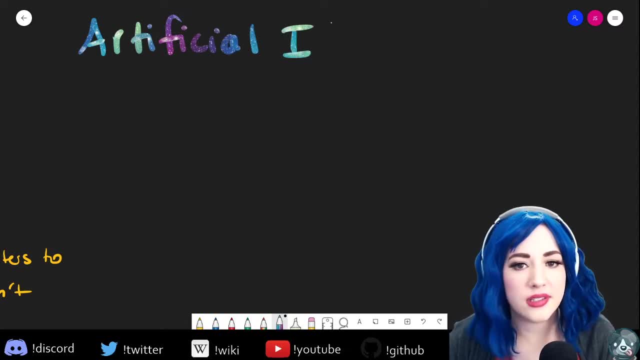 now artificial intelligence. finish writing. this is is more about that outcome. so it's it's. artificial intelligence is: how do we get computers to do tasks that we previously would associate, like you, needing human intelligence for? and so it the debolical you say. I welcome our new Skynet overlords and hi Mexican, I am from Skynet. 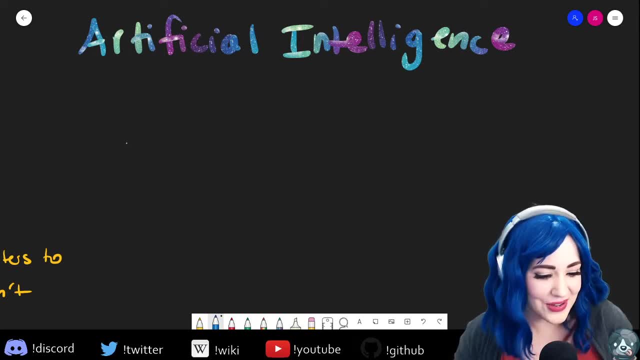 I am from Skynet, Skynet. it's a great place. I was born and raised in Skynet. Skynet is an excellent place for tech and hi. Mehmet, how are you? and no Newton? we don't. we don't rank different stem subjects. 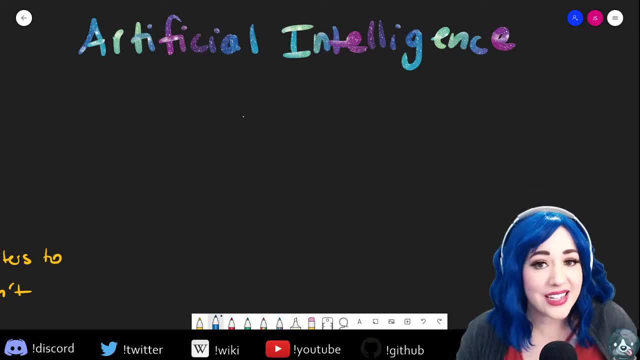 all science. science sunday is about all science. i tend to talk about the science subjects i know most about, um, but science science sunday loves all stem, um. okay, so artificial intelligence is is broadly that category of of trying to figure out how to get computers to to do tasks that we 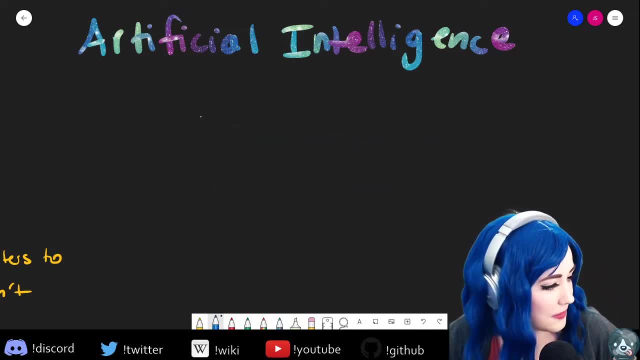 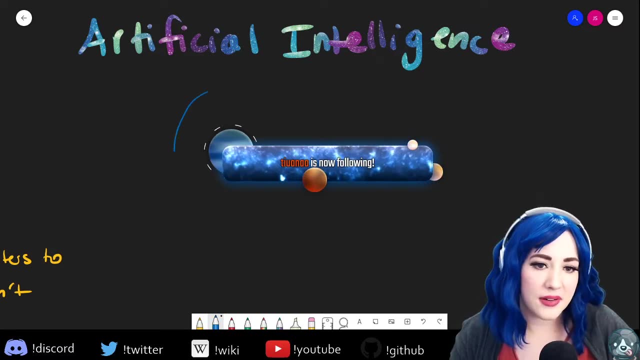 we think require human intelligence, um and mika poel and tijuana. thank you so much for following. welcome to stream. so if we're kind of talking about you know if this is, broadly speaking, artificial intelligence and all of the different approaches to that, machine learning. 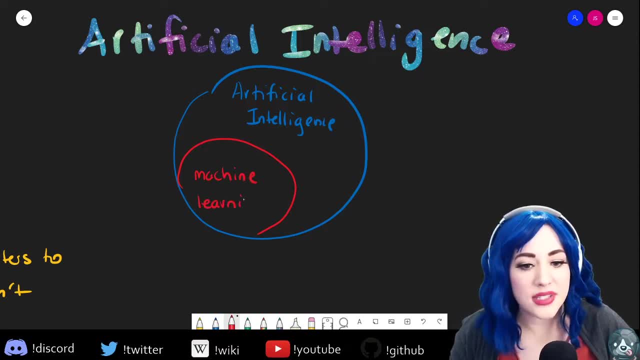 is just one method, and what sets it apart was the end of that definition i gave you. so teaching computers how to perform tasks they aren't explicitly programmed for. so this is like the computers- computers- that's what i get from talking. computers aren't explicitly programmed for the task. 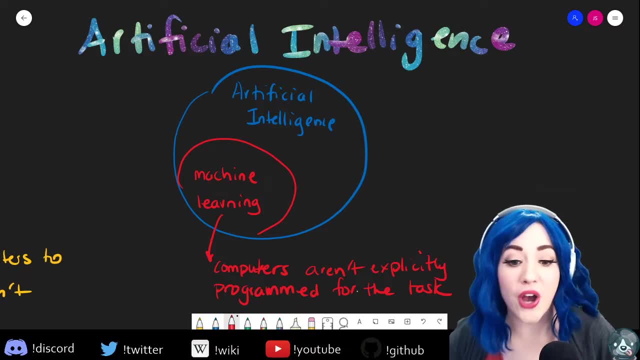 because you absolutely can have artificial intelligence, where the computers are explicitly programmed for the task, and so this is where this is where you might have what i like to call rules-based ai. this is not where we're expecting our computer to learn anything. we're not expecting it to get better, we're merely giving it a whole lot of different um. 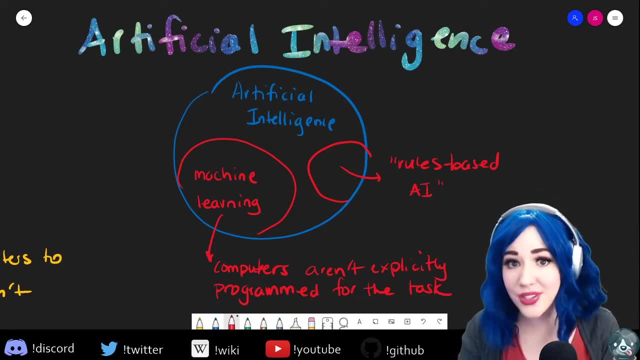 what do you call it like different conditionals? if this situation do this other thing, if this other situation, you know, do a different thing, and you can think about a scenario where you could program an ai with an exhaustive list of conditionals. but it's not really learning. 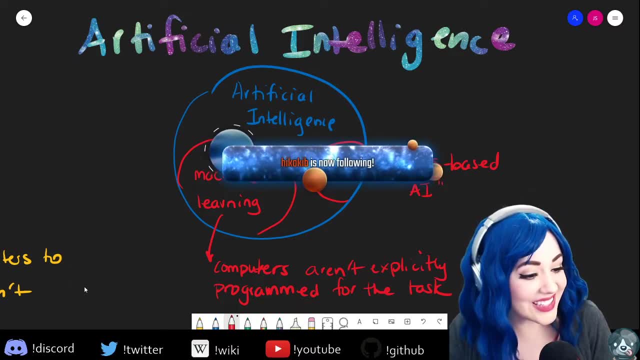 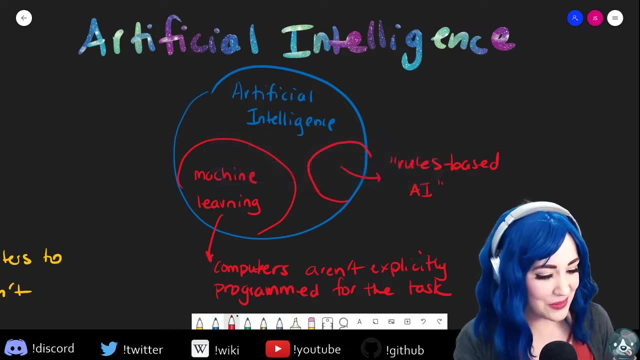 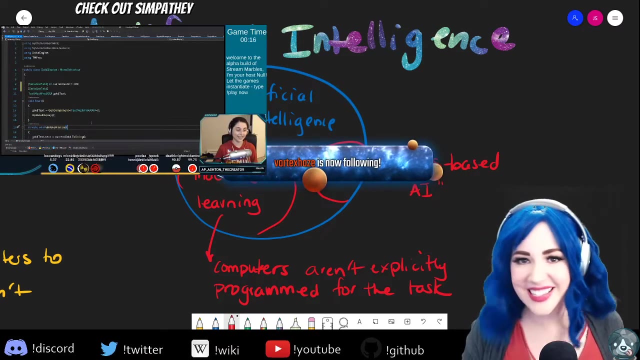 so it's not really machine learning and, oh my goodness, sympathy. thank you so much for the raid. how was your stream? i'm going to give you a shout out here. what? what were you streaming? sympathy, there we go, and hiko, keeb and vortex haze. thank you for following. 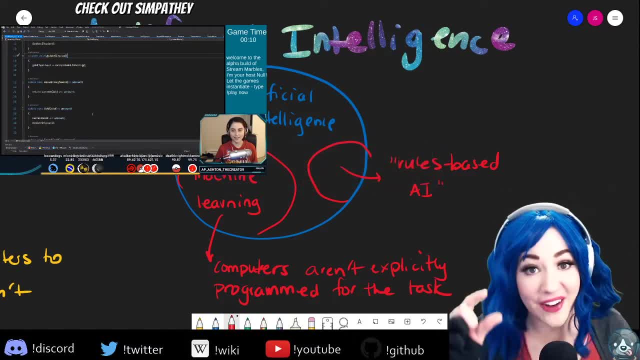 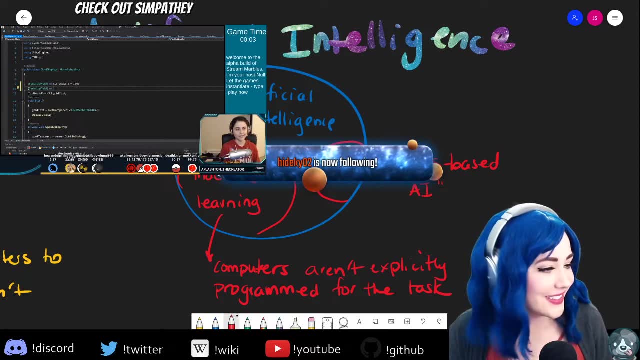 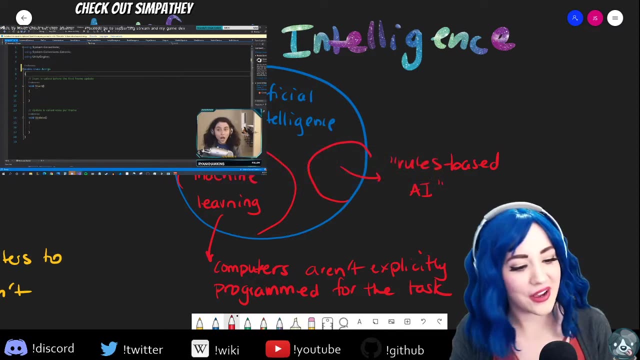 look at that okay. yeah, is that like i? that looks okay. i've got a very tiny window here, but that looks like vs code. nice, i can't even see what programming language you're doing on my, my tiny little like stream lab screen, but definitely give sympathy. a oh low phone, did another shout out? 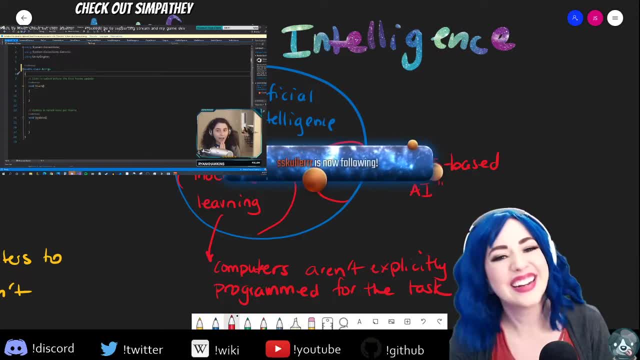 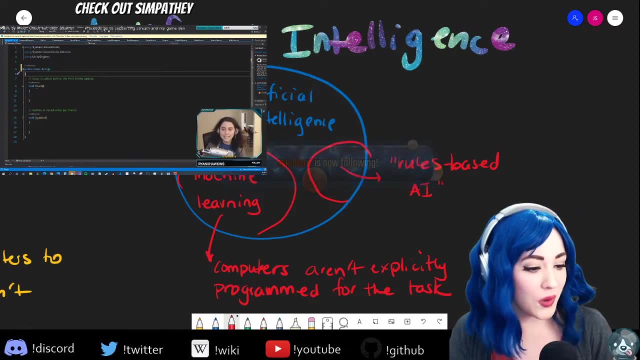 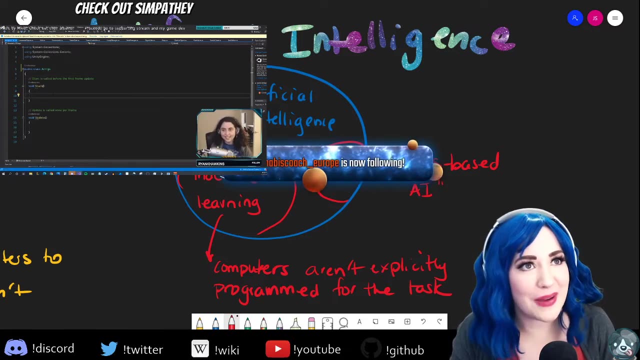 thank thanks. low phone, um, but how, how is your stream? what? what were you all doing? and sculler, thank you for following. oh, working on a mobile game? oh, that's really cool. i'm so new to game development that like even thinking about doing something mobile, i'm just like: nope, i've got my happy little like unity. 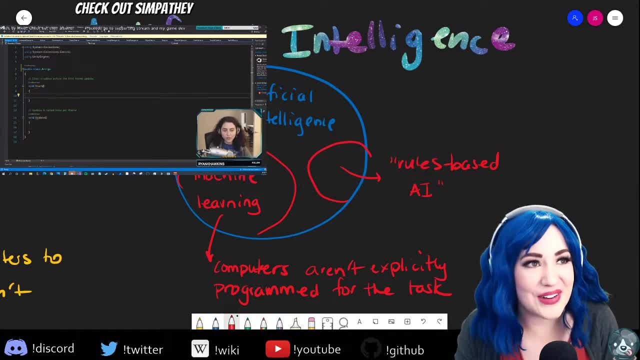 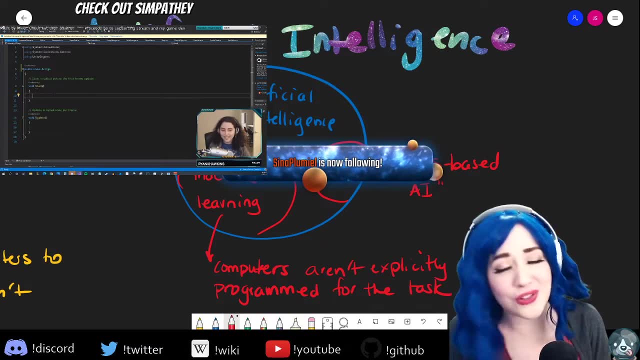 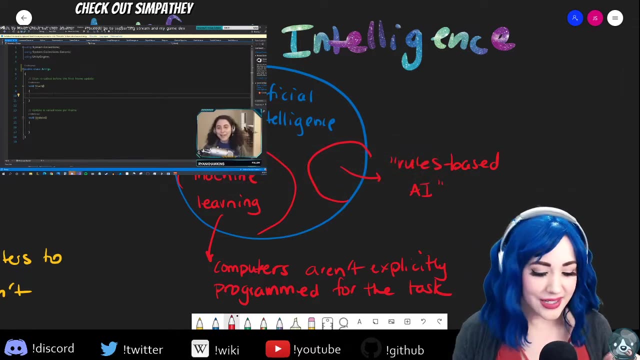 universe where i can do some basic stuff, but i can't even imagine thinking about, like other platforms, um, cannabis, coach europe and sina plumio. thank you so much for following. so for all of you, all of you readers, today is science sunday and we are going to be talking about machine learning, so this is part of a stream series. i'm 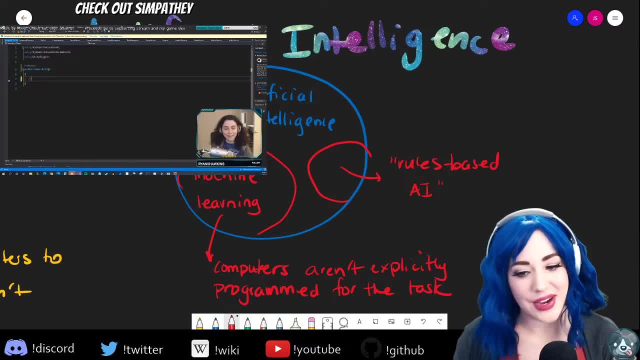 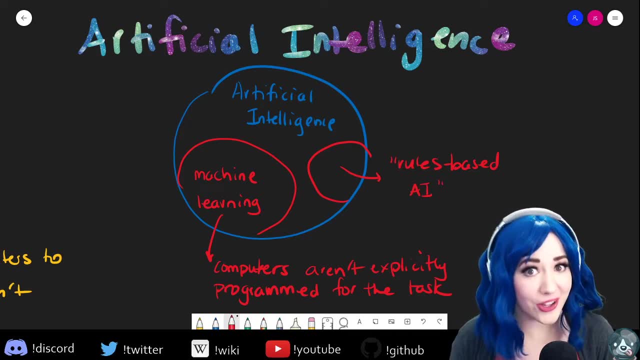 doing called data science fundamentals- um, where i'm covering a broad range of topics all related to to data science um. i've previously done a stream series all on machine learning, so data science fundamentals a little broader. so we've done. let's see the topic of video learning. 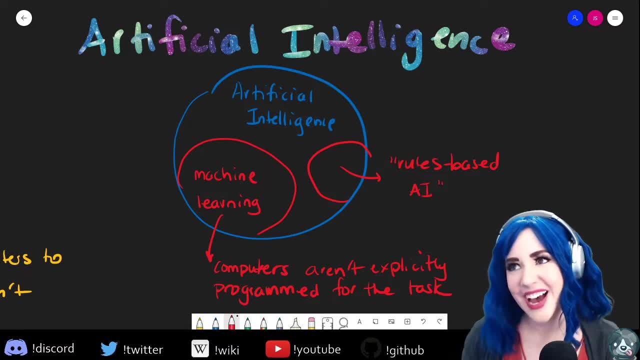 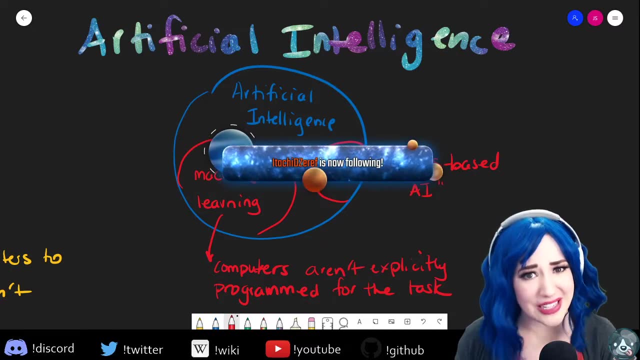 chat, I always forget Exploratory data analysis, dimensionality reduction, scaling, pre-processing your data. But I've gotten a lot of requests for kind of like a help get me started with ML, kind of stream, And so that's what today is, And if you're interested, though, in ML and you want to, 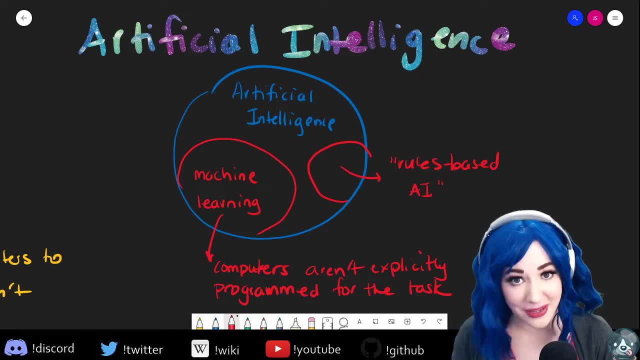 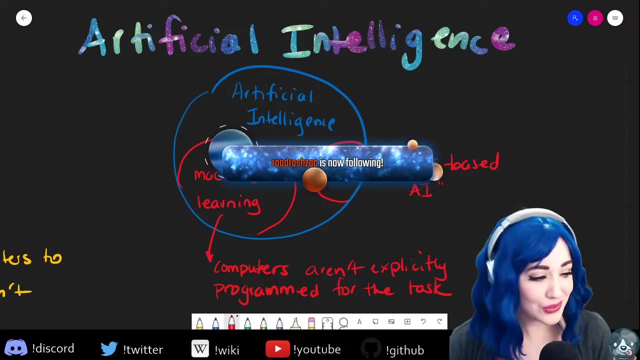 like see what's out there. I would definitely recommend the Machine Learning Mist streams. I cover 12 different topics, all related to machine learning. The code is on GitHub. The VODs are on YouTube, But let's see here: Itachi D Zaref, Road Rash, Zach and Piznaz. 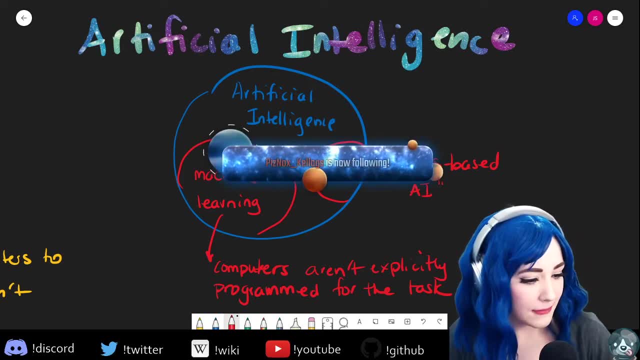 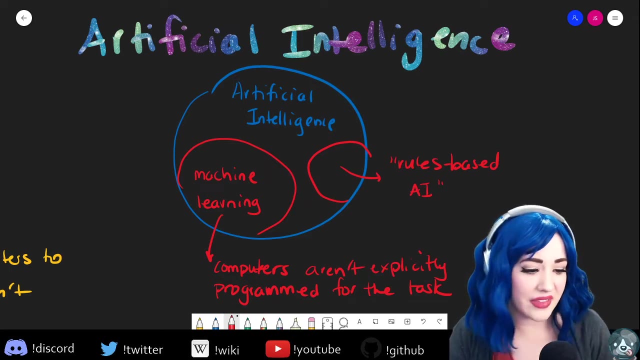 Kellogg's- Thank you so much for following, And Punchy Penguins you. the captions are all in your control, So the caption service that I use is a like a third-party plugin. You can customize it, You can move it wherever you want. I think you can change font size, all of that, So wherever. 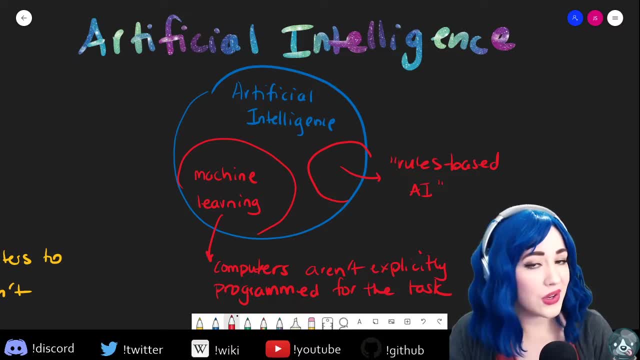 it defaults is wherever it defaults. but you can. you can customize it just for you. And some of you say you're suffering with the gyro of the font. Oh my gosh, I play, so I play. I've played a lot of Switch games that use the gyro. I can't, I can't imagine like. 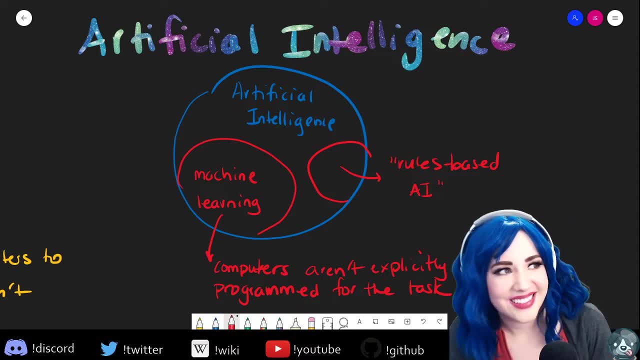 oh so, so cool. Game development is just I don't know. I get, I get hooked and I can't. I can't walk away. And you say you're getting excited to watch this. I'm going to have you on. 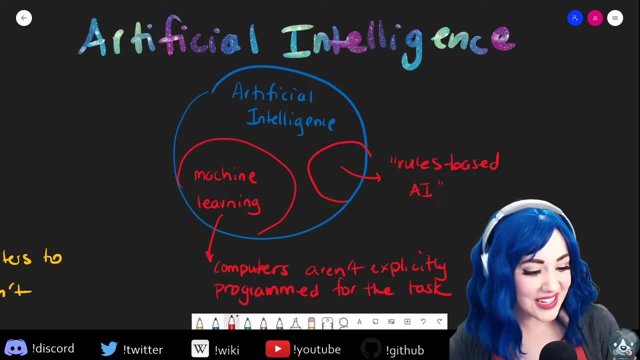 while you start cooking some dinner. Ooh, nice, Cook, cook something delicious. but also, feel free, I know post-it notes are going to be in the chat, I'm going to be in the chat, I'm going to stream. There's always that slump of energy, So feel free to like lurk or like close everything. 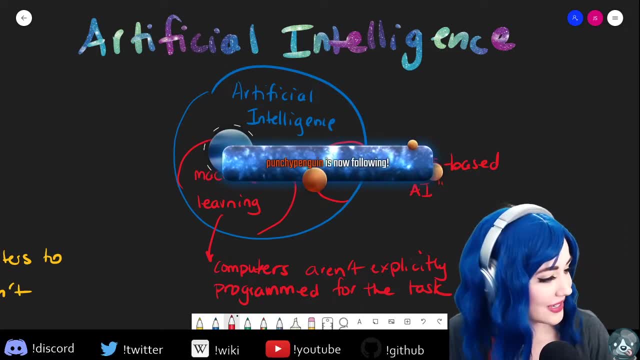 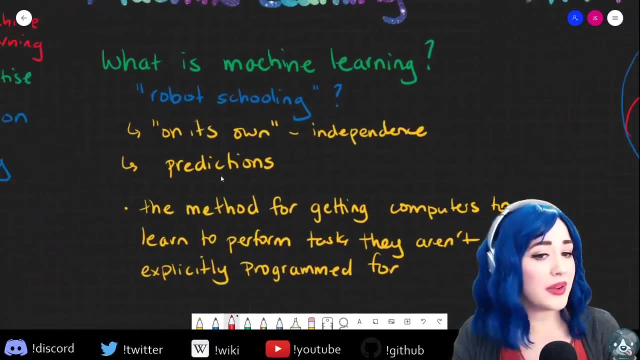 and just relax. Um, I know, after stream I'm usually pretty wiped and punchy penguin. Thank you so much for following. All right, So to catch. catch all of you wonderful Raiders up. all we've really talked about so far. we started out with uh, data science and talked broadly. 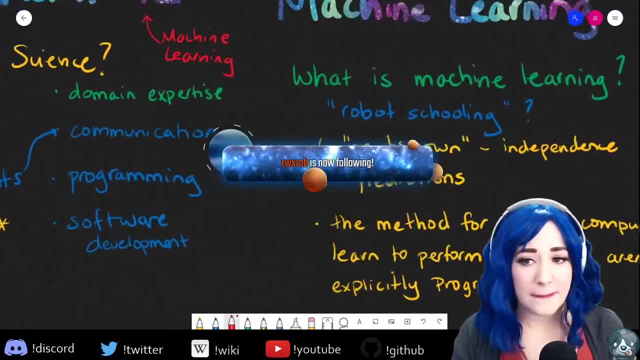 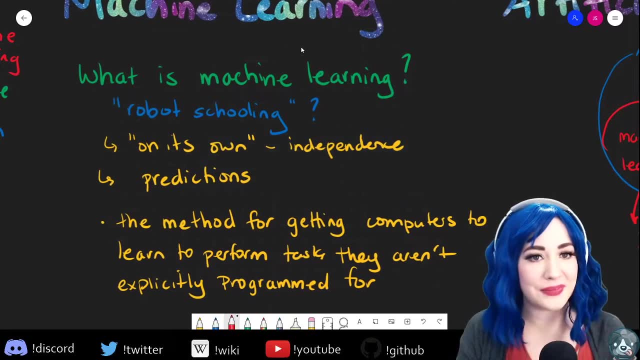 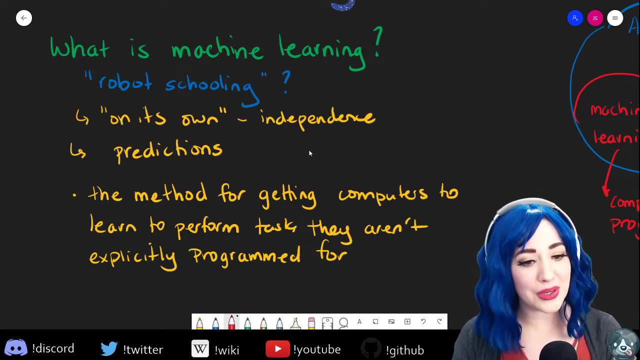 about data science and kind of what it is. Then we were: we were working on a definition for machine learning and RWX- Rob, Thank you so much for for following. And in terms of defining machine learning, what I came up with was: it's a method. First of all, it's a method for getting computers to learn to perform. 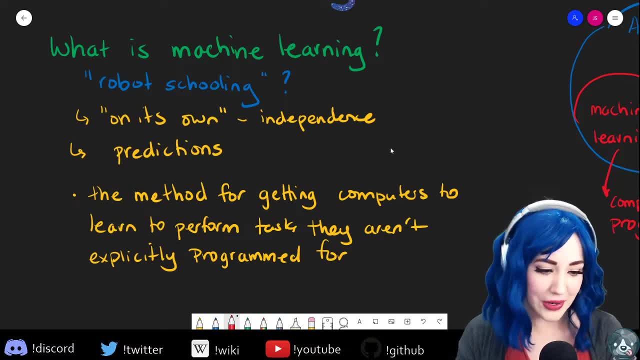 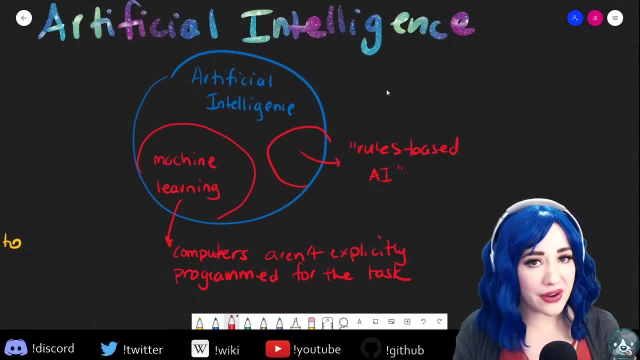 tasks. They aren't explicitly programmed for. now, the not explicitly programmed for part is the really key thing, because in the broader field of artificial intelligence, you can absolutely have something called rules-based AI, And that's what I was talking about. right, When all of you 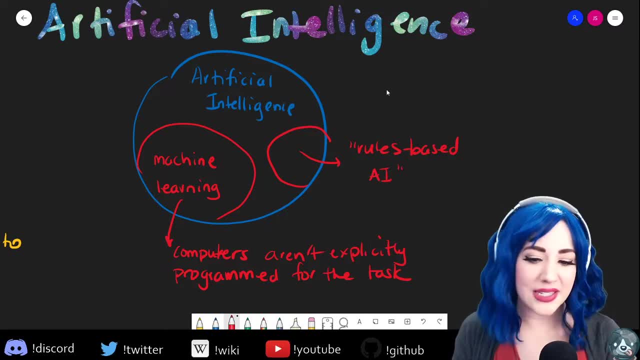 you Raiders showed up Um rules-based AI is is an approach- though It's, it's a valid approach, but sometimes you can imagine it would get really, really tedious, because you'd have to kind of think of every possible scenario that your system would come into contact with And you'd have to exhaustively program all. 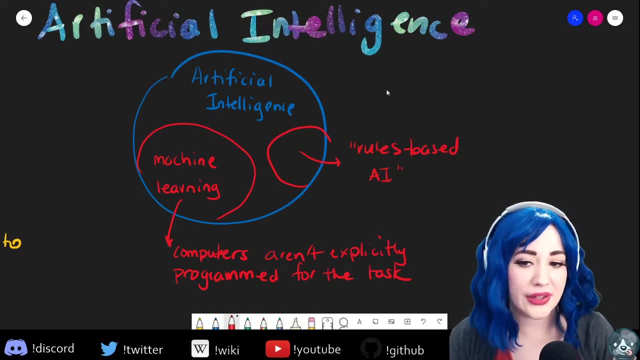 of the different conditionals for what, what that particular um AI would encounter. So, actually in data science or in game development, um, when you, when you hear AI a lot of times, what they're talking about is rules-based AI. So like, how do? 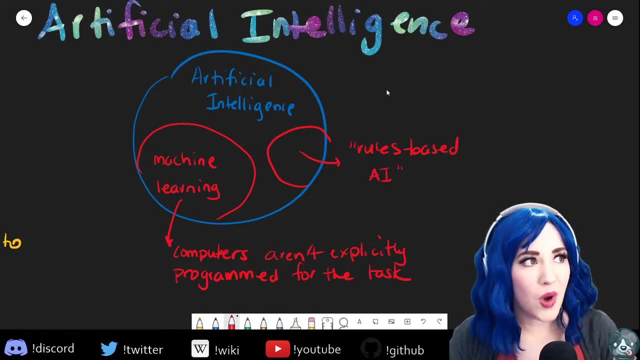 we get NPCs to, like you know, walk around and talk to people and do things, And a lot of times that's based on a series of rules. Now, don't get me wrong. Games are introducing um a lot more machine learning into a wide variety of different applications, But a lot of times when you 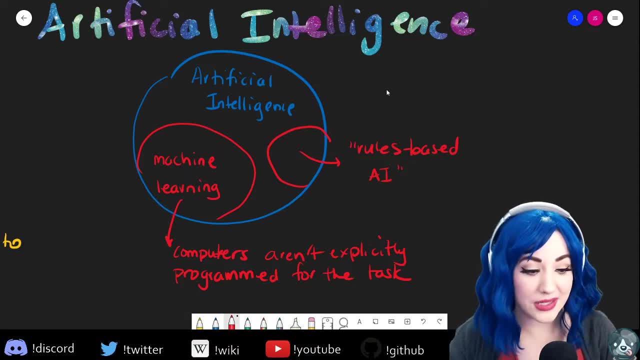 hear game developers talking about an AI, they're talking about rules-based AI. So I really wanted to make this distinction for all of you: that when you hear AI, that doesn't doesn't necessarily mean machine learning. Machine learning is specifically that subfield of AI. 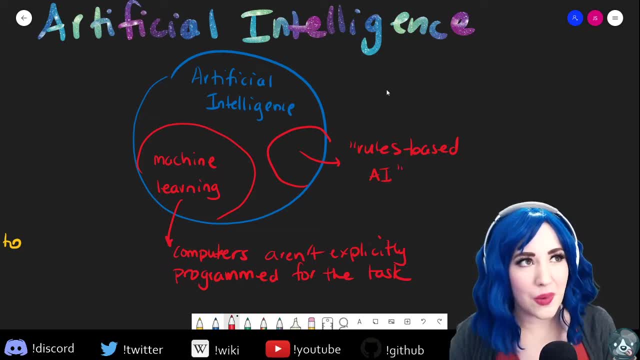 when we want the computer to learn something, We want it to do something that it's not explicitly programmed for. It's not searching through a massive dictionary of like if this, then that It's having to kind of extract generalizations or, you know, general policies that it can follow. 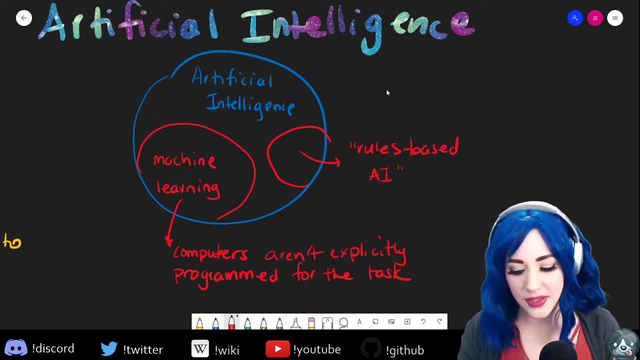 when given completely new situations, And that's really that's kind of one of the things that certain branches of machine learning really aim to do is generalize. So for generalization, that's like if I teach you how to cook a dish, I teach you how to cook. 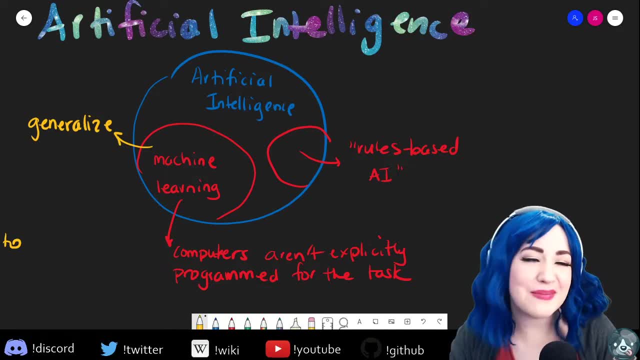 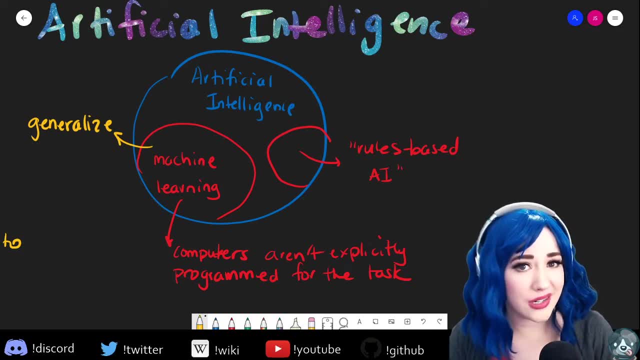 experience that you can do pasta plus sauce plus protein and that will make a meal And maybe there's some nuance there. You got to learn what sauces and pasta types go together or what proteins and sauces go together, But you're learning to generalize principles that you can. 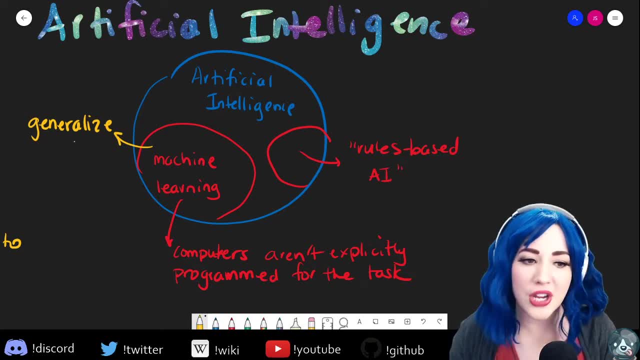 follow when given brand new situations. Generalization and machine learning is the same way. So, while we often have something called training data, where we're trying to teach the model something it's never seen before, because then we're really testing, how well can you? 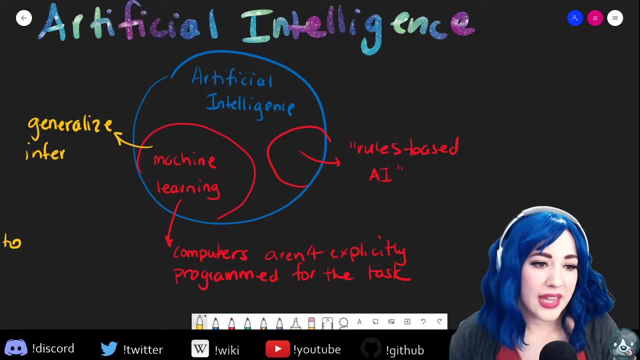 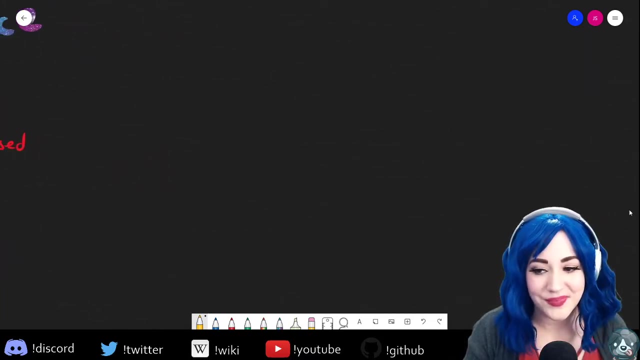 generalize, How well can you infer from what you've learned, How can you kind of apply the things you've learned to something brand new? And that really is what a lot of machine learning is all about. So now in machine learning more broadly, even though I define machine learning as a method, 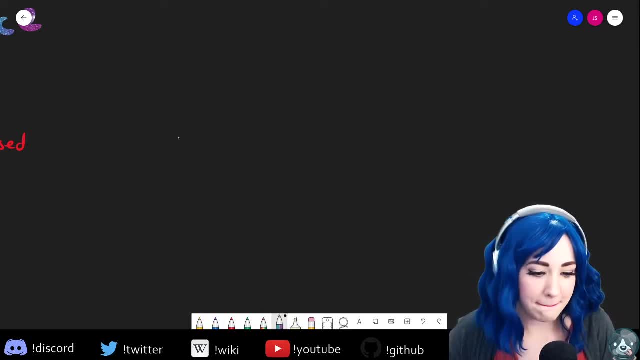 there's like multiple different ways that you can approach machine learning. Throw some cheese into the pasta, Exactly. Well, dairy is a protein. What am I saying? Machine learning? I guess types of machine learning would be a better header here. Types of ML And so machine learning. 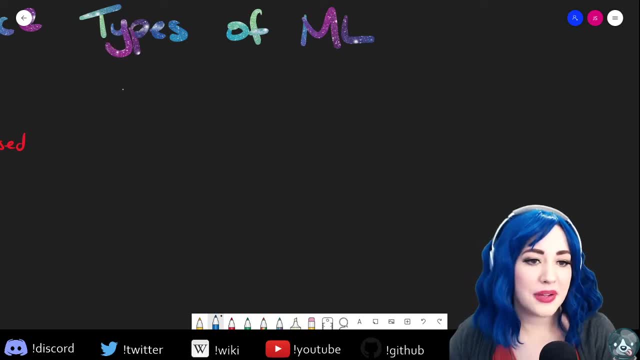 Miss Veterans will kind of already know all of this, But the most common kind of machine learning you often run up against is something called supervised learning, And supervised learning is a little bit of what I was just describing. You have training data, And so this is, let's see, this is where you have examples to teach the model, And by examples here. 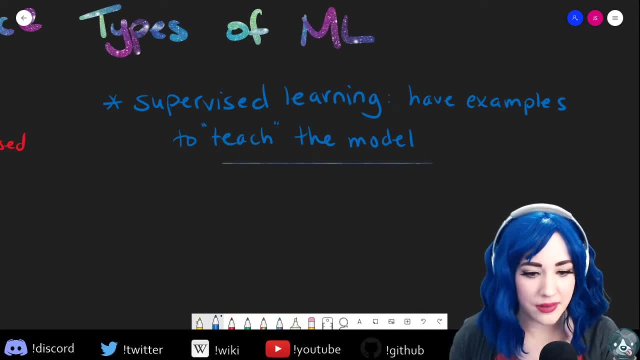 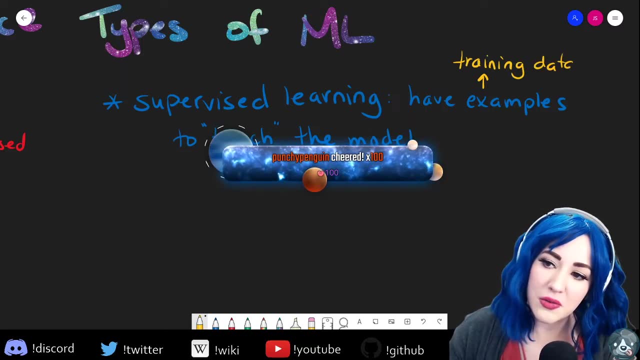 oh no, I wanted a different color. Here we go By examples. I'm talking about your training data. So this is this is what you you train your model with. This is how you're teaching your model And Punchy Penguin. thank you so much for for okay. 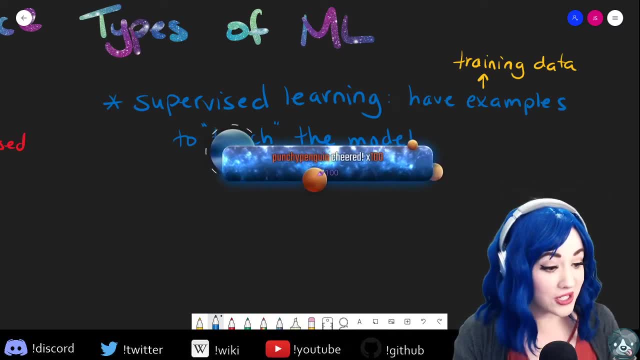 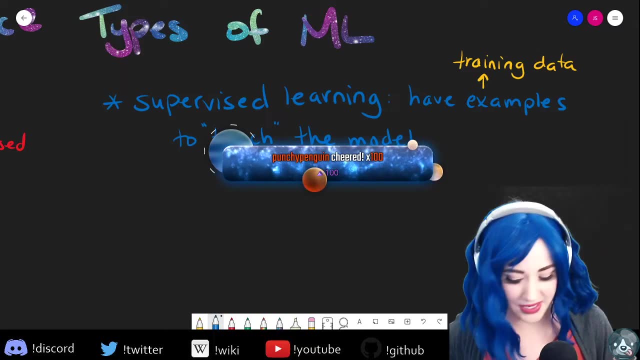 so that gives us one more dog treat, Two more dog treats. Thank you, Punchy Penguin. Okay, we are up to four dog treats, Four whole dog treats. Sweet, I've got my little like scribble scribble note card And I'm keeping track of how many dog treats we have. And 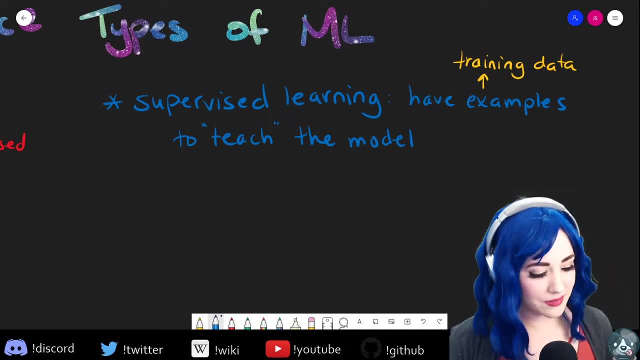 when we hit a good break point, we'll take a break And we'll give the dog some treats. Relax our brains for a minute, One for Hubbell and one for Tennessee. Oh yeah, Um, hell yeah, I get on and find you on. Hi, Lord Azazzle, How are you? Okay, And so supervised learning itself can have. 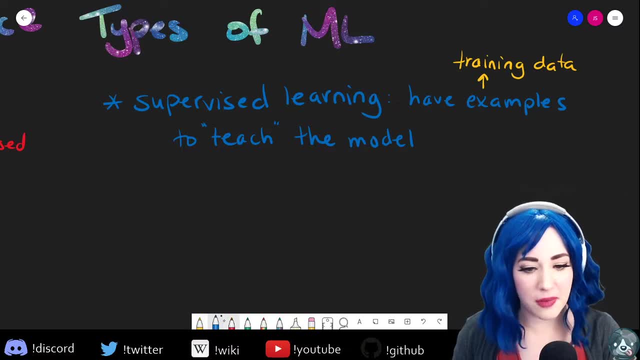 like a lot of different, different approaches and different models. So switch colors again, Let's do light blue. And you Z me. now You ask: what's a model? So a model, in this case, in the supervised learning case. 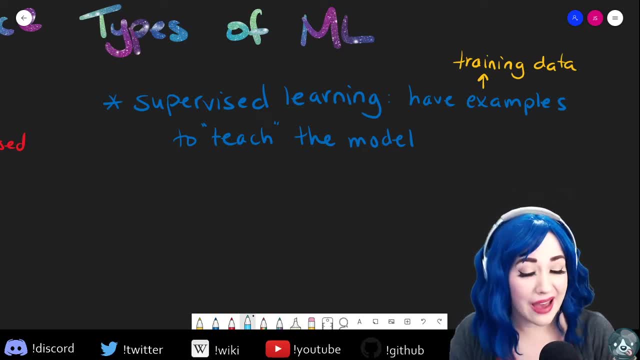 is kind of like an algorithm. It's like- for those of you who were in math, uh, Math Monday last week- it's kind of like a really, really complicated function. So essentially, what you're doing with a lot of supervised learning is you're trying to create, you're trying to explicitly describe the 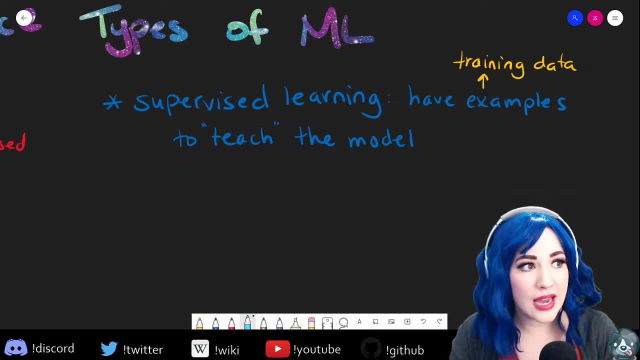 relationship within your training data. So maybe I have, um a whole bunch of pictures of cats and dogs and, um, I have them labeled, So I know which ones are cats and which ones are dogs. And essentially what I'm trying to do is I'm 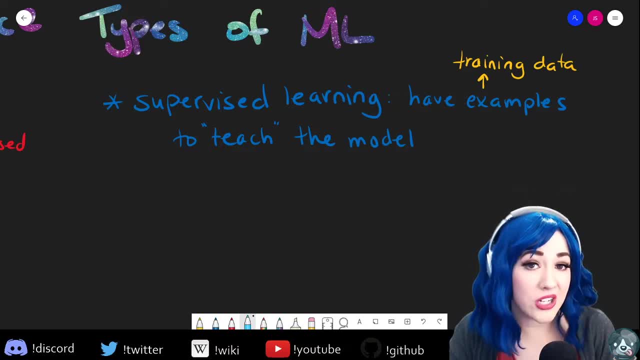 trying to get the, the model, So a really complicated function, in this case, to extract from that the relationship between, whatever I give it, the pictures, and the outcome, which is, uh, a cat or a dog. So actually, let me, let me. 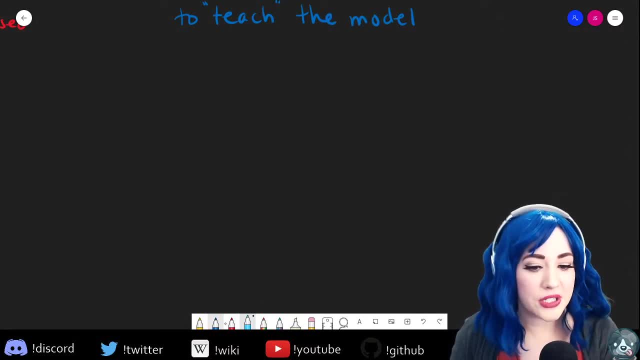 visualize that for you. So there is a key difference, which is that when we're talking about functions, like when you learn functions in algebra, right, You learn, okay, here's your function And what happens. Your function has rules, right, And you input some data and you 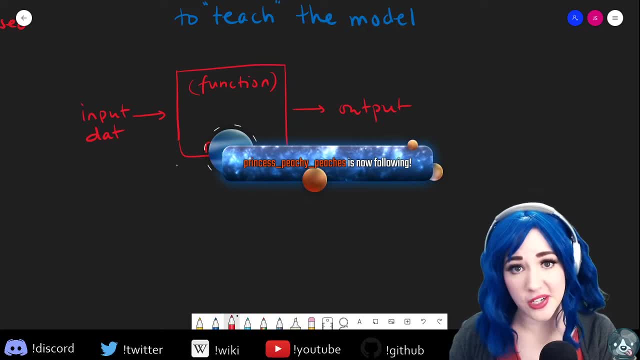 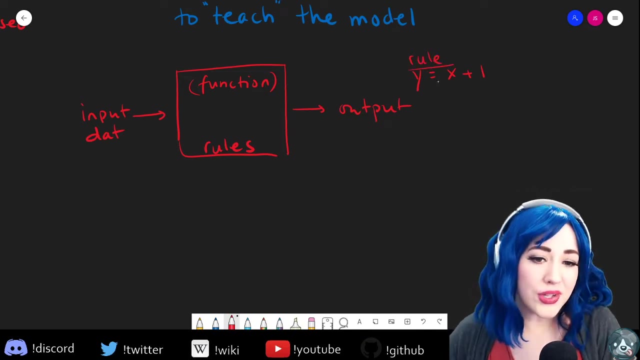 get an output according to the rules of the function, right? So even if it's something as y equals x plus one, that's describing a rule. So I'm saying, when I give you an input, add one to it and that's the output. So in this case, this is our rule And it's a rule It's also establishing. 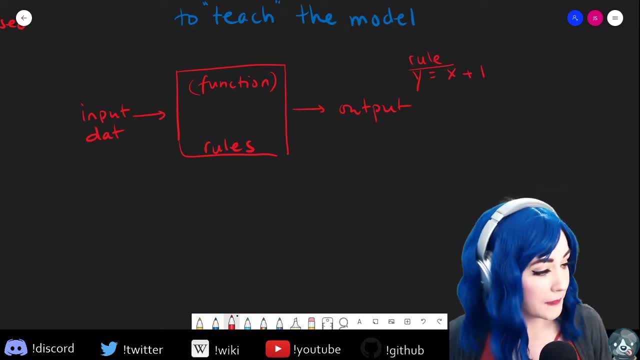 a relationship, how our x's are related to the y's. And Princess Peachy, Peaches, welcome. welcome to Science Sunday. Thank you for following Now with a machine learning model. it's a little bit different, because here's, here's our machine. 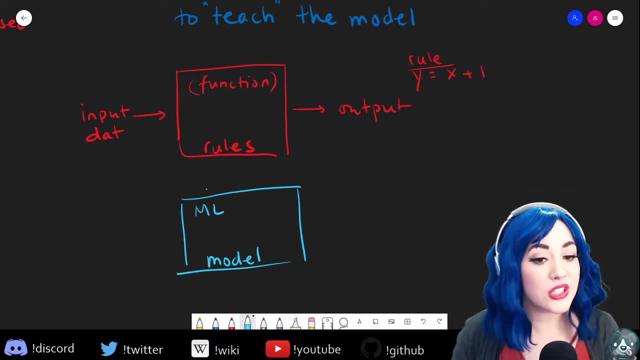 learning model And in the case of supervised, so I'll put SL up here. In the case of a supervised learning machine learning model, what we're doing is we give it that input, a new put input data- No one saw that- And we give it. we give it the outputs too, the expected outputs, And what does? 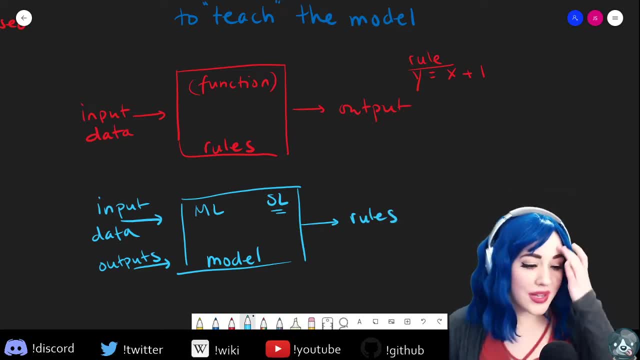 it spit out. It spits out the rules. So it's similar to a function, but it's also a rule. So we're kind of expecting something different, at least in the supervised learning case. And let's see, as we say, model, is you so good looking? Well, that's a different kind of model. 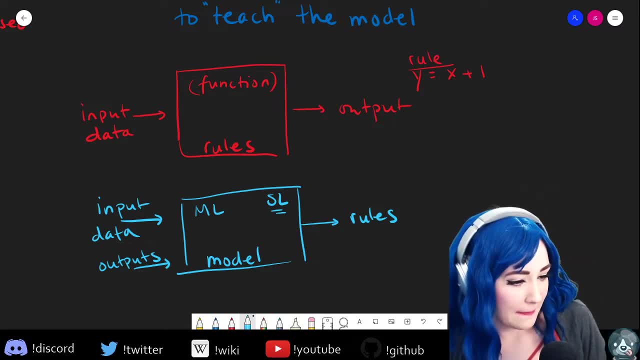 that I know nothing about. trust me. And machine input into machine output. Yeah, so you can think of, you know input, you define rules and an output as being our conventional functions. But let's see Tijuana. you say creating neural nets. I backtracked to the extent of learning. 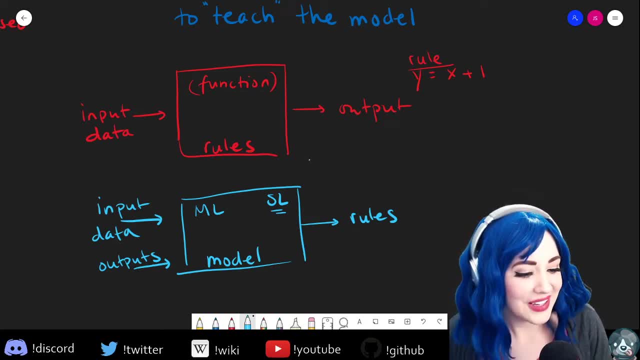 green alphabets to understand calculus and algebra. but I don't know how to do that. How do I do that? That's to understand calculus behind it. That was so wrong, Oh, no, Okay, Well, well, I always feel. 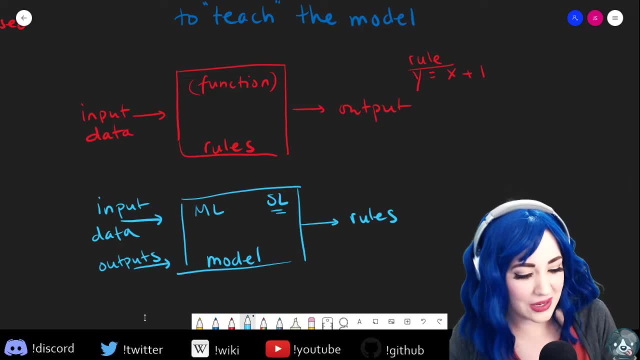 like I always like to give a shameless plug and then I realized like this is my stream, So I should be able to shamelessly plug my own stream, right? I would definitely recommend Tijuana you check out YouTube. In the machine learning mists streams. I do an intro to neural. 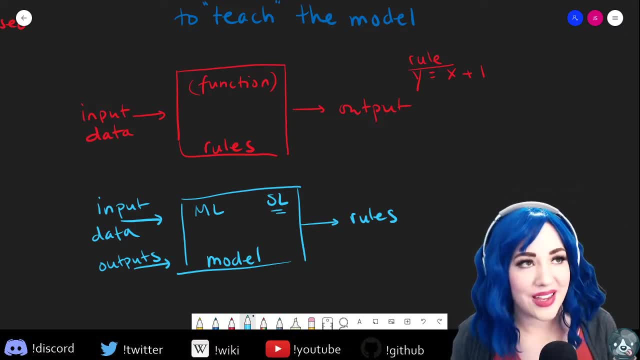 nets and we take it from the very, very beginning And we don't use, like Keras, TensorFlow, anything but we build a multi-layer perceptron neural net from scratch. so we do all the code, so nothing is like wrapped around. you know, charis, dot, whatever, nn dot layer or whatever it is. you know, it's all, it's all from. 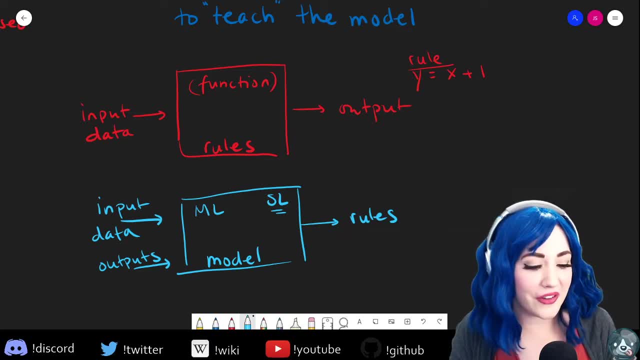 scratch. so if you're interested in kind of getting a feel for for neural nets, i feel like that video is really successful. so hopefully, hopefully it's useful for you. okay, so hopefully this also helps with um. let's see, using me now. hopefully this answers your question about what a machine. 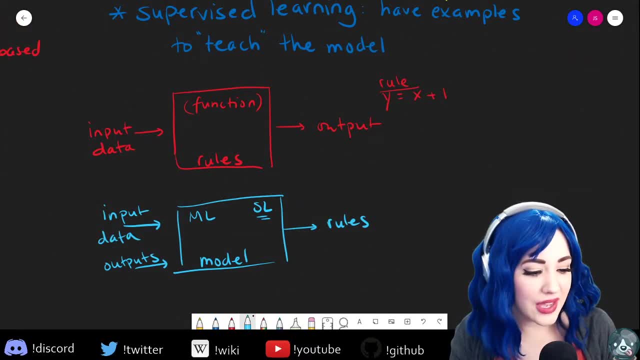 learning machine learning model does so. it is kind of like a function with a little bit of a twist. that really what we're interested is. we're interested in these rules that hopefully, if we did our job right, we can then apply to brand new data that the model's never seen. but to keep 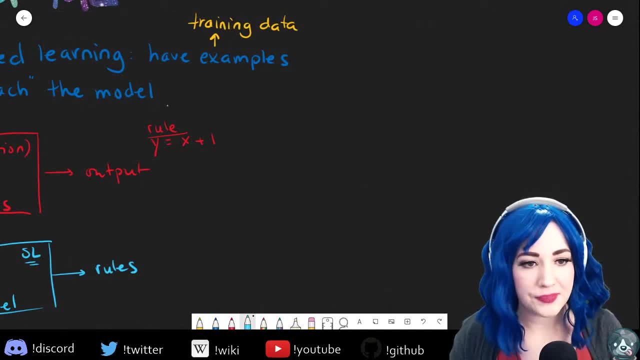 talking about supervised learning for a sec here. there's lots of different kinds of supervised learning. so if you, my, my, my mlness, folks who are in chat, tell me, tell me some supervised learning approaches that you're familiar with, or anyone honestly. but we did, we did two days of two or three days of supervised learning. so 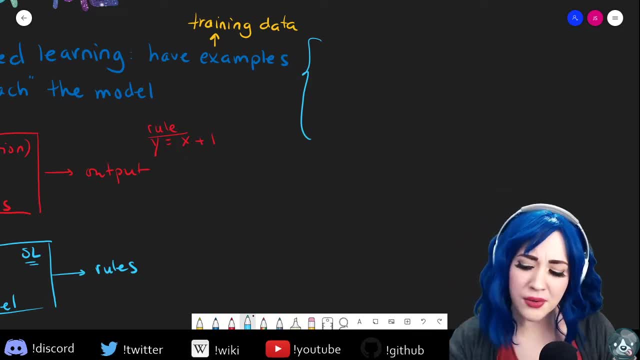 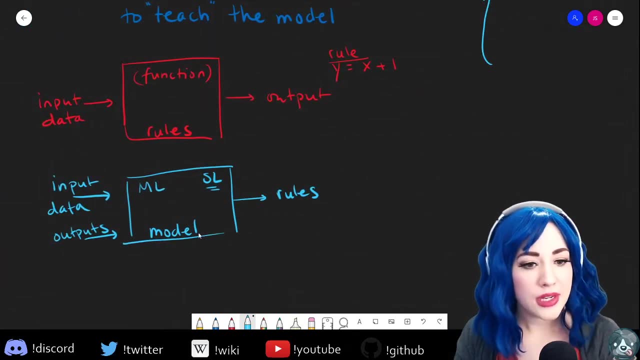 lord is, as you say, this acts exactly like a function, but with more code, more complex rules. not quite so. this is the thing that's really interesting about this is that a function we specify the rules to get a certain output. so in this case, the output is unknown and what we're really hoping to get is that output. 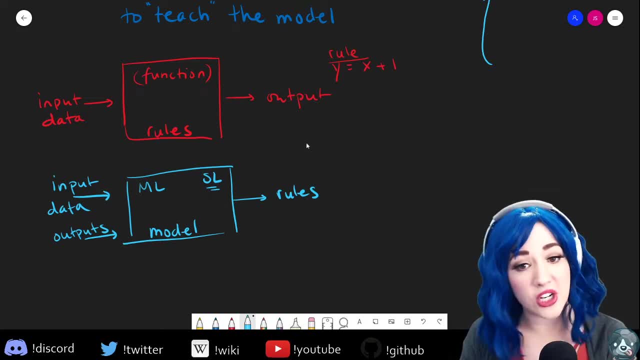 so we specify the input, data and the rules and the function gives us an output. in the machine learning case, we know the input, we know the output, we don't know the rules. so really, what we're trying to get out of a machine learning model are the rules. eventually, once the machine 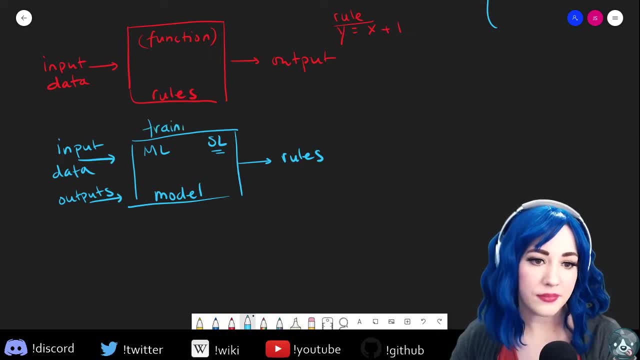 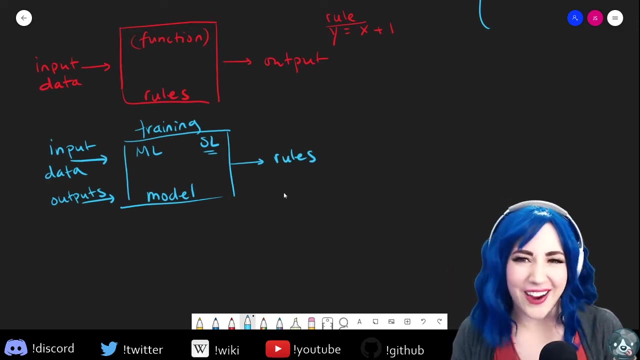 learning model. I should have specified, probably, that this is training. the goal is eventually be able to feed this any kind of data, data it's never seen before- and get the outputs that we don't know. a truth affects another truth to produce another truth. yeah, okay, I could kind of see that applying. 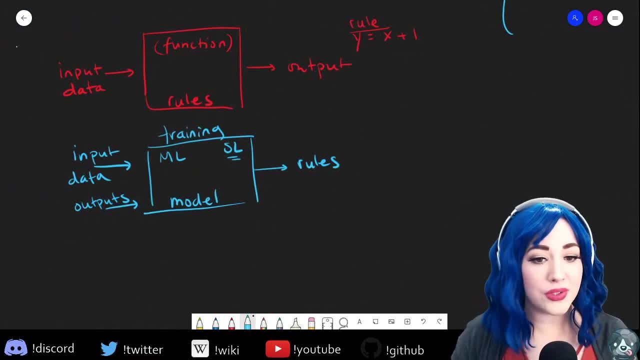 no worries, Lord Azazel, this is only the supervised learning models, so there's plenty of different cases where we actually don't know the outputs and we're still trying to like muddle along. but at least for supervised learning, which is what we're talking about now, yes, we have the outputs. 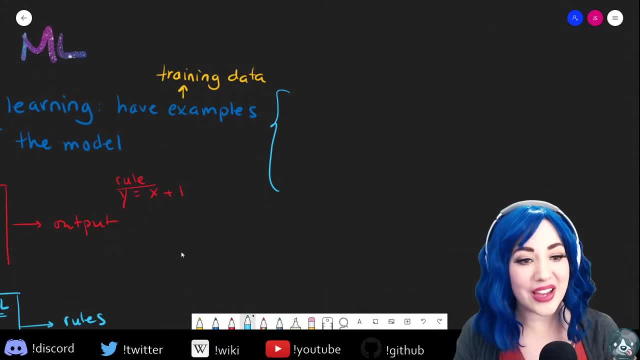 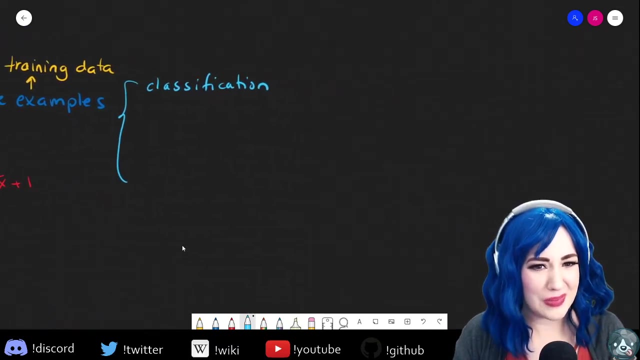 and no worries, no worries at all. okay, so different kinds of supervised learning. so we might have classification, which is what we're gonna be talking about today, which it kind of just means what the word means. you're trying to take something and give it a class, give it a label, but the 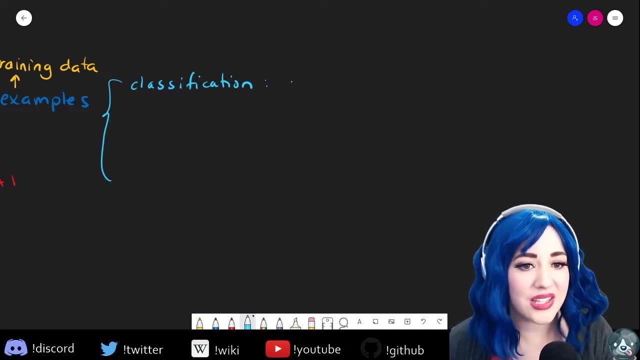 key thing here, as we talk about the rest of the examples of supervised learning, is that classification is trying to classify our data into categories. so this might be, um, like my example with the cats and the dogs images. we're trying to classify images there. we're trying to say here's: 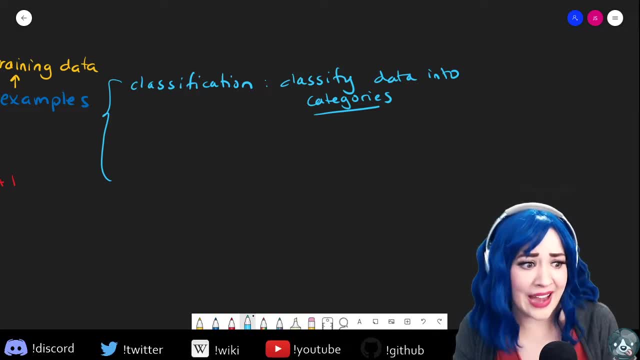 your input. this image now give me out a category: cat or dog. another kind of supervised learning is regression, and this is where, instead of classifying something into like a discrete category- so it's like a separate category like cat, dog, colors- um, in this case, we're trying to predict a value, a continuous value. 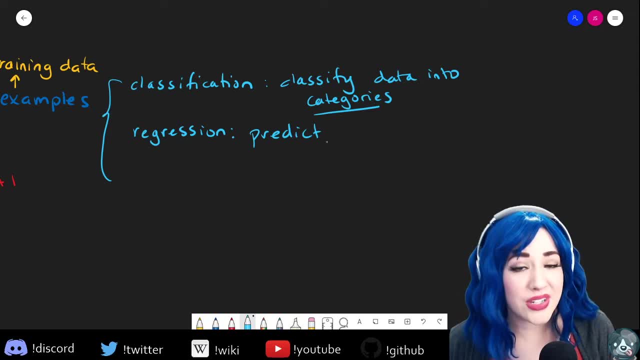 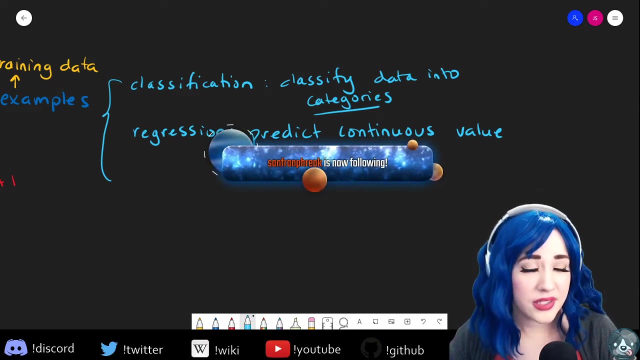 so that might be a price of something. it might be the temperature outside and continues. so one example that might help thinking about the difference between classification and regression is when it comes to predicting the weather. so I could try to predict whether or not something will be cloudy, sunny, rainy or snowy. that's a classification problem. I'm trying to predict. 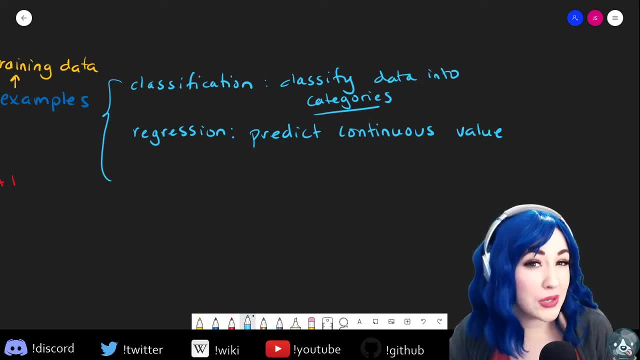 the category of the weather. but if I'm trying to predict the temperature, which is a number that could range in a wide range of different numbers, that's a continuous value. I'm trying to do a regression model. and San Fran freak, thank you so much for following. and hi b4141, how are you? 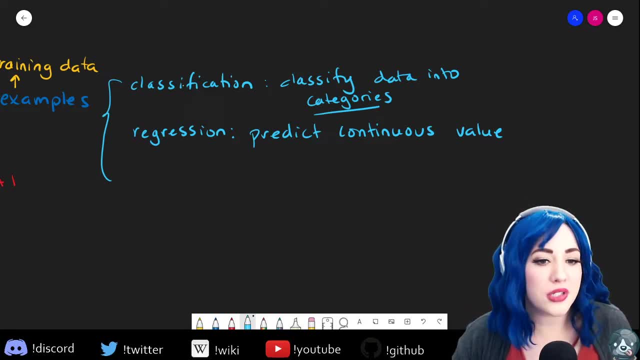 okay, um, some other. these are the two most common, two most common kinds of supervised learning that you're going to run into. but there's a few others, and so I thought I would just like talk about that a little bit. one is similarity, similarity learning, and this is where we're trying to figure out. 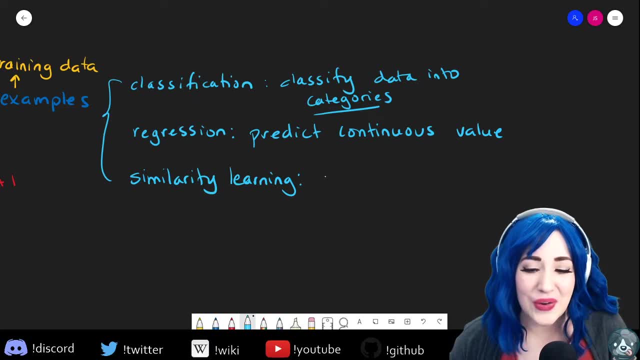 um, well, similarity. so using a given metric, we're trying to classify kind of, but you also are using continuous values, so it's not quite regression. we're trying to figure out the similarity between data. so this is actually something that can be used a lot with recommendation systems. 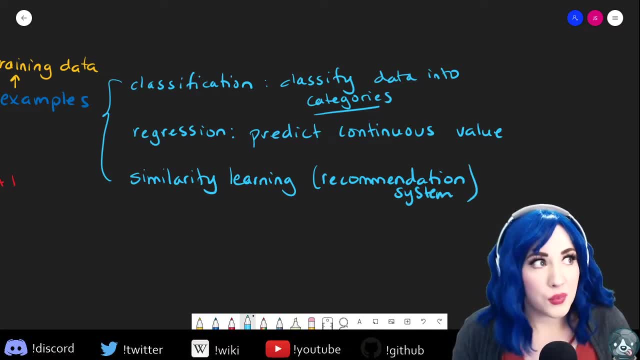 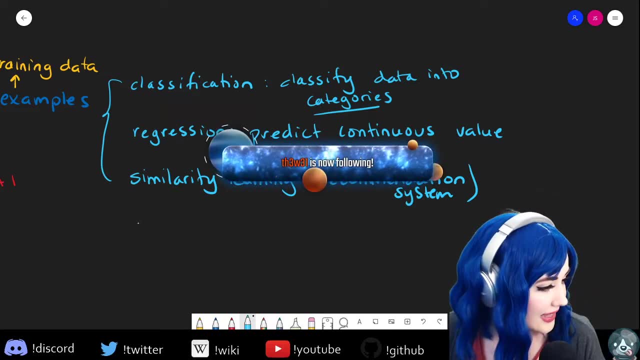 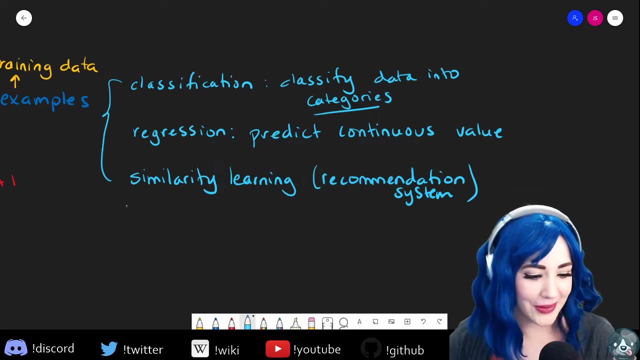 so you know, because I've watched these four shows on Netflix, what is another show that I might like to consider? you know being a regular student or a regular student, but is this something that applies to a person with a really high related learning problem, which I'm sure you're familiar with? so, really, this, this is probably 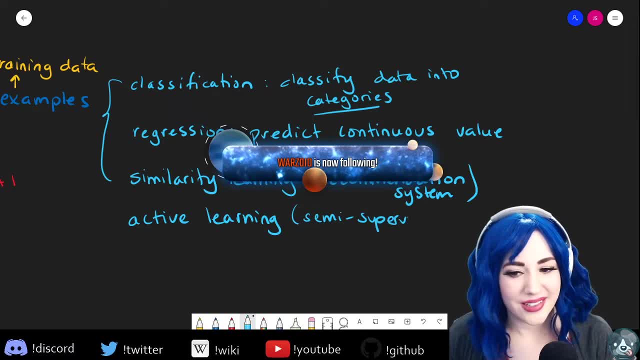 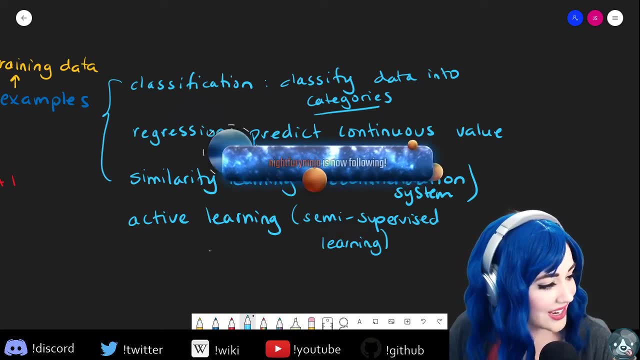 something that you're familiar with in a variety of areas. I'm going to try to find it for you, right? It's a little weird. It's a weird friend. It's the awkward, awkward person in the room. Night Fury Ninja and Warzoid. Thank you so much for following. 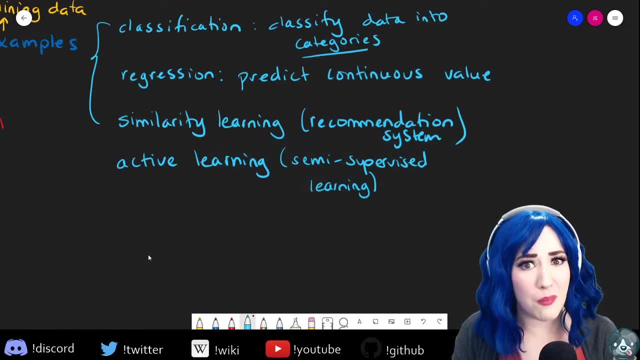 Active learning is where we actually let the model decide what it wants to train on. And so let's say we have a whole bunch of data where we don't have the labels, We don't know the outputs Well, but we know that we can probably get outputs for a handful of the data points. 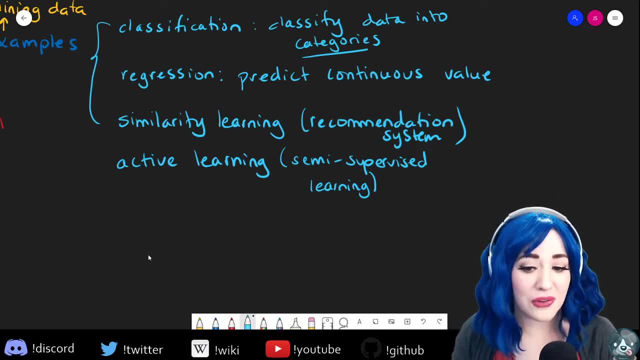 So what active learning aims to do is it aims to have the model tell you what the most important data points are to get a classification for, Or you know the output, the label, And so in that case it's actually querying the human beings. 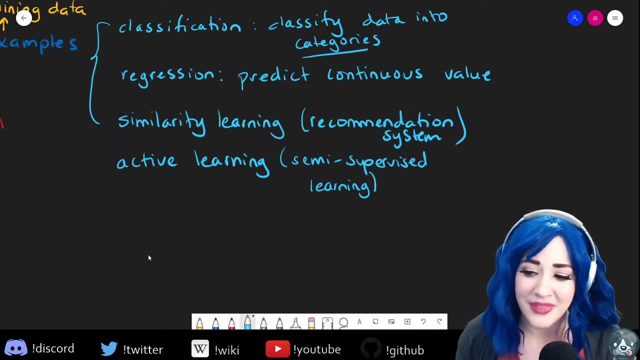 It's saying: OK, of this data you gave me, here is the most important set of data that I need you to tell me The answers for so I can learn to predict the answers for the rest of it, And that is active learning, Really really cool. But definitely it's like kind of unsupervised, kind of supervised, a little bit different. 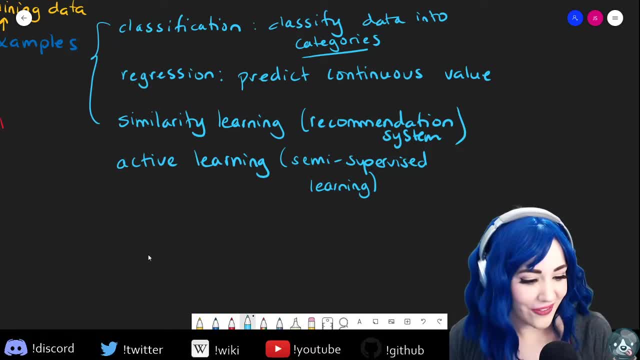 The Llama Legion. Thank you so much for following. OK, let's see, Lord Azazel now could you use this to find an origin point of an anomaly within a closed system? Would this be applicable in a chaotic setting? So I think I would need to know a little bit more. 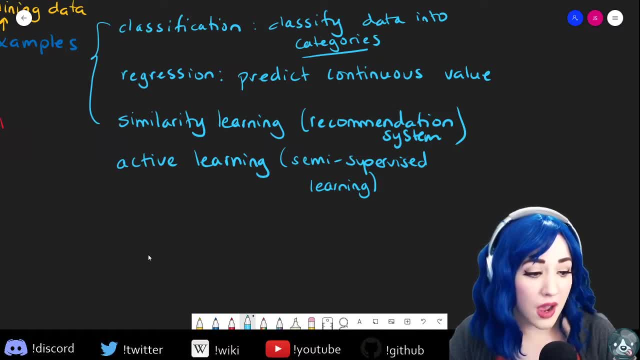 A little bit more about what you're talking about. But anomalies are absolutely origin point of an anomaly. So so it sounds to me like what you're talking about is more of like like kinematics, Right, So it sounds like the origin point of an anomaly, like the anomaly is moving or it's changing. 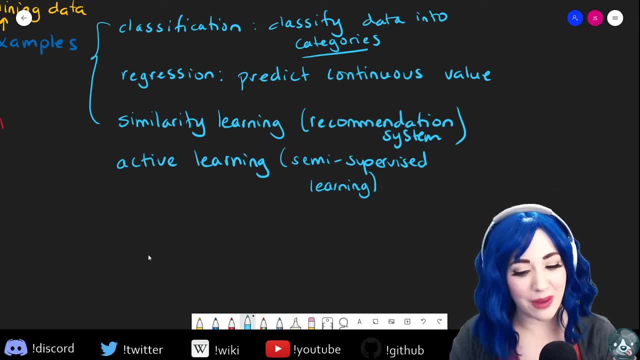 So you absolutely like can make predictions. You can kind of like backtrack to previous states. But lots of machine learning deals with situations where things aren't quite how you describe closed. So this is where you know human behavior is one of those. 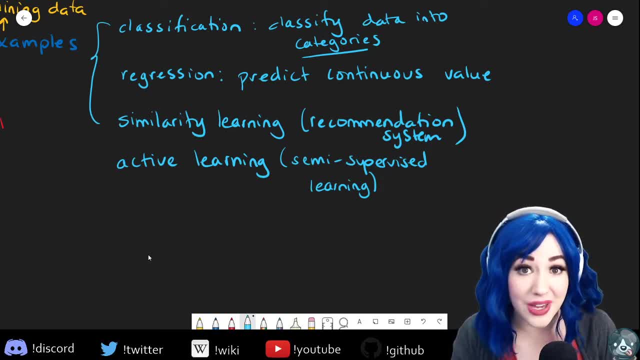 So a lot of the work that I do with video game data is a lot like this. So it's what we call stochastic means kind of like it's got some randomness in there, almost like if we were to make. we have like a data set of 100 things. 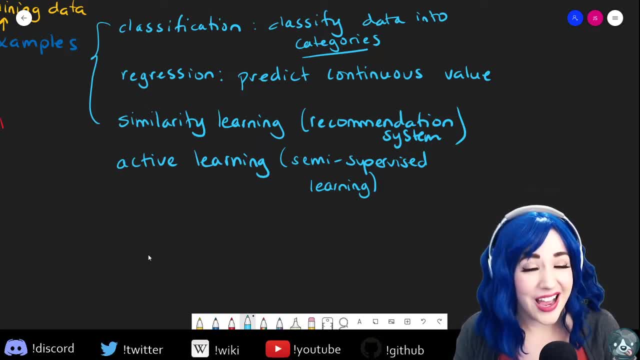 And if I were to fit the model 10 different times to that data? a model that's stochastic would predict something slightly different each of those 10 times. It's not going to be Deterministic, So the inputs aren't going to 100 percent always result in the same output every time. 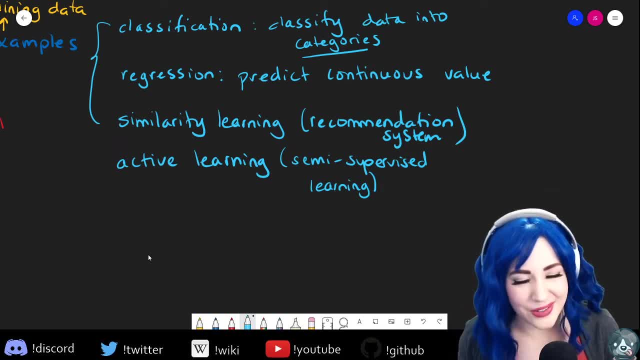 But those models, while they sound like like, well, that doesn't sound consistent. but when you're dealing with human behavior, human behavior is funky, It's random. It's not like you're predicting something as easy as, like you know, an apple falling onto the head of Newton which follows, you know, explicit laws of physics. 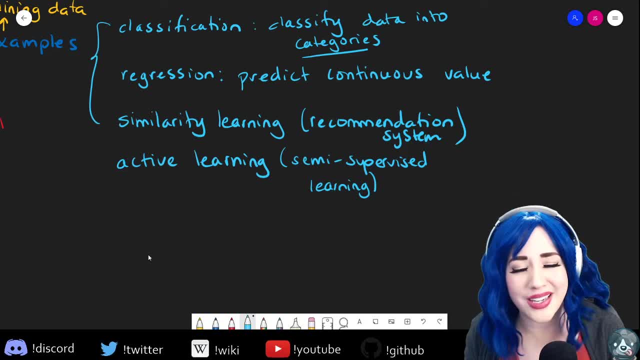 In this case, human behavior is funky and weird, and people do really unexpected stuff that can be really hard to predict, And so that kind of chaotic environment is definitely a challenge, but it's something that there are specific machine learning approaches to handle. And, Baha Asher, thank you so much for following. 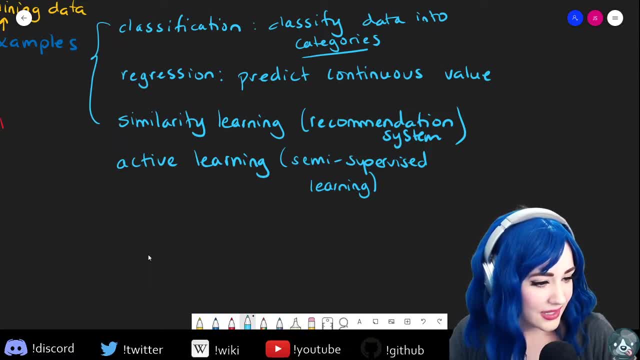 Welcome, Welcome to stream. And let's see yo. is that a penguin? I think it is a penguin and it's a cute penguin punchy. And let's see, here I am, Ben. You say learning C-sharp to make a game. 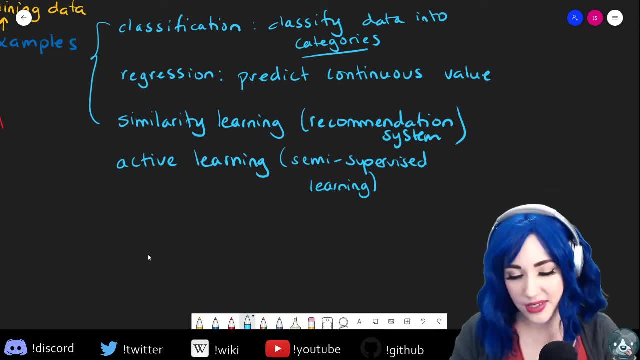 Is this applicable For like CPU players? So I'm actually learning C-sharp and unity to make to make games. So in this case you can apply machine learning to video games in a whole bunch of different ways. So, whether or not you're interested in like player performance, you can use supervised learning to make predictions about how players might might act. 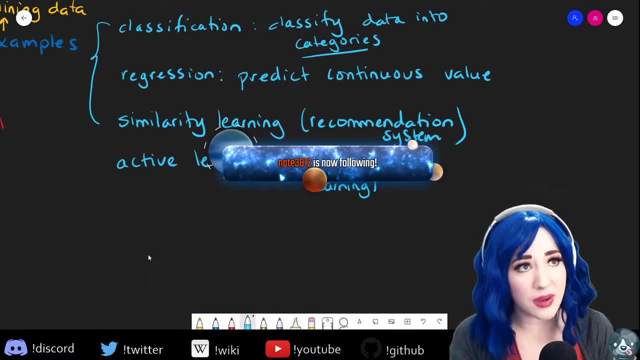 You can also use unsupervised learning techniques, which we haven't talked about yet, to class it like, create clusters of different kinds of players Or different kinds of approaches. You can also, you know, use reinforcement learning, which we also haven't talked about yet, to have a system that actually learns from the player and adapts to what the player does. 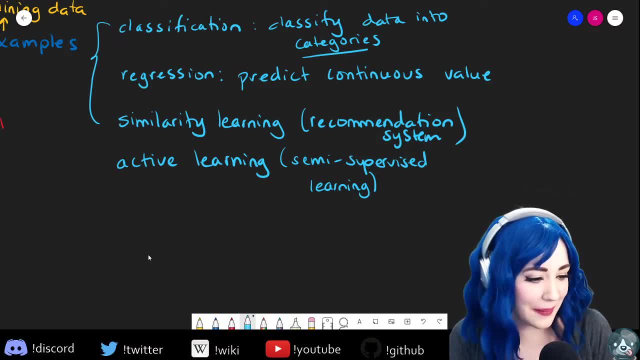 And Nate3812,. thank you so much for following. Okay, And let's see. You say you're interested in this for malware, cybersecurity, research processes or purposes. Yes, Lord Azazel, So for cybersecurity specifically, there are a lot of challenges. 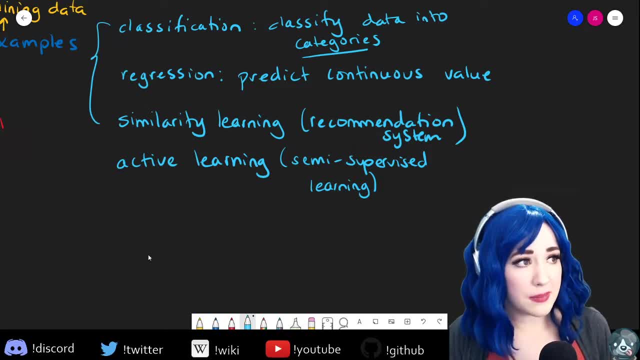 Typically your data is very high Volume. typically the- the things that you're interested in fitting for, the things that you're interested in analyzing and identifying- have low incidence, meaning they don't occur that often, They're rare but they're high impact. 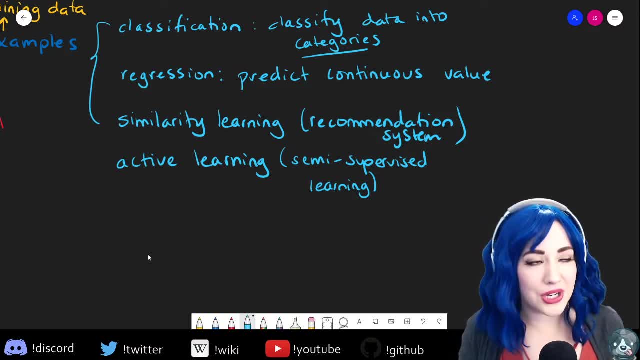 So, like you know, your most catastrophic cybersecurity threat is going to be something that is super, super rare, but absolutely devastating and takes everything down. So there are lots of different ways to handle that. with machine learning- One of the biggest problems in applying- 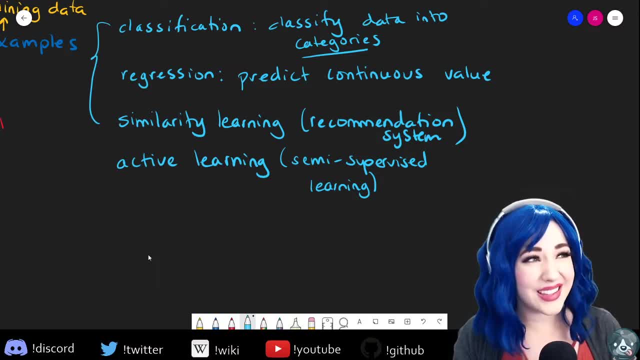 Machine learning to cybersecurity is that there aren't a lot of labeled data sets, so you're really kind of restricted, You. you almost have to have unsupervised learning. And again, just like I said earlier, cybersecurity is dealing with human behavior, so you're always going to have a tough time whenever you're trying to model human behavior and make predictions based on it. 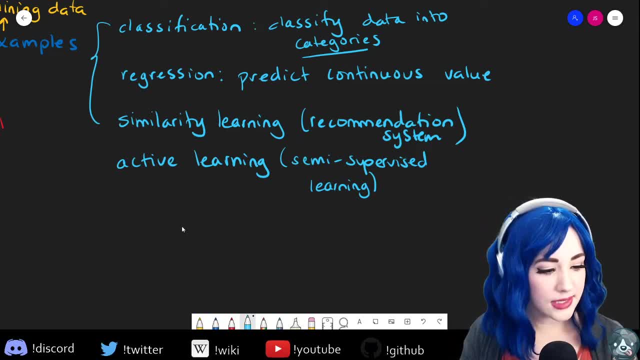 Okay, so let's see here What's that speech to text. Um, it is. Let me give you a link. I'm testing it out. It seems to be very reliable, But this is the captioning. Ignore that backslash. 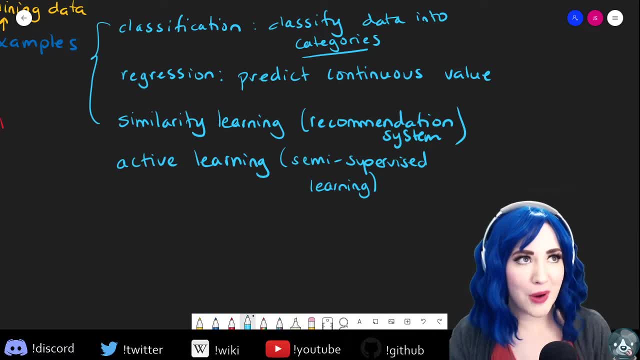 Sorry, But that is the captioning third party Thing that I use. And the llama legion, you say might be a tangent, but is it fair to summarize: a machine learning engineer just as a software engineer but deploys machine learning models to production? 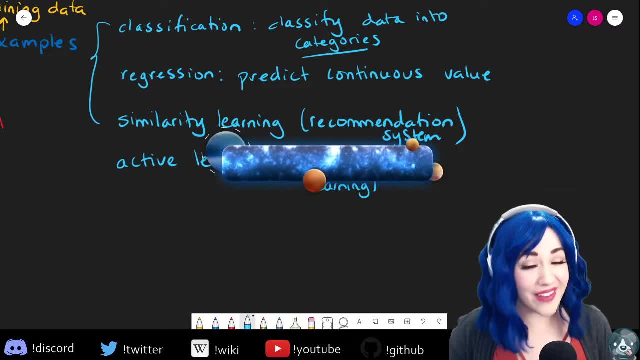 No, And here's why: Because I've actually been in Situations where I've worked alongside software engineers who, if I give them a model to deploy, they know how to do it, But do they know which model to use, if their models have outcomes they don't expect? 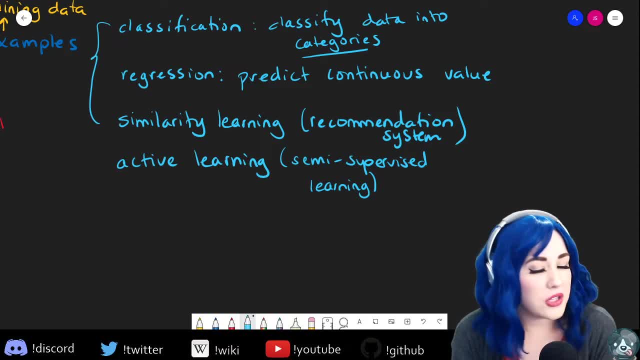 Do they know how to tune? Do they know how to evaluate the, the output of their model? Do they know how to, you know, clean the data? or, you know, generate features? or, when things are breaking, Do they know how to fix them? 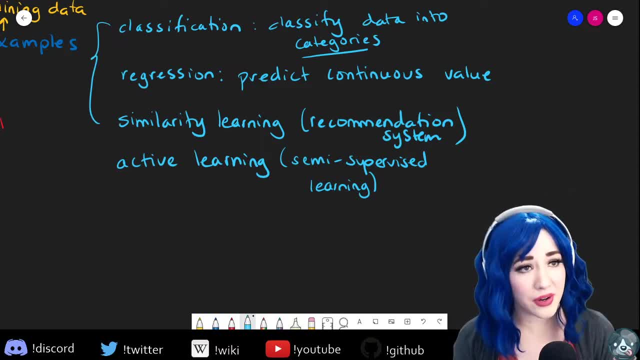 Not always So for me. I'm more of like the machine learning engineer. I'm always trying to improve my software development skills, But really my strength is that I can absolutely contribute to like software development and I can build things alongside a software team. 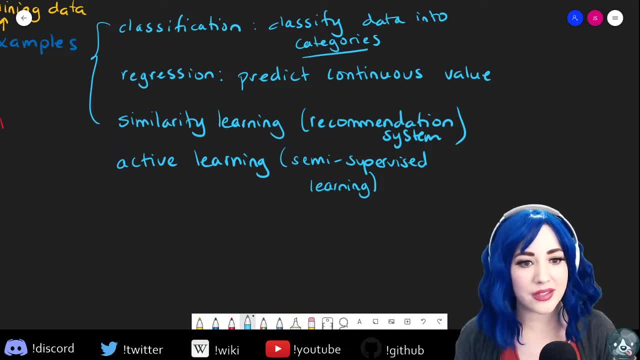 But really I'm usually put on projects because they need a machine learning model And, apart from the basics, they're like either: Hey, like we're using this model, Why isn't working? like they can deploy it, They can you know. 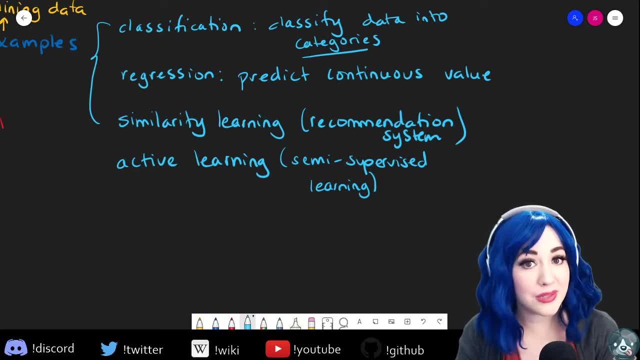 Have that whole wonderful pipeline. that makes things run really smooth. But when it comes to really understanding what's going on- like tuning the layers, sizes, parameters of a deep neural net- they're going to know how best to turn that into software. 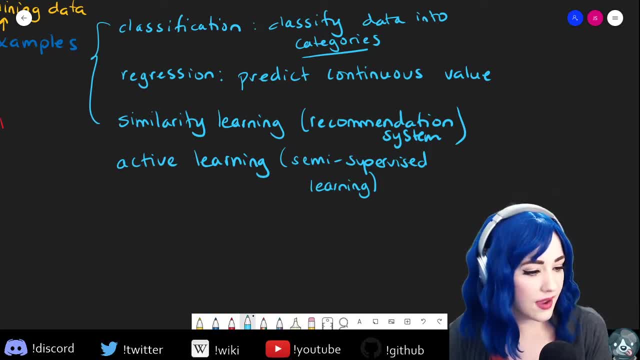 But they're not going to know how best to build the model Punchy Penguin. thank you so much for subscribing. Oh my goodness, Thank you, Thank you so much, Thank you, Thank you. That that means a lot for those of you who are new to. 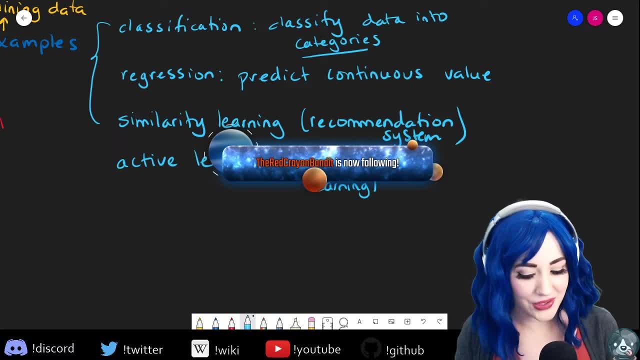 And I see lots of new wonderful people. But those of you who are new to stream all of my stuff as free. all the code is on GitHub. All the notes are free. Fads are on YouTube. I can't control YouTube ads. 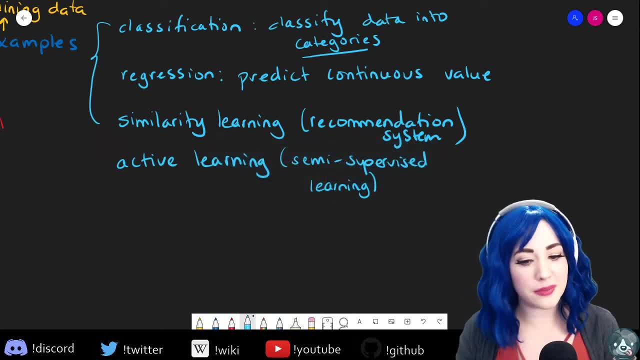 I'm sorry, But I try as much as possible to make all of this free. If you want to join Discord, I'm always available answering questions, helping people with their resumes, all of this stuff I do completely just for the community. so when you do subscribe, it means a lot. but also don't feel pressured. um, and let's see, I am Benny. 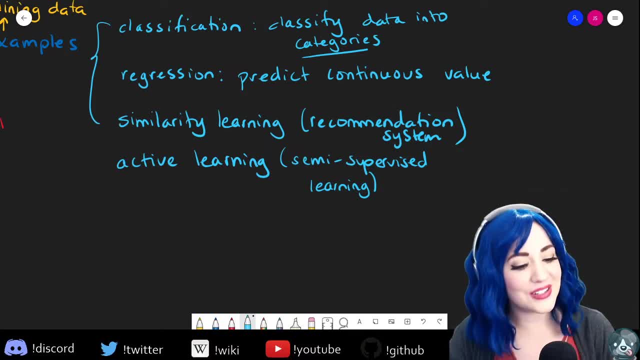 so you feel like you need subtitles, not for what I'm saying, but to dumb it down to your understanding. no, and if I'm talking too fast, please let me know. when I get really excited, I can talk too fast and I have to remember to take a breath. um, okay, so let's see here. oh, and thank you, punchy penguin. 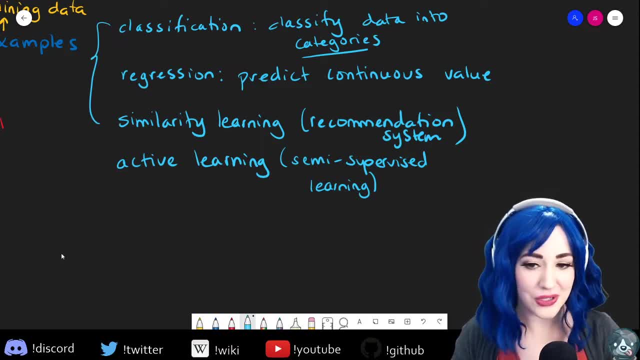 I'm glad. I'm glad you're enjoying it. hopefully you'll check out some of the other stuff on YouTube. um, I realized when I first started streaming science and tech, I guess we're coming up on a year of me exclusively streaming more science and tech. um, previous to that, I was 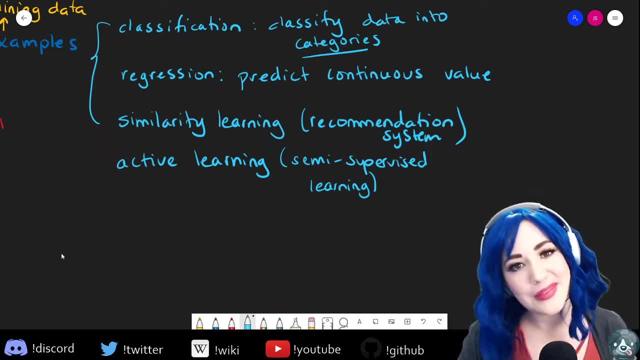 like just streaming for like five people and playing video games, but um, I I didn't even think to save the VODs. like I did this great stream that was um the the math behind special relationships. and I did this great stream that was um the the math behind special relationships. 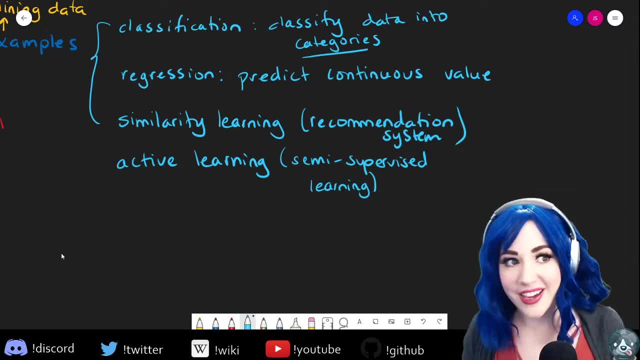 and we did a proof of it and I've done streams all about like intro to black holes and things like that, because in a past life I was an astrophysicist and I should have saved the VODs. so now I've learned and everything's on YouTube, but had to- had, I guess, learn from learn. 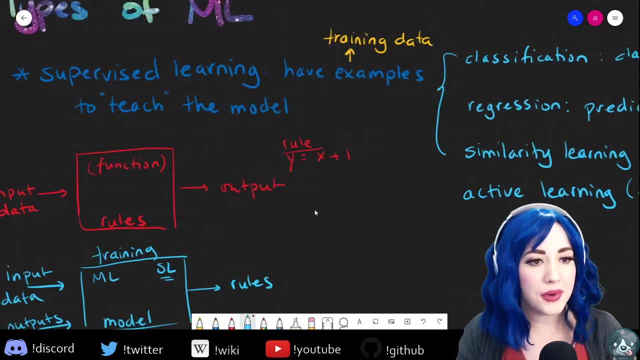 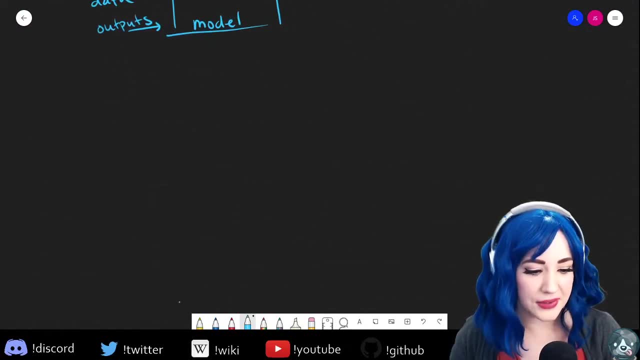 from my mistakes. okay, so supervised learning. we've talked about supervised learning. let's talk unsupervised learning, and I've given you some hints about what. what this was unsupervised learning. now, if the goal of supervised learning is to predict something, it's to predict a continuous value or to predict a category, a class, however you want to think about. 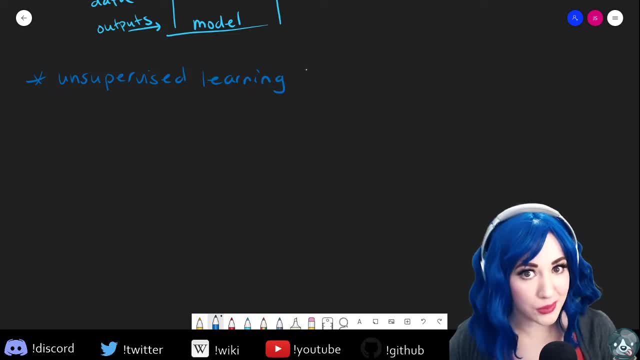 that a label, unsupervised learning? we don't have the labels at all, we just have the data. so, really, what we're trying to do here is we're trying to extract patterns, patterns and relationships in our data. so some of the what are not letters um, some of the approaches that you 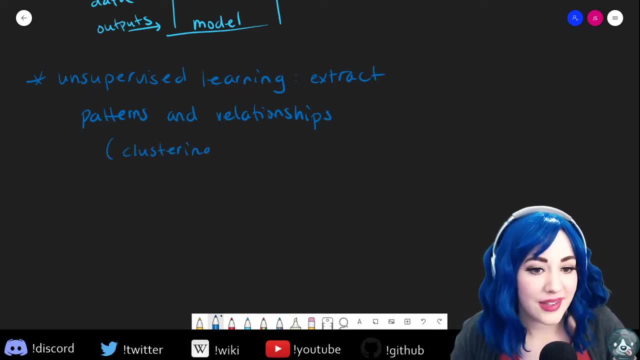 might run into are things like clustering, graph networks- did a whole whole video on that, if you're interested- and dimensionality reduction. once we're through with that, we will move on to the next area, which is document lettering, which is actually like a lot of stuff. it's really cool, but it's it's kind of a little bit confusing, because you 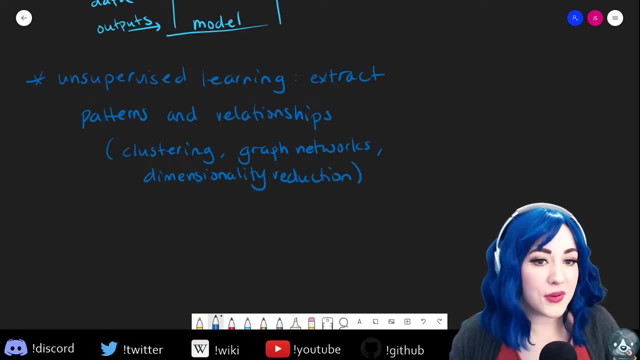 can't really imagine how anything can be so important to you. you just have to be very, very careful on what that means, why I'm doing it, and it's very difficult to do it right. you don't have to read and through talking about the different kinds of machine learning. Ian Alex Hart, thank you so much. 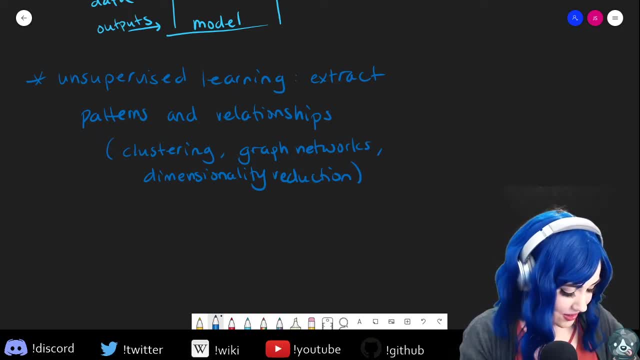 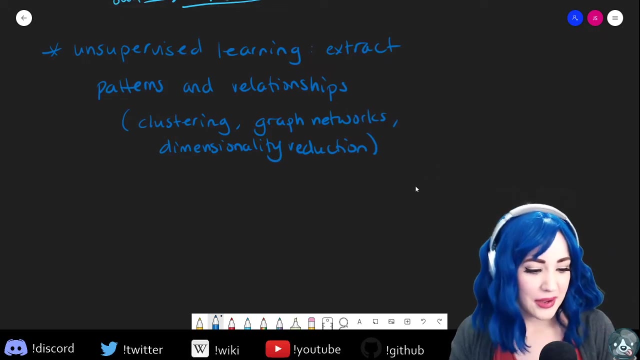 for let's see two more dog treats. We are up to seven dog treats- Six I can count, Goodness Jess. Once we're done talking about the different kinds of machine learning, we'll take a small break and we'll give the dogs some treats, because everybody always wants to give the dogs treats, But okay. 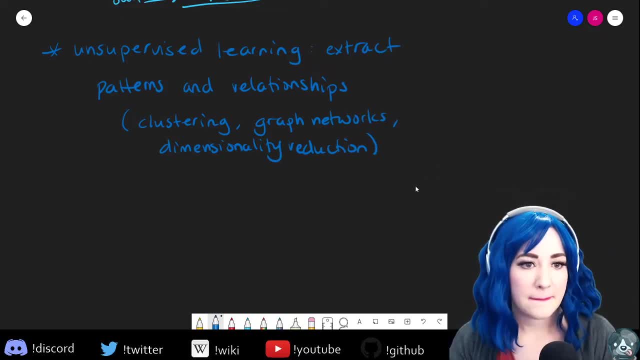 so unsupervised learning. the challenge really is that you don't have labels, And so this is Lord Azazel for you. This is what I was talking about In cybersecurity data. a lot of times we have all of this, you know, maybe like network flow data or something, but you don't have the 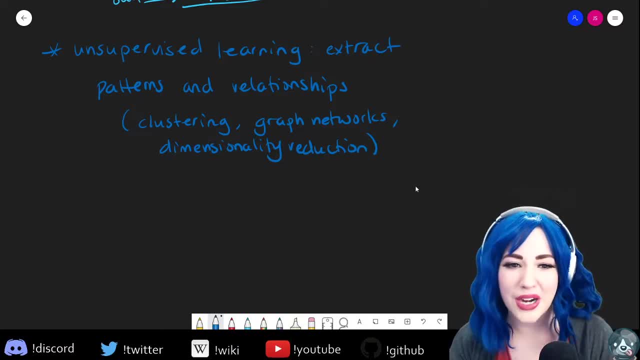 malicious events labeled. So really, what you're trying to do, there is, you know, a branch of unsupervised learning called anomaly detection. Did a whole stream on that too, because I love anomaly detection. But really the challenge is that a lot of times you don't have a wonderful, massive data set with all the bad stuff labeled. 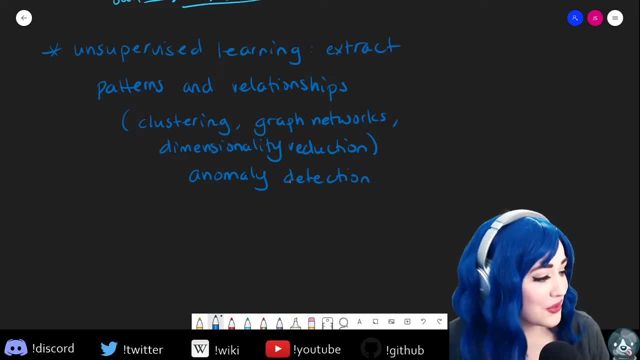 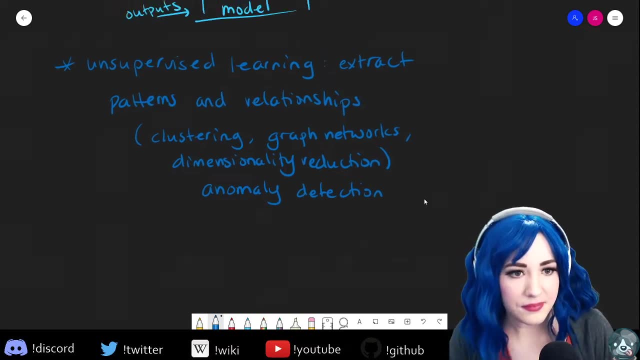 for you. And let's see, Oh, I missed some follows, I'm sorry. The Red Crayon Bandit, Thank you so much for following. And Shigegami, welcome everyone. Okay, And the last kind of. 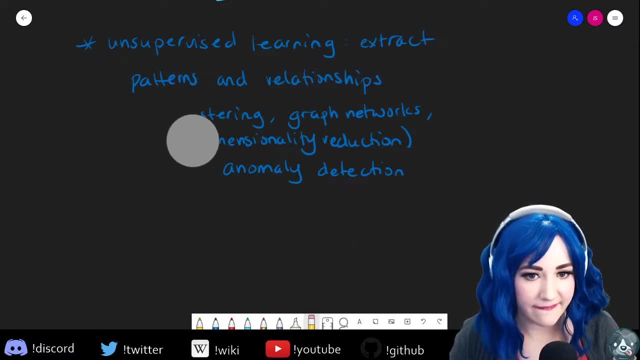 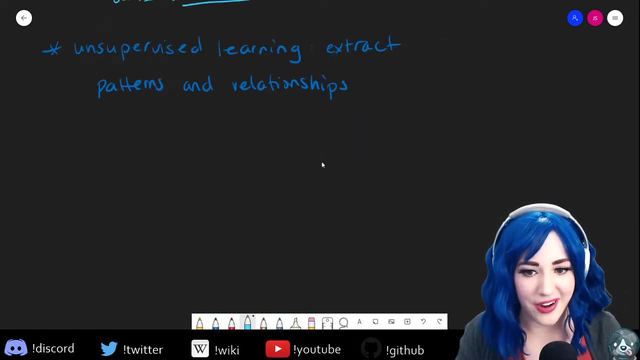 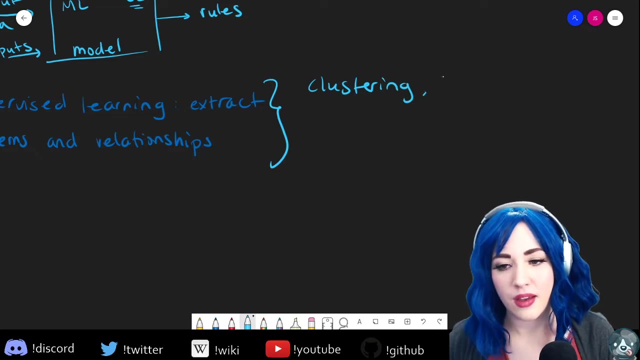 well, this was. I need to be consistent here, Hold on. Thankfully, nobody's turning this into like a textbook or anything, So let's see What did I say? I said clustering graph networks, dimensionality reduction and anomaly detection. 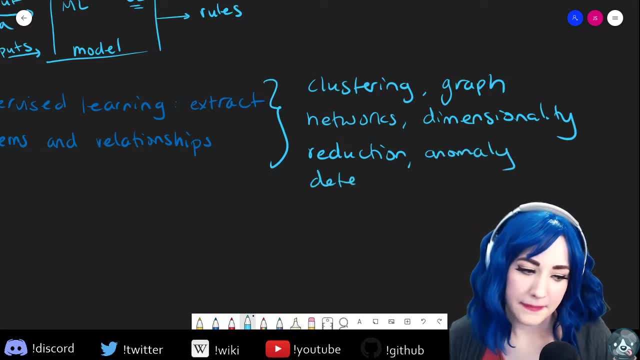 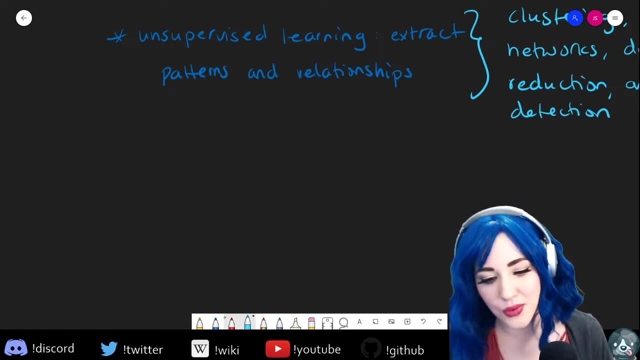 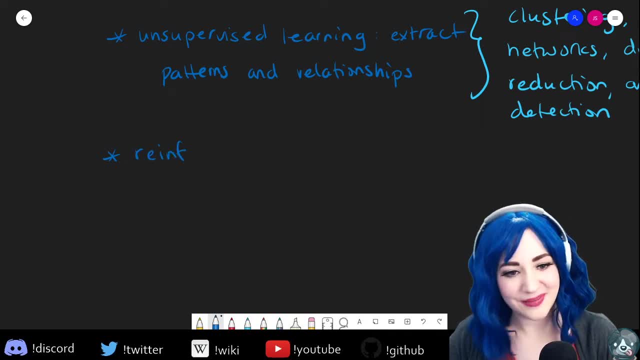 And, my personal favorite, reinforcement learning. And this is where stuff gets bonkers. So reinforcement learning is, you know, very, very different, unlike the previous two methods, where we kind of like have you know, a static data set that we're trying to train a model on, even if we're 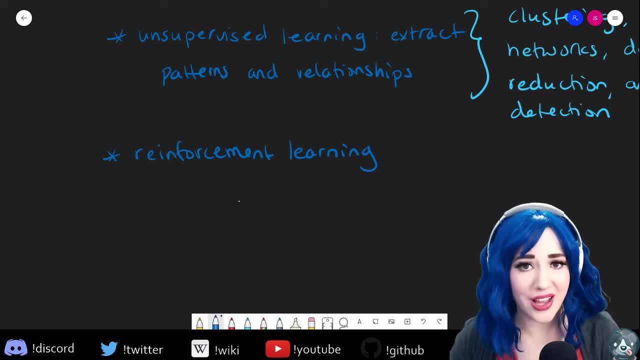 trying to make it into clusters, or we're trying to make it predict a you know, a class, a label. reinforcement learning is actually about teaching an agent to make the best decisions- best decisions here could be. we're trying to optimize a strategy, we're trying to maximize a reward, but reinforcement learning is 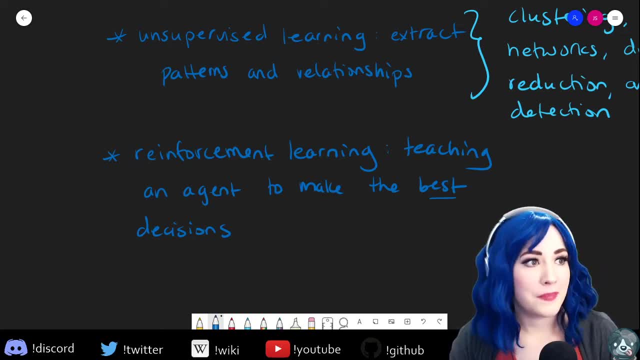 really, really cool, because when you hear about, you know what's it called the AlphaGo or AlphaStar, so computers that learn to play Go or Starcraft or OpenAI- did, did, did the Dota 2 AI as well. this is the they always use reinforcement learning. 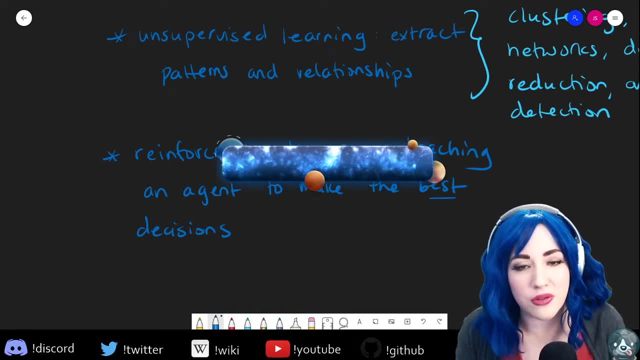 because this is teaching like this is the thing that to me, most resembles what people think of when you say artificial intelligence, because you're teaching a, an agent like it's, not even like a piece of software, it's. you're teaching a decision maker, a computerized decision maker, to make the best decisions, and 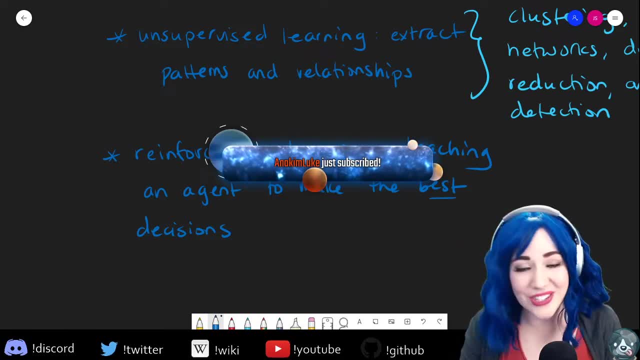 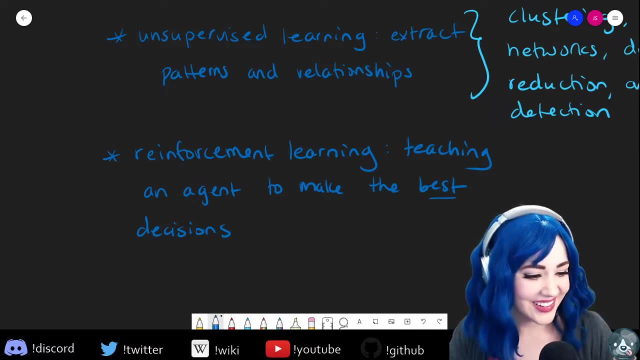 Kevin 21071 and yeah later. thank you so much for following and punchy penguin. thank you so much for gifting a sub to Anikim Luke, thank you, oh, and thank you for answering the tablet question. loaf when, yes, war control, it is an XP pen. all of those letters and numbers works great, it was. 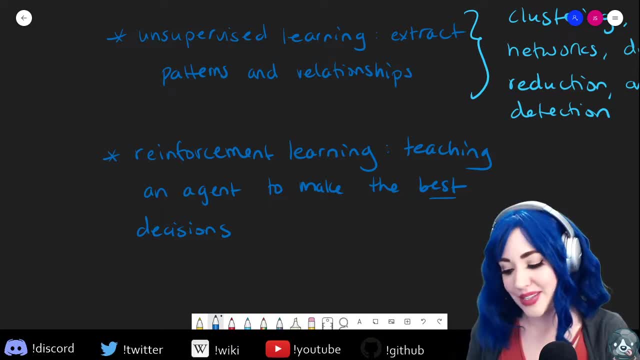 affordable and thanks to all of stream donations, I was able to buy it. so thank you all of you, because clearly nobody wants to deal with my horrible, uh, mess up, and this allows me to actually write somewhat clearly- okay, and subvert us one, two, three. genetic algorithms are a type of machine learning, or is it just a tool? 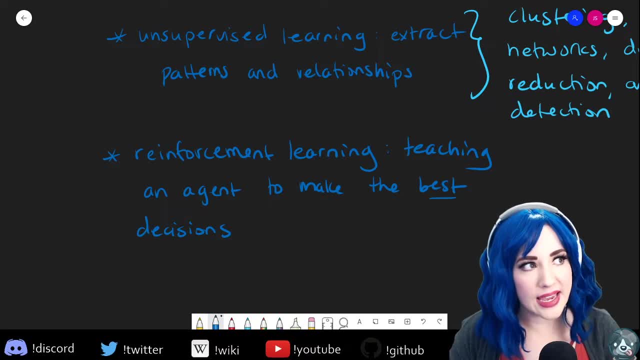 for machine learning. so I wouldn't necessarily say that genetic algorithms fall into like their own category, but they are a type of machine learning absolutely, and it's not one that I've used a whole lot of. I've used a little bit of one for some feature engineering, and that particular one is called the. 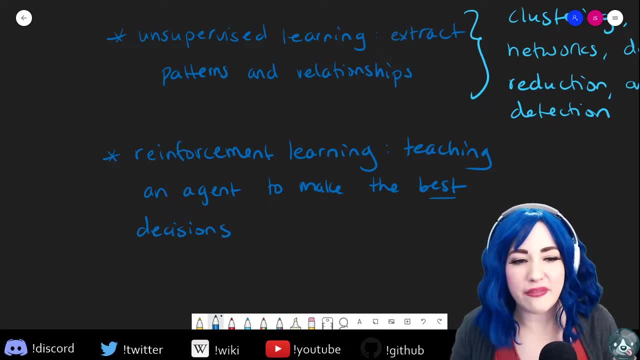 unsupervised learning. so you can still kind of broadly categorize them as supervised, unsupervised or reinforcement. but there definitely are. you know, we talked about earlier semi supervised learning, so there's some stuff that kind of straddle, a couple of these different categories. but one thing that you should: 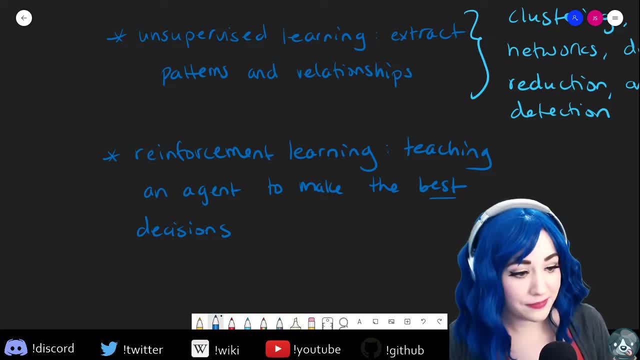 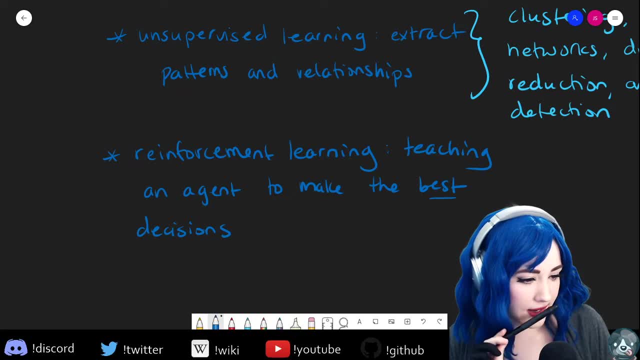 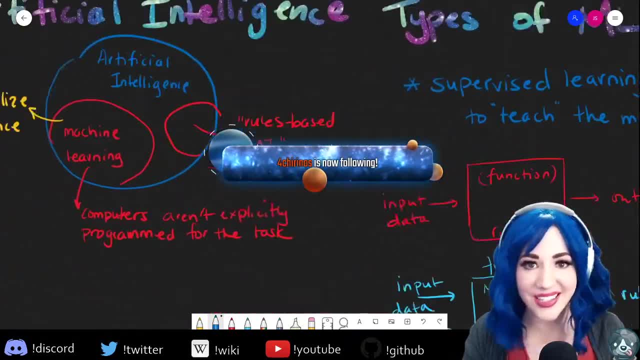 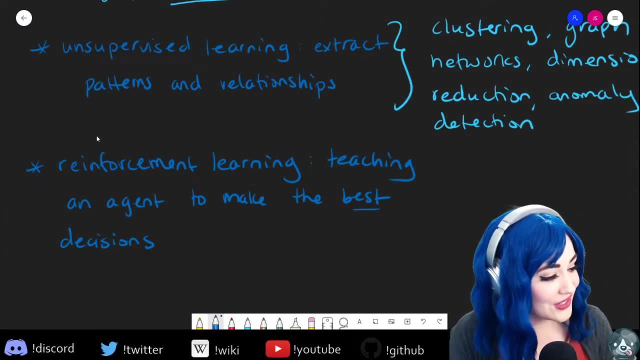 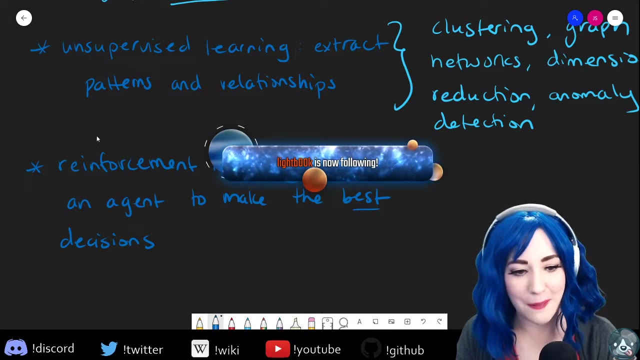 look, look, I got your space colored text. it's just at the top. those are my like headers that I then use with the, the youtube videos, but lightbook and four Carinos, thank you so much for following. yes, Kevin, with thank you. thank you, I love when somebody's like on my wavelength. where does deep learning fit? 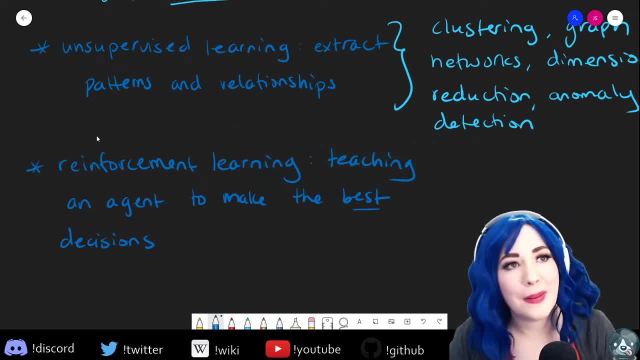 into this and this is where- maybe unpopular opinion, I don't know- some people list deep learning as a different approach altogether. I think that doesn't actually make sense, because you can have unsupervised deep learning. you can have supervised learning. that's deep, deep learning, and you can have reinforcement. 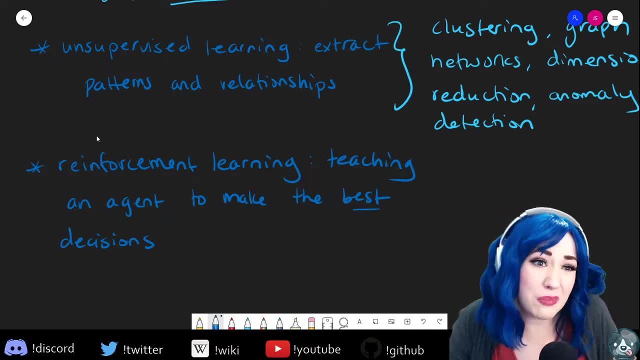 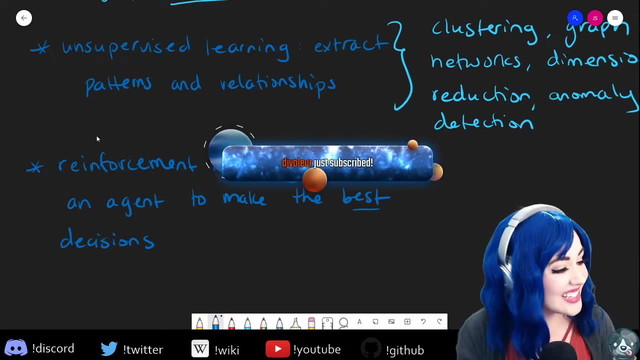 learning, that's deep learning. so deep learning is rather a kind of approach to machine learning. it's not an actual category of machine learning unto itself. and, DJ velour, thank you so much for subscribing six months in advance. holy crap, now you're stuck with me. sure about that cuz now. now, now you're stuck with. 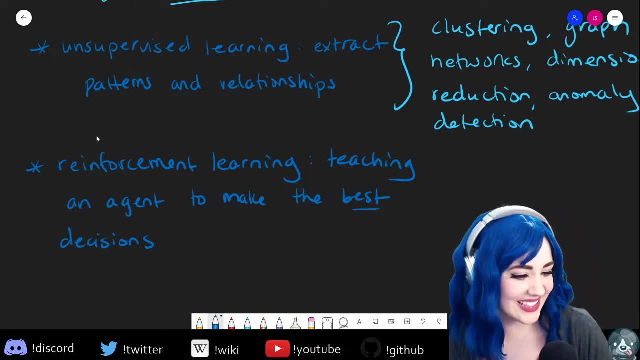 me and let's see, and you say what is deep learning? so deep learning is basically lots and lots of layers of neural nets. and so if you were here for the intro to neural net stream, essentially the multilayered neural net stream is essentially the multi-layered neural net stream. and so if you were here for the intro to neural net stream, essentially the multi-layered 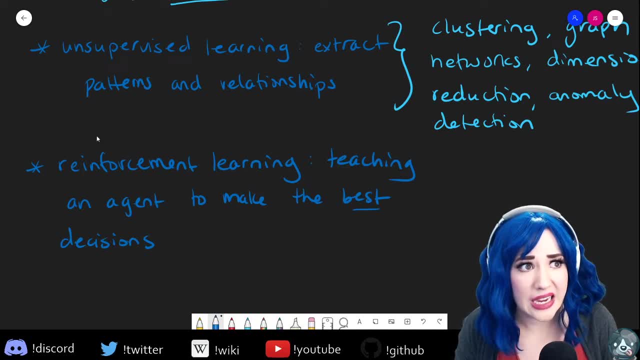 layer perceptron network that we built but like a lot more layers, um, so we just did a couple of layers. but really deep learning- you can think of deep learning kind of being synonymous with neural nets, because largely speaking, nowadays we're not really using neural nets that aren't 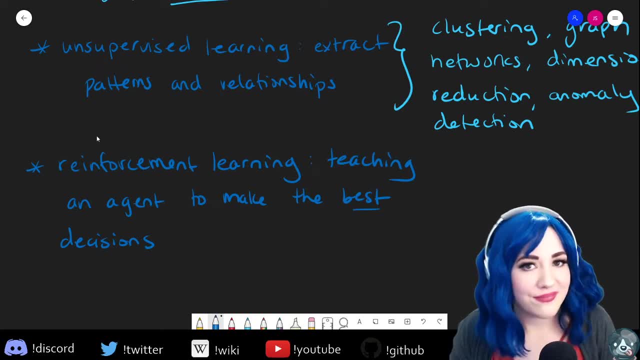 deep a whole lot. um, they're just multi-layered neural nets and if you weren't here for that video, don't worry, you can either watch it on youtube or also i'm. i've gotten a couple requests for a uh future stream doing another. another wonderful introduction to neural nets, so please. 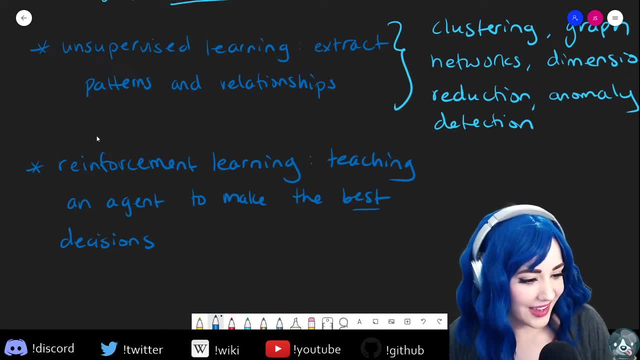 please don't worry um, you're stuck. dj miller, exactly um, and emits you one. you say: where did i go to school? um, so actually, actually i didn't get a stem degree, so i went to the university of virginia for my undergraduate degree and i studied north african. 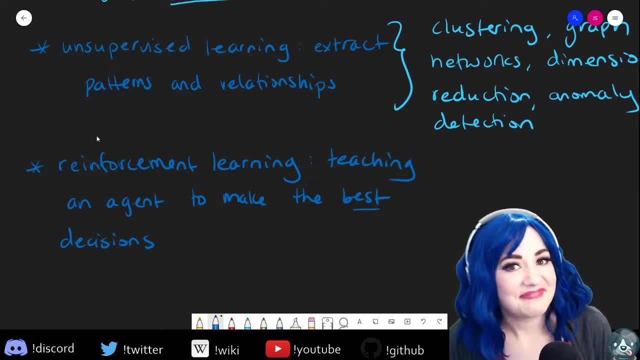 linguistics and philosophy. um, i went to grad school for a couple years in astrophysics and then i left. um, academia wasn't so much for me. i could probably find academia that's for me, but even then i i've really liked working in industry. so jaguar vision. thank you so much for following. 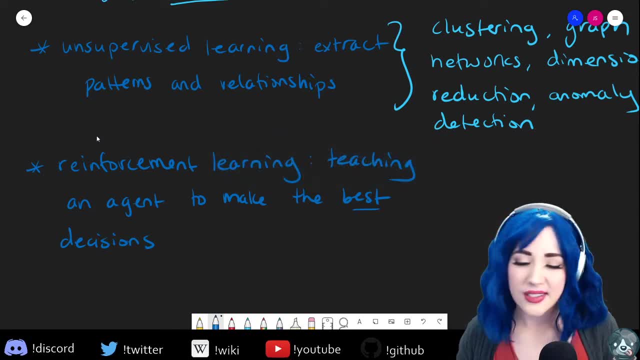 okay, so we're an hour in. we've covered you now. reinforcement learning, supervised learning, unsupervised learning, what even is data science? what even is machine learning? how does this all relate to artificial intelligence? i think it's an excellent, excellent time to give the dog some treats. um, professor, sauce cat, i know, check out. 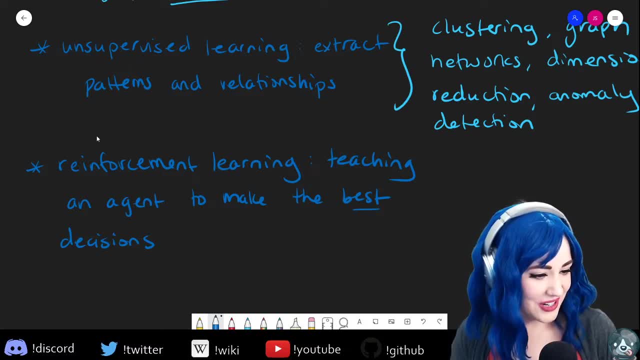 the new pog emote: um and lord is as you say. do i have a list for books about these subjects? um, so i have a couple. i have a couple different books i can recommend, depending on your interest. so i've got a great reinforcement learning textbook. i've got a great like heavy duty, like it's going to beat you over the head. 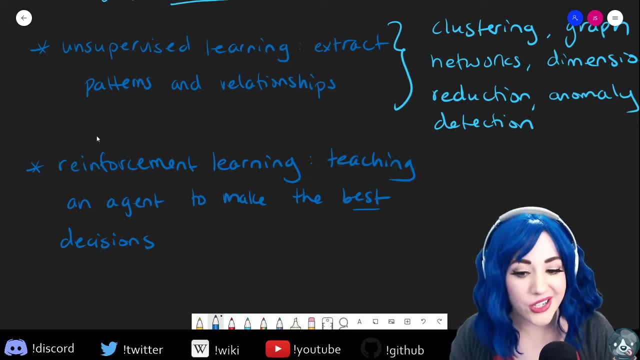 with statistics, introduction to machine learning, but largely you learn the most, just like with programming, by doing so. practice, practice, practice. build lots of models and then dive into the math and the details of the model when you're building it. um, and yes, kevin, absolutely so, if you want to learn more about what are weights, what's back propagation? 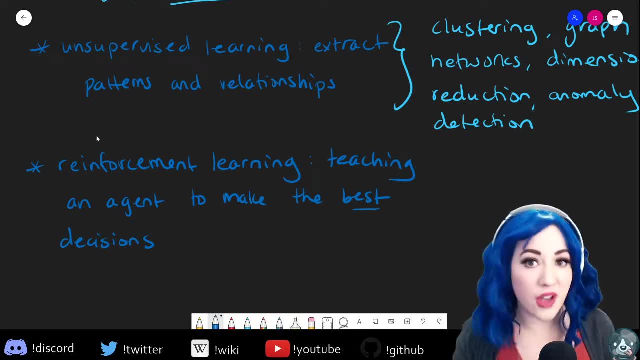 we're going to talk a little bit of gradient descent today, um, which is often used in deep learning. but i do have. i do have the neural net videos, so go check those out. um and work control, i do. i work well technically. my title is lead machine learning developer, but the hats i wear. 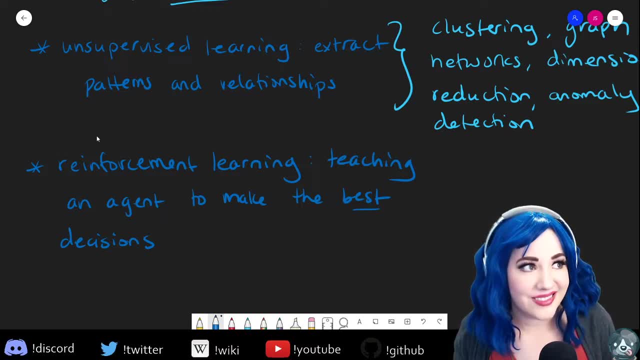 at work are everything from like a software developer to machine learning engineer to kind of a more traditional data scientist. really depends on the day and um. you know what. what's the need is and do. i recommend kaggle. kaggle is a great place to get started with finding new data. 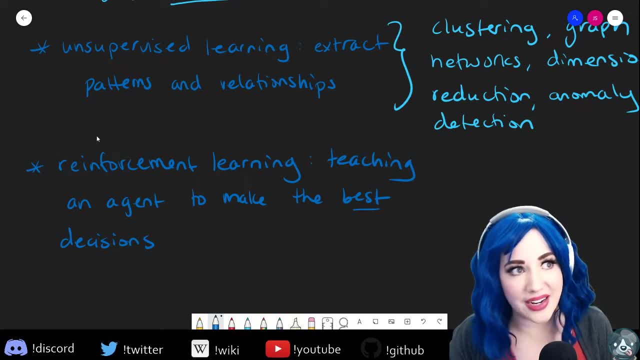 sets and their challenges are often really, really helpful for people getting started in data science. and, dj valer, you said i had your attention when i mentioned anomaly detection. good, yes, so um, can't talk too much about it, but hoping that a patent that i submitted god two years ago- a year and a half patents take a lot of time- was actually 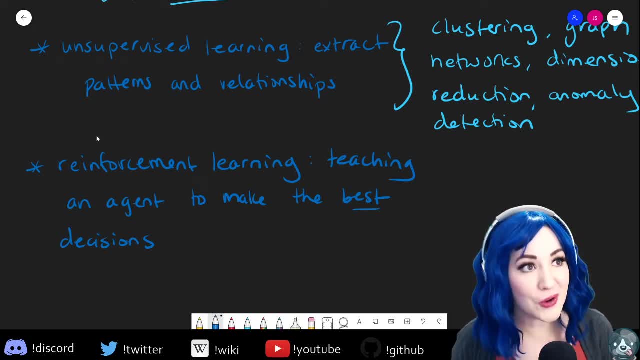 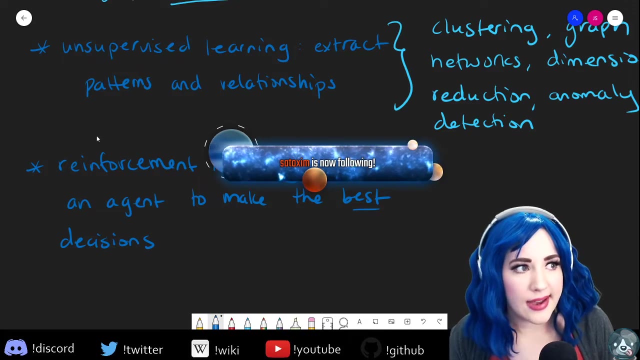 in ai for cyber security, so hopefully someday i'll be able to talk about that when that's all the way through. but, um, war control, i did have a university degree, so i had a bachelor's, plus three, i believe. um, but uh, you know, one of the things i really like with some of the 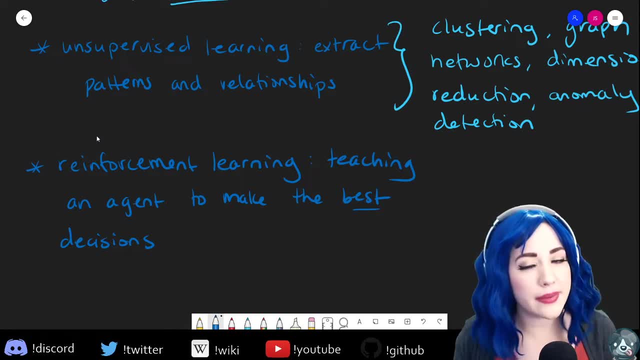 jobs i've been applying to is that they take like a phd or commensurate experience, meaning if i can prove like i know my- i shouldn't swear it's an educational stream- i know what i'm talking about. um, then then they will- uh, they'll- kind of waive the requirement for. 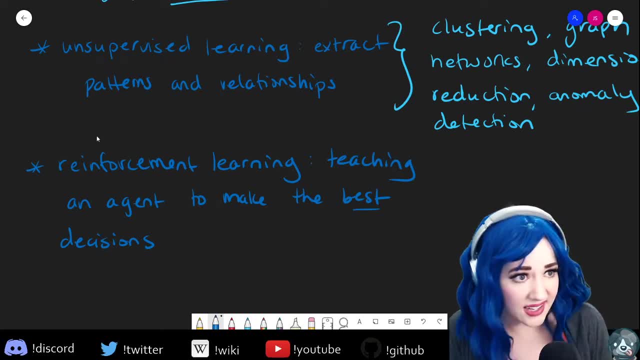 a phd. i'd love to get my phd someday, but i need the right environment and i'm not gonna like work myself to death for less than minimum wage just for the honor of getting a phd. so, drach net, i don't know if i said welcome. i think i said welcome to jaguar, vision um and sitoxum welcome. 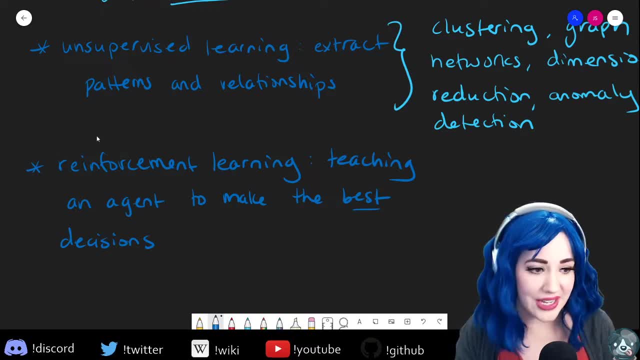 to stream. i know a hacker. i checked it out, but i didn't know what i was doing, so i'm going to try never to swear during the educational streams so I don't put them as marked for kids on YouTube though. so there you go, um, and let's see. here I'll answer a few more questions, then I'm gonna go get. 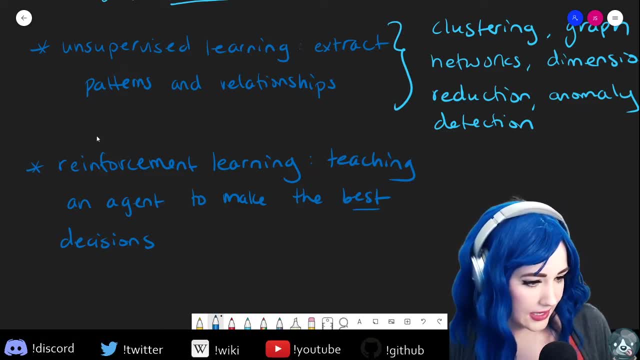 the furbo set up with the dogs. but let's see here, um, I find auntie say I find the best way to learn these things is to implement them yourself before using a library. yeah, exactly, and that's why, for the neural net video, we built our prop back propagation, our feed forward, all of that we. 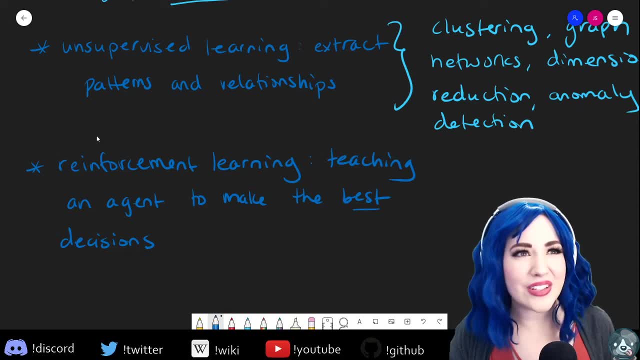 built it from scratch, because I really do. I completely agree, even if it's not like the most optimized, and using a library is far more efficient if you're really struggling with grasping something, sometimes just forcing yourself to go through the the slog of building it from the. 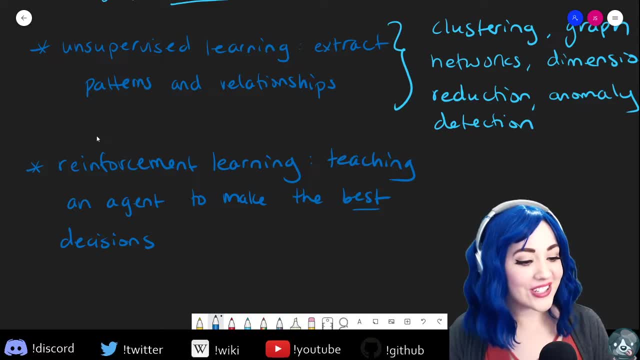 ground up is really educational. and professor sauce cat, what did I learn about your North African culture? it's been a long time. I lived in Tunisia for a while and many, many, many years ago, so actually coming up on 10 years ago, I was fluent in French and 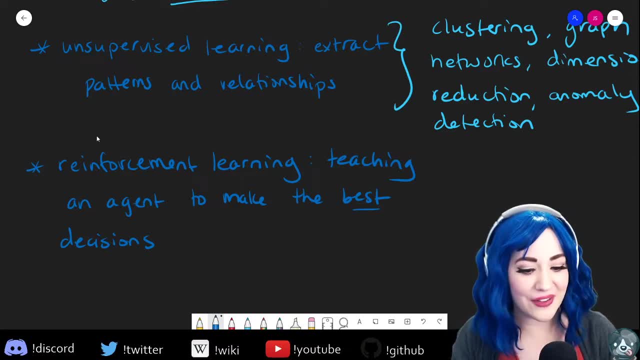 Arabic. um, and that was my, my area of focus, and I was there right after, um, the Arab spring, so it was quite an education. um, okay, so I'm gonna go get the furbo set up so we can give the dogs some treats, because we are up to six, six, whole dog treats. um, so don't go anywhere and uh. 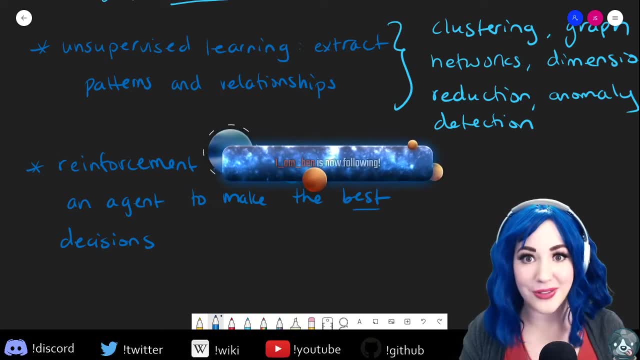 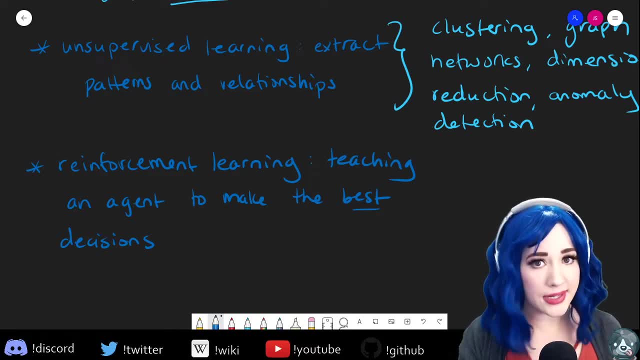 data science is what machine learning is is. we're going to drill down into a kind of supervised learning called classification. in particular, I'm going to be doing a quick review. for those of you who were in machine learning this it'll be an easy review. new folks it might, might I might slow it. 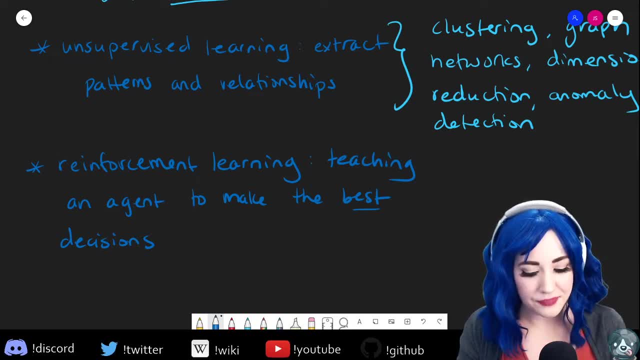 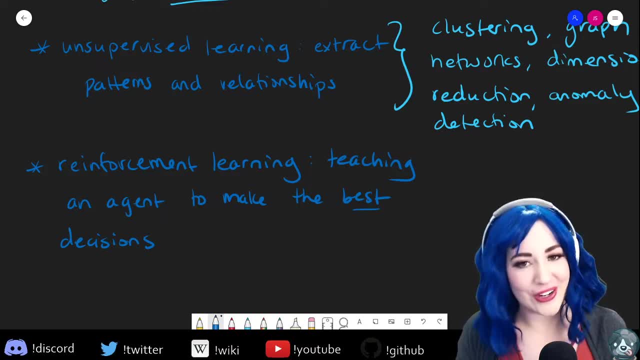 um, that was the thing that I didn't do for machine learning this. I told you kind of how cool gradient boosted trees are, but I left it for another day. so we're gonna, we're gonna come back to it today. not logistic regression, ant, but ah, I love saying this. I have a whole video on that, so if you want, 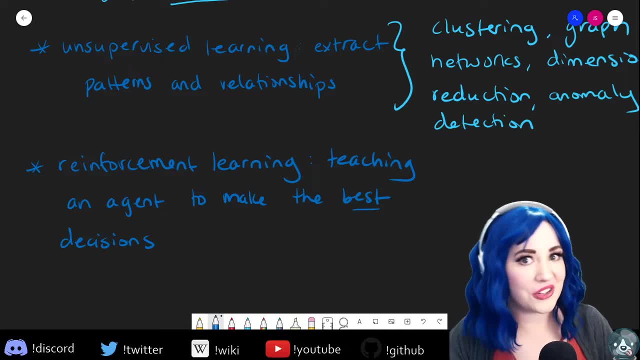 to learn more about logistic regression. uh, definitely check out machine learning- this on YouTube. but I will be right back. don't go anywhere. my dogs will cry. they will think you don't love them. how's that for bribery? um, I'm gonna go set up the furbo. I'll 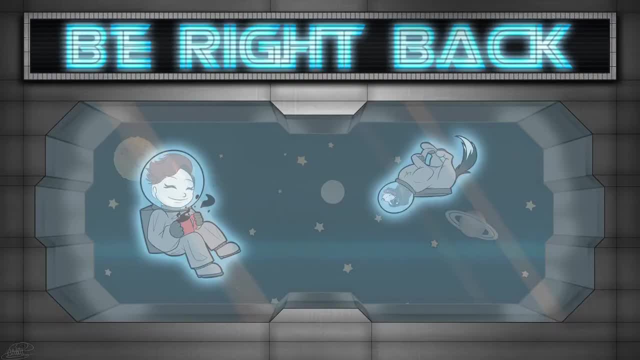 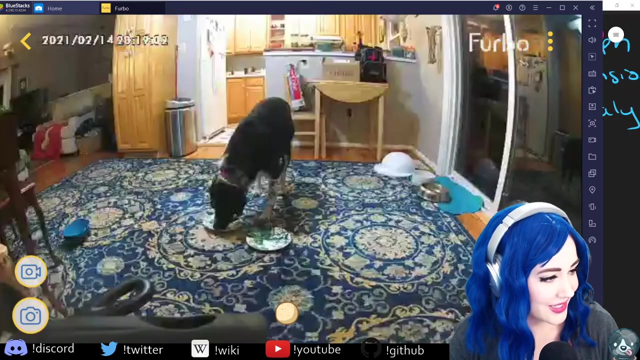 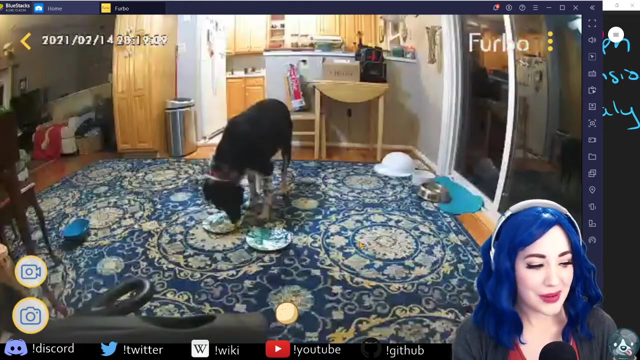 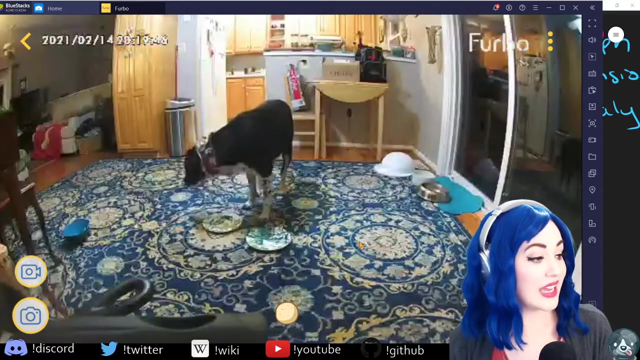 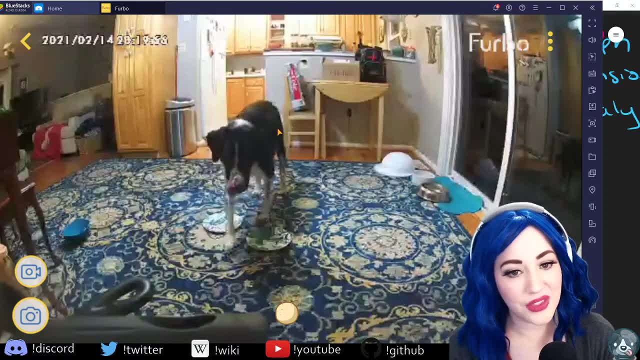 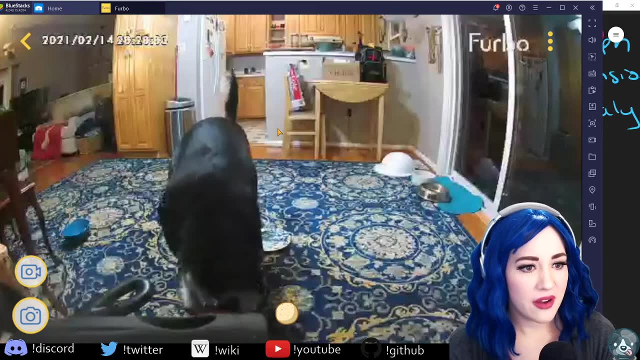 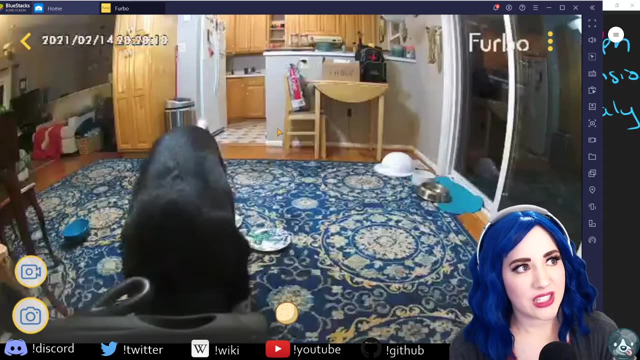 Oh well, So here was the plan. The plan was- You see how there's two plates there. The plan was to put peanut butter on each plate for each dog. Tennessee, though, is under a blanket, doesn't want to move, not even for peanut butter, so Hubble just. 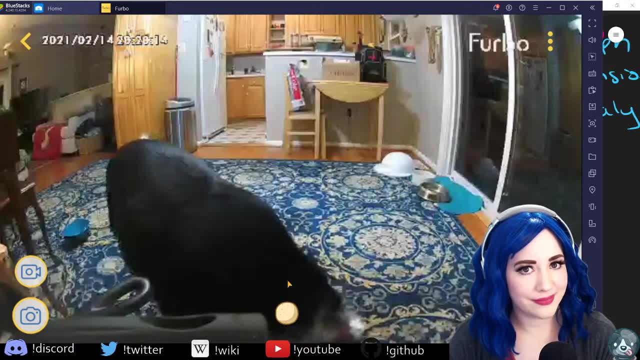 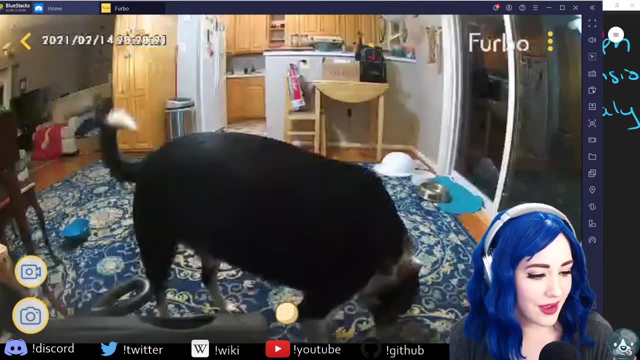 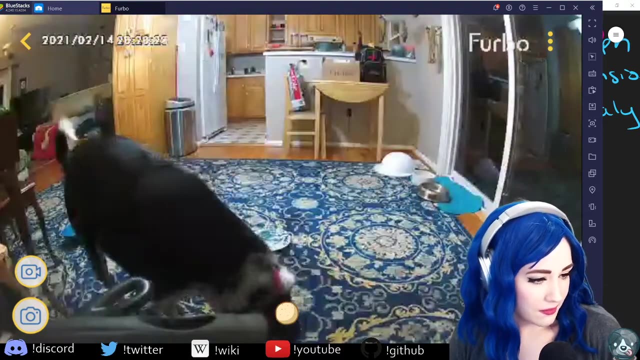 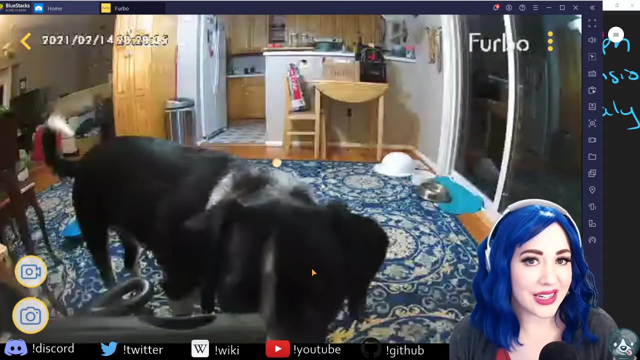 ate both plates, oops, um, but I'm catching up on chat while I'm just gonna throw these treats at Hubble. um, this is Hubble. yes, let's see um. moving backwards, oh, cannabis coach. if you ask if I finish, or if I visited the Star Wars film locations in Tunisia, I absolutely did, the funny thing being. 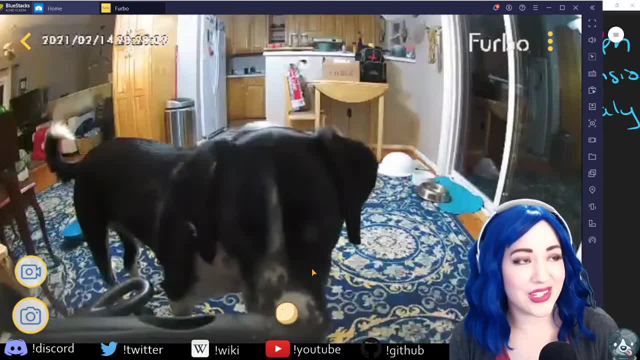 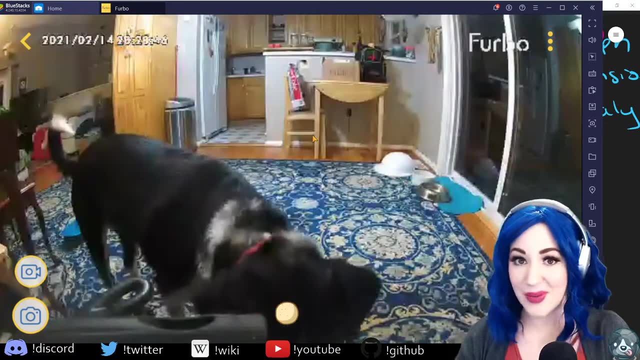 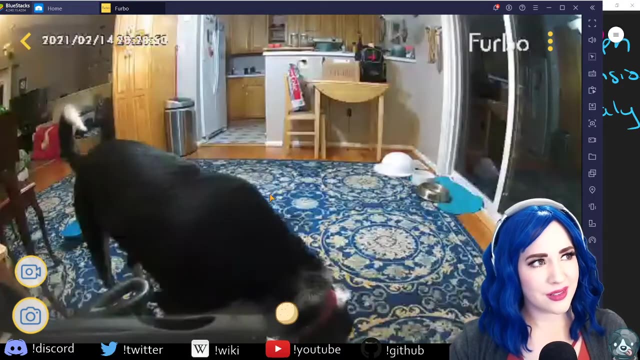 that the Tunisian city of Tatooine is not where Star Wars was filmed, so it's actually filmed in a different area, also within the Sahara Desert, and I went there. so there's pictures of me- probably not on Twitter, but probably on the internet- somewhere- baby Jess, 10 years ago, visiting uh. 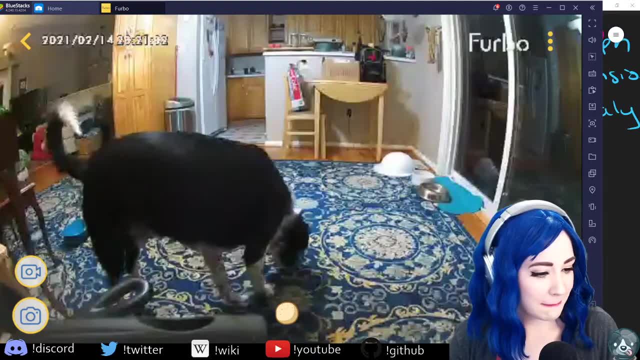 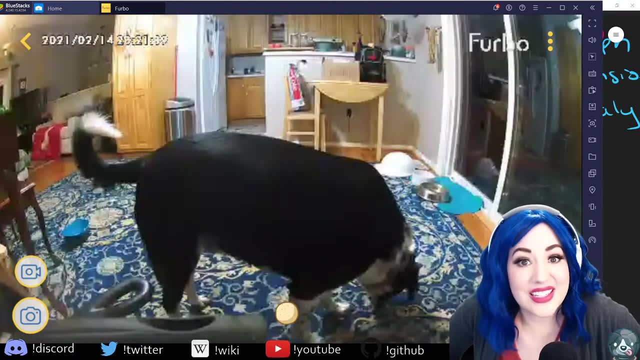 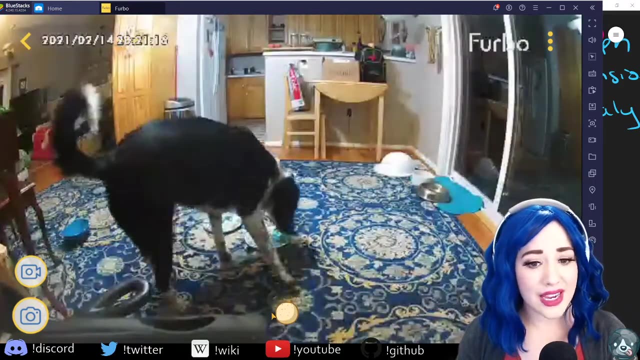 visiting the filming location for Star Wars and let's see gaze into the iris. you say I should do some autobiography streams. well, if you stick with me, I do a kind of open Q&A at the end of streams. folks ask about everything from you know: technical machine learning questions, math questions, space questions. 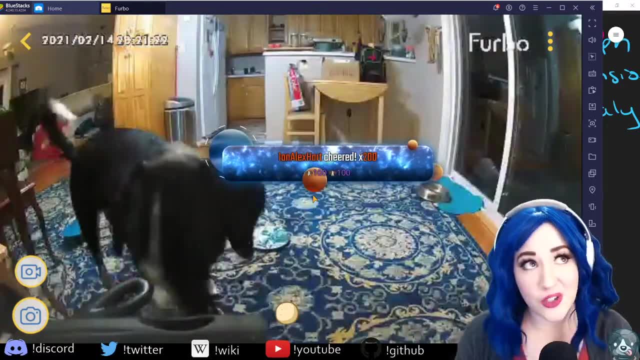 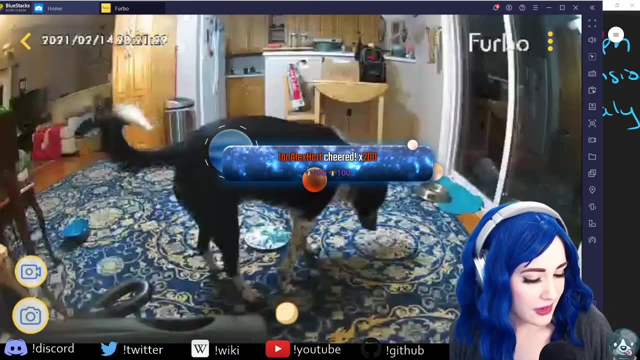 to life questions, or you know how much do I love dogs? kinds of questions. um, I've lost track. we'll give him one more set of treats after this, but let's see Ian and Alex are coming in with two more dog treats. see, okay, now we gotta give him two more. 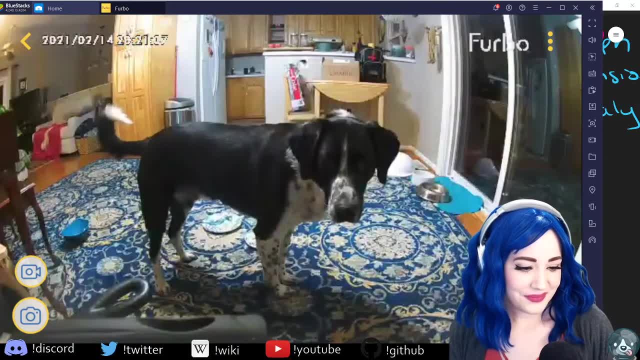 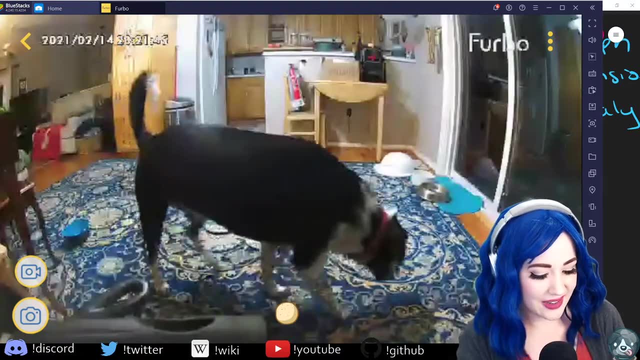 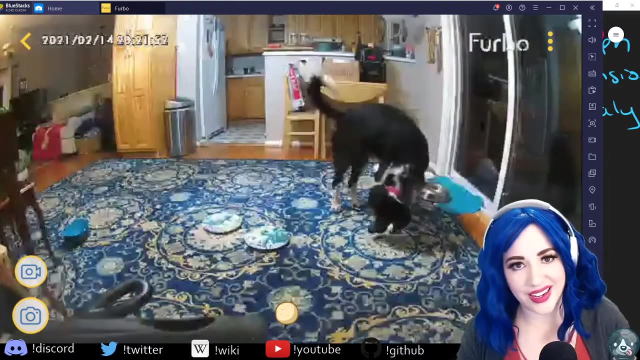 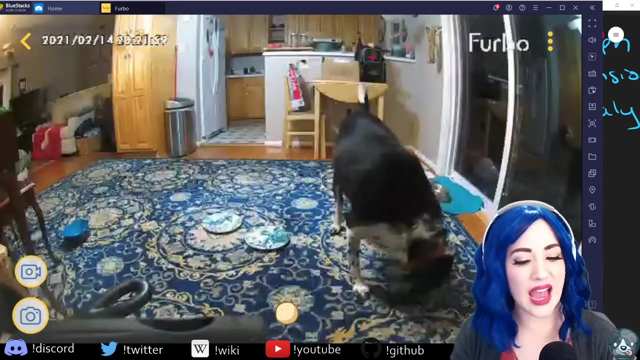 here you go, Hubs, he's so cute. I love Hubble. Tennessee, though, let's see, I haven't updated the 10 and Hubble pictures from the last stream, but you can get. you can get a little bit of a taste of Tennessee there. oh, alliteration, um, did I ever visit the eye of the Sahara? 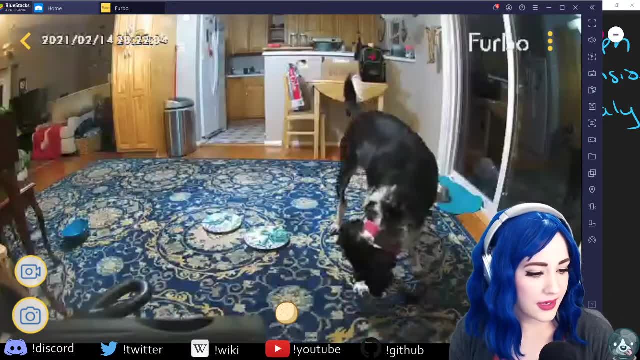 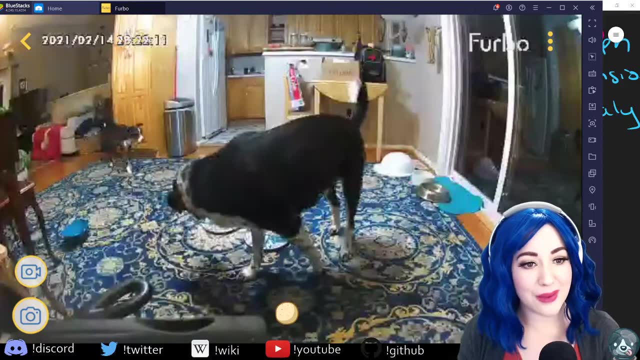 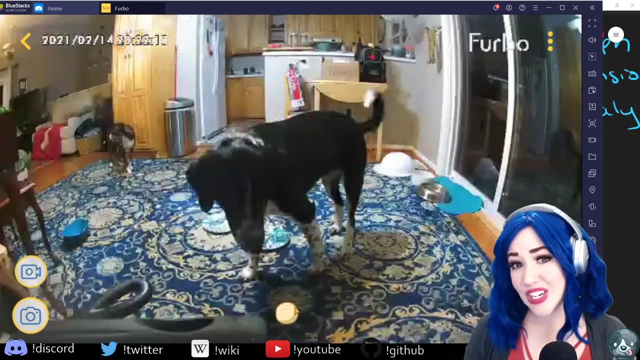 um, I did not. um and war control. you ask: how long do the videos on Twitch last after the live stream? I actually have no idea, but don't worry. the ones where I'm doing, oh, here comes 10, Tennessee little boy, uh, the ones where I'm doing any kind of like teaching, 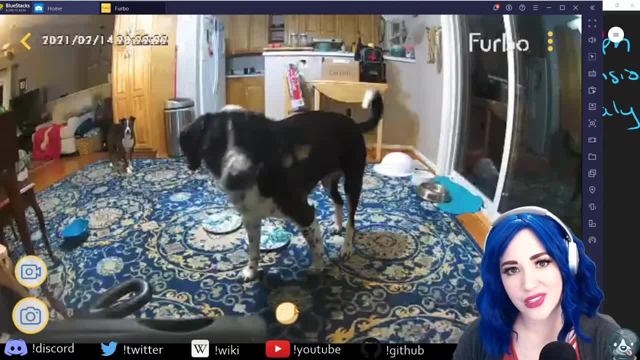 so the ones tagged like tutorial or education. I download the VODs for those and those go up on on YouTube. so I guess it does mean more treats, exactly, Ant. so I wish I could like direct it like, if I toss an I don't know, it's like the same thing to download it and see what works, and like I would actually be same thing if it doesn't work. but I try to keep things up. 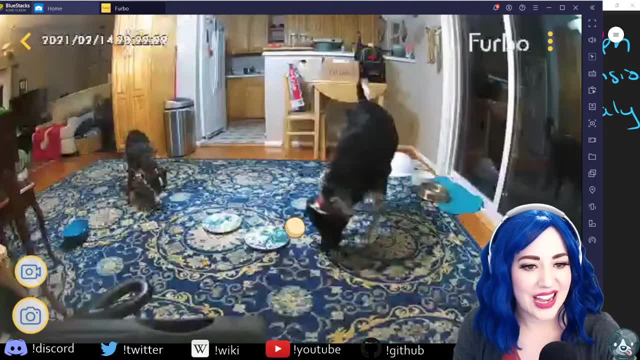 you like. if I don't know what works, sometimes things change depending on what I'm doing, but I I really don't know how to take advantage of all the things that I've done. So I guess it does mean more treats, exactly, Ant. So I wish I could like direct it. 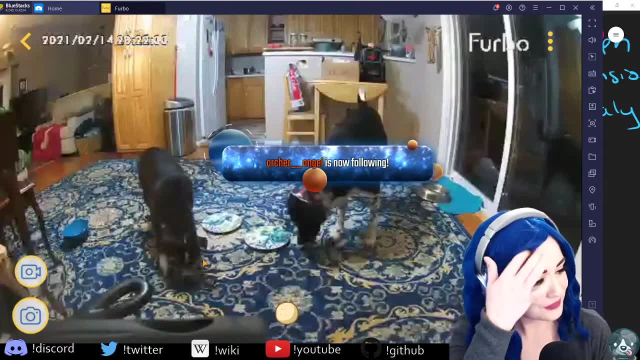 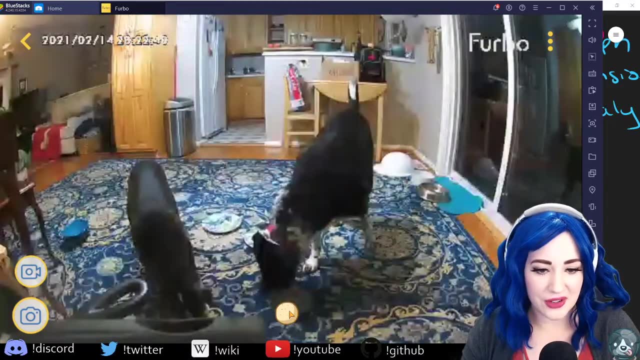 Like, if I tossed the treat to the left, maybe you would like toss it to 10.. And Archer Angel, thank you so much for following. I know Tennessee needs his treats. They're very good at sharing, though, so 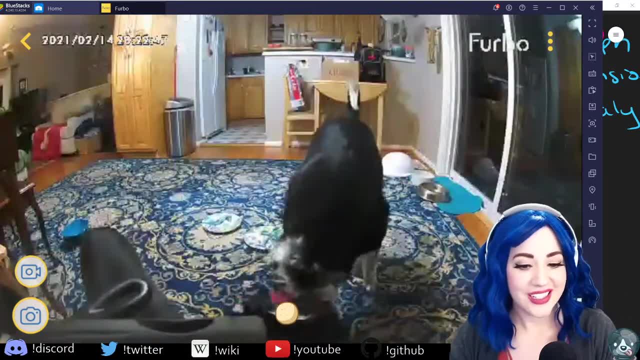 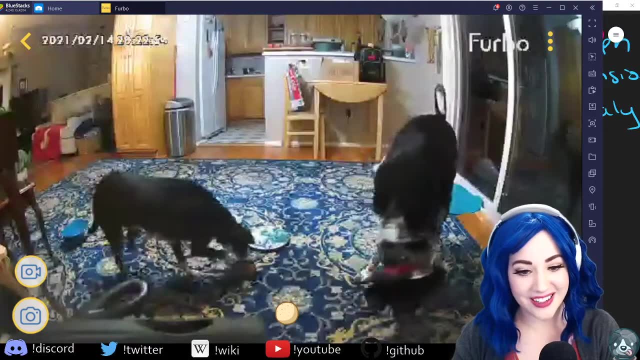 Even though Hubble's the bigger one, he's the far more docile one. So if Tennessee can get like, he's the one that if anyone's going to cause a problem and get bitey and territorial, that would be Tennessee. 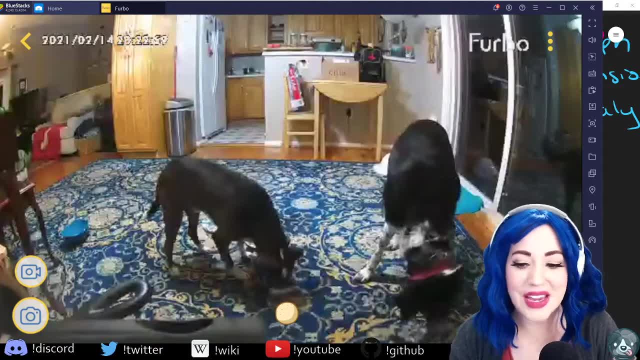 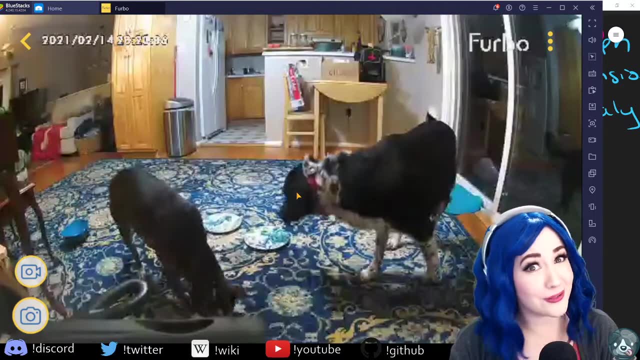 He's a very good boy, but they are both rescue dogs, so they come with their own issues. Both were abandoned. Hubble, in particular, was returned to the rescue three times before I adopted him. Look what they're missing out. 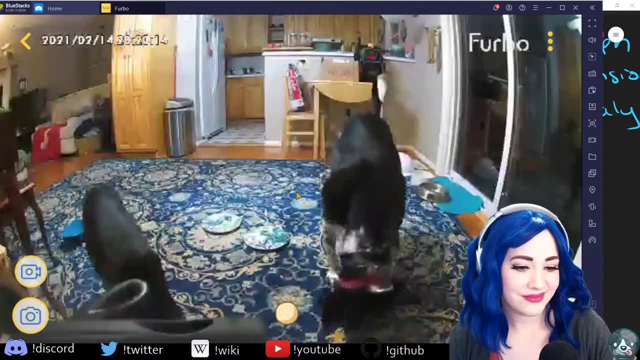 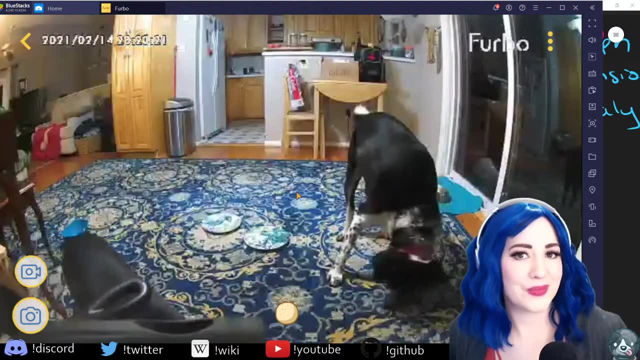 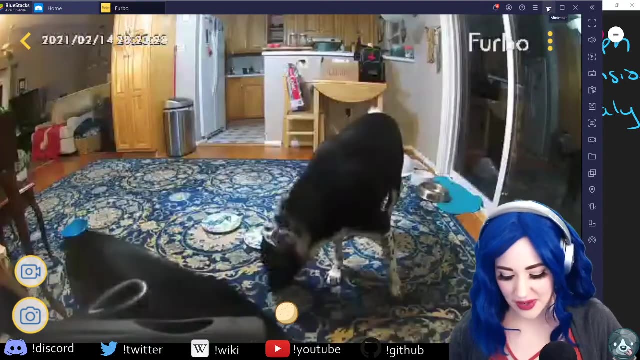 Look at this. very good boy. And Tennessee was very, very scared. Very little boy, And now they're both happy. So rescue, adopt, don't shop. All right back to machine learning. So we have- actually we've just dispensed probably more than eight treats to the boys. 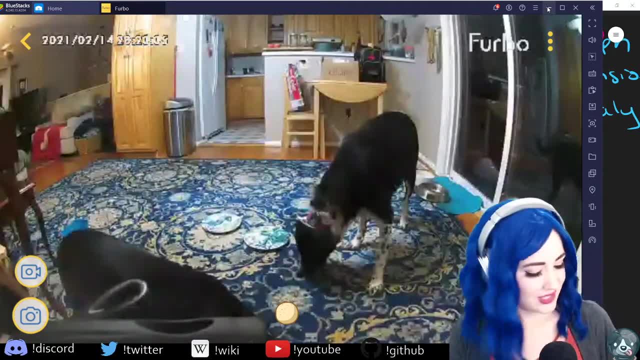 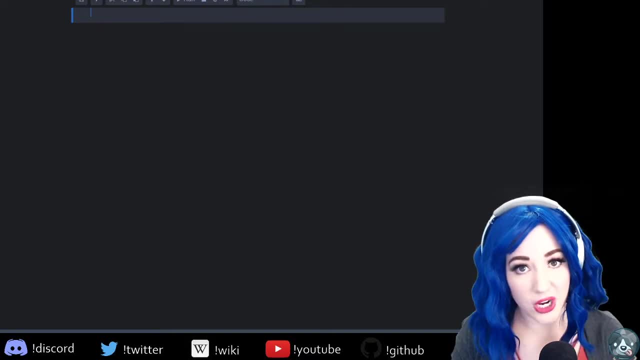 but I will cross out our count. Such such good little baby boys, And have no fear. So for those of you who are interested, here's a preview. We're going to code today. Spoiler alert For those of you who are more interested in the coding portion: have no fear. 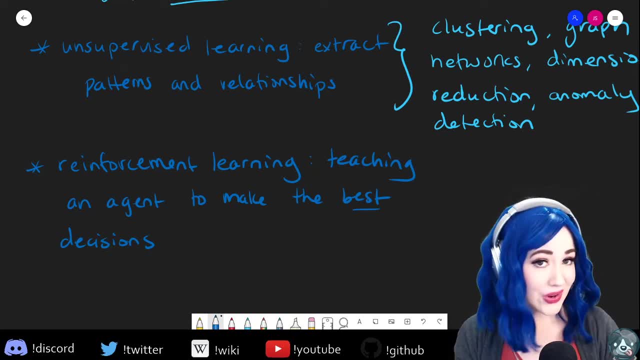 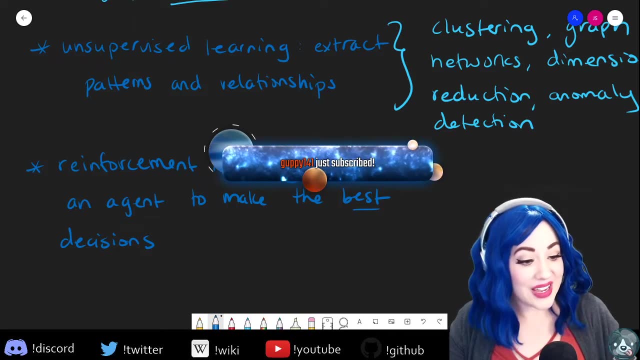 I do like to, you know, keep my streams a balance of the theory and the code. So we'll do some theory and then we'll get down to. you know, put our hands on a keyboard, Punchy Penguin, five gifts of thank you. 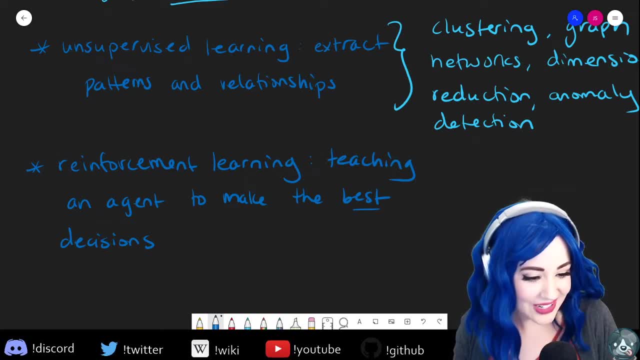 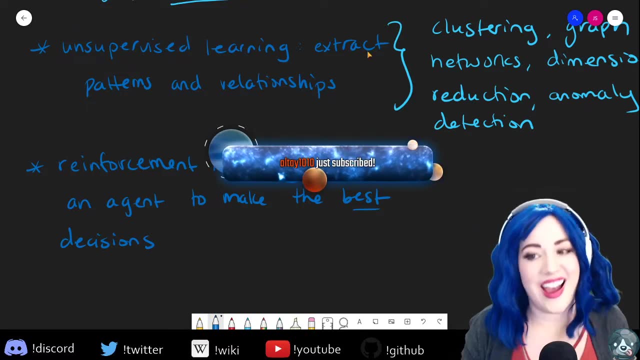 And now Guppy141, Alte1010, Carmagen, Garbage Day, Distant City. Now you're stuck with me for a month. Now you have to hang out. Ha ha, ha, ha ha. No, I mean you don't, I promise. 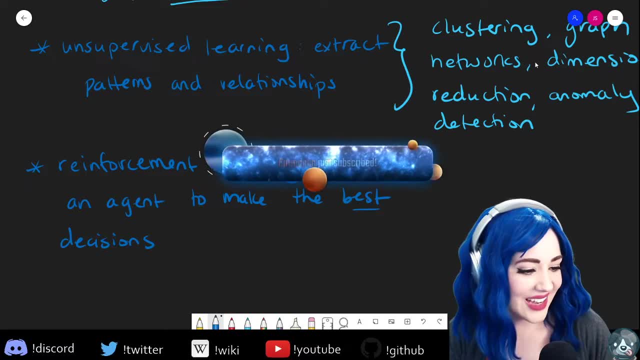 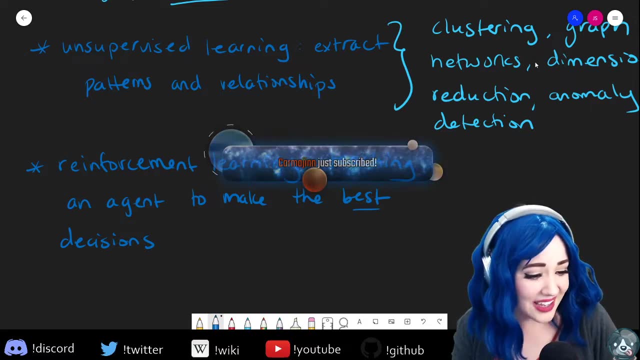 But please, because I love having all of you here. And um and to Ant Punchy Penguin, thank you. Do you stream? Can I give you a Shout out Like thank you so much for for gifting all of these subs? 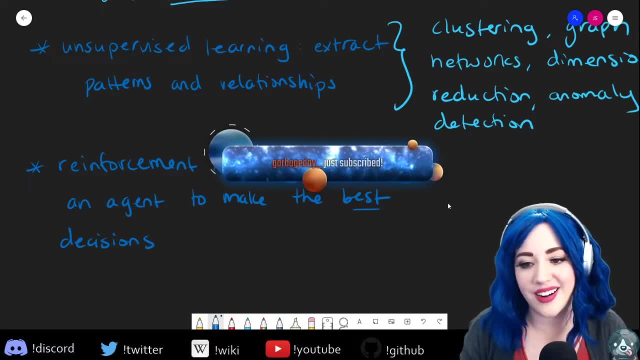 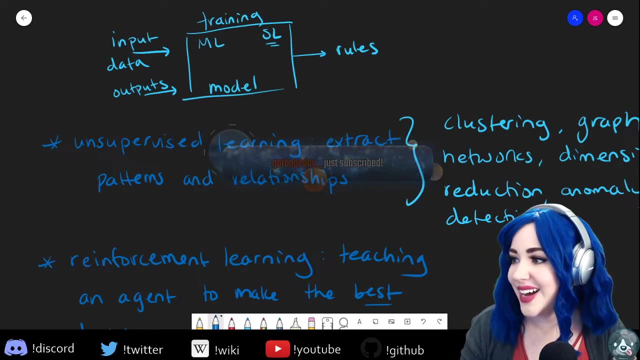 That's very kind of you. It's for the dogs. Well, there you go. All right, Fine, I can definitely. I don't delude myself that people are here more for the dogs than for me. Don't worry Um, but let's see. 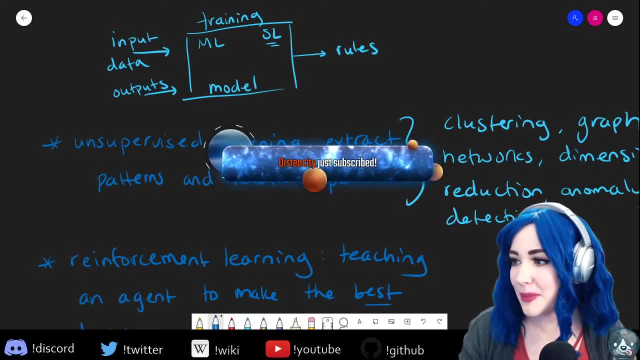 Master Dark Weaver: Yes, Python, We're going to, we're going to be, we're going to be doing some, some Python, All right. So let me see how balanced my notes are. How am I doing here? Okay? 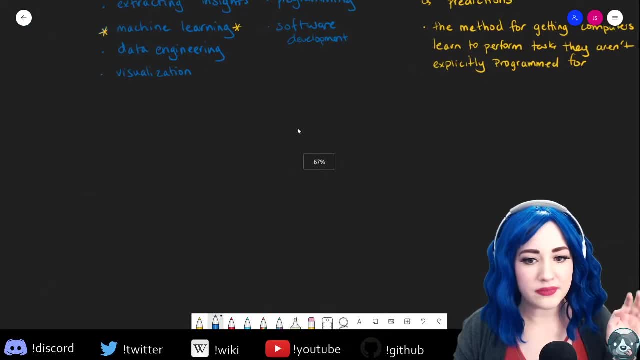 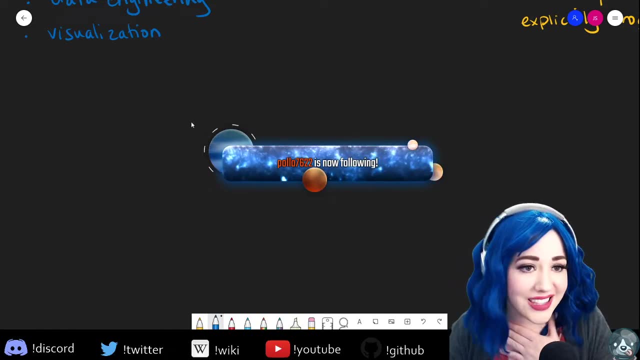 Not bad. Let's go over here. So, like I mentioned, remember our, our lay of the land here, Actually Pola7622, I don't want you to get lost. Thank you so much for following. Welcome, welcome to stream. 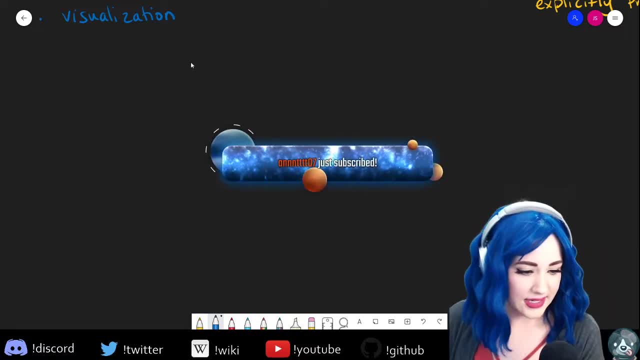 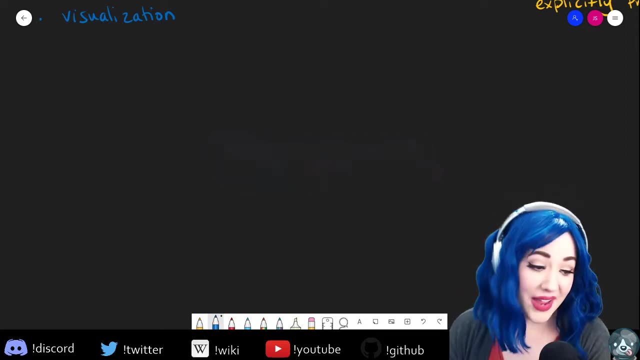 All right. So let's see here: When do you get to see the dogs next A hacker? I just you. Well, you know how I end my streams? You do, But all our new friends probably don't. So guess what friends. 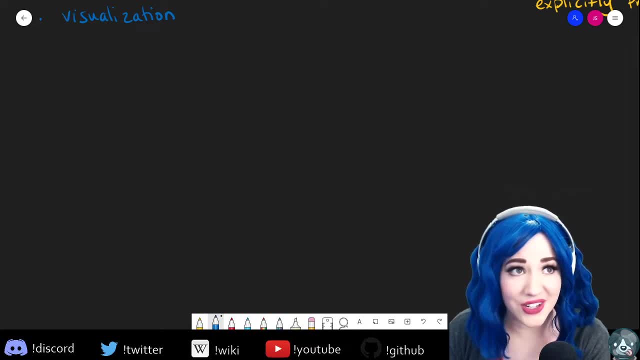 Tennessee sings. And Tennessee doesn't just sing to anything, Tennessee sings to sci-fi TV show themes. In particular, his favorites are Star Trek- Let's see He sings- TNG, DS9, Voyager and the original series And Discovery. 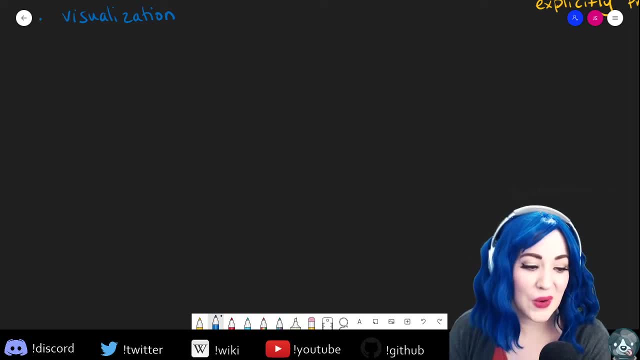 And Stargate SG-1 and Atlantis. So I like to wrap up my streams before V-Ray With with a 10.. So we go casual, I take down my green screen, I bring Tennessee off and Hubble comes too, and uh well, we'll have a song. 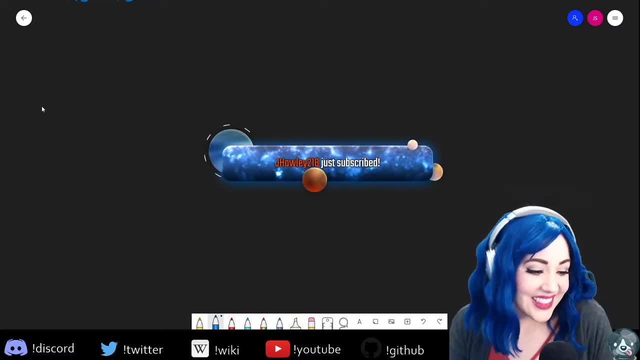 You all, friends, DJ Velour, thank you so much, Oh my goodness. And now there's like a- what is this? a hype train. I, oh my goodness, You all are so nice. Oh, now we get cool hype emotes. 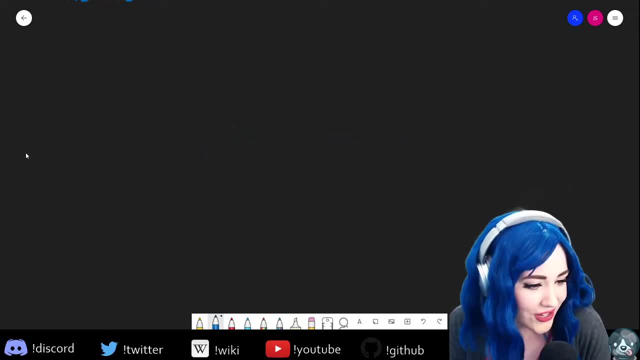 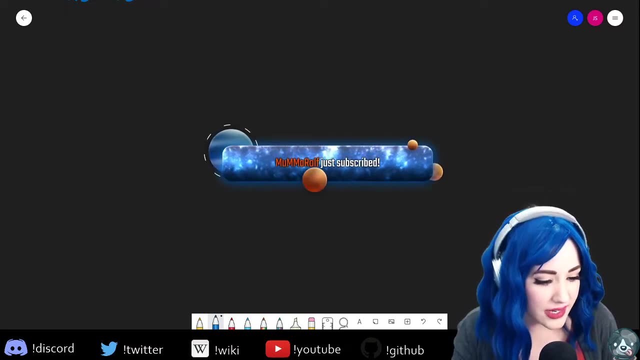 And Warzoid Kaya Razic Mama Rolf J Holly, Oh yeah, And Rattatat, You all get subs, So check out your awesome emotes There are. there is a new one that I've added. 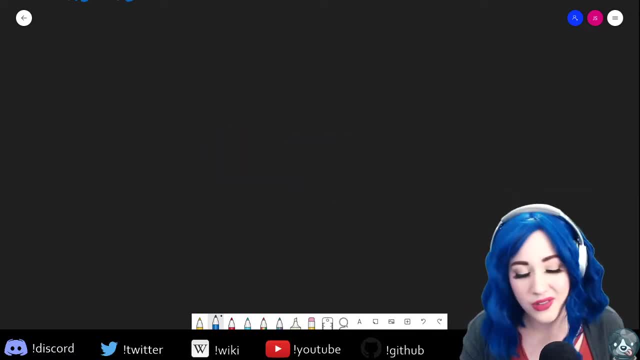 Um, you should see that we now have our own Encella Pog. So now there's like a PogChamp emote Of my face. Um, Pudgy Penguin, You guys, five more gift slips You. this is yeah. now I don't know what to do. 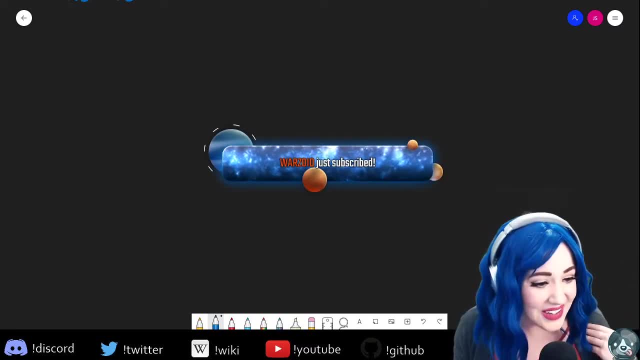 I have to like go hide. I'm going to start blushing And get all red. Thank you. Now C Sharp Josh, Yeah, C Sharp Uh. Hacker Gathering Wolves, Mikey Man and Akashic Sushi Records. 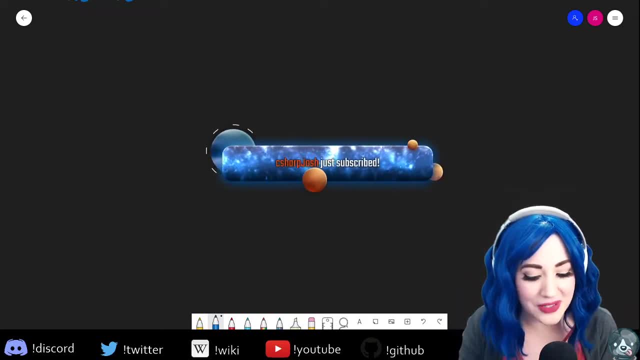 You all have subs. Enjoy the um Hubble emote, Ten emote, Burger emote and the Pog emote. Um, I know, Look, J Holly, It's a new new emote, And Ask RVdar. 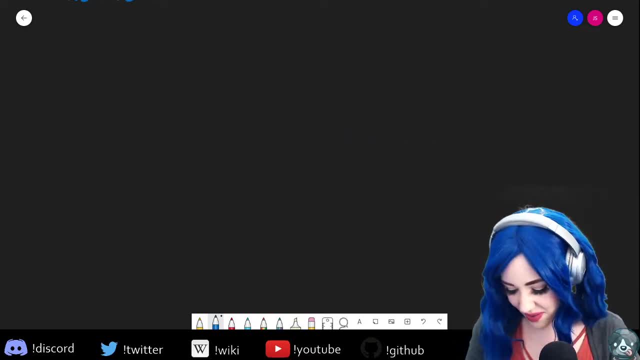 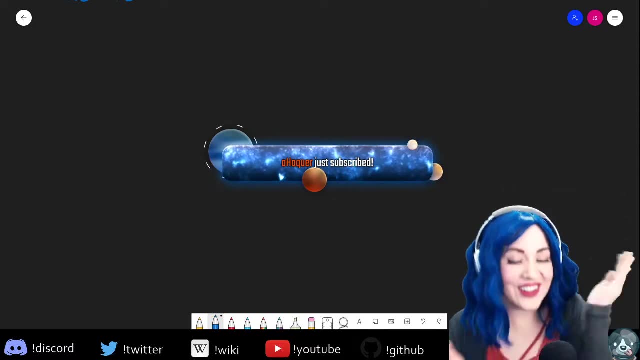 We've got. we've got a treat for the dogs. All right, So I'm starting a new count of treats for the dogs. Holy sh, okay, I can't swear. It's an educational stream, DJ Valur, you guys. 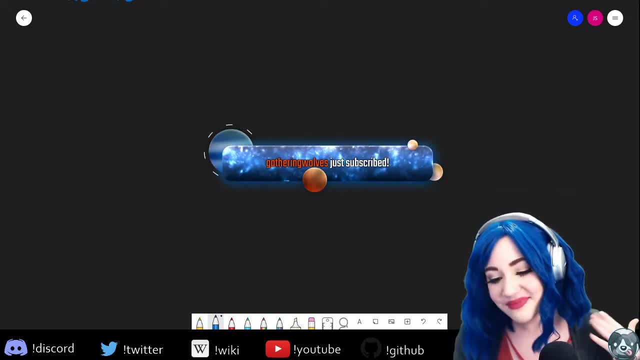 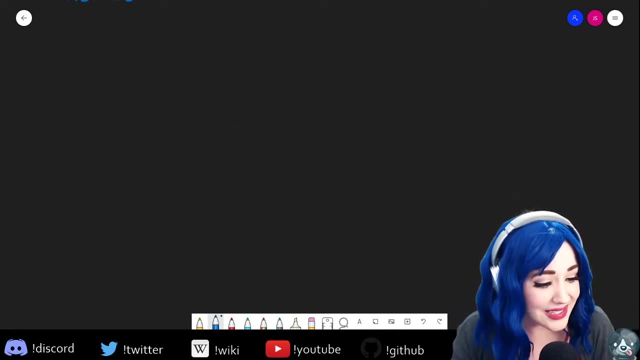 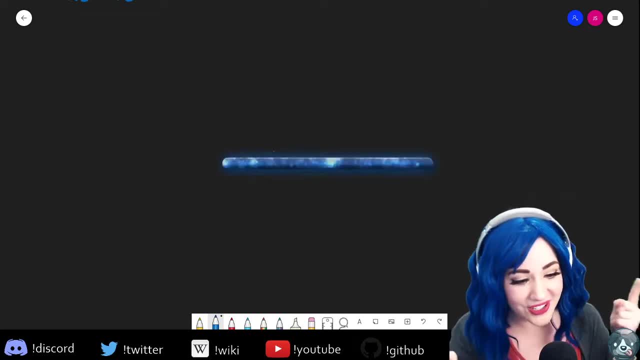 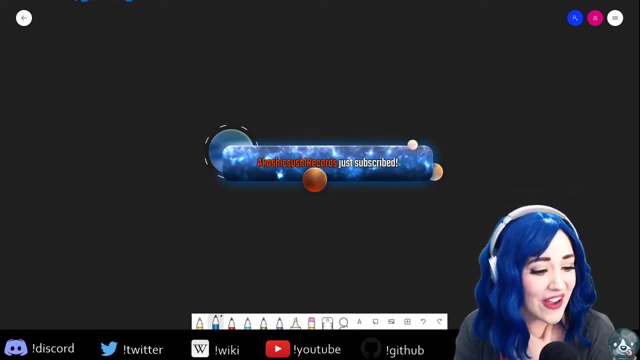 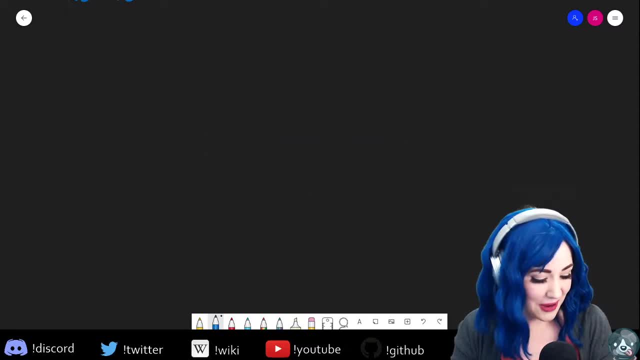 squish, we don't. we don't need a heart rate monitor. i'm actually not wearing my, um, my, my smart watch today, or i would tell you how absurd my heart rate is right now. um, i'm gonna crack my window. actually, give me a sec here, um, blushing overheats me, you guys. oh my goodness. well, now you have subs. 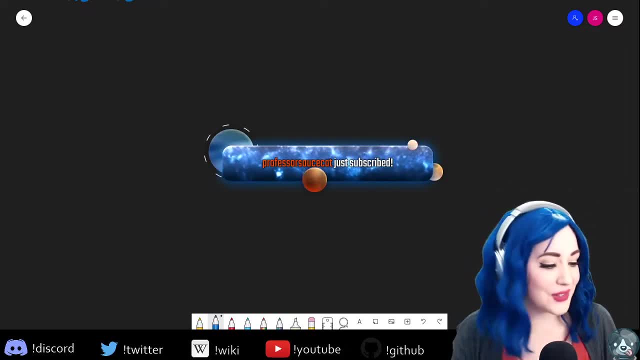 um and and soon probably more, even more, even more emotes. i'm working on them. i'm gonna just mute the alerts for now. they'll still pop up, don't worry. so you get all your shout outs, but that way we don't have the constant dinging um. but you guys a 283. 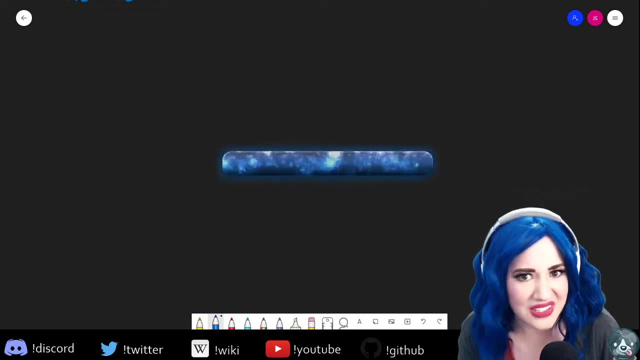 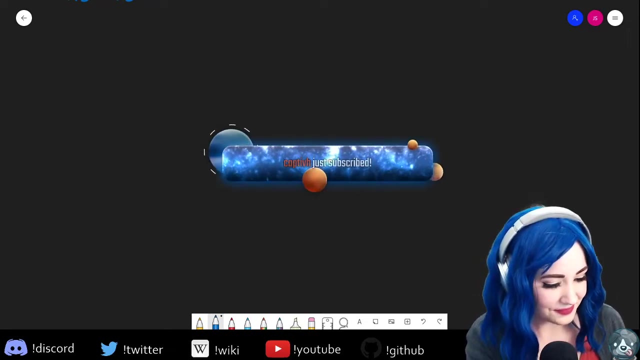 level five hype train. i'm still kind of learning what this stuff is um, but thank you, you are so, so, so wonderful. and third tier gaming. thank you, thank you, thank you. i always appreciate it. let's give, let's give you a shout out um third tier gaming. i'm like seriously losing my voice. um third tier. 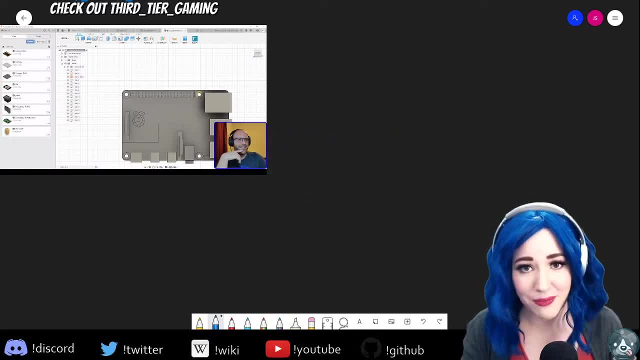 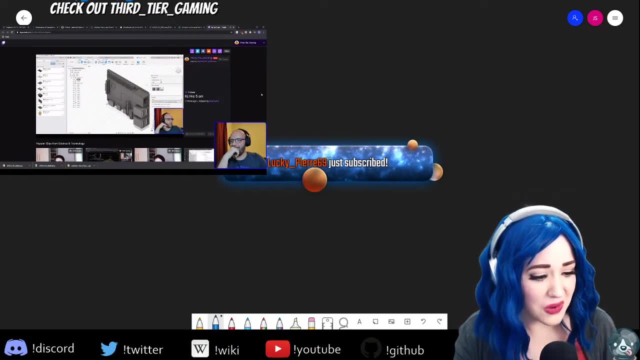 gaming streams. all about mechanical engineering, 3d printing, cool video games. you should definitely check him out, um. but let's see dj velour and punchy penguin. do you, do you all stream? can i give you a shout out? if you don't stream, no worries, but if i can give you a shout out, i would love to um. 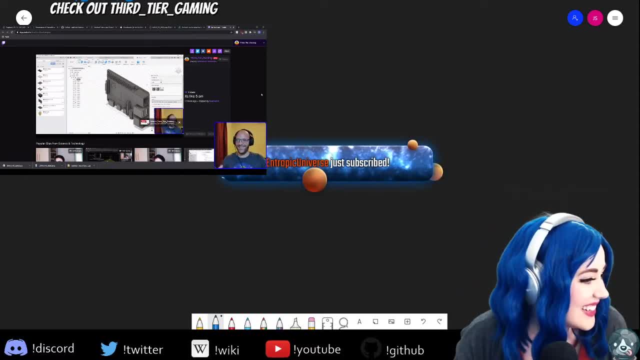 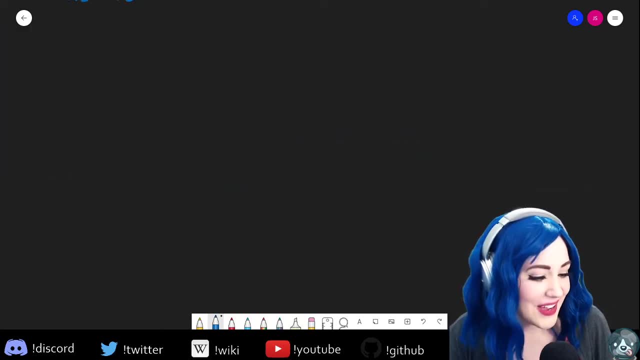 that is. that's such a good, such a good clip. third tier, to to pull for your pull for your stream. not yet. well, you let me know when you start streaming and i'll try to give you a rate, a follow and and definitely a shout out um both of you so. 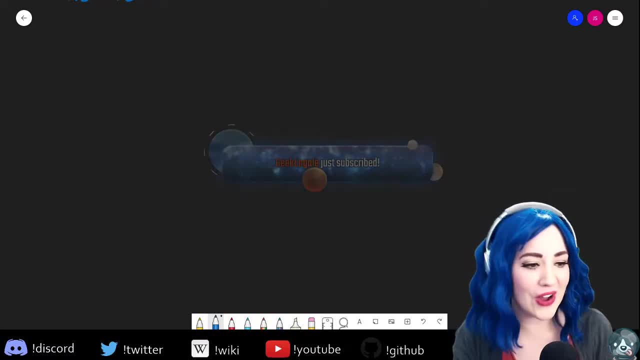 let me know when you start streaming and we will. we will pay forward all of the love um but r litchfield, thank you so much. thank you so much for uh for following. hopefully you'll be streaming um, streaming some science and tech. dj velour i'm for. oh my goodness, you guys. ah, okay, i can handle this like a mature adult. 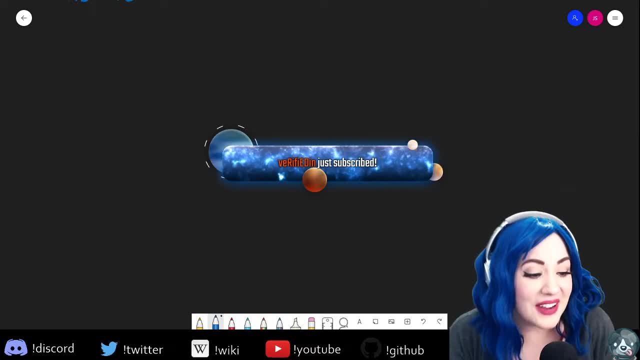 thank you so much. you've gifted 21 gift subs. i don't even know what to do with this, i don't know what the percent thing means, but it seems really cool because it's a really high number, and i'm so glad now that schwarzaq ally cat science streams alex warlock and. 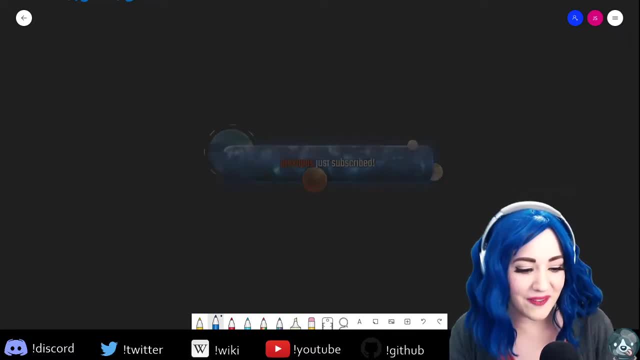 cesare, all have, all have subs. so now we're gonna have pog emotes for everything. um, i know ants 300. is there a level six? no, it says final level. keep the hype going until the clock runs out. okay, well, we have lots of hype. we have lots of hype. 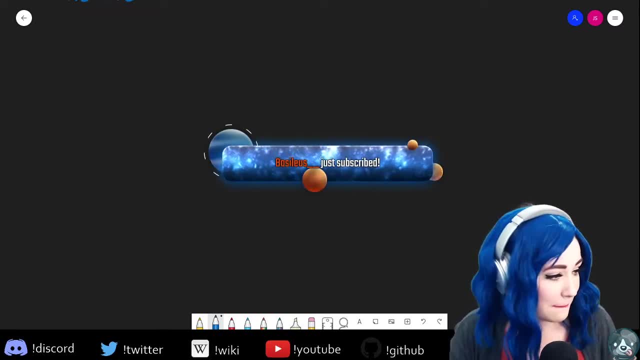 twitch, we have the, we have the hypest of hypes and ir coder. thank you so much for following as well. um, but yeah, like i can't wait to see the cool little like, because i think i still have, i have these two: the little like wizard one and the little like potion one. so we've 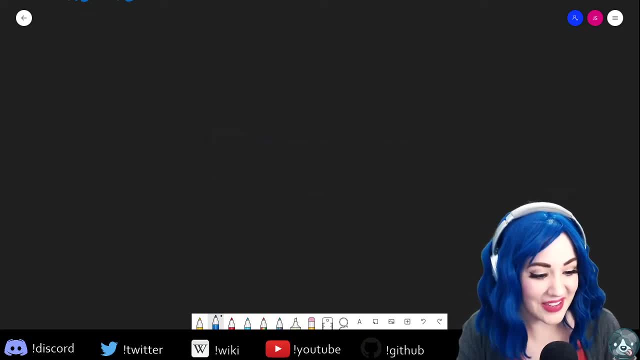 got. we've got lots of cool, lots of cool hype emotes. i can't wait to see what we get this time though. um, but thank you all. look at that, yes, look at this. we've got um, we've got all these different ones. such strong support level five completed. oh, my goodness. 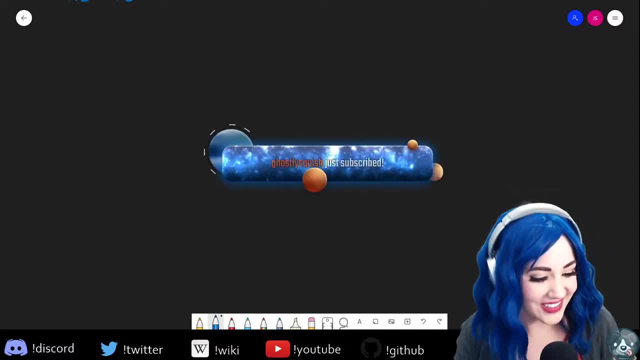 yes, you all are so wonderful. thank you. and look, i like the little sleepy one, i like the the sleepy, the sleepy hype one. that's very accurate for me: 90 of the time. and now everybody is a sub, almost everyone is a sub. wouldn't that be nice? and yeah, lucky pier. i'm so glad. 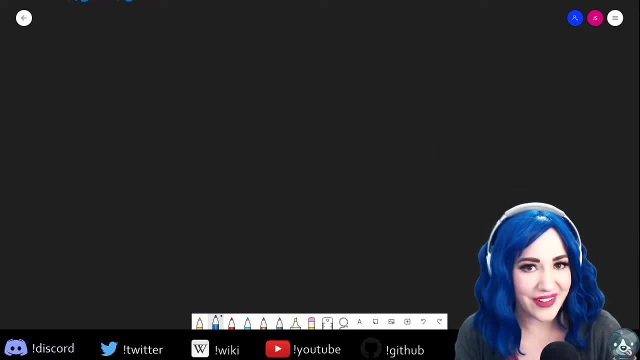 i'm so glad you're here and i'm so glad that you you have um, you have a sub now. and thank you, punchy penguin, i'm, i'm trying, i, i like, i like teaching you all, i like helping everybody learn math or science or whatever. so i'm the. the support is greatly appreciated, thank you. 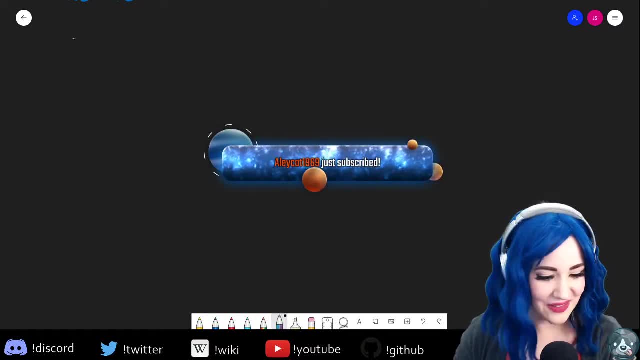 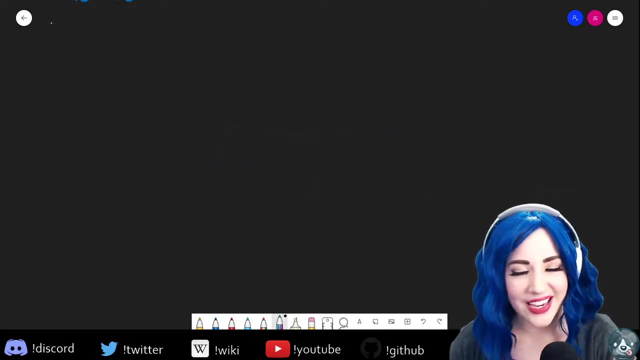 i almost didn't stream today. now i'm very glad that i i didn't give in and i was. you know, i got stuck reading a book- which has been happening to me a lot lately- where i just like i get hooked on a book and i don't want to put it down. i'm just like i don't. 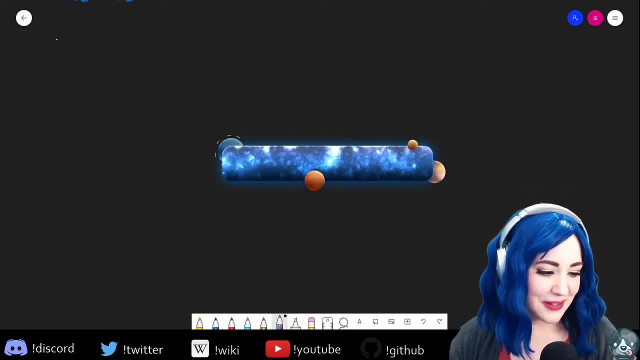 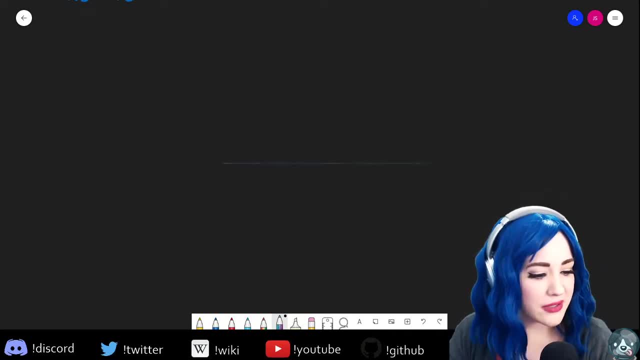 i was making a face at something um punchy penguin. so i guess netflix- i think it's netflix- is doing an adaption of this series. i think the first book is called shadow and bone, so it's kind of like a fantasy series. um, but i was, i was raised russian, so my half, my family. 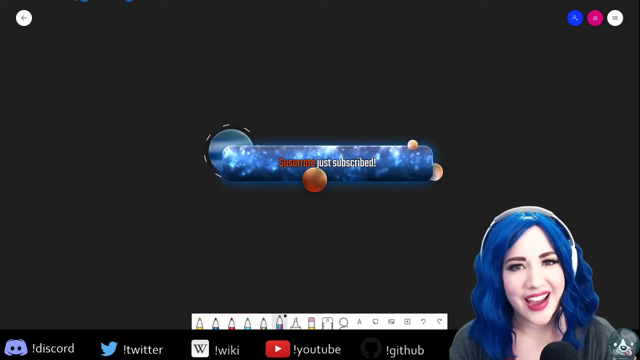 is actually ukrainian, so i'm a russian, so i'm a russian, so my half my family is actually ukrainian. um, but the cool thing that i that attracted me this fantasy series is that it's not like based on medieval europe, it's based on like imperial russia, which is just kind. 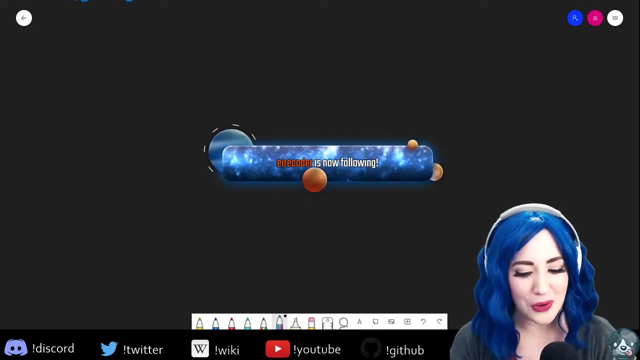 of cool, because i don't see that happening a lot. um, and so i've read book one. did i read book two? oh shit, what did i do? no, i think i'm. i think i'm in book two now, but i definitely accidentally read. i bought the book yesterday and then just read it and bought the second. 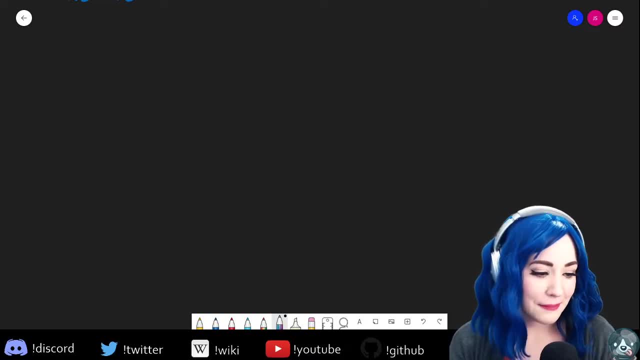 book and i'm almost done with the second book. so i was like, oh my god, i'm like, oh my god, i won't spoil anything, um, but uh, really, really cool. it's also weird to constantly read all these russian words. be like, i know what this means, but like it's all like mystical and 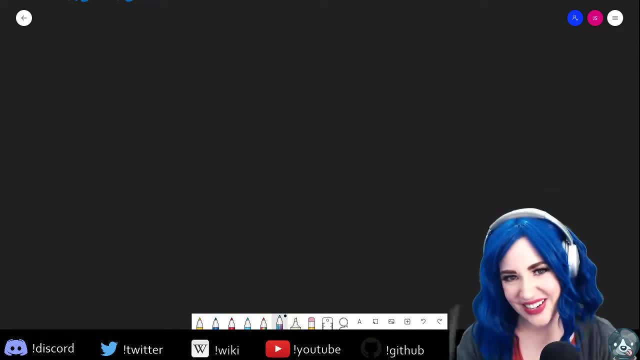 fantasy, um, and a hacker. yes, good, the grisha verse, exactly an aunt. so i've read. that's madeline miller, right? i've read her other book, cersei, and i actually have song of achilles, but i haven't. i haven't read it yet, so it's on my, it's on my list, um, one of my goals for. 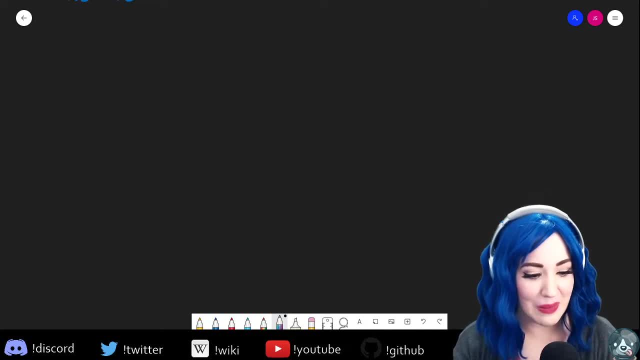 this year is to read a lot of books. so i'm gonna read a lot of books. so i'm gonna read a lot more books. so i have a giant stack next to my bed, um, and i'm just trying to like, read as many books as possible, and my goal is not just to like, obviously i'm gonna read. 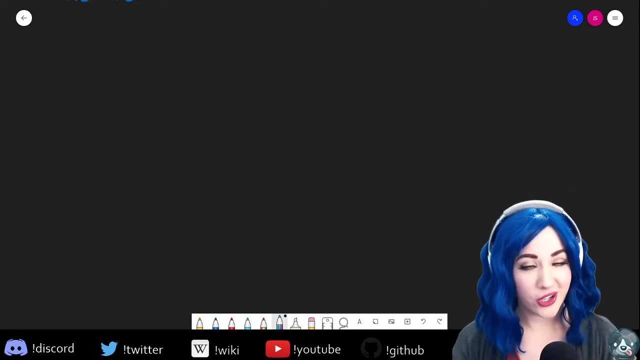 some quality books to, like you know, literature, but also, if i just want to read it and it's fun, i'm gonna read it. so, all righty, let's, let's, let's get back to um, to data science and machine learning, shall we? so let's, let's actually do a tiny little bit of a. 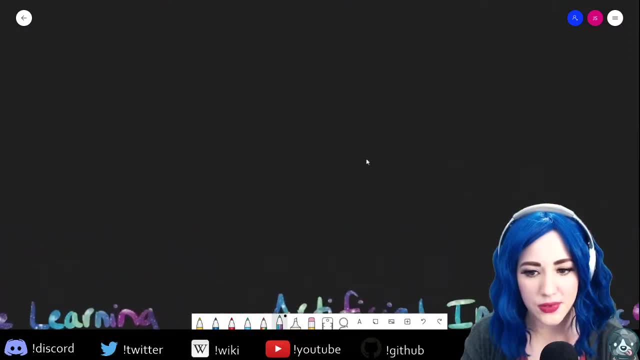 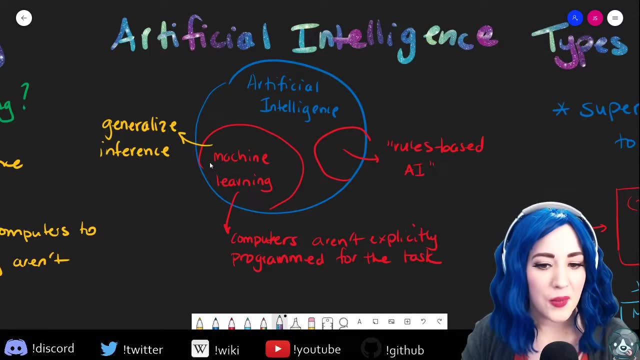 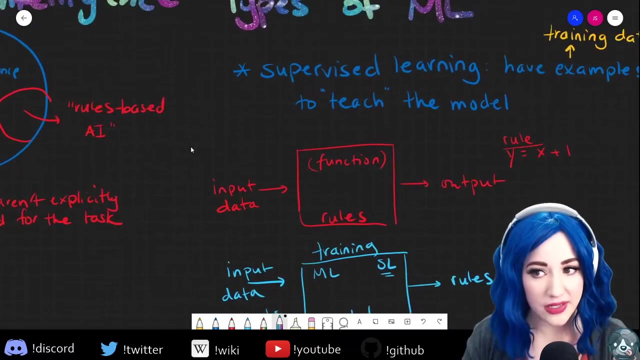 review. so so, so, so, so so. remember, remember, friends, that we're talking about machine learning, a subset of artificial intelligence where we don't want to explicitly program the computer to do the task we want it to learn. we talked about supervised learning, where we have examples to teach our model, unsupervised learning, where we don't have examples, and reinforcement learning. 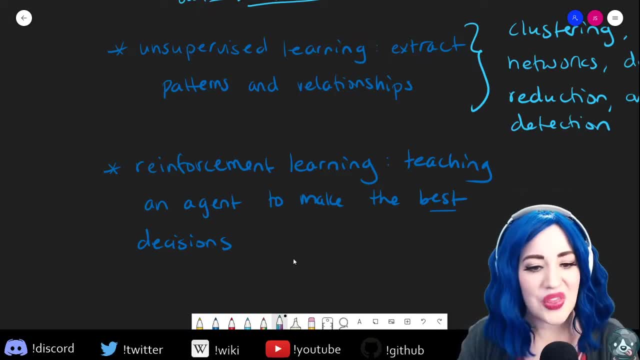 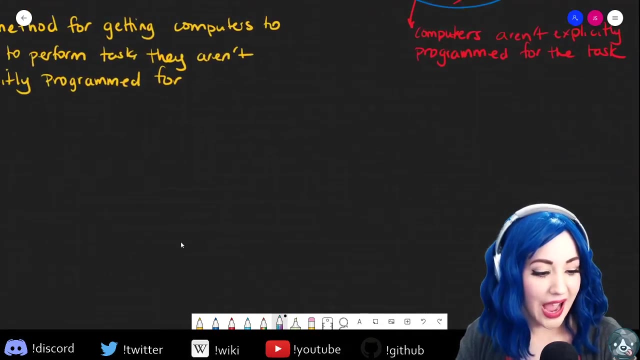 which is the coolest. i am very biased, but that's where we're more teaching. like strategy, we're trying to get an agent to make the best decisions, whether that's by following a particular strategy and optimizing that strategy, or by just trying to maximize the reward. um, i'm. 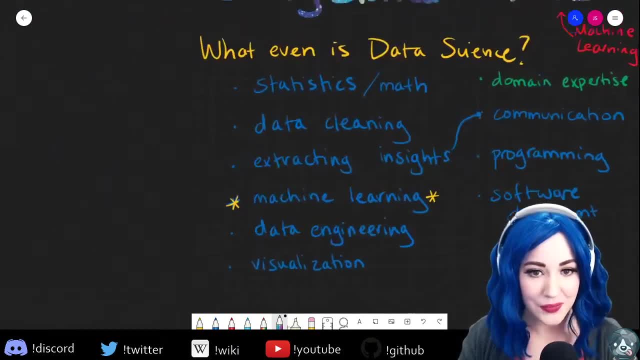 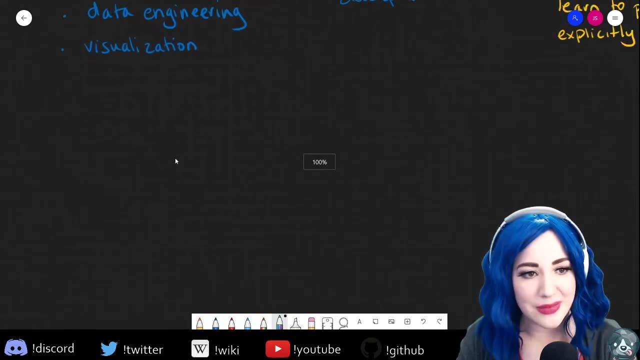 actually not from ukraine, lucky pr. so that's very sweet of you. um, i was partially adopted, so i mean my dad's my dad, like he raised me since i was five, so i don't think about it as like a stepdad. um, My paternal grandfather was born in Kharkov, and actually my family name, so like my surname, I guess my maiden name. 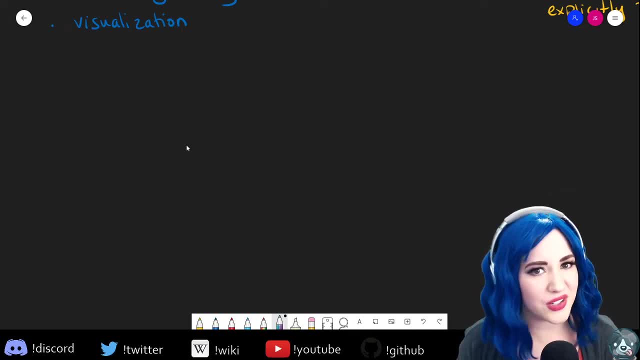 it's really weird, pre the disastrous marriage that I then got a divorce from, last name is actually a town in Ukraine, because my great-great-great-great-great-great-great-uncle composed the Ukrainian national anthem. 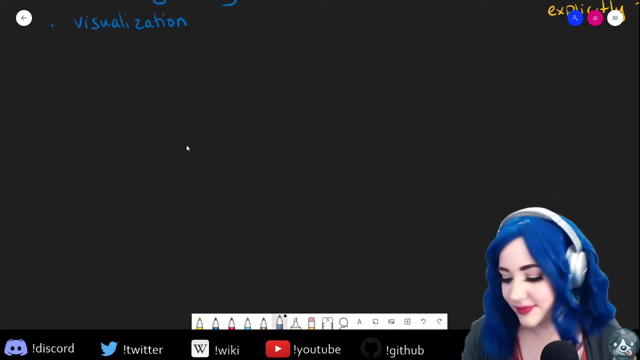 Um so, but there you go Um my like heritage, heritage that is like I don't know technical- is um Scots-Irish mostly, And uh, my biological father was, uh, uh, Indigenous American. so 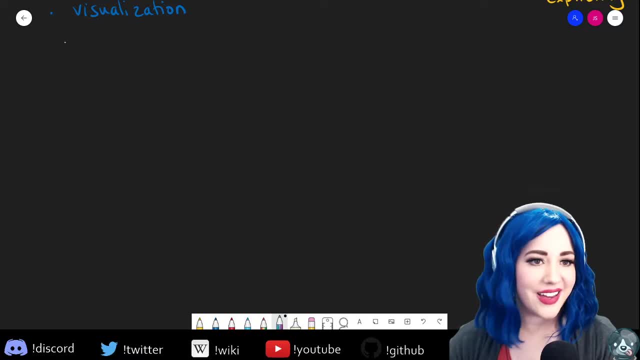 But everybody's beautiful, everyone's beautiful. I like that. Alright, let me see. so classification: we're we're talking supervised learning, classification. in particular, we're going to do a quick review of decision trees, woo-hoo. 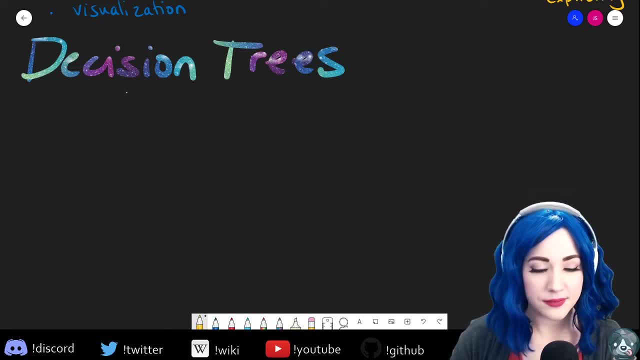 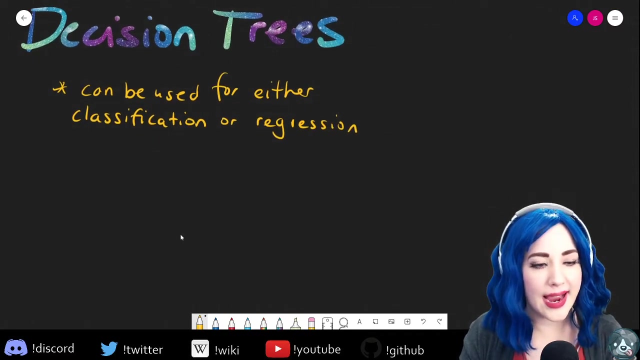 Now, decision trees can be used, let's see, can be used for either classification or regression, But today we're going to be talking classification, So we'll be using a, a classification, a decision tree classifier. Um oh. 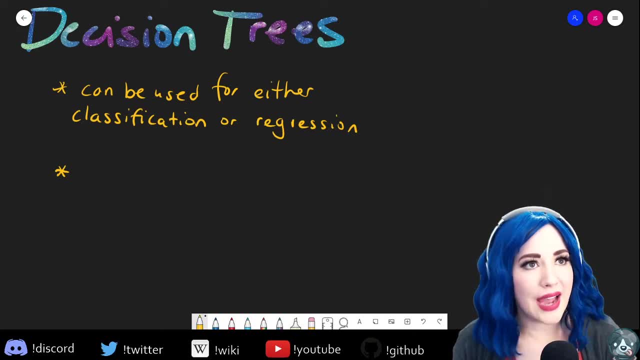 You're Navajo? Oh, okay, so my um, though like I don't claim this as part of my heritage, I was raised white um. it's not like. it's not something like I I put on applications or anything, because for me like 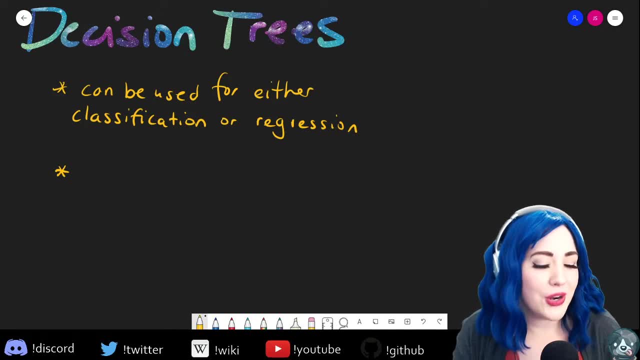 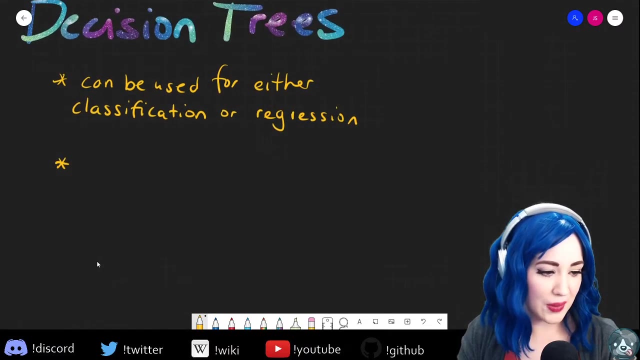 I wasn't raised in in that culture, but, um, my paternal, my biological father, is: uh, is uh Ute. so Alrighty And yes, what a great uh recommendations. so Punchy Penguin recommends that after you read 1984, George Orwell, 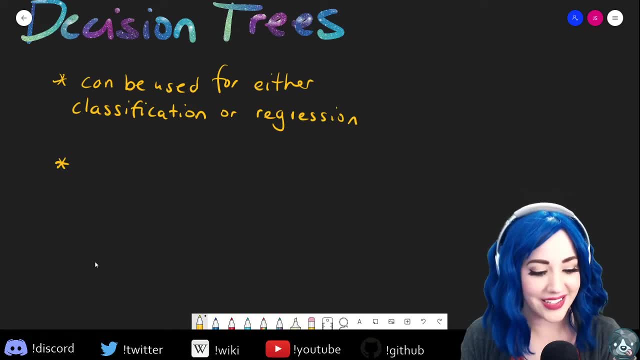 you should read Brave New World. I agree, I read those back to back and I liked that. Um alright, I liked both of them, but they were. they were obviously very different authors, very different literary approaches, But I liked both because they took very different approaches. 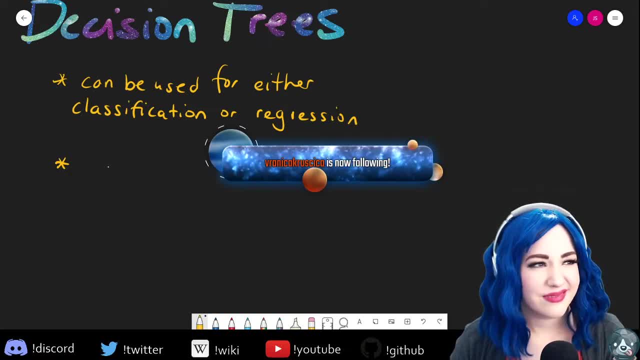 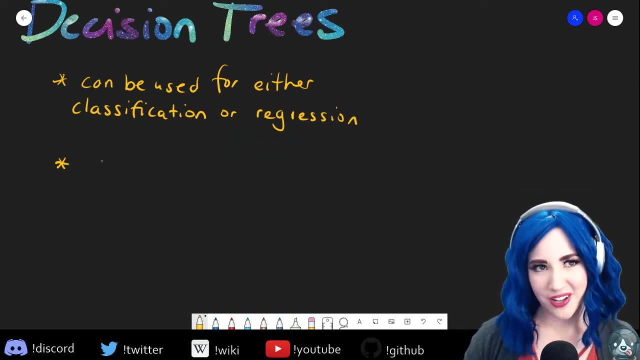 to showing kind of dystopia. So in any case, we should make an Enceladusaurus book club. I've always wanted to be part of a book club. Okay, decision trees- All right. who remembers something about decision trees? 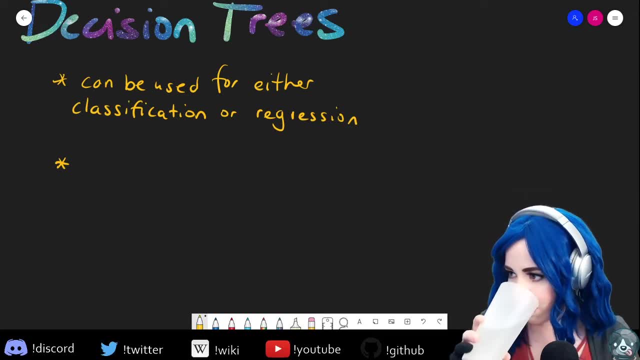 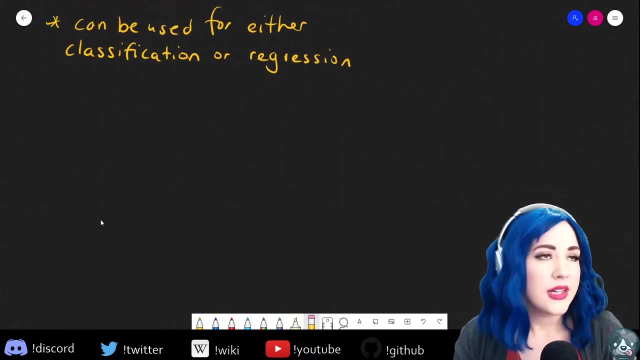 Does anyone remember anything? I'm gonna draw a little picture for you. Help jog all y'all's memory. And you know what I am. Ben, you say I like to read, but not for entertainment, rather education. So I think it really depends for me. 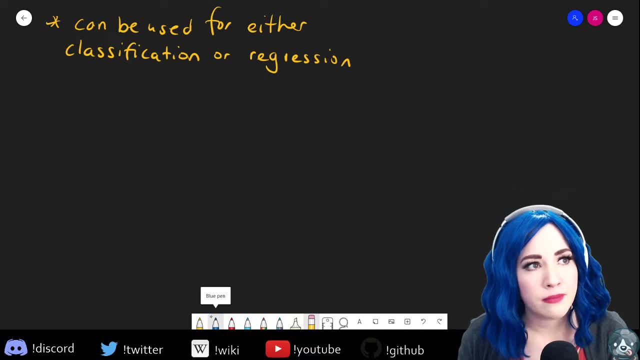 I spend so much of the day using my brain, like analytically so, learning things, teaching myself new concepts, reviewing- you know, reviewing things that I once knew. learning new things, math, programming, all of that that I read, not necessarily not education. 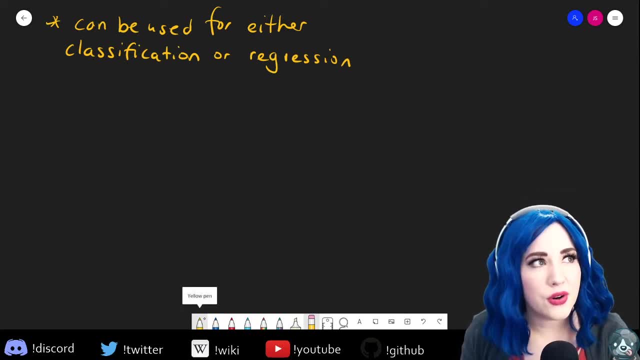 but just to kind of like I need to read something different. So I read stuff that is not machine learning, data science and everything. I love fiction. I particularly love science fiction and fantasy, but I read a lot of historical fiction I love reading. 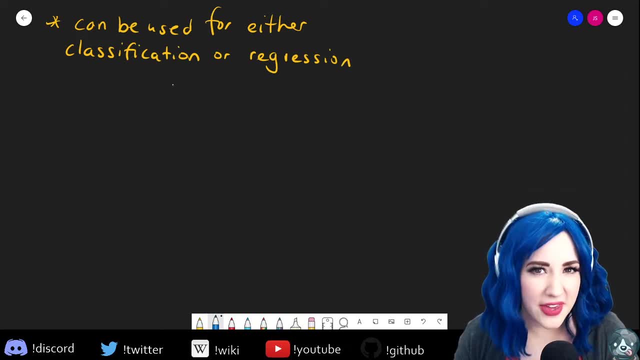 But for me it can still make me think deeply, Like I like to read stuff that makes me think. So it's not about like giving my brain a break so much as just using a different part of my brain, maybe. Okay, so let's see here. 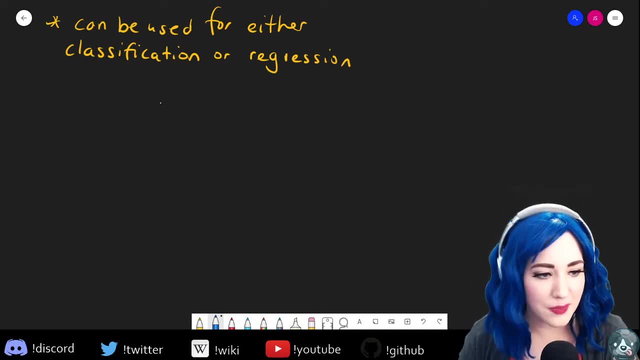 No third tier, That is the word that is banned on stream. I should add it to my auto mod: No black boxes here. No black boxes here, Actually. so, Ant, you say I've read, so I've read Ender's Game. 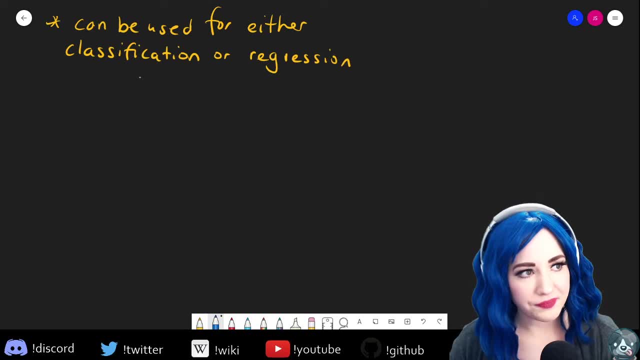 putting aside the horribleness of the author, I actually liked the second book in the Ender's series a lot better. So Speaker for the Dead, which also boggles my mind that such a like aggressively homophobic person could write. Speaker for the Dead. 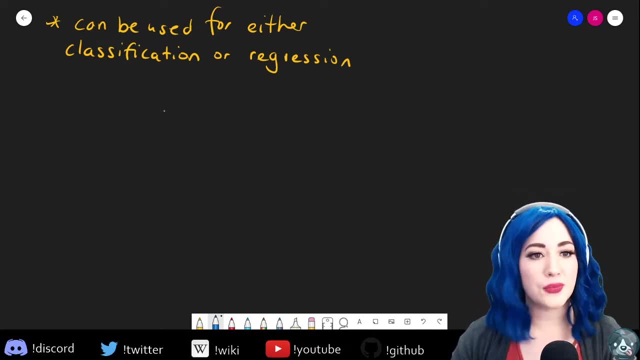 But I think sometimes art is greater than the artist. All right, so decision trees. Let me Why I love decision trees. It's for the soul, So tell me. tell me what you know about decision trees while I'm working on this. 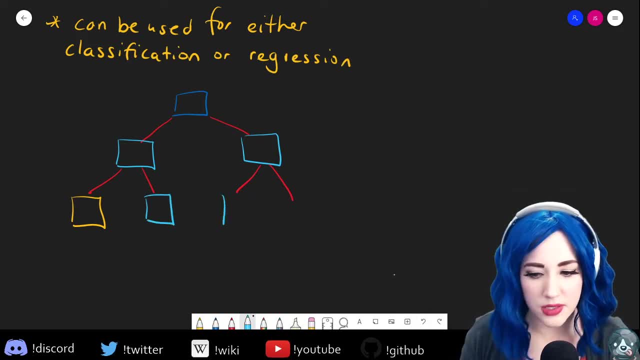 Who knows something about decision trees? Don't let me just talk to myself. silly folks or I'm stupid- is why don't I? Okay, okay, Yeah, Okay, All right, And I'm doing the different colors on purpose so we can label some stuff. 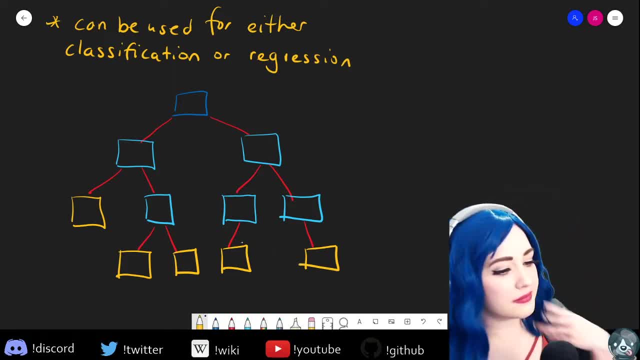 All right, so decision trees. Let's see here There are six books, I and Ben. they funnel info into categories. Okay, yes, so we can do it for classification or regression, And at each knot you make a decision. 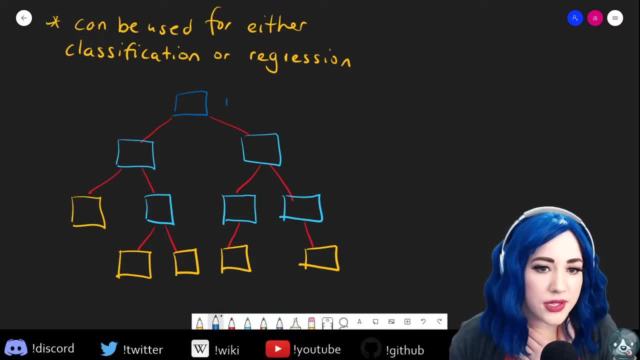 So these knots are called nodes. Okay, so this one is called the root, All right. And then these ones down here are our terminal nodes. You might also hear them called leaf nodes. So these are just nodes, And so you're absolutely right. 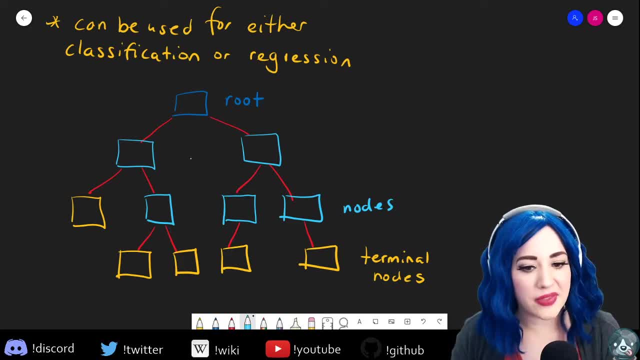 At each node, we make a decision about how to split the data, And these terminal nodes are often what kind of results in our classes, And so we have to make decisions like: maybe I want to classify my images. Let's go back to the dogs and the cats for a sec. 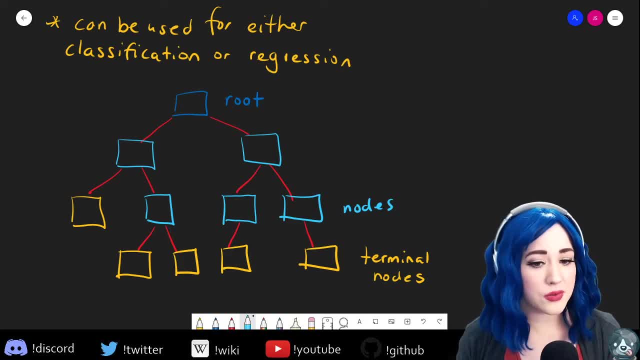 So I've got a whole bunch of images and I want to classify those images. I wanna tell if they're a dog or a cat. So what might we first split on? So we might first split on, like, the size of the animal, You know, maybe, like you know, 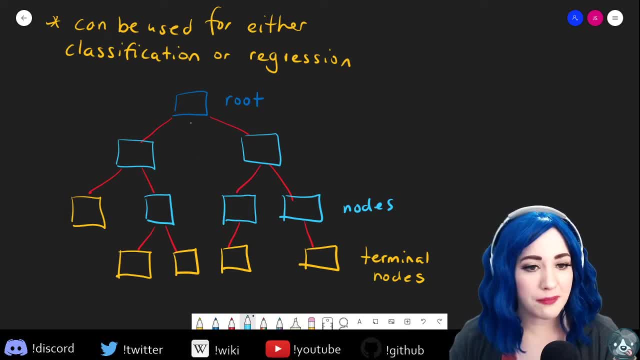 since dogs are often so much larger than cats most of the time, we might split first on size, Then maybe we'll split based on, like, ear shape or snout shape or tail shape, And you continue to split on different features, different inputs, until you get something. 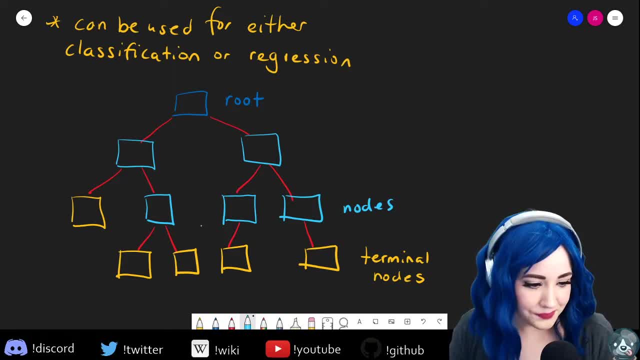 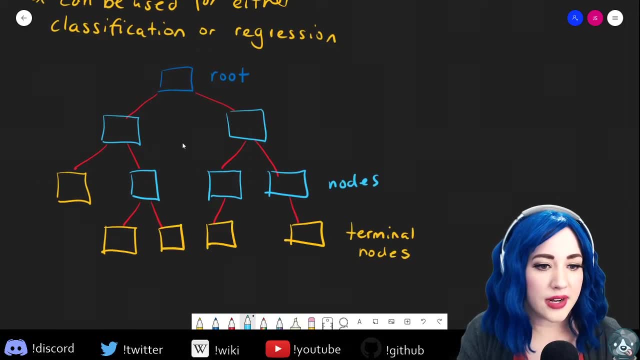 that is able to classify your data well. And to ask: does this relate to binary search trees and other tree data structures? Yes, it does. So it's not, I believe. ooh, I'm gonna get myself in trouble here. 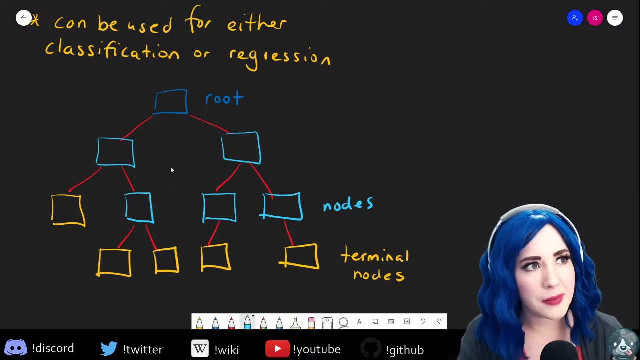 No, I don't think decision trees have to be binary, That is, I don't think each node can only have two, you know, child nodes. I don't think I often see them done that way, but I don't think it has to be that way. 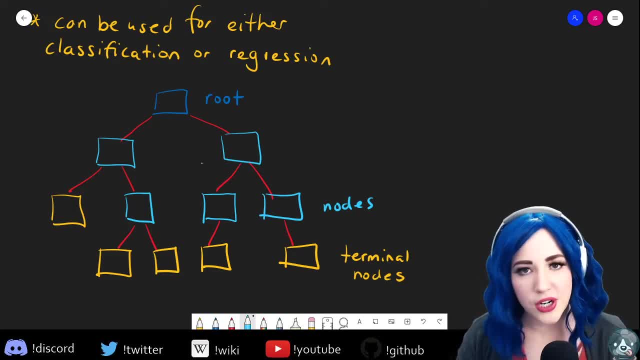 But absolutely So. a lot of the- you know data structures and algorithms approach to trees in general as a hierarchical structure for organizing our data. those apply to decision trees as well. Okay, so let's see here What do I need to read. 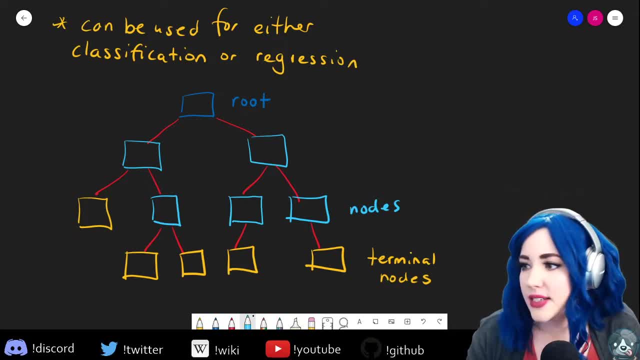 Review. Yes, and so a couple of things. We work from the top of the tree, So we start with our root, It's number one, And we work our way down. Is there anything else? We select a rule at each branch. 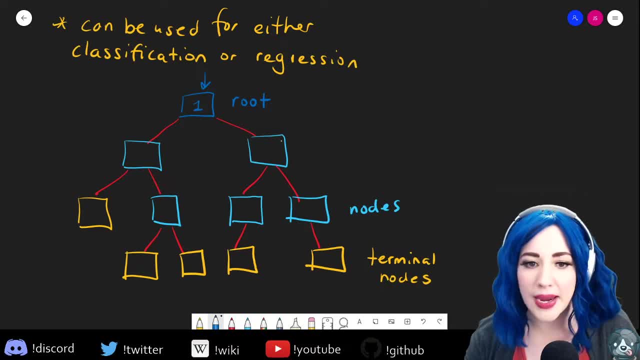 that splits the data into subsets based on a rule. Now, there's a variety of different rules if you want a deep dive into those. So these are things like entropy or the Gini impurity. Definitely check out the Machine Learning Myths video. 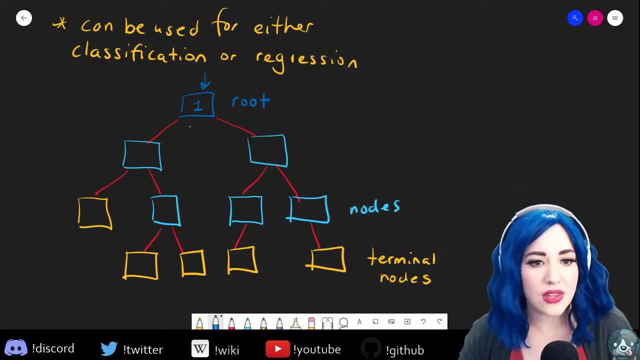 I go through the math for all of these, But suffice to say you can think about it. I think that we are splitting our data, you know, not just based on a rule like snout shape or something, but also because we're aiming to get that data sorted. 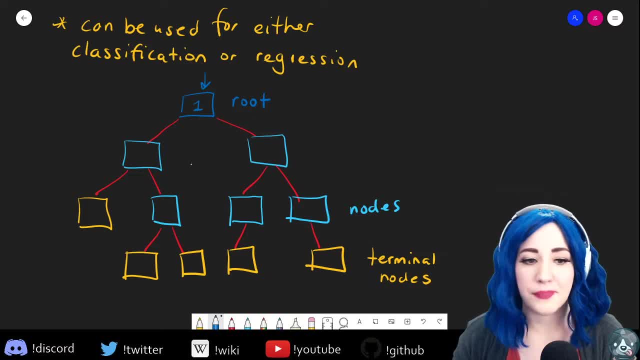 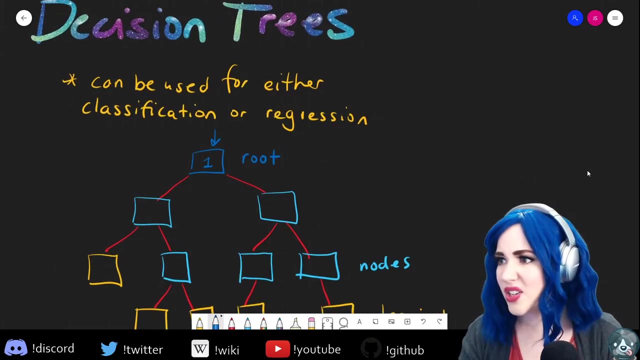 So we have different ways of measuring its sortedness- Those metrics I just spoke of- but a general understanding of how we're sorting it is fine for now. Okay, so let's see here Now. should I do it now? Eh, I'll do it later. 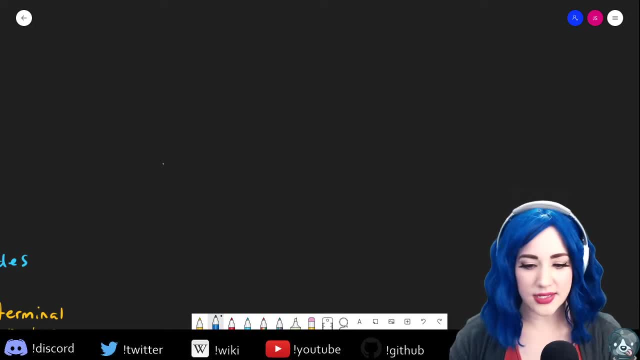 We'll do it later. All right, So if you want to take decision trees and do something even cooler- because decision trees have a lot of drawbacks- you might consider something called a random forest. Now, if you want to learn more about random forests, 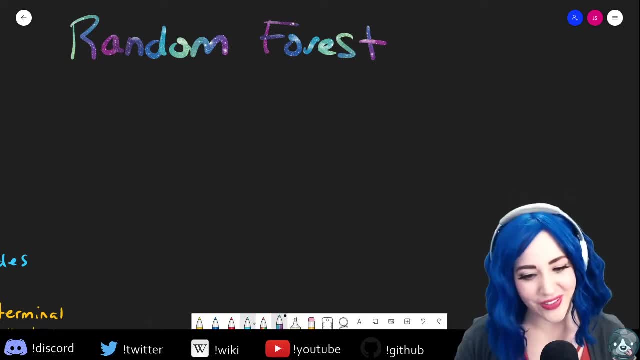 and do a deep dive into those. there's a Machine Learning Myths video on ensemble methods that I would definitely recommend, But for now we'll do another quick review. So this is a random forest, So this is an ensemble method, meaning that we're gonna take a lot of models together. 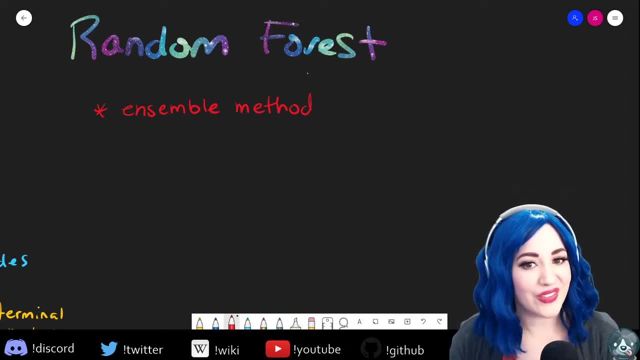 So, instead of just having one model, one decision tree- if the forest isn't a clue- we're gonna take a lot of decision trees, And so essentially what we do is we take a whole bunch of decision trees and we output, in the case of classification. 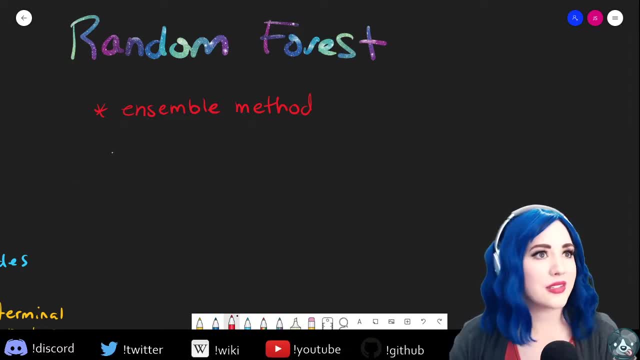 the class that the majority of those trees decide on. So we'll take. let's say we're doing our cats and dogs right. If 75% of my trees pick cat, then cat is the output of our random forest And 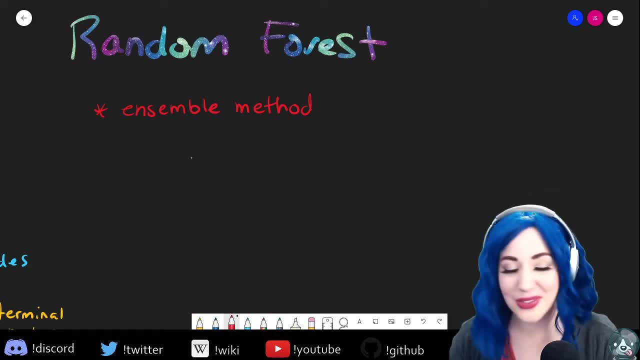 hi, looking for E-game ladies. I'm doing well. I'm so glad that you're enjoying stream. I'm doing well. It's good I've got tomorrow off And let's see. I'm sorry I had it muted. 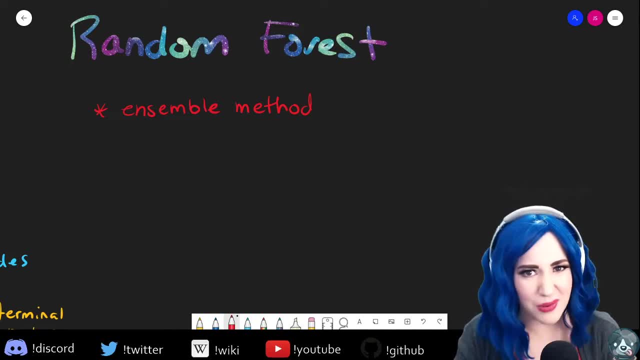 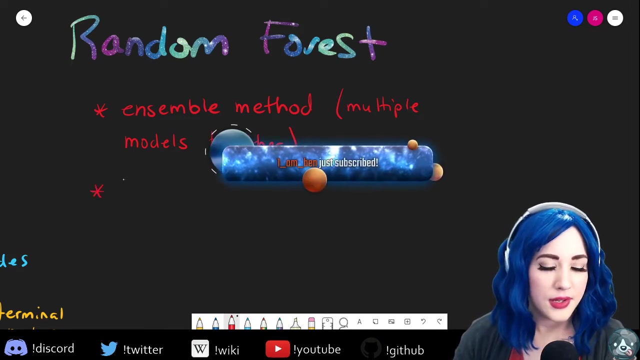 A Vranika Krusekika. I probably butchered that. Let me know how to say it right. Thank you so much for following and welcome to stream. Okay, So let's see Multiple, multiple models together And 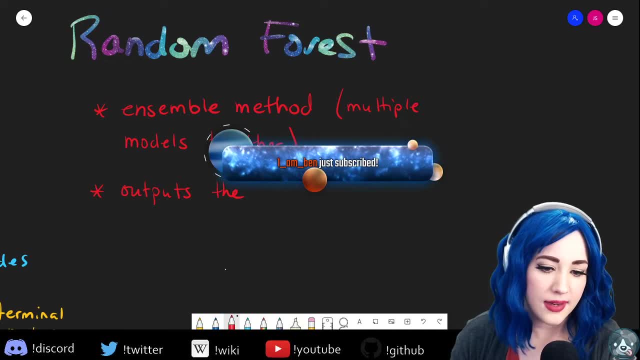 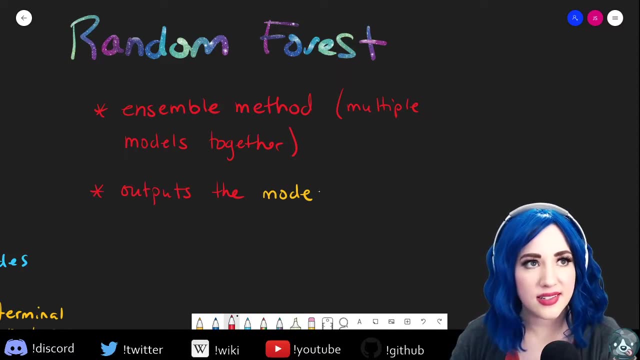 outputs the mode. if anyone doesn't know what that is, that just is kind of like the majority. So the thing that is is the most And Punchy Penguin. thank you for yet another gift. sub to. I am Ben Wonderful. 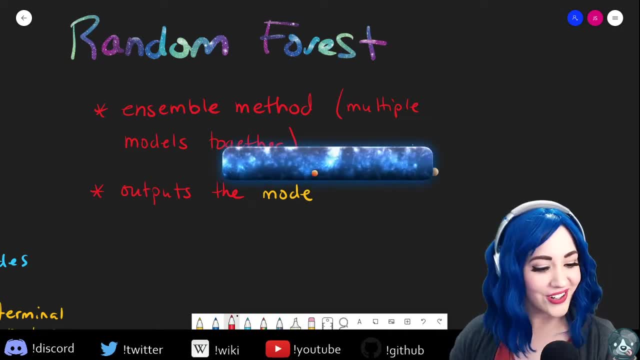 I'm so glad you can, and I am Ben. I'm so glad that you're able to understand it and that you're enjoying yourself and you're not, you know, picking a video game after over this. I appreciate it greatly. 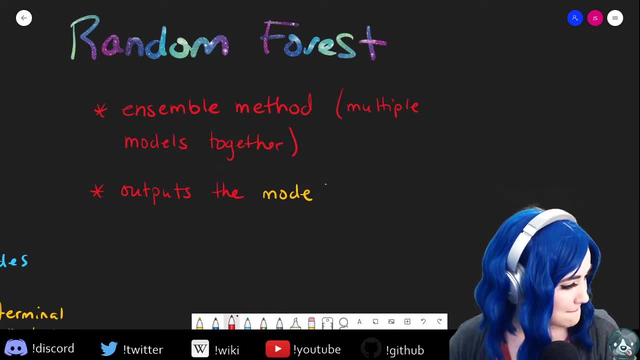 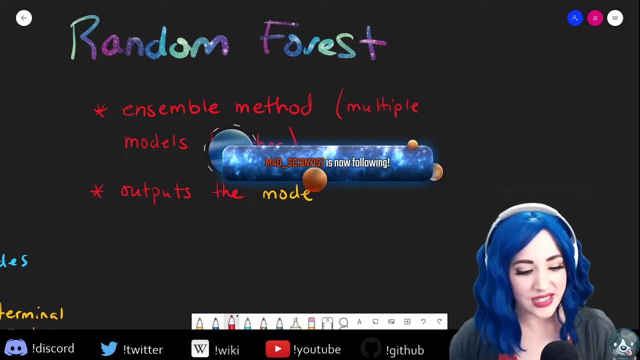 Melbourne. Oh, I will get this. Hold on Melbourne's Melbourne Slots. Man Slots, That's a guess. Thank you for following, As well as Mad Scientist- What a great name. And I know. happy Valentine's day. chat Spending. 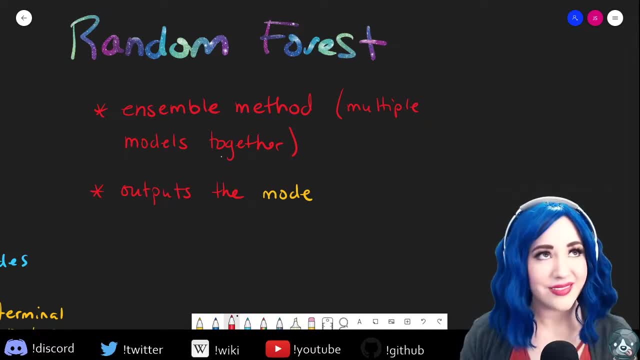 spending Valentine's day with my one true love: Machine learning and programming. Okay, So outputs the mode of. let's see the mode. How to explain this. It outputs the mode of the predictions. My dogs, Yes, My dogs too. 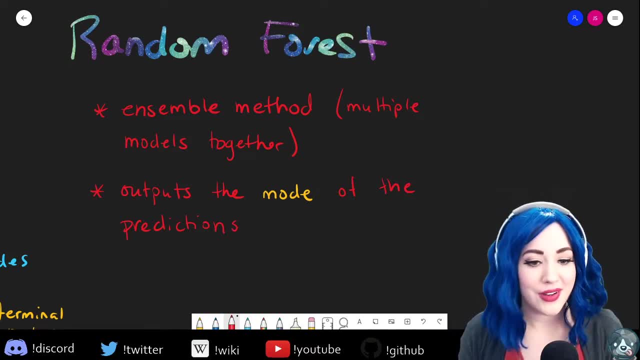 And, uh, I am Ben, So I'm going to ask: what does a sub do? So for you, a sub lets you, I think, skip all like ads and stuff. It also gives you access to emotes. For me it helps support. 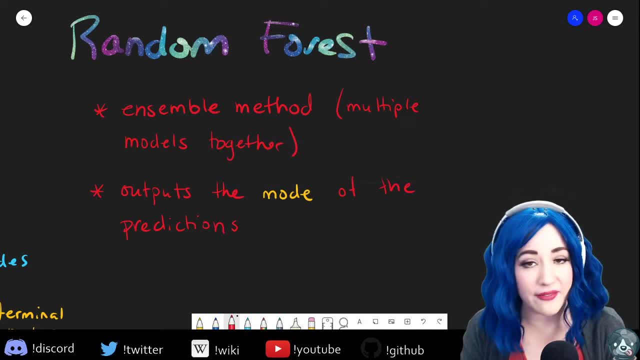 It helps support the stream. So a lot of times the revenue that I get from stream I use to get a better light, get a better camera. I got my green screen, my tablet, So if there are things like that that people want maybe another webcam. 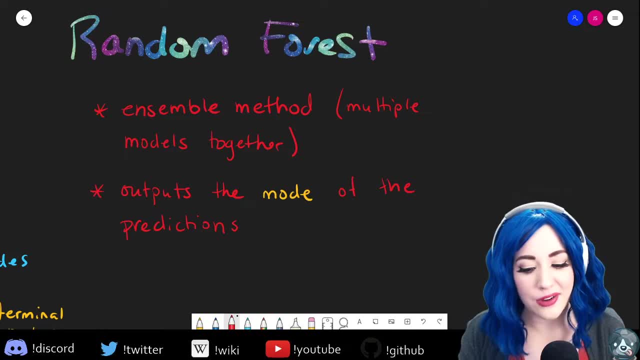 if we're going to do more like hands-on streams. So it allows me to get more things that make stream a better experience for all of you. Let's see, And um, loaf is at work. Sorry, loaf, Loaf is pulling a double today. 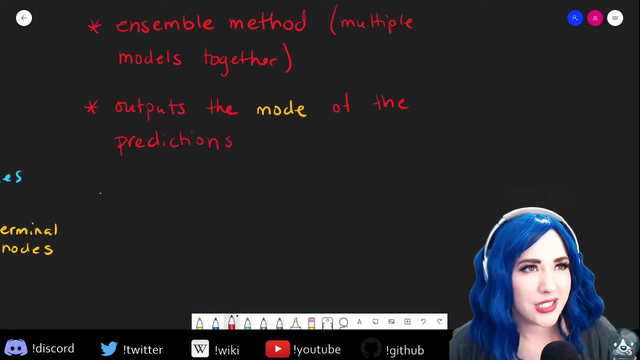 So poor loaf bone is working 6 AM to 11 PM tonight, Sad face, So sorry, sorry. And Apple two games save random force from the three. but I'm sorry, I'm sorry, Three body problem. Now here's. here's the question I got to ask is: 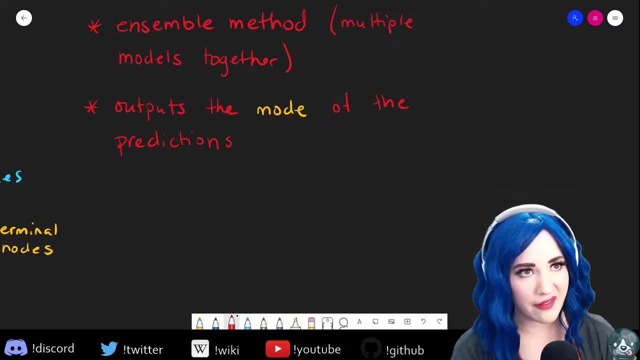 are you talking about three body problem, the gravitational physics problem? or are you talking about three body problem, the novel Um and what winner? and Hugh Cruz, thank you so much for following. Welcome to stream. I Apple two games. This is an embarrassing admission. 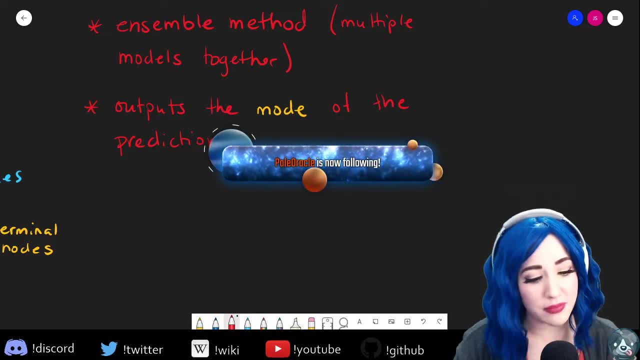 I've read the first, like fifth of that book, probably three times. I haven't finished it. So if you can give me more context I might be able to tell you. um, and let's see pale Oracle. Thank you for following. 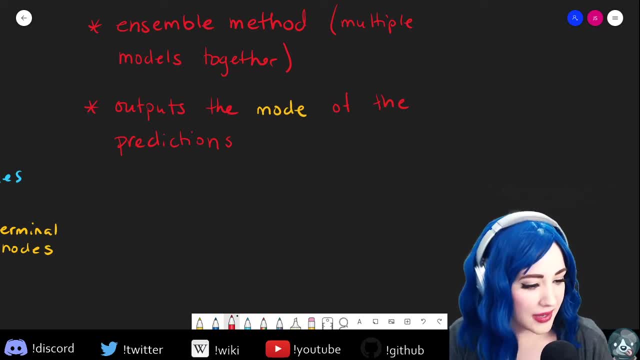 And let's see Brad attack. You say, Hey, you got me kind of an ML with my ML. Miss played around with MNIST data. Good, Awesome, Right now trying to classify beans on a self-made data set. This was awesome. 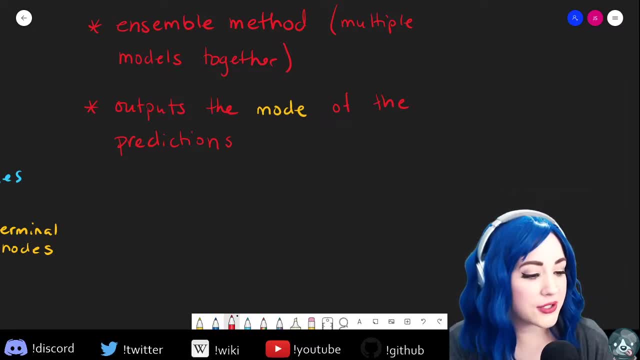 Um works great for just a few classes. Now I want to increase my data in classes. Any tips on designing such data sets in terms of size and split And quality of the picks itself? No, And your English is wonderful, So. 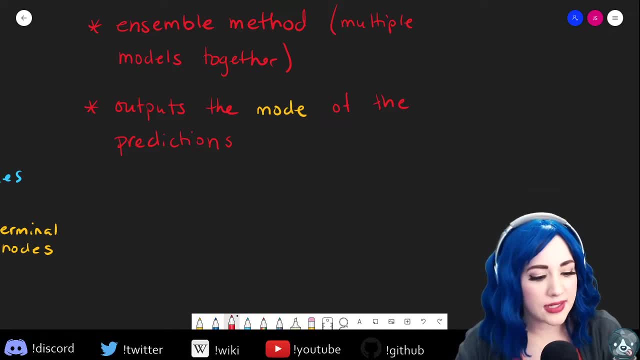 so you're dealing with imagery and you're wanting to add more classes. The first and largest concern when you're increasing your number of classes is class balance. So that's like you know. I guess you said beans, so I'm not sure what kind of beans you're talking about. 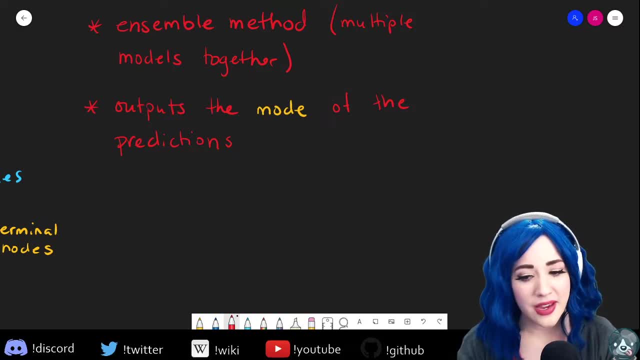 Um, but let's say, for my example about pets, that I have a data set of a hundred dog images and a hundred and 100 cat images and I want to add in ferrets. well, I need to make sure that I have, you know. 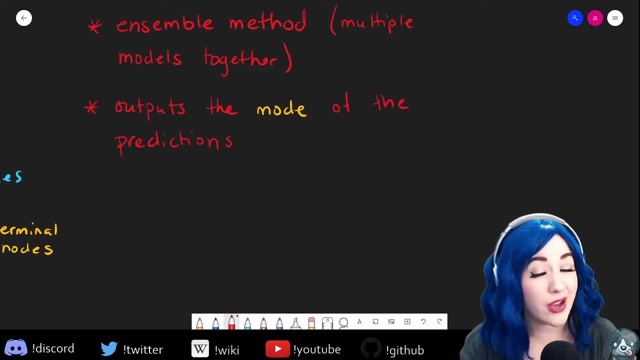 a good sample of ferret pictures, So hopefully, ideally, I would have 100. But when it comes to when you say designing such data sets, class balance is a huge one. I would also recommend kind of you have to think about things with images, like making sure they're either all. 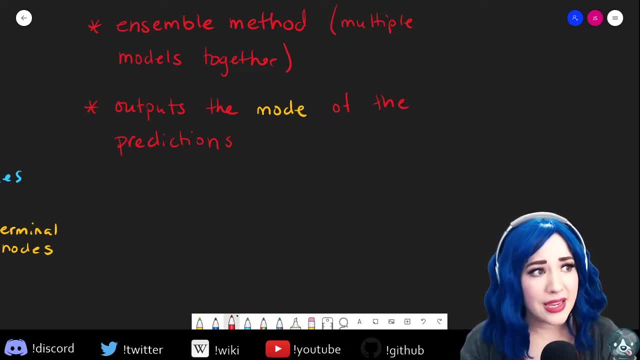 grayscale or all RGB, And making sure that there's- depending on how robust you want your classifier to be, making sure there's like a diversity of angles and a diversity of backgrounds. So I love telling the story, So huddle up, friends. It's story time. There was a classifier. 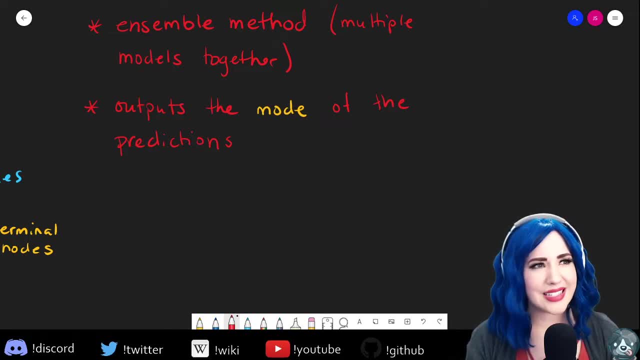 a computer vision classifier to identify dogs versus wolves, And I had- those of you who know how this story goes because I told it during machine learning must say nothing, But you know these- during the training, so they had their training data. 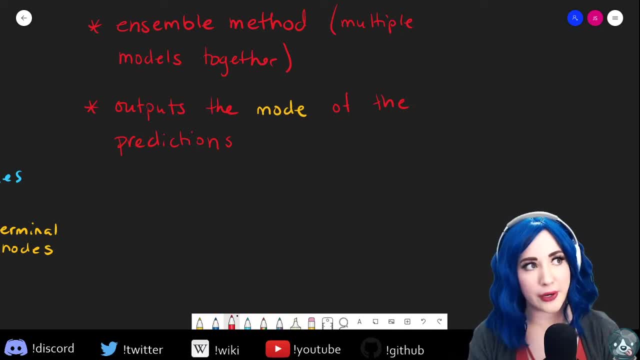 right. These are the examples that they're giving to the model to help it learn the difference between a dog and a wolf. Well, when they tested it- and usually this is kind of how it works- is you have? I'll draw you a picture. They have the data data from a particular data set. 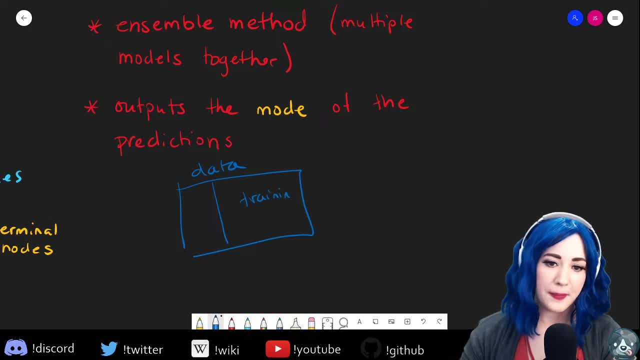 and you split it into your training data and your training data And you split it into your training data And your testing data And your testing data is data that you kind of hold back. You don't really you don't really show the model that And yes, you can do K-fold cross-validation- all that 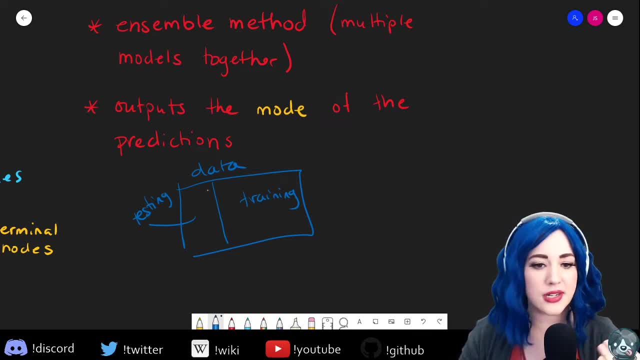 goodness, I've got a video on it, But right now we're talking real simple. We're just going to split it. We have our test data, our training data, We train on your training data and then you test it by showing it the testing data, which is new. But here's the problem: It's new-ish. 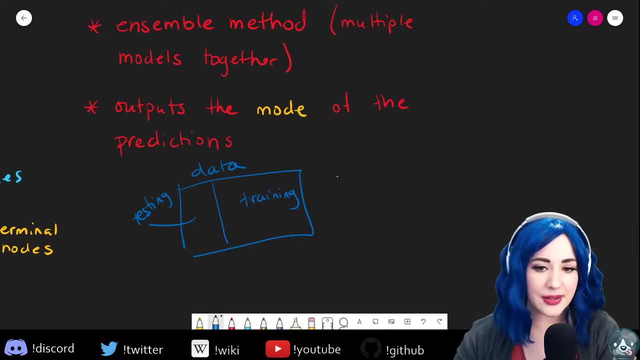 right Because it's from the same data set as the training data. So a lot of times you have another step that is kind of like your inference or your validation right, Where this is brand new, spanking data from like some other, some other place, And then you 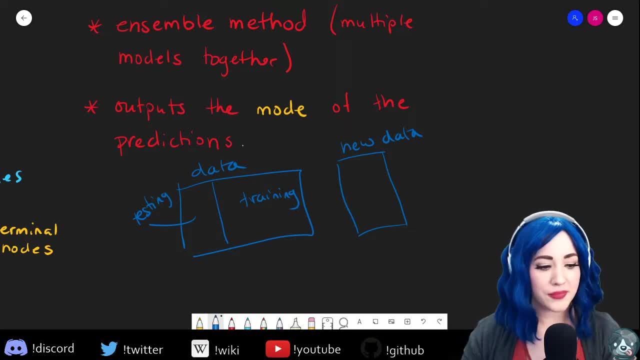 feed this to your model and you see how it performs. So they did a great job. They had your test train, you know great, Here's our wolves, Here's our dogs. Well then, then they fed it their, their, their validation data set And the model did terribly And 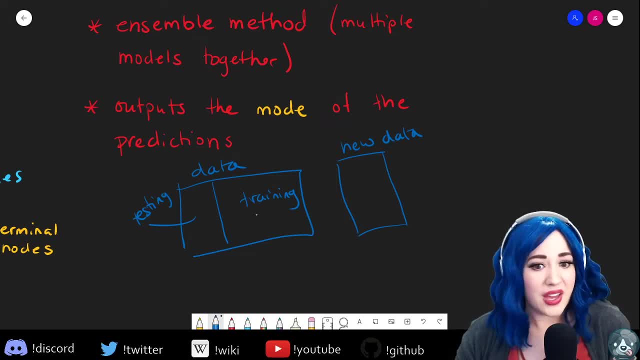 and they were trying so hard to figure out what was going on, Like: okay, it can recognize dogs and wolves in our, in this data set, but not in this new data set, And what they realized? what they realized is that the model had learned not to detect the difference between: 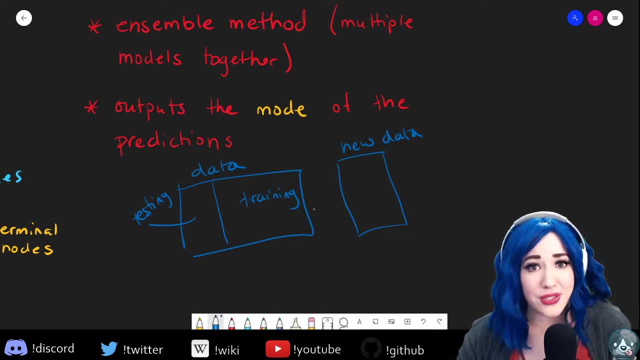 dogs and wolves. It had learned to detect whether or not there was snow in the background because in their data set the wolves were all photographed in snowy areas. So you have to kind of, you have to think outside the box when you're doing your computer vision data sets. 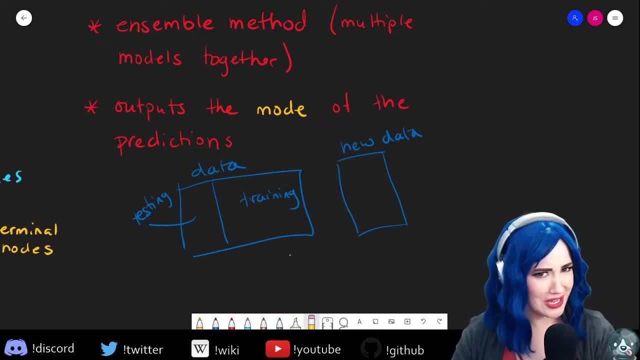 So, in addition to adding your new kinds of beans into your data set, I would also encourage you to make sure that you have different kinds of photos, different angles, making sure you're not all using the same, the same background, because you want to predict your kinds of beans, but not 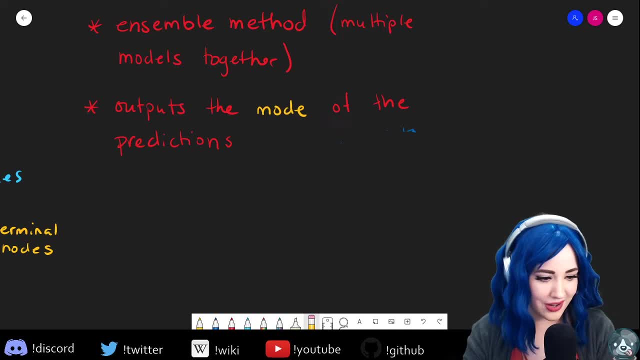 like having it overfit to like I don't even know what kind of beans you're talking about, But um, so let's see. here I'm catching up on the some chat questions. Have I read any David Brin? I'm really horrible with author names, Can you? 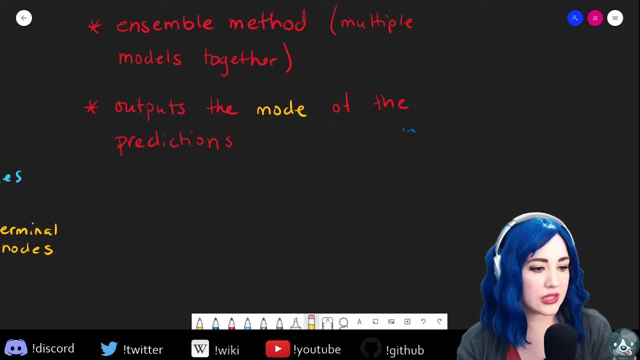 remind me what he's written. And, Ronan, you say lately you've been getting into D3JS and looking at how people use it to visualize data in a creative way. Oh, absolutely So. there's a lot of cool stuff you can do with neural nets and data visualization. Um, let's see. And oh yeah, 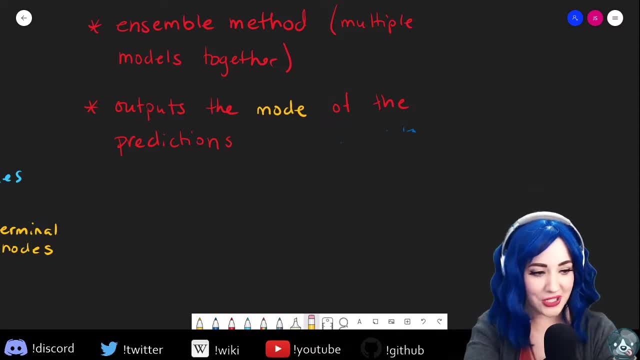 All right. So I am Ben, If you're new, if you're new to Twitch, feel free to ask questions. but yes, you can tag users using the at symbol: Um and Vaughn Wilmore. thank you for following Apple. 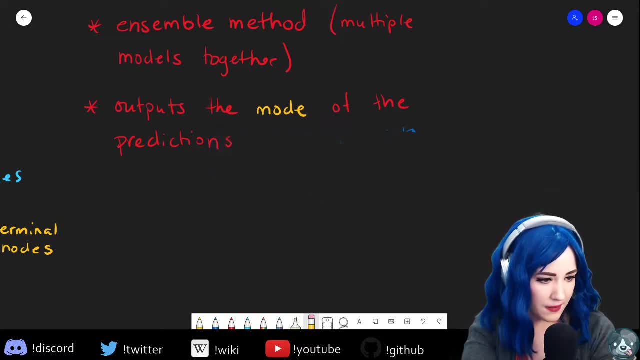 2 Games. you say long time, but um random forest states that we're far enough away from other life in the universe. If, say, another world was discovered, or they discovered us, that it's better chance one would destroy the other in self-preservation, Hmm. So this is a different. 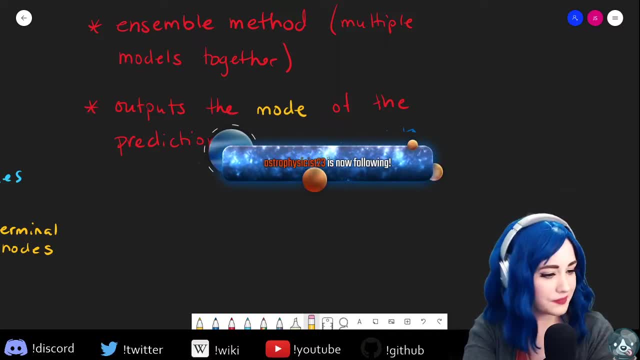 kind of random forest, but that kind of random forest sounds really, really cool. Dark forest: Okay, Slightly different. Astrophysicist 23. Welcome, You are in the right place for- for- uh, for astrophysics, Though I. 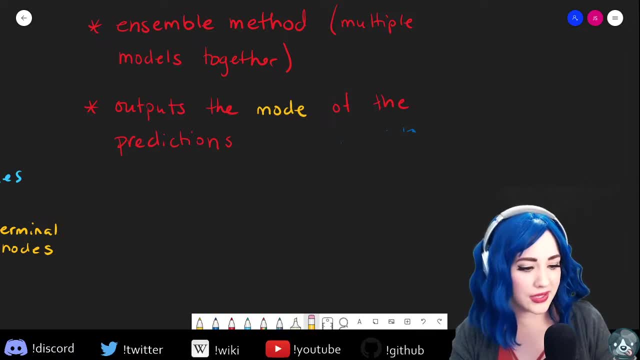 don't do that every science Sunday Sometimes. sometimes we do our astrophysics streams, but let's say um, let's see. Can I suggest an ML book to start this rabbit hole? So it depends, DJ Valour, So um. 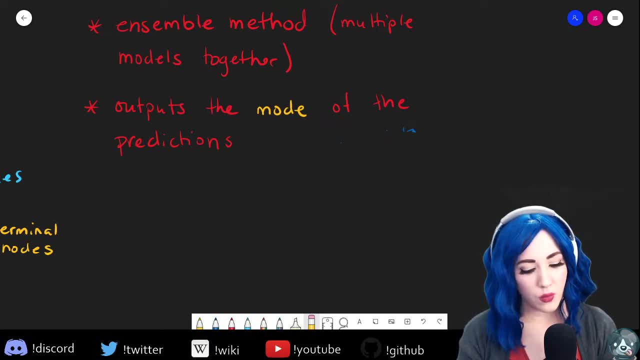 what? what kind of book are you looking for? How good is your math, How good is your programming? Really depends. I try to customize the books um for for, based on what people need. Okay, So we've talked to random forest and ensemble, ensemble model. We're going to stick a bunch. 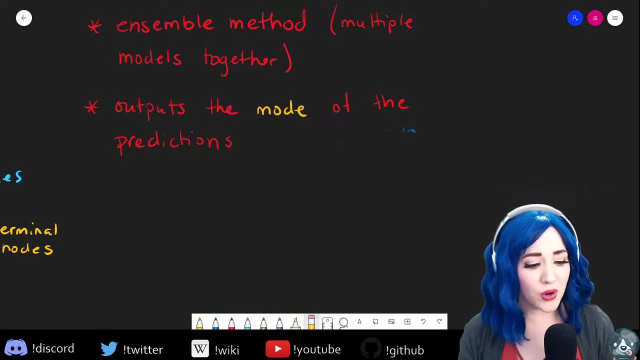 of these decision trees together and essentially have them all working in Tamble, in TAM, in TAM, in tandem as an ensemble. I need to slow down to Dr Lengthy. Thank you for following Intermediate math programming. What programming languages do you know, DJ Velour, Cause a lot of machine learning stuff is going to 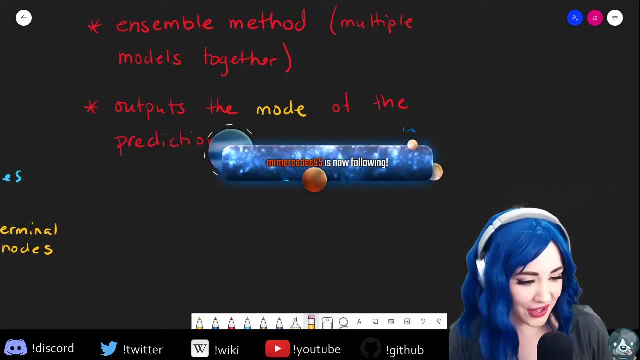 be with Python and M Mercedes. Thank you for following. Okay, Python, Good, Okay, So hit me up on discord. I can't say more, but hit me up on discord and I got something for you. All right, So outputs the mode of the predictions. Let me all, right, So do. does everybody feel like they're made of paper? I don't think so. I do not. I don't think so. I think we're pretty much. I don't think we're made of paper, but I think we're pretty much. I think we're pretty much made of paper. Let me just: I think so. 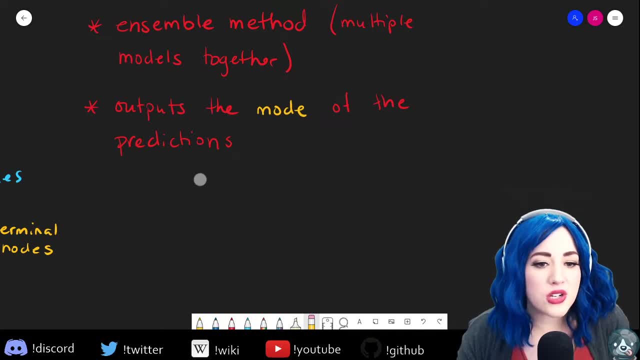 All right, So this, this, this is a technical dig, This is a technical dig. We don't know how that works. All right, so do. does everybody feel good with decision trees? conceptually, Like I said, if you want deep dives, I've got the videos. 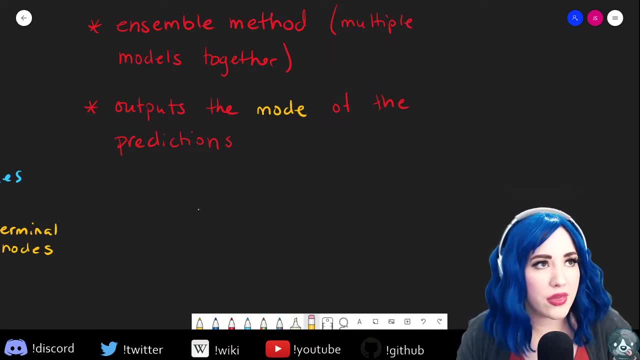 but conceptually does everyone feel good with decision trees and random forests. before we move on to the cool stuff- And Ant, I have not. I have actually not seen Haskell, So there are some. definitely like there's a smattering of languages. 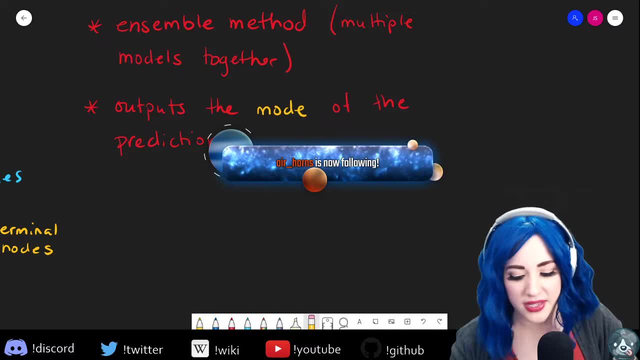 that you'll see used less frequently. So the biggest one is Python. Then, like you'll see a smattering, So you'll see Julia. you'll see C- sharp even So, but like Python's the big one- And Airhorns. thank you for following. 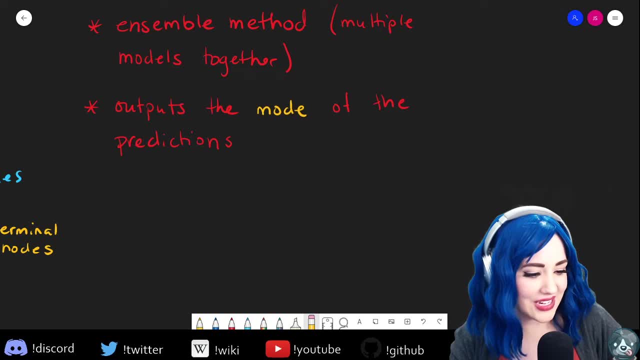 Let's see after learning how AI works. were you bummed about the idea of AI having a consciousness? Was I bummed, I think? like I don't know? I take a very kind of like Star Trek approach where, like 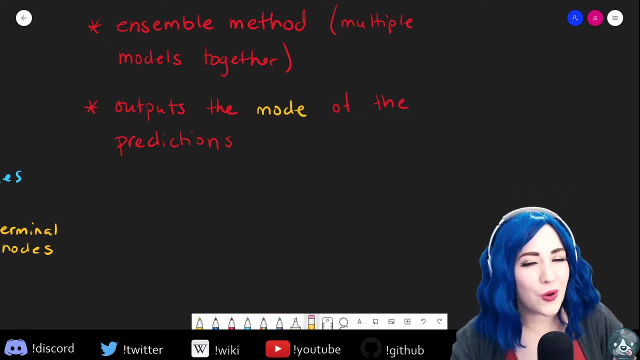 if artificial intelligence acquires sentience, I think that would be really cool, but we need to make sure that we afford it all the same. Well, we're not very good with human rights, So we need to get better with human rights so that when we have artificial life forms, you know. 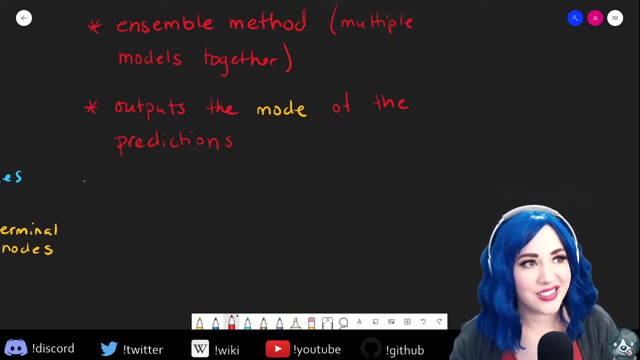 we got our innate natural like earth rights, shall we say, squared away. But okay, what is consciousness? Punchy Penguin, should we do a Daniel Dennett stream? Oh my gosh, I would die of happiness if I could ever interview Daniel Dennett. 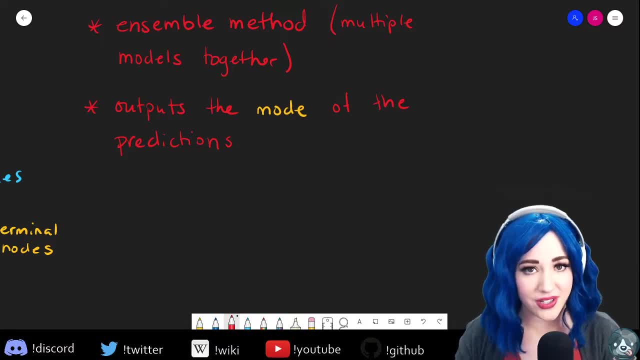 Anyway, all right, Speak now or forever hold your snoot. Is everybody good on decision, trees and random forest, before we move on and start talking about gradient boosted trees. All right, we cool. All right, Hi, Justice, good job. 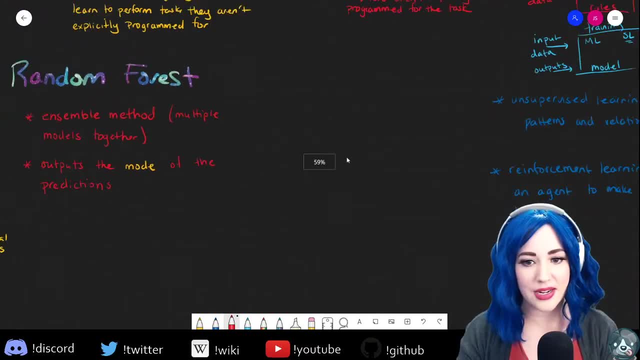 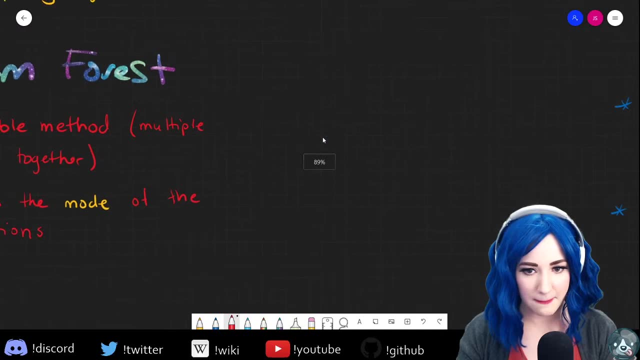 Sorry, I saw you say hi and I completely forgot to say hi back. Okay, I'm gonna need a little bit more space, So I'm gonna draw a really crappy picture of a bunch of trees here to fill the space. Oh my God, come on, there we go. 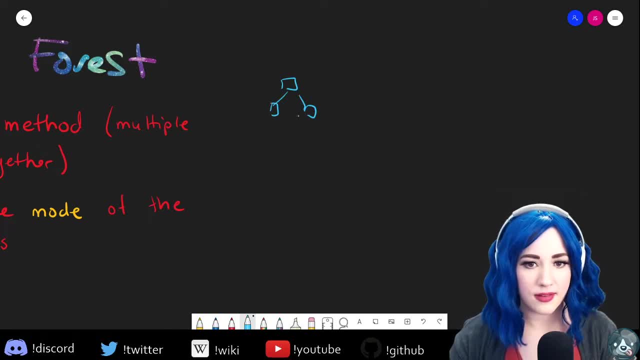 So we got got lots of trees. Maybe this tree does it differently. Oopsies, that's not a straight line. Lots of trees all working together. Look at that. Ha, teamwork. Oh God, I'm like getting so cliche here. 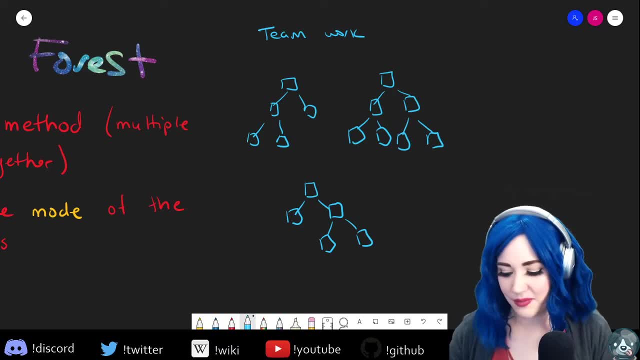 but teamwork makes the random forest work. Oh yeah, There you go, a little bit of a space Taking a little bit of a break. I don't know if you can see it, but it's a little bit of a little bit of a space. 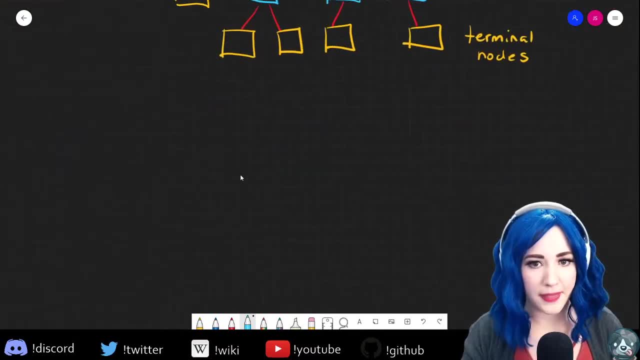 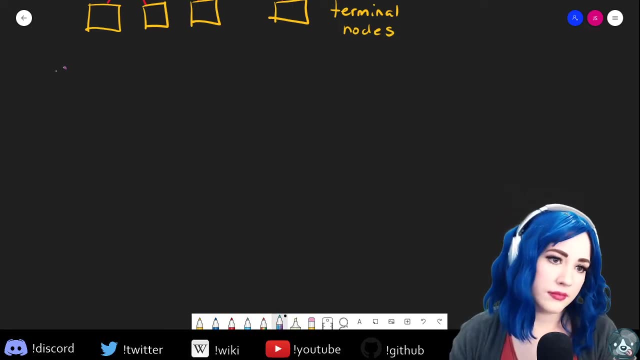 I don't know if you can see it. I don't know if you can see it. I don't know if you can see it. I'm taking up some space, Okay, so let's talk. Let's talk: gradient boosting. Gradient boosted trees. 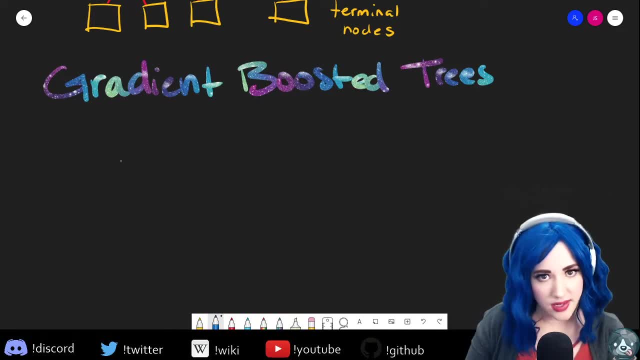 All right. so there's a lot here, There's a lot in just this, this title. okay, No worries, punchy penguin, Hopefully you don't miss the singing dog, Of course. Gradient boosted trees is the last, is the last theory concept I'll be introducing. 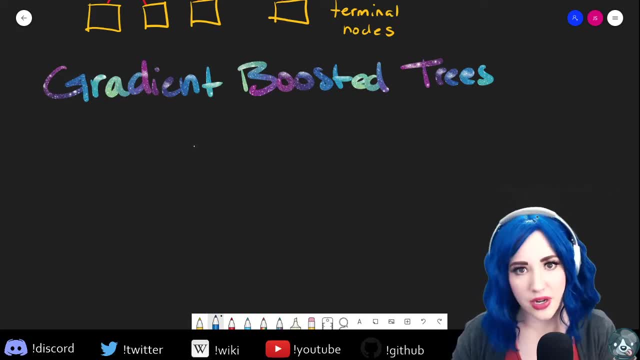 Then we'll switch over to code for a bit, but the code is really straightforward and it's more just kind of illustrative. I've got some data, visualizations and stuff And then we'll, we'll do some fun, We'll do, we'll do some fun dog singing for you. 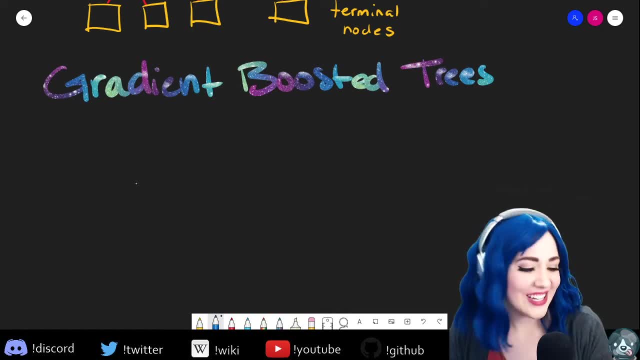 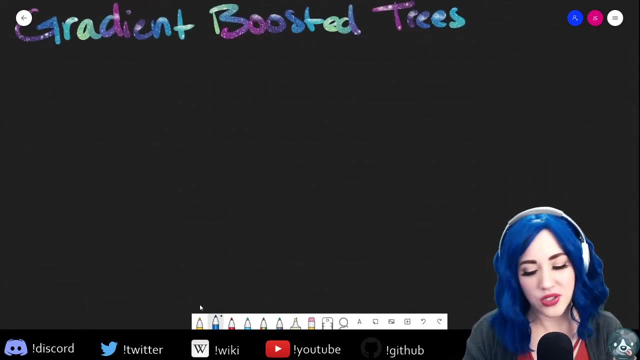 All right, An astrophysicist. astrophysicist, You say I'm taking an ML course right now with applications to physics. Cool Yeah, I've in. in my own astrophysics research I've applied ML a little bit, but it's, it's depends. 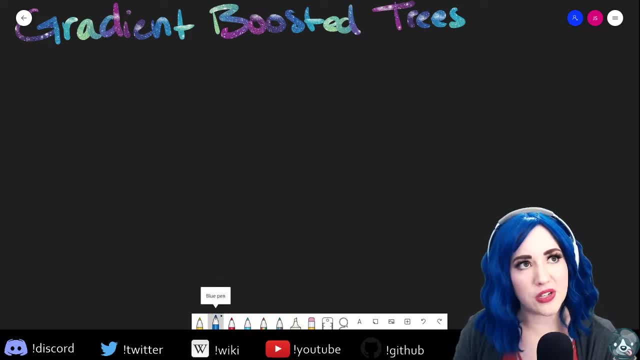 Like, I think, a lot of people, their intuition is that computer vision would be the place to go. but space, space is hard. Computer vision in spaces is extra hard. So, all right, Gradient boosted trees. So I'm going to break this down for you. 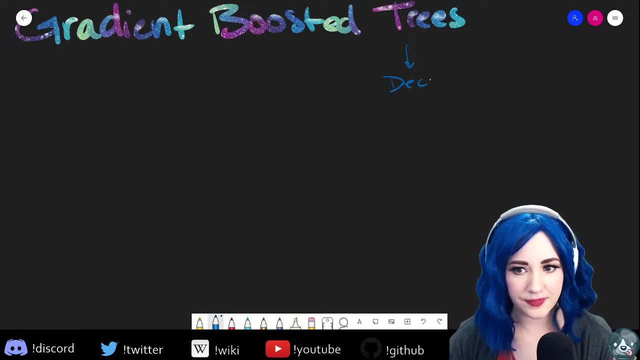 Trees you should feel comfortable with Decision trees, Now boosted. what we're referring to here is kind of it's kind of like random forest, but totally different. So instead of taking a whole bunch of trees and having them all independent from each other, 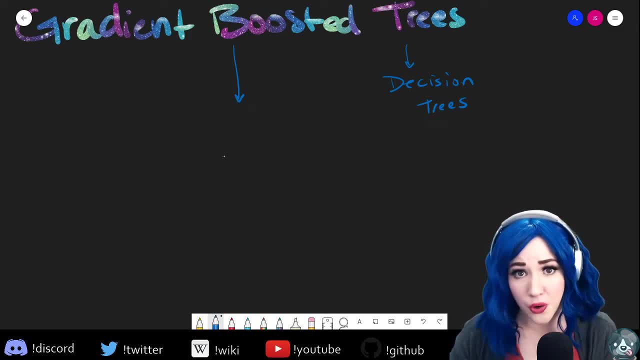 doing their own thing, and then we kind of figure out what the majority has voted on. we're going to take a single tree at a time, And so we've got our first tree right. We train it, we test it. Then we take our second tree. 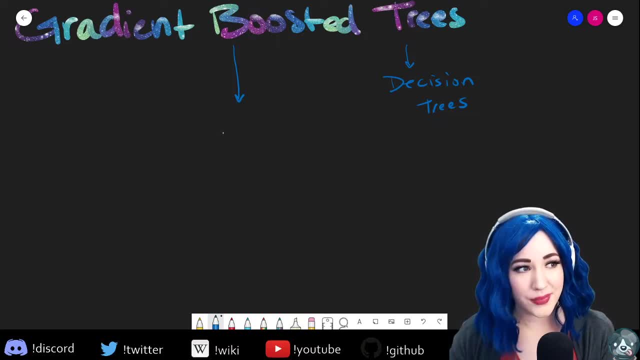 but we train that second tree on the errors that the first tree made. So it's sequential more than ensemble. So a sequential improvement And in fact we're not just going to use any decision trees. I'm going to put this in scare quotes: 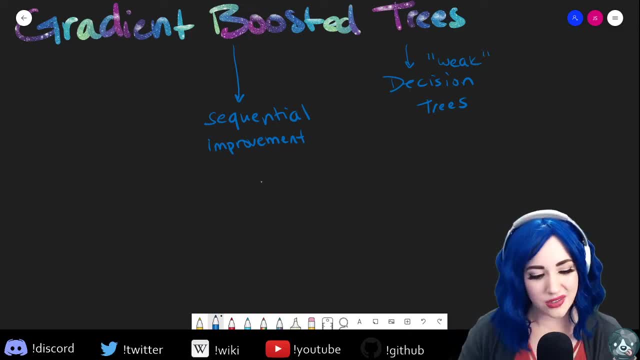 because we'll talk more about what that means. but we're actually going to use weak decision trees, So decision trees where we're like we don't expect it to be that great. We actually we don't want it to be that great at the start. 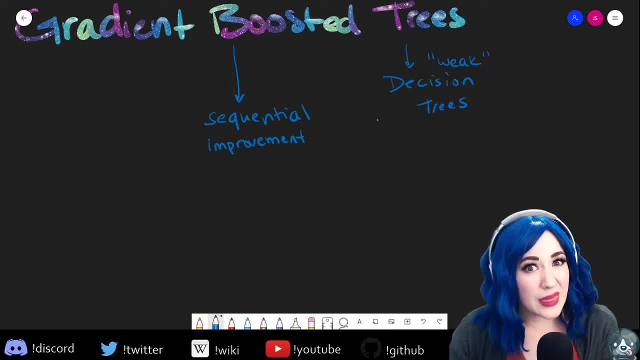 Weak here, meaning its performance is not that much better than random But sequential improvement. So we're additively adding, additively introducing another tree that we train on the errors of the previous tree. Now training on those errors, how do we determine them? 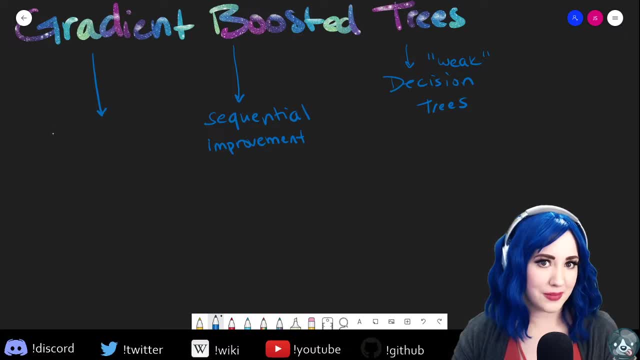 How do we improve? This is where the gradient comes in, So we're actually going to use gradient descent. Now I'm going to kind of summarize gradient descent for you in just a few sentences. But if you want a deeper dive into the math visualizations, 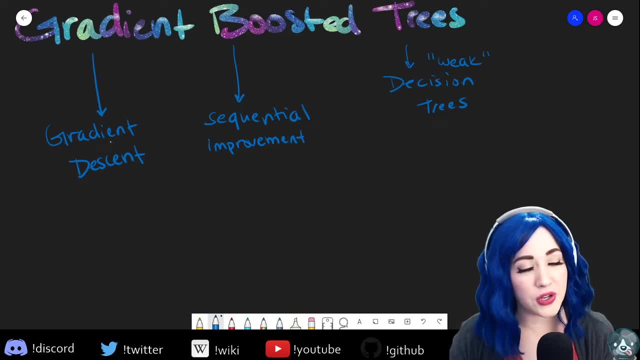 all that goodness. definitely check out the neural net video that I mentioned earlier. that's on YouTube because I do a deeper dive into that. But gradient descent: if you're not familiar with the mathematics of gradients, don't worry. Essentially, what we're going to do: 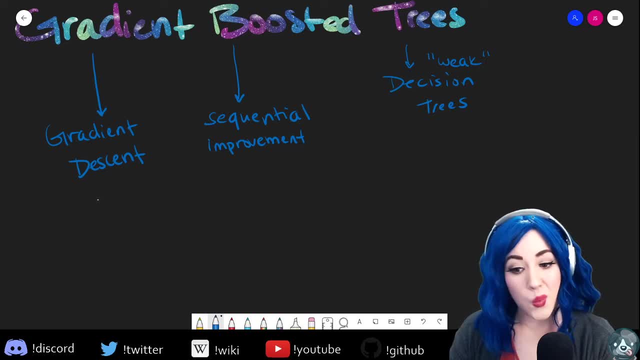 is. we're going to take our loss function, which is a way that we're going to determine how bad we're doing. How do we define an error? And we're going to try to find its minimum. Where is this error function? the smallest it can possibly be. 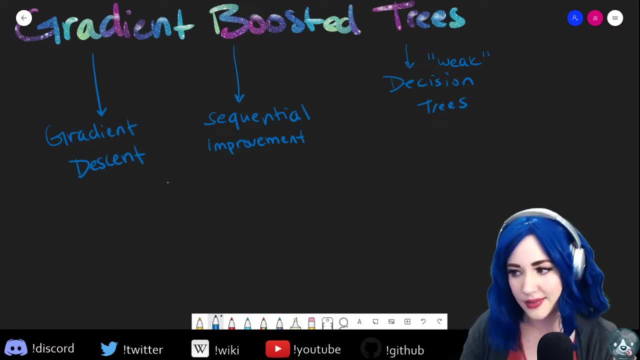 And that's really what gradient descent is about, But we're going to go into each of these in more depth. So, to get started, we need our learner, Which, in this case, is going to be a weak learner, And it's going to be a decision tree. 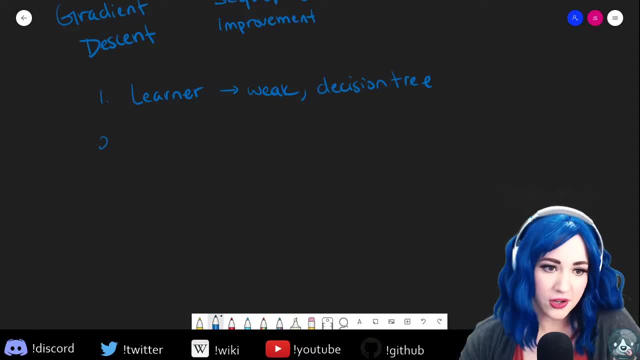 We also need, like I just mentioned, we need a loss function. You also might hear this called a cost function. This is just a way of how do we describe our error And if you've been on previous streams, you know we've used 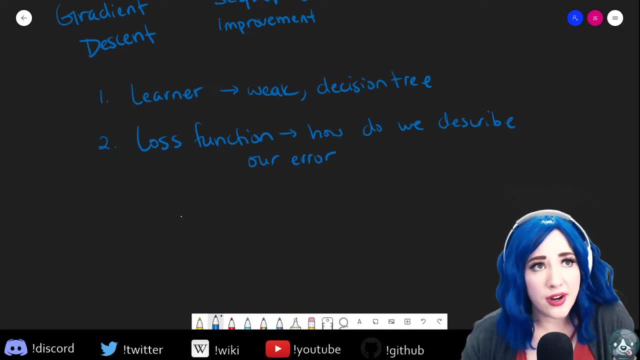 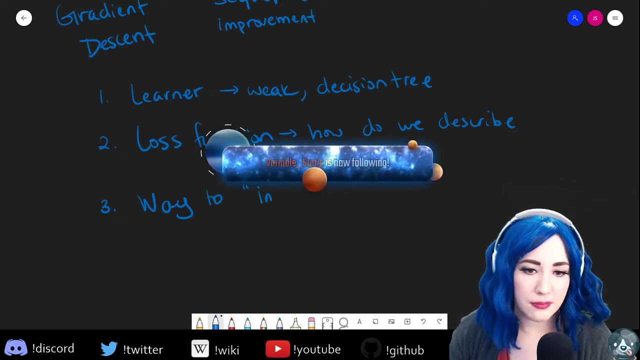 like Sum of the squared error, And we've used mean squared error, root mean squared error. These are all different kinds of loss functions And we need a way to improve, And that is really going to be about our sequential adding and our gradient descent. 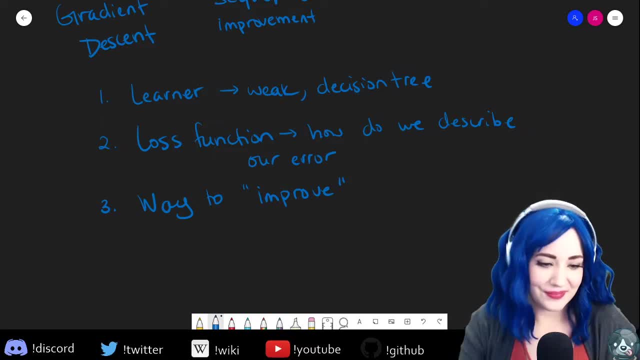 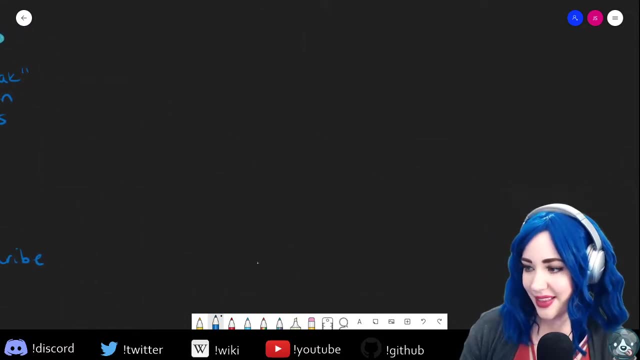 And variable static welcome to stream. Thank you so much for following. OK, So Let's, Let's, Let's take a little detour. Let's take a little detour into math, Math, Gradient boosted trees- OK. 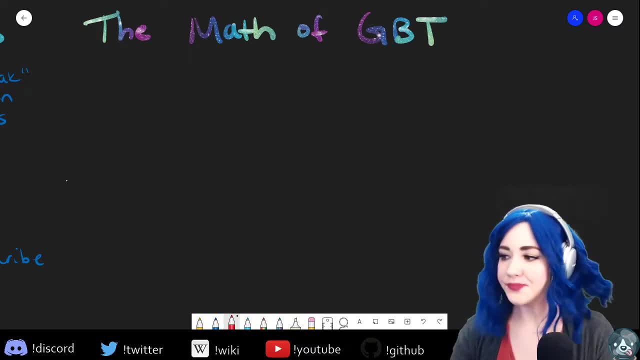 So Let's say, Let's say that we have our tree. We're going to call this tree T0. Don't worry so much about like oh T, Oh zero, T for tree zero, because it's our first one. 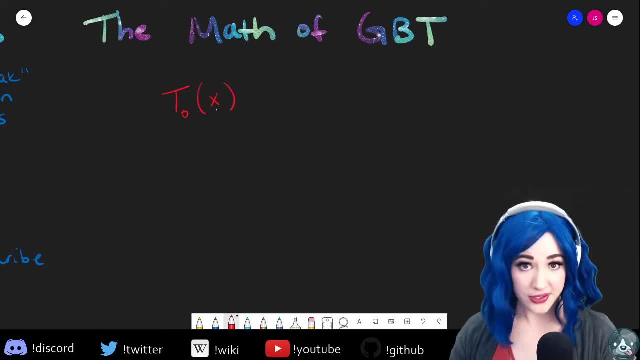 Now we're going to feed it, We're going to stick. So we're going to stick our features, our predictors, into that tree and it's going to give us an output of some kind. It's going to make a prediction for us. 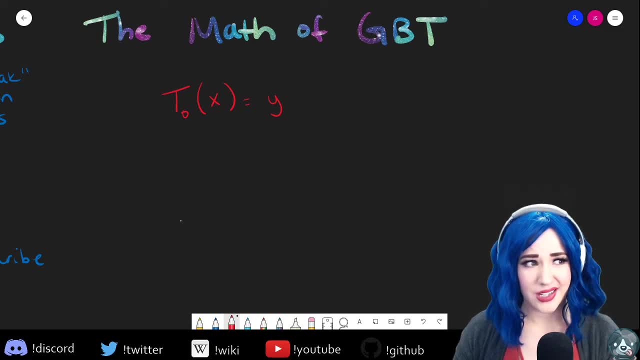 OK, Then we need to figure out: well, how bad did we do, Right? So for now I'm going to use a very, very simple kind of explanation of that Is: let's just see how, How Bad Was our output. So 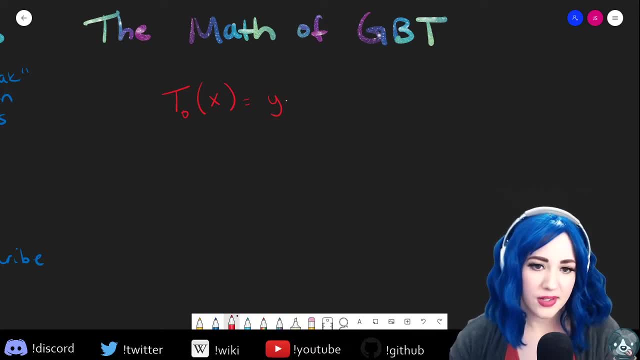 so if we have, I'm going to put little like um, so this is our, our predicted why. So if we have kind of like our, why actual minus? hopefully people can tell it's a minus, minus our predicted why. you know a difference between what we did and what we should have done You can think about. 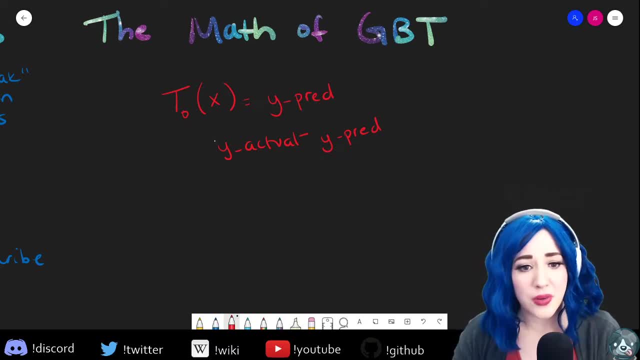 this kind of being like an error measurement. So there's different ones, right, We can square them. we can do, uh, you know, add them up and square them and then take the root. We can take the average. all kinds of different things, But for now, let's, we're just for conceptual, we're. 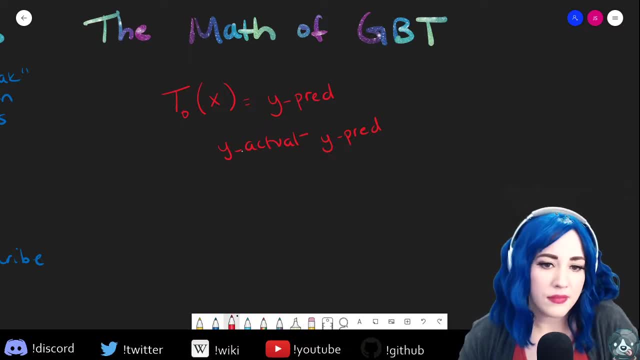 going to talk about this. So we've got, we've got this, this error right. So you can think about this is, if I can draw an arrow, this is our, this is our error, And what are we going to do? 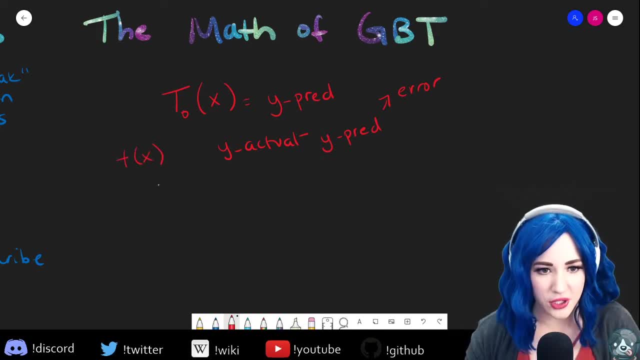 Well, we're going to introduce another tree, a little baby tree, Okay, And we're going to fit that new tree to this error, Okay. Then our next, our next, our new tree, our new, new model. See, we've got a one, because 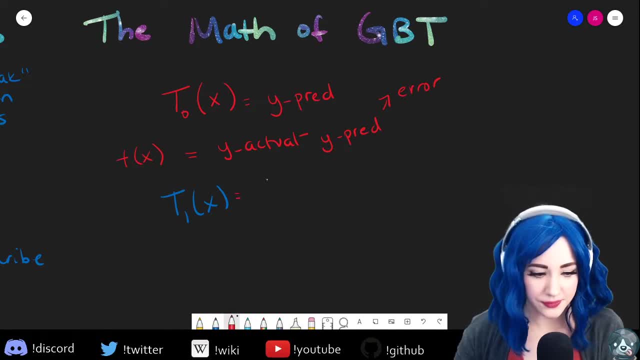 it's. the next one is just going to be equal to our old one plus plus the one that's fit on the error. So this you can also think this is also called residuals. and oh my goodness, it's 3 AM. Okay. 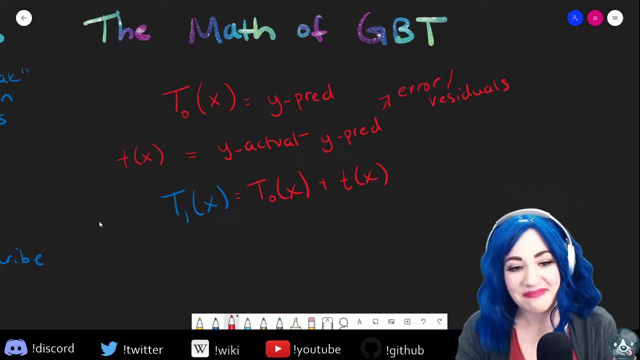 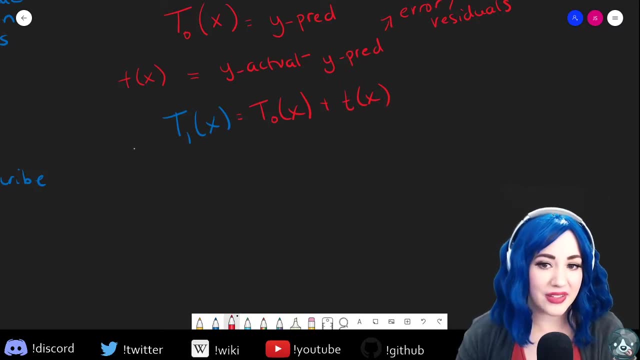 Rattatat, go have sleep. Um, I'm so glad that you were able to join. Um, hopefully I'll see you next time And we can do this again so we can have, like you know, ah, don't fail me now, Don't fail. 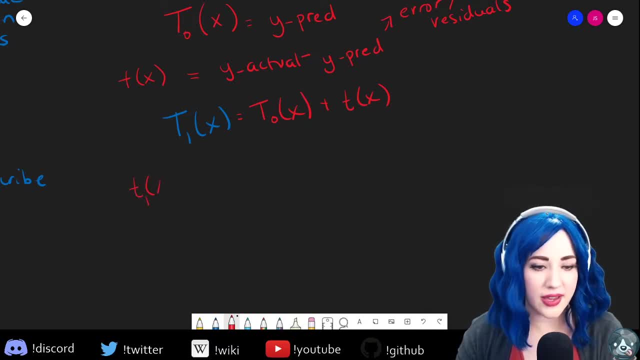 me. now You can do it All right, here we go. So maybe we've got now another one, And this is going to be why actual versus, why one prediction. So these would be why zero. now, maybe our next model is going to be: well, we don't even need to write it all out, It is going to be. 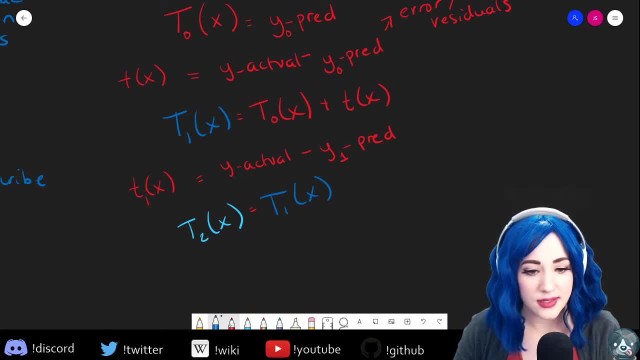 T one. This plus this new tree that is fit to our residuals, to our, to our errors and high C films. It's good to see you, Welcome. Welcome to stream, And I'm sorry my handwriting is starting to like creep up the side, but hopefully you're getting the pattern here We're adding a new tree. 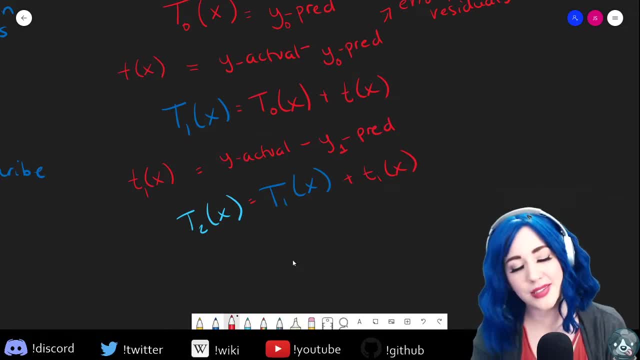 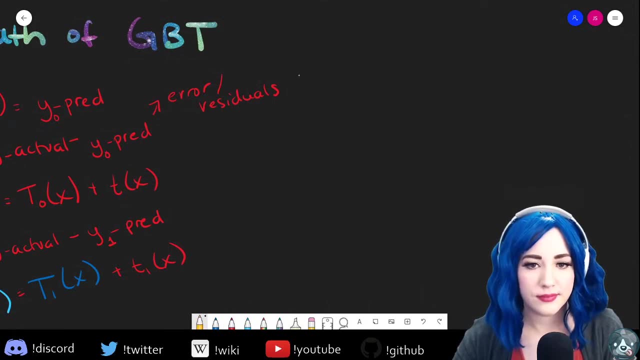 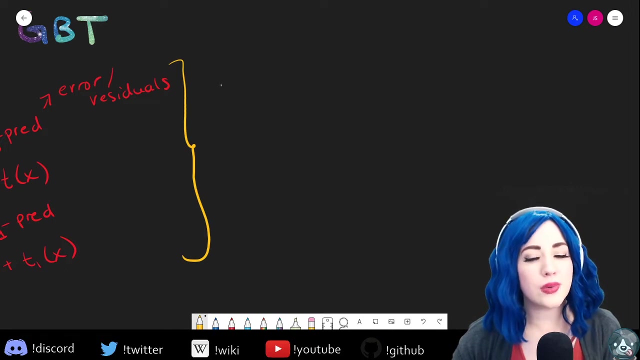 fitting it to the mistakes of the previous tree and then sticking it in with the rest, And so all of this we can summarize. So we're going to keep going, and keep going, and keep going until we hit some kind of stopping condition. So maybe it's like a performance measurement, Maybe it's, you know, a certain error threshold, but we're going to go until we hit some kind of condition that we've specified for it stopping. 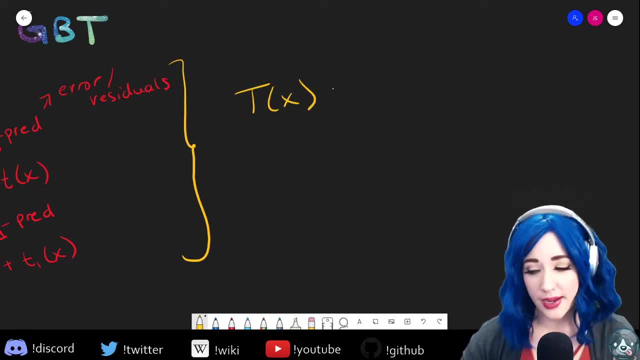 And we're going to generalize our model. It's going to be adding up right. Sigma is just a sum We're adding up for N number of trees, Number O trees, adding up The tree That we stick, all of our. 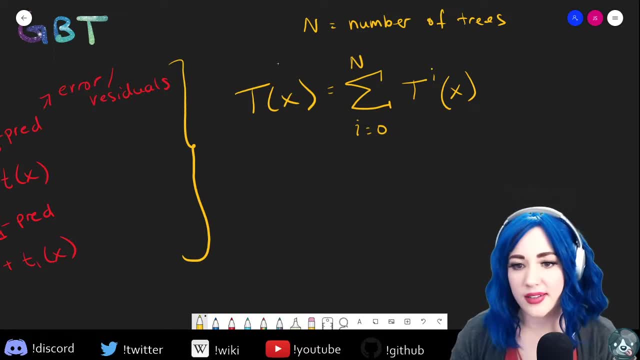 All of our features into. So we are summing up all of these different trees that we've made, each one learning and iterating on the previous one. So, for example, if you're more of a visual person, let's visualize some of this math a little bit. 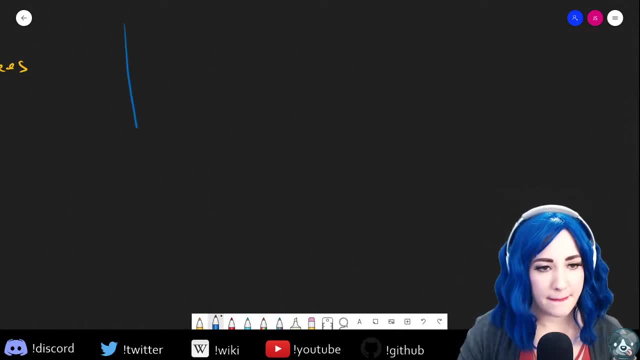 So maybe Give me a second. I'm going to make up a function here. Maybe we got something sort of like sine wavy happening. Oh, we're getting some lag in the whiteboard. That's a sign that it's going to be time to code soon. 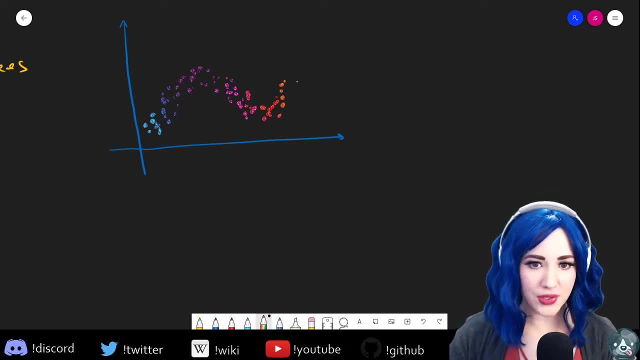 All right. So the world's worst sine function, Whatever. And so maybe, Maybe our first attempt, our first attempt to our first tree, does something like I don't know, like this. It's not great Right, But you know, we're going to, we're going to start to learn from it. 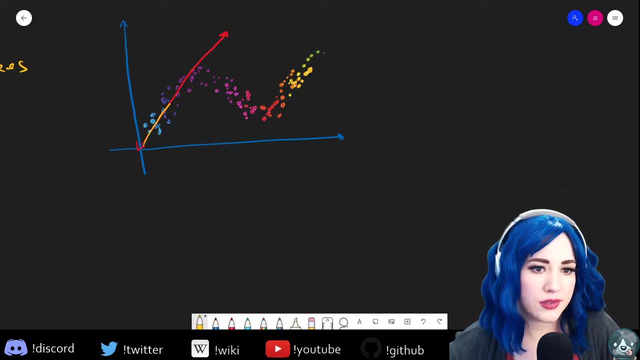 So maybe our next, our next one kind of goes, Kind of goes Like that, And maybe our next one after that Goes like that, And you can see that we might keep going, each learning from the area that the previous, the previous tree, failed at the most, until we can, we can, you know, visualize having one. 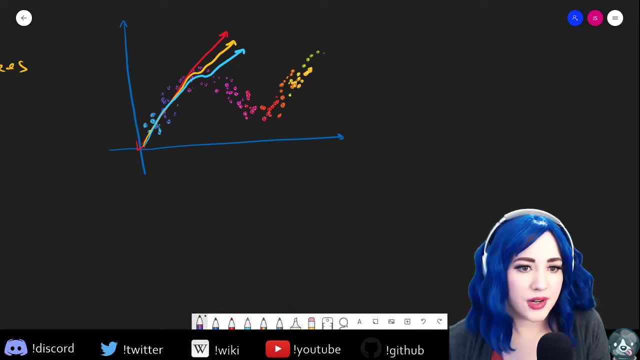 I need another color. You know we've got something that does like, oh, like this, But maybe it goes down, and then you know we keep going until eventually we have something that actually fits our data, And so this really is kind of what we're doing by adding, adding all of these different trees and see films. 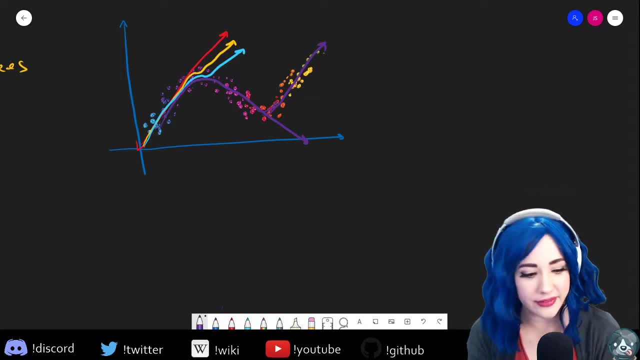 We are doing nodes as part of this, So our trees will have nodes, not tokens, though That's more of a natural language processing term. But for our gradient boosted trees, Yes, they're going to have nodes, and we can actually restrict something called the depth of the tree, which is kind of how many layers of nodes we have. 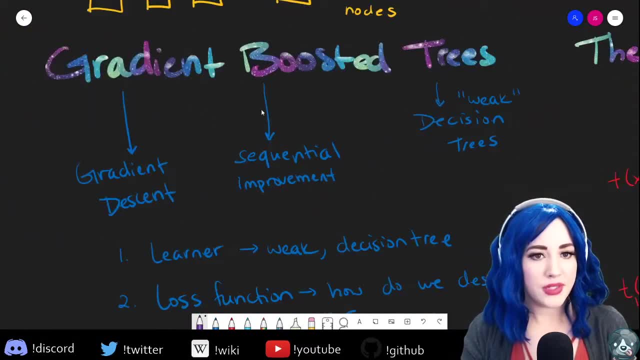 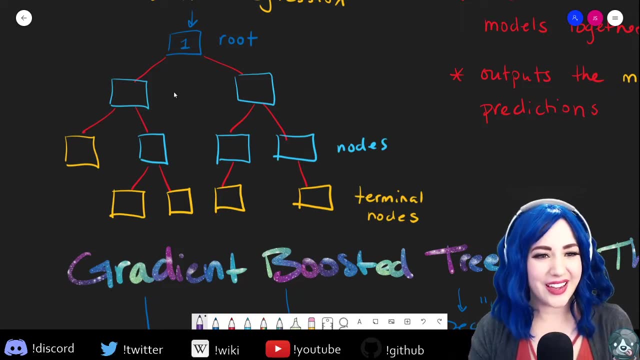 So if we go back to the terrible drawing I probably drew somewhere, you know this has a depth of- Oh my gosh, One, two, three, four, four. So that's kind of like you know you can think of like this is a layer of nodes. 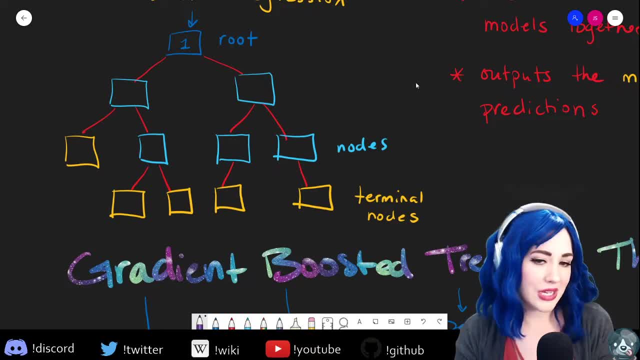 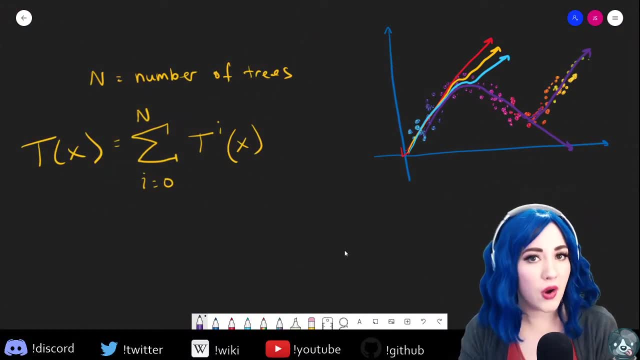 These four here are a layer of nodes, So this particular tree has a depth of four And we can limit the depth if we want to, To avoid overfitting. So one of the problems with decision trees is that the deeper they get, the more splits you make, the more they have a tendency to overfit to the data. 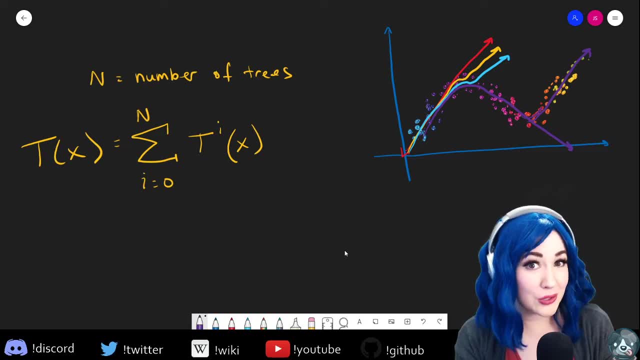 Meaning that our testing data it would do really great at. But if we tried to do inference, if we tried to test on like a validation data set, it would do really, really badly because it's not generalizing, It's not learning those general principles that it can apply to a new situation. 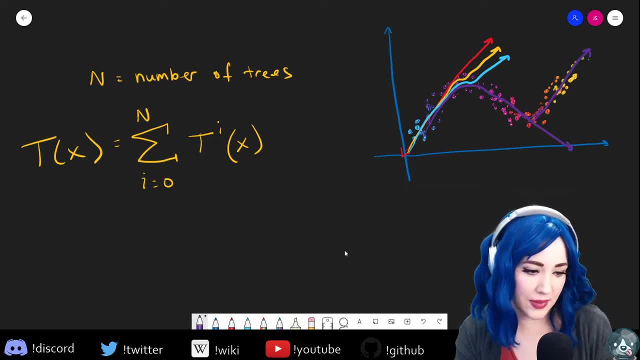 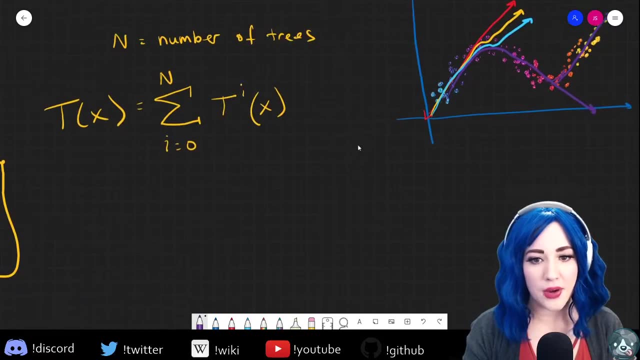 It's just trying to exhaustively describe the training data that we give it. And no worries, I am Ben. It was great to have you here. Hopefully I will see you. I will see you next time, Okay, So Let's see. 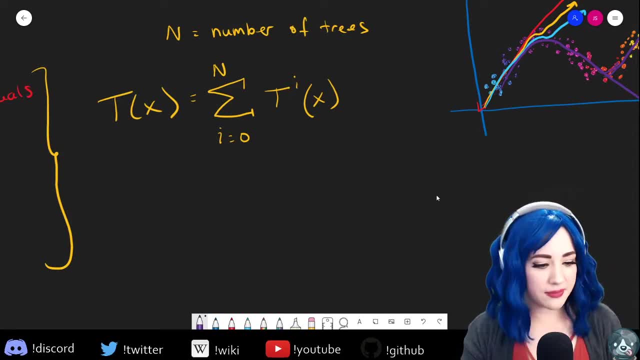 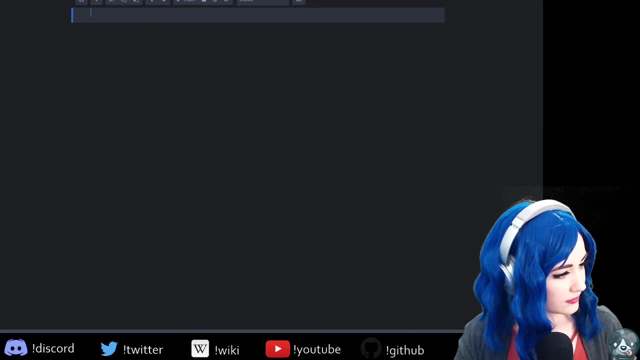 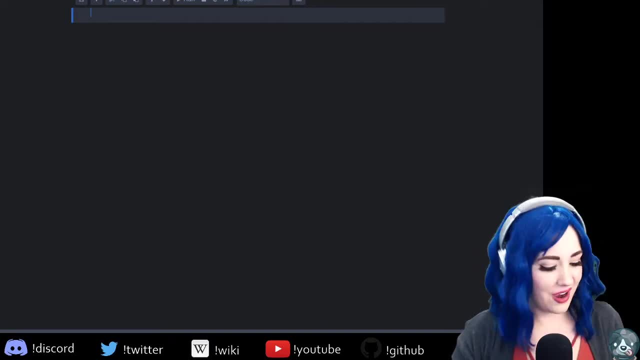 And thank you. augmented mode: I'm, I'm, I'm glad you are are finding my, um, my explanations useful. Okay, So we're going to be using a data set, that is. let's see how to explain this. 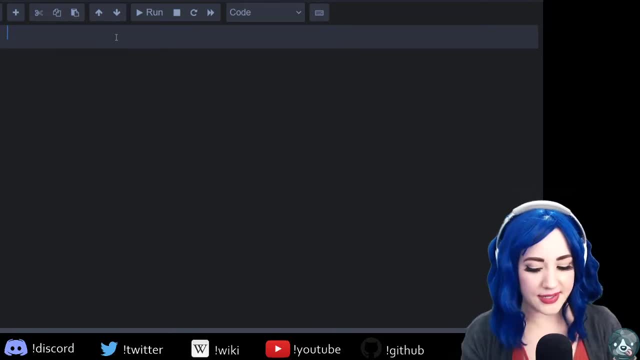 So if you saw days one or two of the fundamentals of data science, you'll notice that this is of the fundamental of data science. know that the wonderful, perfect sample data sets that we often get aren't so great when it comes to doing stuff in the real world. They're great for learning how a model works and for kind of 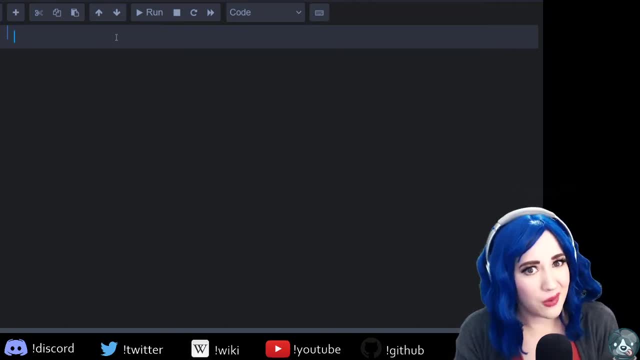 practicing, but they're not what real data looks like, But because we're learning a brand new kind of model today that I haven't taught you all before. we're going to use one of those nice cleaned data sets so we don't have to waste all of our time with EDA and data cleaning. We're 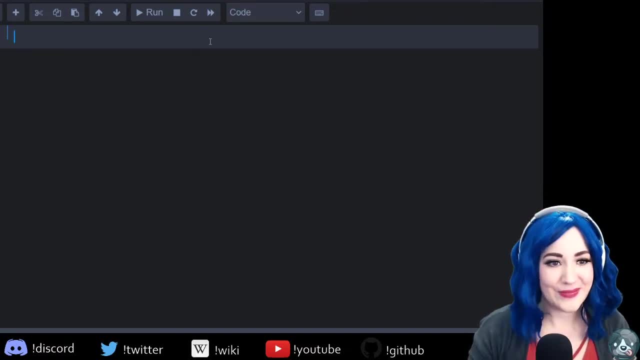 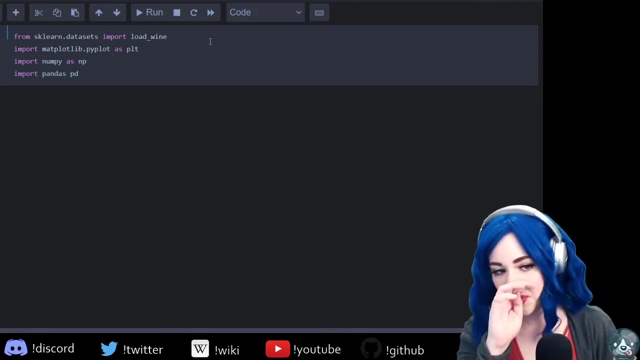 going to be using a data set of wine data, And let me tell you I don't know anything about wine, So this I can. I cannot explain the features as well as I could with other other data sets, unfortunately. All right, So those of you new to data science and Python, we're going to be using 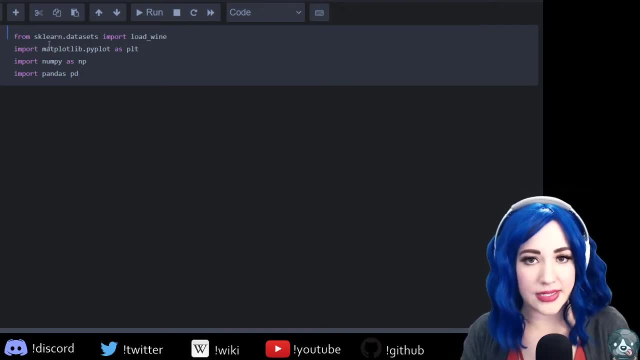 scikit-learn, which is a great, um, uh, a great library for doing machine learning. We're going to be using matplotlib for visualizations and NumPy, of course, numerical Python and pandas, which, which are all great, good libraries that. 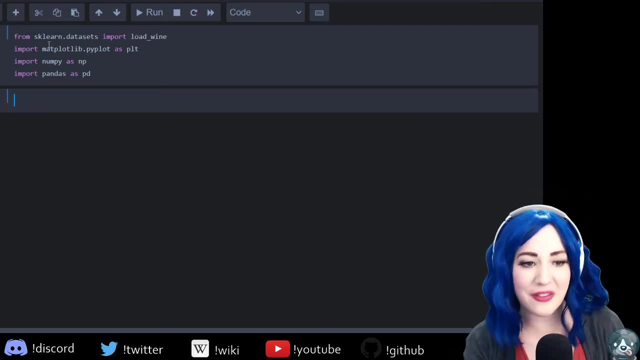 you should try to familiar, familiarize yourself with um if you're interested in data science. I'm going to copy some uh, um, I like to do that. And then let's, let's load our data- See films. Thank you so much for the raid. Welcome Raiders. Thank you absolutely so much. 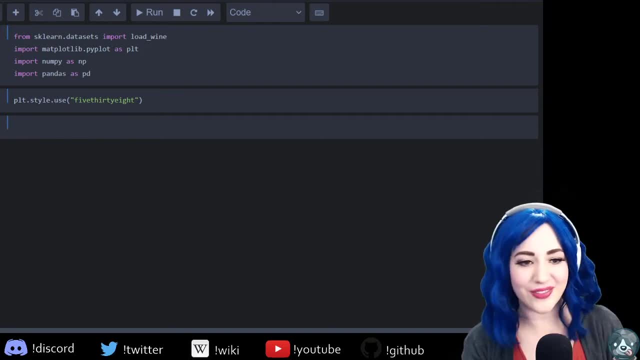 Um, I love raids. It's like suddenly there's an influx of new friends. Um and Kevin, you say you use pandas every day. Yep, The funny thing is is that so I will. I will caution people with this. Panda is great for um, for your kind of more ordered data, And it's great for um for. 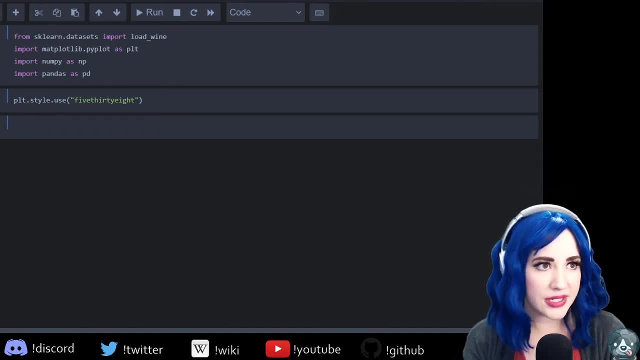 smaller amounts of data. but pandas really does have kind of like a computational trade-off where, if you're dealing with larger data sets, if you're dealing with larger data like imagery or something or um, very large feature vectors, pandas really does have a drop-off at some point. 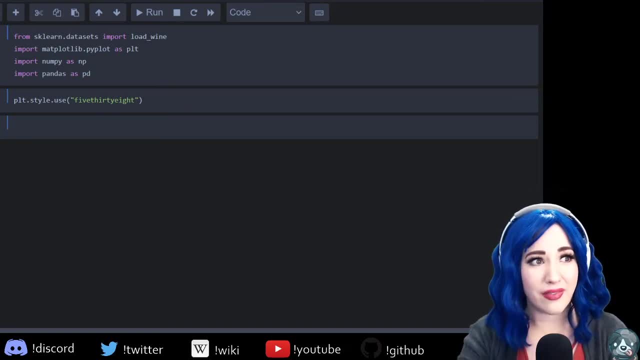 So, while it's great, I've actually found that the like deeper I've gone into machine learning, the less and less I've gotten into machine learning. So I've actually found that the use of pandas, um, and yes, there's a point in which you need to consider spark, or just there's. 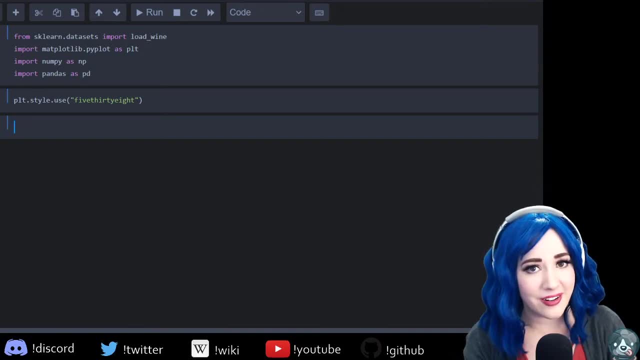 a point at which you just convert everything to like numpy, arrays and numpy, numpy, whatever, um arrays and and do it that way. Also, if you are interested in accelerated computing for data science, um, it would like, do not become super reliant on pandas, but okay, So let's see here. 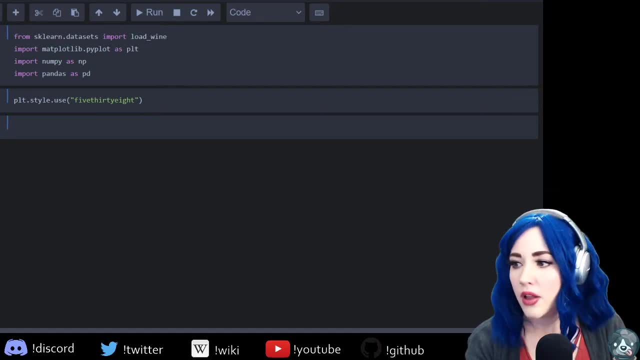 We are going to use. let's let's get our data and I'm going to make a pandas data frame out of it, And this is a great way to just look over your data. It's kind of like, you know, an Excel spreadsheet You can. 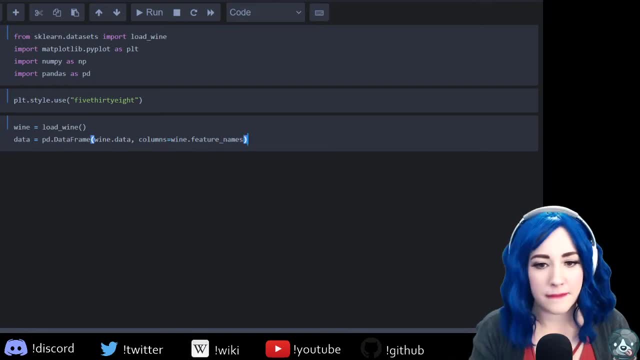 think about it like that. All I'm doing here is I'm getting that data from the scikit-learn wine- Actually, I forget where exactly the the wine um data set comes from. Scikit-learn is using it, but I it's not from scikit-learn- And I'm setting our, our label, our target uh column as well. 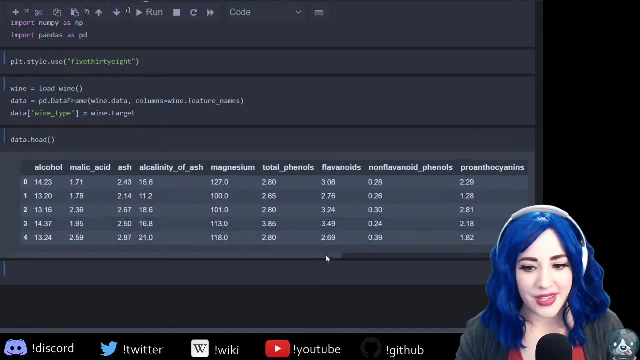 And so now, if we look at our data, you can see that we have all of these different, uh, different features. These are our different predictors. Have I ever used the data classes package? I don't believe. I have Um, so you have alcohol, malic acid, ash, um. 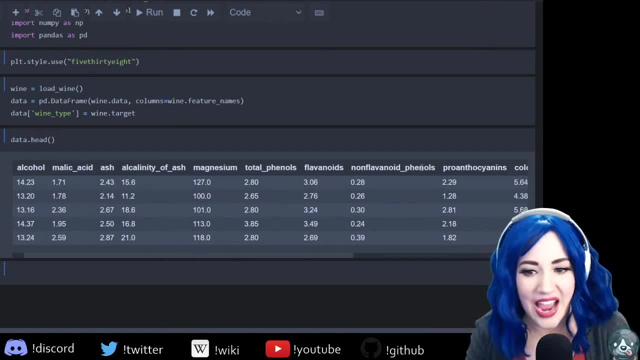 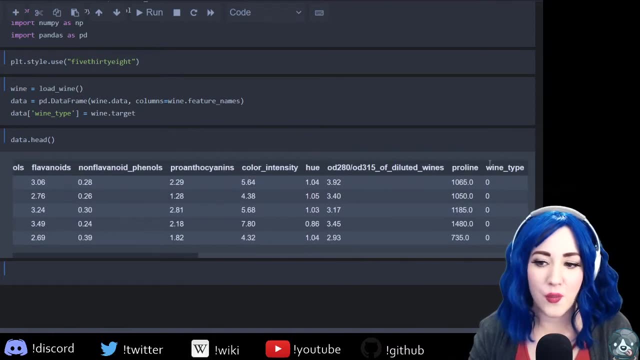 alkalinity of ash, Like I have no idea what a lot of this stuff is, but these are characteristics of wine, And then we also have the wine type And that's what we're going to be really trying to predict here. So we're going to- we're going to import some stuff from scikit-learn. 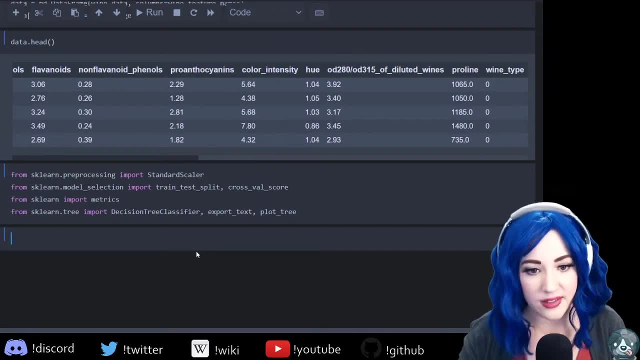 Those of you who are here for machine learning this know scale your data. So we're going to be- we're going to be- scaling our data. If you're interested in learning more about data scaling and different kinds of scalers available to you, definitely check out. 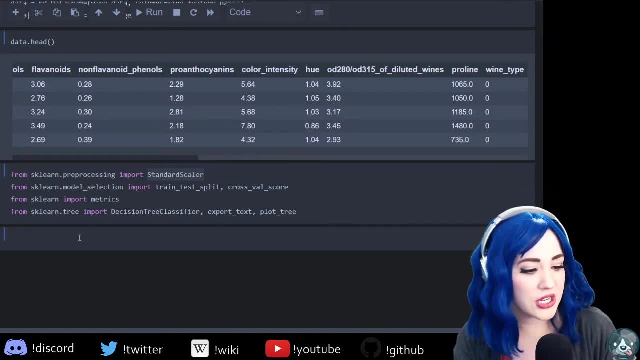 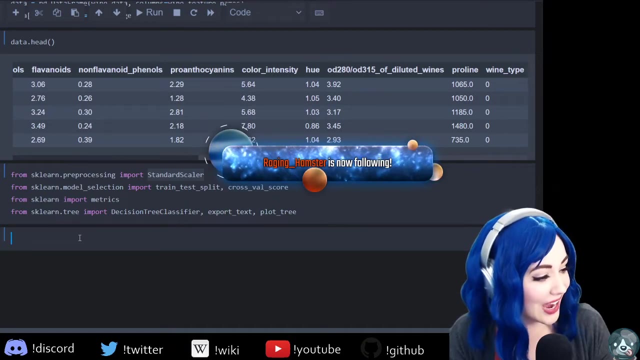 um the pre-processing stream and have i tried neural evolution to train deep neural nets? i haven't had a chance to do it for work, so i've kind of like dove into it for fun, because it's really really cool, um, but i haven't had a chance like to build it for work yet. so and hi raging. 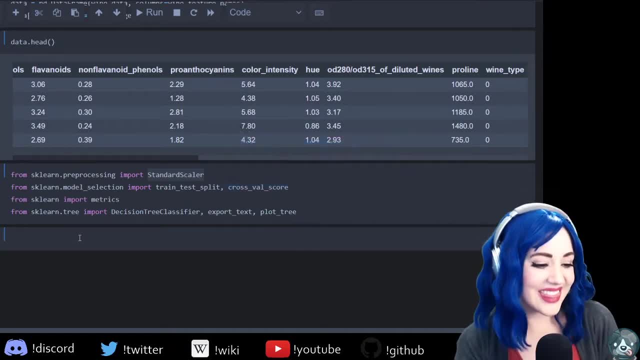 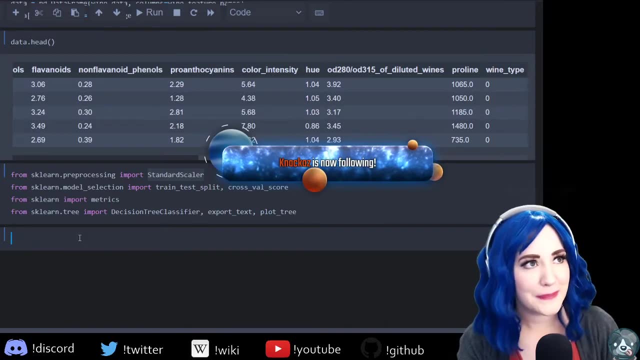 hamster, welcome, welcome, welcome to stream and thank you. kevin, you say i'm a great teacher. i'm. that means a lot i i like teaching, but it's always good to know that, um, that the effort i put in is reaching you. so, and k nakas, thank you so much for for following and hi raging hamster. 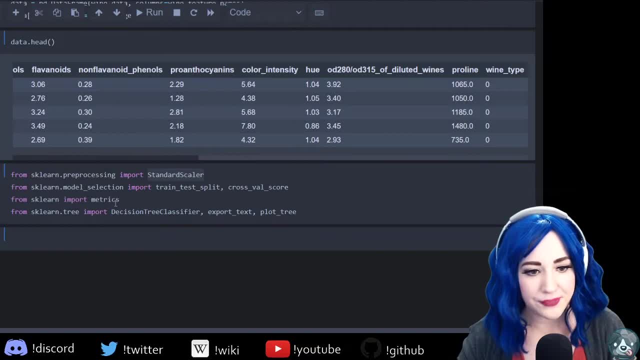 all right. so we're gonna- just, we're gonna import some stuff, we're gonna import a scaler, we're gonna import a tr- uh, test, train, test, split. right, because, just like i described to you, we gotta split up our data into our training data and our testing data and we're gonna do some cross. 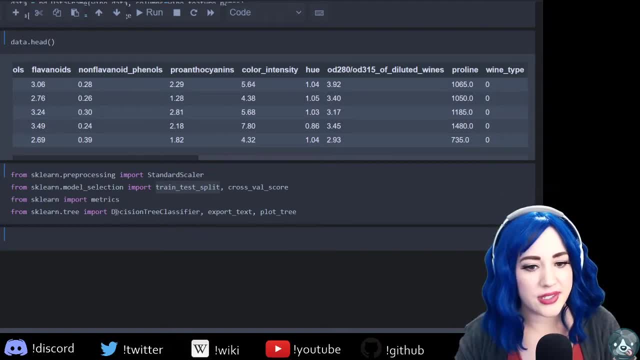 validation. um also need some metrics. here's our, here's our model, our decision tree, and we're going to use it as a classifier, because we're trying to classify a category, a type of line. and these are some visualizations. i don't think i need export text, but just in case i do, i'm going to. 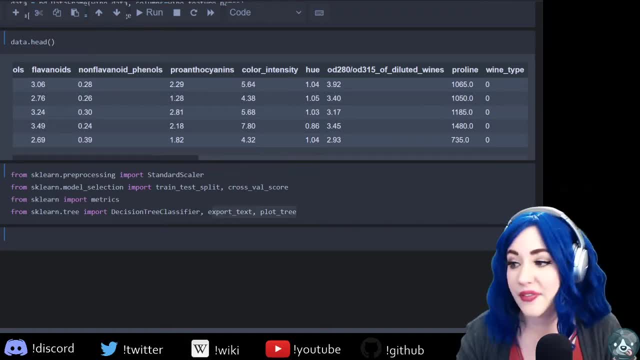 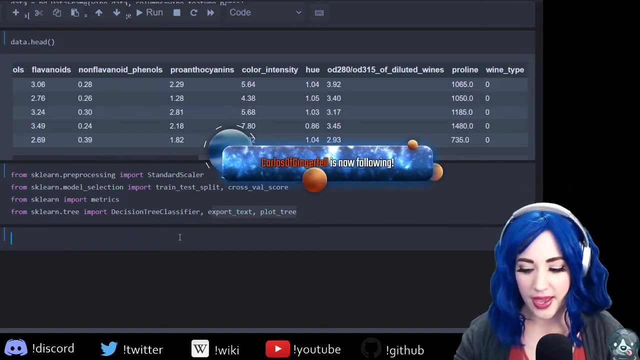 leave it there, but this will help us make some visualizations of our tree. so first, what we're going to do: remember we talked about decision trees, then random forests, then gradient boosted trees, so we're going to do that in the code. first we're going to do is: 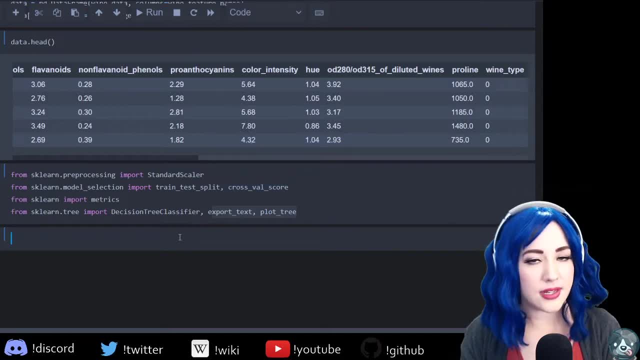 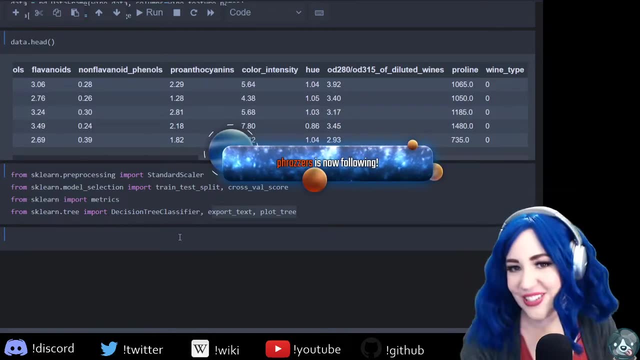 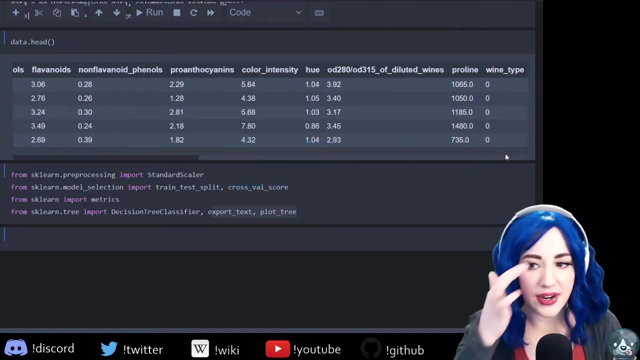 a decision tree, then i'm going to take you through a random forest, then we'll do our gradient. boosted trees and carlos of ginger fell- it's a good name- and frazzers, thank you so much for for following. welcome to science sunday. okay, so one of the things that you can see here, especially when you're 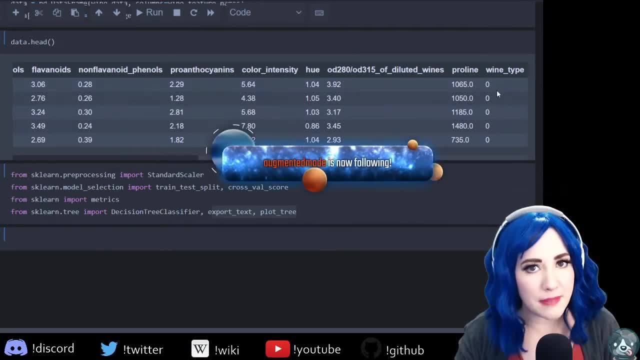 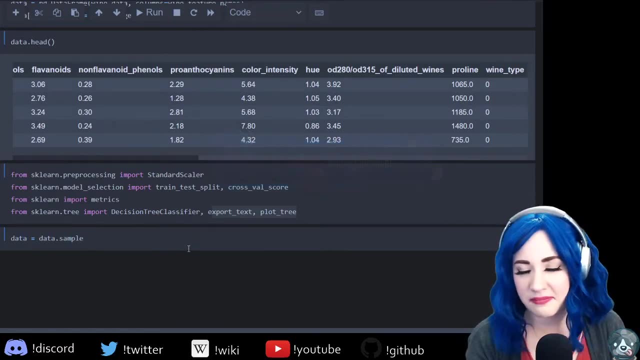 loading data sets from scikit-learn is that they're sorted by by the label. so we need to shuffle. so this is my very um how to put it. this is: this is my lazy way of of shuffling, as using you're, you're asking pandas to. 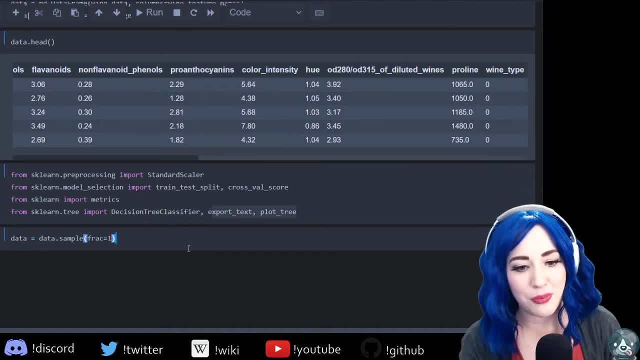 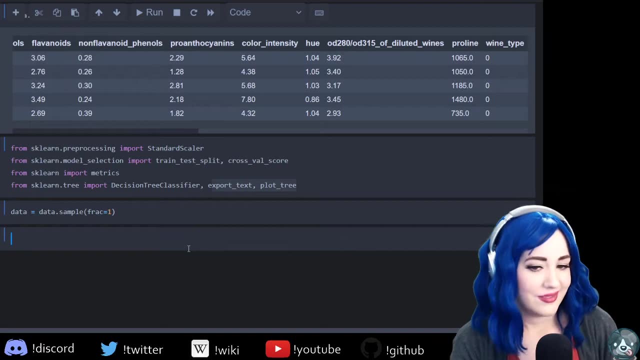 sample the data, but you're putting a fraction of one, so it samples all of the data, but it shuffles it, so there's a lot better ways to do this, but whatever, it's fast, um, all right, and hi, yeah, hi, carlos of ginger fell, welcome, all right. so the first thing we need to do is we need to make our 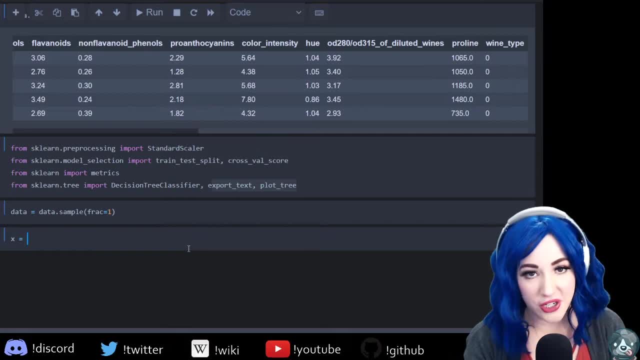 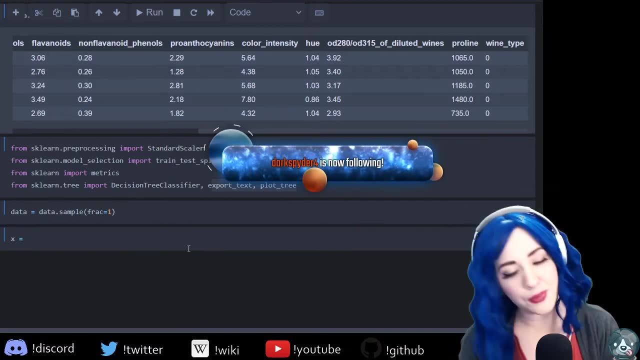 features: right. this is our feature vector. our x values- right? if you think back to the map, it's going to be a little bit more complicated, but we're going to do that. so we're going to go ahead and do the type set values. this is the byte we just did. this is the stuff that we are going to input into. 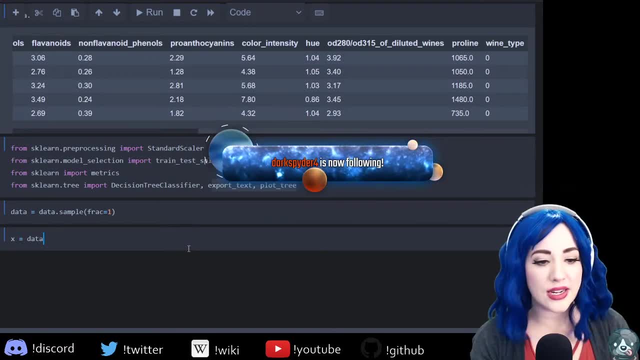 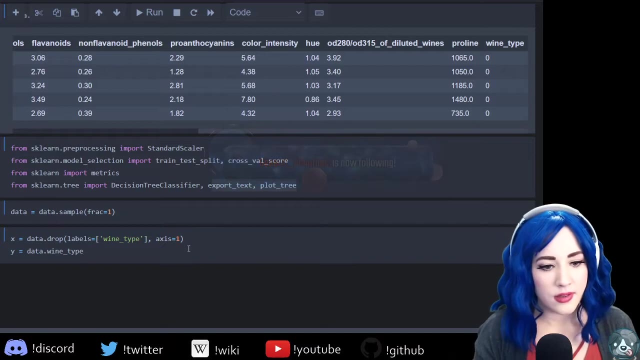 our model and dark spider. thank you for following. all right, so we're going to need all of our data, except the thing we're trying to predict, right, because that's our y. so our y, like i said, is our wine type, that's what we're trying to predict, and general phantoms. thank, 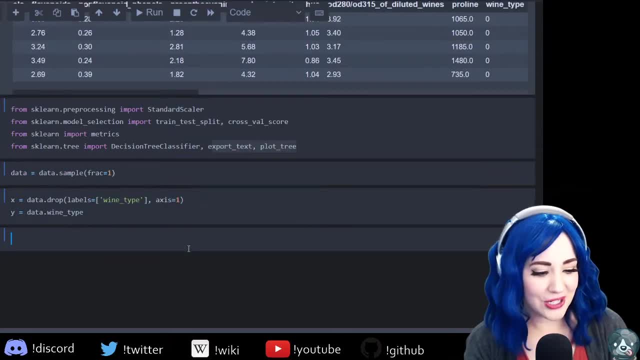 you so much for for following All right. and then I'm not sure I don't see many people from machine learning here, but those of you who have been around for a little bit, hopefully one of you will come in. What is our next step? 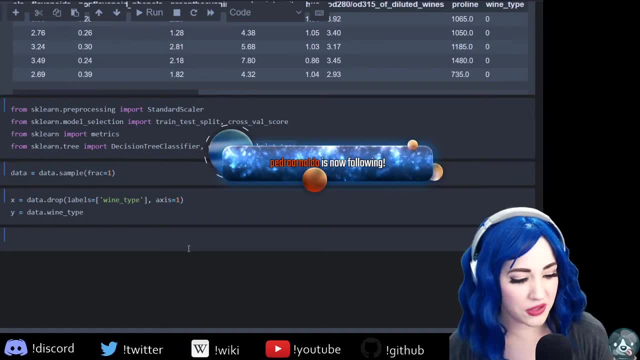 Carlos of Gingerfell. you say you're from the UK, so it's- oh my God, it's 2.30 in the morning. You say you should be asleep, but this is the most interesting thing to watch: while you crochet a blanket. 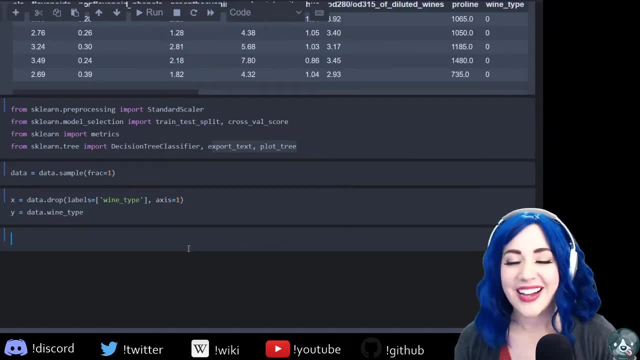 I love crocheting. Good luck with your blanket. Hopefully I won't keep you up too late. Sleep is a good thing. I have a day off tomorrow, so if I wanna be a little irresponsible and stay up too late, I can. 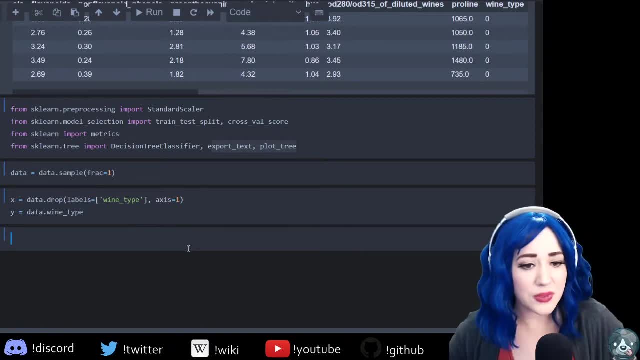 Pedro Arnaldo, thank you so much for following. All right. so what's our next step? Are we done? Boom, I just give this to my decision tree. So augmented mode. you're right, we split. but even before we split our data, what should we do? 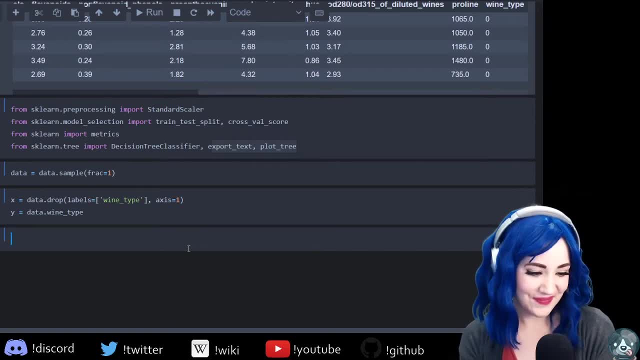 And Casado Conheos. hi, how are you Not yet, Kevin? So fitting comes after splitting, but what comes before splitting? So here I'll to help, so we'll split and then oopsies, then we'll fit. 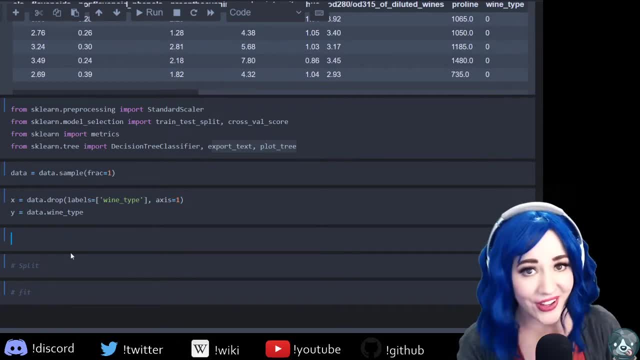 Yes, Casado Conheos, coming in with the answer: We need to scale our data. So we are going to, we're gonna scale it, which is really, really, really important. This is something I've talked about almost till I'm blue in the face or blue in the hair. 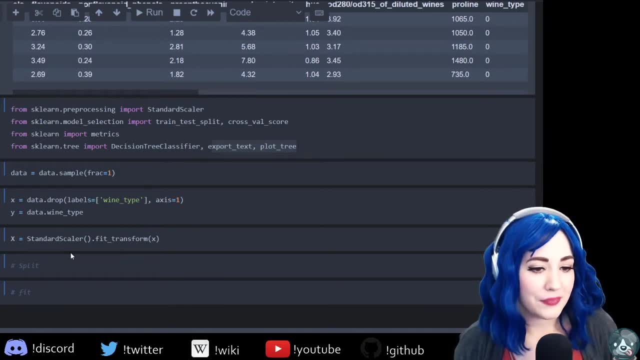 which is, you are introducing a lot more problems into your data set when you're not scaling your data. So, and yes, Casado Conheos, you say, 12 days of machine learning is paying off. Nothing makes me feel better than when people remember something that I taught them. 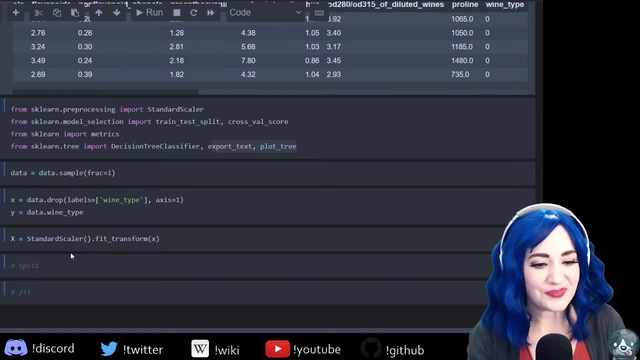 or it helps them in some way. It's like the best feeling. I actually so tiny story time before we get back to the code, but I was recently interviewing for a job and they asked me what my favorite part of the job was. 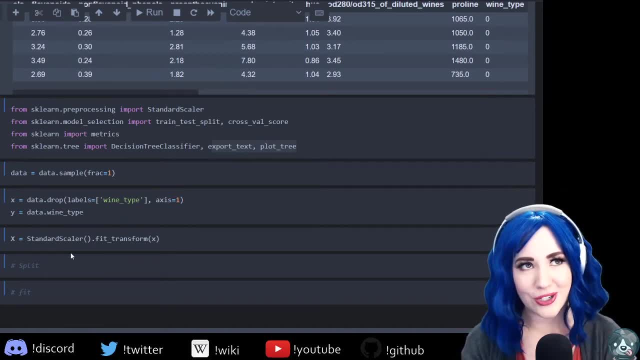 And I answered honestly and I get. I kind of get the feeling like maybe I shouldn't have, but honestly it's not my coding, Like that's definitely up there. I love when my code works and I make it like real efficient. 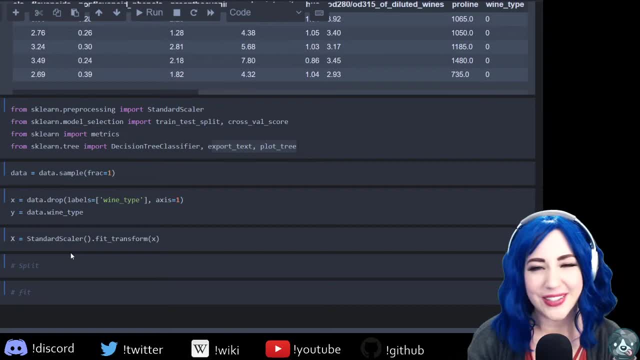 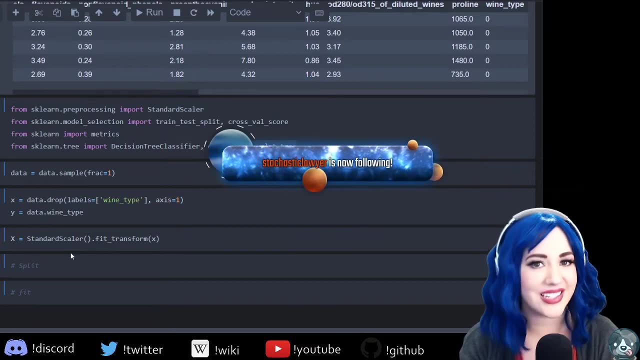 And I know it's like real elegant and you just feel like you're on top of the world. That feels great. But the best, best, best feeling I get at work is when somebody I've mentored is successful. So when somebody I've helped or I've taught. 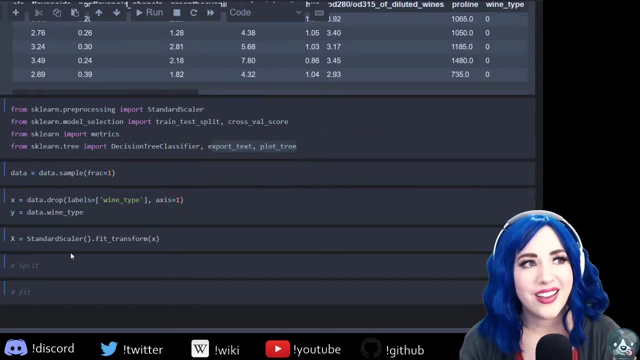 or mentor them in like any kind of way, whenever they are successful, like they get a job they want, they get a raise, they get a promotion, their code works, whatever, they fall in love with programming or with math, Like that is the best feeling. 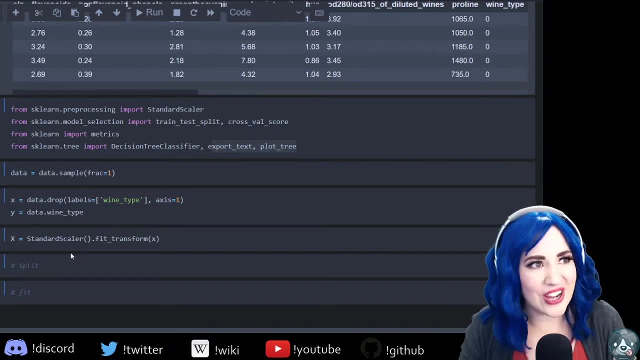 So it's not even like my own success And like I kind of like tried to talk to the recruiter about it and I was like you know, don't get me wrong- Like I love the technical work I do, I really do. 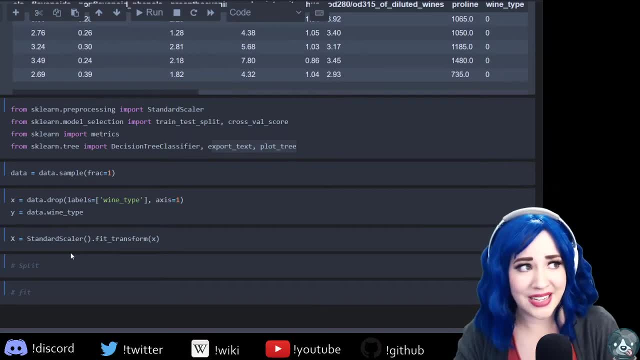 But, if you're asking me, the thing that makes me feel the best it's when somebody, like on my team, does well. So I don't know, And it's a great feeling because I have. I have all of you wonderful Twitch people. 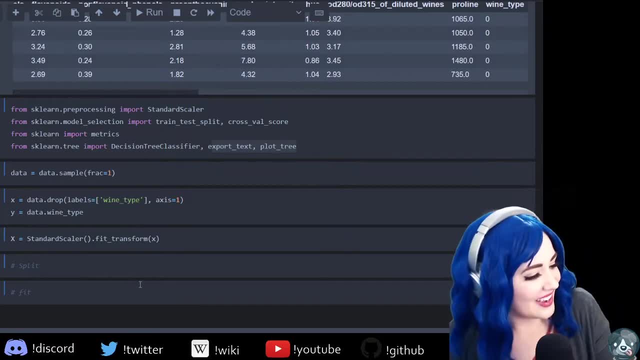 And so when all of you get it, oh, I get to feel great And Stochastic. Lawyer, what a great name. Welcome, welcome to welcome to stream. And Jay Holly is a future teacher. See, my mom is a teacher. 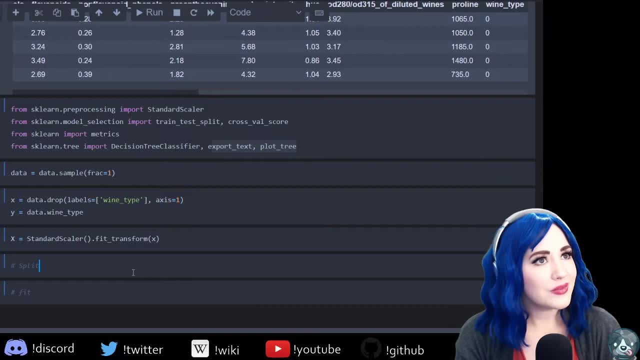 And she's been trying to get me to be a teacher. I don't want to teach, at least not in the American public school system. I've tutored for years. I love doing more mentoring because I feel like teaching professionally I'd have to do with like one hand tied behind my back. 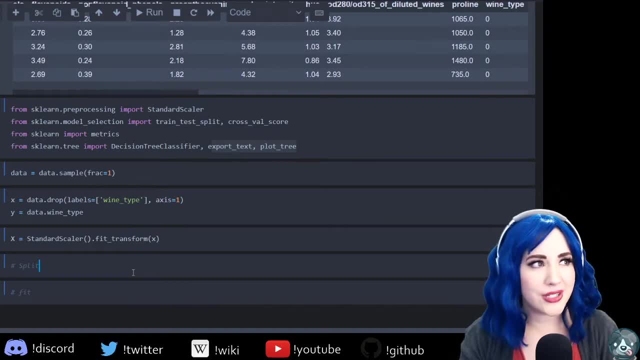 because I'd have to follow a curriculum and I'd have to make sure I'm teaching to a test. Not that like there's many teachers that manage to balance that and still be good teachers like my mom, But I I'd much rather like. that's why I like Twitch. 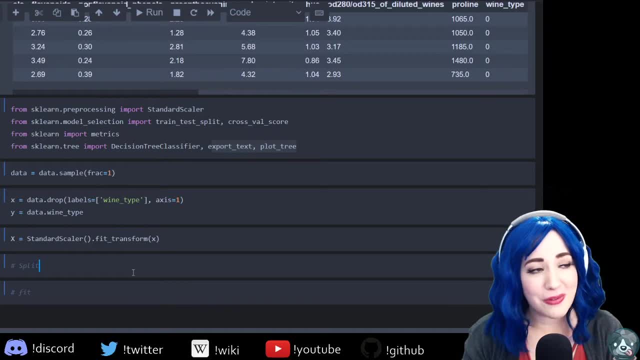 is. it's free. Anyone, hopefully, with a device, can like pull it up And you know, even if they can't make the time of stream, I try to put stuff on YouTube, all the codes there for all of you, the Blackboard images. 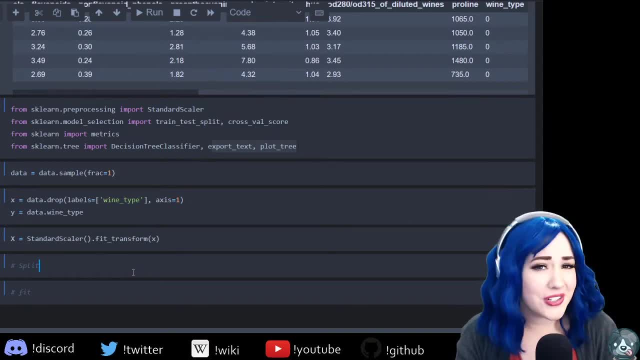 go it at your own pace. You don't have to pay for it, There's no test, there's no anxiety. So like it's a way for me to still reach people, but kind of doing it in the way that I would prefer to. 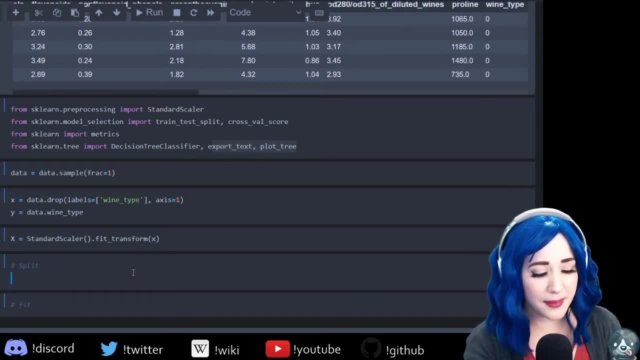 So okay, But yes, folks, we're right. Augmented mode: We're gonna split our data now We're gonna do a train test split. I always wanna reverse that- And so we're gonna need our, our feature vectors. 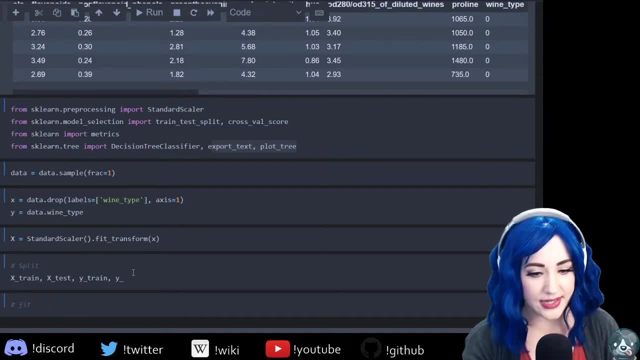 We're gonna need our X, our training X and our testing X, And we need a Y train and a Y test as well. And today, sploit, split. We are going to do a 70, 30 split, So our test size is gonna be 30.3.. 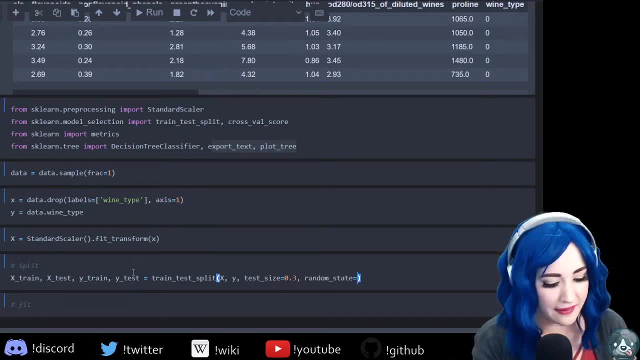 30% of our data And we're gonna put a random state here for anybody that gets the code. All right, We have split it And as a kind of like pro tip. So one of the things that I do, that's a notation for myself. 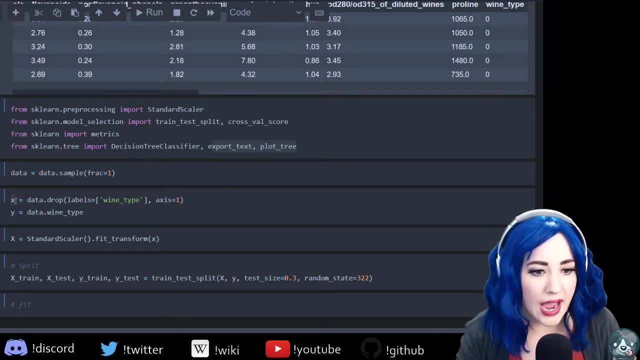 is that when I haven't scaled my feature vector, my X, I make it lowercase, And then when I've scaled it, I make it uppercase, And so it's kind of like this reminder for me when I'm- you know, train test splitting. 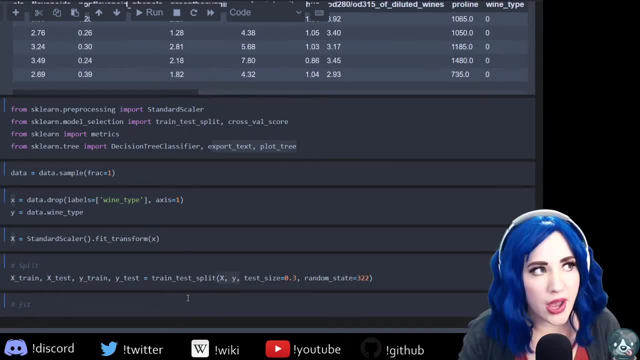 or where I'm fitting or anything. it's a reminder of like whether or not I've I've scaled my data. So little pro tip if it helps you And let's see. So you say really need to understand cross entropy loss function. 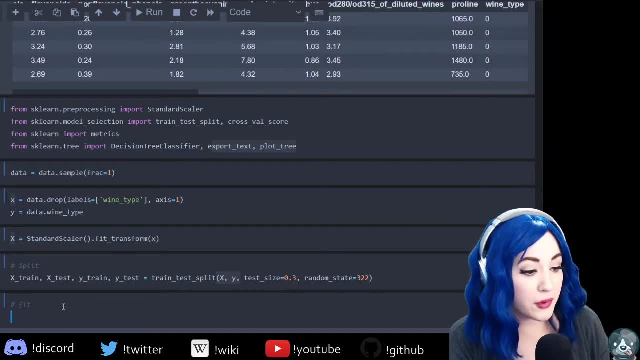 Maximize the maximum likelihood of function, or what so? lecture day on Fourier transforms. Fourier transforms are awesome Cross entropy loss functions. So that's a little outside the scope of today, but maybe I'll do. let me add this to my stream list. 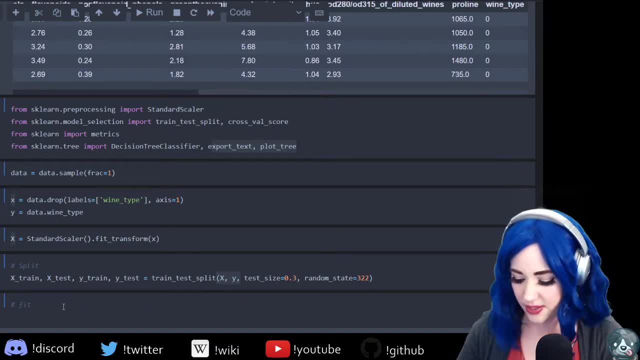 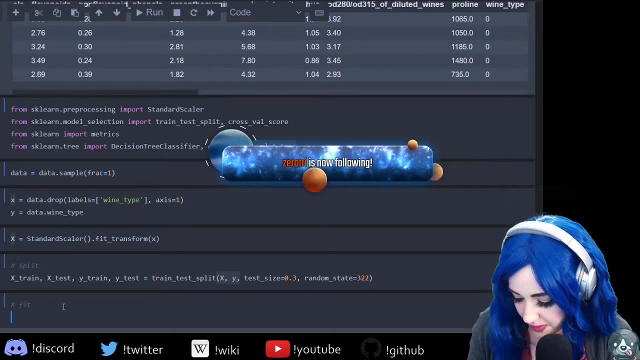 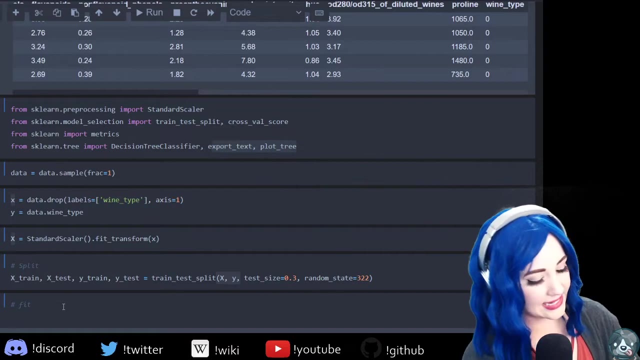 but I feel like I've gotten enough questions about different loss functions, that talking about doing a whole stream on loss functions Loss functions might be a good idea And Zero Tree and Meek Tactic welcome, Thank you. thank you so much for following. 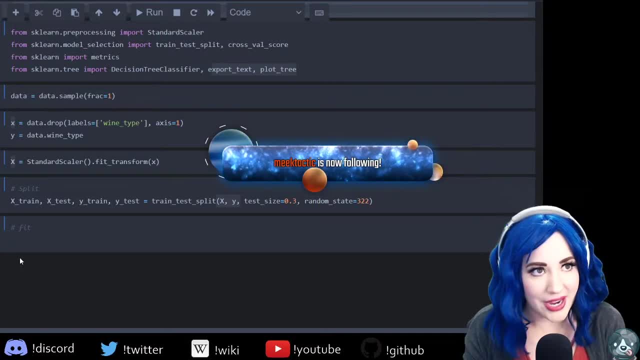 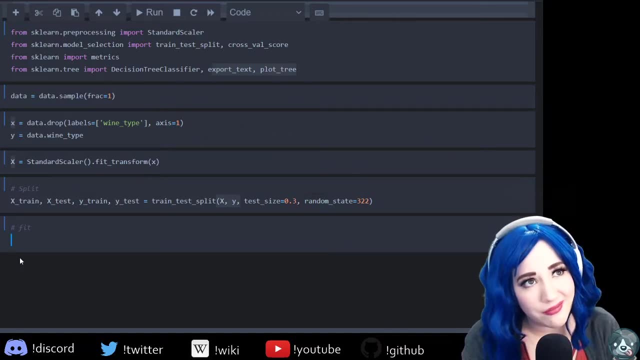 And yeah, I'm so stochastic lawyer, I'm always open to taking more ideas for stream topics. There's a lot of times I'm sitting here and I'm like: what do I stream? What do I do? And I'm like tired or something and I don't have any ideas. 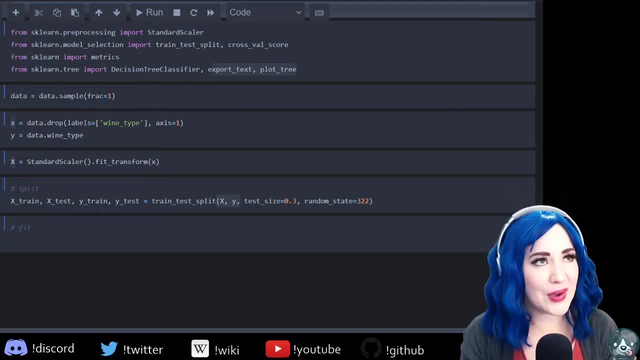 So definitely love, definitely love getting ideas, So I will. hopefully I can put together a stream on loss functions and we can talk about cross entropy. Z hi Zorkenheimer, Hopefully you're in chat. I try to tell myself to wait. 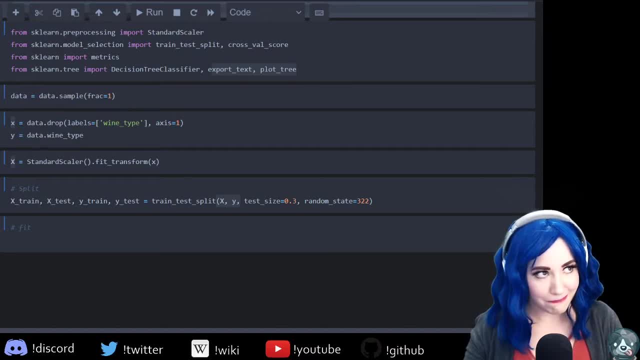 So I've got my little raid command. that's like wait, I've been great. Thank you so much for the raids. Let me give you a shout out. So what? how was your stream? What were you doing today? Oh yes, look at that. 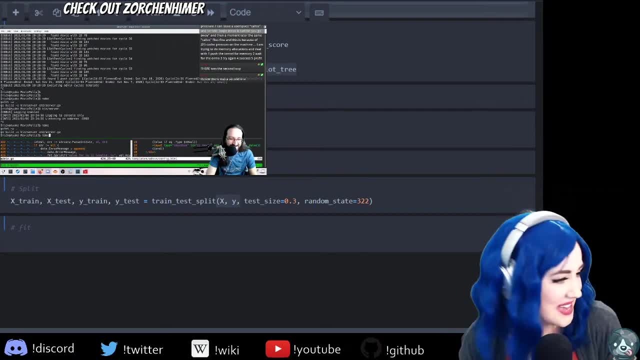 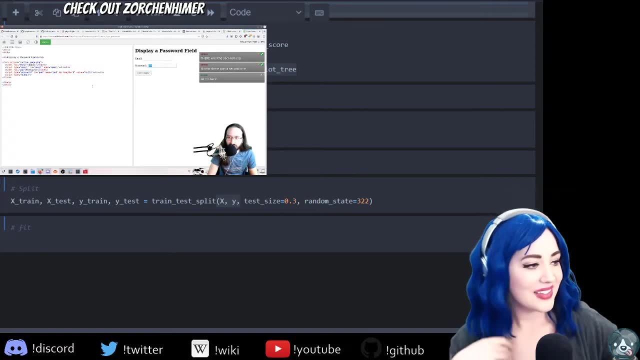 Look at all that code. Oh, I love when the clips are so good. It's too small for me to be able to tell what you're doing, but hopefully you had a good stream. You say you were actually productive. Oh my goodness. 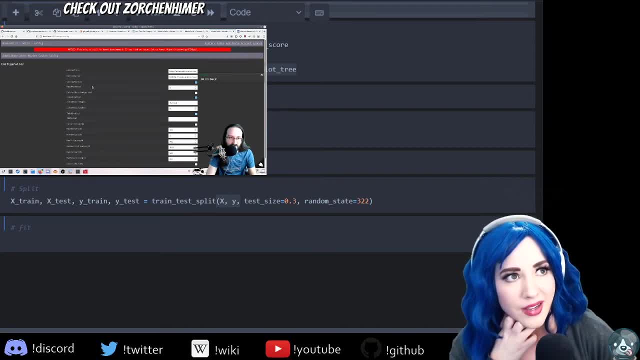 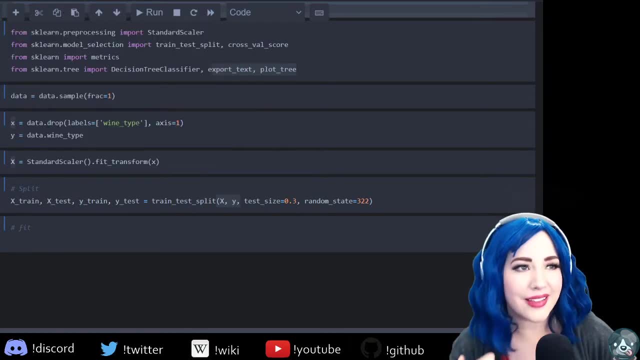 Productivity on stream. Oh, it depends. Like I feel like I get distracted with tangents but I love like I love tangents, I love talking to people about different things, but I actually had a really productive stream, I feel like Thursday I stayed up way too late. 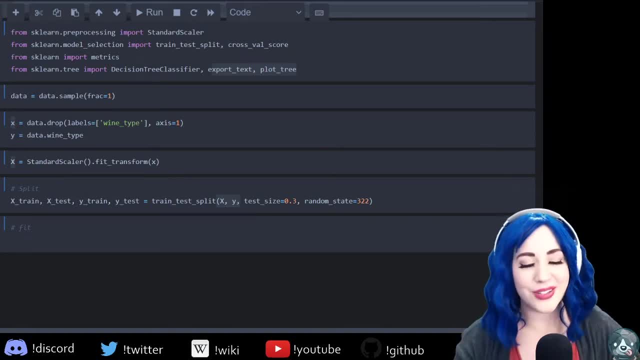 I made some bad decisions, but I got to do a lot with game devs So it was really fun. A hacker quote generator, What He went on? a half hourish tangent on V2.. Oh God And Melcore, thank you so much for following. 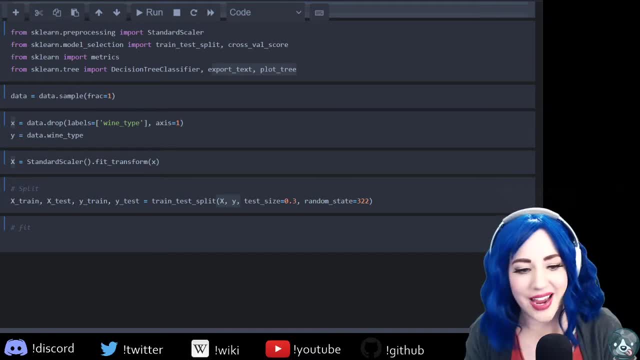 You know what, Luke? those are the best times when you're just kind of like messing around, having fun. So to catch you all up on what we're doing today, I did here go back to our whiteboard for a second and I'll zoom out so you can see the lay of the land. 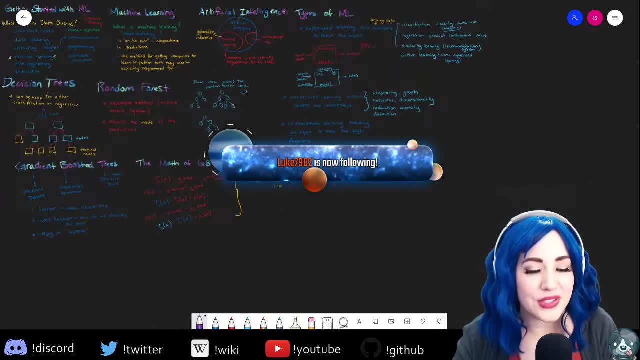 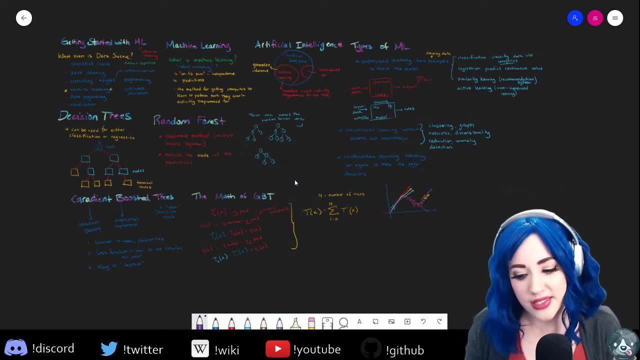 for all our Raiders And thank you for following Luke. So today is part of a stream series I'm doing. Well, first of all, it's science. Well, it's science Sunday, but other than that, it's part of a series of streams I'm doing. 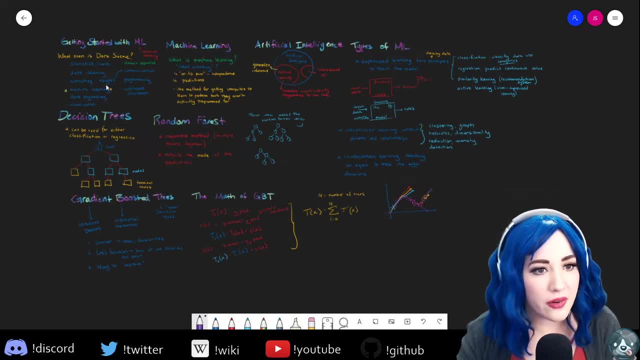 on the fundamentals of data science. So kind of did a little bit of review: What is data science, Did a bit of a review of like what is machine learning, What is artificial intelligence, What are the types of machine learning? And today we're doing gradient boosted trees. 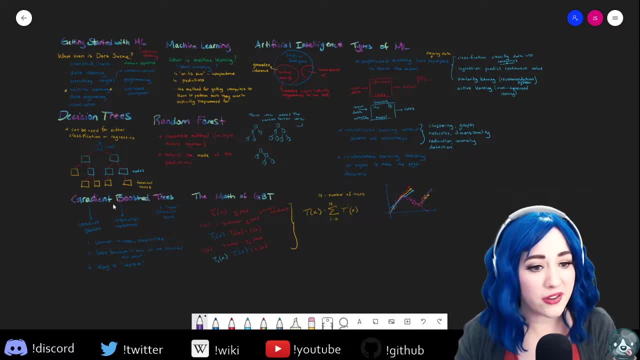 So I did kind of like a quick review of decision trees and random forest models then introduced to what gradient boosted trees are A little bit of some math too- not scary math, Don't worry- basic math. And now we're getting into the code. 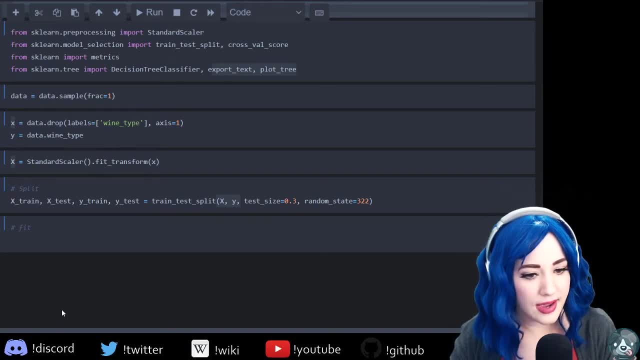 So now we are building each of those three models that we talked about, So a decision, tree classifier, random forest ensemble of models and gradient boosted trees. So we just started actually with the code. So you're here right in time, And JL354,. thank you so much for following. 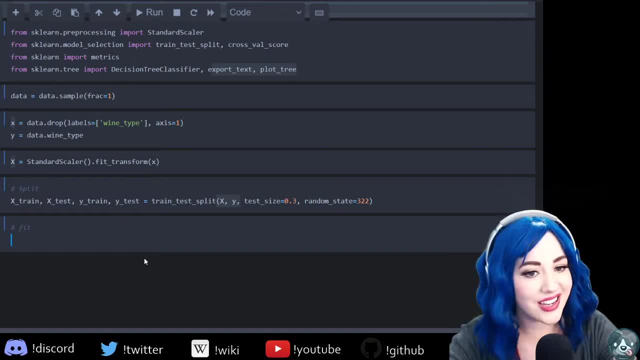 Now let's see translation. the way to a girl's heart is through gradients. Translation. the way to a girl's heart is through gradients, So let's do that. So Awesome, Did you see? Okay, so I love translation. I can translate this into juga Chinese. 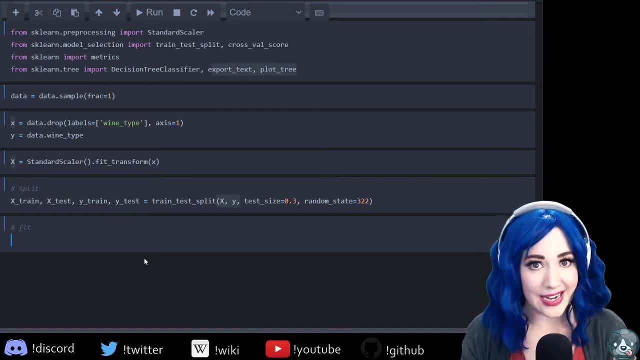 I've been trying to change that to English so it's easy. So we hope you guys have fun. I'm somehow not manuallyneck. I think this is the easiest way to useritoanline. Sie is unlike the trust test- and i keep slurring these words- unlike the training and testing data which 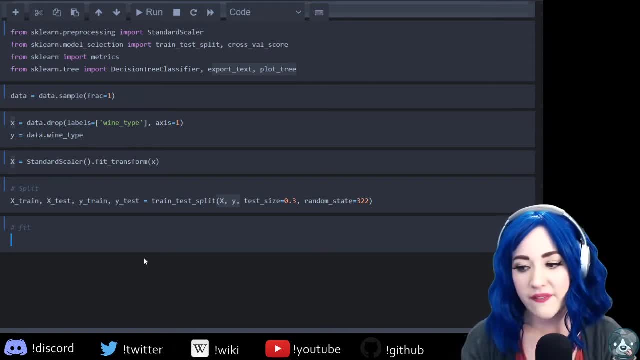 come from the same data set. they're just split um. our validation data often comes from a completely different data set, so in that way it's kind of more of an authentic test for how our model's doing um. and so let's see, you know those hacker characters and movies that spew techno jargon. 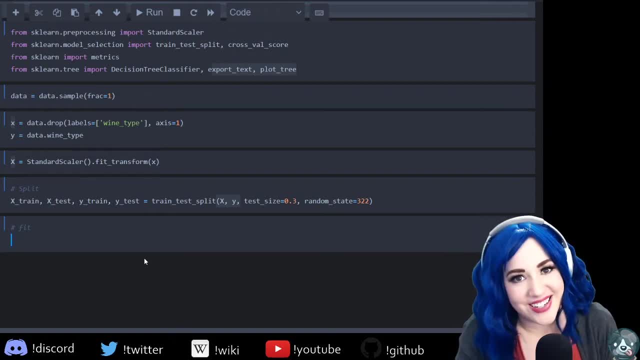 oh my gosh, you made like like a text, like a speech generator, but for like- oh my god, i'm sorry, i'm like just sitting here dying because that is hysterical, and i bet it is. did you so? did you have like a data set of movie lines where you were just kind of like training? 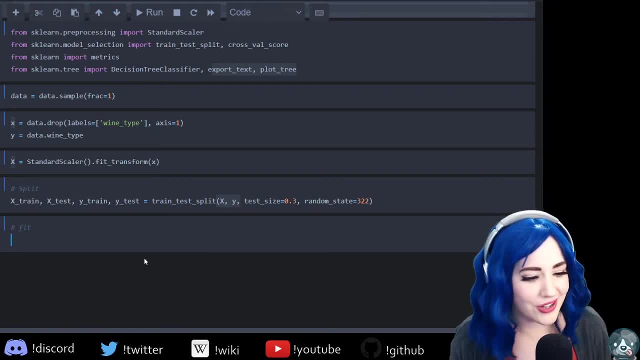 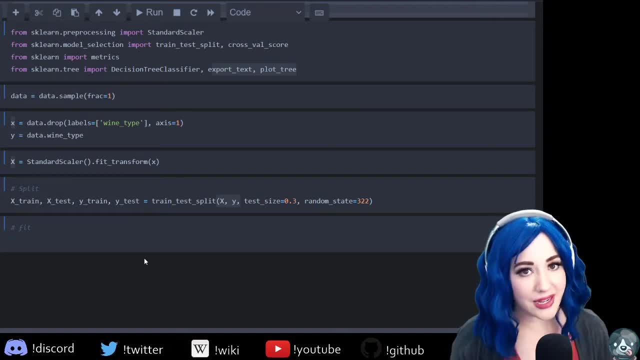 actually actually so mondays. if sundays are for science, so we do science sundays. on sunday, uh, mondays are for math and i do math mondays and we're starting with algebra. so literally last week our math monday stream was like: what's a variable? 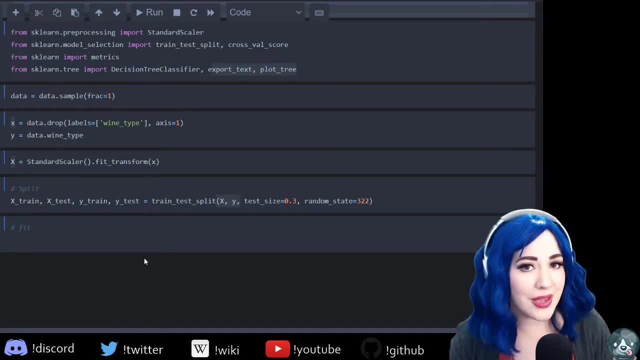 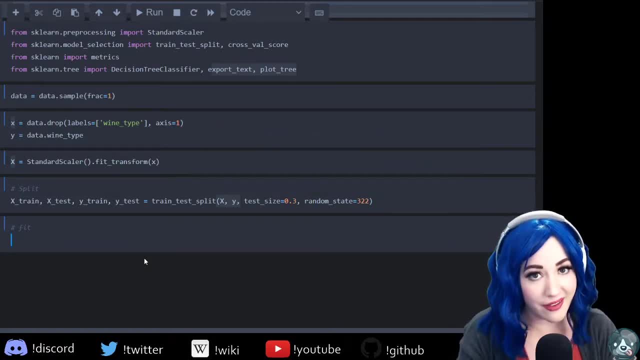 I love math and I hope to convert everybody, whoever talks to me to love math. but you know it's a process. And wow, Jinxy, thank you for following. Let's see. So you say I'm porting a project I found in Python to Go. 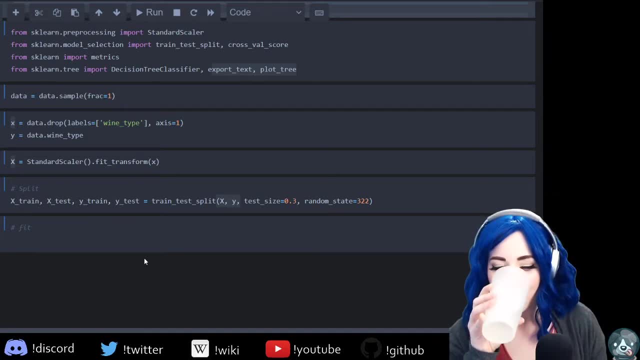 Oh, cool, wait, it doesn't use any ML. You can't bypass an offline interface, it'll forklift. Okay, All right, so it's more of a randomizer. That's hilarious, though. Also, how is Go? 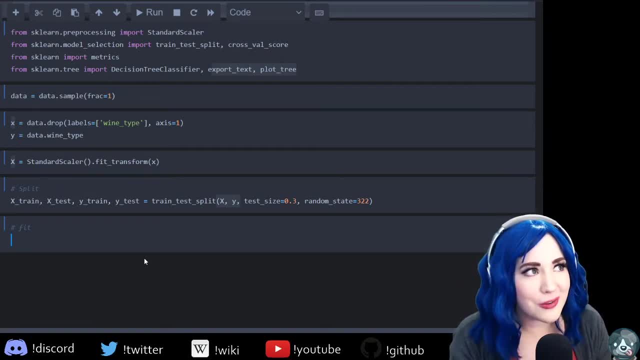 Like it's been on my list to learn for ages, but I'm like juggling way too many languages right now. I'm learning C sharp. I need to brush up on Julia again. I probably have to learn JavaScript at some point. So Go is on the list, but like the list is long. 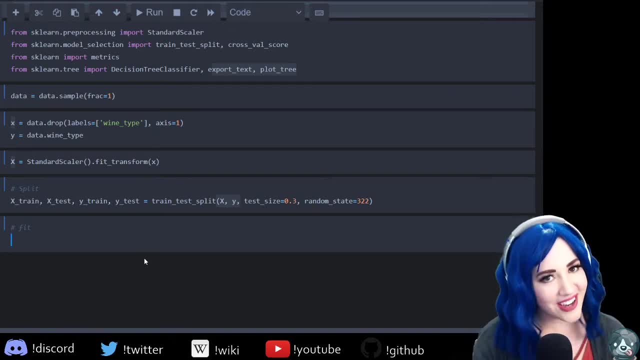 but I've heard really good things about Go, So it's your go-to language, Oh, lately. So I feel like I'm getting more comfortable with C sharp. I really like it. I really really like it. I just do. 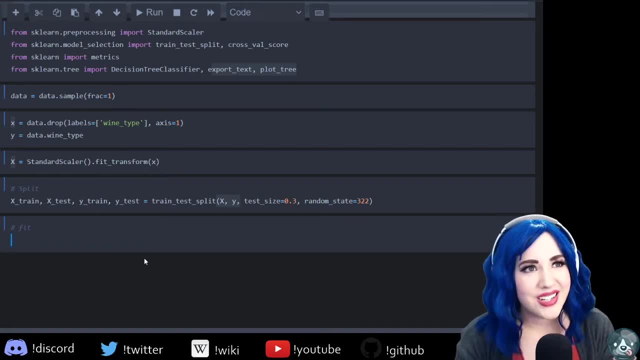 But Python is like it's what I use for work, So it's always gonna be the language I think I feel most comfortable in, because it's what's at demand for. like, I pay my rent because I code in Python. So, and oh, C sharp is actually what you use professionally. 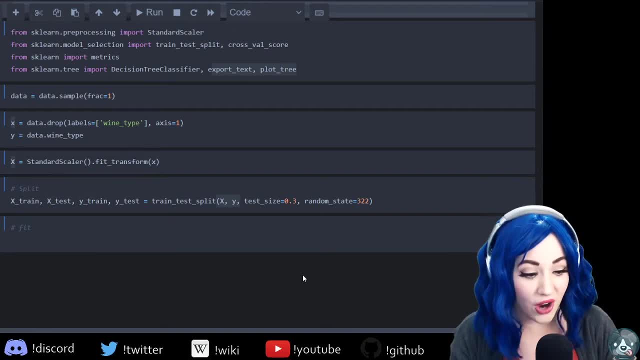 Well, don't come to my stream on Thursdays because it'll probably make you cry because I'm still learning C sharp. I know I love it. It doesn't love me back yet. So I guess perfectly themed for Valentine's day: My C sharp. love is unrequited. 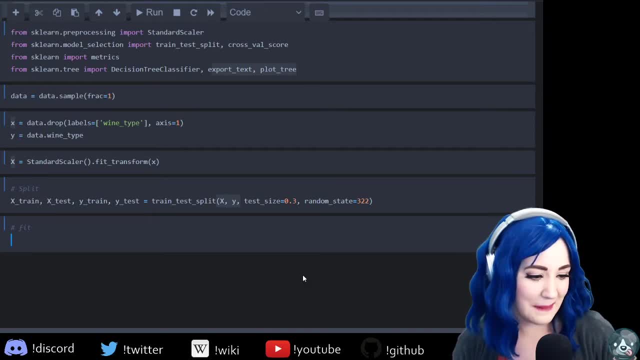 I love it so much, I'm just very bad at it right now. but and, Carlos of Ginger, you say you're going back to extreme basics with math to relearn from scratch. oh, that's awesome. like one of the things that we talk about on math mondays is that, if you feel like you're bad at 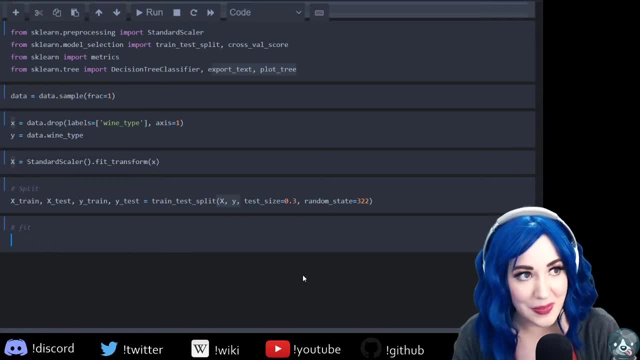 math. i will make you a bet- okay, i will make you a bet- which is that you probably aren't actually bad at math. you've probably been taught terribly. and i say this: i've tutored for 15 years. i've tutored all levels of math, from like second grade math all the way through differential equations. 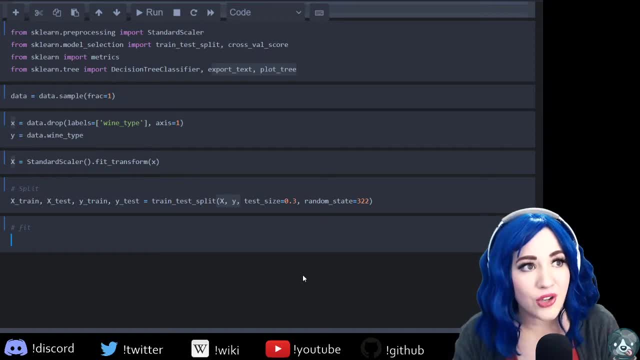 i have tutored so many people who thought they were bad at math. i've tutored a variety of different ages learning disabilities and not a single one of them was bad at math. i haven't met somebody bad at math yet so shifty, shifty. thank you so much for following um, let's see. uh, yes, using it. 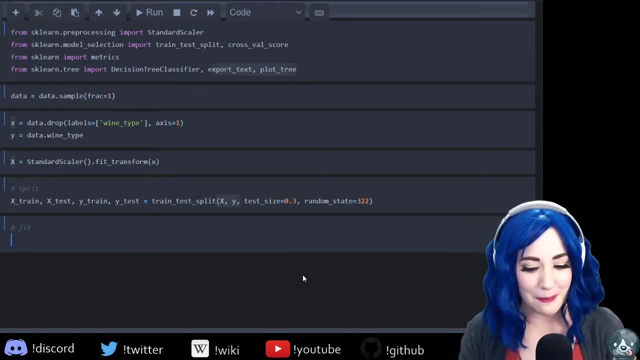 for game design. exactly, kevin, that's what i'm doing is i'm learning unity and c-sharp, but like kind of on my own when i'm not doing game design with c-sharp. um you, i'm just like doing c-sharp for fun. i don't know, i really like it. 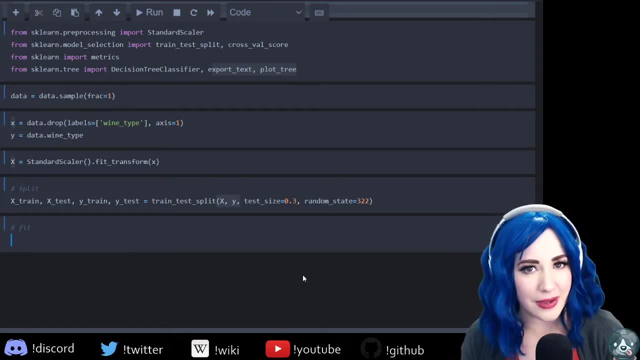 it's cool like it takes everything that i love about c and like it basically has a baby with the things that i like about python and i like that. so, um, c-sharp, josh, saying you love c-sharp, and no worries, have a good night. i'm glad you were here. 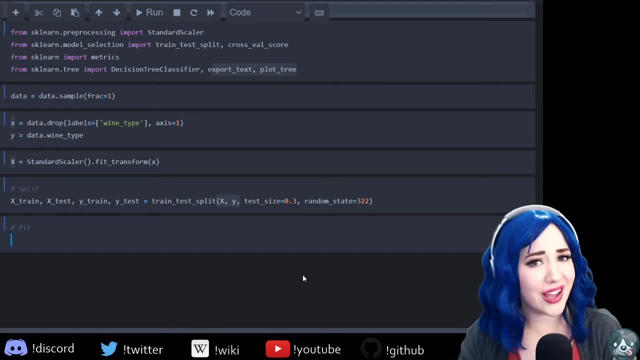 i should guess i should do a learning c-sharp stream at some point. but y'all got to be gentle with me because i'm new. i'm learning um. but, master darkweaver, you say you have this book, math adventures with python. that sounds really cool. um, j holly, bring it on. you say no one's bad at math, hold your beer, bring it on. 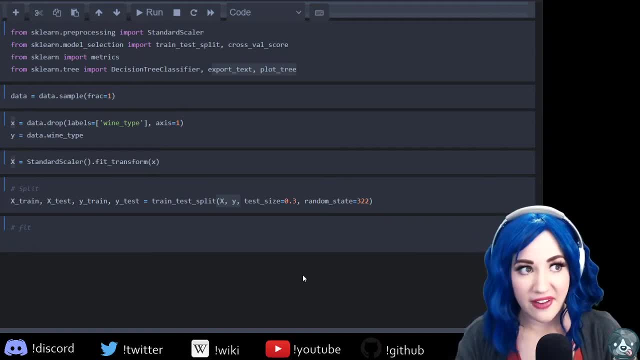 might take time. i've never met a single person that is bad at math. i've met people who have years and years of ingrained beliefs about their own math proficiency. um, i've tutored people with extreme anxiety and stress around math. extreme hatred for math i've never, ever experienced. 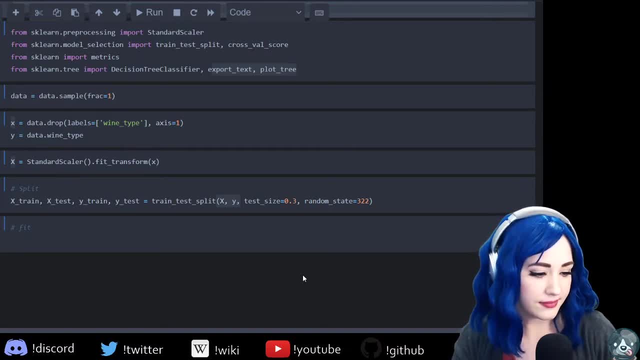 somebody that was just bad at math. um, and let's see the oh goodness um the epic unknown. you say: go as the modern version of c, as rust is the modern c plus plus. i've heard good things about rust too, um, but i i guess what i liked about c sharp is that it took 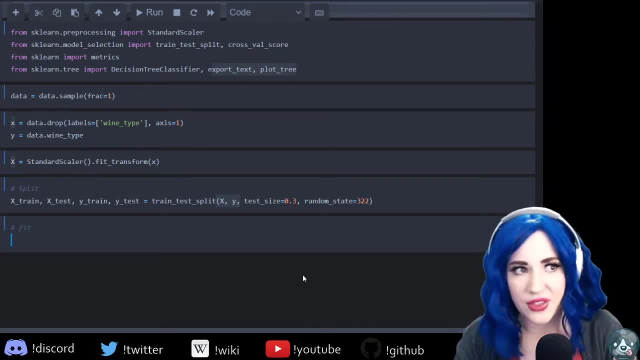 some of the things that i've loved about python and it didn't take the things i don't like about python and so for that reason i've really liked it. but also, like i've talked to a lot of you about this early in stream, but like my origins were as a linguist, i love languages, human or like. 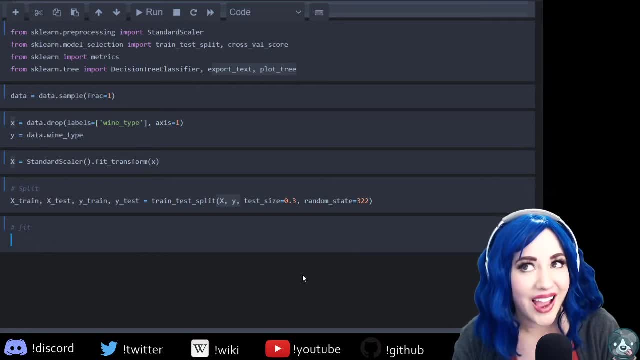 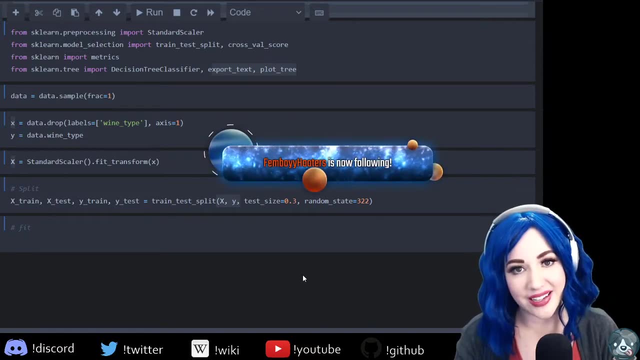 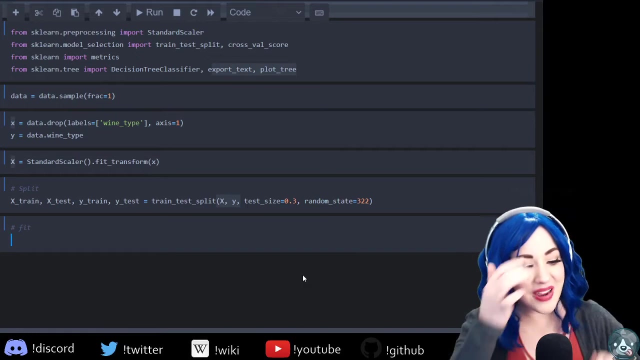 programming, and so i think i just love learning languages, so i'll probably. i've never had a a language i've hated, but i've never had a language i've hated, but i've never had a language i've hated- really sort of um and femboy hooters- what a name welcome, welcome to stream. have ever made a? 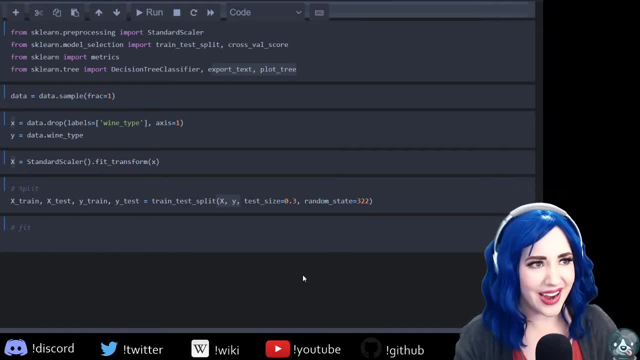 conlang, please. how do you think i got through like high school having no friends? i had more conlangs than i had friends. and julia is very cool. yeah, i've enjoyed. i've enjoyed learning some julia as well. um, and yeah, see, master dark weaver, you say you had a math tutor in junior. 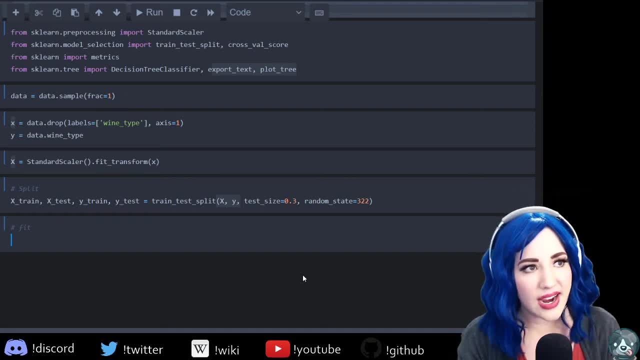 high she had you play bridge. yeah, there's like a lot of times if somebody feels they're innately bad at math, it's bad teaching probably, plus maybe um, like not not strong enough number sense and so just like a muscle you don't use if you haven't. 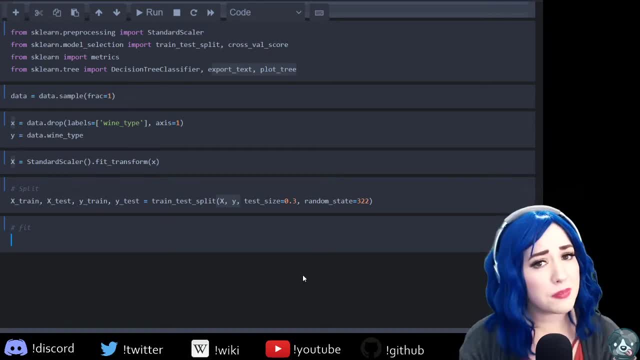 trained your number sense and really like developed it. that can help. that can make you struggle too, and there's lots of um, lots of cool ways to to learn better number sense. and pope gecko, you ask what other human languages, if others, do, i speak, so right now, sad pandas uh. 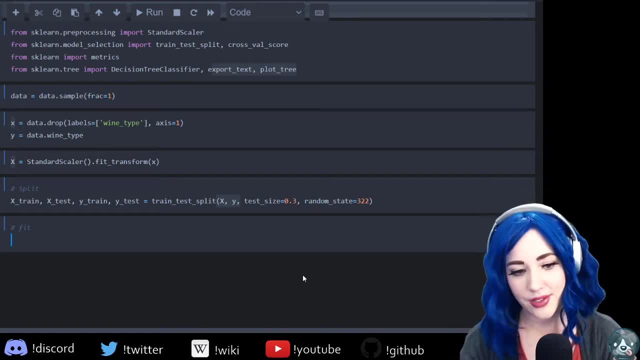 since, since switching careers and doing um ml development, i have lost my fluency in pretty much every human language but english. previously, i was fluent in- uh, french and arabic as well. all right, let's, let's fit our model while we're talking. so nothing funky going on here, folks. 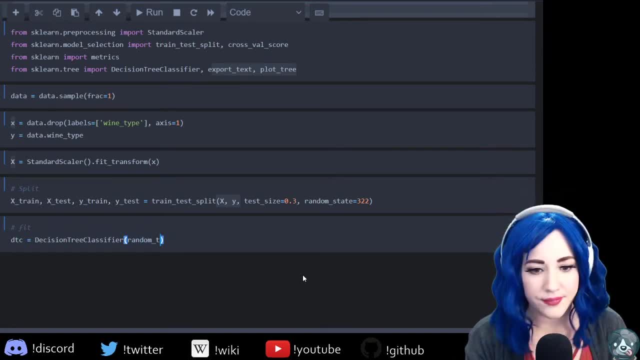 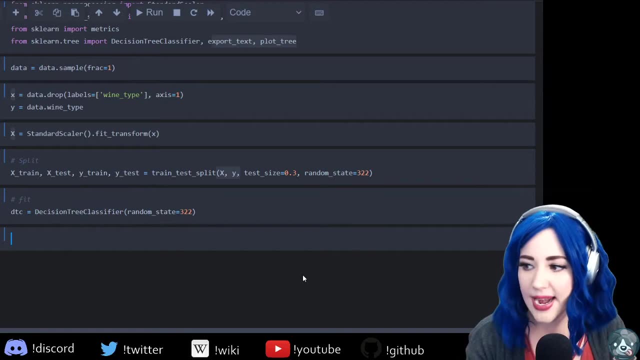 we're just taking our random tree. we are taking our decision tree classifier. we're taking our, we're just gonna instantiate one with a random state and now we're gonna fit it. So let's feed it right. We just wanna feed it our training data. 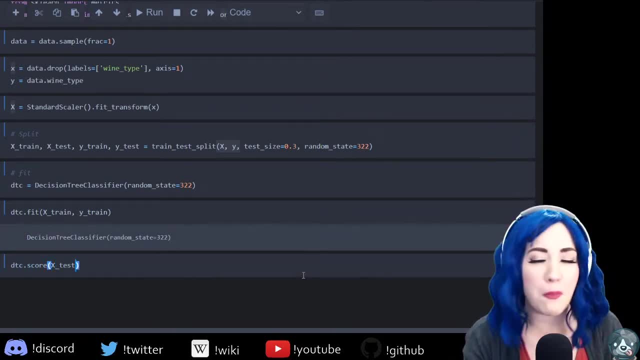 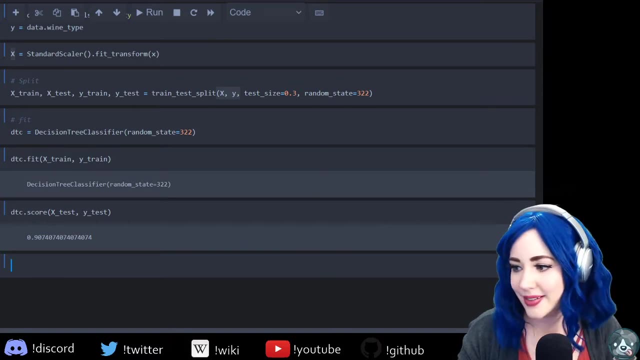 and let's score it. So this is doing just basic, basic accuracy. Hey, not bad, not so bad. right, It's not the worst, but you also gotta remember, right, This is one of those like really nice clean data sets. 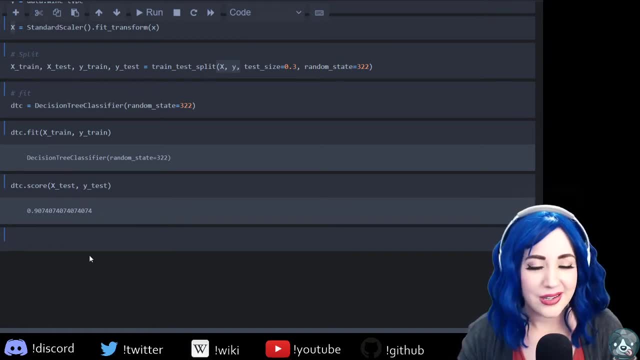 Like I'd be pretty happy with that on a trash data set. but this data set's like cleaned and balanced and like smooth and suave, and we should be able to squeeze some more performance out of this. Let's see. oh yeah, no worries. 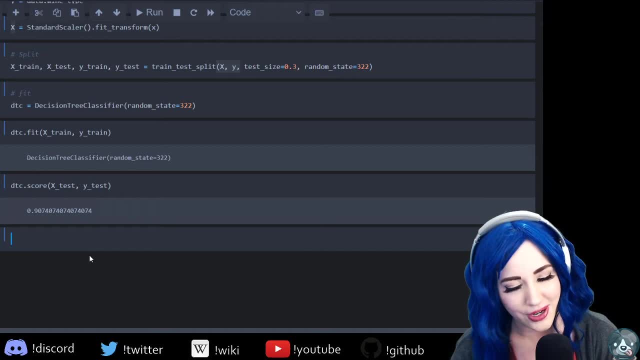 Seriously, Z. I know what it's like after a raid where you're just kind of like: oh I've been streaming, So relax, you don't have to. you can lurk if you want. but, like, please feel free to just do whatever you need to. 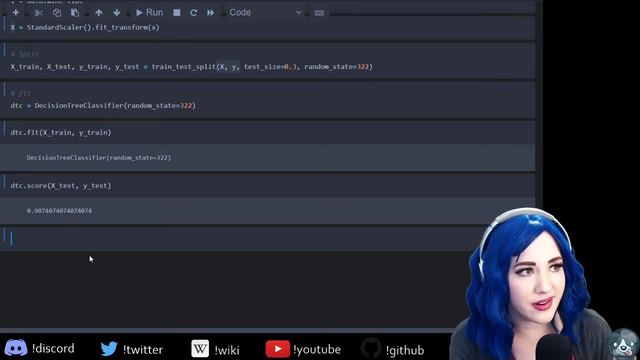 And ProfessorSaucecat, you missed getting a gift sub. We had a bit of a hype train earlier. it was amazing. I got really flustered. I got really like red. I had to open my window. I started to overheat. 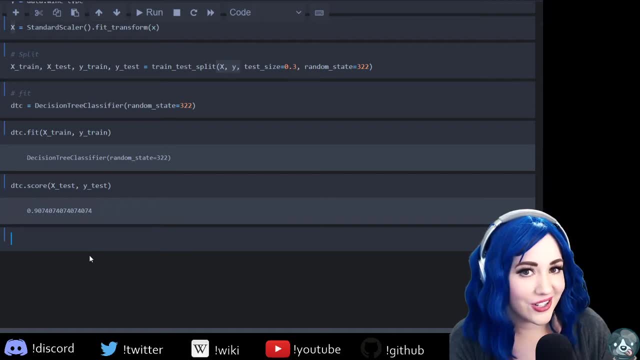 It was amazing though- And I'm pretty sure you got your gift sub during that rate or that hype train, And let's see. And, Pablo, when you say you feel like general culture convinces people they are bad at math, they see it in TV shows and movies and internalize it. 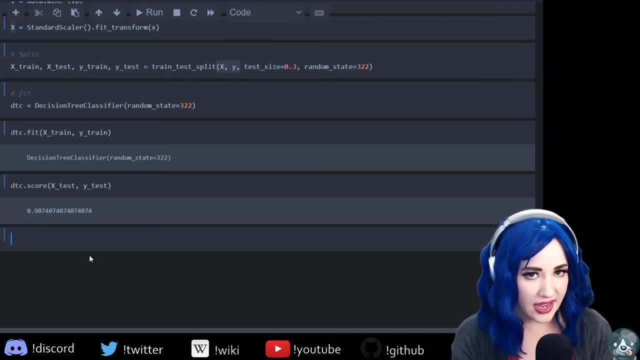 Also- and I'm sure that math teacher has seen this, but I've had math teachers where they don't seem to like math. They're like: I'm sorry, we've got to do some math And you're sitting there like 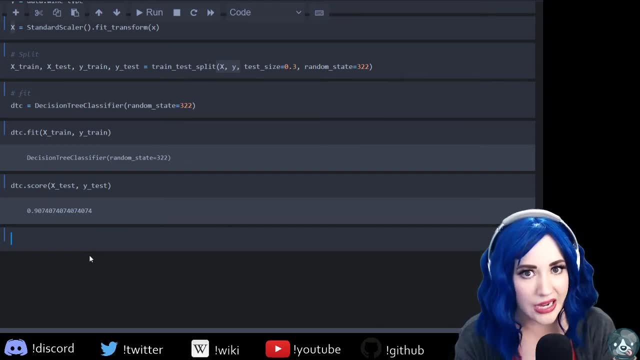 how am I supposed to love this if you yourself are teaching it to me and you don't like it? So sometimes it's just like it's enough to just love it and be enthusiastic Like that has made a huge difference when I'm teaching. 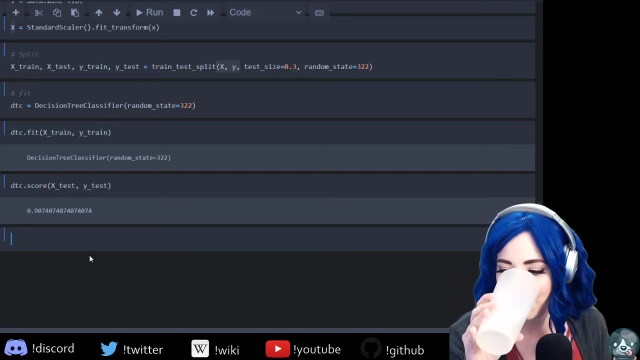 But gaze into the iris. I will hydrate, thank you. I also need chapstick. This is what I got. I got really flustered. I started to lose my voice Because I was like screeching so much with the hype train. 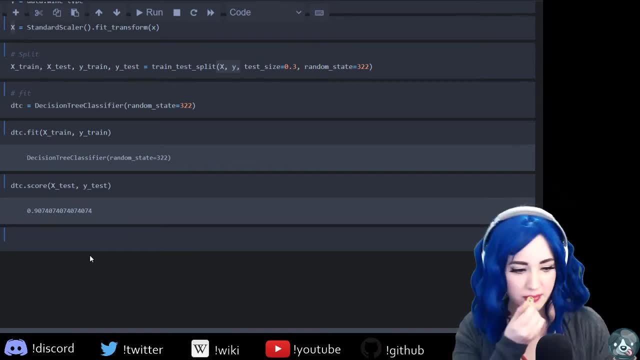 So probably not my most elegant moment. Oh, I agree that math teacher they shouldn't be. They shouldn't be math teachers. Okay, I have not tried Unreal Engine, Luke, just Unity so far, because I'm a beginner And Stochastic Lawyer. you are predicting my next thing. 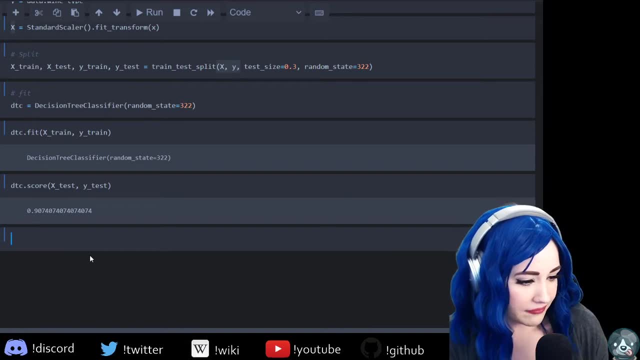 My next thing I'm going to talk about, So stay tuned. And, Dominic Evans, let me give you a shout out. I love your stream, All right. So I know you're not streaming right now, right, You're still working on like film, disc stuff, but, Dominic, 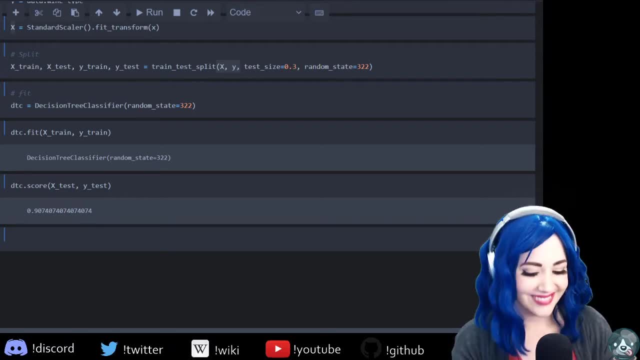 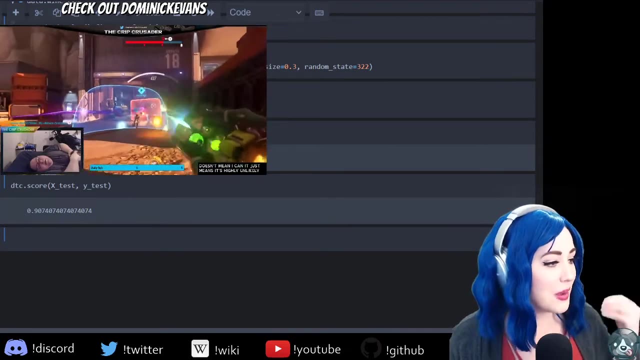 Okay, Well, I just turned you into it. Hold on, I got so excited that I didn't even do the shout out command. You all should seriously give Dominic Evans a follow. Amazing, amazing stream. Fellow disabled streamers. I love you. 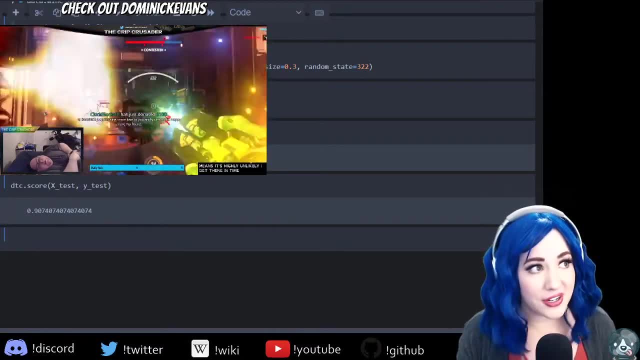 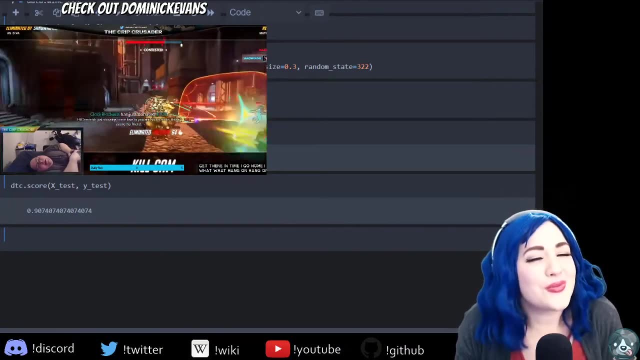 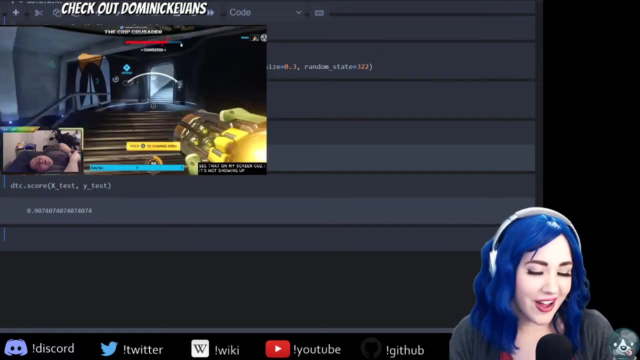 I'm a gamer streaming all about accessibility. So we were talking earlier about accessibility in games today- No Thursday probably, And just a wonderful, wonderful stream vibe. So definitely, definitely check out Dominic Evans and throw a follow. throw a follow. 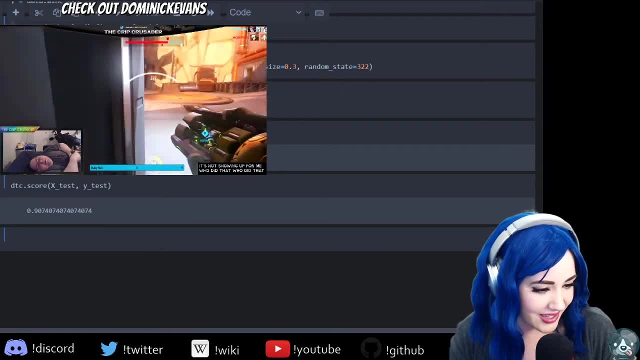 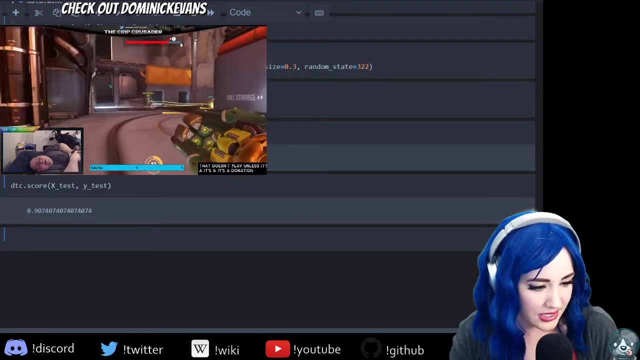 Also look at this. I like your emotes. I think, yes, Do I have emotes? I think I subscribed last time. but I also like: okay, I have too many pages of emotes- Crap. It's gonna be forever to scroll through those. 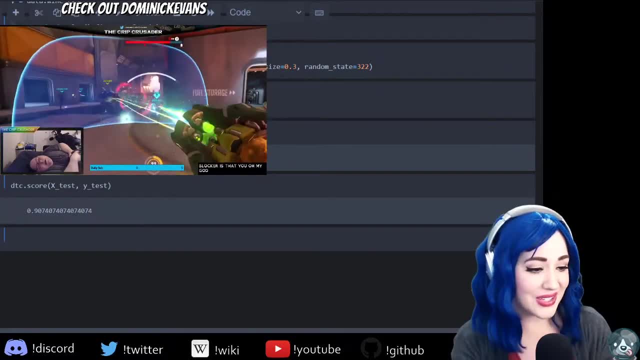 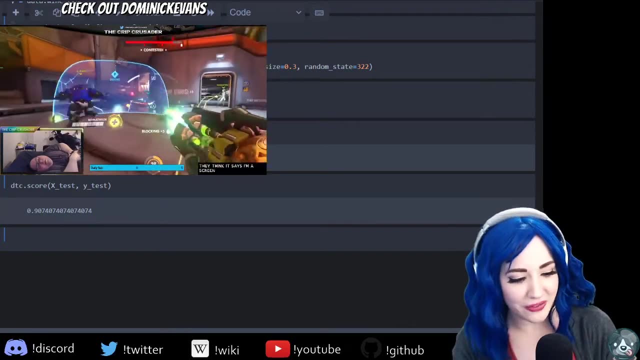 But in any case, welcome. It's so good to see you, please. Yeah, you said lurk, Feel free to lurk, relax. And math teacher you say math is such a beautiful thing. If only more teachers could share the joy of math. 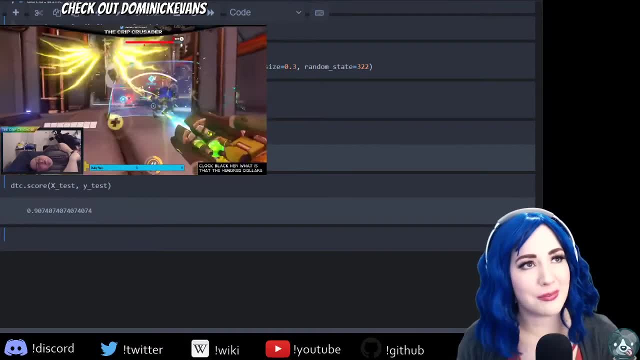 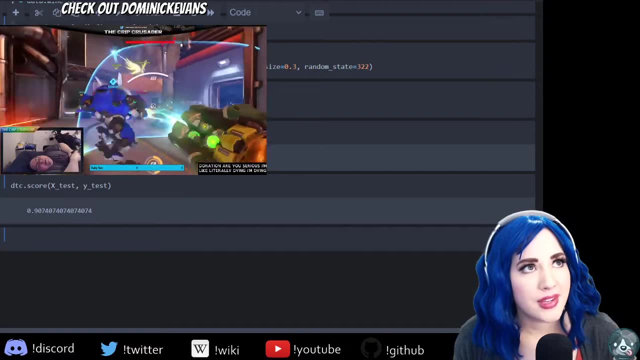 Agreed, And you know so. my mom is a perfect example of this, where she thought she was bad at math. She was really intimidated by math at first, Literally. when she comes into stream, she might be here tomorrow. Her handle is math, mom. 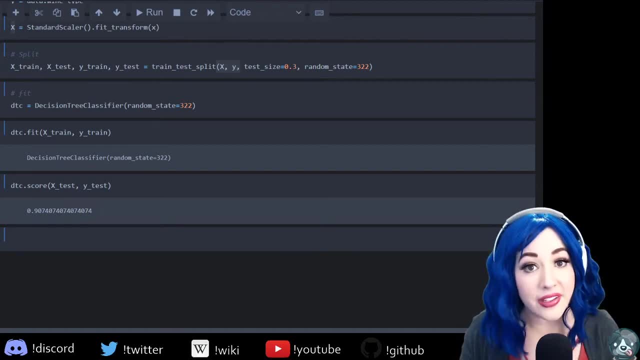 Because she became a math teacher, She started to learn math and she fell in love with it And she's a really good math teacher too. So like I definitely have some inspiration there, But because I think she used to face so much anxiety. 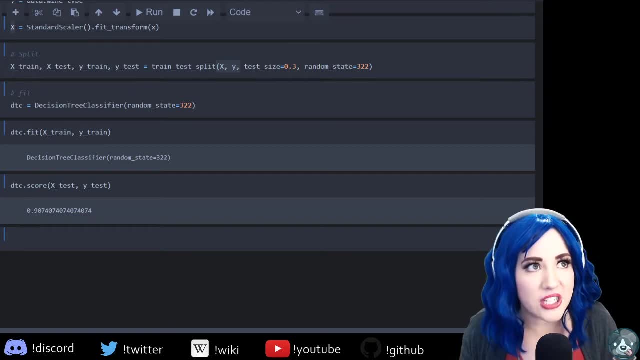 about math and think she was bad at math. She's perfect for kind of reaching those students that really struggle. I think she also got she got really burned out kind of doing public school because just the grueling, teach to the test, follow the curriculum. 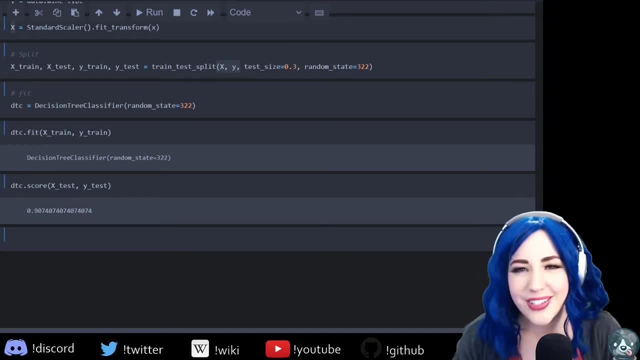 When she really wanted to be able to kind of challenge her students and create such a positive environment for math. But I really look up to her when it comes to teaching math, Cause she is one of the few few math teachers I've had that are amazing. 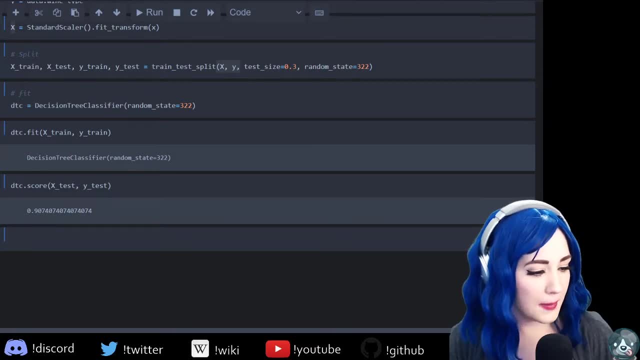 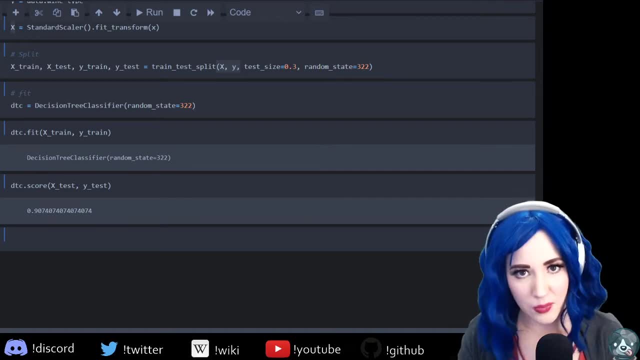 So we've got science Sundays, math Mondays. It says starting soon, but they've started. I need to correct that. Videos for those streams- science Sunday and math Monday- streams up on YouTube, code on GitHub, et cetera. Tuesday: right now is viewers choice. 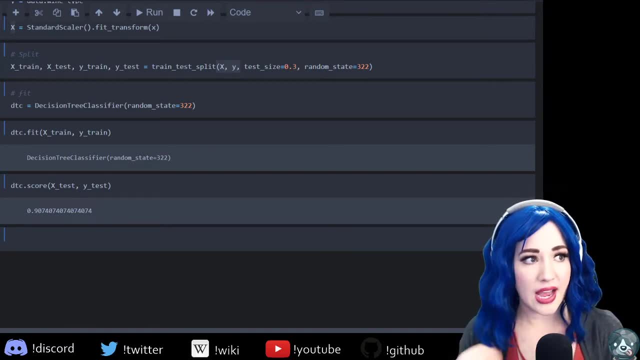 But I found that especially with my own chronic illness I get really exhausted after the Sunday and Monday kind of back to back streams that I've been having to put off the Tuesday streams. So I'm thinking about moving Tuesdays viewers choice to Fridays. 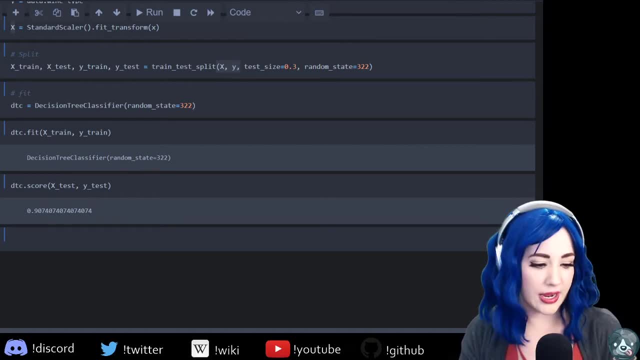 So then we would have Sunday, Monday, and then we would have Thursday, Friday, Because so far I have it like my stamina hasn't been able to handle it. It's not so great for my joints and I get really wiped out. 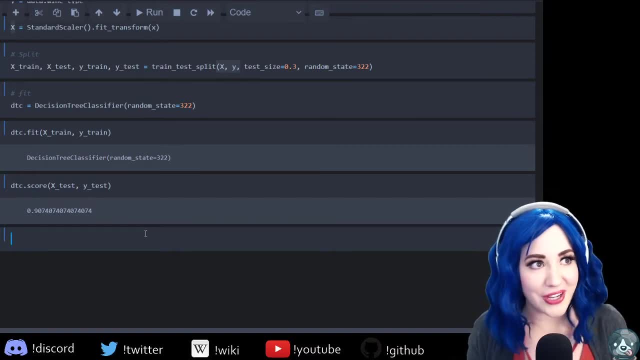 So I want to be able to. we've got lots of wonderful redemptions for games I need to play. So Fridays, fun Fridays. I'm going to keep with my alliteration here. I couldn't get a good one for game dev Thursdays. 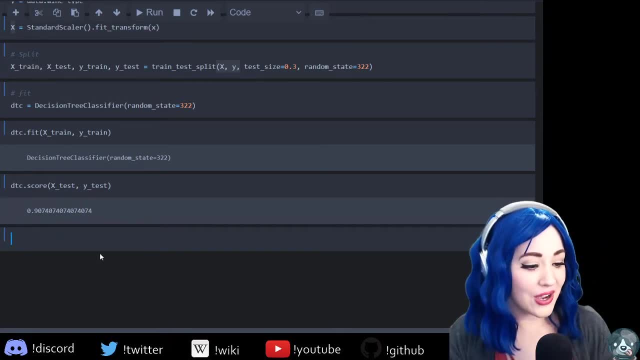 So sad face to Thursdays. but and yo, no, no, no, Lurk, all you need to. it's totally fine Lurkers, I love lurkers. They're like this constant, steady presence. So have no fear if you need to lurk. 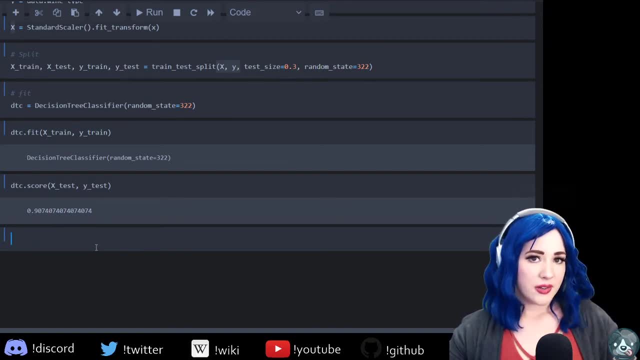 Okay, but so is this the end? All right, we got an accuracy measurement for our decision tree. Is that it? Are we like, yeah, we trust this 91%, We're good. Is this an accurate, an accurate decision tree? 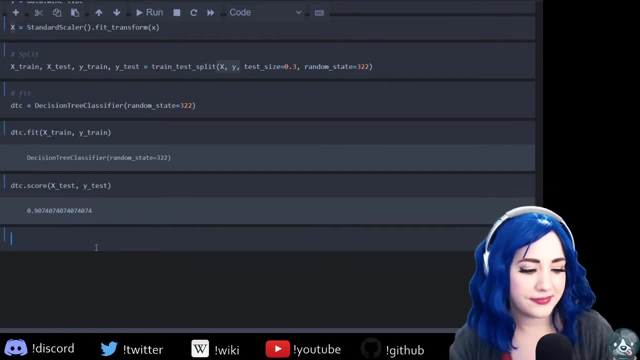 Is this an accurate measurement of how our model's doing? Looking at all of you machine learning miss folks, you should know the answer, And obviously some of you who know data science know the answer too. but I'm looking at you machine learning people. 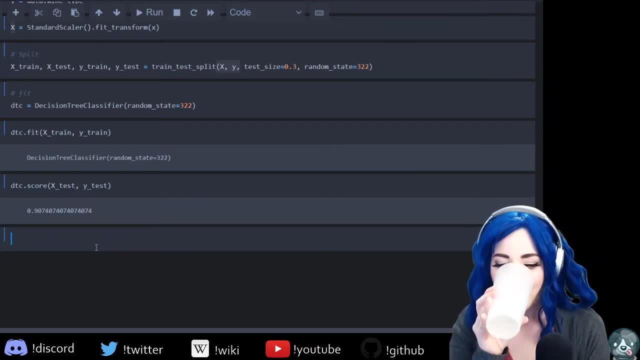 You spent 12 streams with me. you know the answer to this. So, Casa del Coneos, you bring up validation. Yes, so if we had a validation data set- we don't right now, but if we did- that would be a great way to test our model's performance- 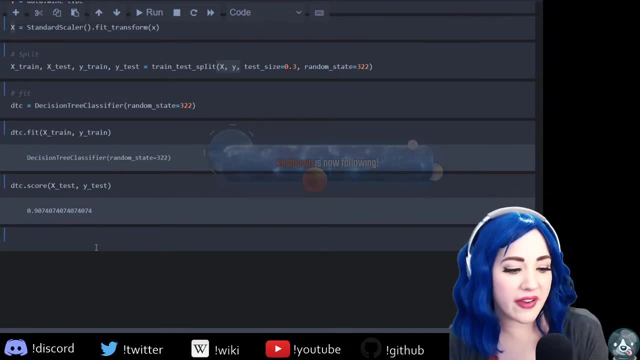 But other than validation. we don't have a validation data set. We don't have a validation. We have something. I mentioned it very, very briefly And Kind. Pawn, thank you so much for following. And oh, this is so, Luke, this is just a Jupyter Notebook. 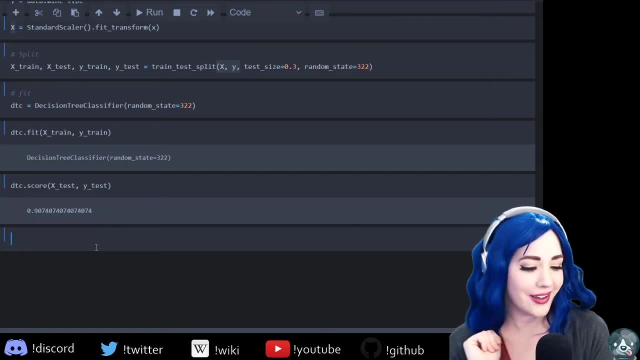 So formatted for all of you wonderful people in dark mode but, and with some extra things for me. but this is just a Jupyter Notebook And, yes, I'm never alone when I have lurkers. exactly, I know DJ Velour. 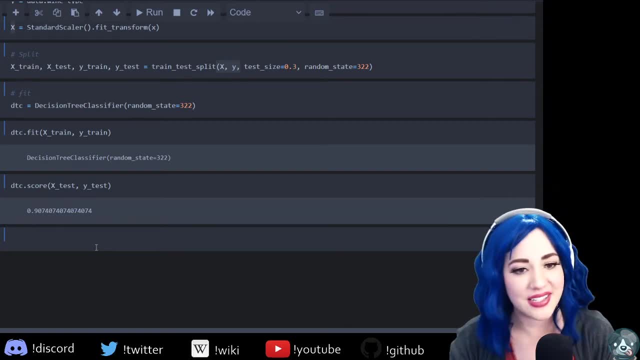 I spent the time customizing this because I was so tired of just the extremely bright Jupyter Notebooks. Stochastic lawyer says: the good news is there's no overfitting with 90%. Yeah, So probably not. but what are we missing here? 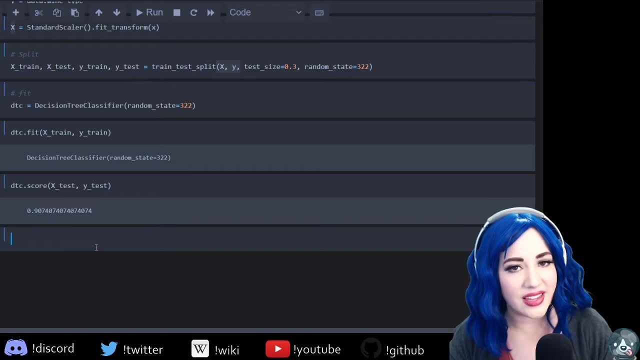 So I know it's been a while. We did. we did machine learning this in late December, so it has been overwhelming just trying and having fun with the thing. right now been over a month since our classification streams and and the last time we did decision trees. 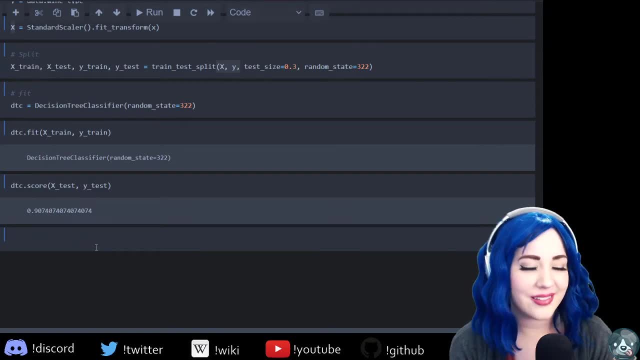 but think, think back, try to, like you know, bring yourself back to the past, or even think back to the picture that I drew. right, I gave you like a chunk of data and I said we could take this little bit for test and this little bit for training, right, but it's kind of. 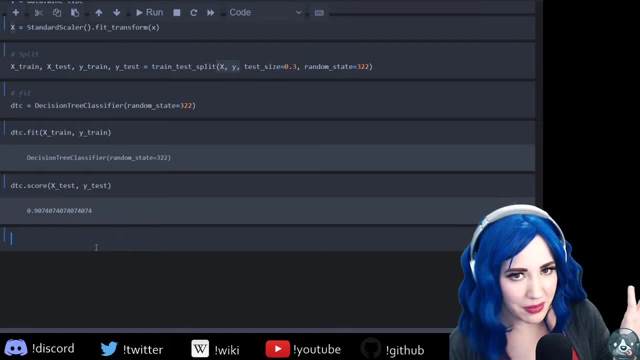 random. which data we pick for training? which data we pick for testing? so what? what might we be able to do here to get a better measurement of our models performance? give y'all time to think hydrate. yes, Kevin, you weren't even here. I don't think for machine learning myths, but you have the answer. 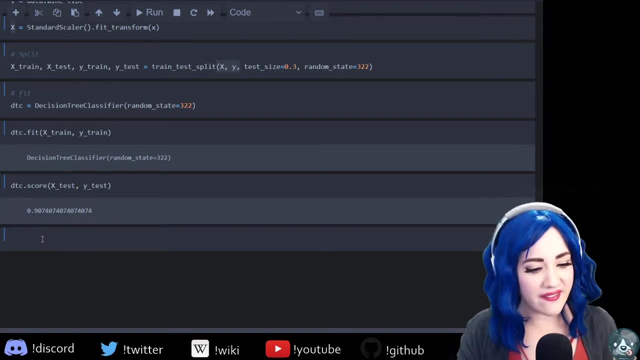 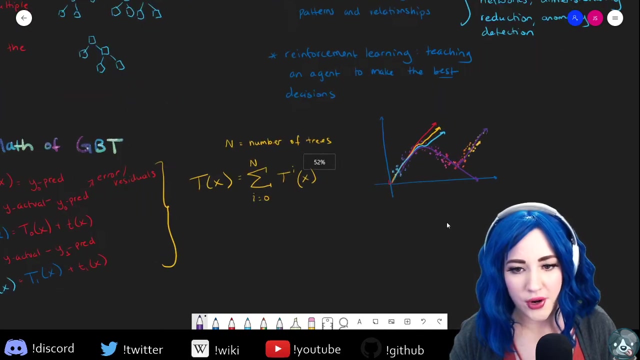 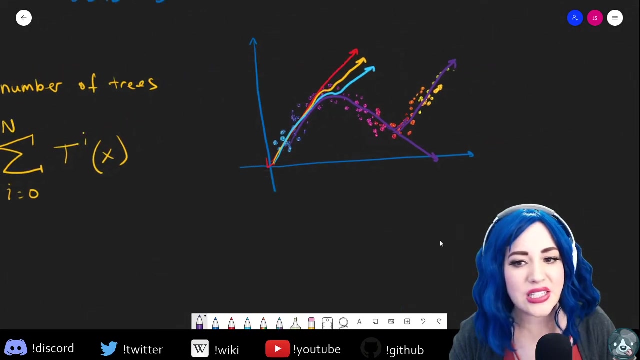 yes, yes, cross validation. what the heck is cross validation? so, ah crap, all right, we're gonna go back to the whiteboard for a split second while I just review for you what what cross validation is. it's best done visually. I could explain it verbally, but I just I don't know, at least for me. 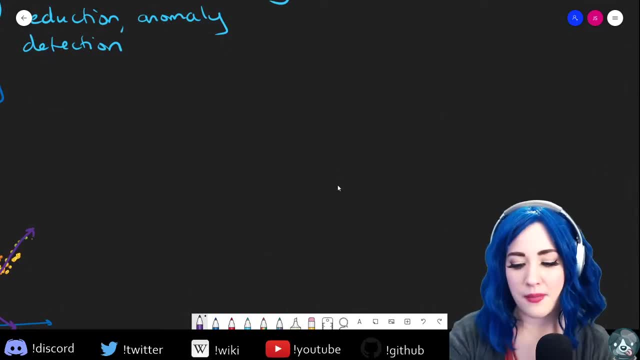 like it sinks in a little bit better when, when I draw it. so just give me one sec here I got a plug in all right cross validation. we're not gonna go to, just gonna review it. so the way we were doing things previously, oh shit, I bet that wasn't muted. knowing my luck, is it better now. okay, sorry, I need a new mic. I've said 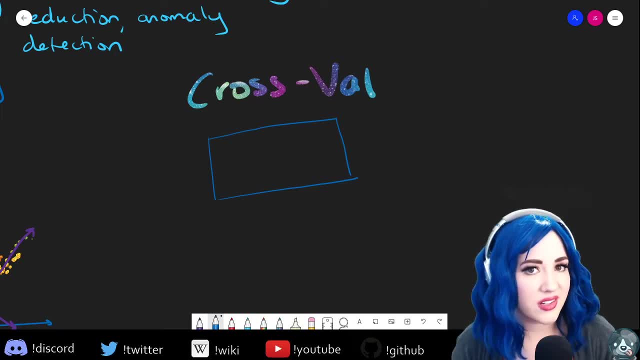 that for months, this one, if I like, breathe on it. weird, it stops working. so my apologies. um, I've replaced the cable, even, and it's not the cable, it's the mic. so, yeah, all right. um, okay, and uh, Kevin, no, no, but I thought I didn't think that you were in our machine learning miss. so it was. it was a 12 days of. 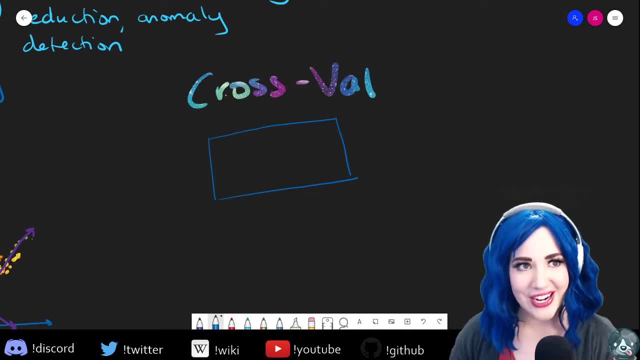 machine learning miss. it was a marathon of 12 deep dives into various machine learning topics designed to give people a familiarity with as much machine learning as possible. so somebody said it was like the same, like the same syllabus, as like a semester-long course they took in machine learning. 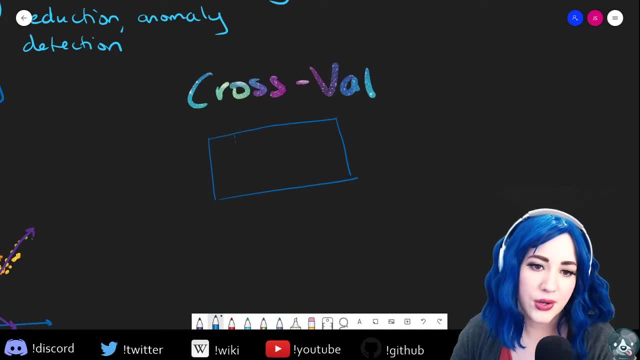 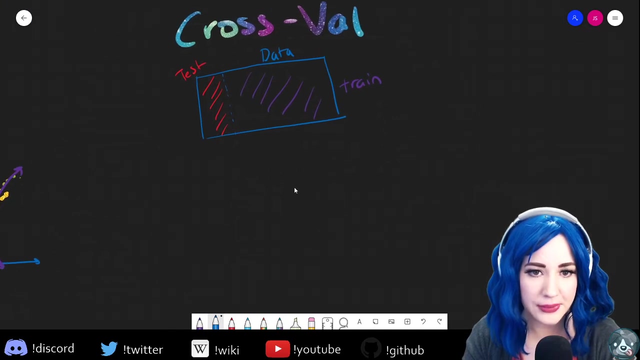 and I was like, oh my god, this is awesome. it is on YouTube code is on GitHub, all right. so we talked about how, if this is our data, we can divide it into our test data and our training data. right, training is what we feed our model. testing is how we evaluate performance, at least for now. 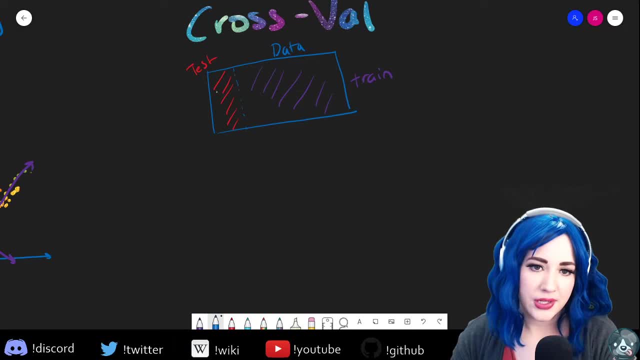 however, we run into some issues because it's kind of random how we select this, but we run the risk of overfitting to our training data. we run the risk of not. maybe our test samples are just easy. so cross validation or k-fold cross validation: okay, fold cross validation. 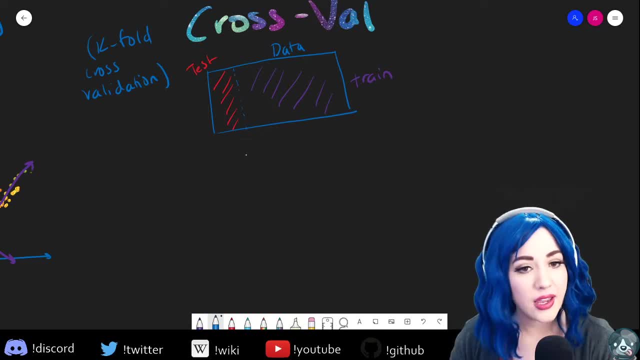 is a method that we can use both to avoid a little bit of overfitting and also to get better measurements, better metrics for a model's performance. and how we do this is we're going to just iteratively repeat this process, so maybe step one, this is our test. 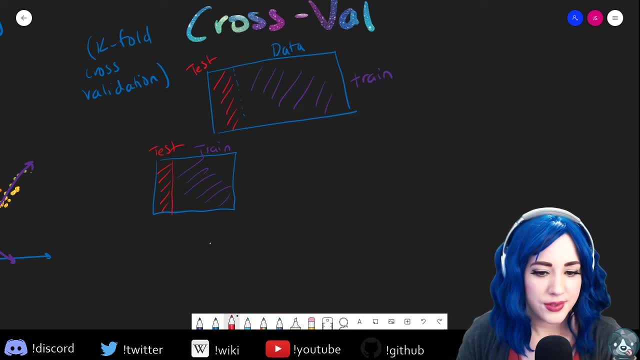 this is our train and oh no, I want a different color. hold on, we get a score, right shaped like an accuracy of our classification. then maybe next we grab. this is our test, this is our train and we get a score. each one of these kind of like shuffle and reselection is called a fold. 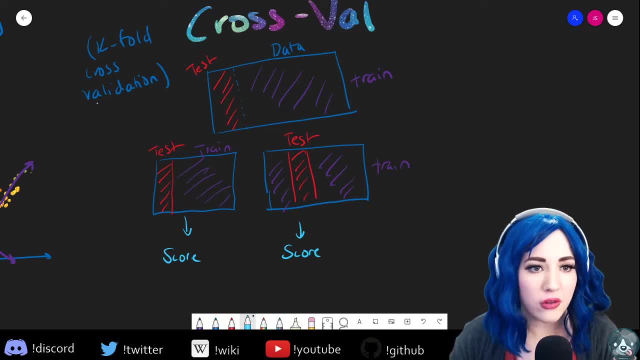 and so k-fold, you can do a five-fold, you can do a 20-fold, whatever you want. the thing is is that they've done a lot of studies on this and for most situations five or ten-fold cross-validation is best. the math's kind of cool. they've tried to explain it. i'm not entirely sold. 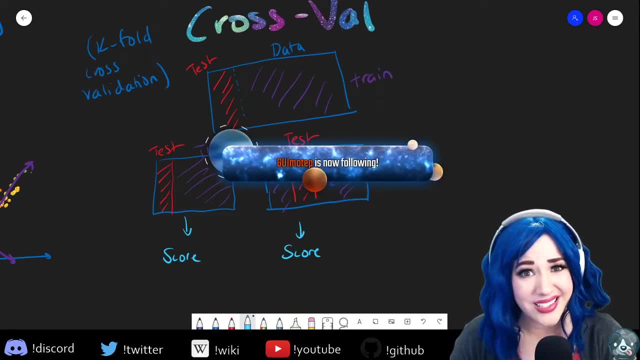 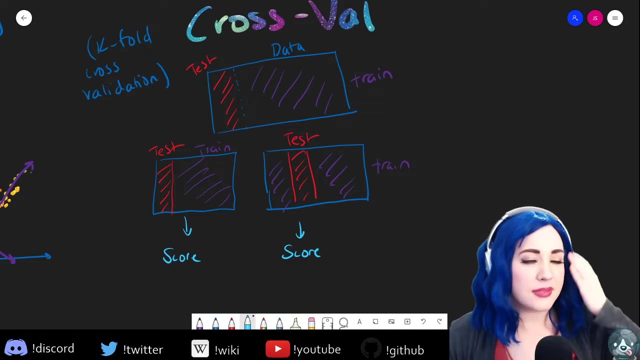 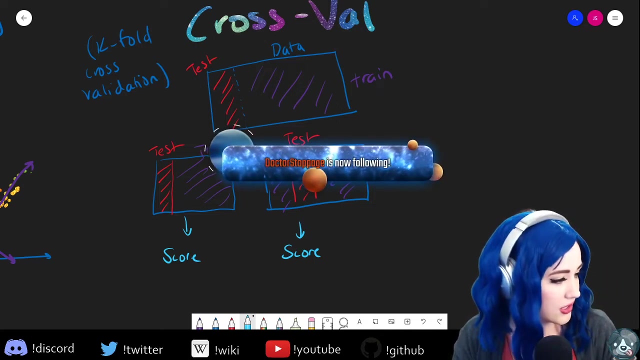 but that's, that's what has worked. so consider five or ten-fold, um, and let's see gooey motep. thank you so much for following. welcome to science. sundays: um, and yes, k-fold cross-validation is, is is much better now. i will caution all of you with something, which is that the and doctor stoppage. 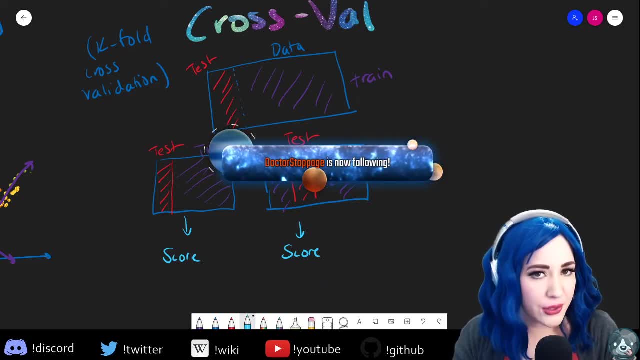 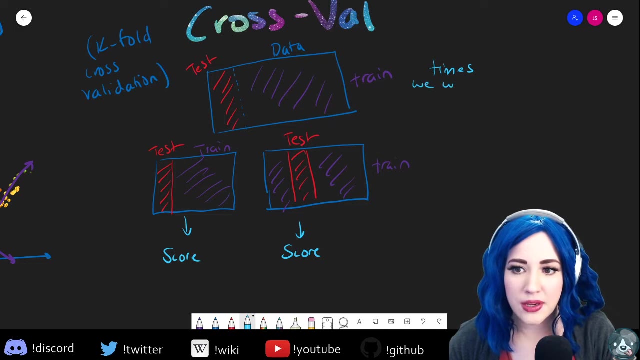 thank you for following, which is that we are using a singular metric here, even when we're doing k-fold cross-validation. we are measuring accuracy right, which is like how many times we got it right. so you can think about that like you know the times we were correct over all times. 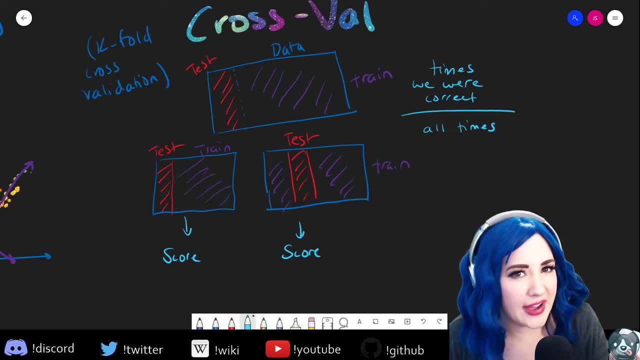 right, but when it comes to classifiers, that's not quite the best way to evaluate our performance. so if you're interested in this topic, i did a deep dive into it. um videos again on youtube. which stream was it? if you look in the descriptions of the videos, there's one where i talk about. 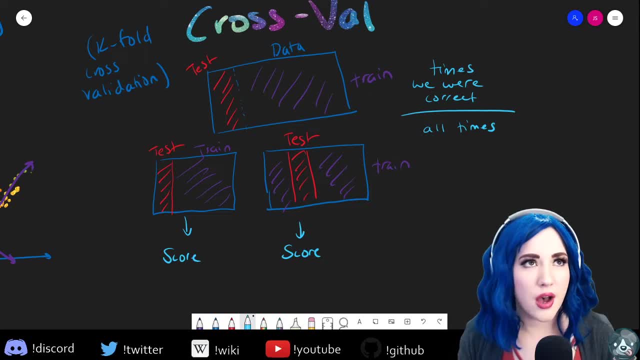 accuracy, precision, recall um, confusion, matrices, and these are ways that we can evaluate our classifiers more robustly. because the interesting thing about classification is that you might not be interested in accuracy, you might care about one class more than the other, and you might not care about one class more than the other. you might care about minimizing it, minimizing the um. 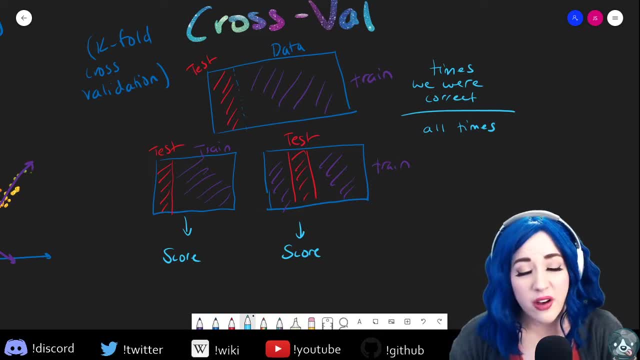 false negatives or minimizing the false positives. there might be one particular kind of error that you're really interested in minimizing. we talked about the example, for for example, of of using a classifier to detect cancer in a cancer example. a false negative, so where somebody has cancer. but 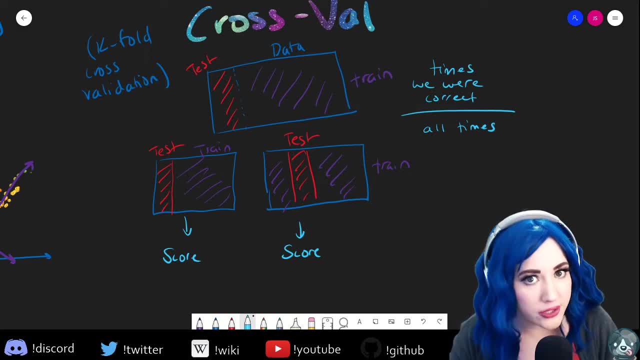 our model predicts they don't is far worse than a false negative. so where somebody has cancer but we say they do like, better to accidentally tell them they have cancer than to tell them they're fine when they do. so if you're interested in learning more about that, please check out it's. 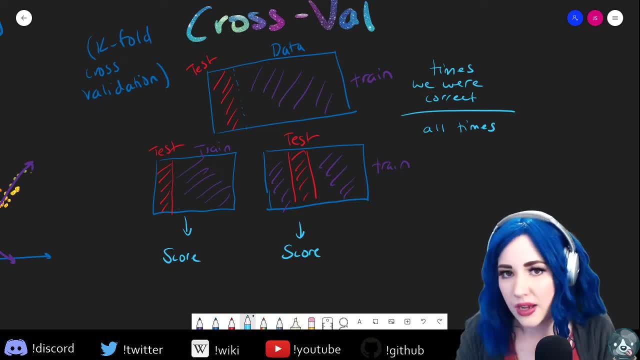 one of the machine learning myths videos. um, we talk all about classifier metrics and i talk about, you know um accuracy, precision, recall, false negatives rate, false positive rate, etc. etc. um so good stuff, but in any case, hopefully you have a bit more of an intuitive sense of cross-validation. 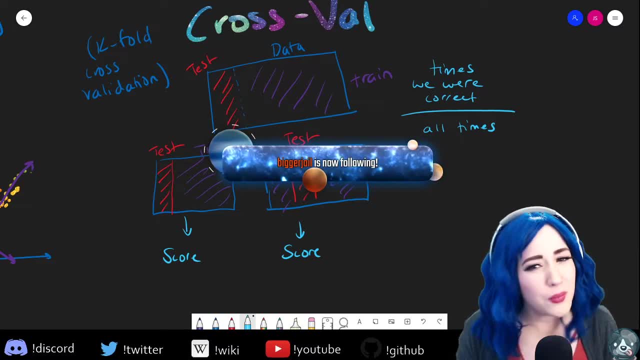 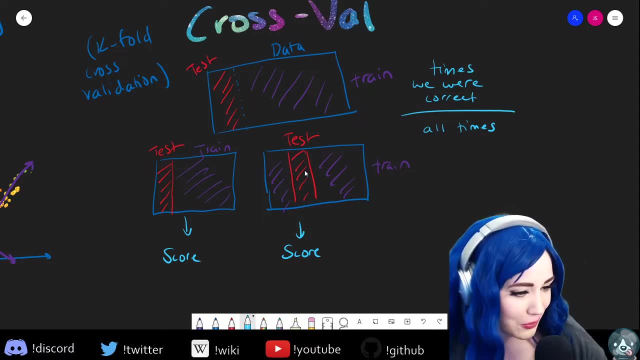 so we're just going to be repeating our test train split, but we're going to be grabbing different portions of our data each time and bigger jail. thank you for following. let me catch up on chat, because i just rambled for quite a bit um important stuff. i'm teaching good, yes. 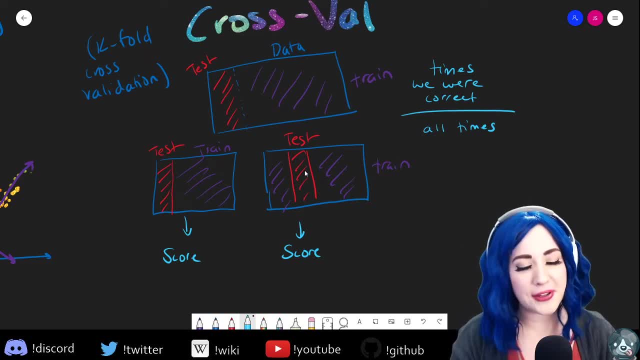 cross-validation is important, but also this is: this is what we were talking about earlier. someone asked me- and i apologize, i don't remember who- asked me: like is a machine learning engine a software engineer? just basically a software engineer that can deploy a machine learning model? and i said no because, like as a machine learning developer myself, like: yes, i can write software. 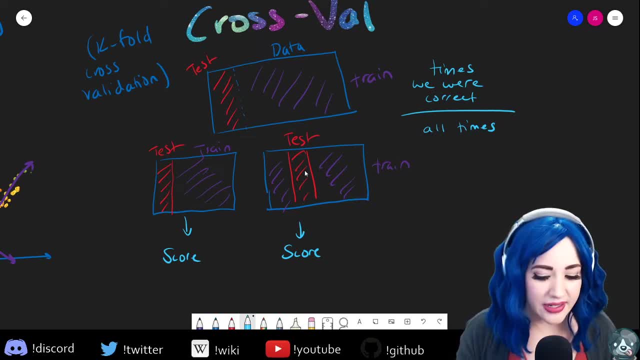 but really my strength is in that i can. i know how to build these models. i know the best choice of model. i know how to select the right parameters for a model to make it perform the best that it can. i know how to evaluate a model. i know when something's going wrong, how to kind of diagnose. 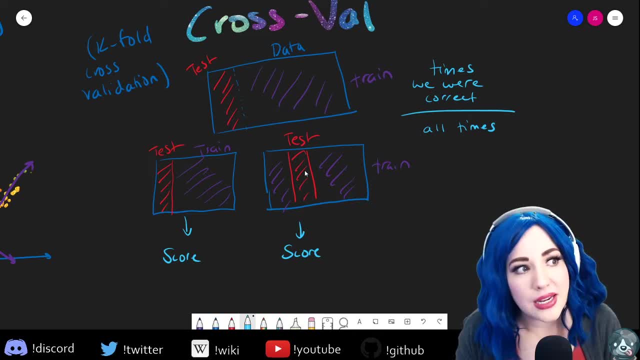 what the problem is. i know how to evaluate a model. i know how to evaluate a model. i know how to evaluate it. but also i can't tell you how many times i see lots of you know great, wonderful software devs just kind of build a machine learning model. they don't really understand it. 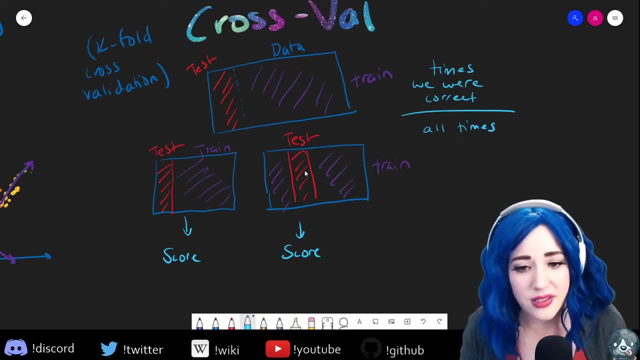 they're trying their best, like this isn't a criticism, but like they're trying their best, they build a model. they don't really understand it. they don't know how to evaluate it. maybe they have a classifier and all they look at is accuracy, singular accuracy, no cross-validation, nothing. 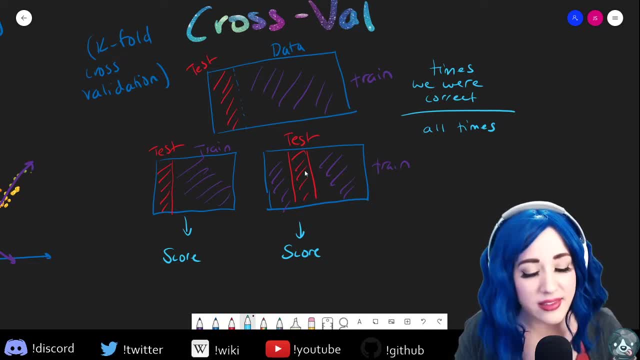 well, if you don't study this stuff and you study the math and the statistics behind it, you're not going to be able to build a good machine learning model. and just like how good of a programmer you are, you're not going to be able to build good machine learning models. so it's more than just 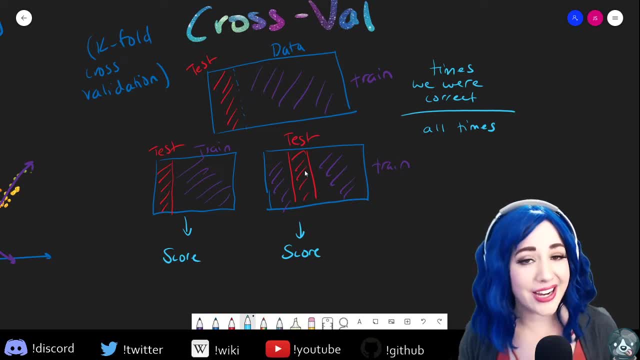 being able to build good software. for me- and lots of people come to it differently, but for me i actually started with theoretical math, so that's my strongest suit is the math um, and then, of course, like the different model types and everything like the statistics, and then i learned. 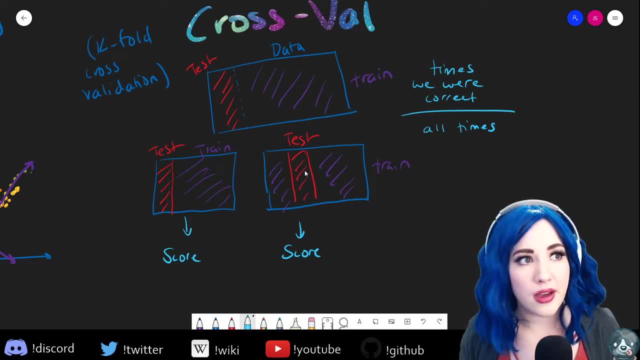 programming, like i was okay at programming, but it wasn't until i really um, i got a promotion at work and started to lead more projects that i realized that my biggest gaps were in software development and that's when i started focusing for the last few years on really improving those skills. 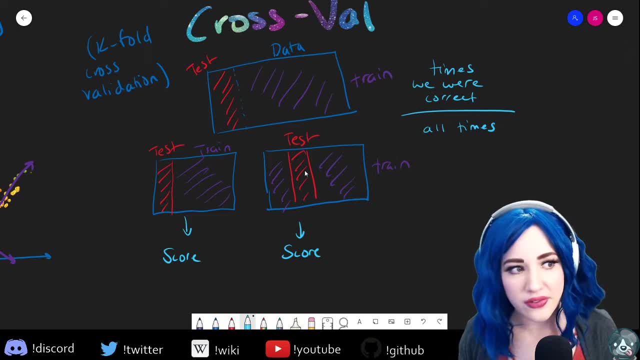 so giving myself a cs background, giving myself software development, software engineering skills, and i'm still working on it. but machine learning developers are. i'm straddling two, two fields, well more than two fields here, because it's not just math, it's not just programming, it's not just 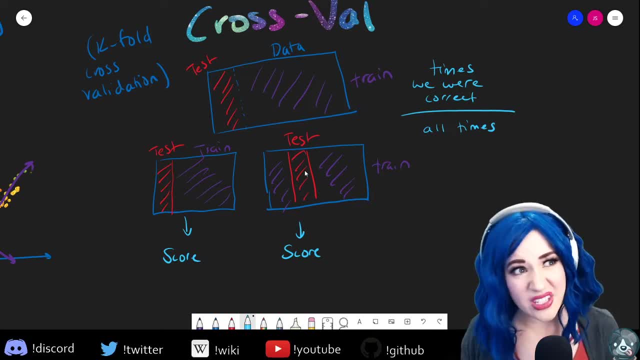 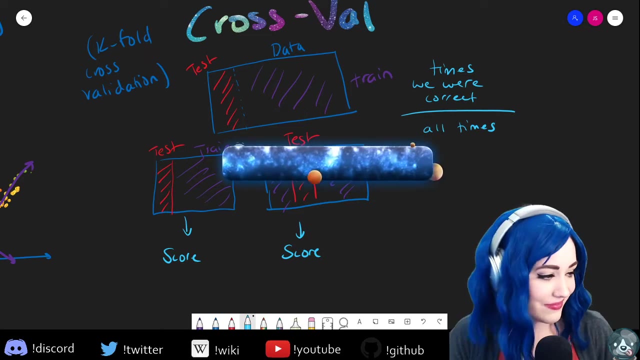 statistics, it's not just data science, it's all of this smushed together with a whole dose of added problems. so, um, and i have not opened up the mic yet- oh, trust me, i have such such a little free time now. um, i keep, i keep saying yes to things, so i have very little free time. 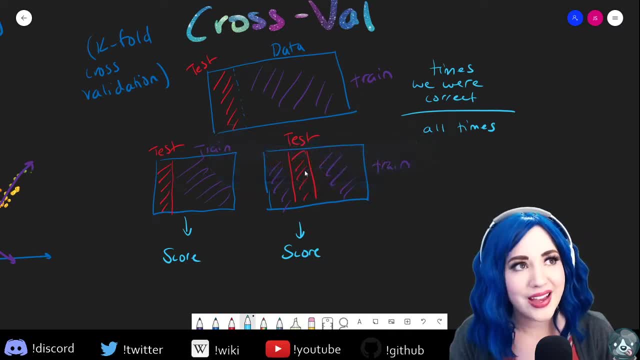 and i got my. i got my covid vaccine, so i also i'm going to start to need to go back to the fire department as well. so my, my, my free time to do fun stuff is like zero. it's actually the negatives. but uh, joe, let's see. joe vega and path of inspiration. thank you for following and um you. 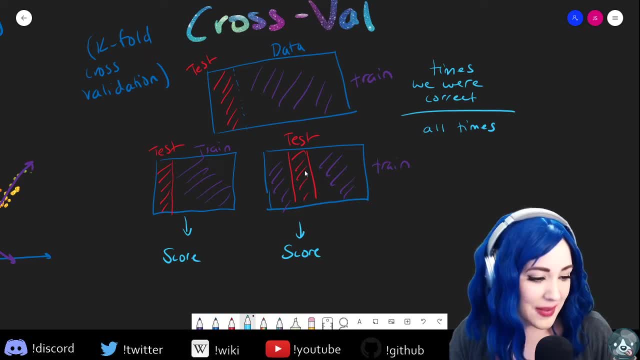 might or might not have cancer. yes, exactly, um, and kevin, you're absolutely right. you say, on top of that, your model could work completely differently in real world situations. you understand the struggle, thank you, yes, i do understand the struggle. i also understand the struggle of like. 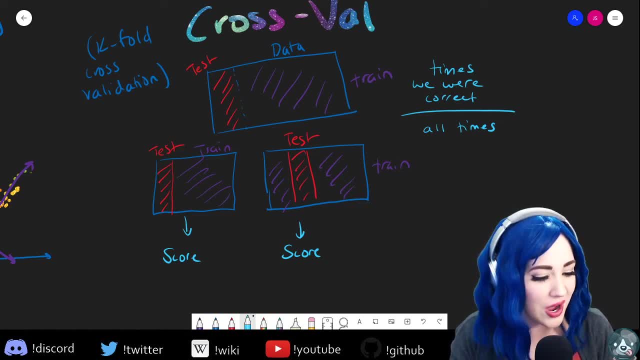 all right, i'm gonna. i'm gonna like we have a soapbox command for this, because i do this too often. it's a new command, but i will be honest and and i'm gonna get on my soapbox for a second. i have been called in so many times to clean up after people. 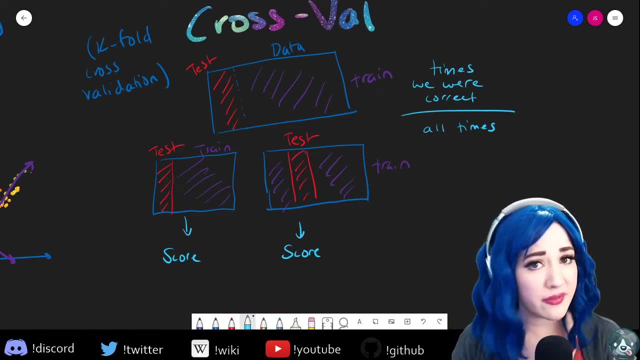 who one. all well-meaning is not a criticism of the people, our software developers, who are implementing models. they don't understand and the models aren't working and they don't know how to fix it- machine learning people who are just very junior. but the broader reality of it is that our government is gonna work with everyrees and 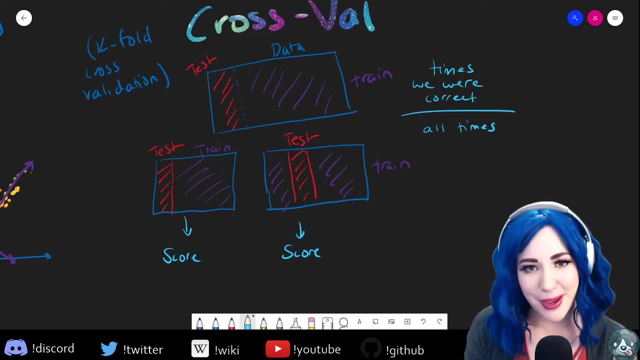 everygr находing and Source five, and so they're affected by, like the shiny allure of deep learning which i feel i get you. you read the latest paper that does something really amazing and unfortunately, academic papers are like two-third science, one-third propaganda, and you get, you get. 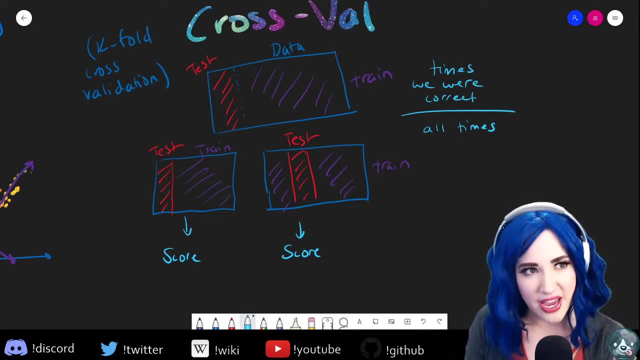 sucked in by the propaganda and you think this is gonna like cure all the problems. so suddenly you want to like it's kind of like a version of is a deep learning situation, and so suddenly you're applying models like this one specific model to everything, when it doesn't fit um, or situations where the person's so obsessed with 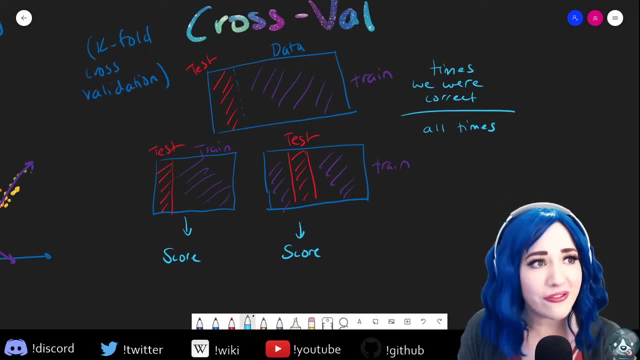 the machine learning, that they don't look at the data, they don't clean their data, they don't do feature engineering. they're not. they're skipping out on their eda, which i get it, i can't. i like some eda but like i get you the model's, the fun part, but like don't do this if you're not willing. 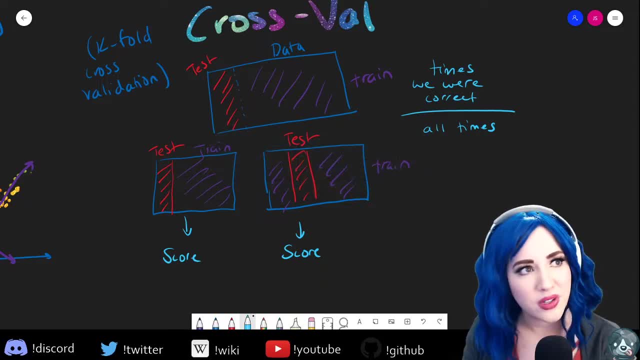 to clean up the like. every job has the cleaning of poop, like the poop differs from job to job. but like everybody's got that kind of aspect to their job and you, you're not doing your due diligence if you skip it, if you, if you skip out on your eda, if you're not cleaning not feature engineering not. 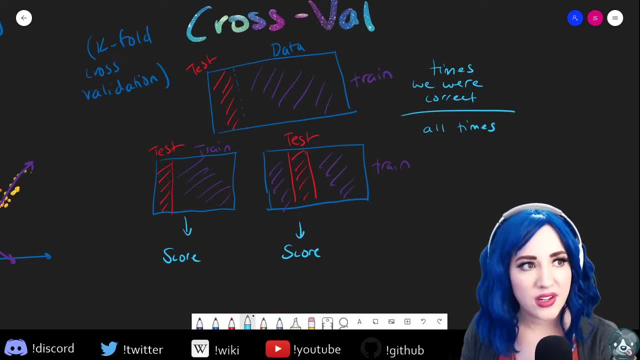 you know deeply understanding relationships in your data, no matter how great your model is like. i try to not swear on educational streams, but there's, there is a principle here which is: shit in, shit out. no matter how great your model is, you're not doing your due diligence if you skip it, if you're not cleaning. 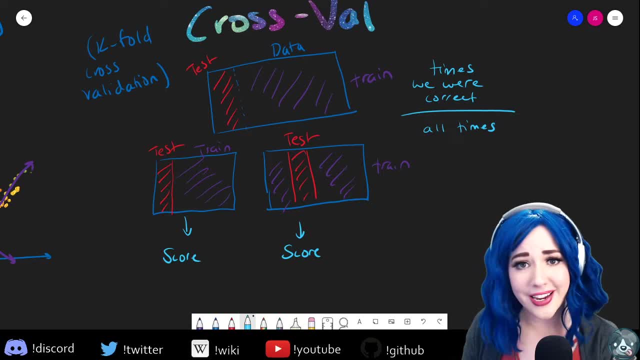 your model is: if you feed it poor quality data, you're going to get bad results, and so those three situations are frustrating for me, because you know it's one thing, if you're inexperienced, I get it, but like I object deeply to this idea of a black box. I understand that, like we don't always need 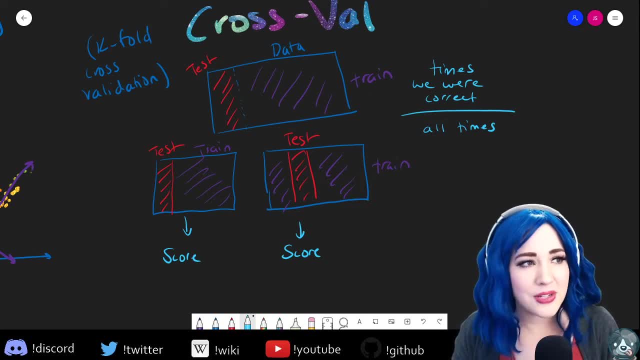 to write out all the math by hand or anything. that's not what I'm talking about. I'm talking about this approach of just neural nets, and deep learning is a black box, so I'm just going to slap it on stuff don't like it's. like don't drink where's. don't drink and drive, bro, but like don't. 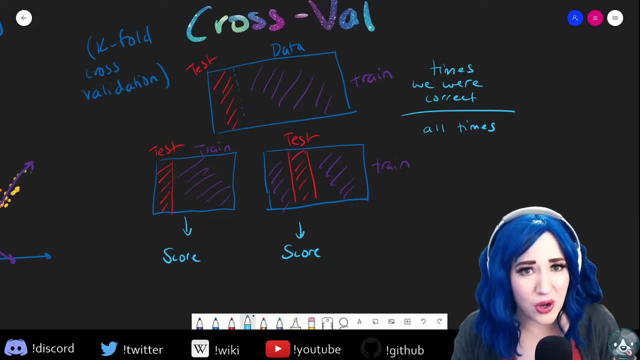 it's like a version of don't drink and drive, like don't build machine learning models, with no understanding. now my streams are here to help you all build this stuff. I'm not talking about all of you like, go build it all on your own, you know. yes, build bad models, build good bottles, make. 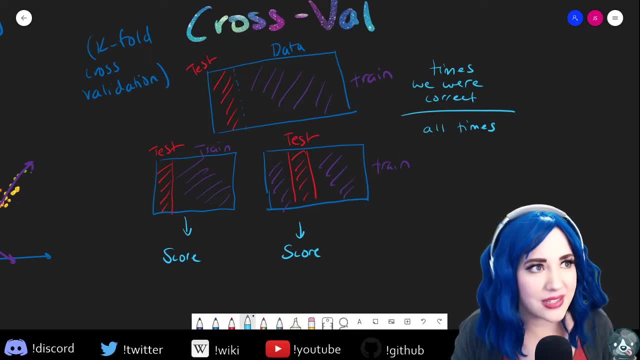 mistakes. that's how you learn. I'm talking about the people who do this for a job, sell it to companies that then use it to make decisions. I'm not talking about learning you, but like it's frustrating because I don't know. I guess that's why this is a soapbox, is that? 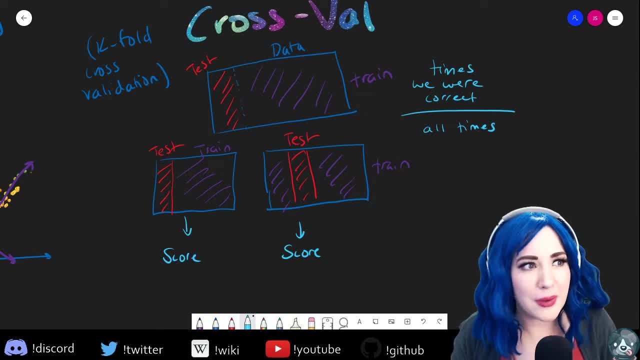 I feel frustrated because for me especially, am I, do I exist? okay, the mic glitched for a sec but, like, especially for me, I I struggle with a lot like imposter syndrome and stuff, like feeling like I know what I know and so I just I don't know how people get so confident to build things they don't understand. 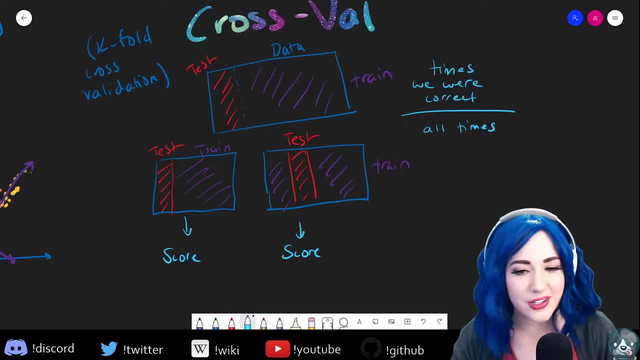 to tell people to make decisions based on things they don't understand. don't do that, friends like. learn along with me. build your machine learning models. break them, but understand them. take the time, do your due diligence seriously. I promise it's worth it. it's worth the struggle, it's worth. 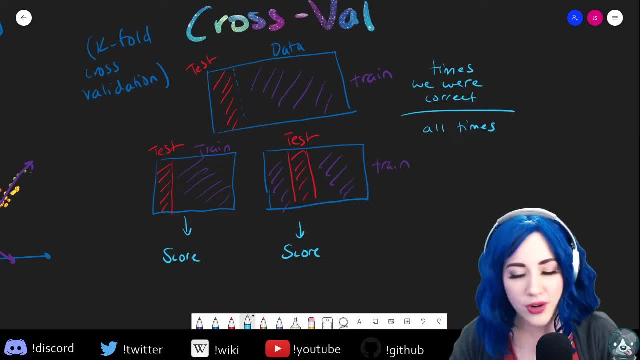 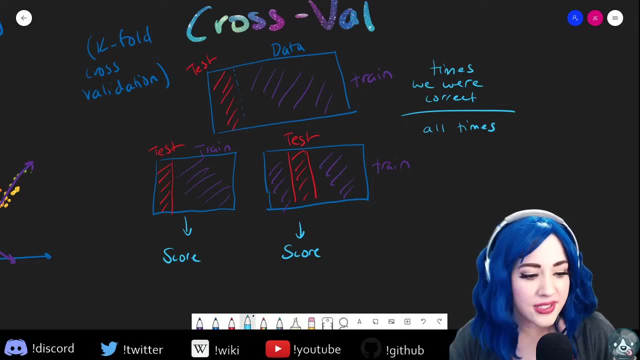 I promise. yes, ignorance is bliss, Kevin, but like there's often consequences to it and learning might be uncomfortable but it's worth it, like last bit of my soapbox, and then I promise we'll get back to this. but one of the things I learned about in philosophy is that Socrates slash Plato, because Plato wrote about Socrates, but still. 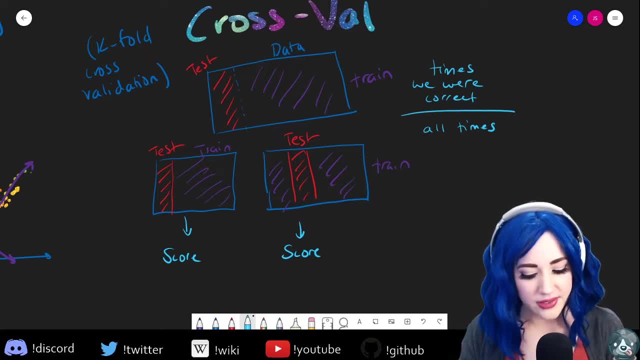 has this great idea, this, this kind of concept- and I'm not gonna use Greek words for it, I'll just describe it in English- but like essentially of like a paralysis that people experience when they don't know something, when they think they know something and they they're shown to be wrong, and 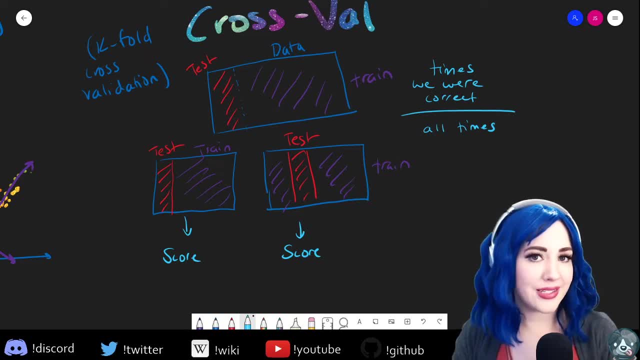 one of the things that he noted is that most people can't push past that, they give up. so when they experience that paralysis, that painful moment of like I don't know this or I thought I knew this and I don't, don't push past it. to learn and to, to grow and to find out what, what the answer really is. 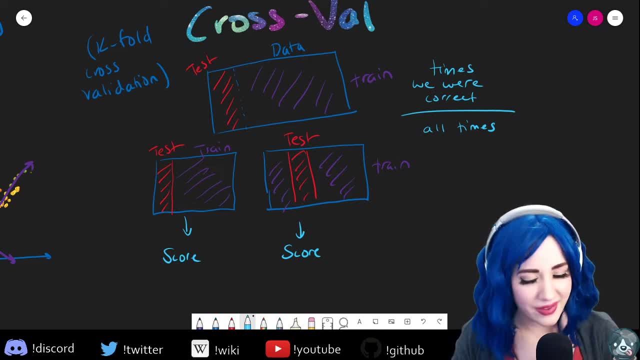 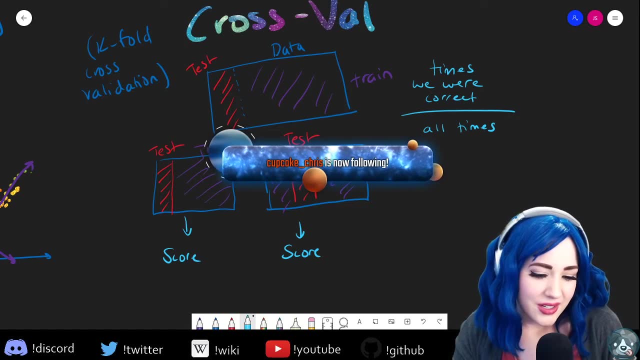 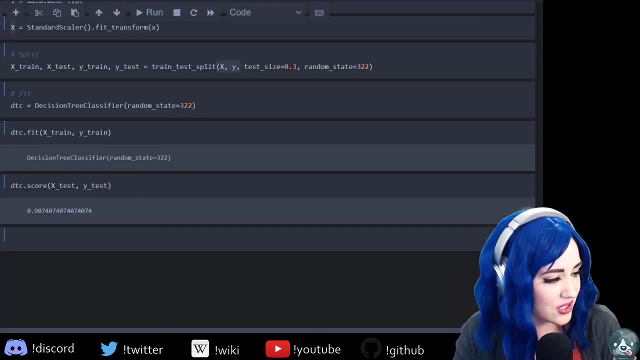 um, don't, don't be like that. be better than that, like I promise, like I can make it fun, we can do streams about it, but but also just just don't build models. you don't understand it. some of me is just salty, because most of the people doing this make a lot more money than I do and are lauded for. 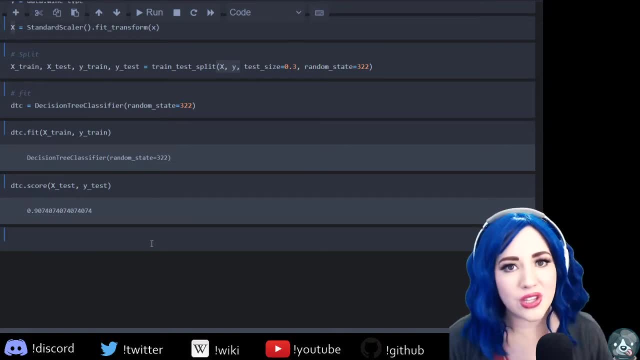 learning knowledge that they don't, but really it comes down to the damage that you do. machine learning more and more is becoming used by companies to make decisions, and those decisions have impact, often on real people, like there's a reason that AI ethics is a huge and important. 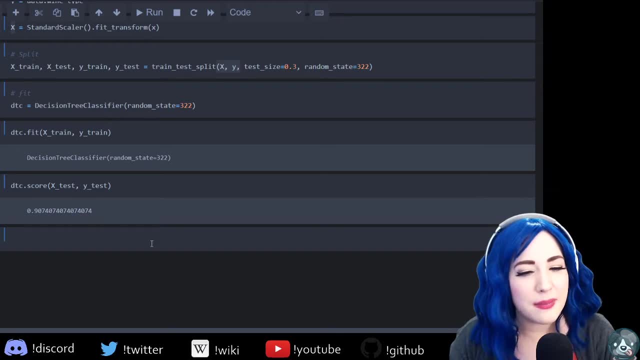 field. like it's okay to be a beginner and to not understand and to break things and to make bad models and to like make mistakes, but like keep, keep a hold of your humility. maybe it's okay to use the better way to say it. it's like: keep a hold of the humility to to know the difference between. 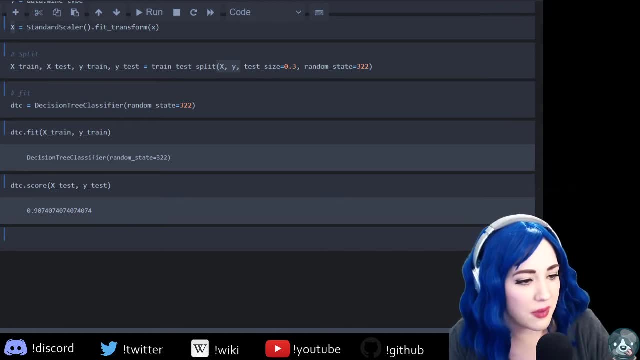 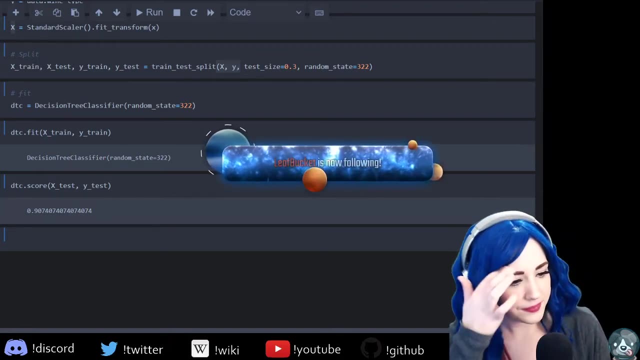 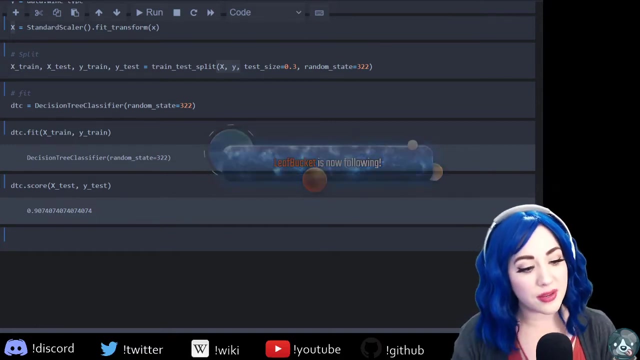 like to know the limits of your own knowledge. all right, I'll get off my soapbox. let's go um and let's see. I'm catching up on checks. of course, I had to ramble for forever. um, and let's see and eat, or, Faust you say? implementing something well is one thing, knowing what you should. 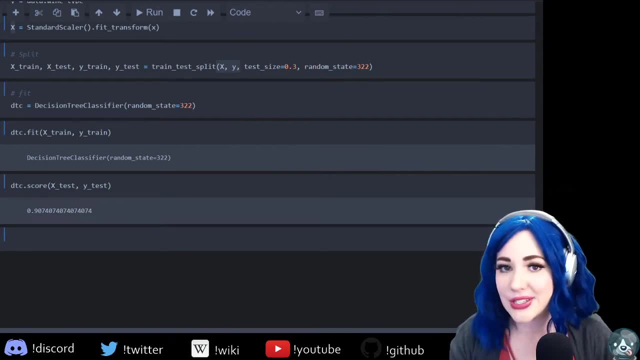 implement. that's a different thing exactly. and, Luke, I'm a volunteer, so I volunteer with my local fire department, um, but because of covid I have some high-risk family members so I had to pause. but now that I have my vaccine I can. I can go back to it and let's see that. North boy cupcake, Chris leaf. 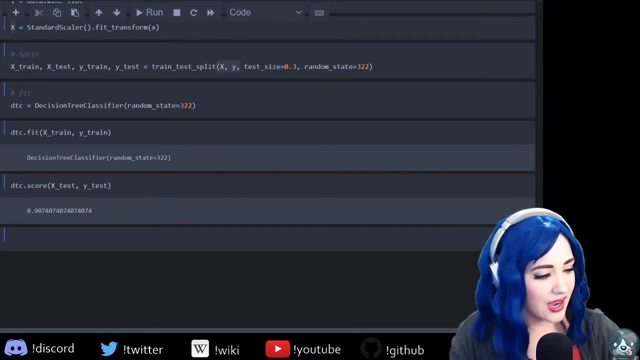 bucket and squanto yikes. uh, thank you so much for following. um, okay, hi, Whiskery Ant, it's good to see you. I'm green. Jenny, hi, it's good to see some some old friends coming into chat and it's perhaps thank you for following. I know I'm sorry, a hacker. you leave for a few minutes and I get on my. 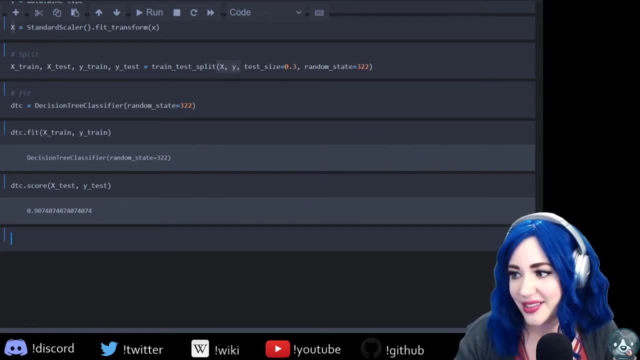 soapbox. I just I feel very strongly about a lot of this, like I see so much bad ml and like companies making decisions based on bad ml or unethical ml and it just makes them want to throw chairs. um hi, Enigma dev, no, you should not stop your pixel art. it's different. it's like like: for me, I love power. 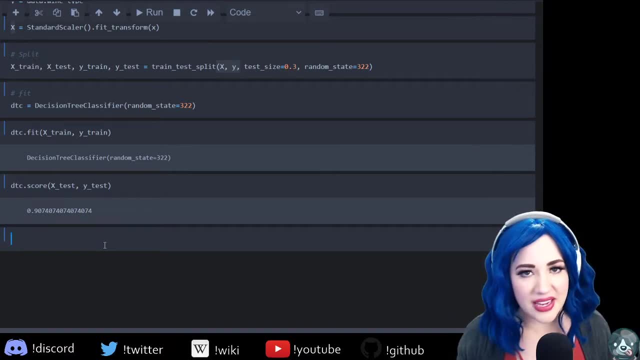 right, I haven't done it in a while because you know pandemic and everything, and I'm gonna build a home gym, I swear, but it's costly, um, but like I know my limits, I'm not gonna sit here as a beginner, as somebody who like is not great and like try to put myself into the Olympics, so it's one thing. 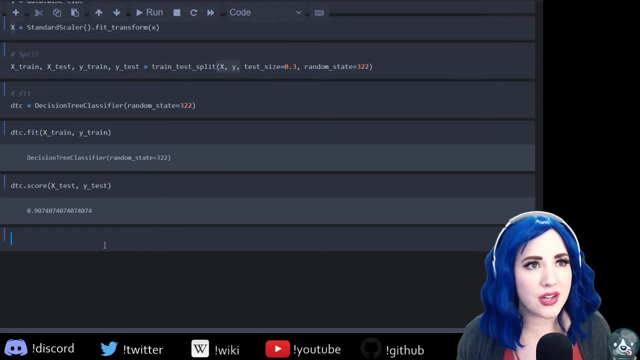 when you're learning, when you're practicing, when you're refining the things that you do. it's another thing to like go in, having, just like having not as much understanding as you should and telling people how to do things. um proto man and smiling Buddha. thank you so much for following. oh, you just okay. so augmented mode. 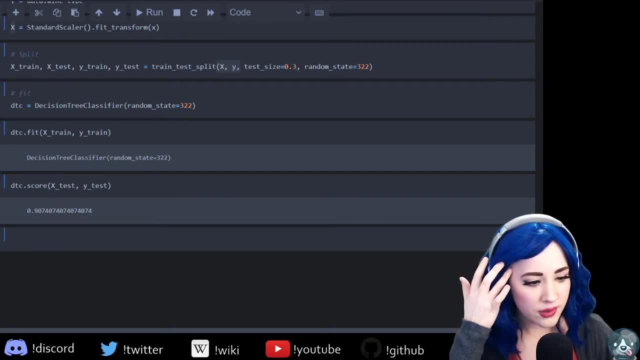 isn't? is that um Timnit gebru's paper? I've had that up on my computer for ages. um, but also machine learning models should not make critical decisions by themselves. I am a massive, massive fan of something called human in the loop, which means that you take your, you take your machine learning. 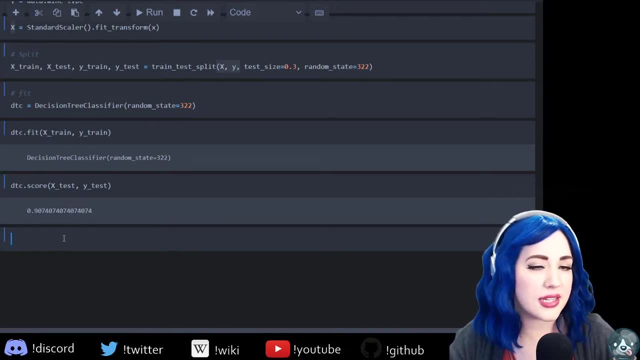 model and it is a tool that a human being uses to make a decision. it does not make its decisions independently like. it's one thing if you're using it to like sort stuff or like it. the problem arises when you start to use that model to make. 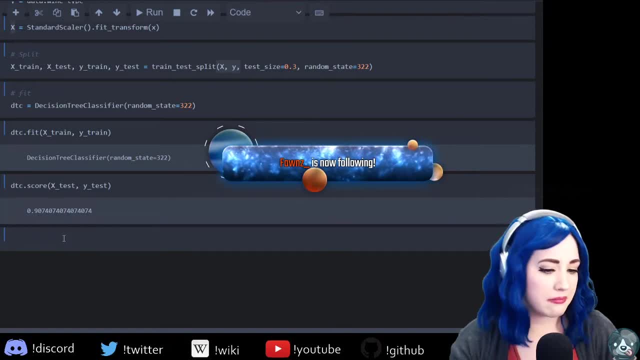 decisions that have really critical impacts. so, like I'm very anti-autonomous weapons, I'm also anti like automated targeting and things like that. um, but also I'm anti like machine learning models just being left to make a bunch of decisions on their own. like I, it's also. 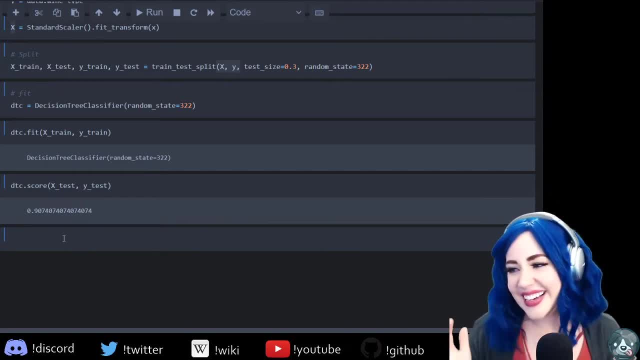 proven. I got science to back me, you know it. it's proven that the performance of human in the loop, so a human working together kind of with and providing feedback to um a machine learning model, is much, much greater than a human on its own or a machine learning model on its own. so, um, Fonz, thank. 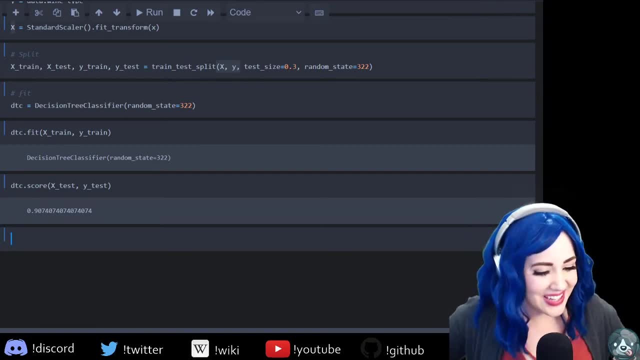 you for following. welcome welcome to stream and thank you, Katya zeros. I'm so glad you're so glad you're here and Kevin, oh, you had a seminar. I'm so jealous. I really just she's gotten. she's had a really hard time lately, um, and 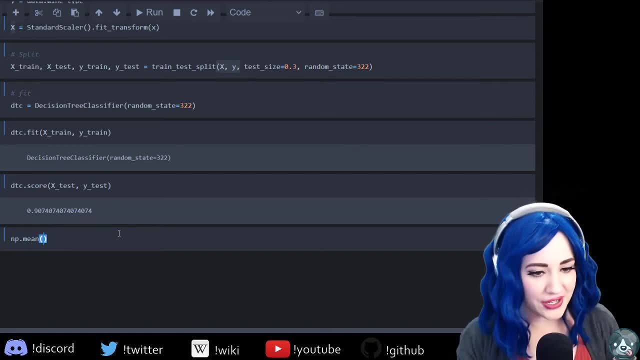 been treated very unfairly and largely due to her gender and the color of her skin. but I look up to her so much like she's. she's absolutely brilliant and she's like actually speaking truth to literal power. lots of people use that and they're not actually. 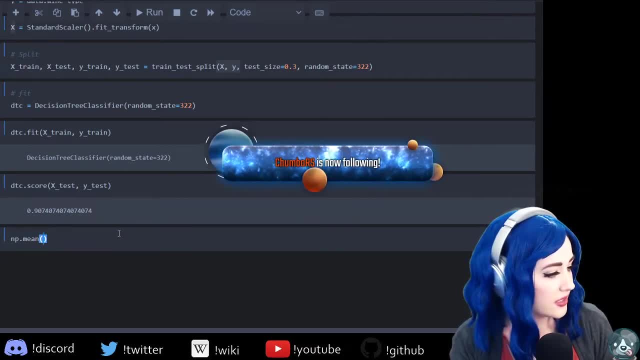 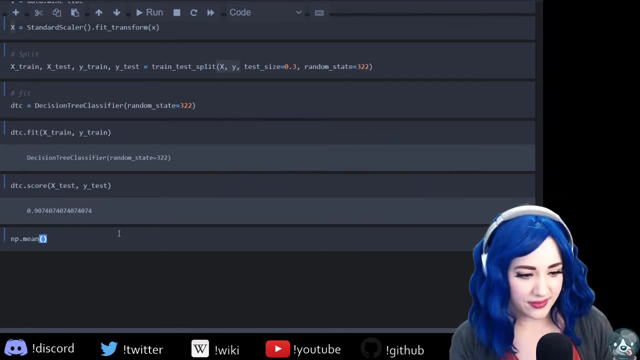 doing it like- use that phrase, but she is, and she's incredible. um chumbo RS. thank you for following. um, she's so intelligent, also a hacker like I know the limits of machine learning. machine learning is nowhere near robust enough yet to be making the kind of decisions that 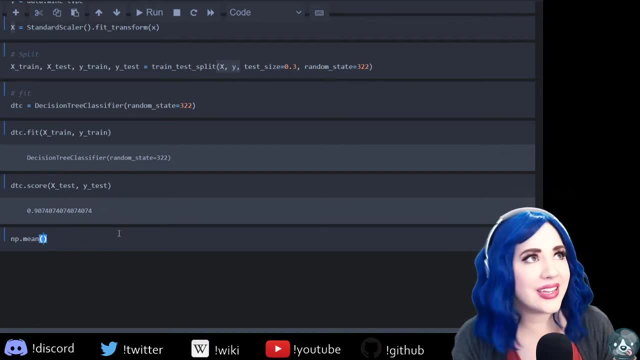 people want it to make. we're learning, but we're in the infancy of AI, like we've been doing it for some decades, but like it's nowhere near stable and reliable enough to be using it to make decisions. um, it's just not, especially not decisions involving targeting and weapons. 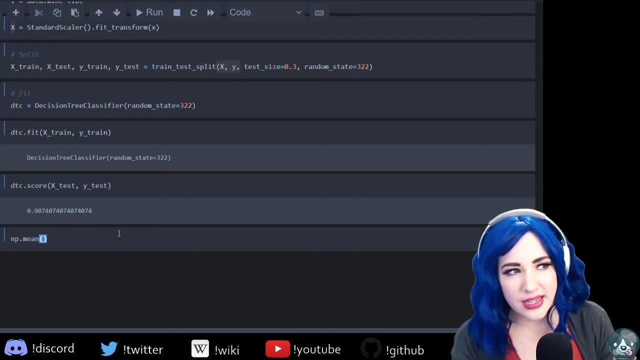 but even beyond that, I could go into ethics for for hours. but um, yeah, the problem is so many like greed, right, people want to make money. they're gonna make a lot of money telling people their models can do things they can't. and you know what? 90 percent of 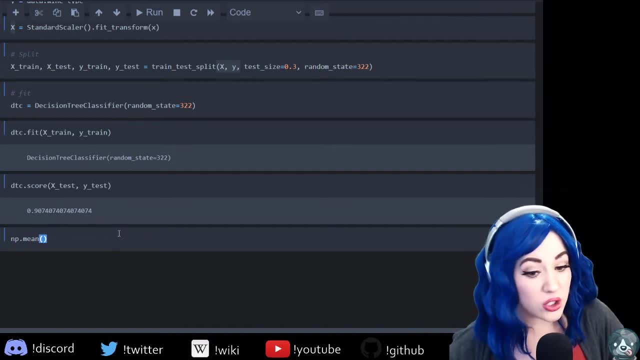 my job is actually coming in after somebody has sold a client or a customer on a machine learning, promising them the earth, moon and stars, and it's not working or it's doing bad things, and I have to come in and clean up their mess. so I'm also a little salty because that's a large portion of my 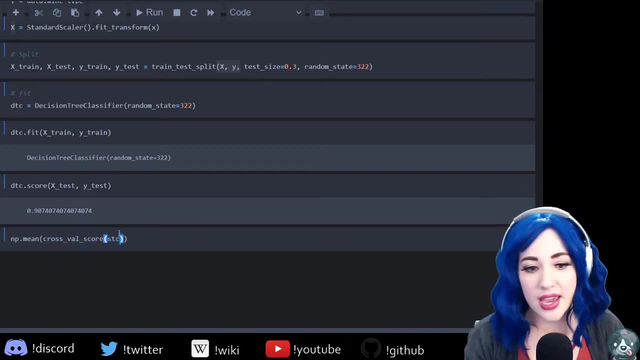 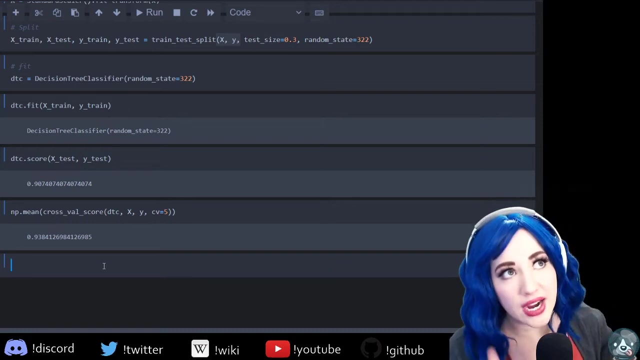 my work is coming in and having to be the bad guy and saying: I'm sorry, they told you this could do this and it's not. it's not no, just no and um, okay, so well, actually one tiny, tiny thing, and then we'll get back to this. one of the problems there is that I- I've gotten this feedback in my career of like. 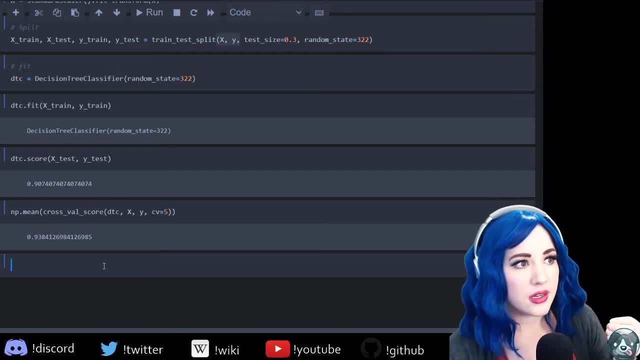 people thinking I know less than I do because I have to be the one to say no, it can't do that. it's not me saying no, I don't know how to do that. I'm saying literally: this model that somebody else sold you on is not doing the thing that you you know. I'm sorry, but it's not going to do what you. 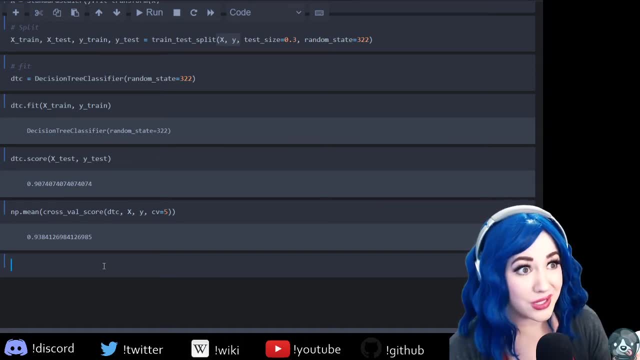 think it's going to do. that's not because I don't understand it. I'm telling you literally, like you got bamboozled, I'm sorry. um, also, neural nets aren't the solution to everything, don't it? there's so much overkill with neural nets. they're beautiful, they're awesome. don't get me wrong. I love losing myself in some. 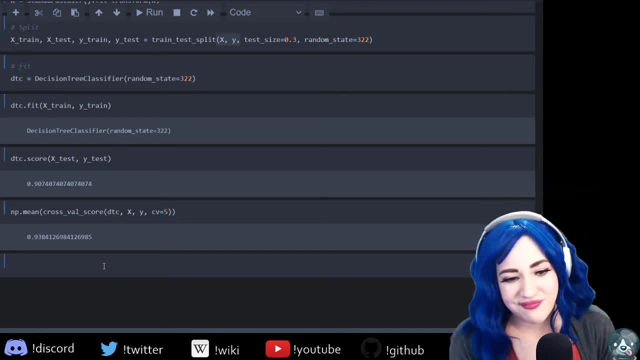 cool, like neural net architecture, but there are times when just a very simple model will do so. oof, um. and Fonz, you say, for things like machine learning, do you think I should major in computer science or computer engineering? right now you're in mechanical engineering. um. 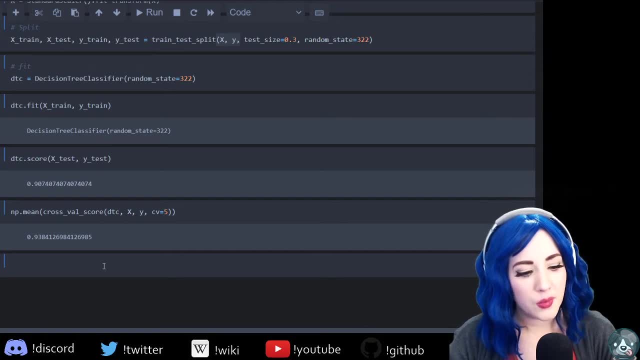 so for machine learning, well, I might suggest computer science. if you're able to minor, or at a double major, I would suggest math. um, because the problem comp sci, like I think you do some math, but like real machine learning, you're going to need, you're going to need some good applied math. 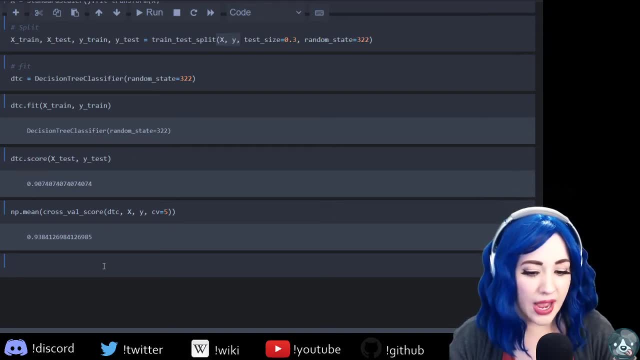 so, um, I might, I might recommend seeing if you can incorporate more math. like, if you have a computer science major, you're going to need some good applied math. if you have electives or something, that's fine, but also if you're able to like double major or 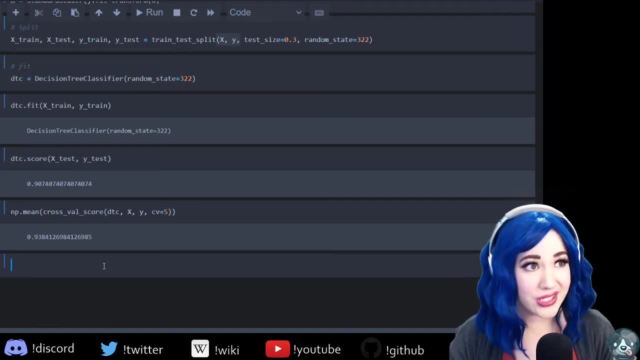 major, minor. you need statistics and not just like frequentist- you know there's 10 marbles in a bag- kind of statistics, but also like Bayesian statistics. you need more advanced statistics. you also need calculus. I'm sorry you do. I love calculus. calculus is beautiful. we'll get there. 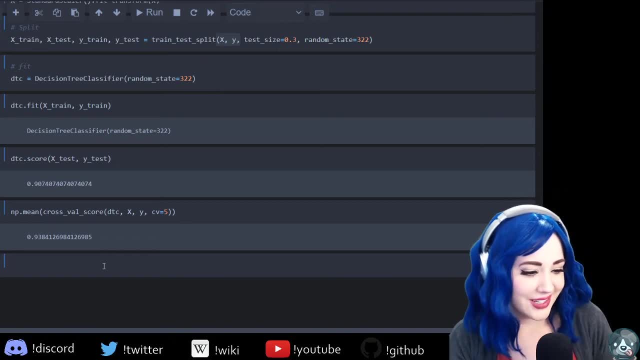 on math mondays, but you do so. and double minor philosophy- great Jenny word. double minor in ethics, um, I studied philosophy and it's come immensely in handy. this is like possible like hot take unpopular opinion moment. philosophy taught me more than math, physics, any science. philosophy is what taught me how to think like a scientist, how. 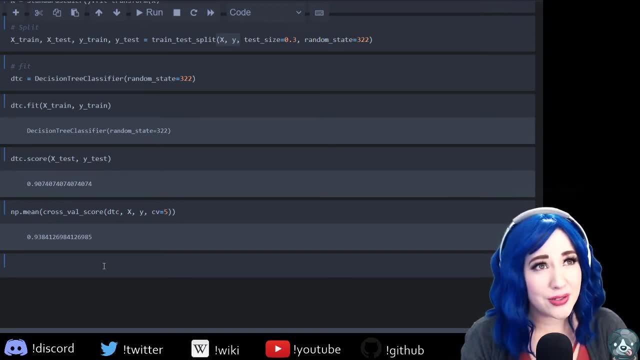 to rationalize how to evaluate arguments, how to like- even sometimes like- design software, like to be able to take something complex and distill it into its premises and its conclusion and evaluate it. hmm, I love philosophy. all right, let's see. and you know, pasta cheesecake that's. 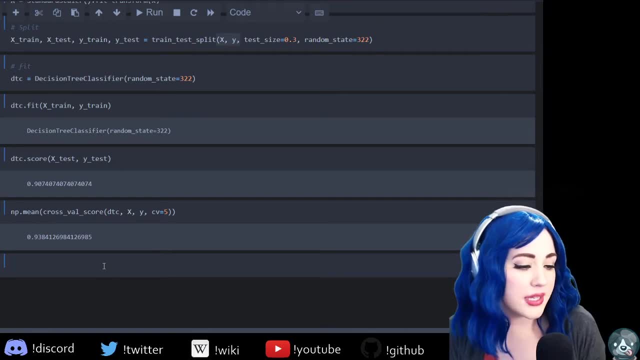 a really good point. you say what? what you were saying before. it's just one example of a much bigger trend. most programmers don't really understand how a computer works, etc. at this point it is so complex that no one can fully understand everything. yes, I would say, like not all developers. 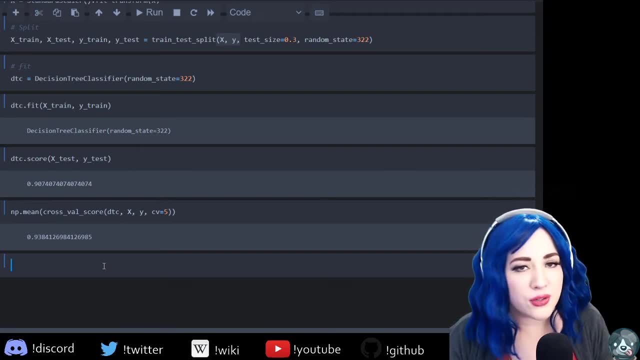 need to understand, like you know, how, how things are, how a CPU works. I mean, I watched a bunch of videos on it because I thought it was cool, but you don't need to necessarily understand that. that said, if you are starting to make recommendations to people based on things that have like a result, 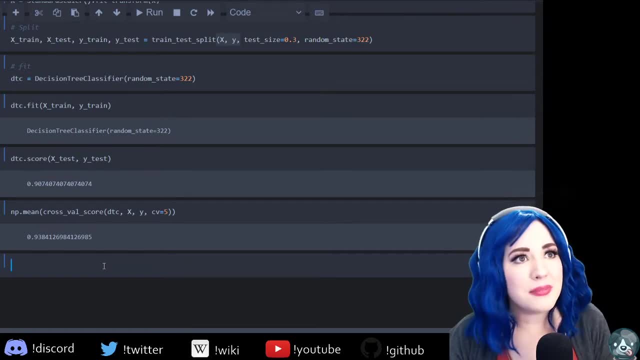 that's when you stop. not all like a web dev I don't think needs to deeply understand. like the history of computing and like how things are, are like how how a CPU like does. it's like different processes and stuff, but so it's also about knowing your limits. but like, for example, don't like as a 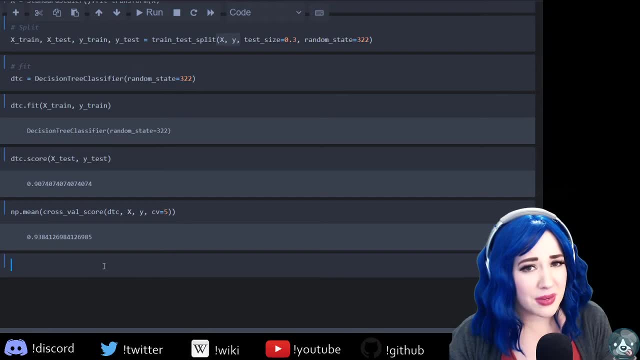 machine learning developer. don't try to say that you can build a model optimized for GPUs if you how a gpu works. so like, you've got your scope, like i also don't want to be gatekeeping and say, like you know, to, to, to. to even get a job in this, you have to know everything. that's not what i'm. 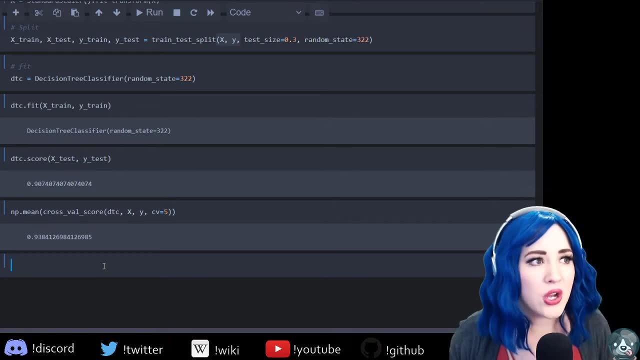 saying. i'm saying, by the time you get to a level of seniority in your career where you are like telling people what to do and advising them and saying this is the model we should do, this is the like, at that point you should have done your due diligence to really know what you're talking about. 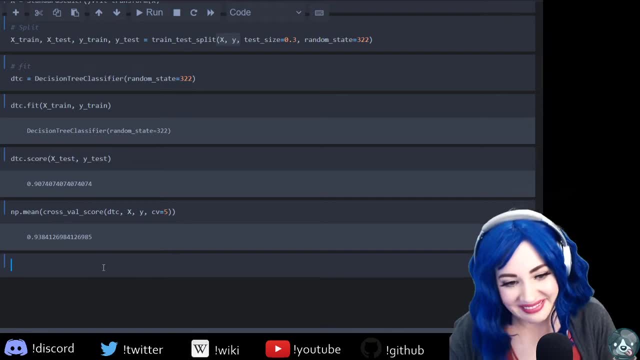 you might not feel like it, though if you're like me, you'll never. maybe never feel like you, you know as much as you do. but still, um, exactly, third tier, all right. so we did our cross validation score right: k-fold cross validation. i picked five folds and see we, we got a higher thing. sometimes you'll. 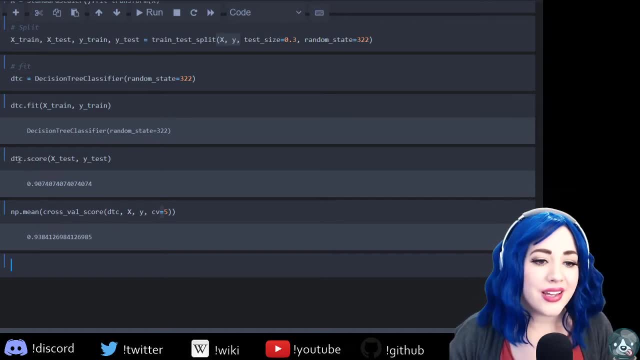 get a lower result. sometimes you'll get a higher one, but the point is that our original just one off uh test train split isn't enough. all right, cross validation is a great way to deeply evaluate how your model is doing and make sure that it's doing what you think it's doing. hi, triumphant base hi. 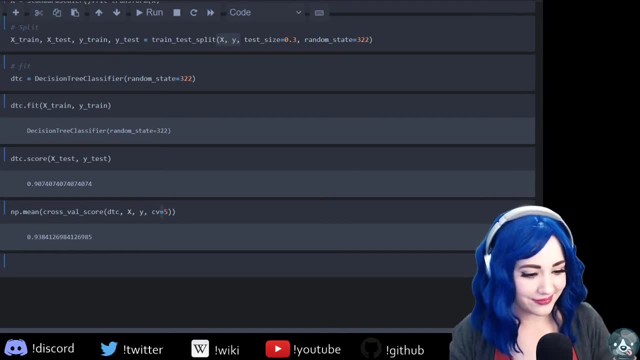 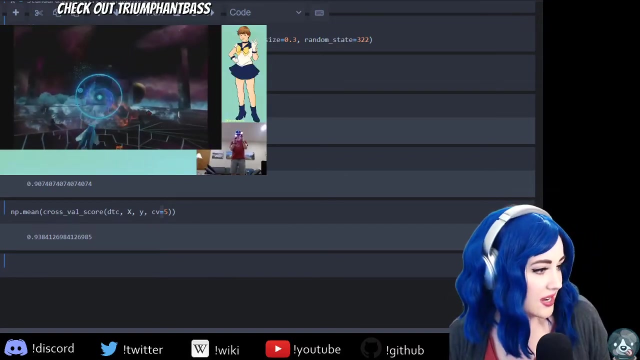 cassie. all right, let's, oh wait, hold on raid. yay, okay, you're in chat. all right, hi, welcome, welcome, raiders. let's give a shout out for triumphant face. okay, cassie's amazing. he does like cool video games streams. and, uh, like you said, you promised me some sewing streams, cosplay. 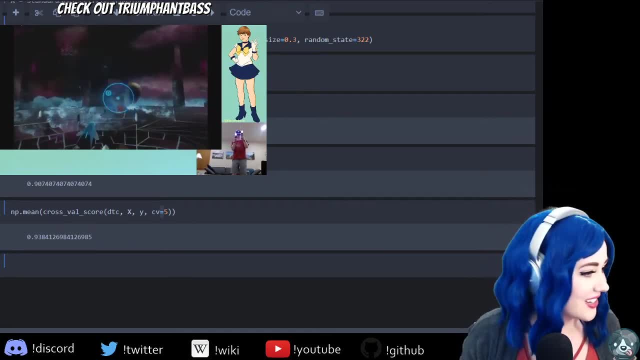 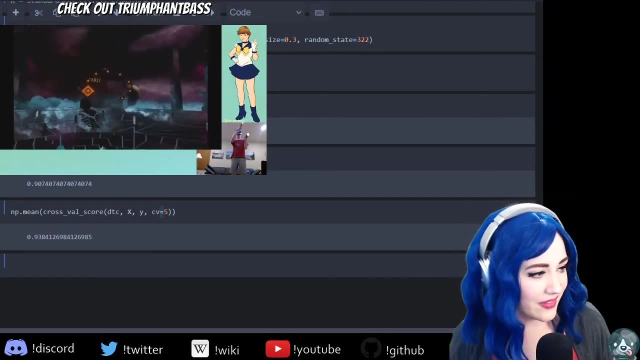 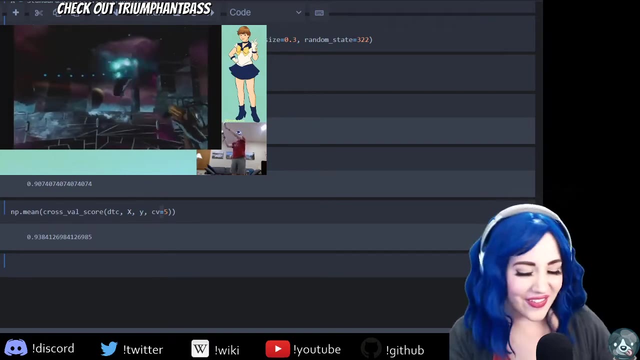 yes, yes, and that is. is that is a good soundtrack as well, if i am, if that soundtrack is from your video, which i think it is, isn't that from transistor so good? all right, in any case, give, give, give cassie a follow, all right, or is that autica? okay, but the the soundtrack is is 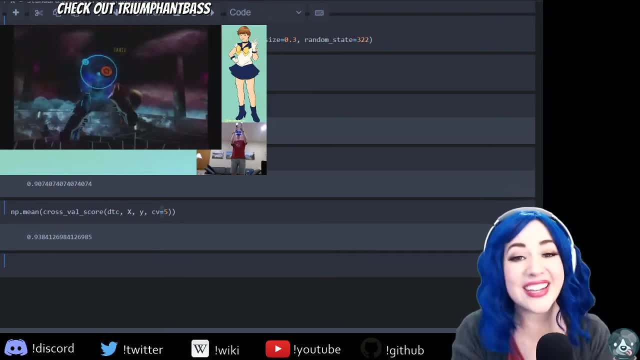 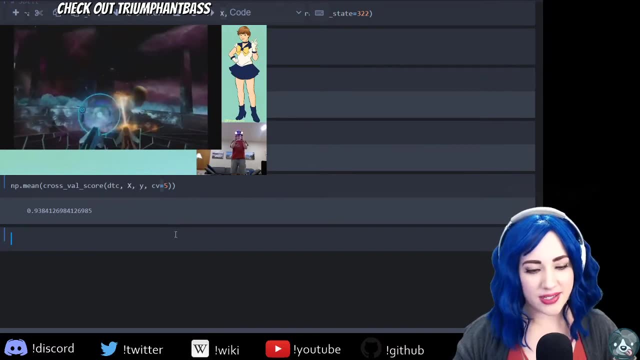 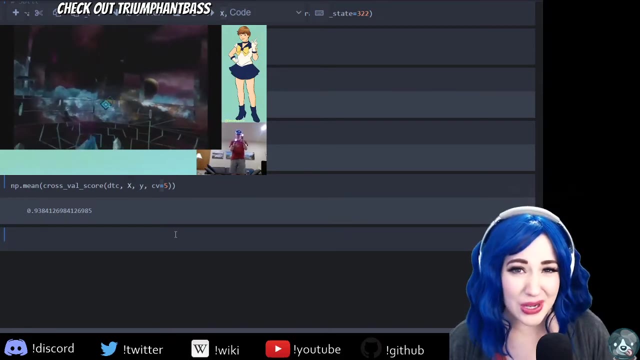 transistor, i think, which is an amazing, amazing game. but thank you so much for the raid, welcome, welcome. we're doing. we just did a decision tree, but i'm gonna, i'm gonna plot our decision tree for us so we can have a- uh, um, i know, third tier the promise. i've also got music going, so i'm keeping. 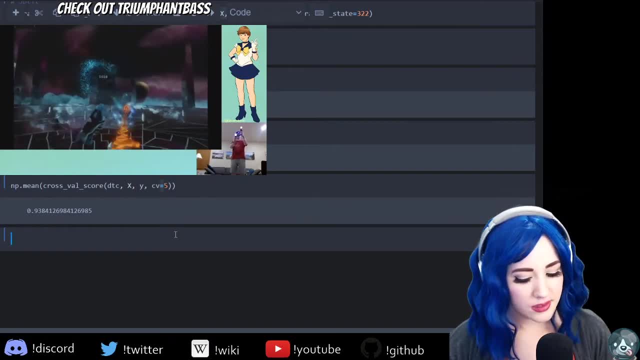 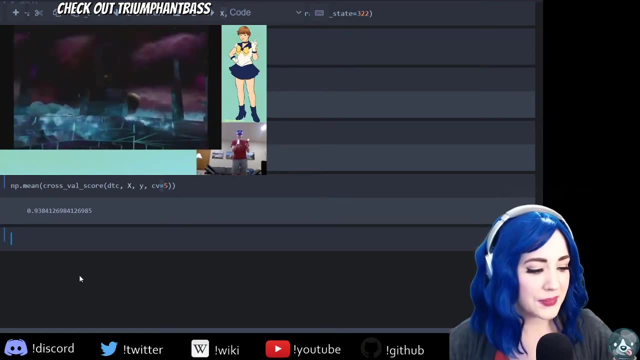 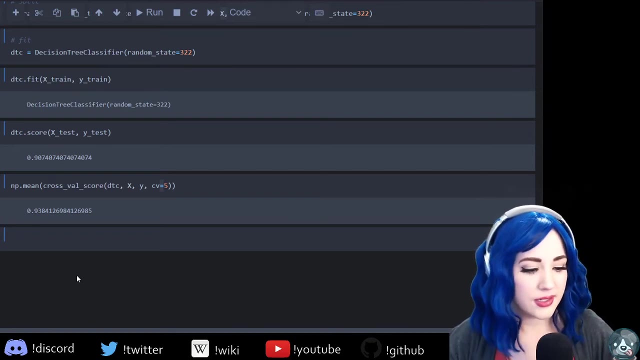 the, the um, the volume for the desktop a little bit down because, um, previously people have said it's too loud. so the downside is the clips. i'm gonna see if i can mess specifically with a shout out clip sound, but right now, um, in any case, right now we're, we're, we're stuck with with my. 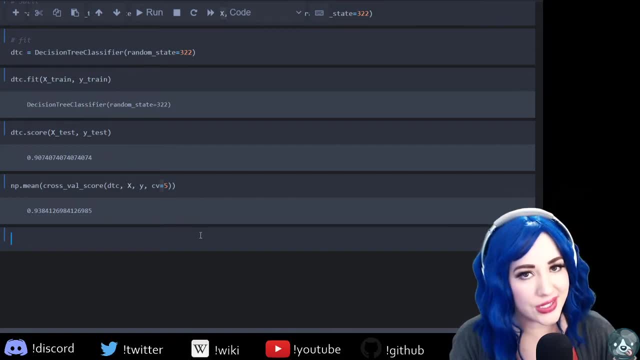 approach. all right. so one of the great things about using a single decision tree instead of our ensemble or our boosted trees is that we can visualize it. so let's, let's take a look at what this looks like. uh, what did i want here? oops, that worked. and then 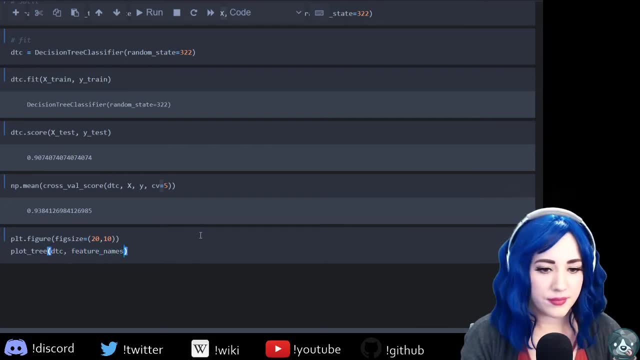 all right. so here i'm just giving it our classifier that we've trained and we've tested um and i'm giving it its feature names. the reason why we're doing negative- one right is our last column- is the label. it looks like a font size of 14 worked for me last time. columns is not defined. 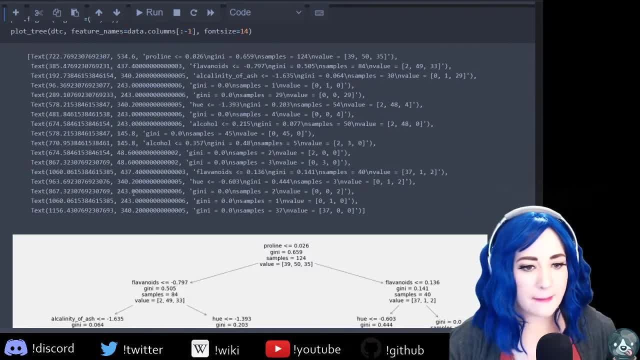 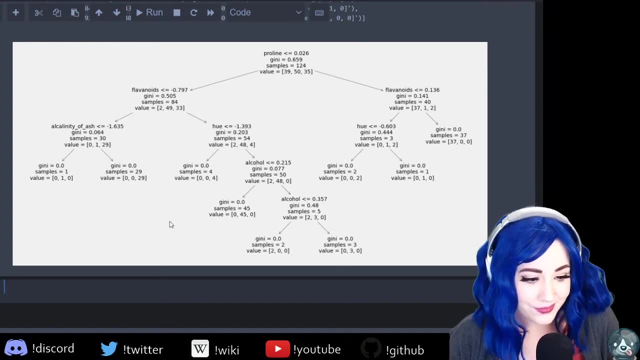 well, because i'm a dork weasel and that's not how you do it. all right. so here's our decision tree. so we're going to take a look at our classifier and we're going to take a look at our decision tree. doesn't look totally different from what i drew on our whiteboard, right? so hi. 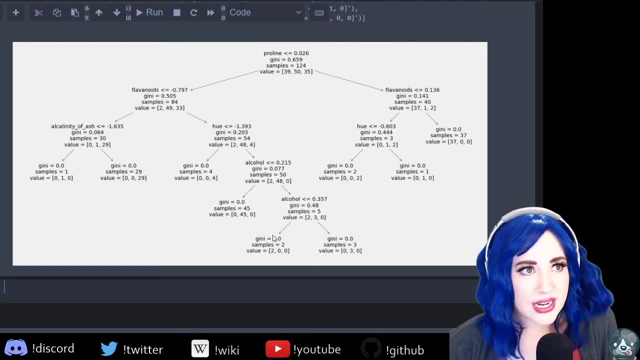 nickwan data science. so, like i said, if you're really interested in evaluating the metrics that we use for a split, so things like the genie, impurity or entropy, um check out the machine learning miss video on classification, um specifically, actually do that, do the one that's? 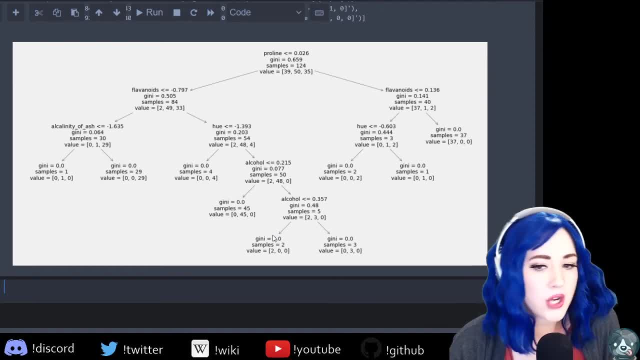 um on ensemble models, because that's where i explained all of these different ways of evaluating splits in this case. i know i'm sorry, dj velour, it is, it is. it is a little bright, but check it out so we can see that whatever a proline or flavonoids are flavonoids and alkalinity of ash, i don't know. 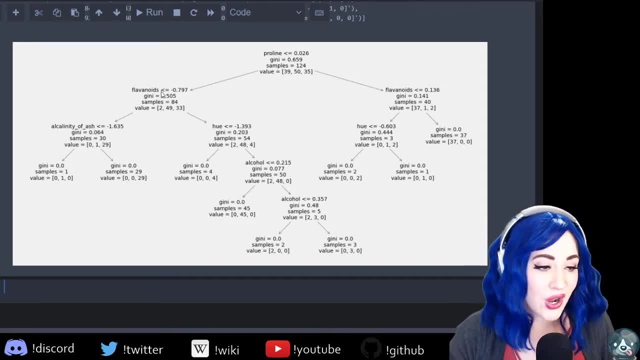 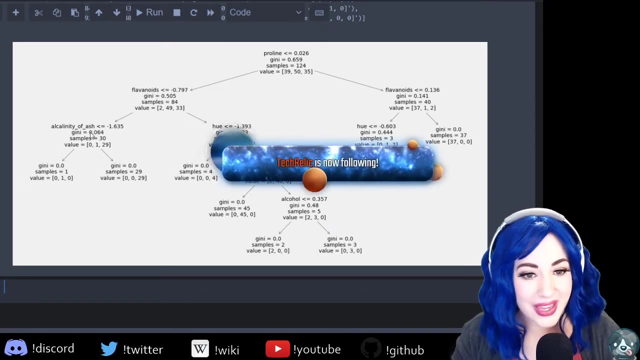 why, um that splitting based on these features, we can see the rules of how we get, how we get our leaf nodes that allow us to make classifications. so this is really cool. we're able to- we're like literally able to- see exactly the decisions it's making. 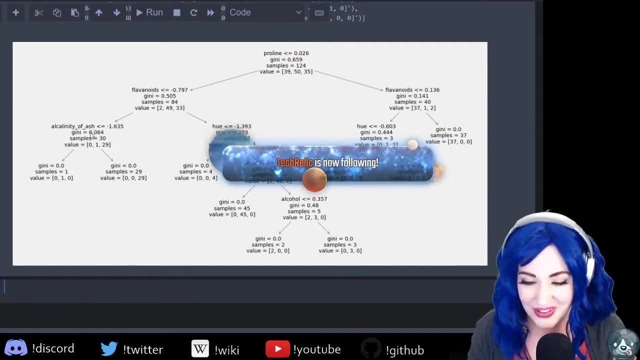 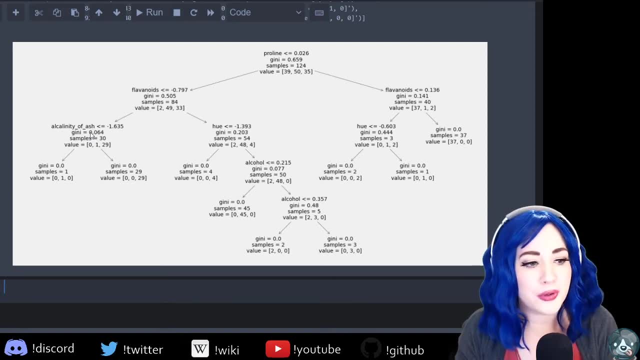 and for this reason, tech relic, thank you for following. for this reason decision trees are really great: because they're explainable, they're interpretable. you can take somebody that doesn't understand machine learning. we've all seen decision trees like this. they make memes out of them, right? maybe they don't have like as much num, as many numbers and things, but still it's an. 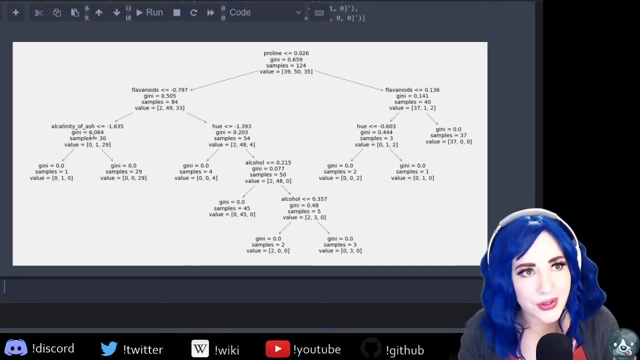 intuitive concept. now there's downsides, like we talked about earlier: overfitting and, and you know lots depth and and complexity and things like that. but i will say this in their favor: when you can, you can grab a visualization and literally walk somebody through exactly the. 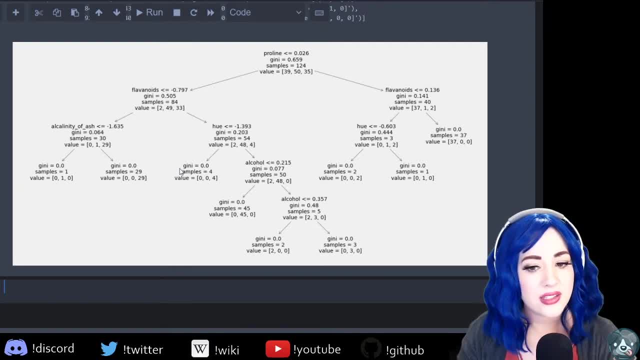 model's decision making process. it builds trust, and so this is where, like you know, for those of you interested in becoming data scientists- or maybe you're data scientists already, or machine learning developers- one of the things they don't teach you a lot of times is that they don't teach. 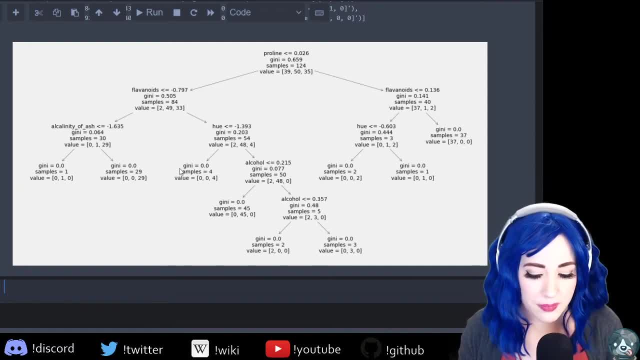 you a lot of times in a boot camp is is it's more than just picking a model based on the best fit for your situation and data. there's a people and culture component too, and building trust in a model and integrating a model into an existing workflow- that's that can be a real challenge. 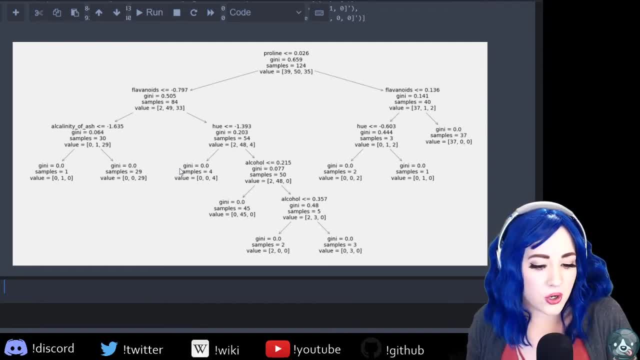 and so maybe you want, like, maybe maybe your gradient boosted trees or your random force performs better. but you know that without the explainability of a decision tree, somebody is not going to be able to do it right, so you're not going to be able to do it right, so you're not. 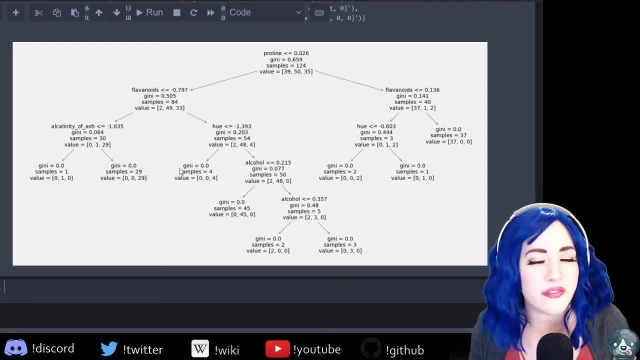 going to adopt and use your model. so it is a bit of a trade-off. machine learning is full of trade-offs, but in this case one of the perks of a decision tree is this wonderful interpretability. so if you're picking a classification model for a customer, for a client that has a suspicion of 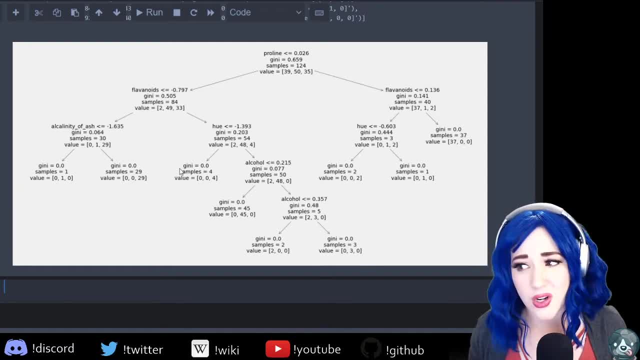 machine learning. they don't understand it, they don't like it. they're you know you have yet to build that trust. a decision tree is a great way to go because it's so explainable, so interpretable. you can literally walk them through, step by step, what it's doing and for that it's it's, it's great. but we got no clients here. we got no customers. 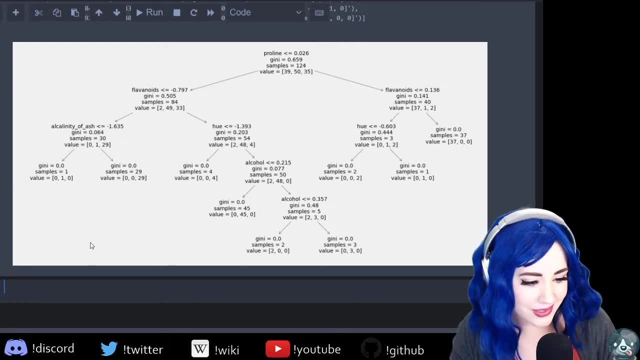 no way. so. so we're going to build some cooler, cooler models. um, and gaze into the irc, say, apparently, ash is actually ash that you get after burning the residue left from the evaporation of wine. cool, all right, wine is wine is wine is amazing. um, okay, let's see, i had some fancy. i had some fancy, some fancy visualizations, yeah, so i'm going to. 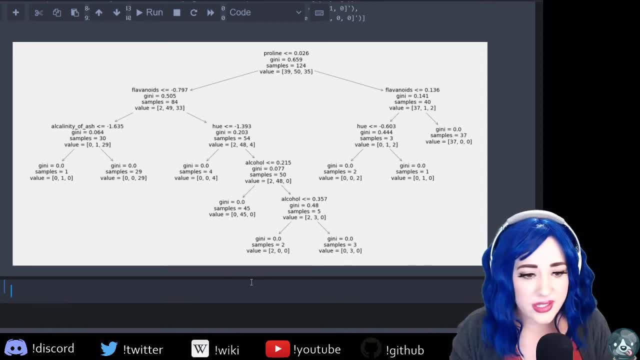 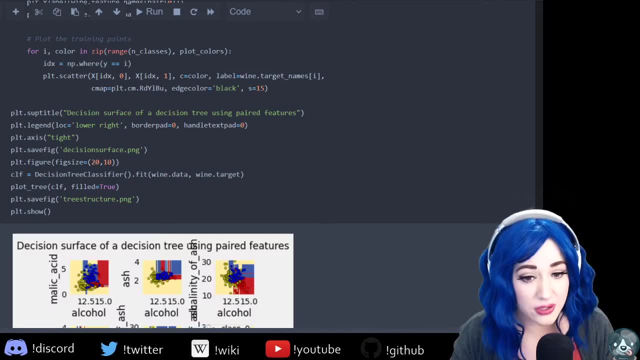 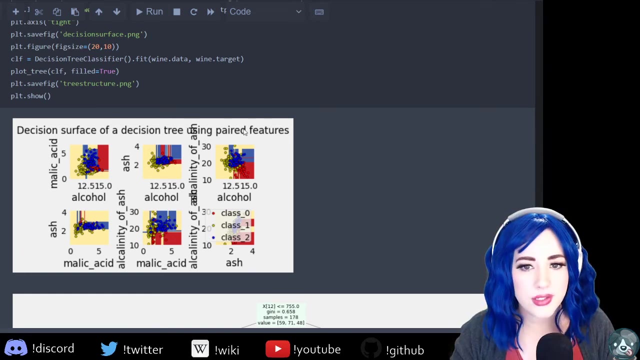 copy and paste some code. i didn't write this code. this is in the scikit learn documentation for making really cool visualizations. i don't like visualizations. i am bad at them. they are useful. i am bad at them, let me grab. so, um, i adapted code that they had written for for a decent. 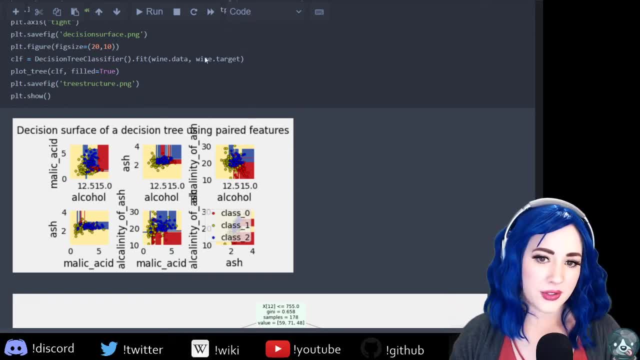 visualization here. so what i'm going to do is i'm going to copy and paste some code and i'm going to look at the password at the end of the, or rather at the end of the description, and i'm going to paste this code. that's here, and now i'm going to add all of the. 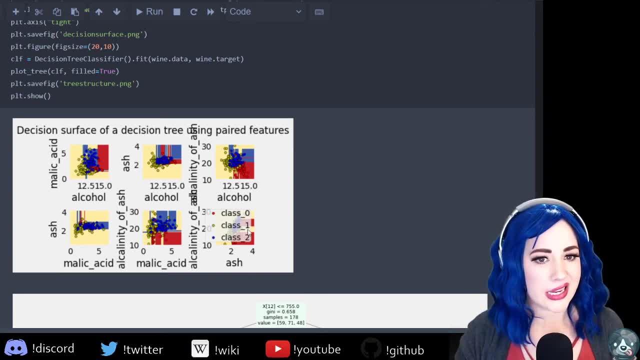 colors to that. i'm going to add um here and then i'm going to edit this out, so i'm going to paste this in there. sorry guys, all right, so now i want to change this so that i can see what the version okay is. so part of it is. i want this to be the sample content, obviously. 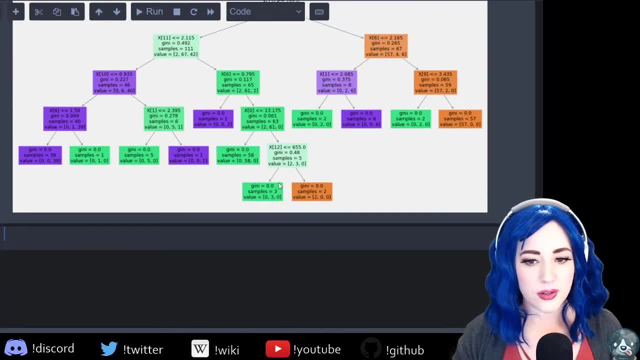 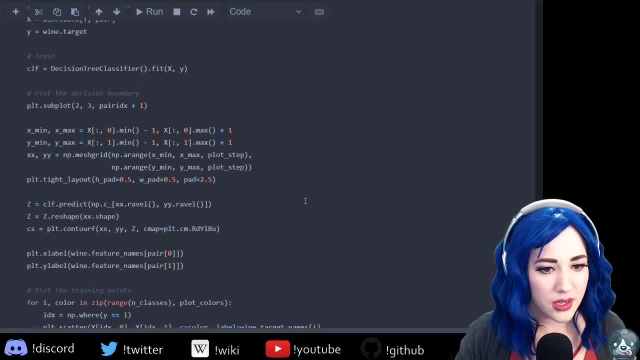 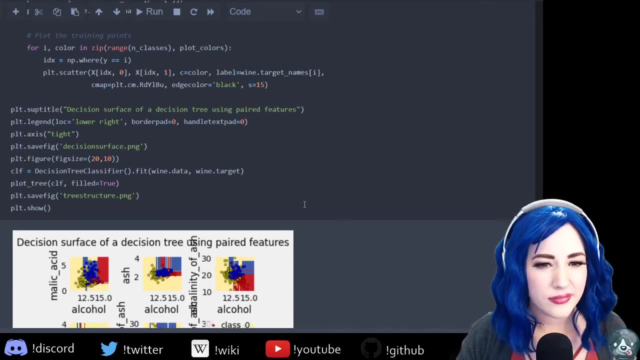 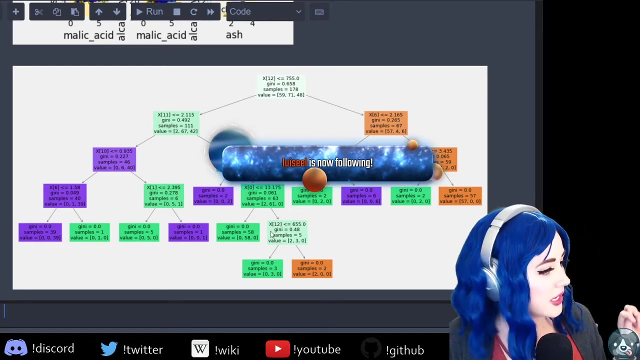 i want this to be. the И Empire is also. we've got. we've got some cool color coding with our, with our. how did they color code it? i forget color coding meant something and then i promptly forgot about it. crap, i did this right before stream. maybe it's just. oh no, i didn't put in the feature names, but in any case, 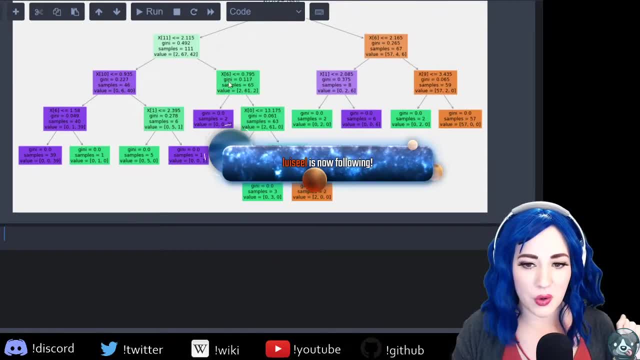 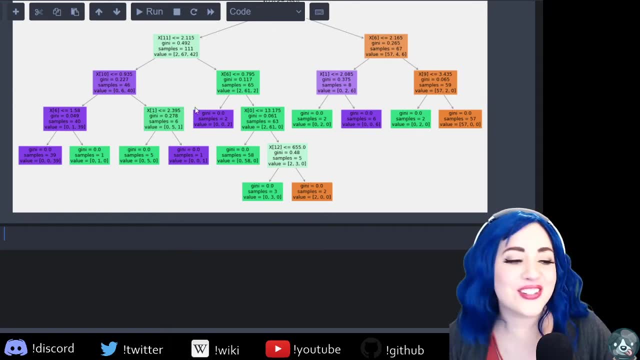 louis seal, thank you so much for following. we've got a more colorized, cool, nice version of our decision tree. um, that north boy, you hope you get an a. there's no grades here. this is an anti-grading, anti-grading stream. um, this is just all of us learning together, having a good time. 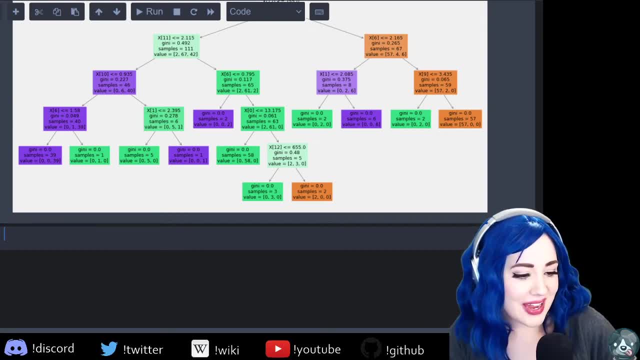 all right. uh, kevin, you say being bad at visualizations is what made you not go into being a data scientist. that's why i mean, that's why i i, even though i can do like the analytics and the eda. that is why i explicitly reinforce the idea that my title is as: 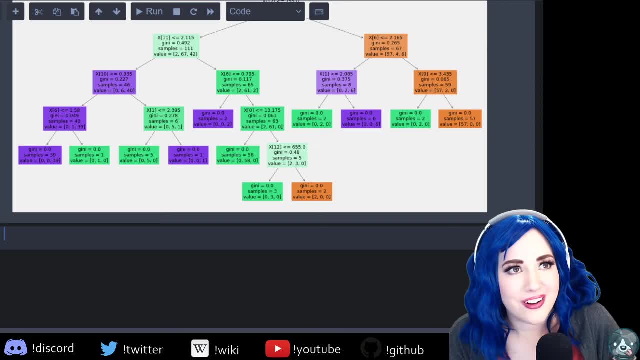 a you to like a machine learning developer because i'm so tired of being put on on projects or being asked to like build tableau dashboards. i'm like that's not, that's not my strength. i can visualize things all right, but like my strength is in building. 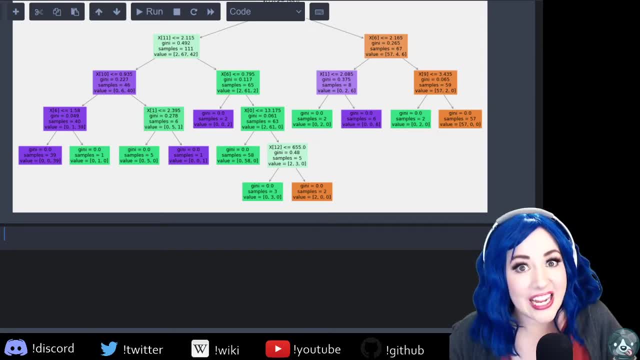 these models and evaluating them in like designing the architecture, so um. in any case, i hate making dashboards too, though that is like the most hireable talent i feel like right now is dashboards. actually, let's make sure i label things for you friendly folks. so now we're going to do uh, random. 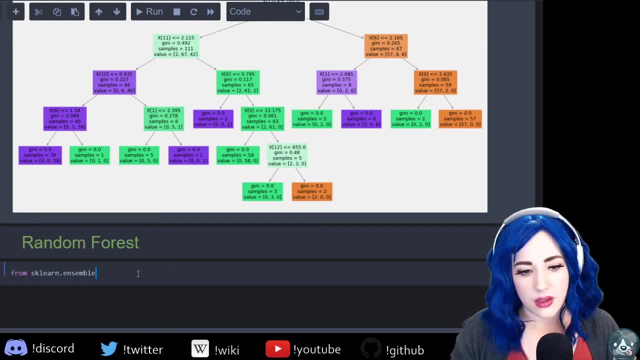 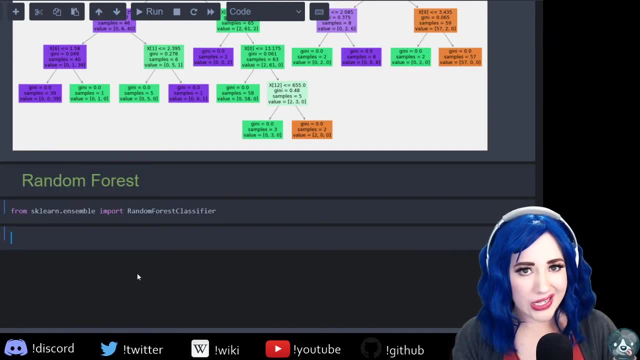 forest. so we we already got our data scaled, train test split, so this is going to go a little bit faster. of course, i've heard of edward tufty. yes, i actually own all of his books to try to help myself and i did it. i did like a two-day workshop with him. two day, one day, i forget regardless. um, he's. 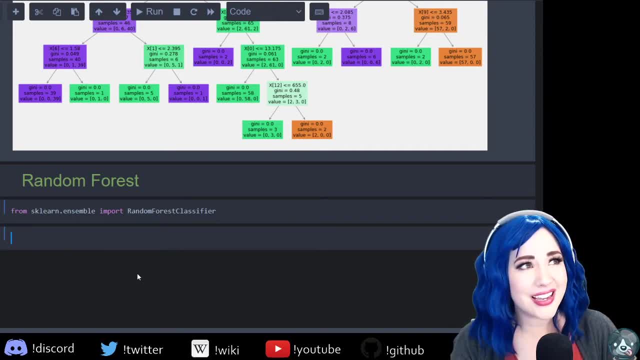 brilliant, he's wonderful, i love his books. but to me it's like i can look at it, i can understand it, i can be like, yes, this is good, i understand why this is good, like i can evaluate data visualizations just fine. can i build them myself? no, i lack an eye for design, and i know it. um, i can replicate. 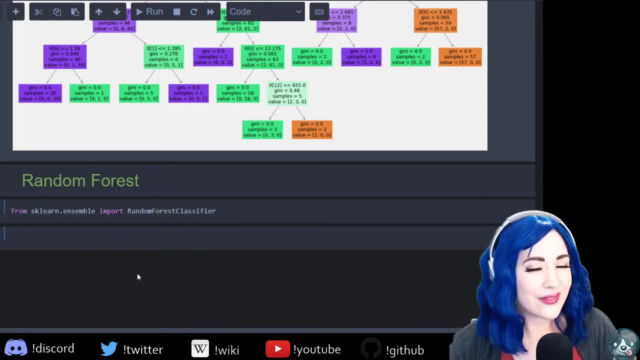 stuff really well. so even when i like i wanted to go to art school and everything, and even when i wanted to go to art school, i was good at like portraiture, so like looking at somebody and like making a portrait of them. but if you wanted me to like create something brand new out of my head, i 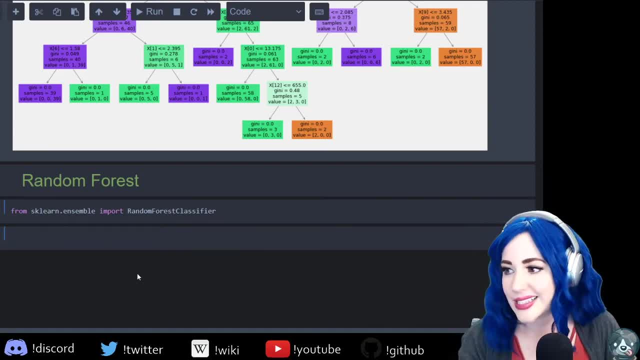 struggled with that. so, alas, we all have our strengths. it's cool, um, all right, so let's, let's, uh, let's, build our random forest classifier and candy cane. you say, do you plan for a� laugh science classifier? and i didn't even wave at you last time. 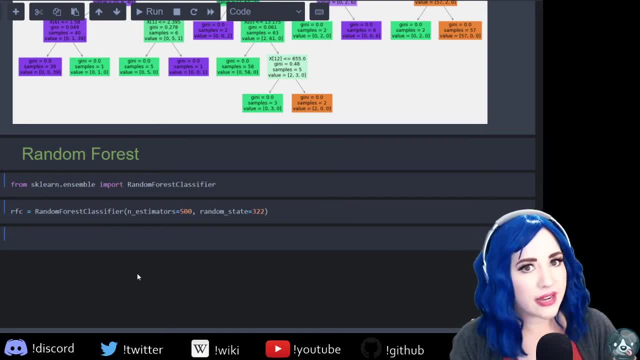 i'm just kidding. it's super funny if you guys use continuedDaVa, just until you don't這 littleiven call it an arm Floyd. what is do you plan for? ết have to do a lot of powerpoint presentations. i used to have to do a lot more and i i talked to. 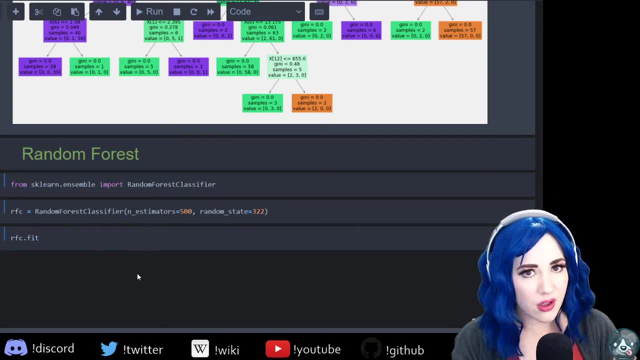 my work because i was like: this takes me like 20 times as long as it would take an actual designer. i'm tired of having to do this. my strength is in writing code and all of my time is being taken up with writing power like: what do you want me to do, which? which thing do you want to pay me to do? 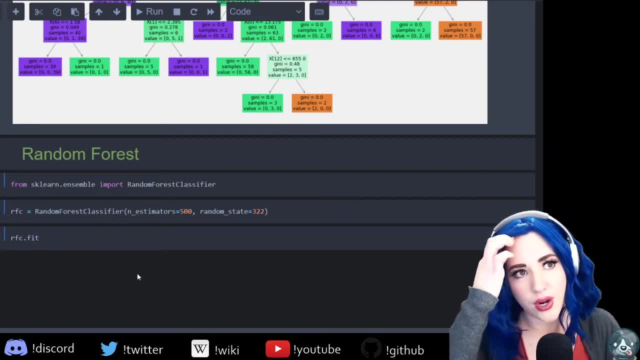 so i like negotiated with my work and got put on projects where, like i have to do decks for the client of like summarizing the results, but like it doesn't have to be super fancy. so now i'm way happier and i do have adhd, kevin, can you tell? 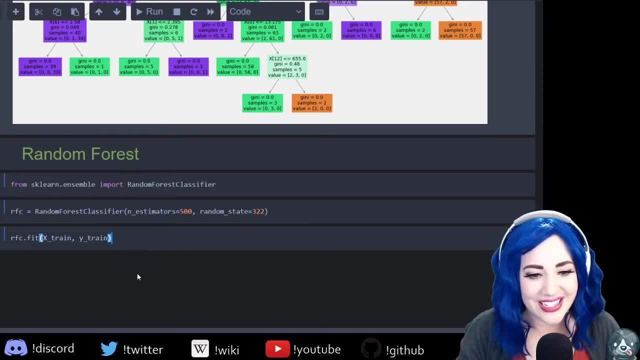 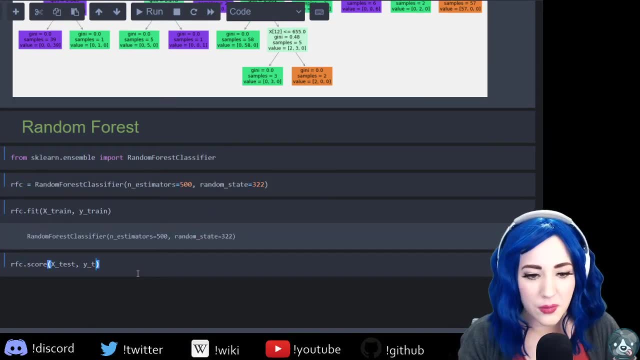 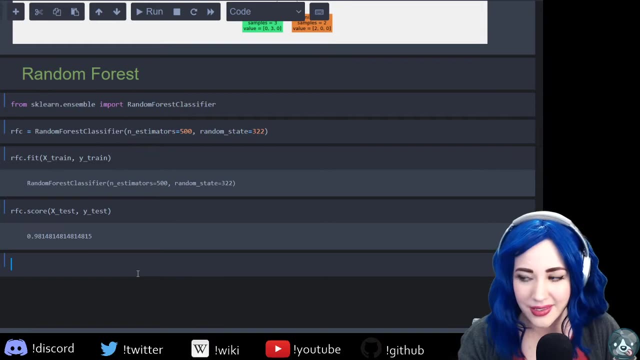 i've learned to live with my adhd. i don't mind there. there's days i hate it more. um, so again, we can. we can try our our blank. oh, that looks nice, that's, that's fancy. look at that, look at that wonderfulness. but let's, let's you know. 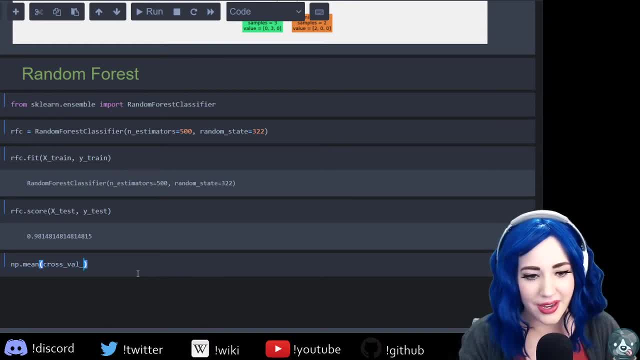 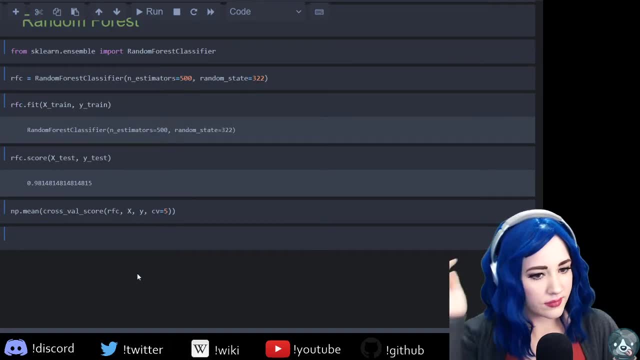 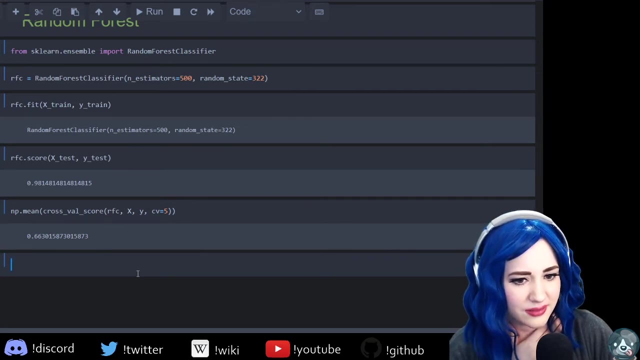 you, let's, let's do our due diligence and let's actually do and get our cross validation score. and then my chug-a-lug for a second. um what? oh well, no, hold on, give me a sec. what did i do? i goofed something? uh no, you don't. you don't cross validate. 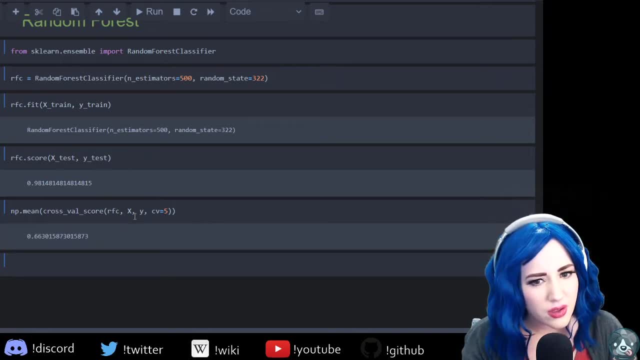 what on earth hold please. what did i goof? i was talking and let's see here. all right, let's debug this. um, because running the exact same code right before stream, i got 90.93. What happened here? what did i goof? have i redefined the delineating system? 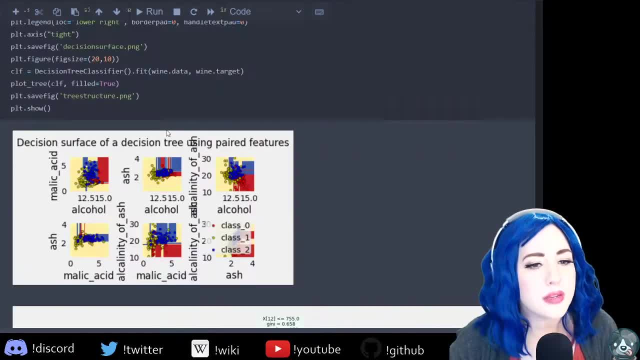 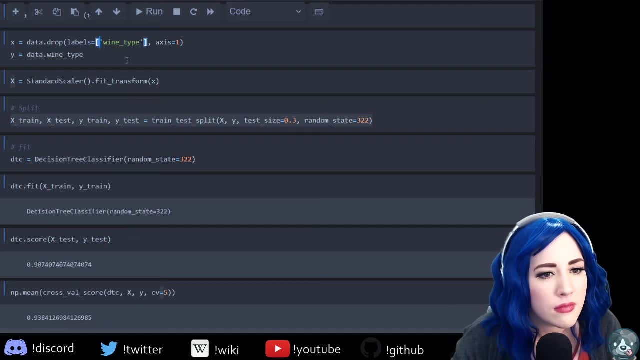 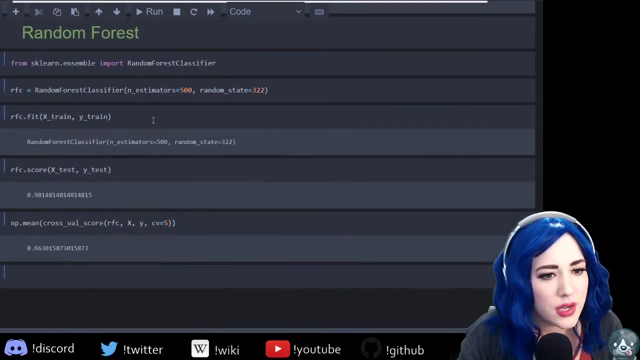 what is wrong? oh wow, redefined. So sometimes this can happen. So I do remember just a sanity check. Hold on, I don't think. I think I might've redefined X and Y in the previous plot is the problem? 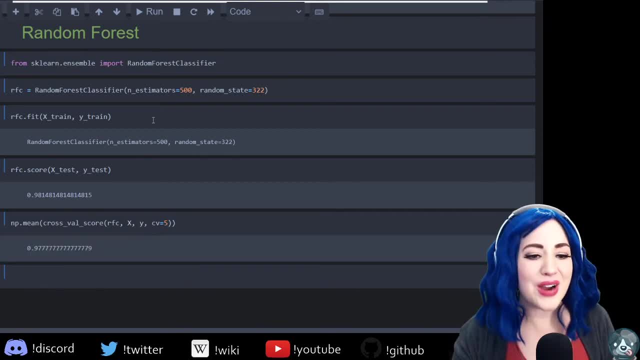 And that was that was my fault for copy pasting code. There we go, All right, So that was the problem. in the previous visualization I redefined X and Y, and hence why we got a little bit of a funky answer there. but all right, this is looking a little bit more more like what we 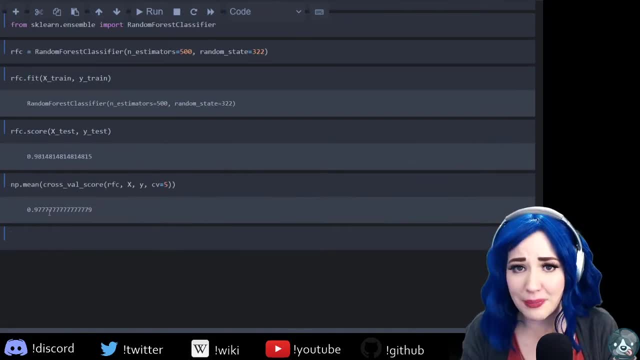 would expect. So we still have a great jump in our performance, but again, our initial accuracy score was a little bit misleading. Um and let's see. uh, yeah, you know, ADHD for me, like there are days when I am grateful for it because that hyper-focus. 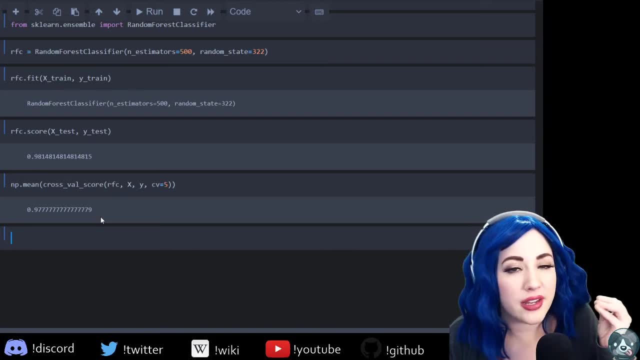 that I sometimes get means that I can get so much work done in a short period of time. And then there's days where I feel like I'm fighting my brain all day, and that's a real challenge. So it's, it's, it's it's a thing, All right. So one of the cool things that we can do. 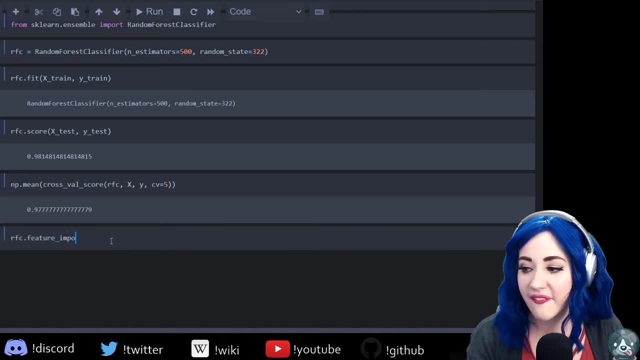 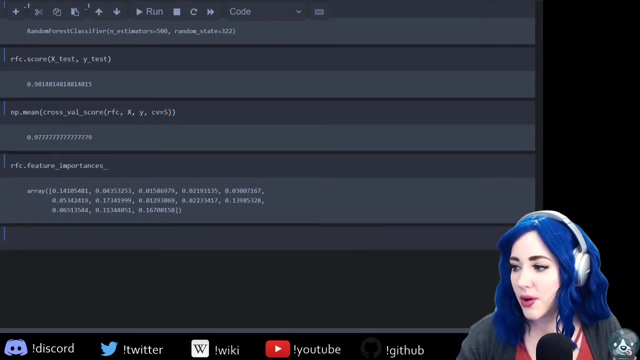 both with decision trees and with random forest- is we can look at our feature importances. So this isn't super helpful because we need our columns. So, guess what? I found some nice data visualization code. That's not my own, So I'm going to go ahead and do that. I'm going to go ahead and do that. 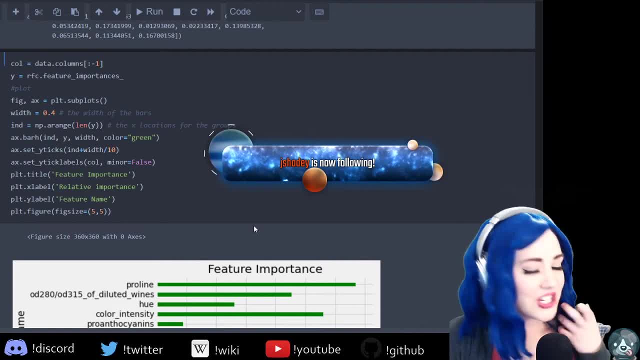 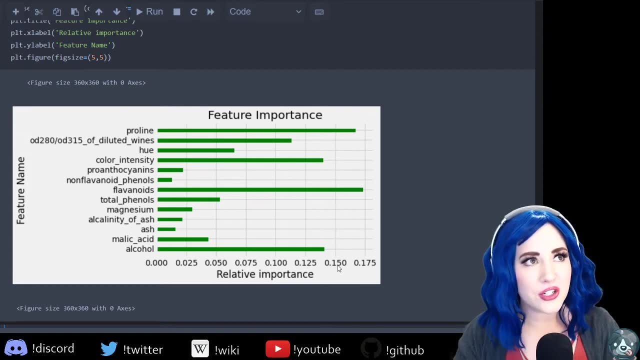 Um, um, and let's see Jay Shady. thank you so much for following, All right. So feature importance: what does this show us? What is feature importance? So feature importance is if we feed a whole bunch of different features- right, X, different Xs- into our model, not all. 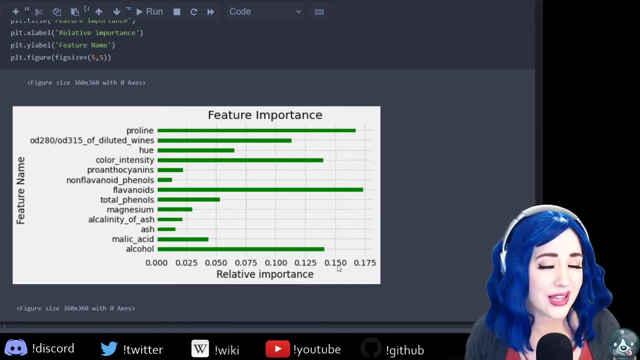 of them are going to be as useful for making those classifications. Some features are going to be more important than other features when it comes to classifying our data, And this is telling us that proline, whatever that is, um, color intensity, flavonoids and alcohol content. 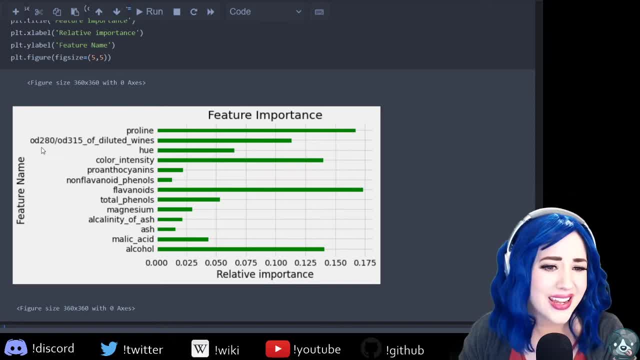 are actually the most important things And whatever OD, 280, OD, whatever this is, those five features are the most important when it comes to classifying different kinds of wine. And hi Jay Shady, Welcome, Welcome. And hi Cfilms again, Um. 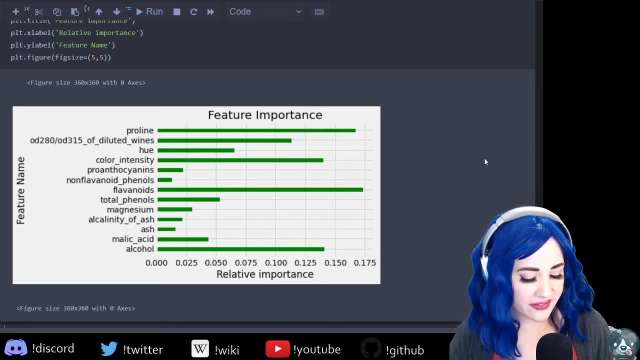 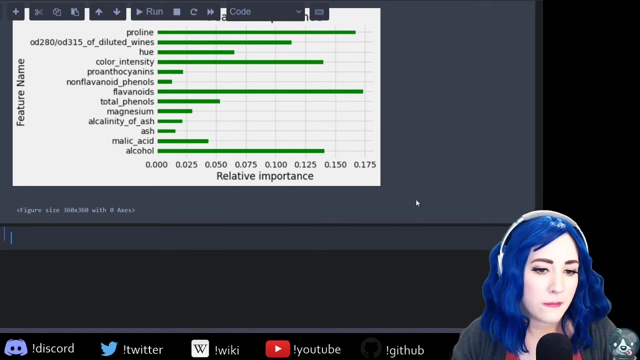 and you say honestly, I find if I'm not medicated on stream, it's more difficult to interact with chat Um. most times I stream on the weekends I'm not medicated. today I was because I was very tired and I knew I wasn't going to be able to prep, prep stream um without my ADHD medication. 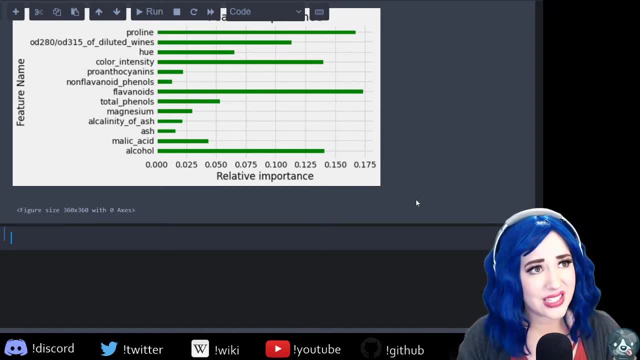 That said, I made the mistake of- and this is, this is the dangerous. I love my ADHD meds, but whatever I am doing when my ADHD meds kick in is the thing that I will be stuck doing for a while. So the problem was is I was reading a really good book? 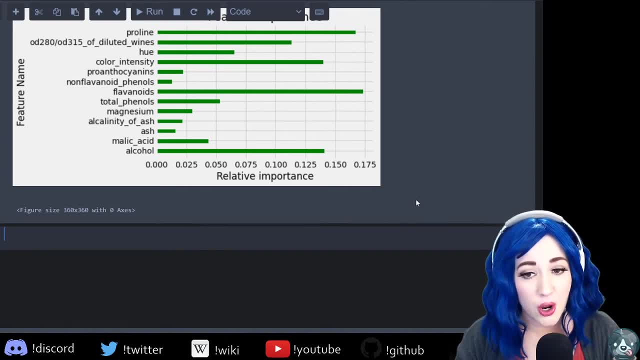 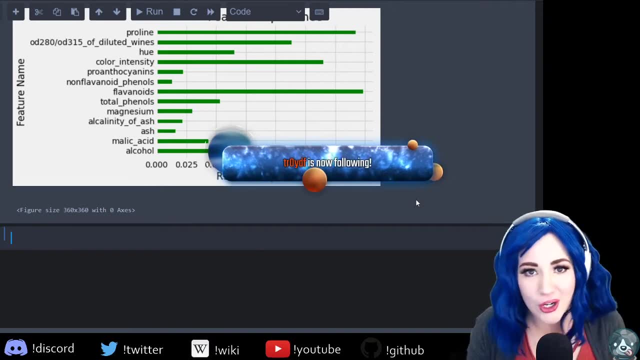 When my ADHD meds kicked in five hours later, I went: oh crap, I'm streaming, I need to write some code and figure out what to talk about tonight. So it's, it's a challenge. if I'm like coding or cleaning or something when my meds kick in, it's great, I get so much done. 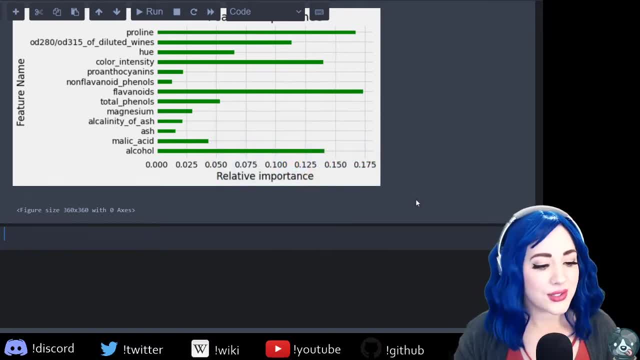 Troy DF. Thank you for following. All right, So let's, we're going to be able to use this, this feature importance to um, help our performance for our gradient boosted trees, Um, and so we're going to use the word max depth. It's basically a tree, which means we can use. 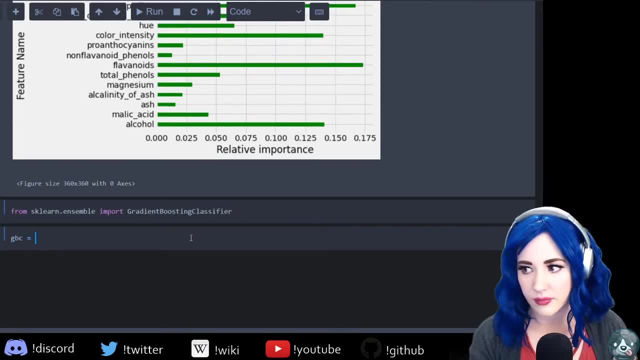 the same number of- uh, kind of the same amount of trees or the same number of trees we were doing in our previous one. So, um, if we use the x, we're going to be able to use a number of, a number of a number of trees that we're also able to use as well. You can see that I have. 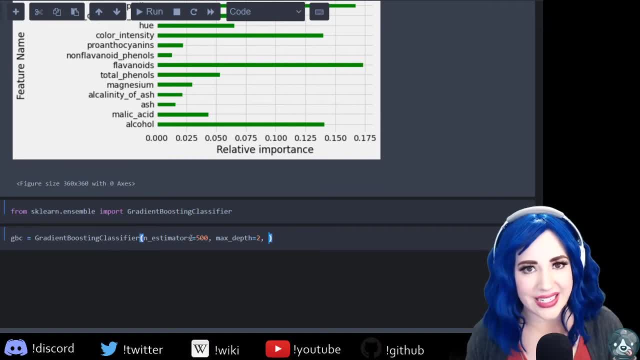 the song number right here, which is the number that I put together. So now I'm going to use the um, Like we don't need this extreme depth, because really, what we're trying to get out of this is right. we're just trying to get these weak learners. 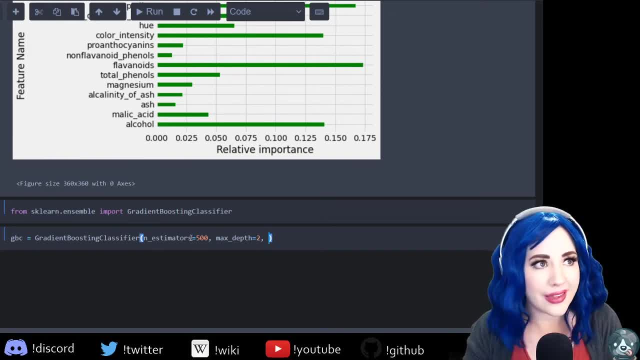 and we're just trying to quickly, iteratively improve on them. We don't need like the best decision tree And Jay Shady. yeah, I like to be really open about my mental health, So I'm part of the accessible stream team as well. 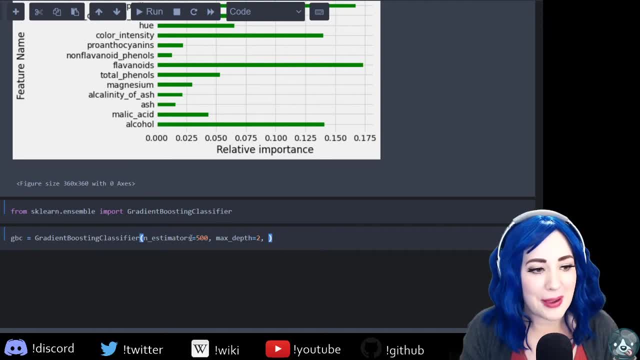 and started out as mostly gamers, but I'm trying to bring that culture over into science and tech because I have both a chronic illness and I have ADHD and anxiety And I feel like we need to talk more openly about these things because a lot of people 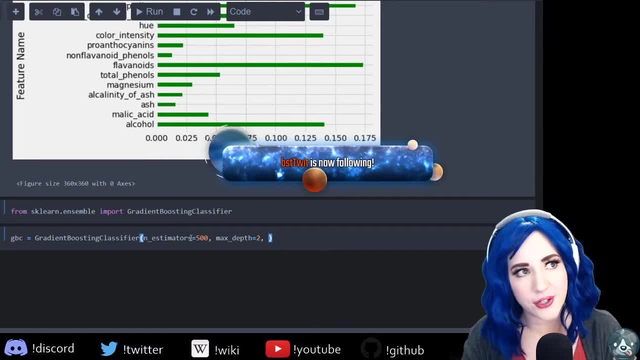 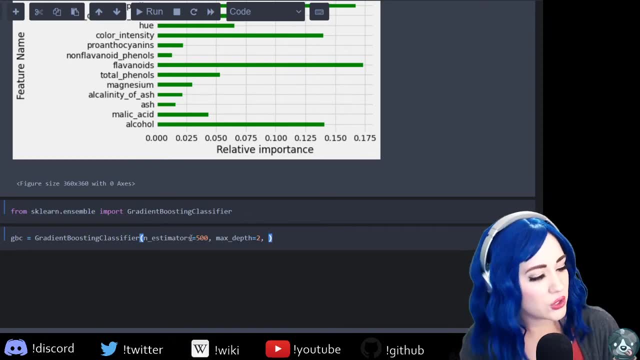 a lot of people struggle with them And if we want society and our jobs and Twitch to be more accessible, then we got to talk about it. BST Twit. thank you so much for following. But yeah, on previous streams, especially the Math Monday stream. 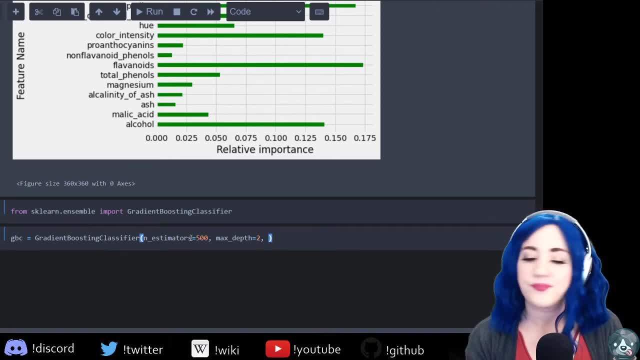 I feel like we talked a lot about mental um. okay, So also max features. Why might we limit the number of features we're going to use? Someone, someone. let me know what you think. Why might me? why might we limit the number of features? 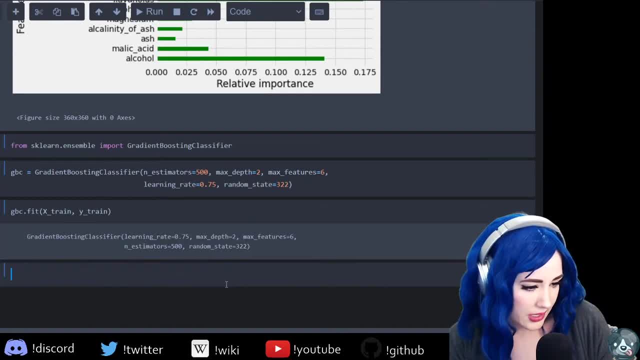 Let's see So we can only get the more important ones. Yes, But why? why do we want that? And with screen it might be the curse of dimensionality, but here we don't have a lot of features, So I'm not necessarily super worried about dimensionality here. 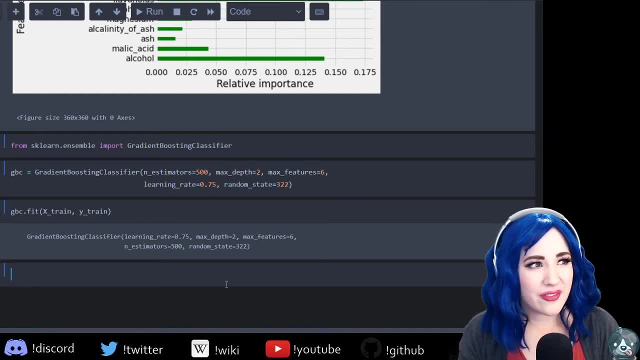 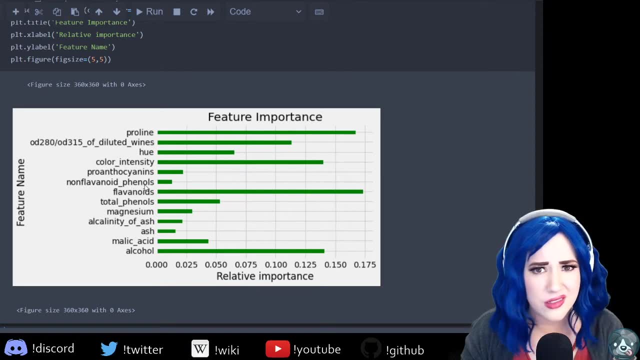 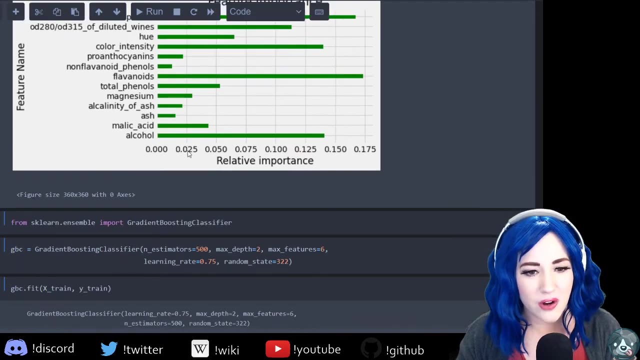 Here I'm really worried about noise. right, If we have a way to simplify our data set, if something like ash or non-flavonoid phenols, whatever that is, if these aren't contributing very much at all to the decisions of our model. 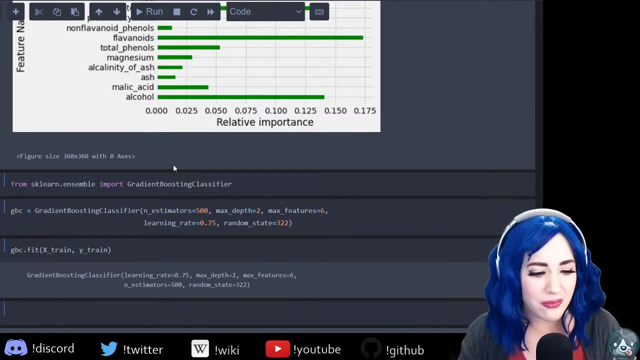 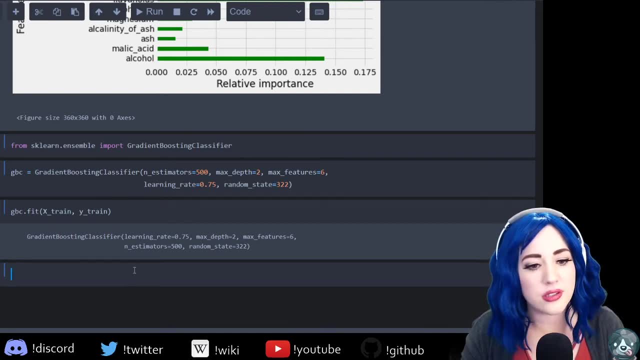 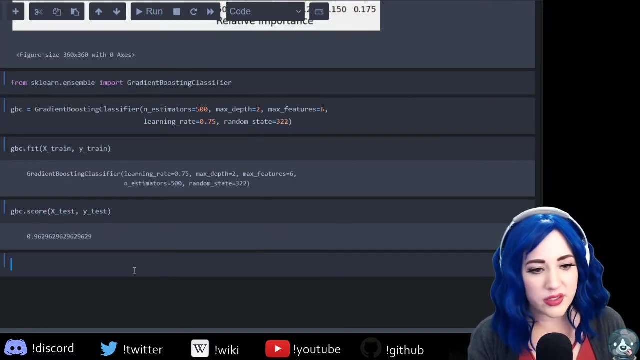 including them is just giving more things Our model needs to fit that are not helpful. So we're able to simplify, to improve the model performance by just limiting ourselves to the features that are the most helpful. So again, let's score ourselves worse. 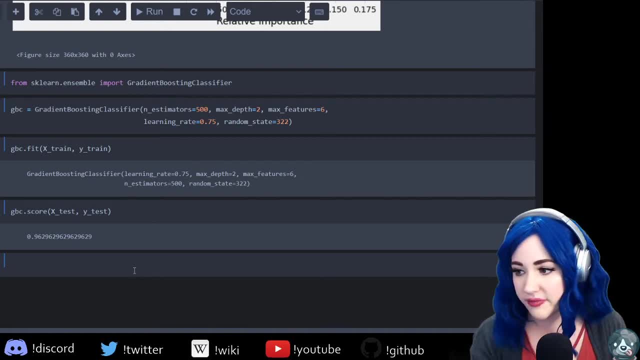 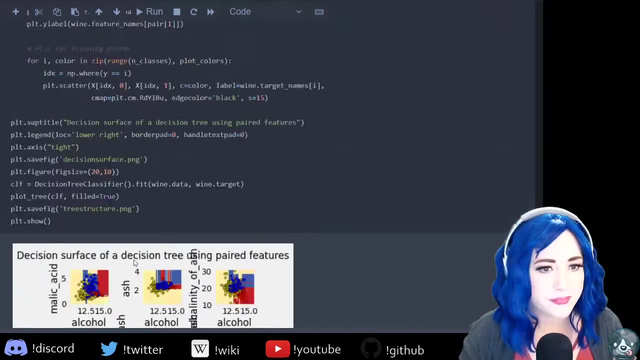 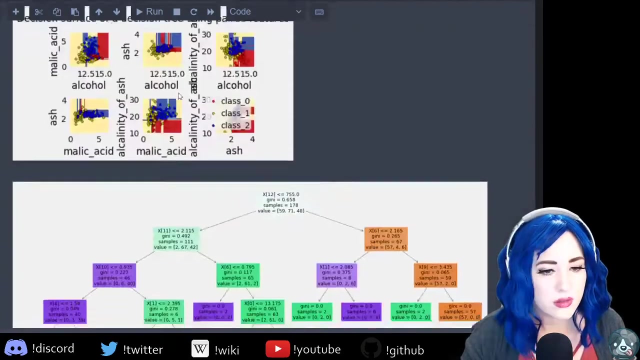 actually worse than than our random forest. What did I do? Oh, I did this before. Hold on. This is what happens when I goof. things Should work. I'm hoping that I was able to get a little more information. I'm not sure if it's going to work or not. 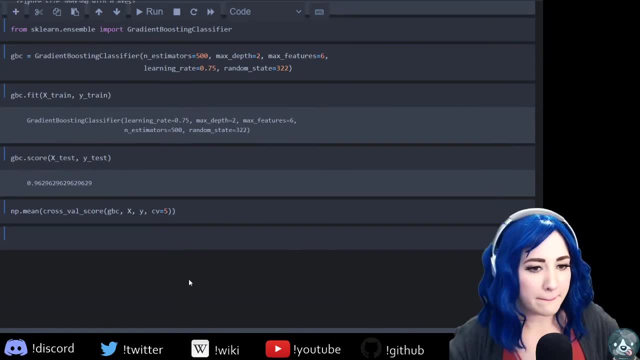 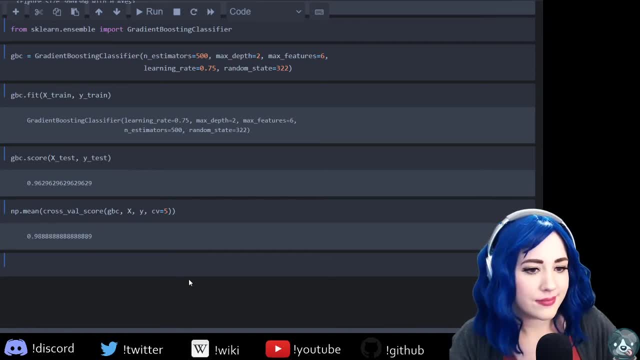 I'm not sure. Um, there we go. Best performance we've had so far for rounding. we got 99% accuracy. Gradient boosted trees are awesome. Um, and let's see. Jay Shady, you ask what is the difference between a gradient boosting? 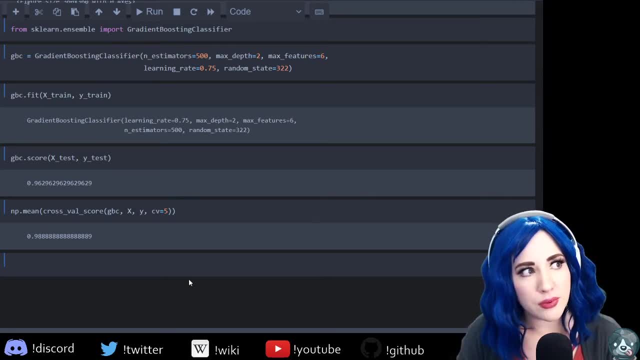 classifier and a normal decision tree. So in a gradient boosting classifier. so our gradient boosted trees. the simple answer is that instead of just having one tree, we're gonna have a lot of trees, but unlike a random forest where you have all of those trees, 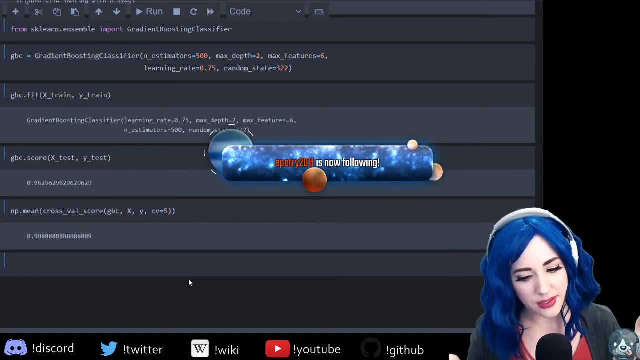 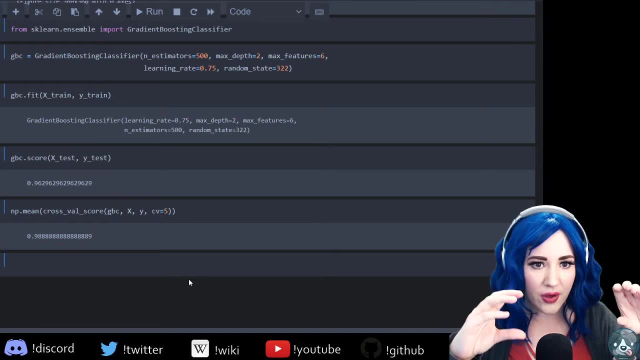 acting kind of like they're all independent and they're all doing the same task. what we do is we start with a really crappy tree and then we train the next tree on the errors of the crappy tree, And then we add those two together and then we have another tree. we test this one. 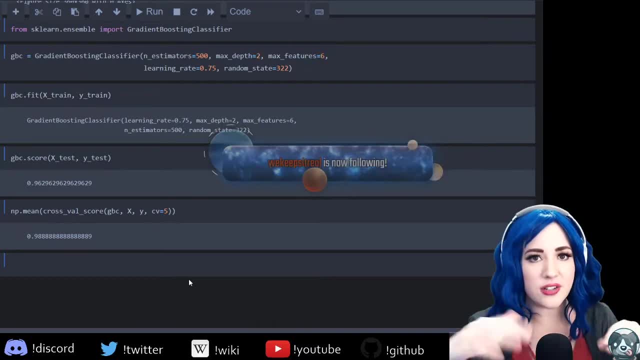 and then we train on the errors of that one, then we add it, and then we train on the errors and you iteratively, essentially, are sequentially adding more trees to your model, each one fitting on the mistakes of the previous one And E Perry 2011,. and we keeps it real. 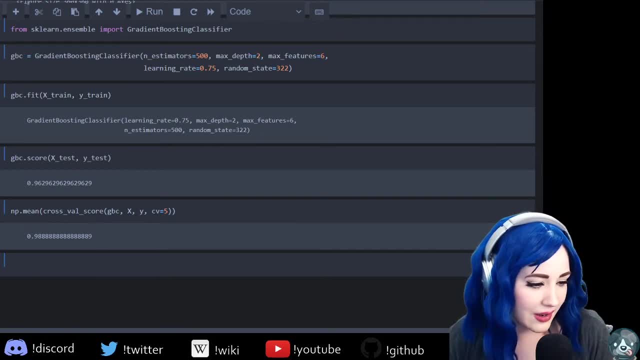 Thank you for following. Welcome. welcome to stream. So let's kind of talk a little bit about what we just did here. We built a single decision tree, We evaluated it, We talked about you know how. maybe accuracy isn't the best metric for all classifiers. 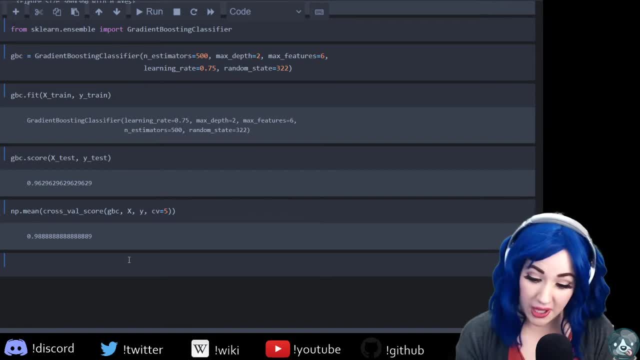 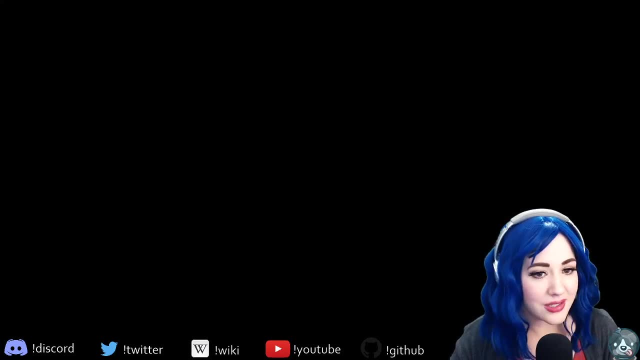 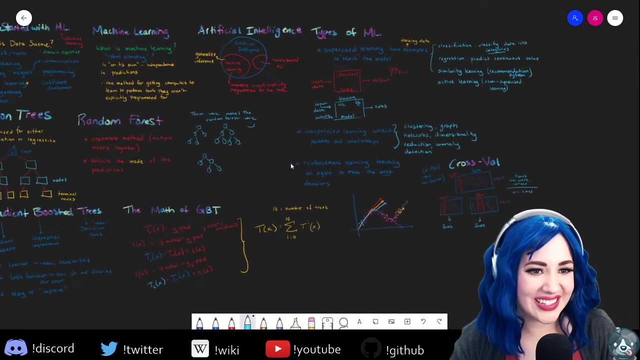 We talked about cross-validation. We built a random forest, We evaluated that. And we built a gradient boosted classifier, gradient boosted trees, and we evaluated that. Plus, we talked broadly speaking. if it'll scroll out, it's a little bit struggling. 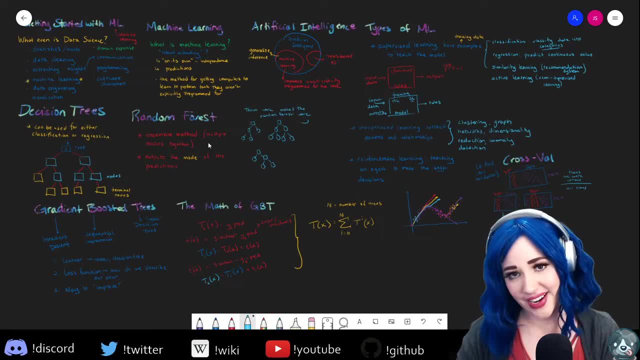 We talked about getting started with machine learning: what data science is, what machine learning is, what AI is, different types of ML, talked about the theory behind decision trees, random forest gradient, boosted trees, including some math, and then a quick little like a refresh. 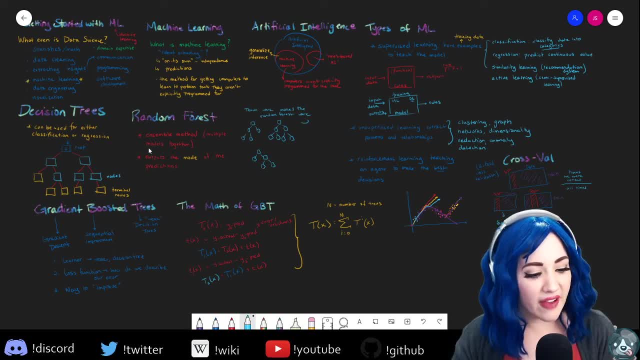 So that's pretty much for what cross-validation is. And Casadoconhio's 500 estimators mean 500 trees, So we're gonna add 500 trees. My ID: yes, so for stream tutorials I like to use Jupyter Notebook. 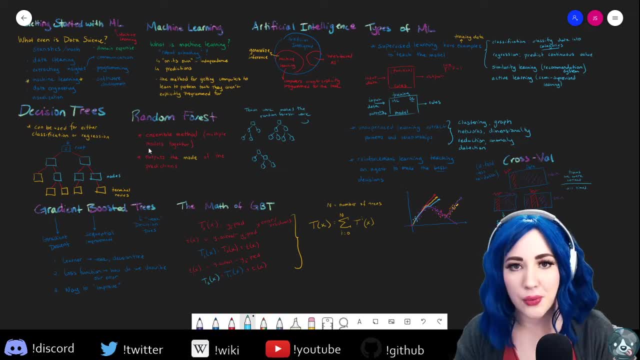 because I can kind of run people through code line by line. I get you know inline visualizations. It's really great For work. I use VS Code though, but I've used Atom, Sublime Text, Pride, PyCharm. I didn't like it. 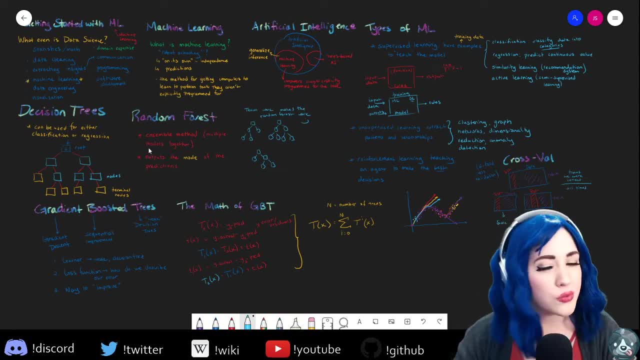 So you know, to each their own. IDE is just a tool, so whatever you like works. In any case, though, this has been your whirlwind tour of one way to get started with machine learning, which is classification right, Supervised learning. 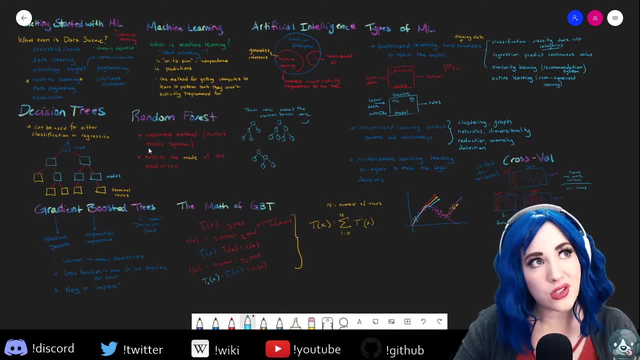 And kind of. I wanted to show you the evolution there, how you can start with a really simple classifier like a decision tree and you can iterate it and make it better and better by you know, either having it on software or you can do it, you know. 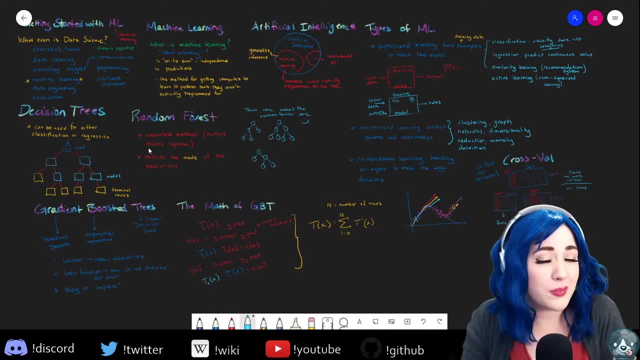 with an ensemble approach, like a random forest, or a sequential ensemble approach by, you know, training each sequential model on the errors of the previous one. And hi forked, get forked, bish, How are you? And Casadocanios, yeah, VS Code does have. 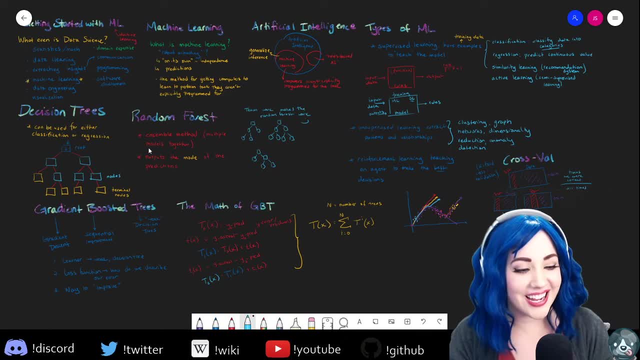 and yeah, third tier, VS Code has a Jupyter extension. It's not as nice as like my custom Jupyter themes that I've tweaked and gotten to where I like them, So I prefer to use these for stream, but VS Code absolutely does have a Jupyter extension. 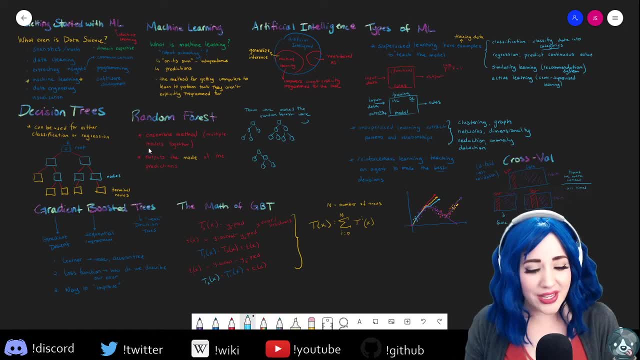 All right, how do you feel? Are there any questions about this? We can talk. This is probably gonna be our Q and A portion of the stream, So we're gonna- it's a little bit more casual- Ask some questions. Let me see how am I doing on time. 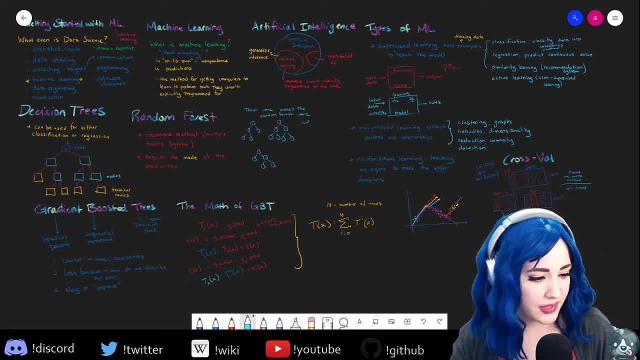 I'm not the worst, not the best, but not the worst. I talked a lot. Have I found the paper about dimensionality and distance measures you mentioned? Oh shoot, it wasn't a paper, It was a website. Let me make another note. 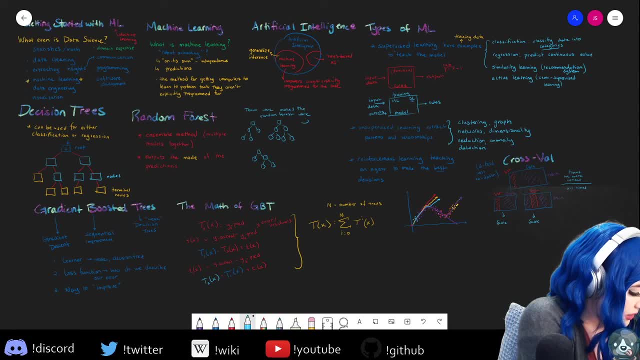 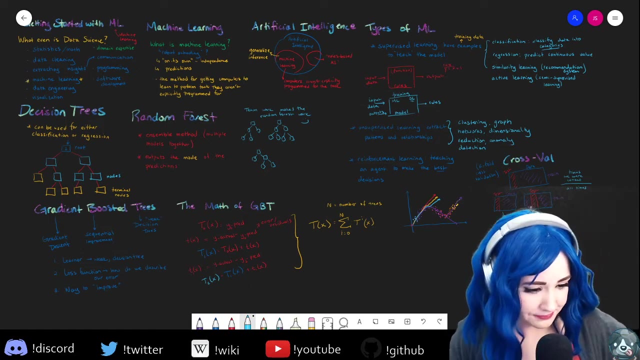 I'm so sorry, Strawberry Jesus. Hold on Distance measures for Strawberry Jesus. One of the downsides of ADHD is, if I don't write it down, I forget. And absolutely, Casadocanios. you can glance at the code all you want. 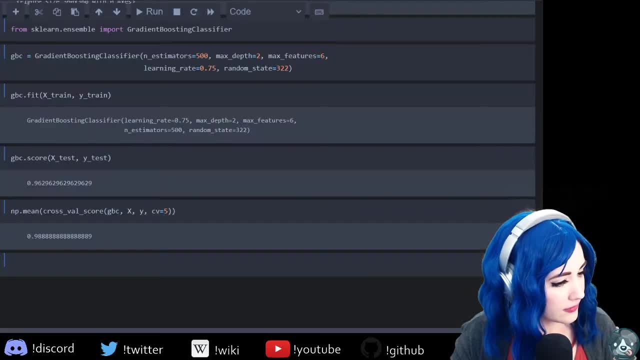 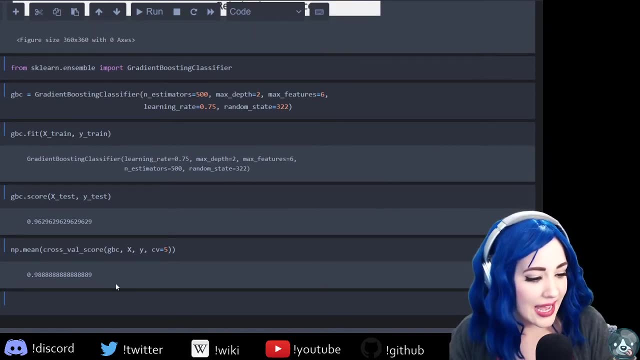 Give me one second here. There you go. So if there's one specific area of the code you'd like to look at, just let me know. I can scroll to wherever. And yes, that Northway, this is going to be on YouTube. 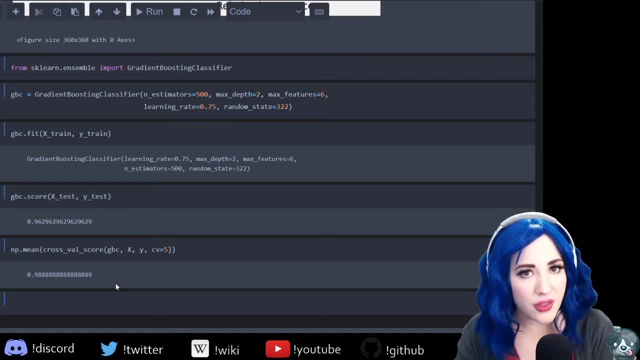 So, just like with the machine learning mistreams, this is part of another series, Fundamentals of Data Science, And this will absolutely be on there along with also the Math Monday streams. Let's see, I'm so glad, Jay Shady. 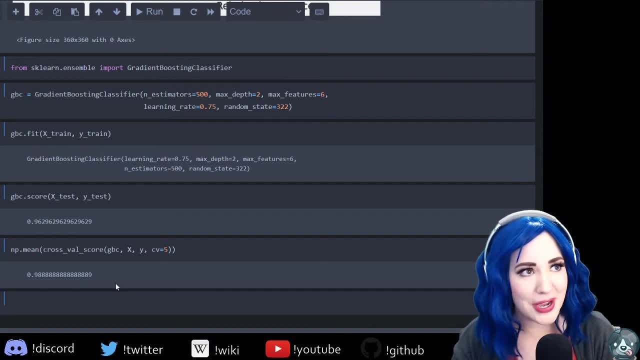 Yeah, I'm constantly on the lookout for more science and tech people, But you know, machine learning in particular is really fun, So I love seeing how people are gonna use ML for different things. All right, so let's see here. 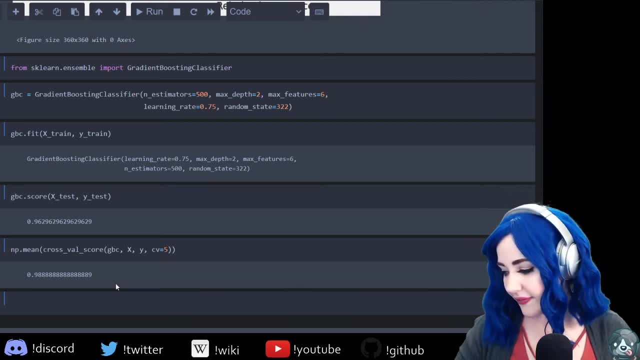 It is 10,, 10- 40. So we got a couple options. If there are lots of questions, we can kind of have a little bit more of a casual Q&A. We can go through parts of the code that people might have questions with. 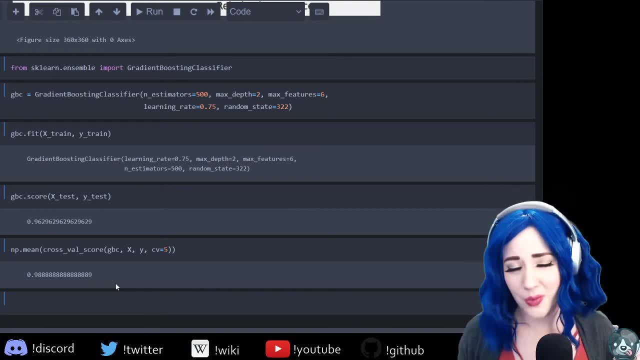 If folks feel really confident with this, though I have no problem if you just want me to whip Tennessee out and you want him to sing for you. So actually let me see if stream polls are working. Can I manage a poll? New poll. 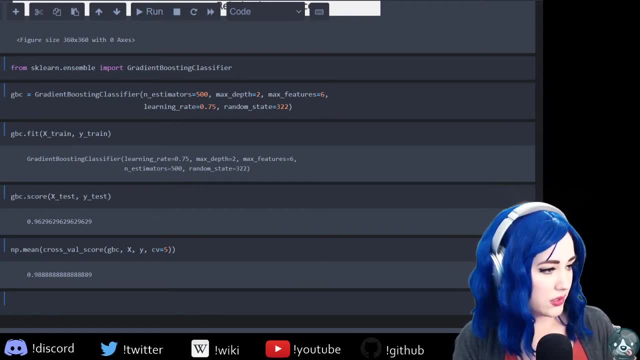 Next? Oh, what to do next? Hangout plus Q&A or 10 song. Did it work? Oh, look at that Actually got it working. Let's see. I'm interested in the visual computing side of ML. So are you talking? give me more details. 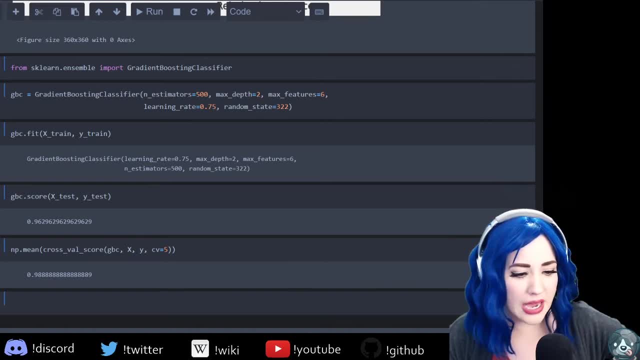 Are you talking about, like visual programming, or are you talking about computer vision or something else? And Whiskery Aunt, just feel free to DM me any links. So I got some trolls that are happening as the stream is getting larger, And so I've had to turn off allowing everyone to post links. 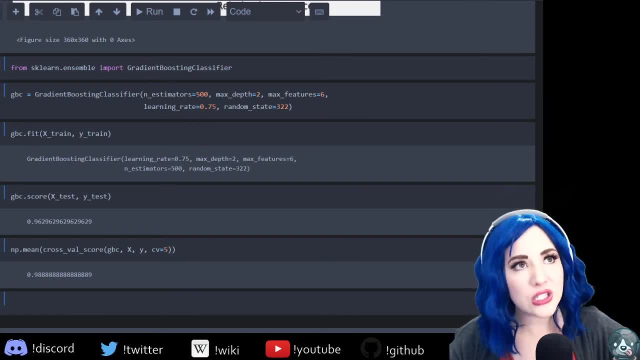 I apologize. Computer vision- Yeah, so I did a stream on computer vision and I've gotten some interest in doing more. I think it could be the problem with CV, just like with a lot of deeper neural nets and deep learning in general. is that the training time? 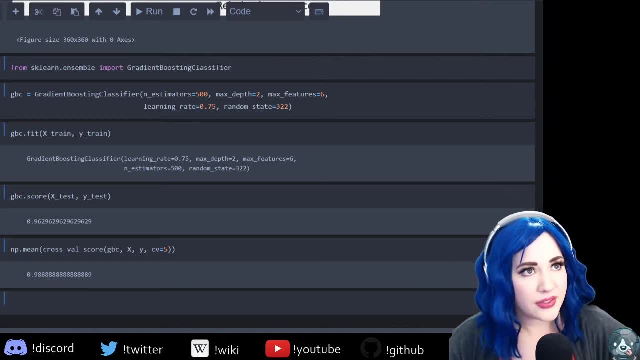 like to do really cool stuff with CV. like, the training time is just prohibitive for Twitch. So either, like, I walk you through like how to build the model but I skip, like the training portion, or I train like off stream and have a pre-trained model. 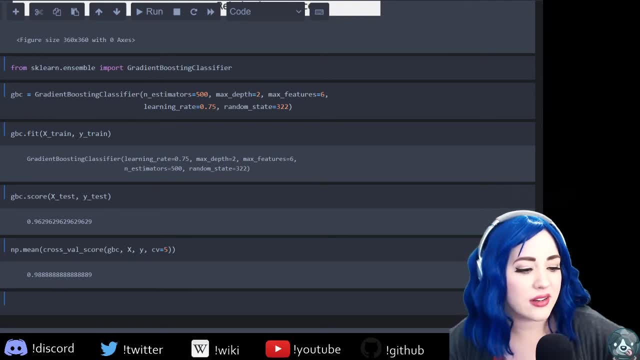 with pre-trained weights or something Like. I'm trying to figure out how to do that well enough, Cause I really like to show each step so that everybody can learn from it. But with CV, like, the training time will kind of sucks And let's see lots of people. 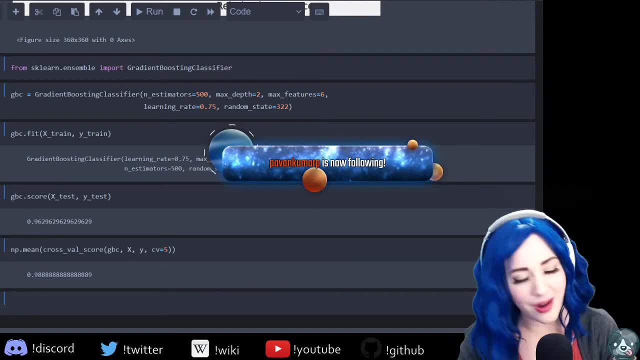 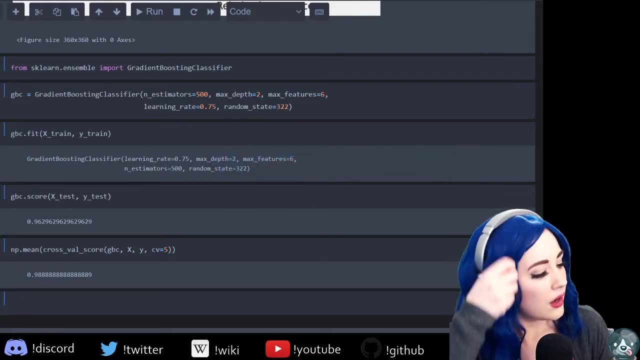 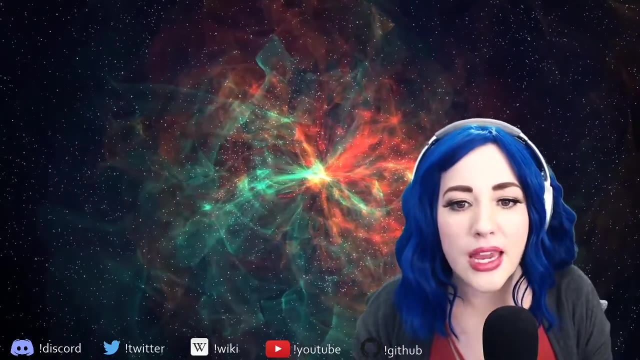 Everyone wants to hang out and Q&A. Okay, so, Pavan Kumar, thank you. Thank you so much for following, So we'll hang out. Let's see here. I will go into our just chatting here And did I set that up right? 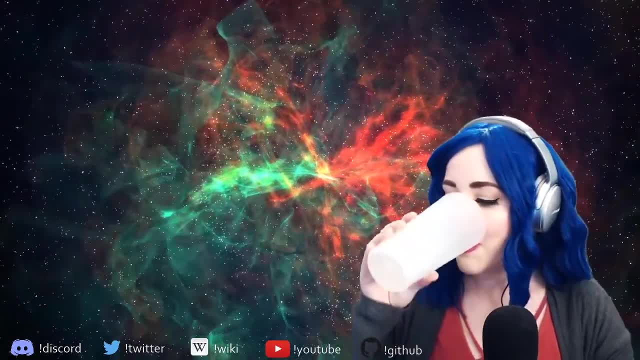 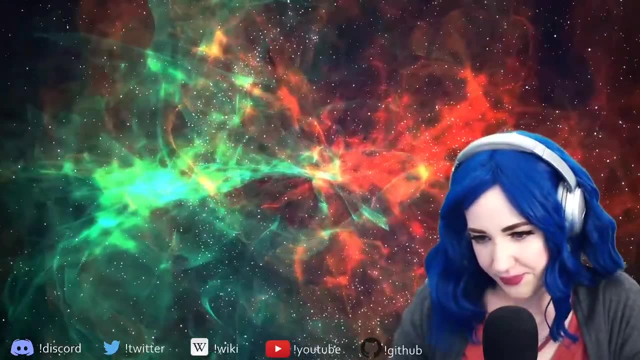 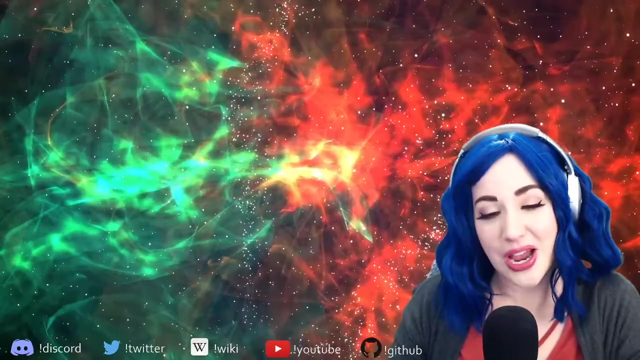 Yes, I did. Okay, So we'll just hang out and we can talk questions. And let's see here: Kevin, you say you think you'll start with an NLP chat bot stream. Yes, I would love that. Like I'd love to build a chat bot. 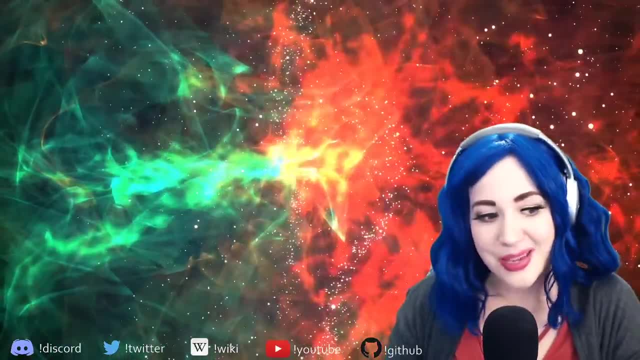 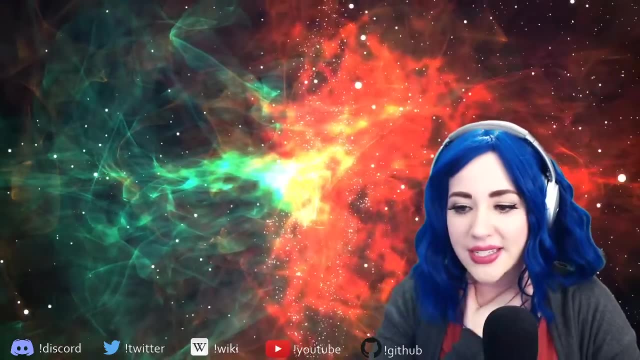 I've done some NLP, but it'd be cool. It'd be cool to see a chat bot, for sure, And Jay Shady, so maybe I could do it on a smaller data set, just to show techniques, Yeah, so I'd have to kind of do like a. 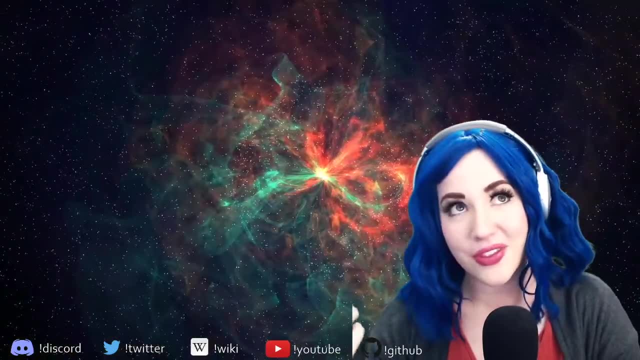 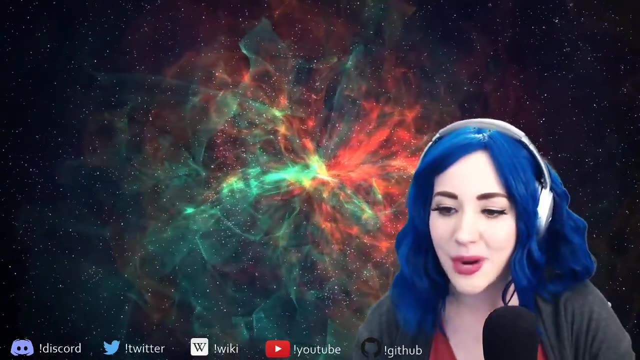 not like a content warning, but like a. I'd have to preface it with telling people that this was not gonna be indicative of full performance, But- and let's see, Strawberry Jesus, you say a deeper dive into dimensionality reduction. 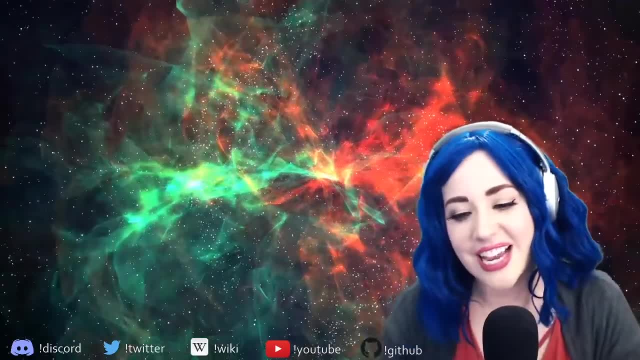 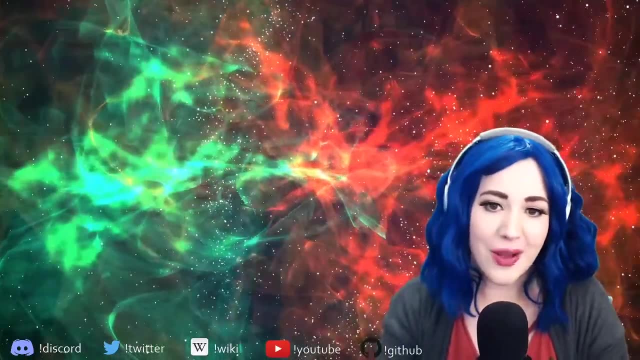 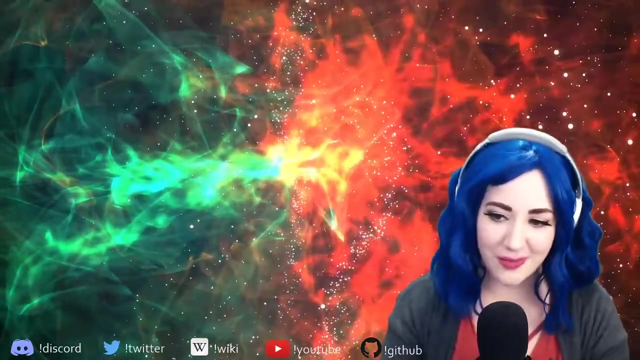 So yeah, so the previous stream for the fundamentals of data science was dimensionality reduction, but we focused on PCA, So I could definitely look, do a deeper dive into more dimensionality reduction methods. And I am Scoots, you ask: why are ants immune to COVID? 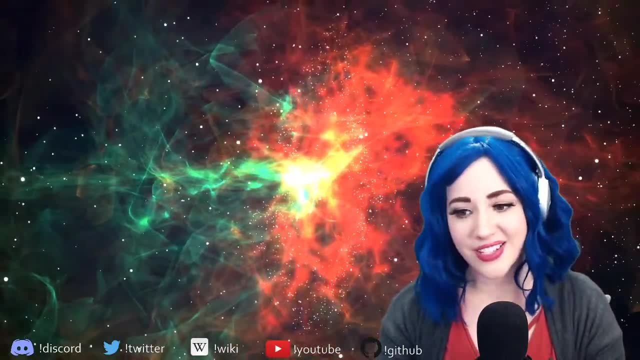 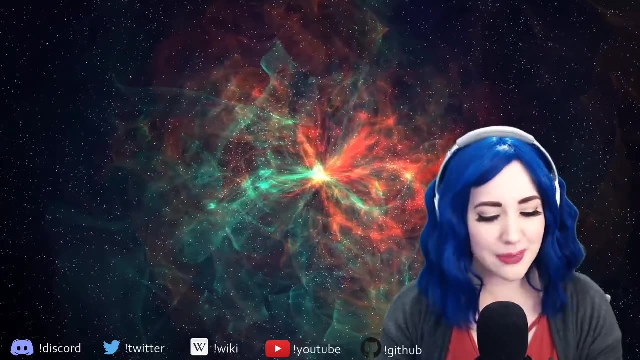 Friends, I am not a biologist, but I am a scientist. I'm guessing that they lack, like like the proteins or whatever, right, Cause it's a protein spike that they did for the N-line. See, I don't know. 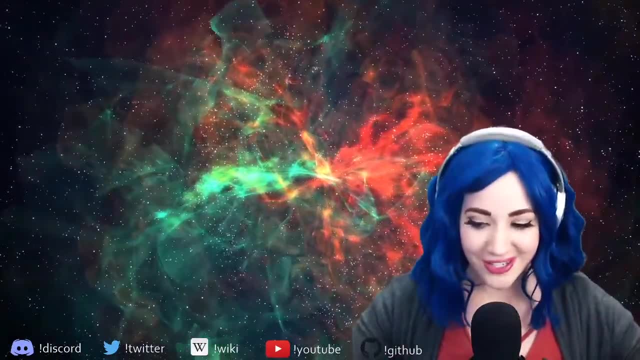 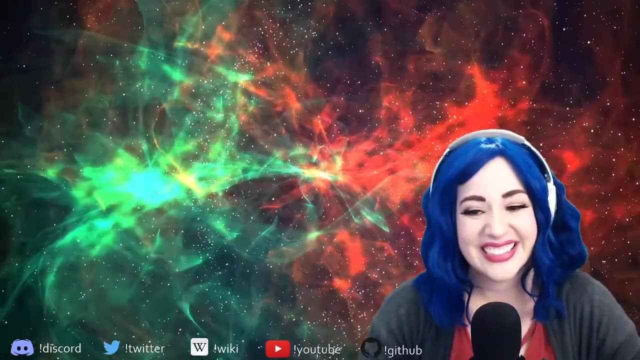 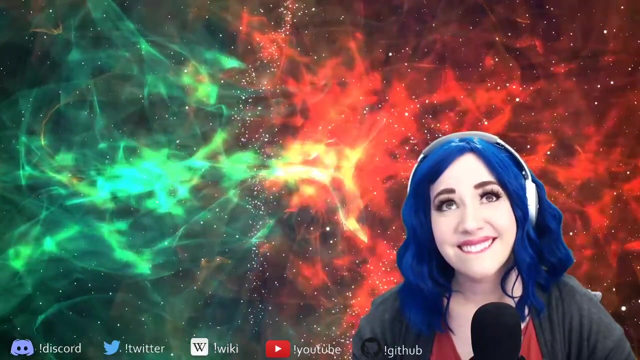 All right, I like I'm an emergency medical professional, but like pre-hospital medical provider, but like I'm not a, they have tiny antibodies. Oh my God, It was a pun. I love that so much. I love that so much. 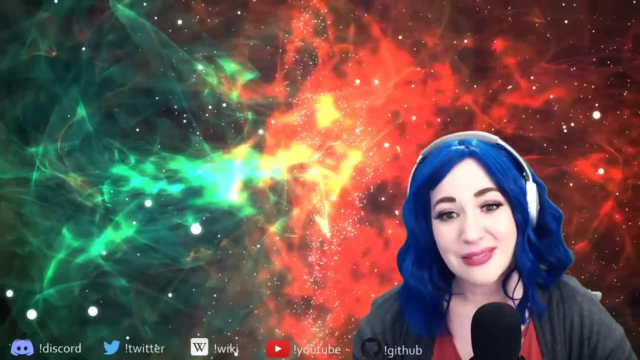 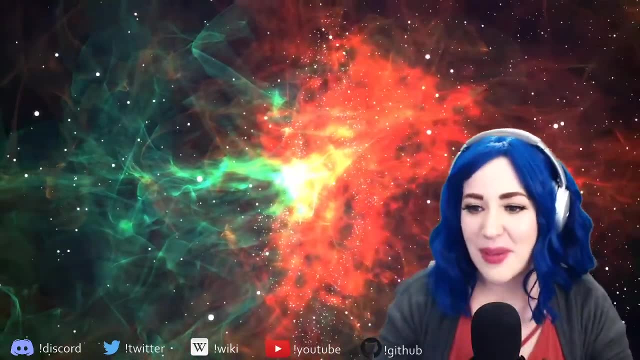 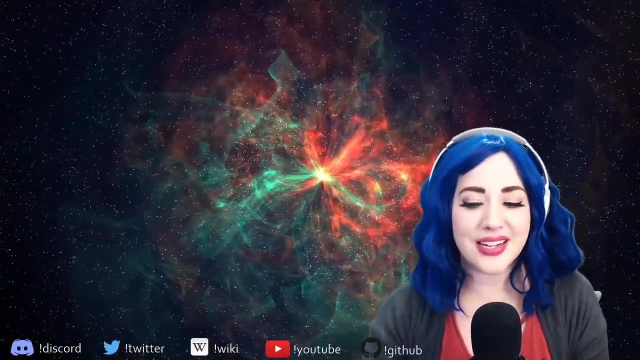 I love that so much I'm going to steal this and tell it to my dad and claim it as my own. Thank you, Yes, Okay, And Pale Oracle, you say you got inspired to revise your Pomodoro schedule and put more effort into supplementary studies. 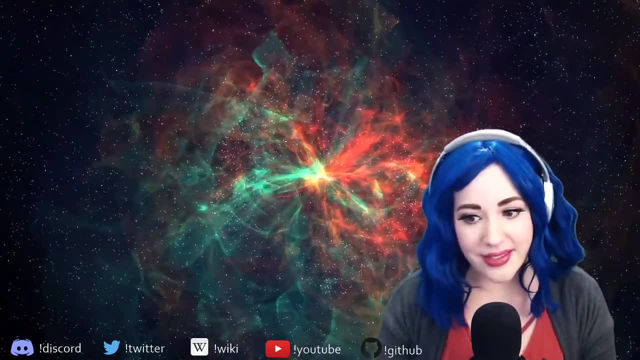 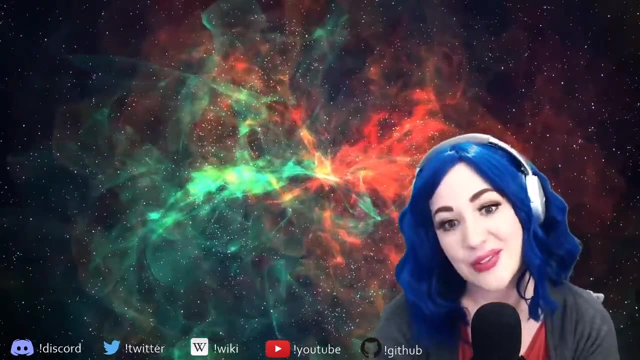 Well, one of the things I've been playing around with is doing some Pomodoro streams together. So, especially for days when, like I really need to be productive, I've been toying with the idea. I did one and it was like moderately successful. 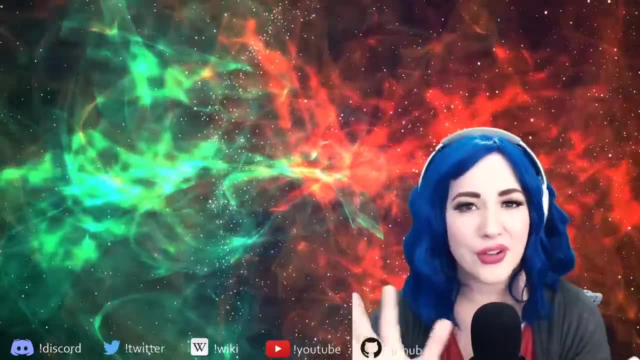 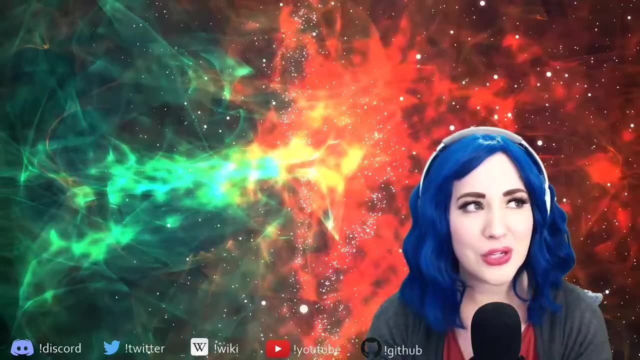 So it had about like two thirds to half the normal folks that I have show up but doing kind of like a coworking stream. So we do Pomodoros, We work for 45 minutes, We hang out for 15 minutes, but we can all be productive. 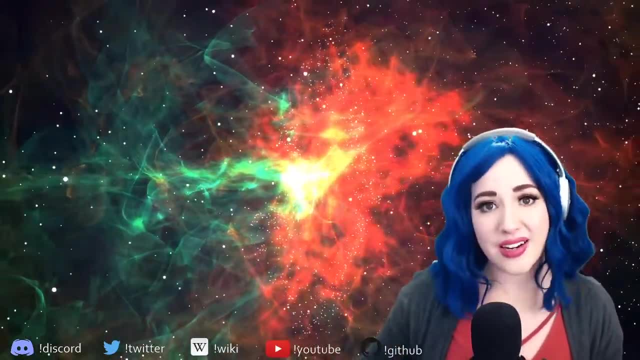 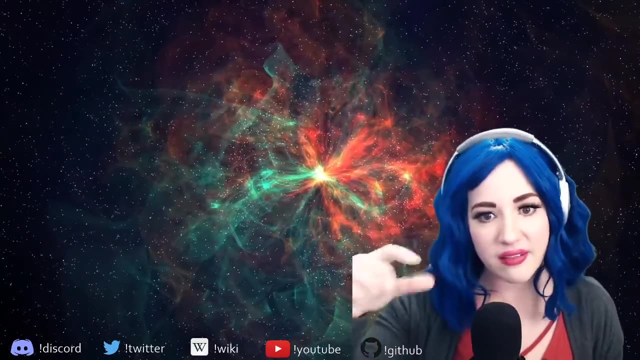 One of the things I really want to do- All right, I have zero fricking idea how to do this- is I want to do for the coworking stream a way that people can submit like what they want to accomplish in that Pomodoro segment. 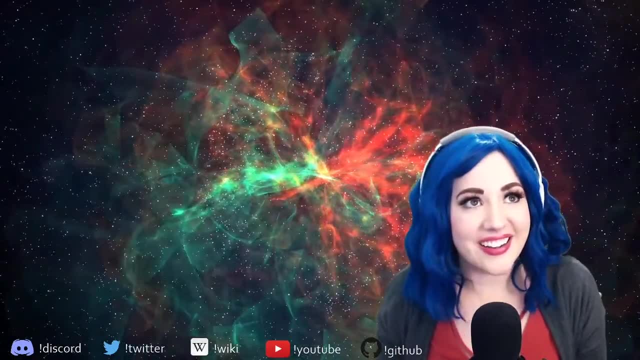 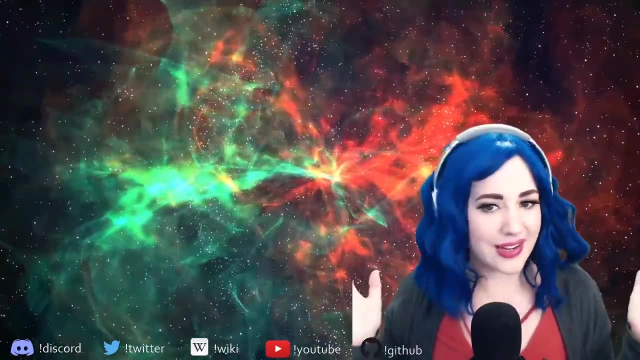 Right, And then people can like they can get like a I don't know like for words or like we can have like a leaderboard of people who are accomplishing like awesome things. So like I have no idea how to do this myself. 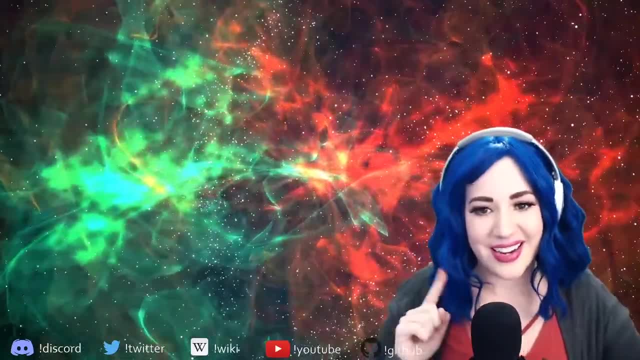 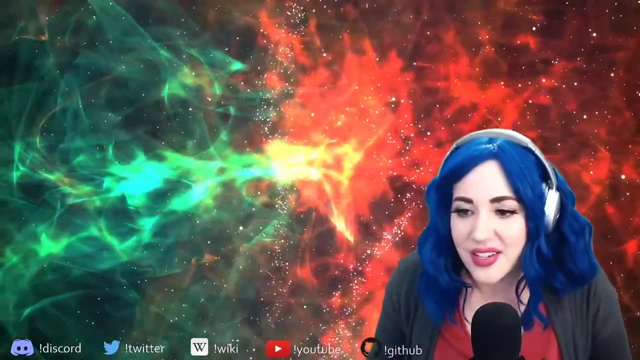 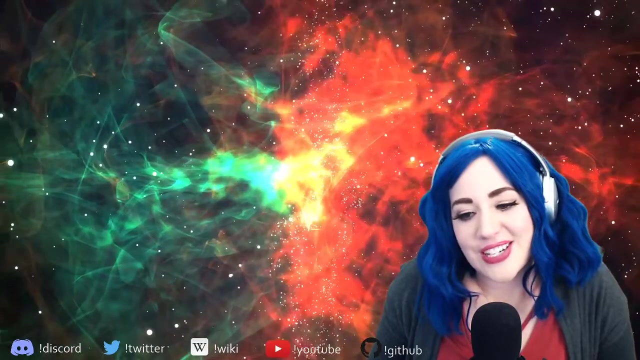 Okay, Jay Shady, say there's a bot for that. Like, hit me up, friend, Cause I want to know. and Loaf Bone, Ouch, Yeah, My aunt isn't immune to COVID truth. And what is your favorite? Ah, you say I love a good dad joke. 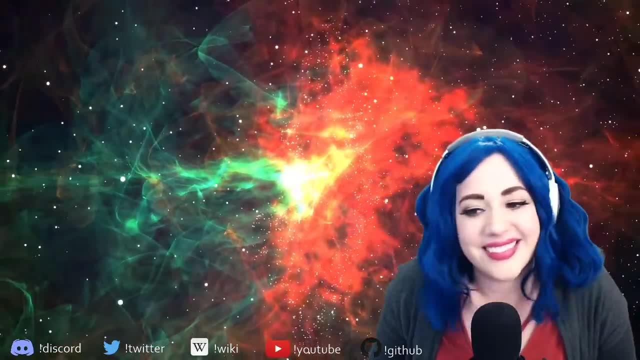 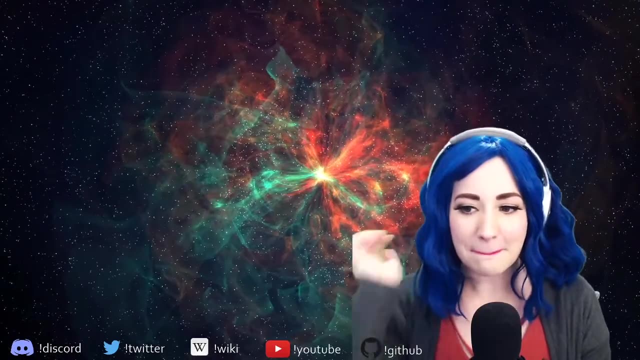 but I myself I'm not a dad, I'm with the French, call a faux paw. Huh, Hilarious. And oh, you say you like Jay Shady. You say like coworking stream, So awesome Okay. 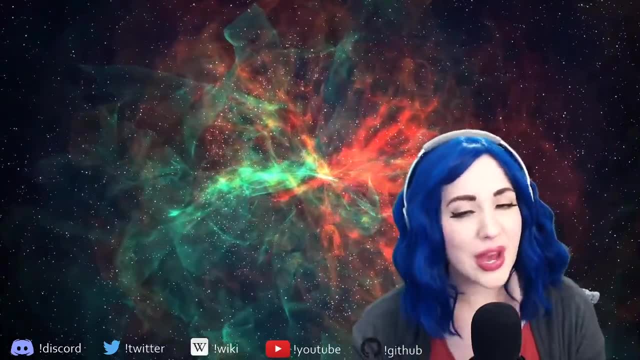 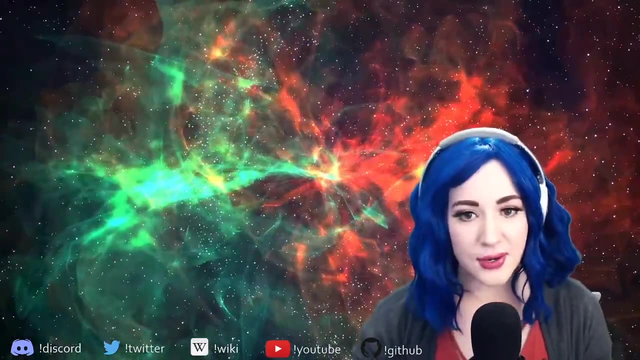 I usually don't do Pomodoros myself, So they help lots of folks with ADHD. But for me, one of the things that I've noticed is that like I'll get in the zone right as the Pomodoro ends, So it'll take me like half an hour. 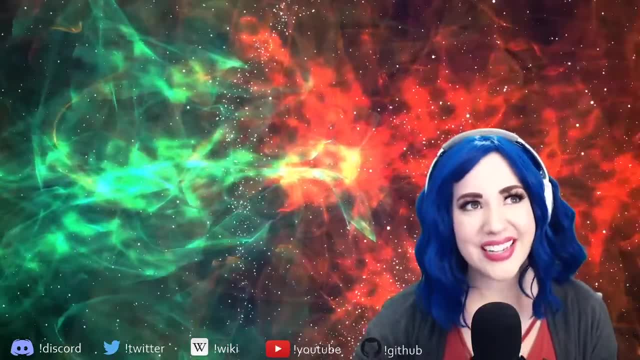 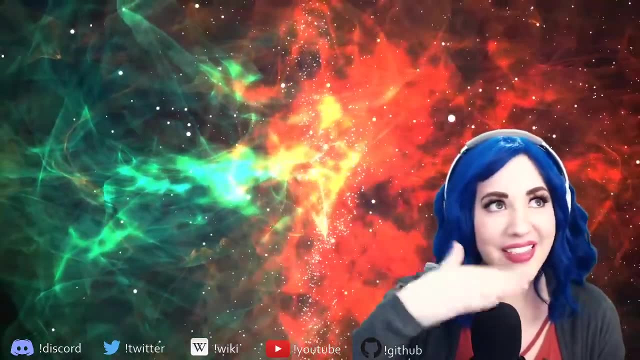 to get into like the focus zone, And then I, then it's time to take a break, And then I'm like distracted for 15 minutes And then I go back to it And by then I've like lost my distraction. So I, but I've, I've, 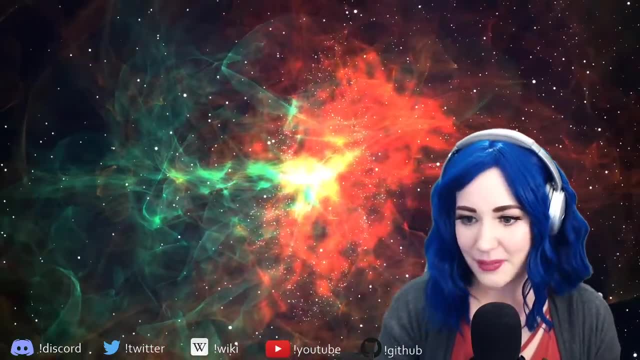 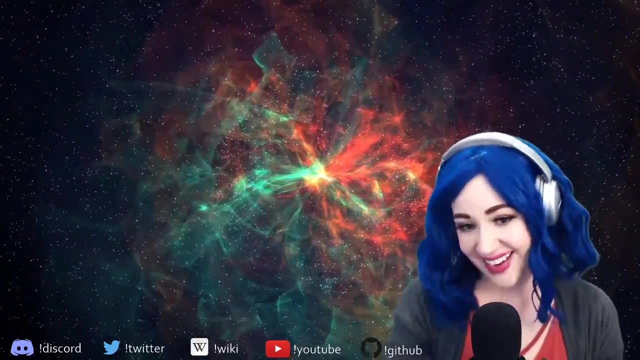 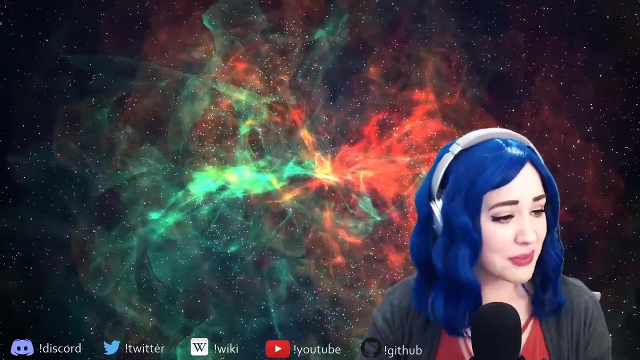 I've enjoyed doing the coworking streams for sure, And Guzco do. I like web development, I appreciate web development. I do not know it And it's. it's not so much for me, but 80% people said hang out and Q&A good. 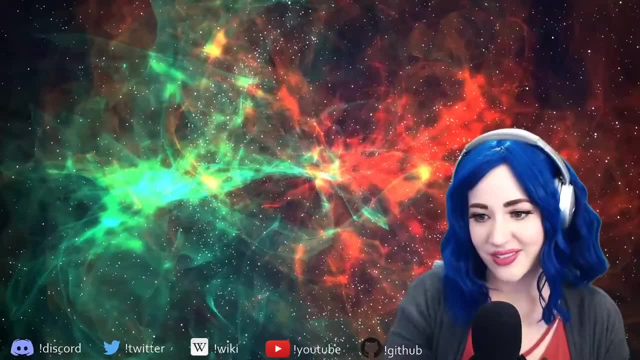 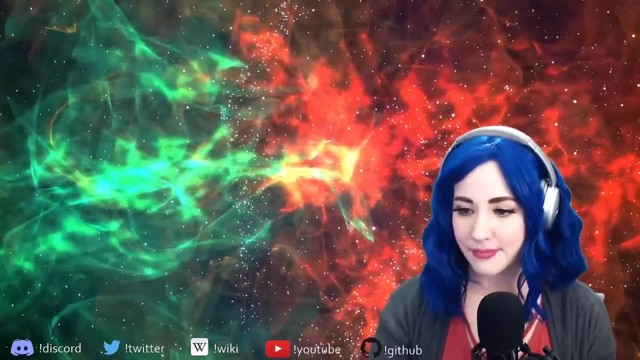 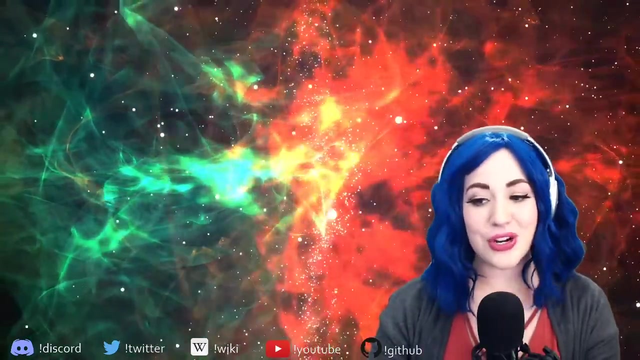 So like no one wasn't this massive like change. but I don't do web development myself, but it is important and I appreciate good web developers. And let's see pale oracle. You say it's always good to have other people to continue the journey with. 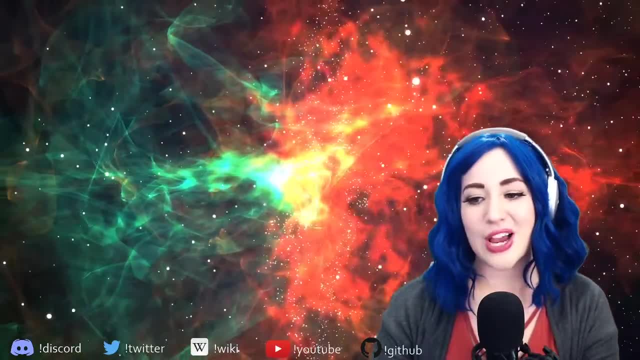 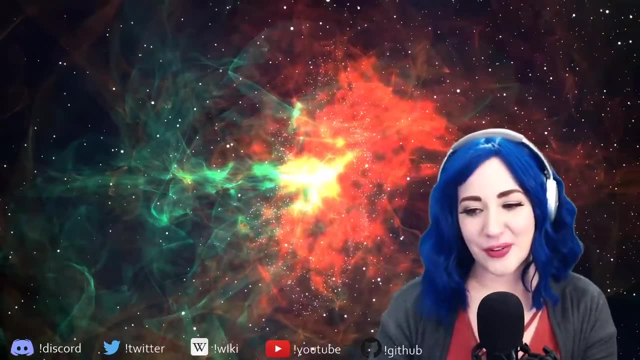 I've thought about doing something in discord but haven't gotten around to it. How many times in life have I said this: Oh, truth, truth. There are so many wonderful plans I have. If only I got got around to it, but alas. 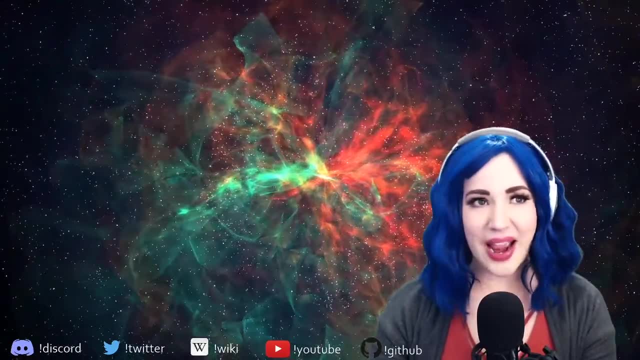 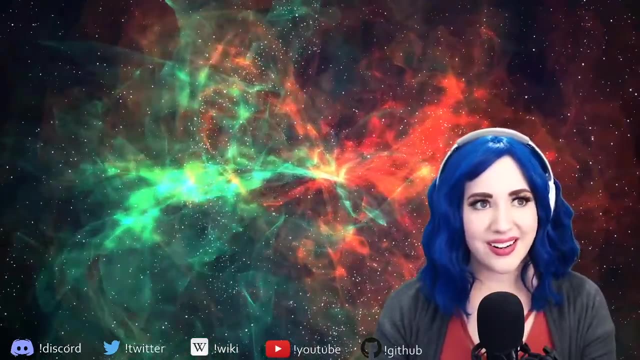 I haven't gotten around to it. I also I have this. I have this deep character flaw which is I just can't say no to people when they have cool projects. So I overextend myself incessantly because people have cool projects. 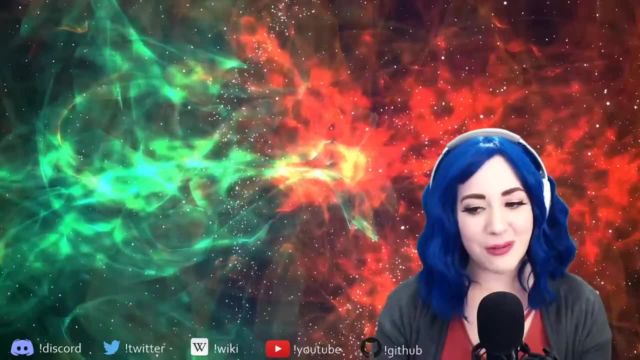 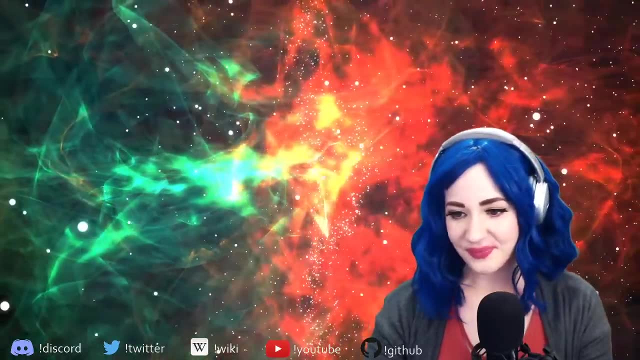 I'm like I want to do that Or I get all these project ideas and I have trouble like sticking with it. So it's an ongoing challenge. I'm working on it. Let's see Starby Jesus. you ask: how do you manage ADHD and off med days? 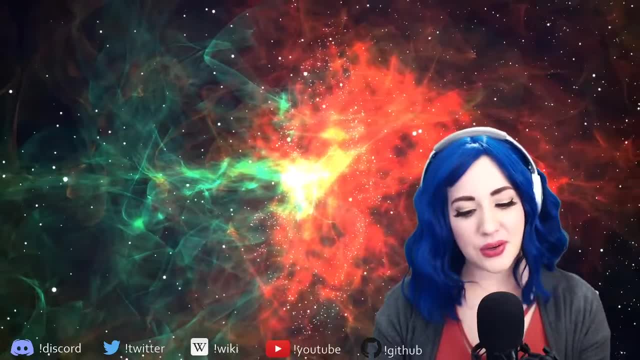 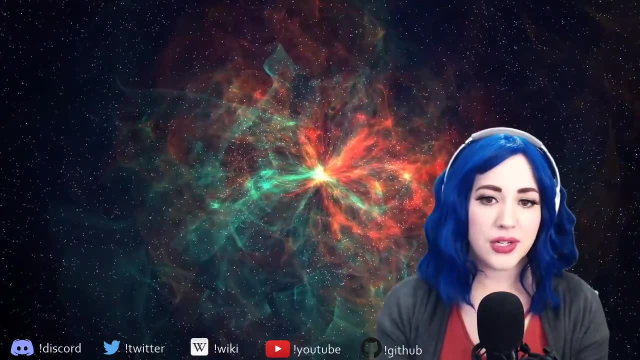 So caffeine? not because it gives me energy, but so folks with ADHD, our brain chemistry is different and we will have a paradoxical response to caffeine. So instead of it being a stimulant, where it like wakes you up, gets you jazzed, it actually like slows the brain. 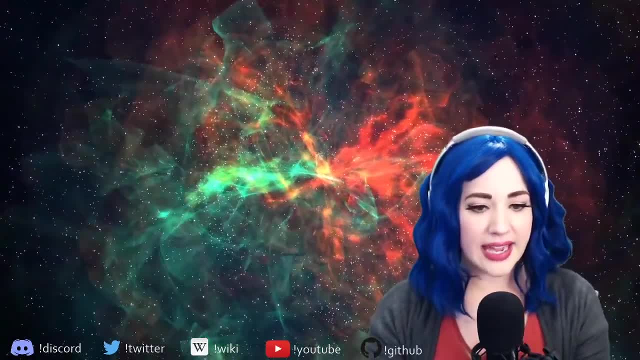 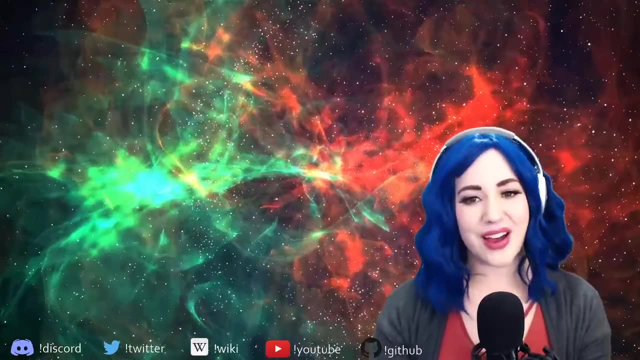 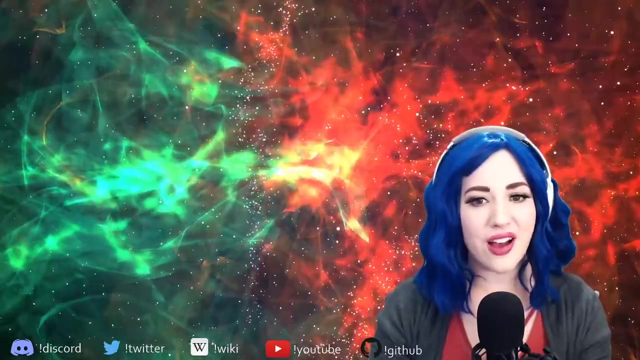 and calms down, So caffeine and also kind of like use of like Pavlovian response to music. So I've got music that helps me focus and tricking my brain, So I'll be like it's okay. We're going to have like Netflix on and a stream on. 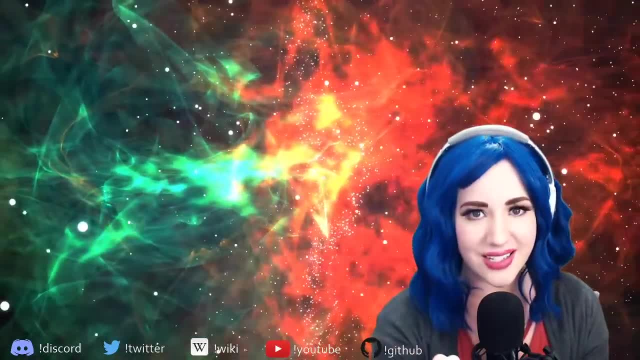 and then you can start the thing And it distracts my brain long enough to get sucked into the thing I have to do, And then I'm like, oh, what's all this noise? And I turn it off and I'm able to focus. 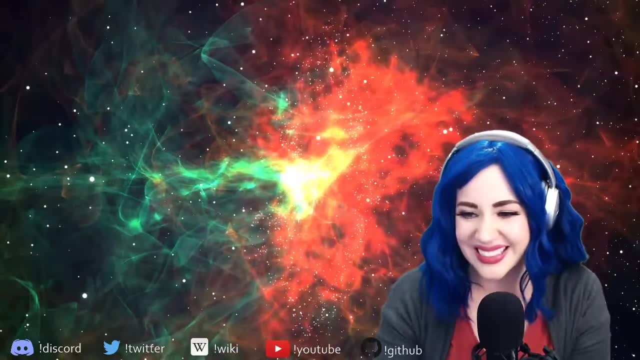 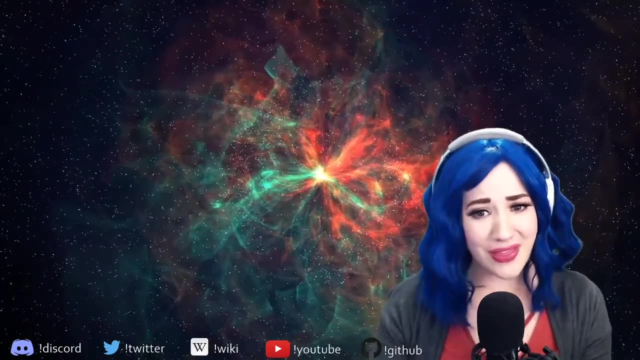 So a little bit, a little bit of some some tricking my brain. But to stay organized I use a bullet journal. So not like I don't follow the methodology a hundred percent or anything, but I writing things down helps for sure. 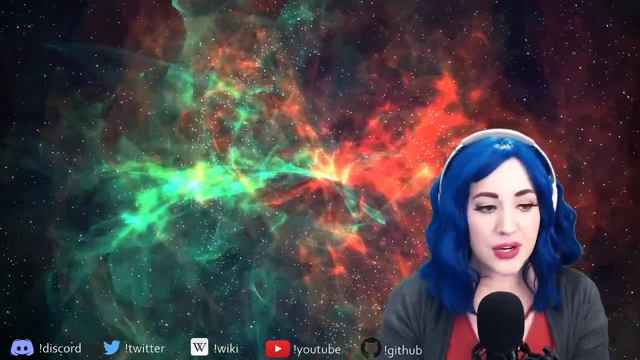 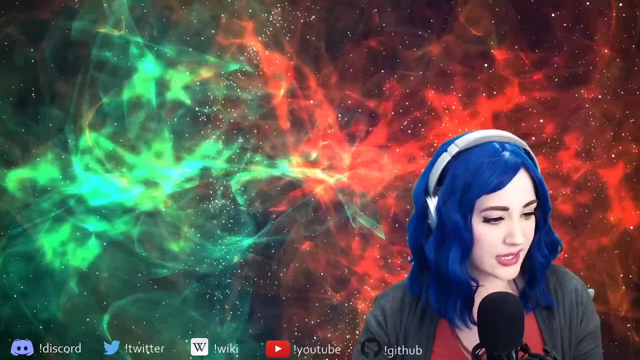 And Troy DF. you asked if I work in data science. So I work more in machine learning than data science, So I work as a machine learning developer. Okay, And I'm sorry, whiskery aunt, I just saw your message. Ooh, thank you for sending me this paper. 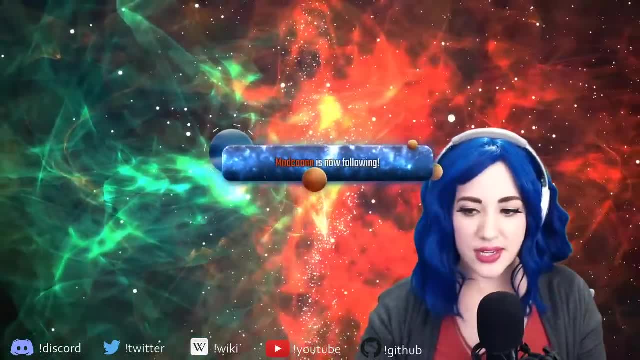 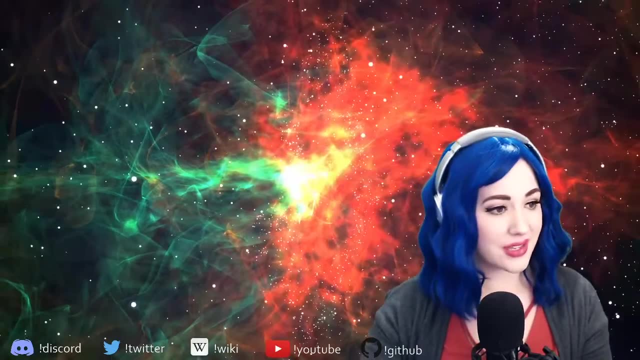 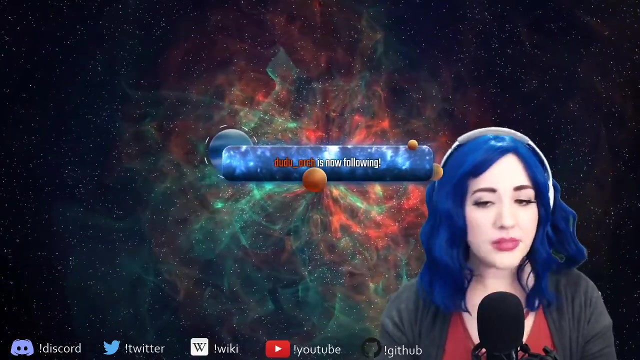 I will post this in in chat So for people interested, I think, Strawberry Jesus, this will be a great paper for you- The behavior of distance metrics and high dimensional space. And for folks new, don't worry if that seems like overwhelming. but we talked about dimensionality reduction. 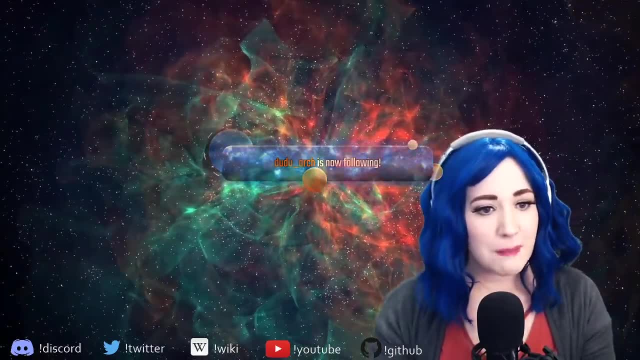 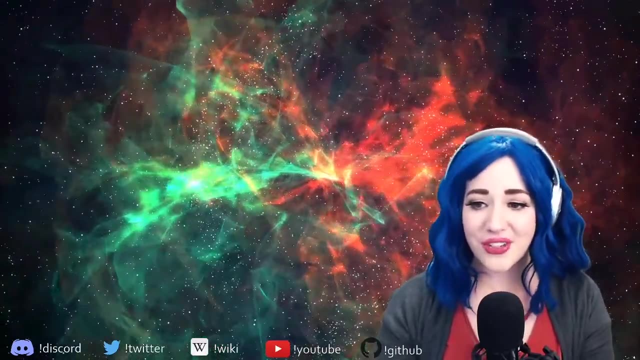 and the curse of dimensionality on a previous stream, Madcon and Dudu Arch. thank you for following, But let's see here. Oh, no, worries, Carlos of Gingerfell, have a good sleep. I'm so glad you enjoyed yourself. 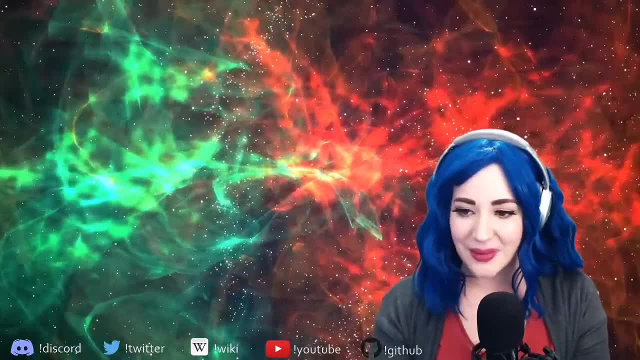 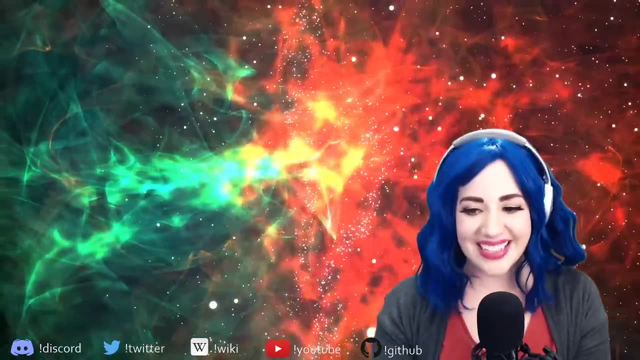 Hopefully I'll see you. I'll see you here again. And third tier, gaming. You say you're watching three streams YouTube and doing a 3D print right now. Yeah, And C films: I don't know R. I don't know R. 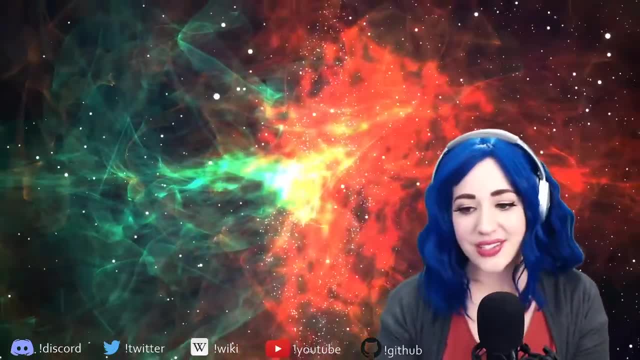 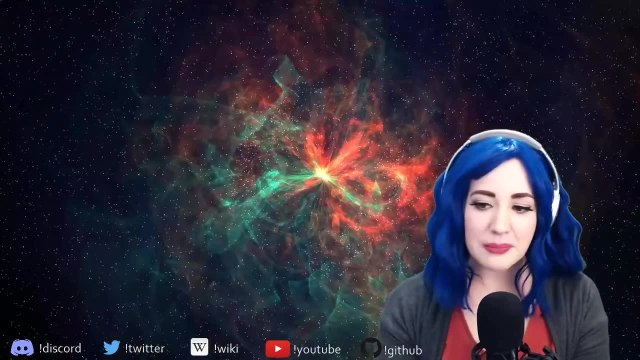 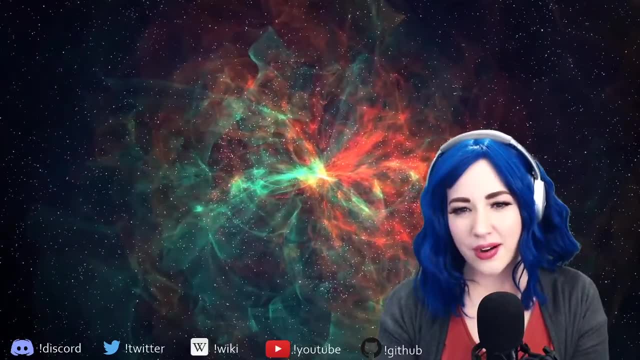 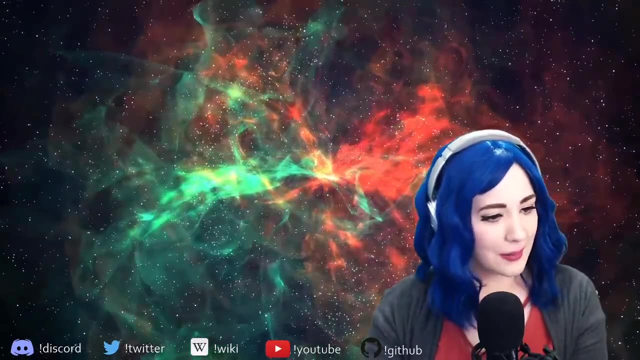 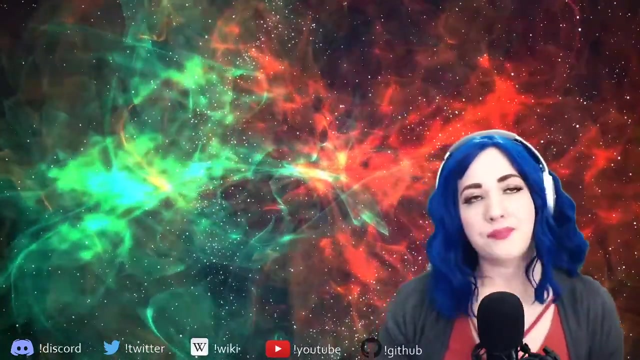 So like I've heard jobs to be like, it's okay if you know R, but we prefer Python. So but no, no, no, no R for me. Let's see here What do I like and dislike about Python. 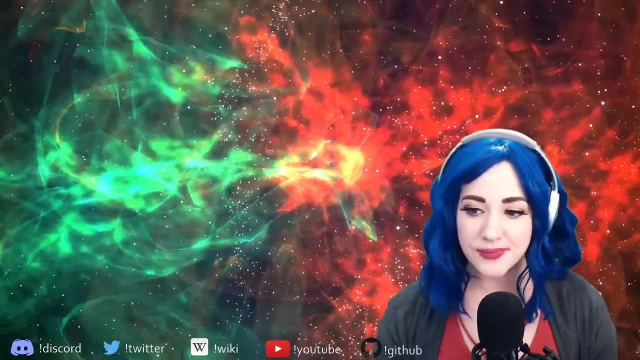 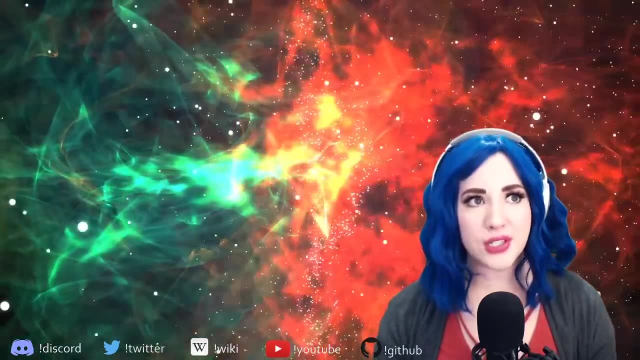 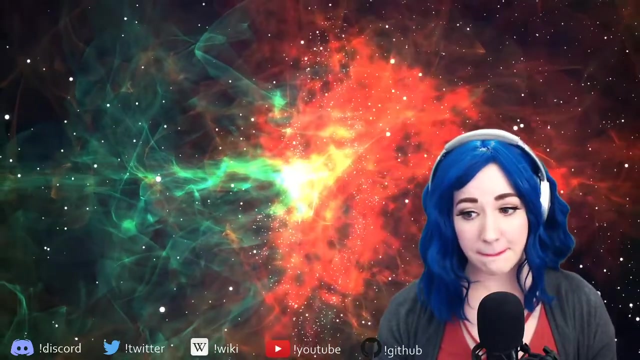 Okay. I like that it's really accessible, So it has a readable syntax and it. I feel like it's very- I feel like it's very good for people getting started with using their first language. It's a great start. I like that it has a lot of libraries for machine learning. 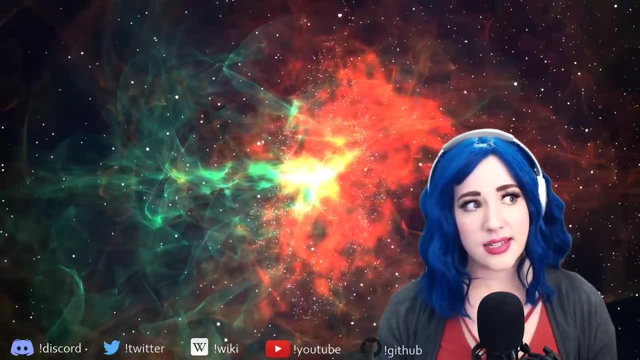 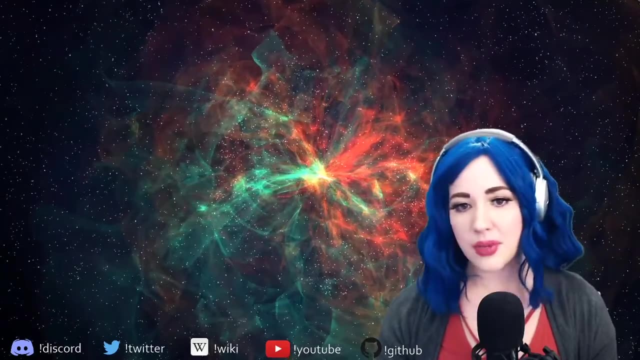 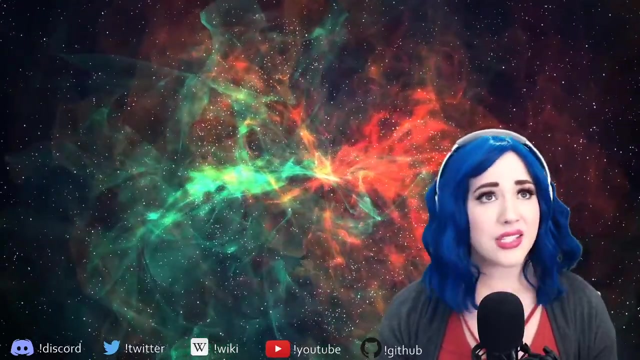 And I like that, like a lot of those libraries, have really good documentation and that you know there's a whole community of people using Python. It's very common, So it means that there's lots of stuff out there for getting help, lots of like resources for people learning. 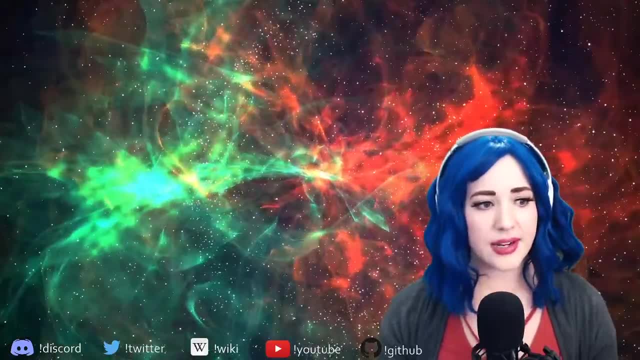 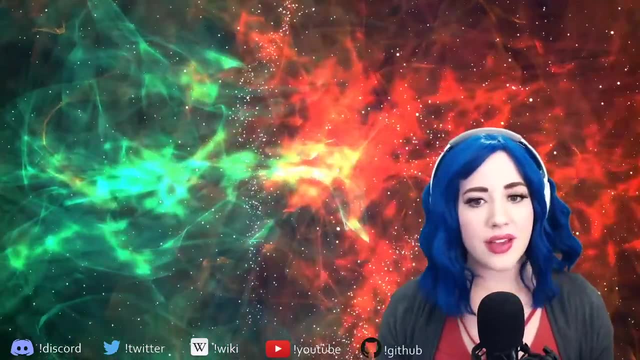 Things I don't like. Things I don't like about it is that there's a lot that happens under the hood, So especially like it's great when you're getting started and there's people who use it like I use it for work right. 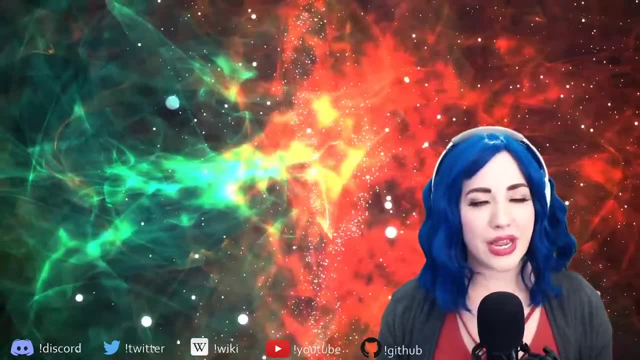 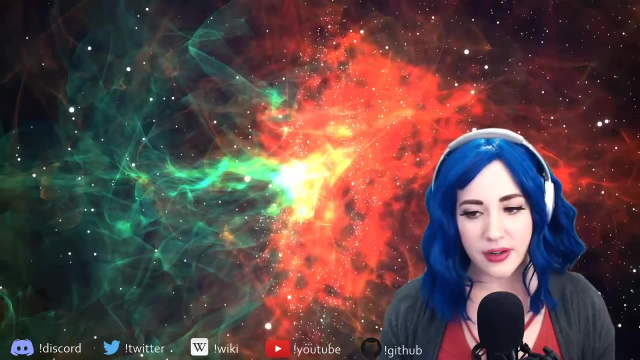 It's great, But I found that if that was the only programming language I learned, like I'd be missing a lot, a lot like Python does a lot for you and it doesn't tell you about it. So I feel a lot better now using Python, that I've gone off. 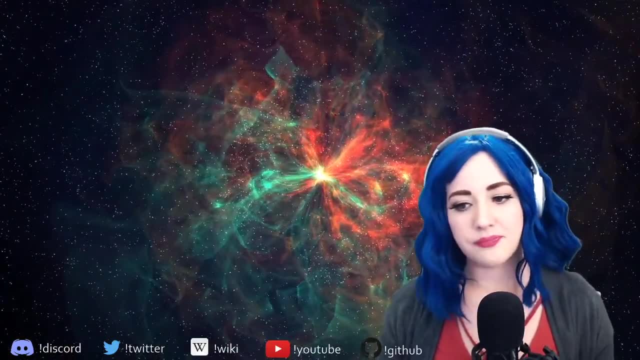 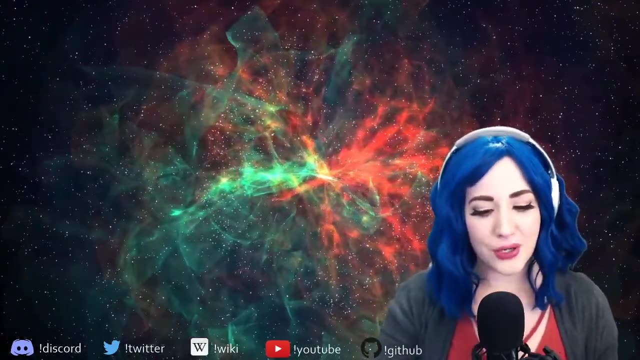 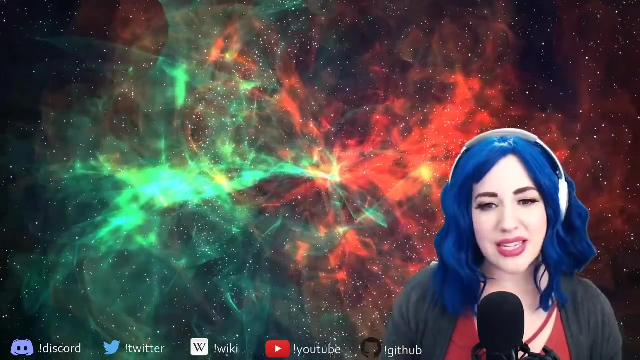 and I've done more kind of like lower level languages And I like I feel more comfortable using Python now. So it's like it's a great, a great thing to get started, But then, once you hit a certain level, it's almost like it becomes dangerous. 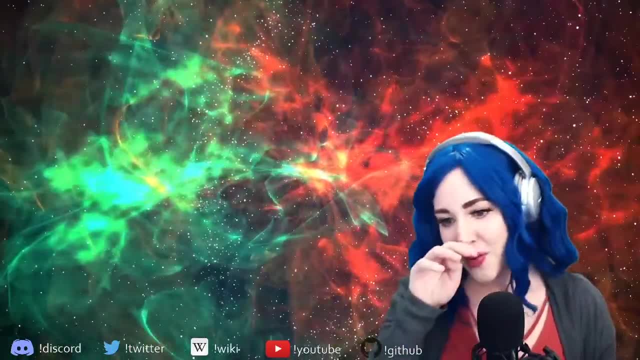 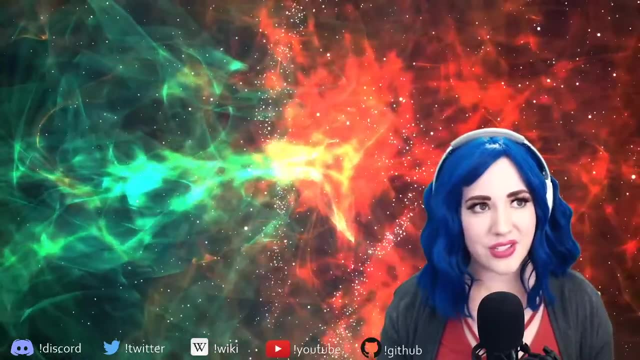 not knowing the things that Python does for you- And I know Enigma Dev- like white spaces, syntax, whatever, Like that kind of stuff doesn't bother me, Like people can argue about spaces and tabs And I feel like it's just lots of ways. 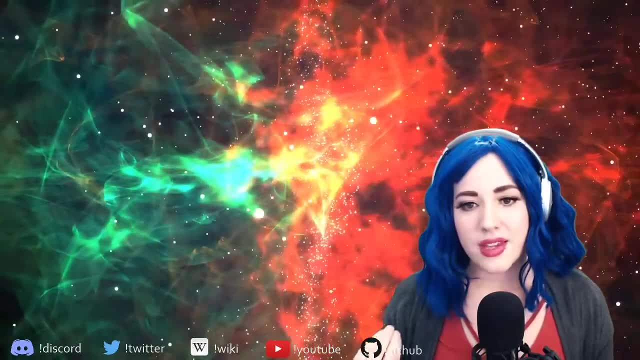 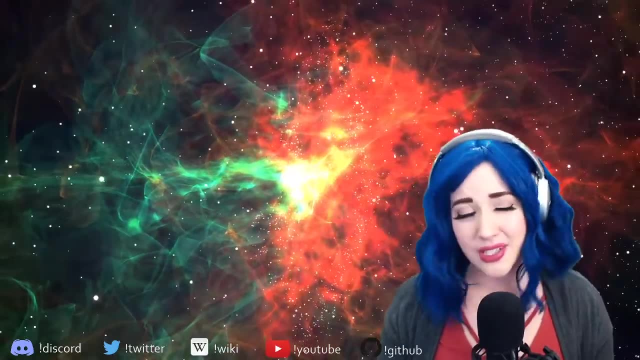 for people to feel important, but it also can be really like, especially when you're dealing, like, with high, high volume optimization problems, Python can get slow, Even if you're doing your best to like optimize as good, like as well as possible. 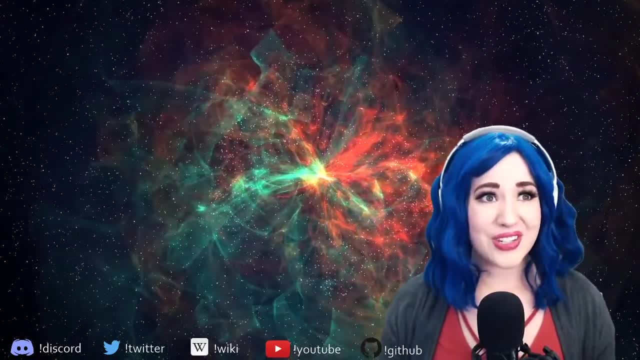 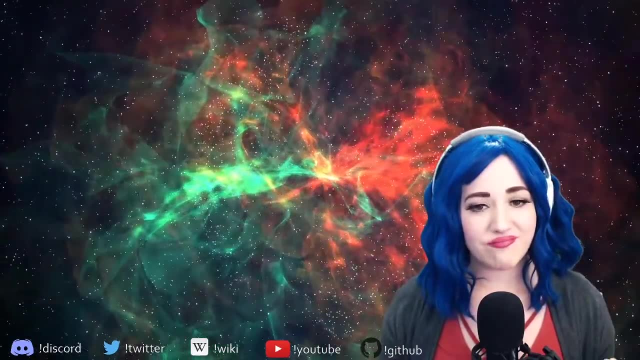 I also have found, the more that I program, that I actually maybe it's like my own preferences as a programmer, but I much prefer like statically typed languages. So and like you can do things like functions right. So, and like you can do things like functions right. 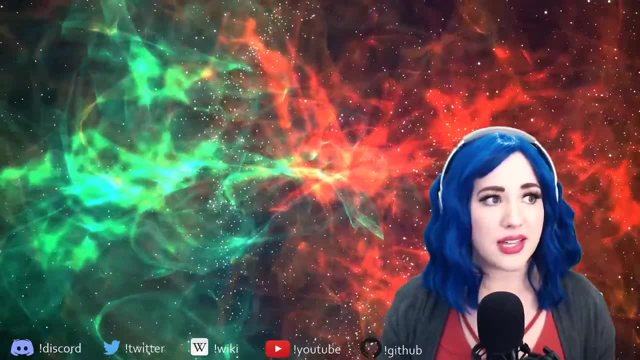 So, and like, you can do things like functions, right, You can do things like function couple or function annotation and Python. But the problem is: is that if you, you know, if I? But the problem is, is that if you, you know, if I? 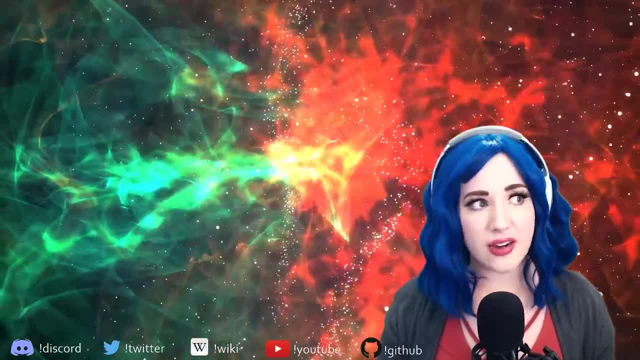 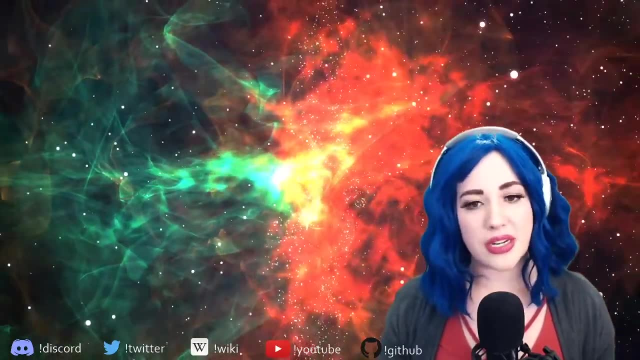 if I have, like this wonderful function that I've annotated, if I feed it an argument or a parameter that is not the type I've specified, it doesn't throw an error. So, like you, as the developer, need to put those like checks in. so I 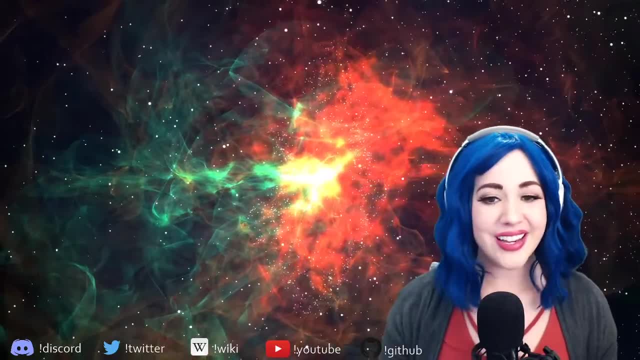 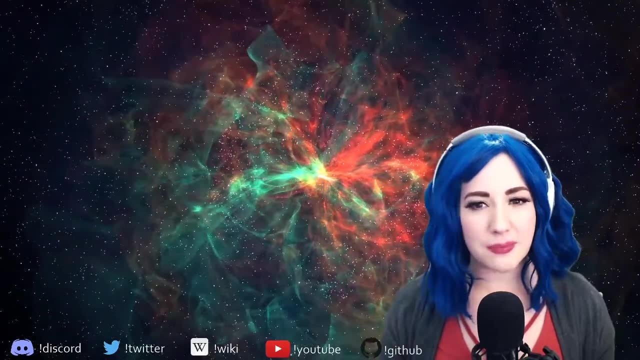 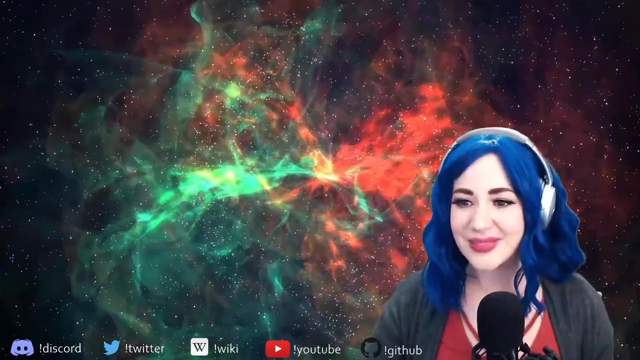 so I as much as it has. there was a challenge to learn. at first I've liked static typing quite a bit because it it forced me to be a lot more explicit, because it it forced me to be a lot more explicit, and I also like it helps with bugs like I don't know, um, but so, but again like a programming. 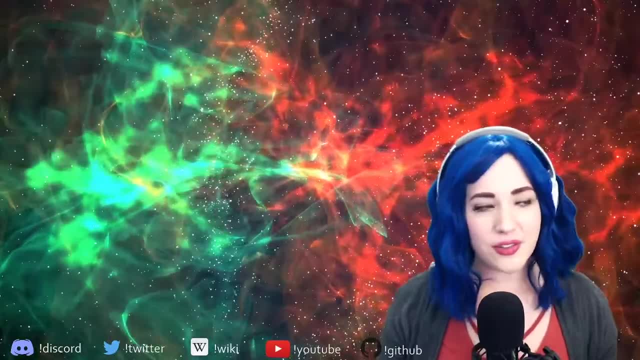 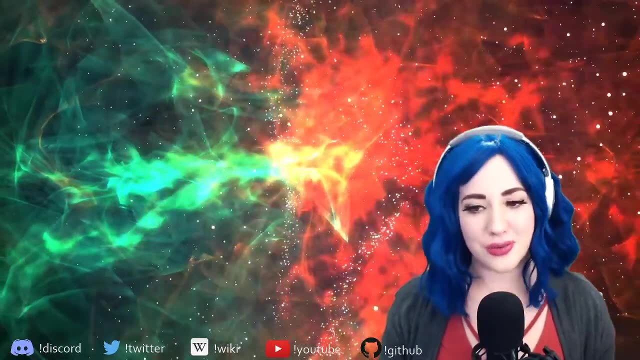 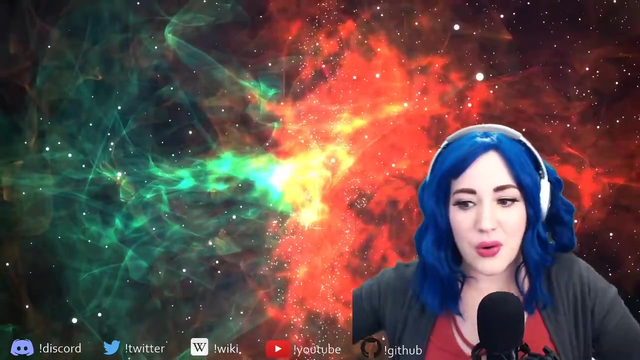 language is a tool and just like there's so many different kinds of people, there's lots of different kinds of programming languages. one isn't just inherently better than another. this is a tool that you're able to use, and whatever works for you, whatever you like, is totally fine. so I a hacker. 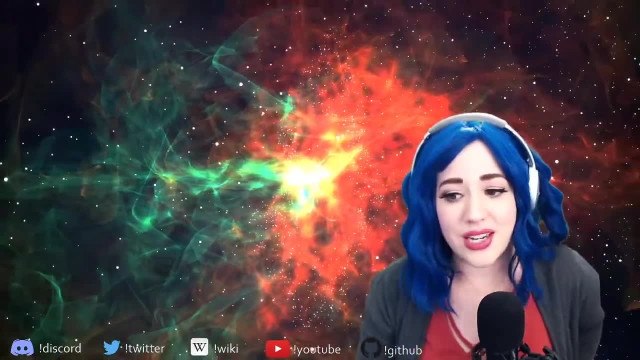 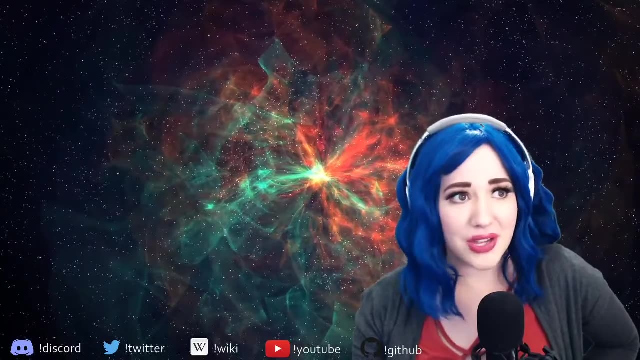 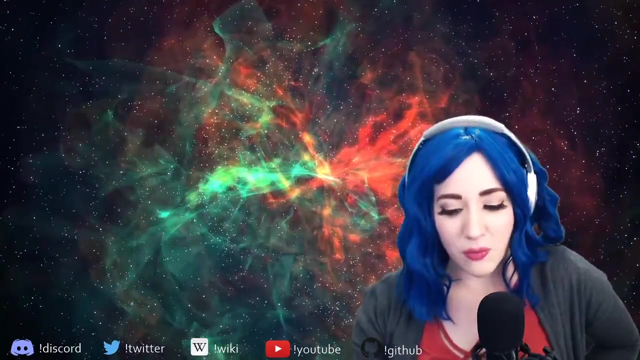 I I recommend Python to anyone interested in getting started with programming. I do, and if I am trying to just like sketch something out, it's still the language that I feel the most comfortable in and I think it is one of the most accessible programming languages. it has so many more tools. 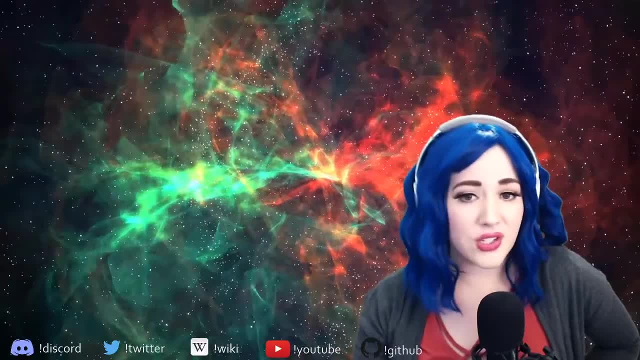 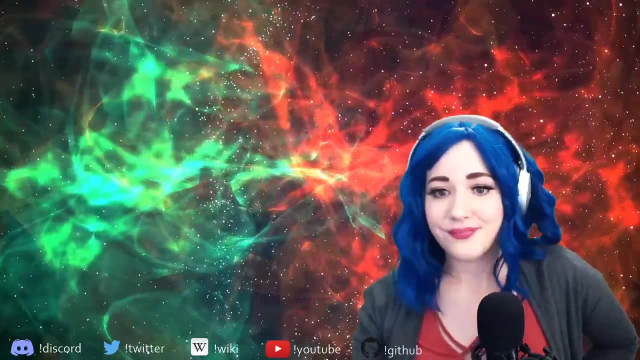 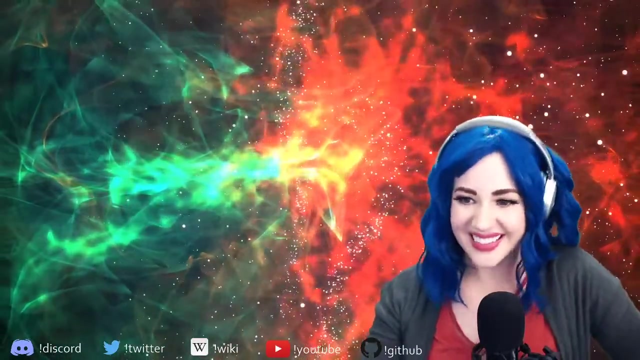 than any other language that I've learned, at least for getting started, for learning, for having interactive kind of like education sessions. so I don't know. it's great. it's got lots of things to love about it. I don't dislike it. I use it every day. um, and let's see. 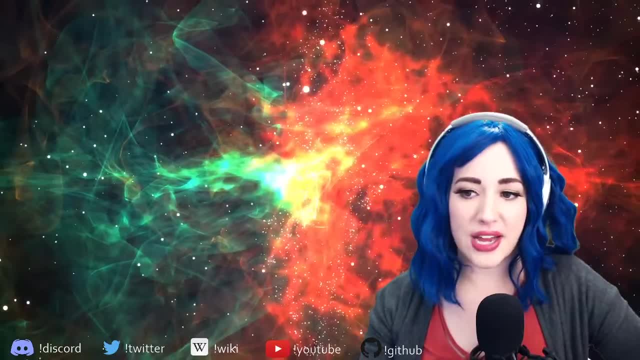 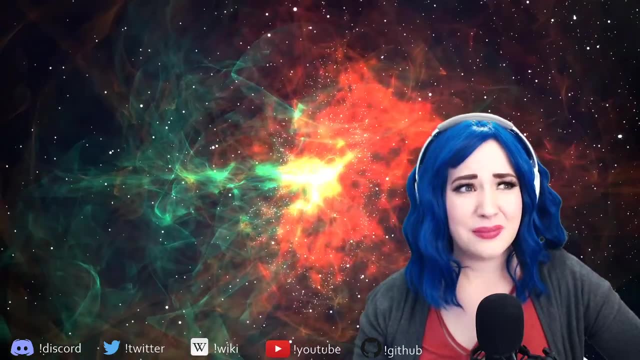 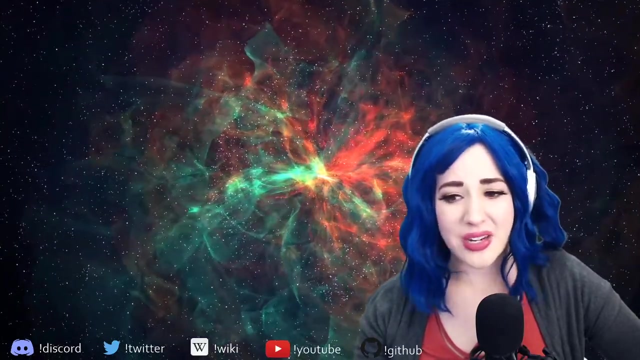 and jshady. you can make more efficient code if you know the data structures and algorithms. yes and no. yes, but like the way that we beat people over the head with it and the like arbitrary, random, just divorced from reality way that it's taught is not helpful. so there are a lot of 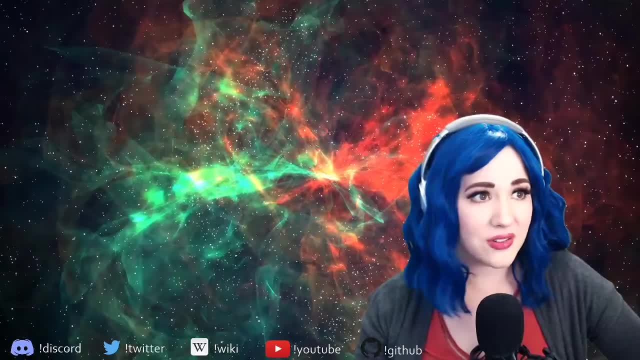 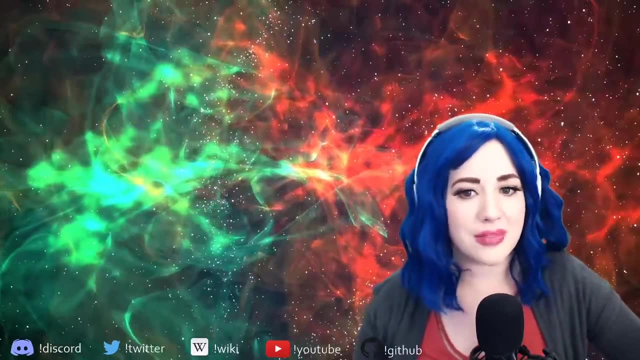 lots of, lots of developer jobs that do not need to know every single, like data structure that we talk about or all of the different algorithms, like it's okay to have an appreciation for those things, but not every job needs them. so, just because you can like, your job involves writing. 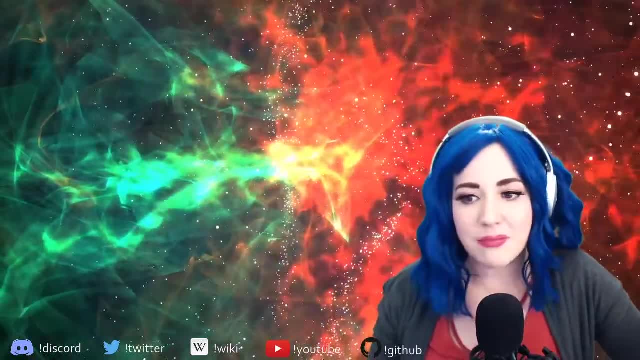 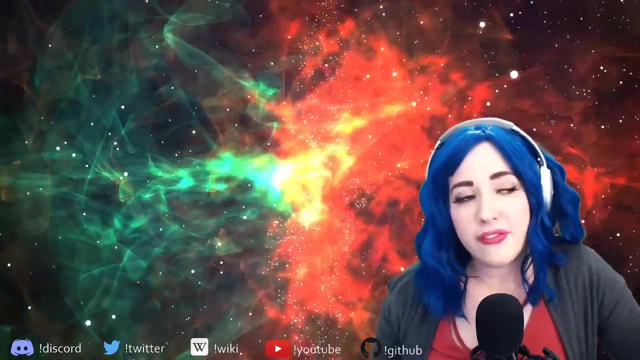 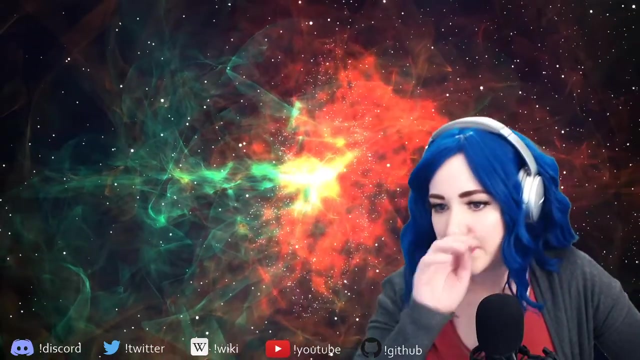 code like unpopular opinion doesn't mean that you need to know. you know a doubly linked list. but that said, for me at least it's. it's made me more intentional about what data structures I do use. so, and cactal, fractal, you say, if I was given a one year, if you're given a one year sabbatical, 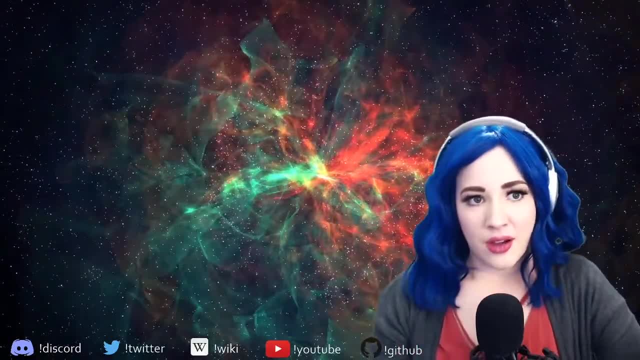 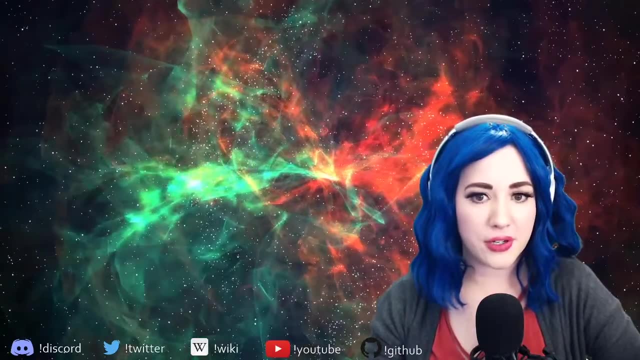 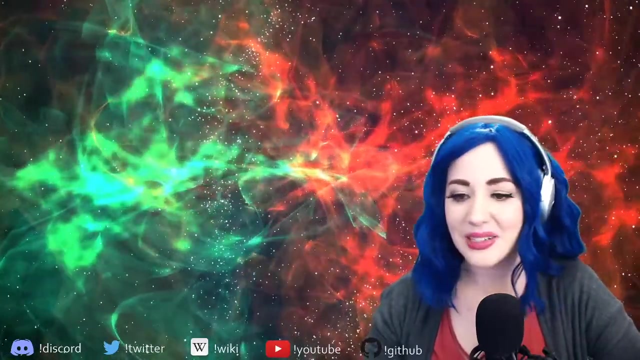 what would you do with it? stream a lot more, um, probably do a lot more educational content, write a book and have the most amazing garden ever. I like gardening, um, and see films. you ask what do I mean by a statically typed language? okay, so in python, I can type in a language and I can type in a language, and I can type in a language and I can. 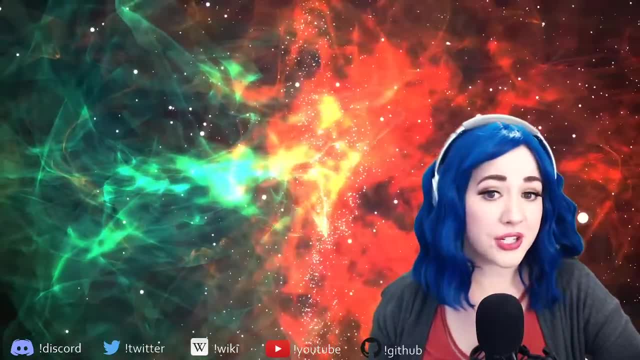 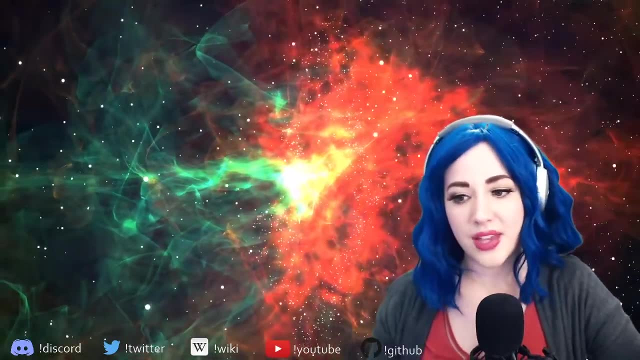 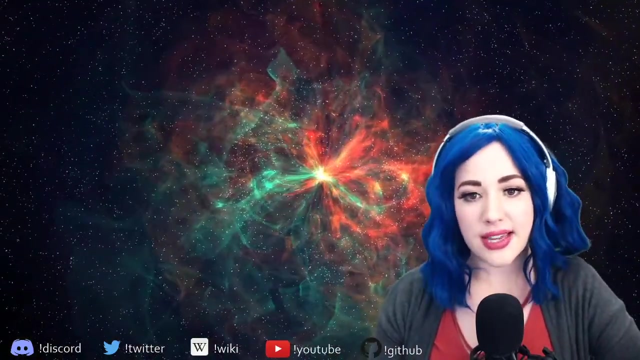 say something like x equals five, right, where five is an integer. um, I can the next line of my code. I can say: x equals in quotes, frog. it equals a string. it's dynamically typed, it will. I can change the types after I declare a variable. there are languages like c, sharp c, for example, where you: 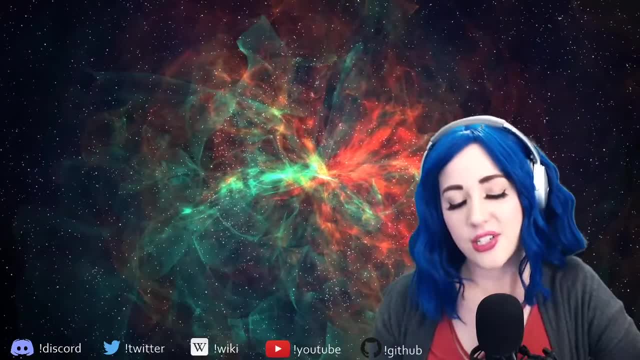 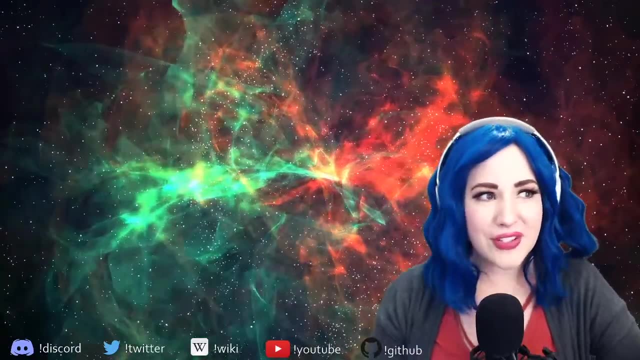 specify: x is an integer, an integer equal to five, and if I try to change it later I can't, so the thing I locks in the data type and and then I can type in a language and I can type in a language. and at first I hated it. I was like, oh, this feels really restrictive, but it actually took like it. 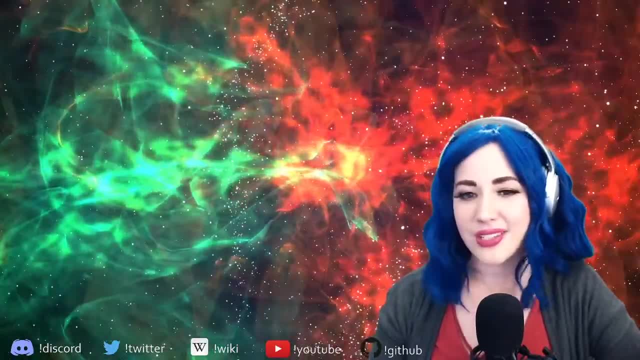 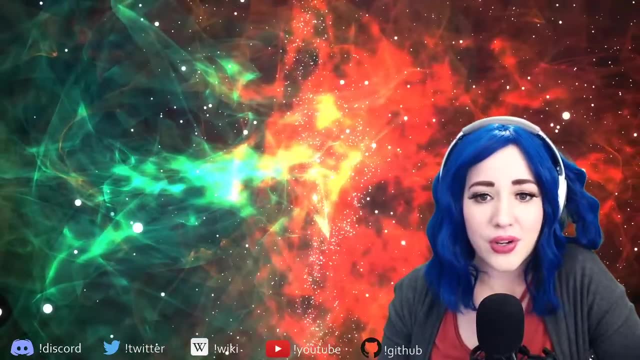 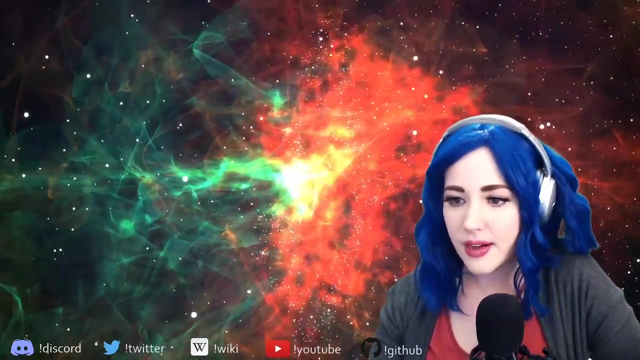 cut down a lot on the guesswork and the like bug chasing sometimes that I have to do in python, even with function annotation, and with python it just means I have to write more lines of code making like checks to make sure that things are the right data type, essentially, um. well, let's see. 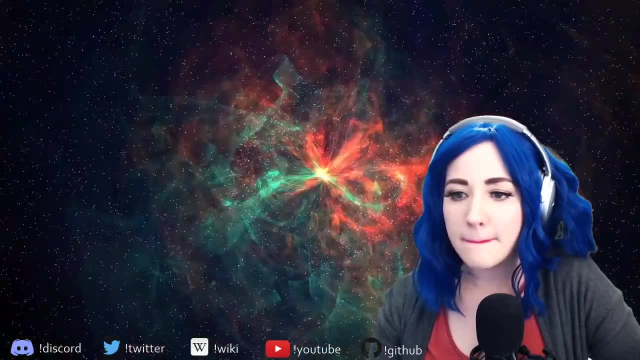 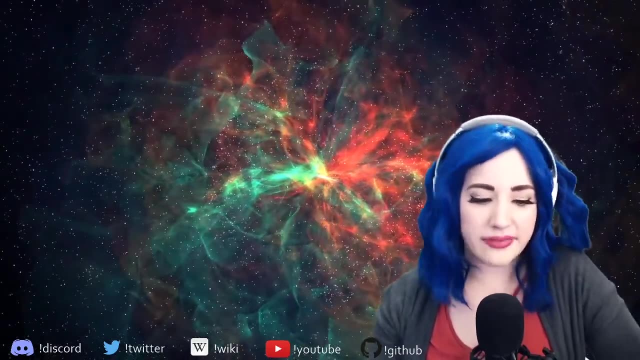 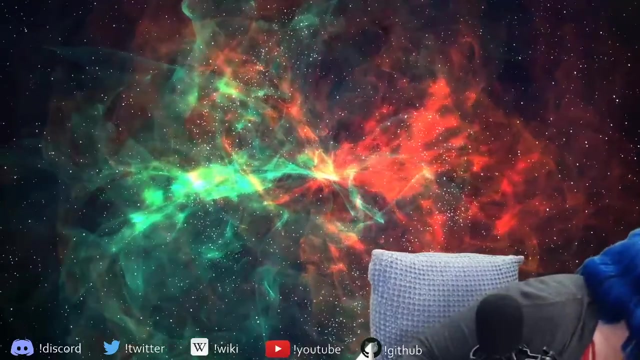 um, so, pale oracle, you say i've. so you have math, astrophysics, programming, a few languages under your belt. what other things do you actively study? um, so, speaking of the data structures and algorithms, oh, hold on, this is gonna move my. okay, i'm looking through my pile of textbooks here. 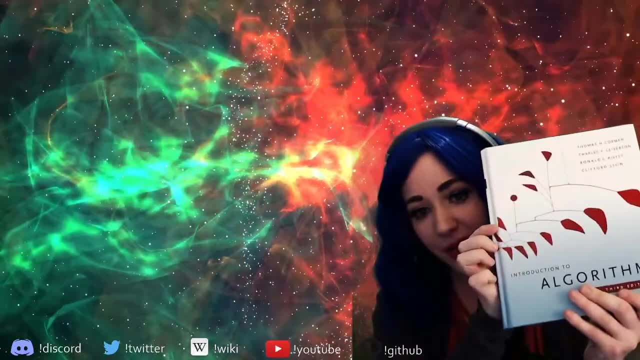 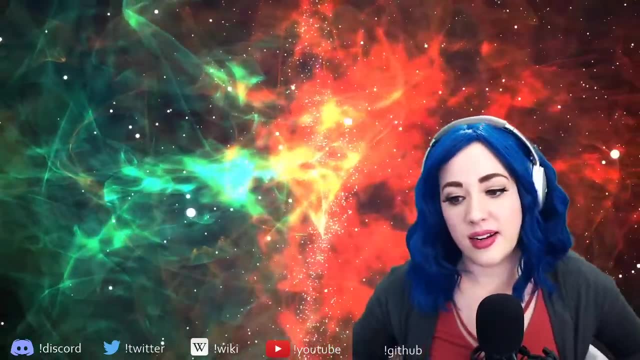 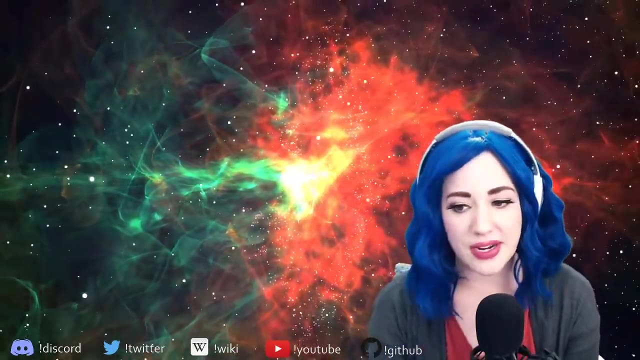 this bad boy is something i'm actively reviewing, mostly because i'm like kind of doing the job search game, so, uh, that comes up a lot in in interviews. um, i'm also actively learning more about reinforcement learning and about the statistical underpinnings for machine learning. 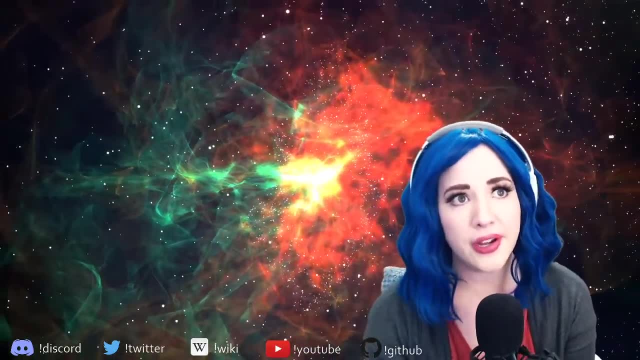 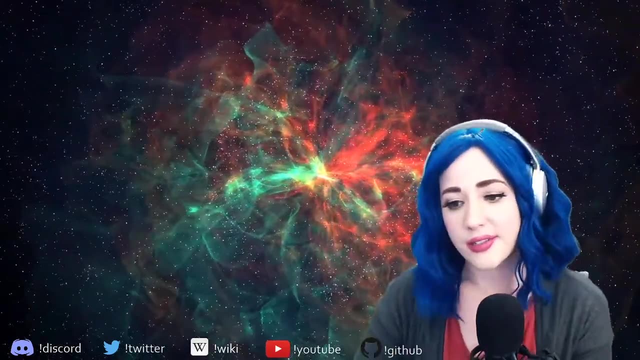 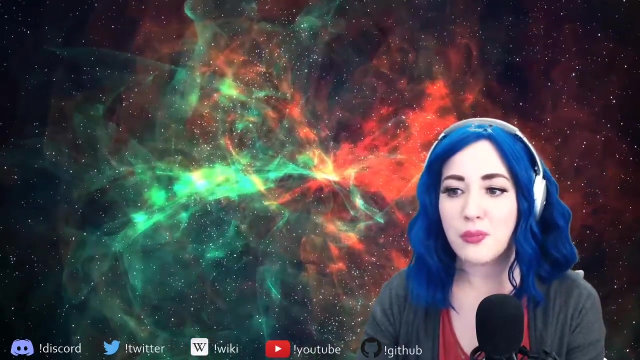 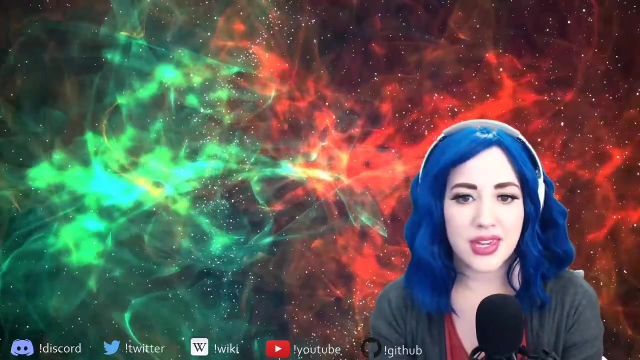 as well as like software development as a whole. so i'm trying to learn better software development best practices, um, because that is that is something that, like, i'm not formally trained in, so always trying to be better, uh, let's see. what would the book be about? third tier gaming, um. so i talked to my mom about this, actually, but we were thinking about 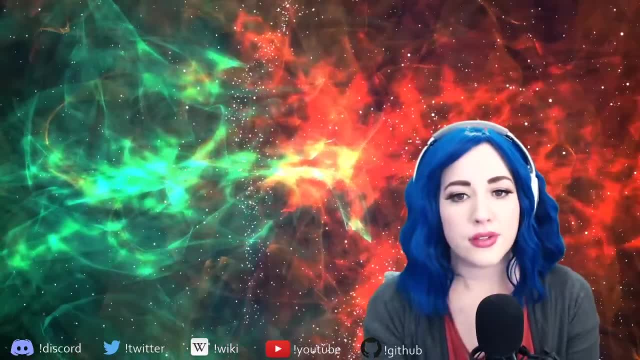 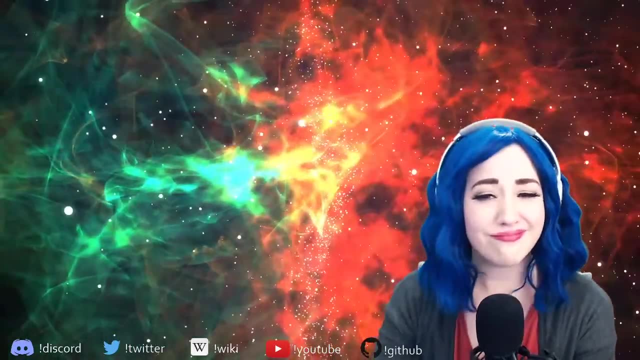 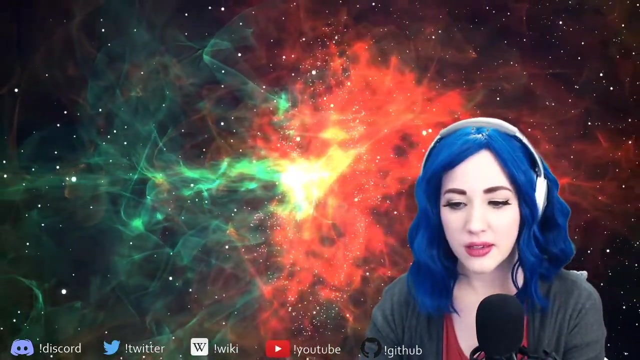 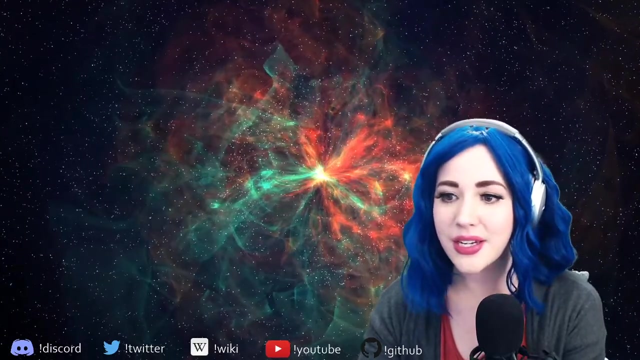 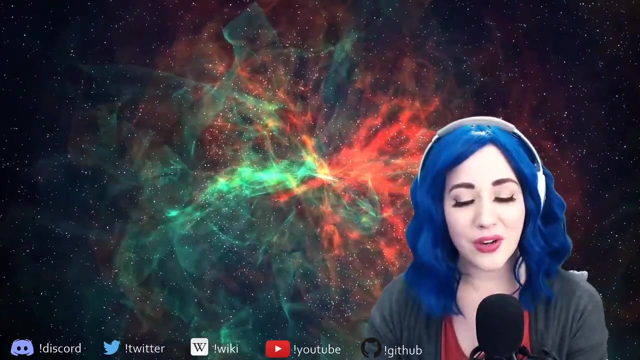 writing a book together on teaching math. so, um, yeah, i'm like, i don't know, demystifying math, making math less scary, stuff like that. you lost me. um, my mic still shows. i'm here, hopefully. hopefully it isn't broken. um, let's see. oh hi, lofbone, welcome. everyone's been behaving great. there was just the one. 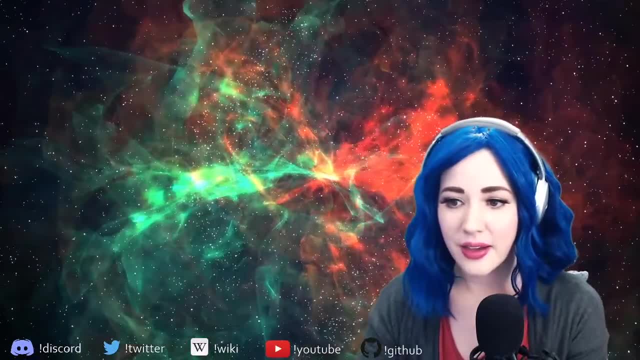 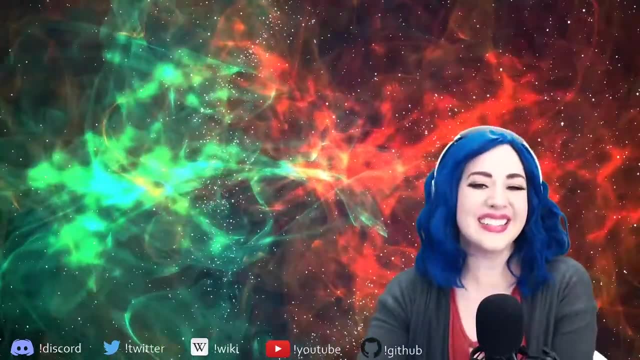 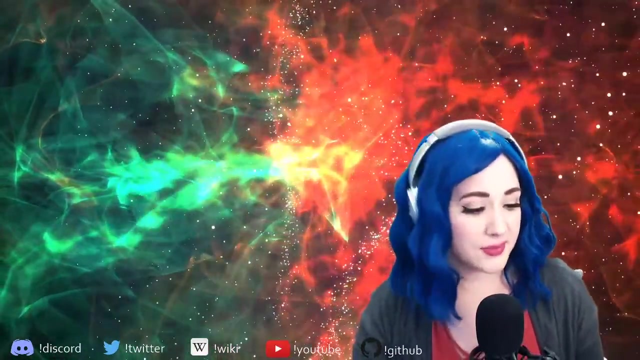 person you banned, but otherwise everyone's been been lovely. um, and let's see that that book is currently holding up my bed. though it's, it's a chunk, and i'm i'm telling you this like i can see why it is like an excellent reference. is it taught the greatest? no, 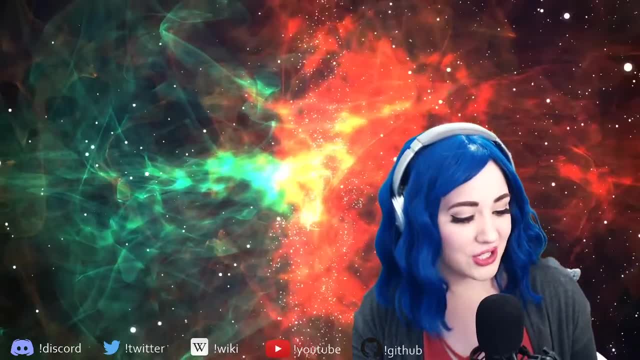 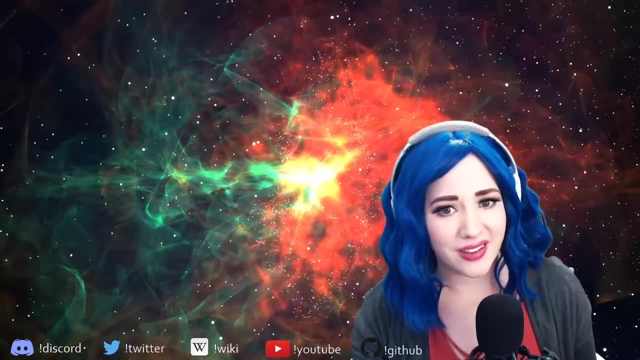 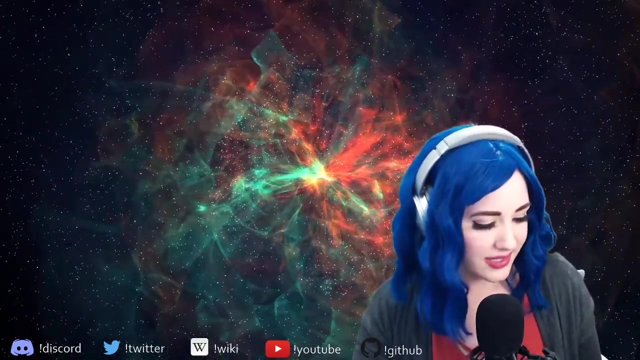 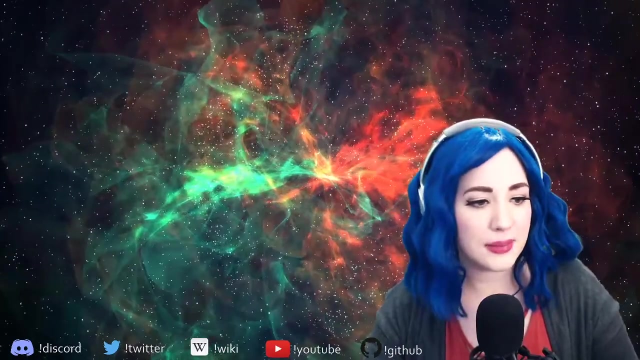 it's, it's dense as hell and i'm not sure that everybody needs to know like the proof for why. uh, like linear probing, open addressing whatever. like not everyone needs to know that. and king, it's a corman, it's clrs is, is people abbreviate, but it's corman, lyserson, rivest and stein um. 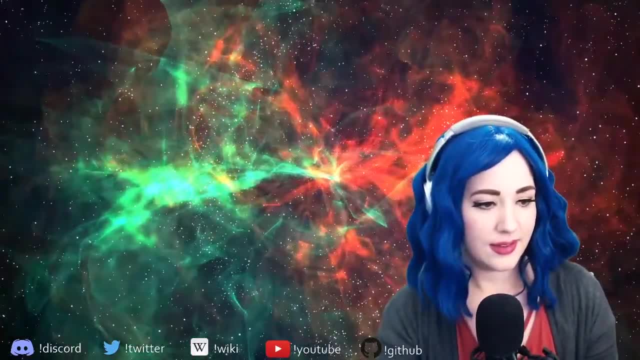 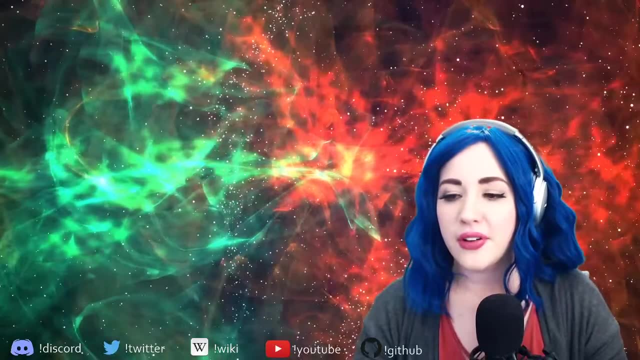 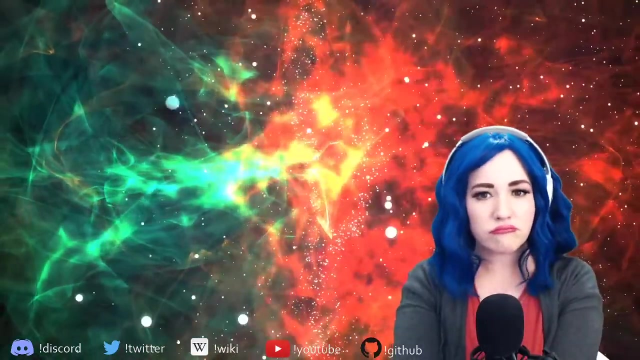 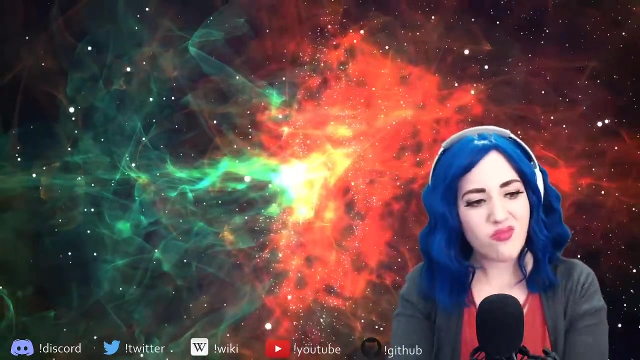 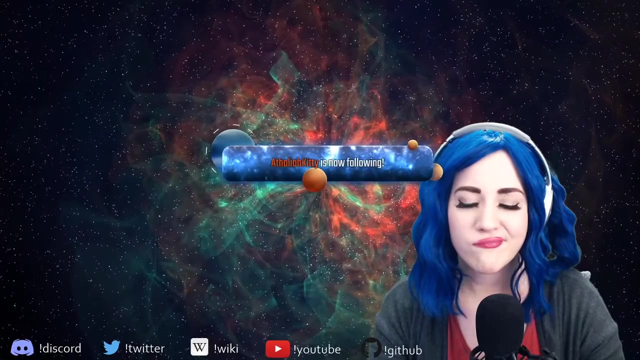 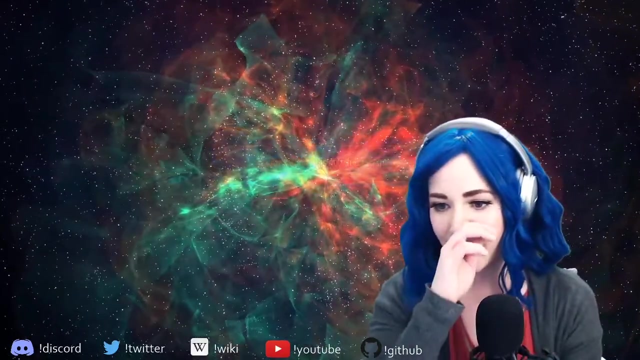 okay, let's see. has any programming language you felt you've learned, felt like it had too much boilerplate code? if so, what programming? i'm not, maybe not really um, um, um, yeah, i don't think so, at least not yet. a thal, a thalia kitty. thank you for following um. 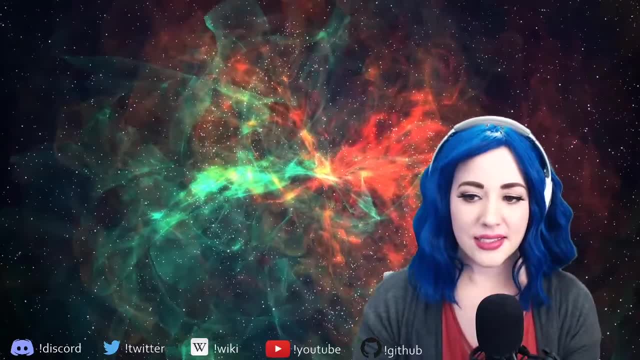 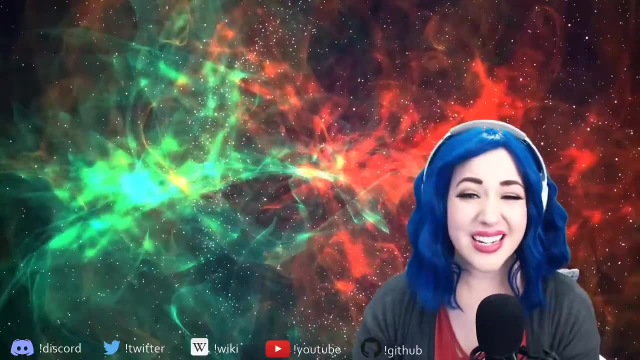 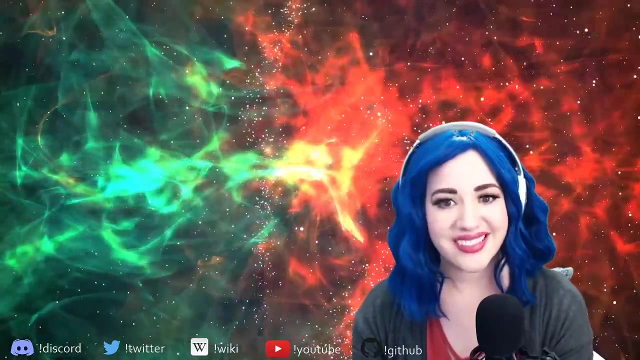 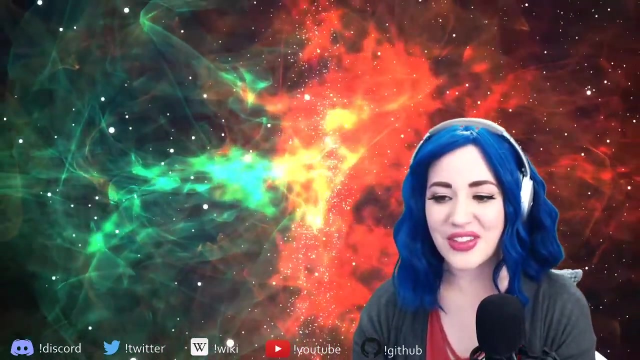 yeah, please, uh, please, please, uh. post a bunch of links on discord. strawberry jesus, i love recommendations for new, for new books. um, i've got an entire great, wonderful textbook on bayesian statistics that i need to go through, but i've been lazy. um, um and arrhythmia, you say. i think if you've studied computer science in the us, you for sure have that. 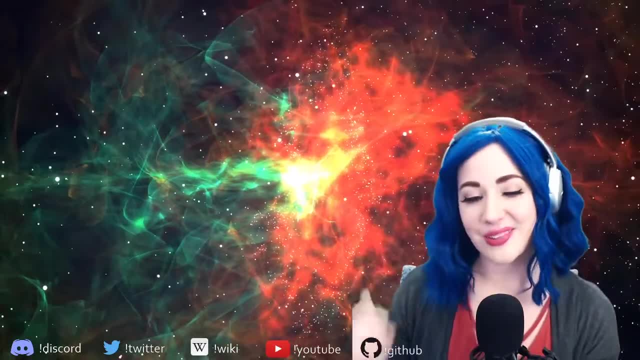 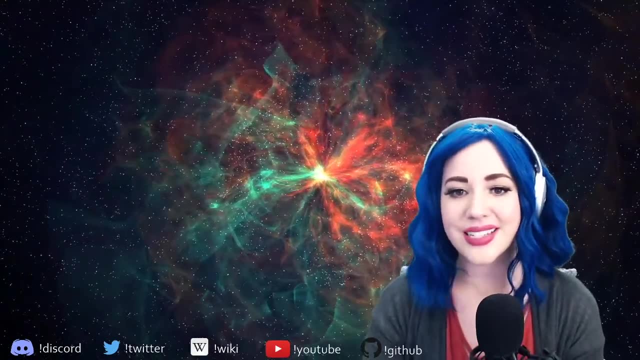 book. um, i i haven't studied computer science in the united states, so i just i i'm taking an online class right now and this is the book they recommended, so it's, it's a chonk, though it's a bit of a struggle. um, and professor sauce cat, you ask how did i find the north african dialects? well, 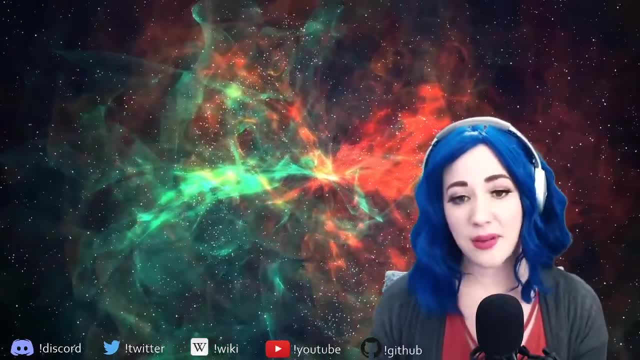 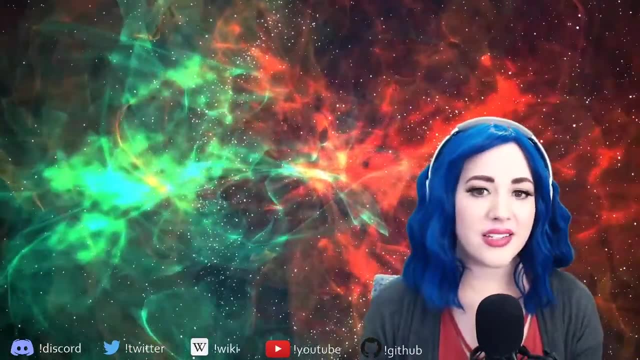 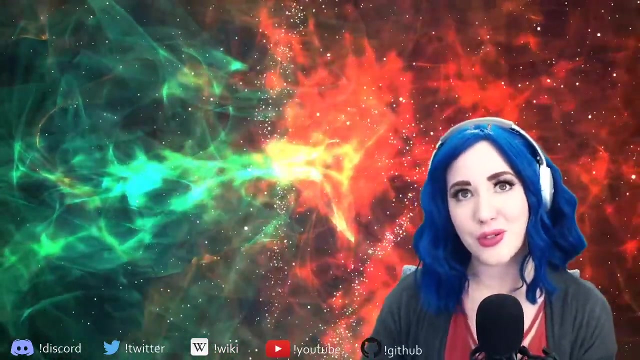 interesting, funny story friend. so i was learning arabic. um the sort of thing that i was learning is sort of mid 2000s and um i was getting a lot of pressure to apply my arabic fluency to government and or military service, which i was ethically opposed to. both of those, um i wanted to be a translator. 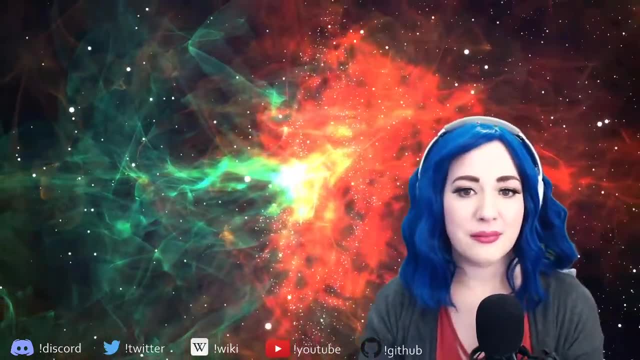 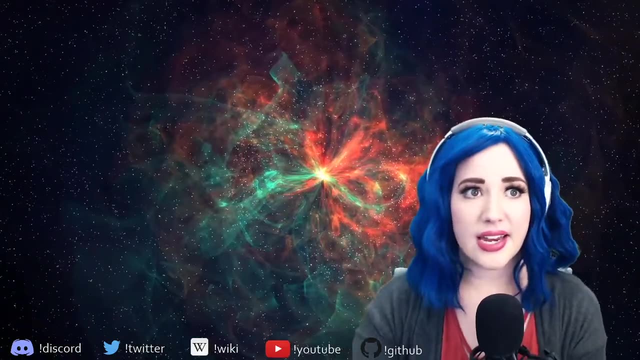 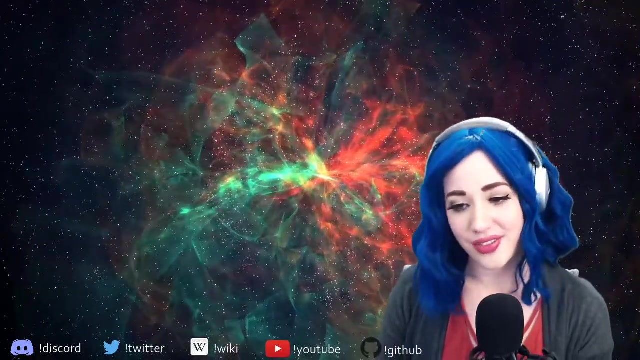 like a literature translator and, um, i was looking at different dialects to kind of focus on, and it was twofold. the rational reason is that at the time, uh, like i thought you know, nobody was interested in tunisia at the time. like it was, it was not it. 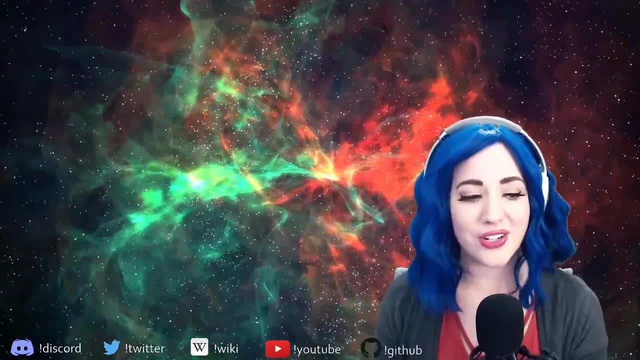 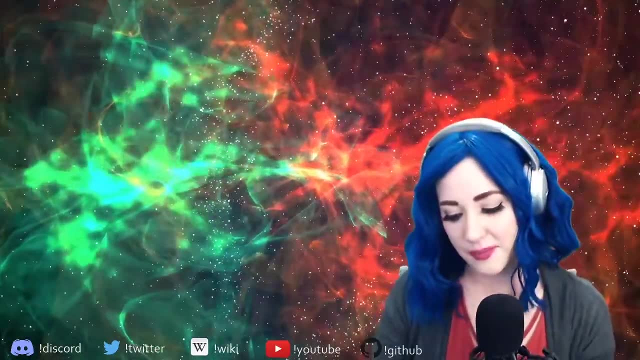 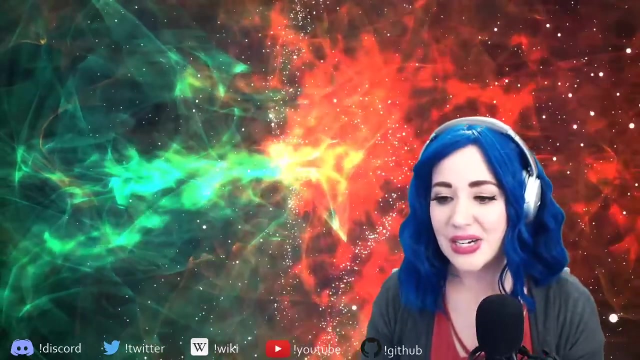 didn't have oil, like it wasn't, it wasn't like a politically charged country, um, and so i focused on tunisia, and then, of course, the arab spring happened. so, oops, um, also, i had a big crush on my professor, and he was from tunisia, if i'm being real, um, but also having having a professor who can. 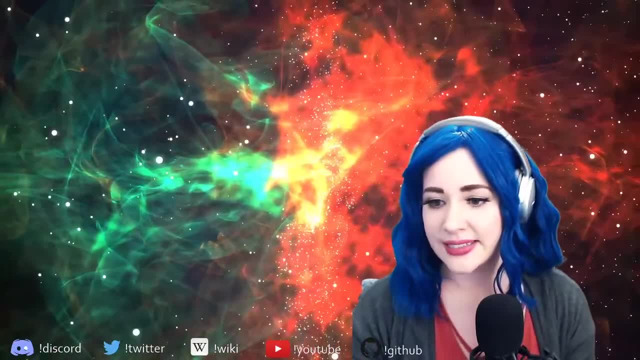 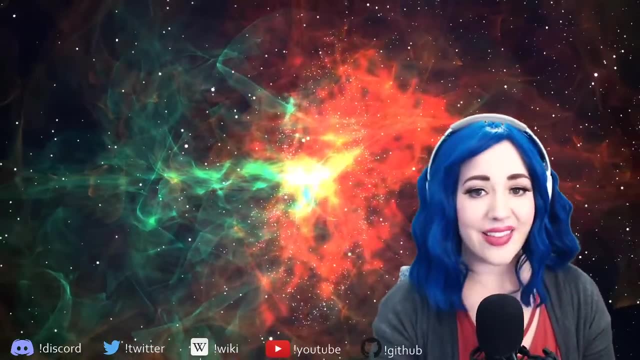 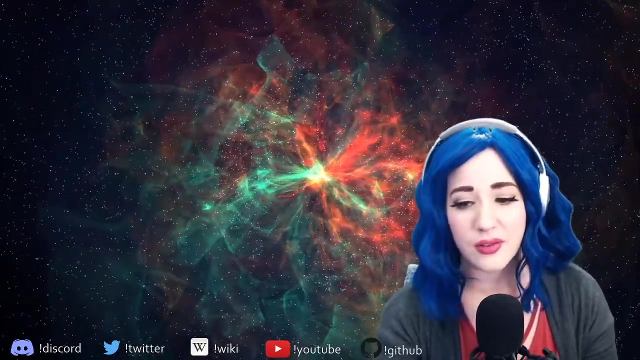 teach you. the dialect is important. nevertheless, um, diatoms attack. hi, let me give you a shout out. so if you are interested in scanning electron microscopy, um, loaf bone, can we get a ban for the person trying to make a butthole picture? thank you, um, let's give diatoms attack. i can. i think i. 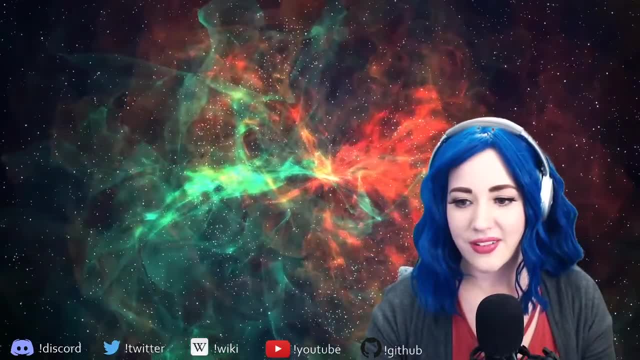 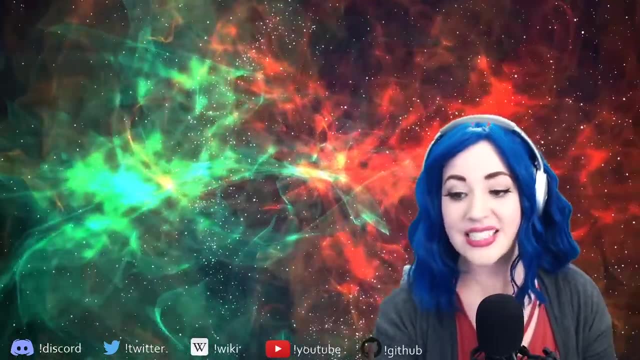 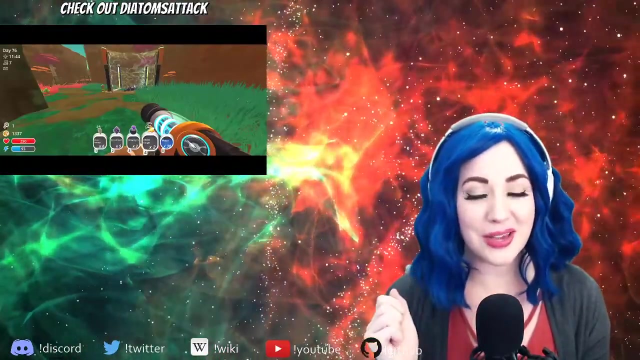 can get this. can you do it faster than loaf? i can ha beat loaf bone to it. um, um and uh. let's give. let's give diatoms attack a shout out, because if you're interested in scanning electron microscopy or i guess also video games, um, you should check out his channel. he looks for. 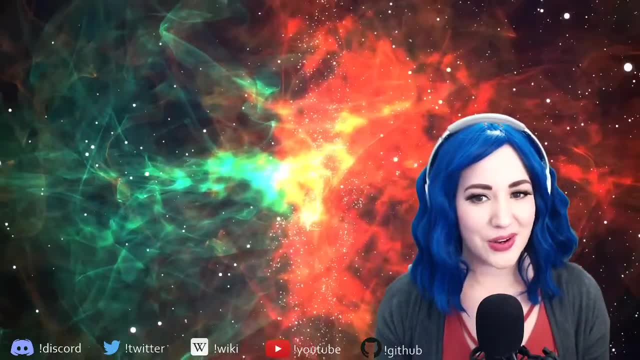 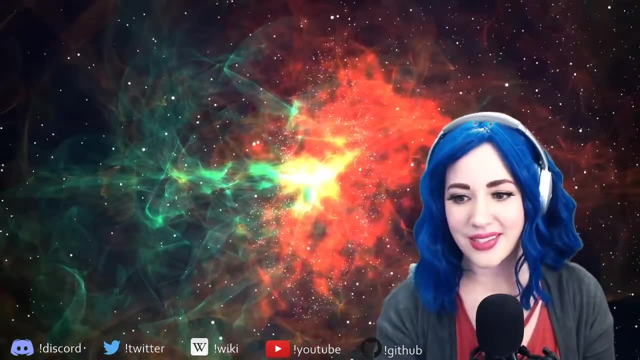 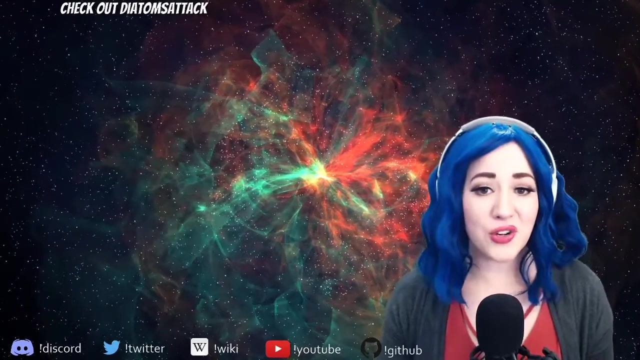 diatoms which are like oh crap, like oh, no algae. no, they're not algae, they're like little like like plants. right, and what happened? okay, that was that was like the shittiest shout out. let me try this again. i was right, okay, and they're cool and they have like beautiful symmetry and also it's a freaking. 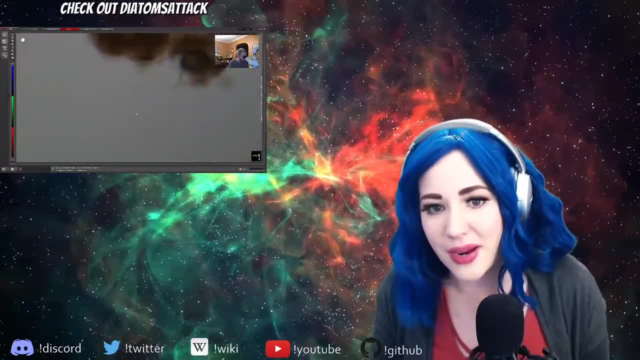 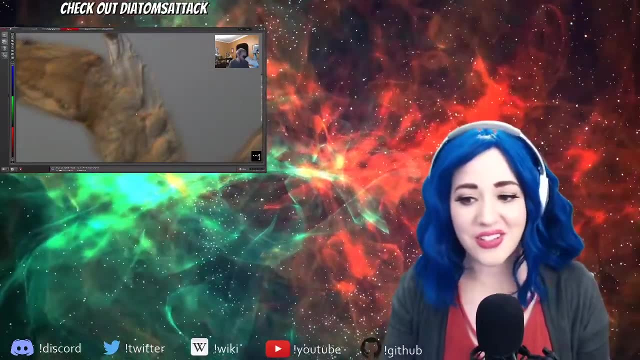 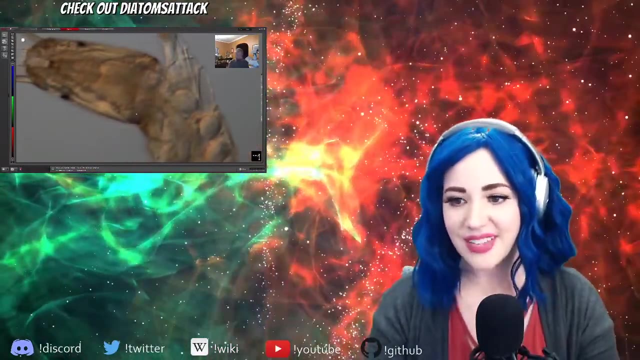 microscope like we. who gets to look at an electron microscope on a regular basis? not me. so really, really cool stream lots of stuff to learn. beautiful, beautiful, beautiful images. so give a follow. spread the science love. no worries, loaf bone i, i took care of it. never seen an ascii butthole before. 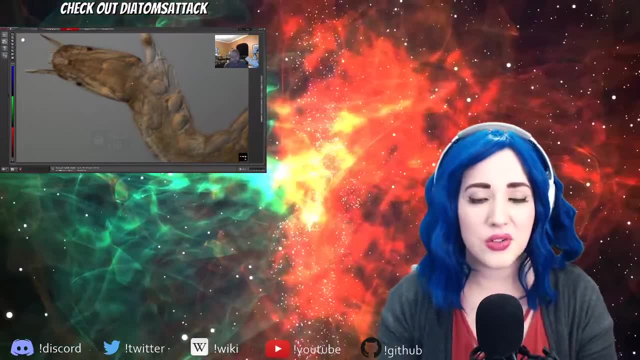 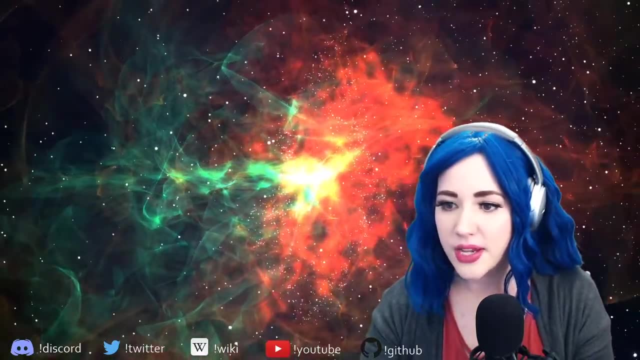 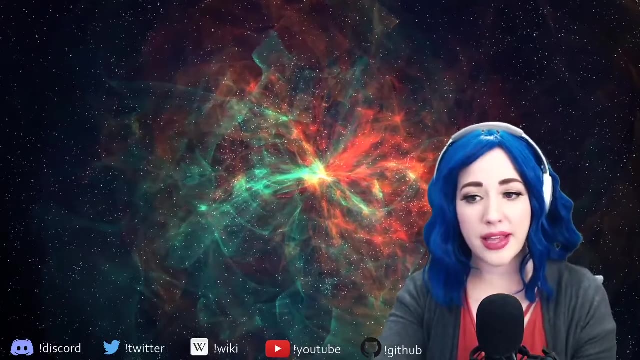 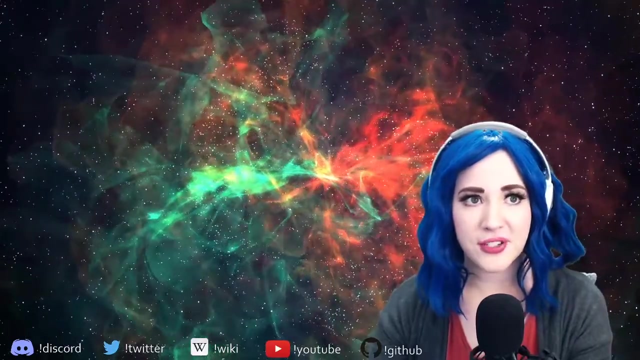 so that was a learning experience, but thank you to the uh troll for that, um. but let's see here, um, still catching up on some of the questions. i did not give up on learning arabic collided scope, so i was fluent for a while, um, but after, after the arab spring and after, just like lots of pressure to join the military. 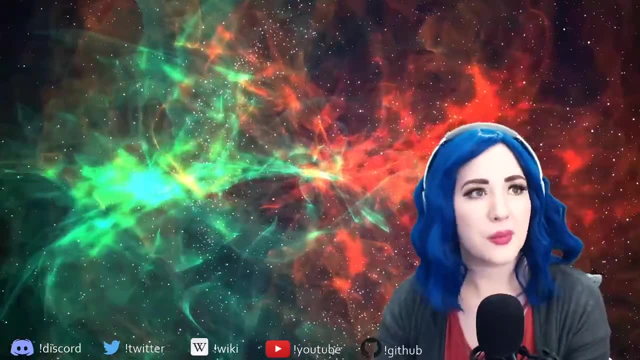 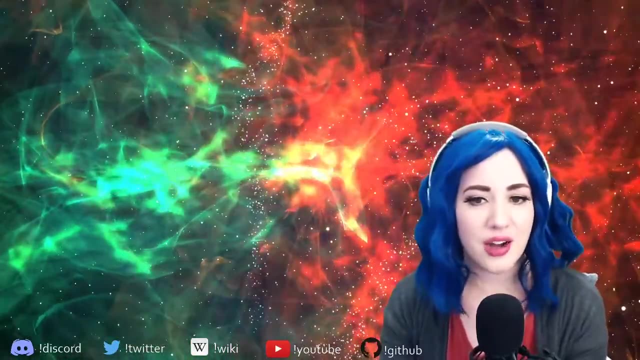 and some drama happened at my university with our arabic department, where a vast majority of the arabic professors quit in the space of like a month. like i actually had an arabic professor, like walk out on class and just never come back. um, i have no idea what the drama was, but it meant that, like i 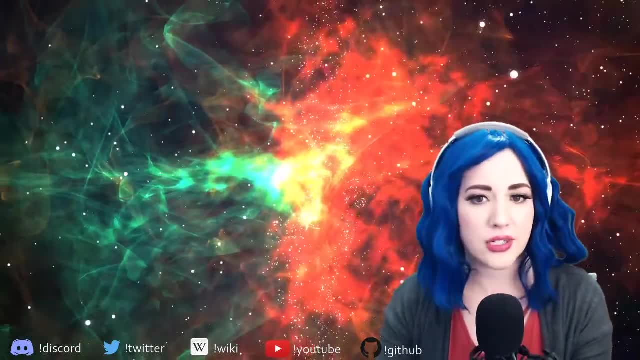 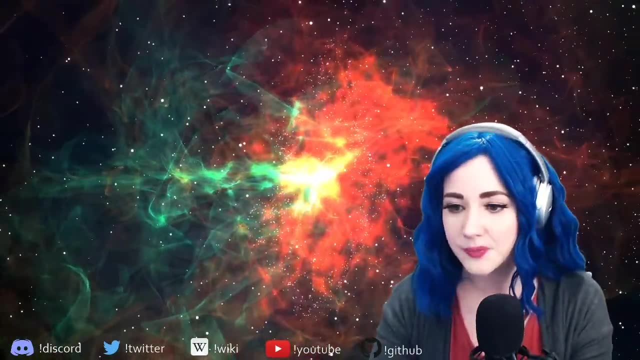 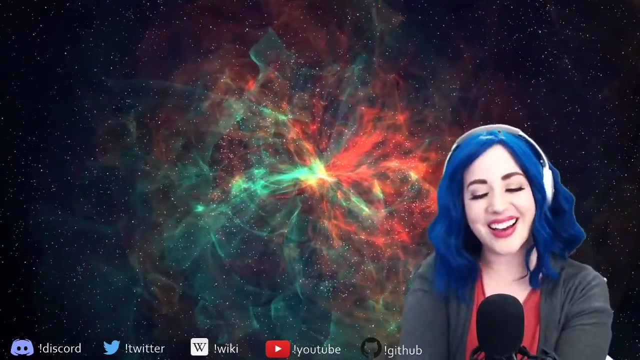 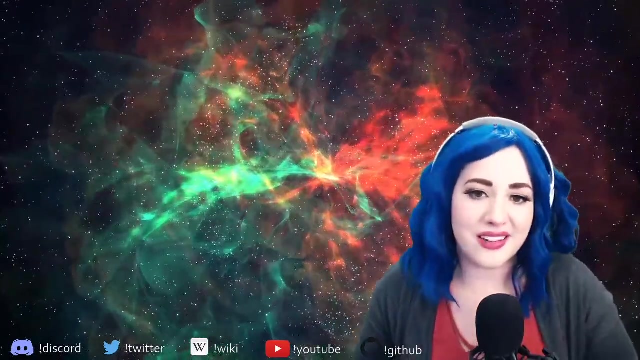 lost all of the support and mentoring that i needed for getting into grad school. so, alas, i miss it, though i love it. it's to me the most beautiful language i've ever studied. so, um, nevertheless, ah, that was seven. uh, yeah, hi, welcome, welcome, um. say something in arabic. um, oh gosh, you say that. and then i'm sitting here like what do i say? i don't know. um isn't tunisia one of the more stable countries right now? yes, so, especially in terms of looking more broadly at the arab spring, um, uh, tunisia by far is is one of the most stable. i can say like: 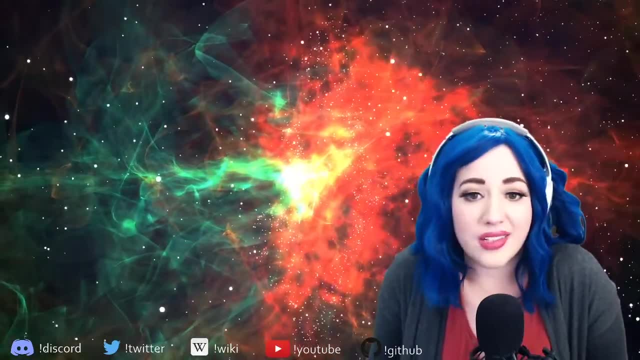 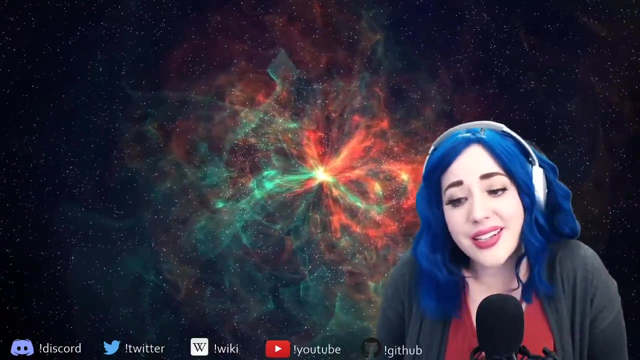 kefa halleck, which is like: how are you? so there you go. it's been a while. it's been a a long time since I studied Arabic Um, and Professor Soskat is absolutely right: The Arabic taught is modern standard and isn't used on a daily basis, So that's part of the 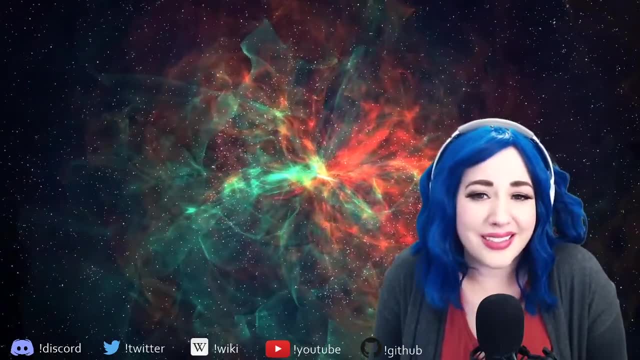 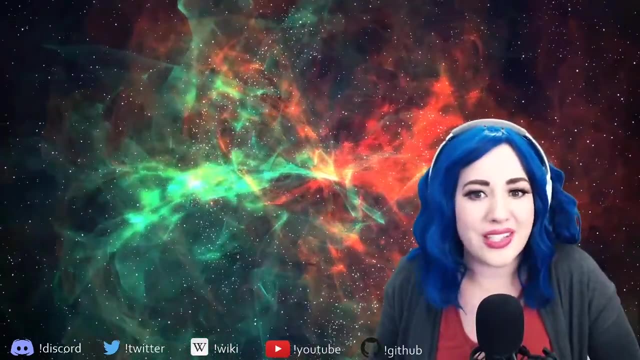 difficulty. Yeah, Also, when you think about it, that the Amiya are, like it differs so greatly from modern standard, right? So, like, sometimes it's like you have to learn a second language. So, in any case, how different would it feel to think in Arabic? Um, when I was? 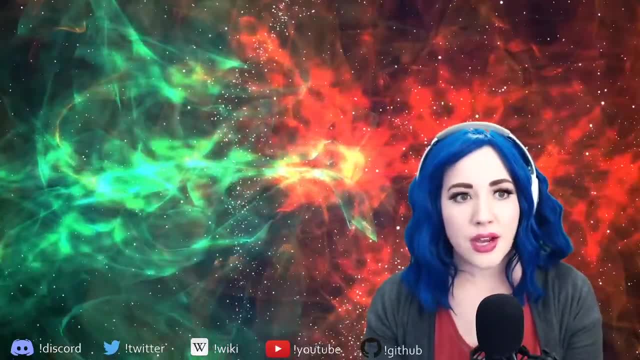 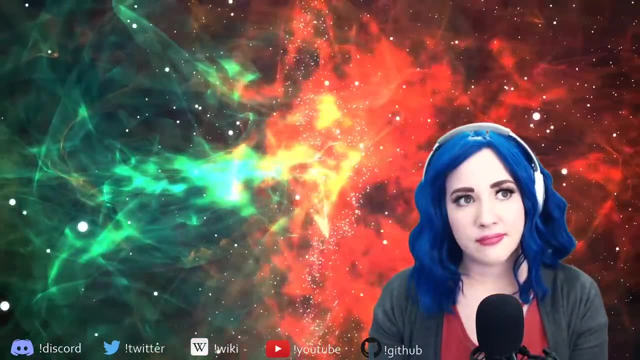 in Tunisia and I was speaking it daily. I I started to dream in Arabic and I started to think a little bit. So that was a really cool feeling. Um, I would, I would say that like it never got like where I was thinking only in Arabic, but there were a few times. 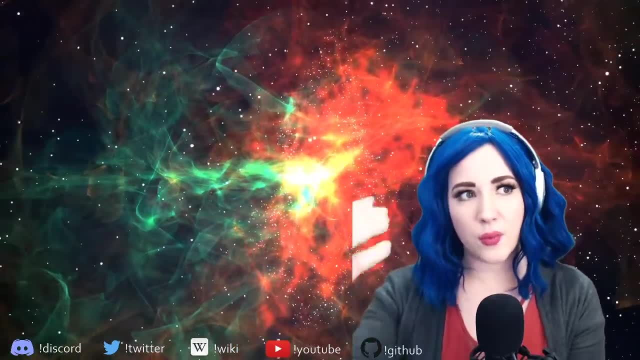 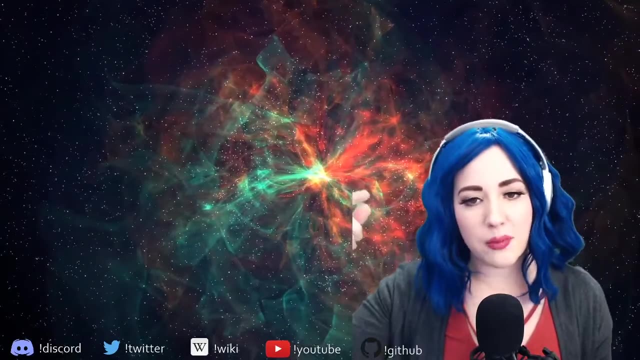 where I was speaking and having conversations where they're like, cause I feel like when you're first learning a language, the English pops in your head first, then you translate, then you speak, And so there was a time where I was proficient enough where the English 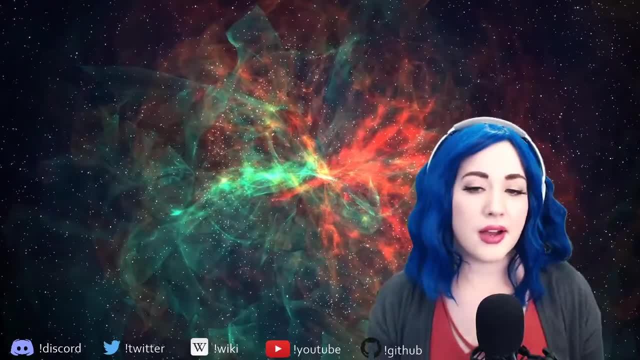 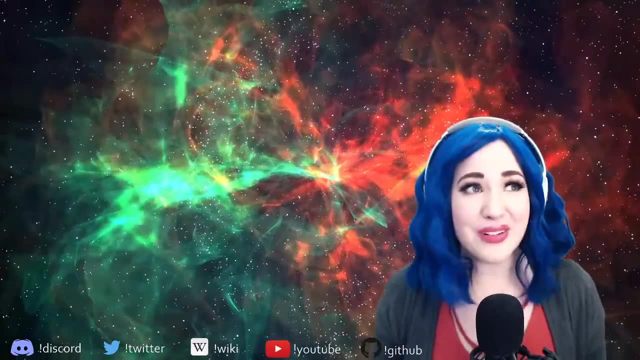 didn't pop into my head. first, The Arabic did, which was really really nice, Um, but it never got to the point where that was like all the time, Um. then I came back to the U? S and didn't have an opportunity. 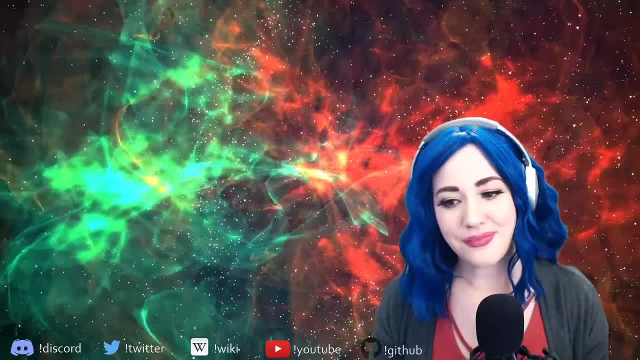 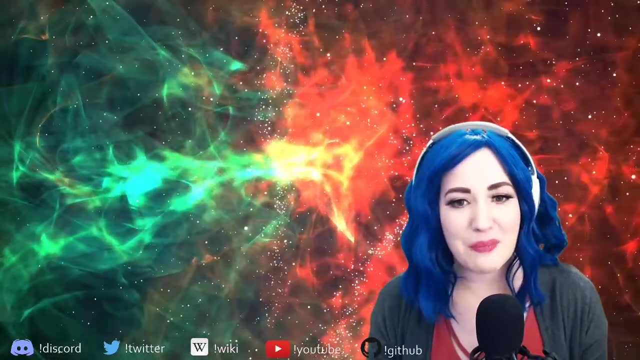 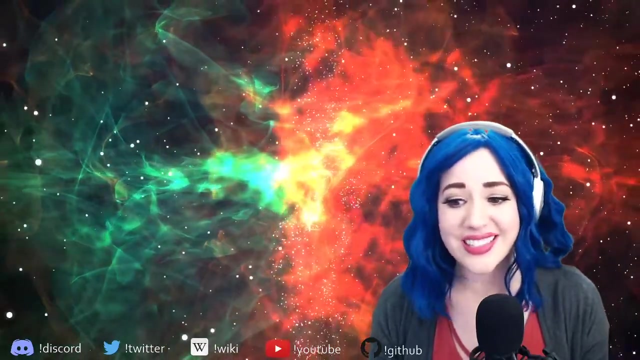 to speak it every day and lost my fluency. So I'm so out of practice, Like I have to sit here and like, like, remember the words and like actively. I'm not even sure if I remember like all my conjugations and stuff. 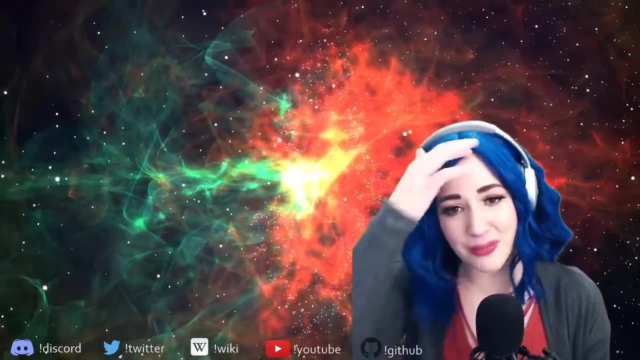 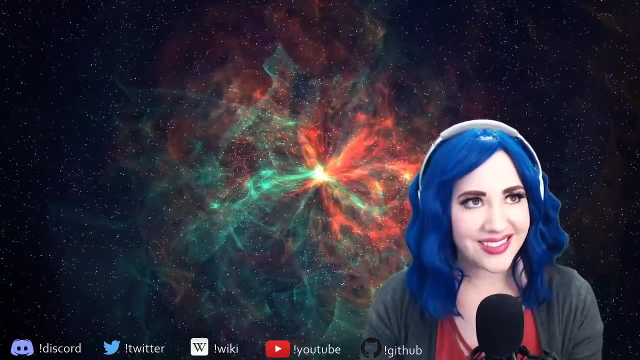 So I miss it. I miss it a lot, but also, I'm learning so many things right now that the thought of trying to learn Arabic again is as much as I want to, And my brain is like, yes, add something else to your plate. I also know that I wouldn't be able to give it the um. 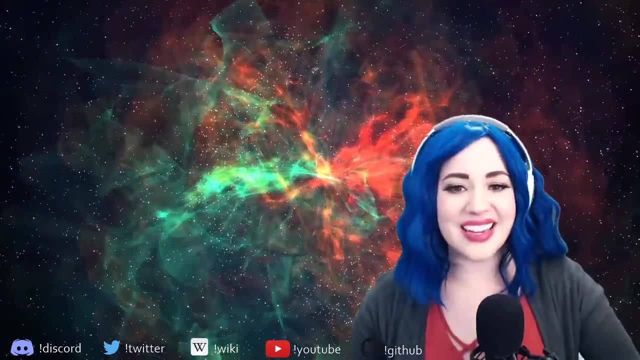 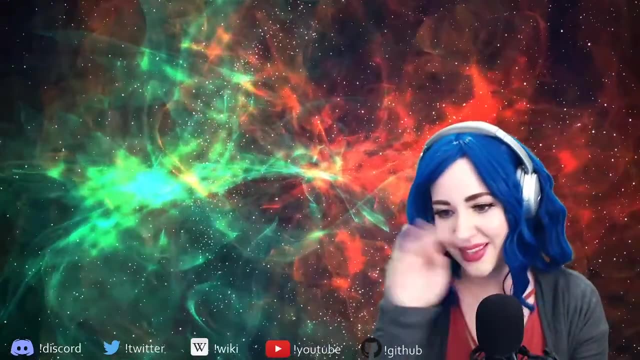 the time that it deserves. Can we practice Arabic again? All right, Maybe we should make an Arabic study group? Um, that would be, that would be amazing. And yes, And actually so it is. it is 11 my time. 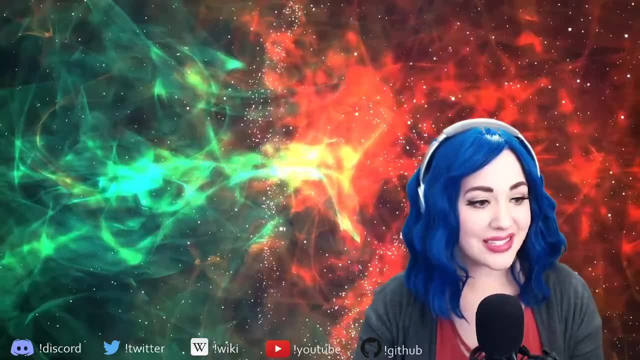 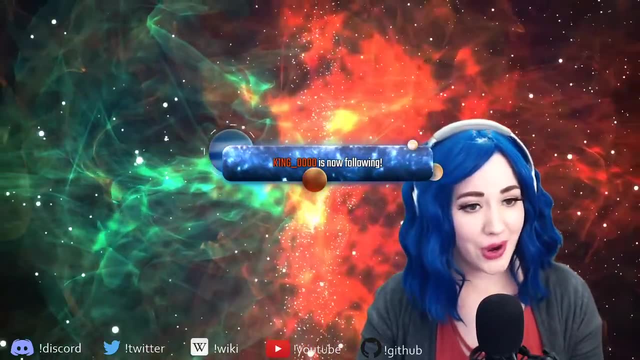 So I I think it's time for a Tennessee song, So let me set up. let me set up a poll really quick. So the polls are working for me again, So maybe we're lucky and they'll. and they'll work, King. zero, zero, zero, zero. Thank you so much for following. What should Tennessee? 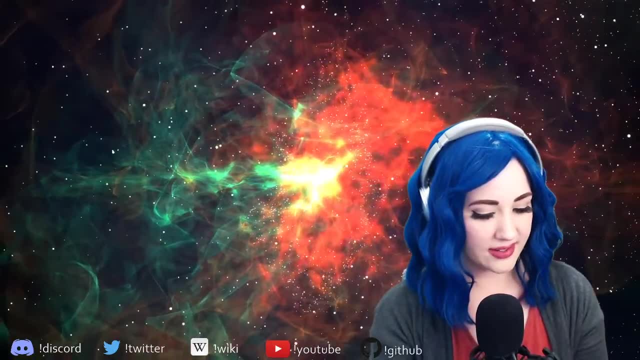 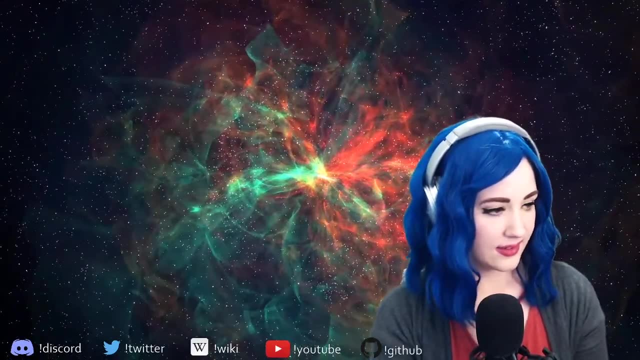 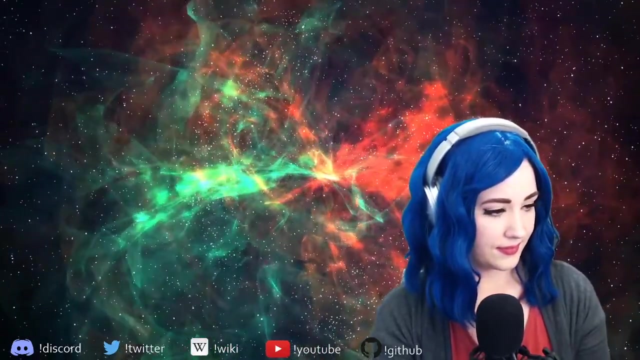 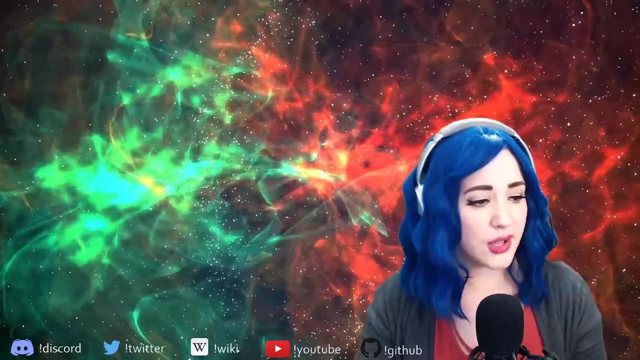 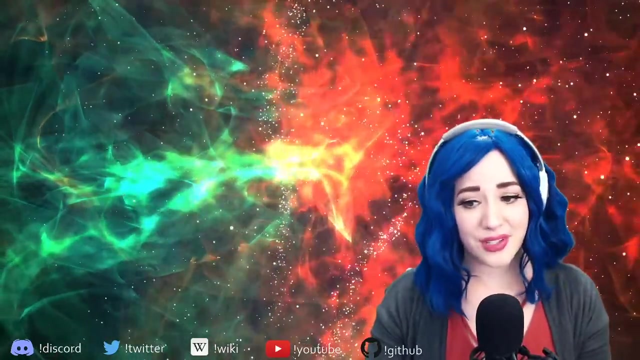 sing. And let's see, here We've got this. Will it work? Oh, hey, it worked All right, So I'm going to go get his divaness set up. Jay Shady, Tennessee, is my dog. So I have two dogs, Ten and Hubble. They're both. 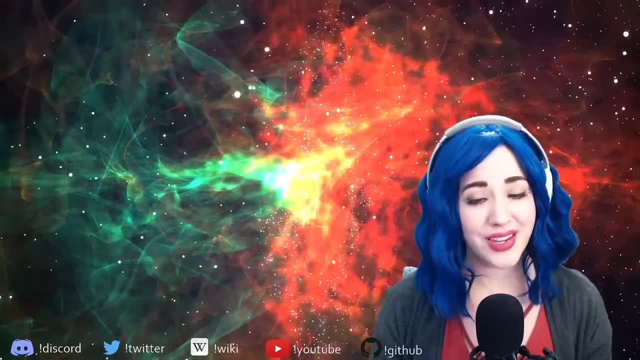 very good boys, Tennessee sings for you, And so I always love to do this once we've kind of finished our hard work of coding and learning the theory and math. And so I'm going to do this once we've kind of finished our hard work of coding and learning the theory and 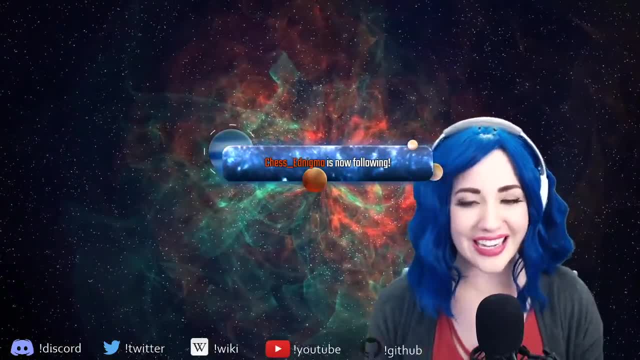 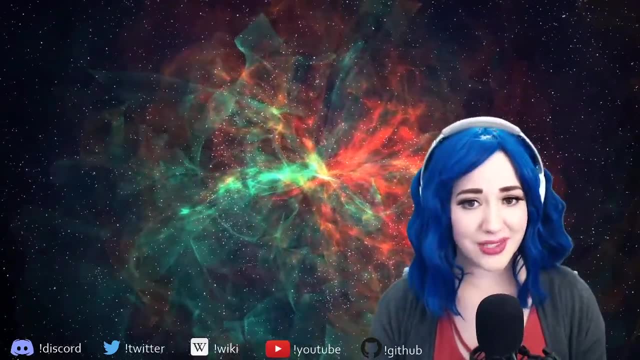 math, And so I'm going to do this. once we've kind of finished our hard work of coding and math And all of that goodness, I like to reward everyone for sticking through it with a song from a beautiful little dog who loves to sing to science fiction. TV show themes. 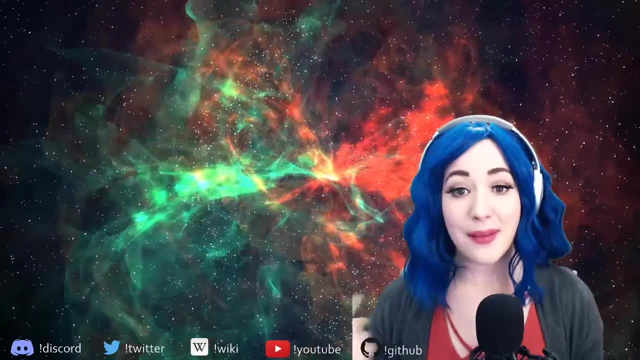 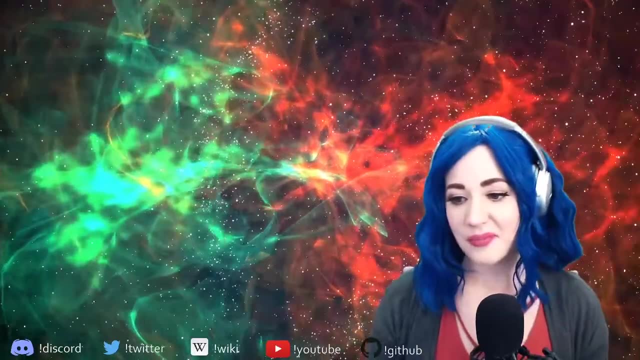 So, Chesednigma, thank you so much for following. I'm going to go get his, his royal highness, ready. He's a bit of a diva. I've got to prepare his treats, his throne, But while I'm doing, 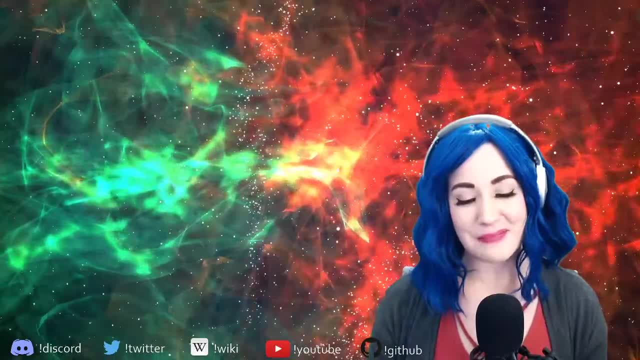 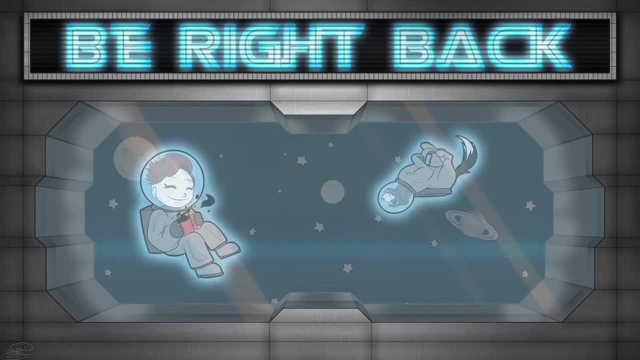 that vote away. Let me know what song you want him to sing, And I will- um, I'll be right back. Let me know what song you want him to sing, And I will- um, I'll be right back. 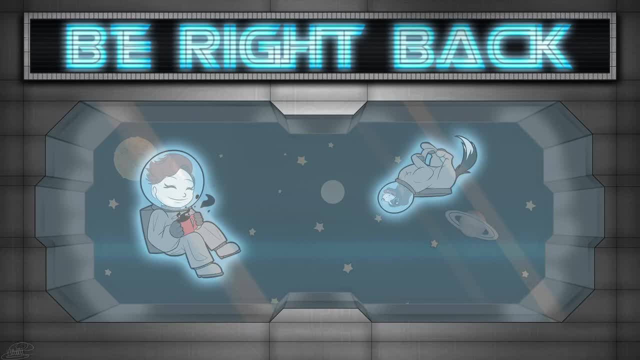 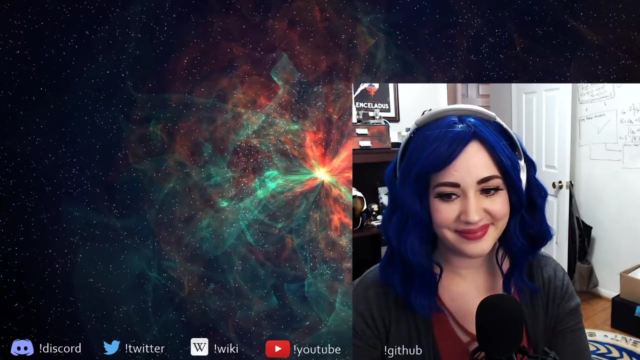 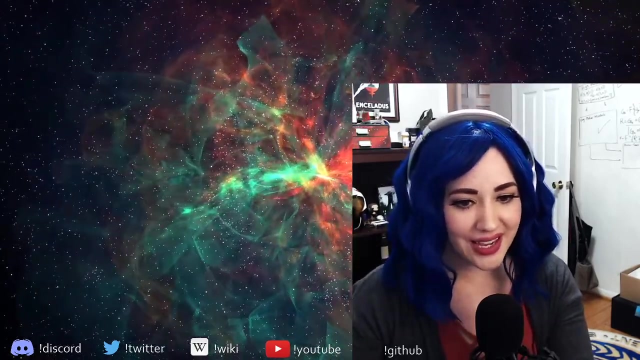 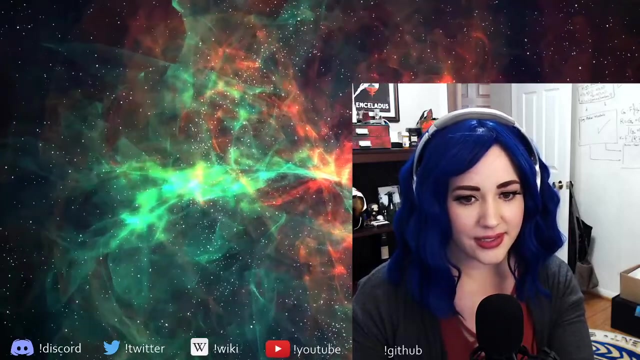 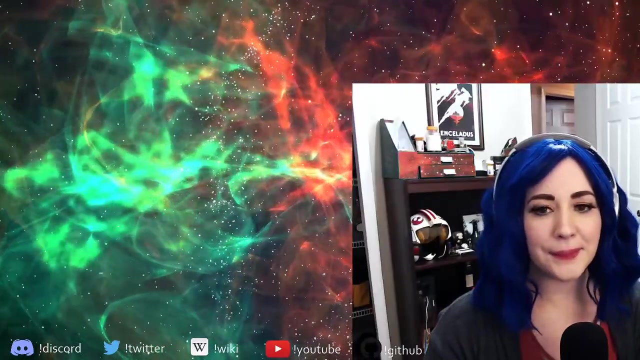 Let me know what song you want him to sing And I will. um, I'll be right back. All right, friends, Give me one sec here. I took down my green screen but I have to take the the cropping off of my webcam, So just give me one sec here. There we go, And 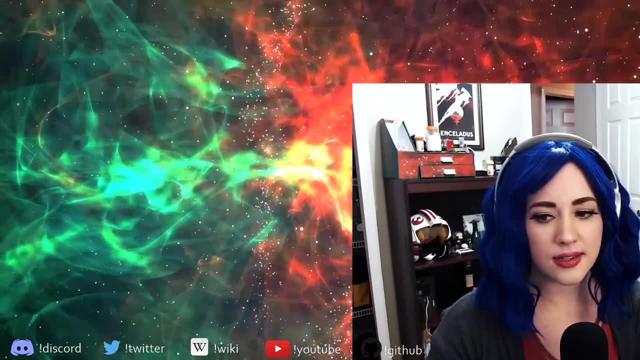 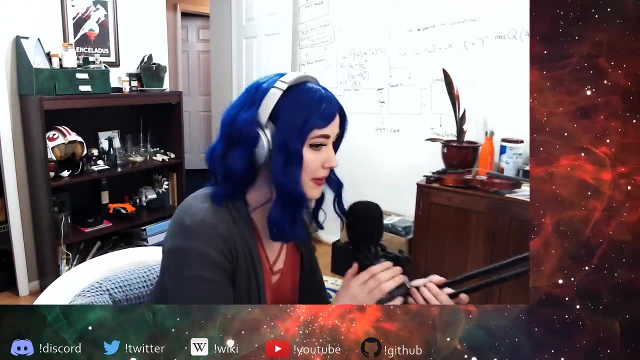 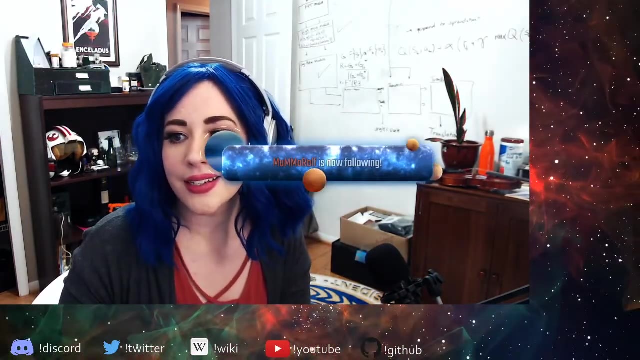 all right, I'm going to get a couple other things here set up. Let's see How is our poll going. Ooh, SG1.. Woohoo, All right, That's. that's my favorite, And Mama Rolf. 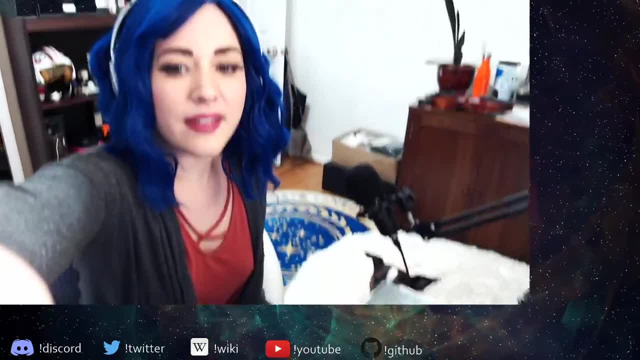 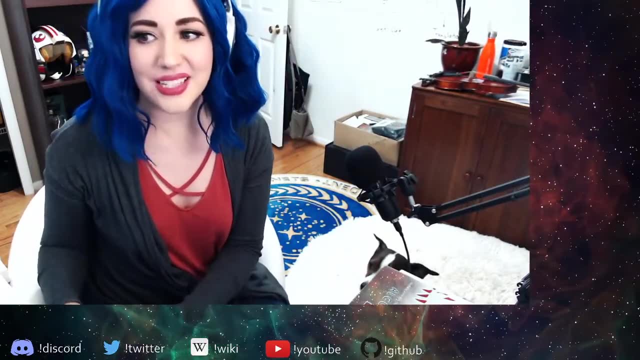 thank you so much for following All right. Look at his beauty. You can see that he's got a lot of hair. You can see his ears. I know it's going to be SG1. So I'm going to give it. I'll give. 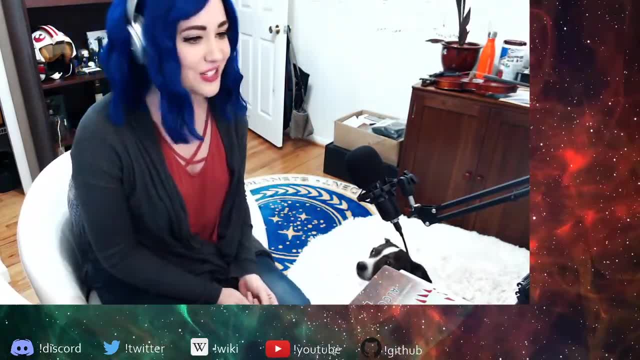 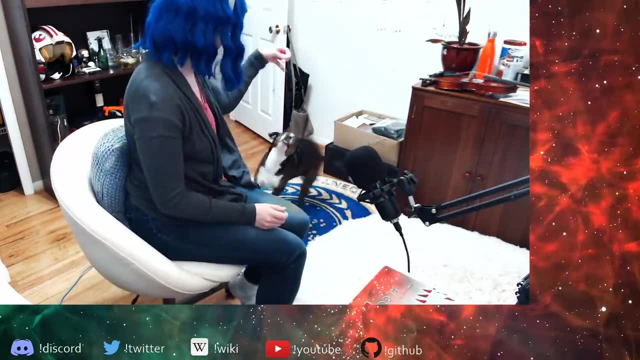 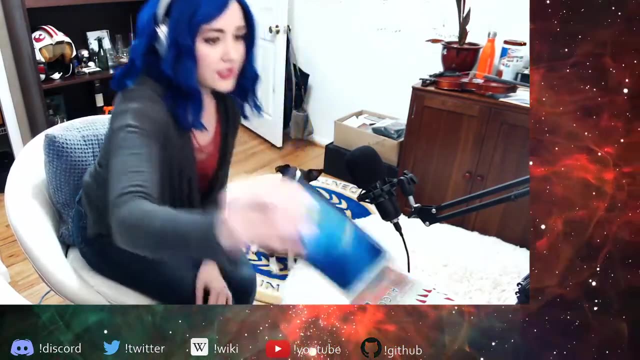 it like a couple more seconds And then I'm just going to call it and say it's SG1.. Volume warning, because he does get loud. Sit, Sit, Good boy. Can everyone see you? Okay, All right, Let's get your song. Let's get your song. I know You're a very good boy. Tennessee. 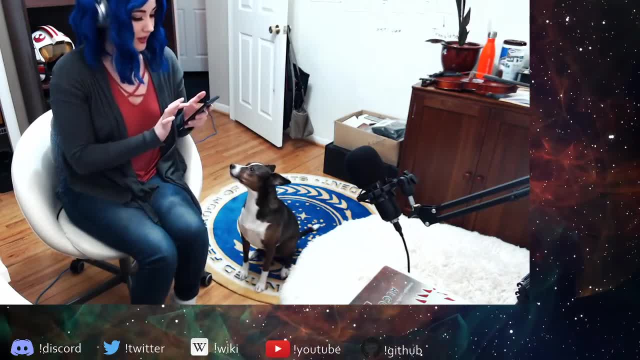 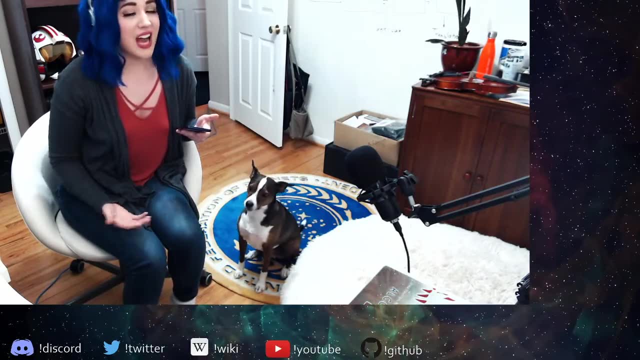 I know He's so excited- He loves singing for everybody. Like it's so sad because sometimes when I don't stream and I'm in my office, like I'll just leave my office, and he thinks I'm coming to get him to to to sing on stream. It's very cute. All right, I'm turning down the uh the. 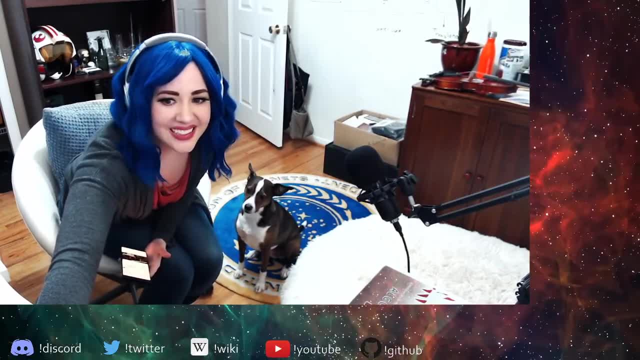 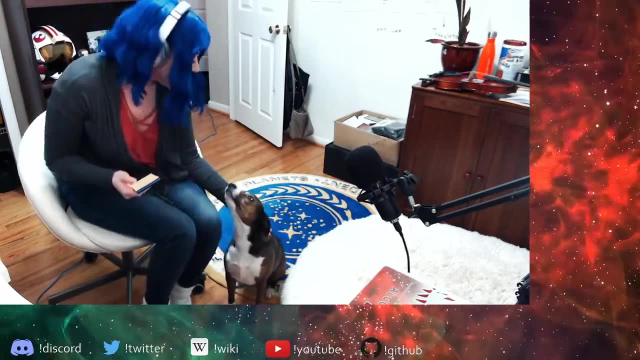 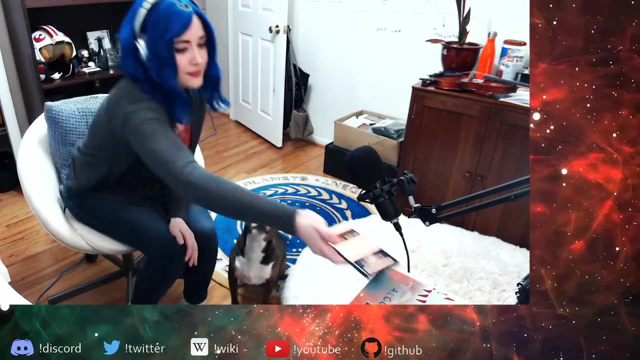 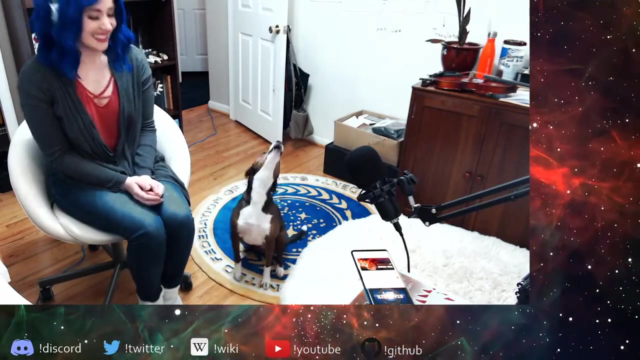 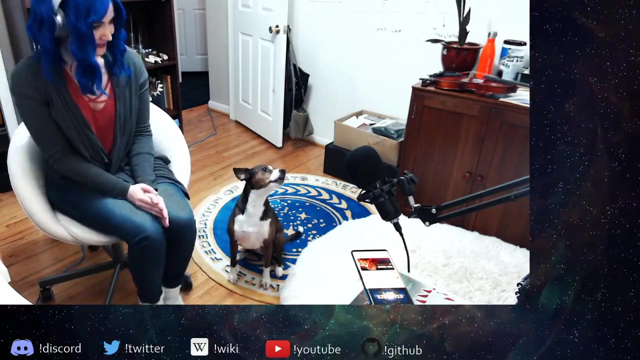 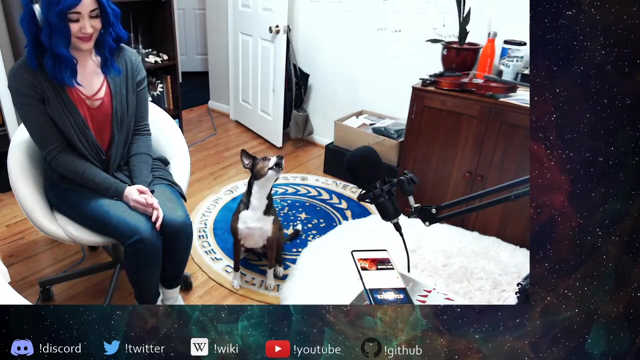 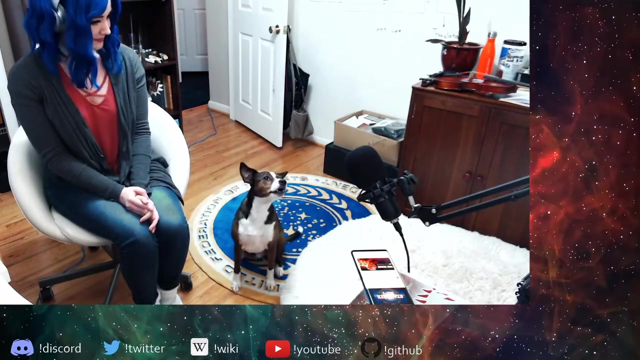 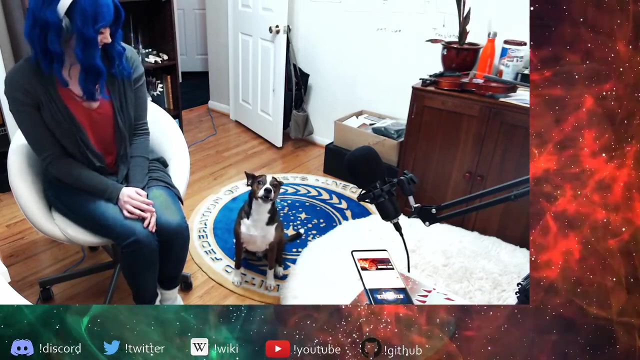 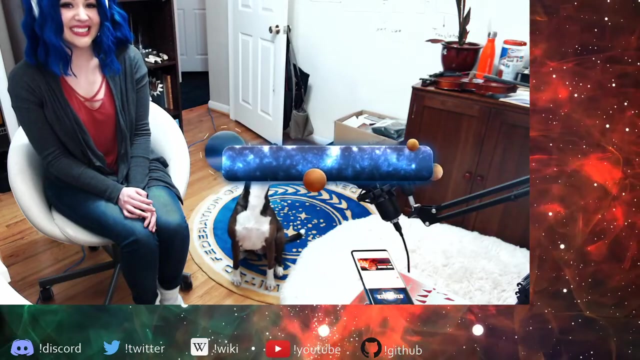 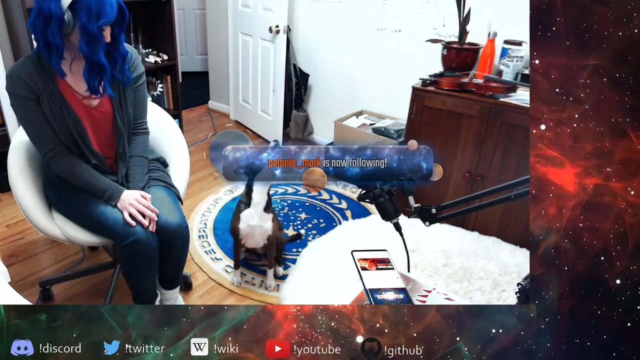 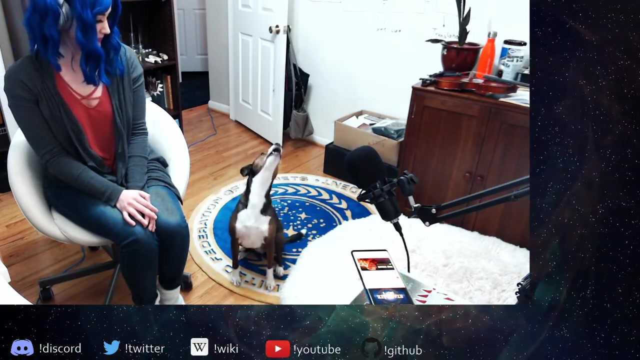 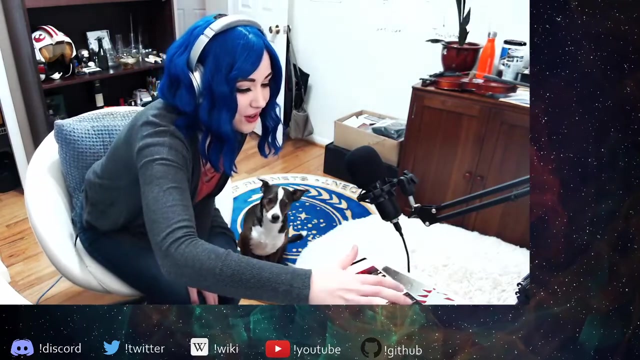 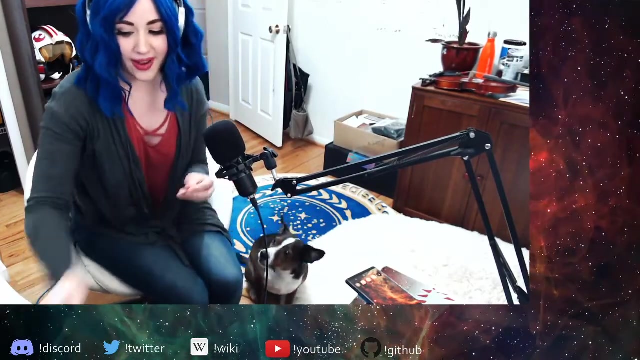 the mic. Hold on, Okay, I don't know. Oh, that was such a good song. That was such a good song. Oh, my goodness, Such a good boy. The bestest boy Is this cheese for you. 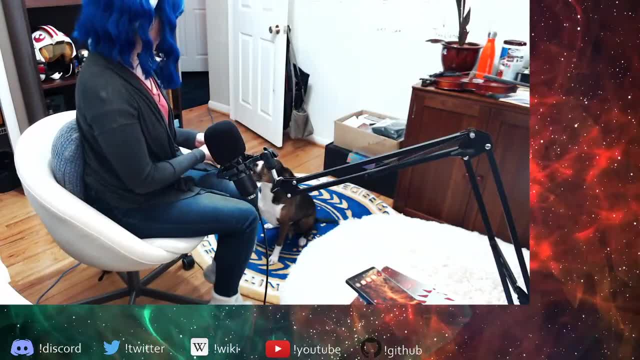 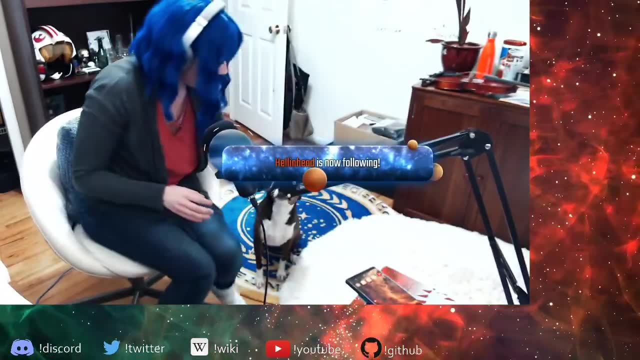 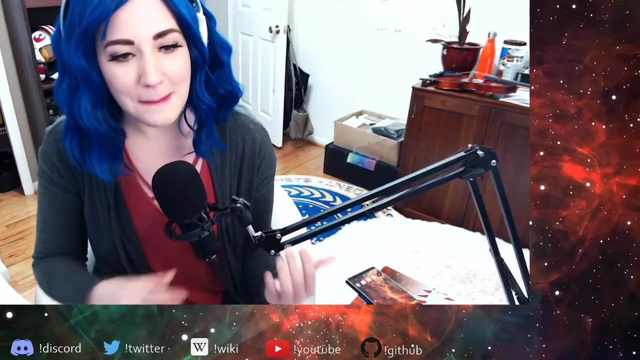 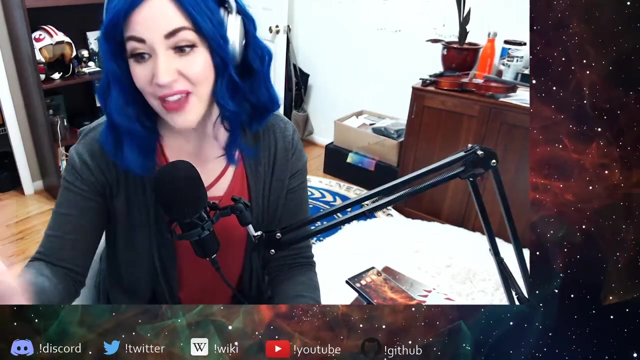 Tennessee said: Everyone on the street loves your songs, Fat, They love your songs. You did such a good job, Good singing And also excellent timing. to Palante, Mark and Helen Head for following You showed up right at the right time to catch a Tennessee song. 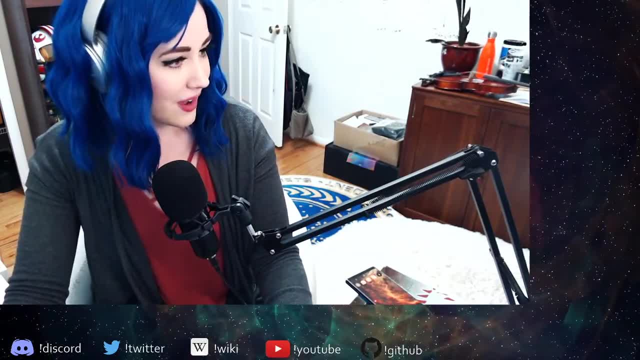 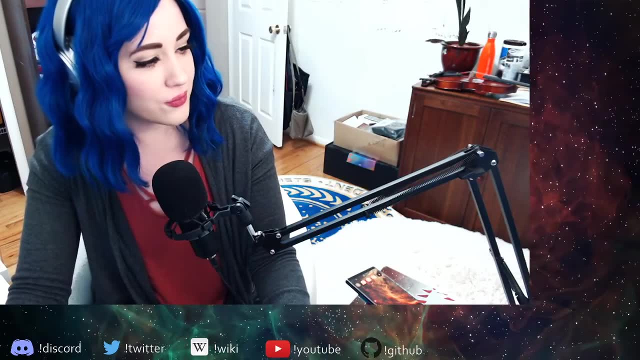 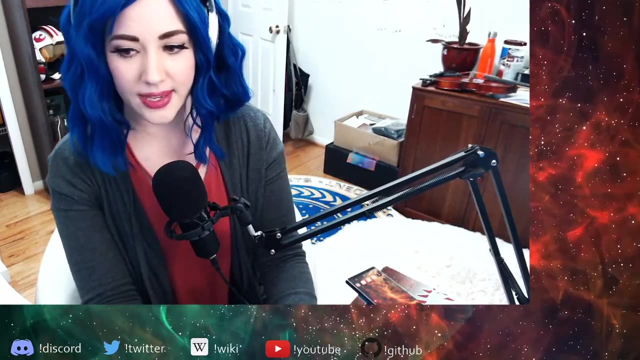 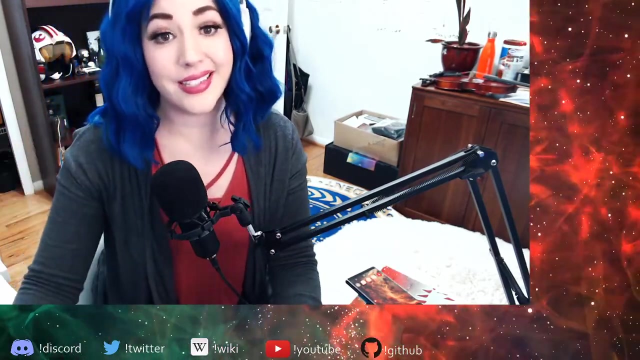 He's such a very, very, very good boy. All right, Let's see here Thinking about who we should raid. So many people are offline, Oh, I know. So if you have an interest in game dev, this is a good stream, just for you. 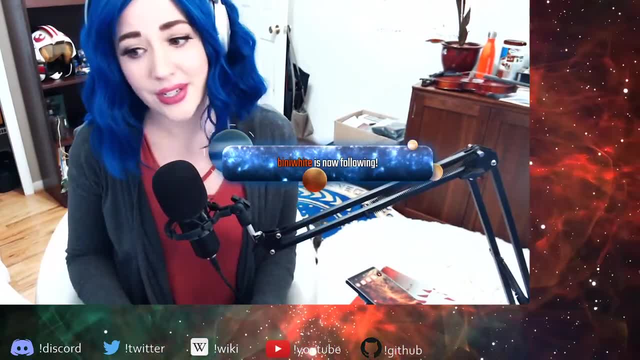 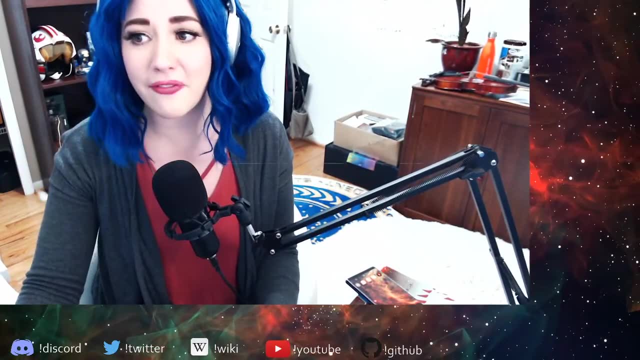 But also please come back tomorrow. We're doing Math Monday tomorrow. Game dev on Thursdays. Join the Discord. Check out YouTube if you feel like you missed something, But let's pass some of this love forward And, be nice, Send some love. 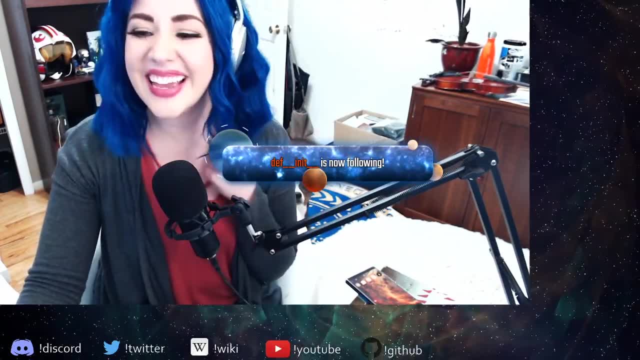 And I'll see you all tomorrow. All right, Good night.